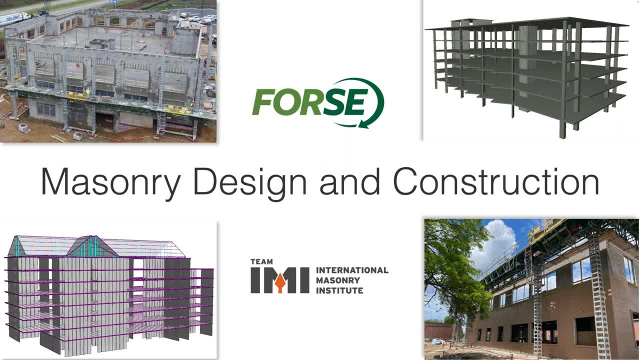 will be how you submit any questions you might have during the webinar, And then please feel free to ask any questions at any time and we will answer them at the end of each section. For any other issues that happen to come up, you can call Half Moon's customer service. 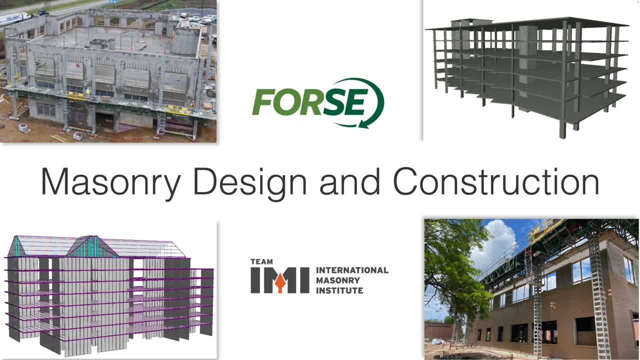 at 715-835-4255.. And I'll post that number in your chat section. You can email me and I'll post my email in the same place, or you can just submit a question as normal, and I will get it that way With. 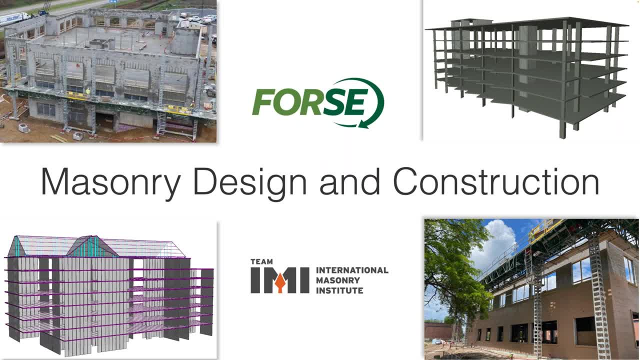 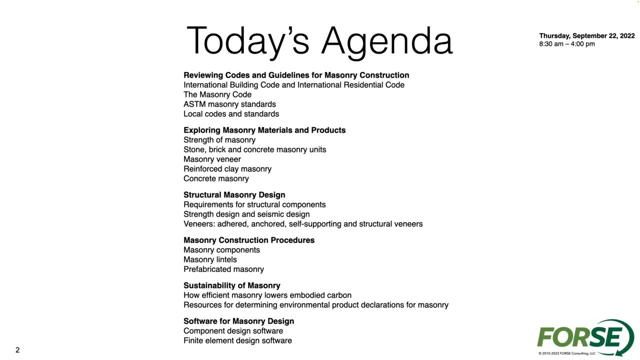 that being said, I am pleased to be in our program and welcome our speaker for today, Sam Rubenzer. Good, All right, so masonry design and construction. So today we're going to talk about a lot of different topics related to structural masonry design We're going to talk about first we're going 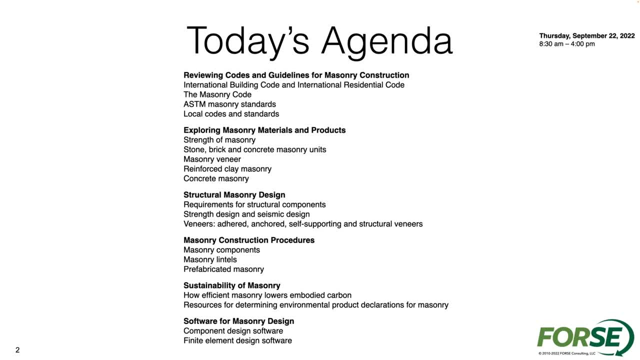 to go over some codes and guidelines for masonry construction, Just kind of a broad brush overview of kind of what you should be looking for with masonry design and the codes that you should be exploring. Then we're going to look at the different types of materials that we 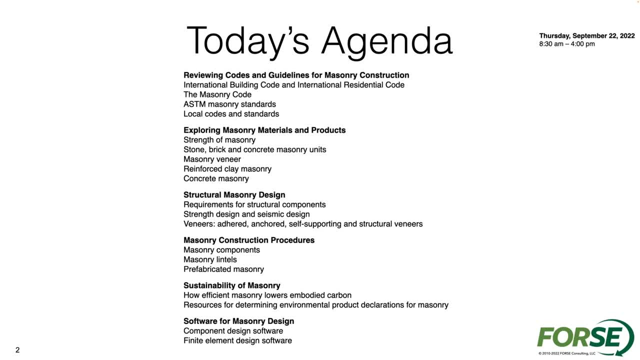 have for structural masonry. We have a lot of the common things that I'm sure are all aware of- the gray blocks and you know stuff like that- But then we also have a lot of other things that we're going to talk about today. So we're going to talk about the different. 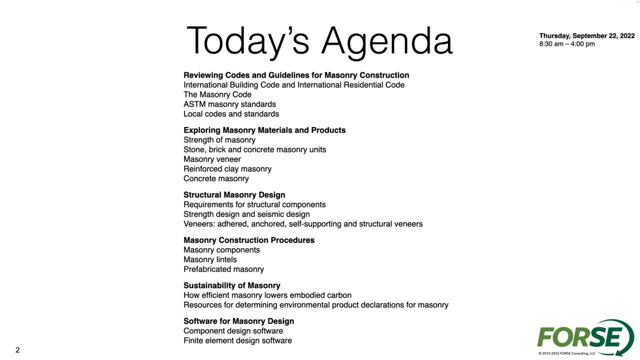 types of materials that we have for structural masonry. We have a lot of the common things that we have for structural masonry. We also have reinforced clay units and we'll talk about some other stuff related to the materials of masonry. We'll get into some of the design. 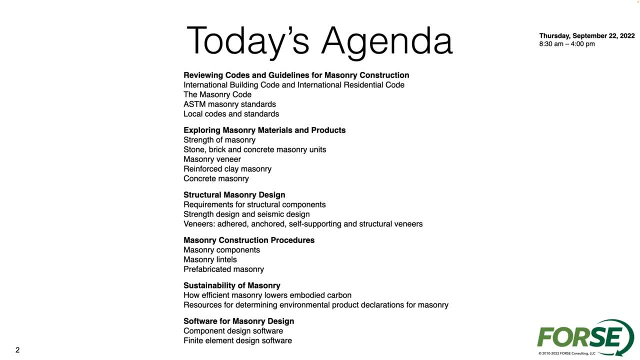 requirements for designing structural masonry. We'll look at some construction procedures. We'll look at the different types of elements of masonry that we want to look at designing. We'll briefly look at the sustainability of masonry, kind of look at some of the environmental. 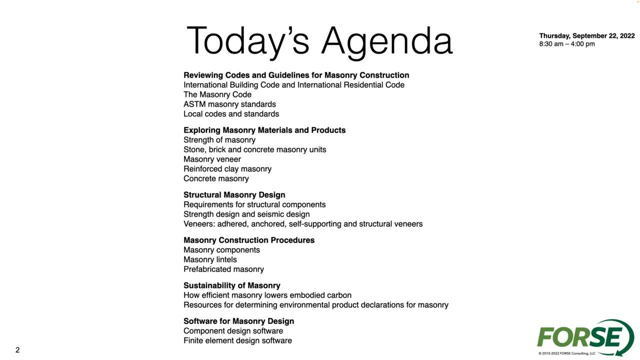 impact of masonry and kind of how to help with some of the those elements in design, and then, lastly, we'll wrap up with the software for masonry design, just kind of talking through some of the different options that we have for design elements. so i appreciate the introduction. my name is sam rubenzer. 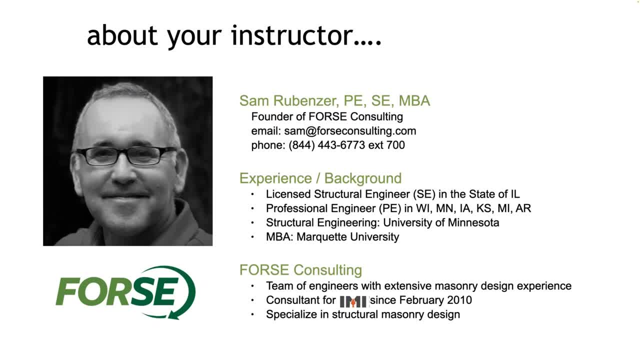 work in eau claire, wisconsin. i'm licensed in a lot of midwestern states and structural engineer in illinois, went to university of minnesota for the civil engineering degree kind of emphasis and structural and then spent a little time at marquette university. i am a consulting engineer. 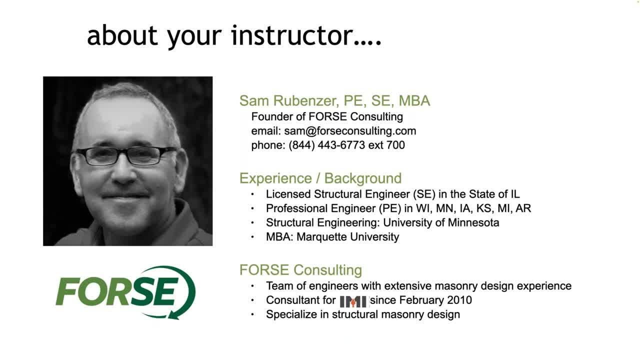 a lot of the work that i do covers all kinds of different materials, just like any other engineer: steel, concrete, so on and so forth. so we we cover a lot of different things. i'm i'm a consultant for the international masonry institute, so you're going to see them referenced on many different 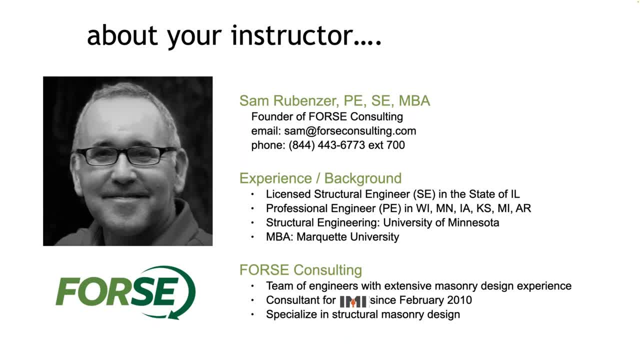 slides and a lot of different topics that we use. so i certainly specialize in structural masonry design again here in the midwest, but then also uh, oh, oh east, out west, and kind of pushing the borders of the country, so, uh, kind of designing all over the place. so, like i said, you know, and i'm a one of 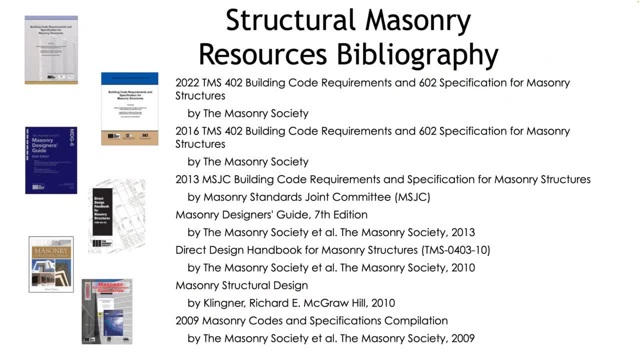 several people that work uh at force. so we have a lot of different things going on um some of the different- uh, excuse me, some of the different elements that we have have or codes that we are looking at. there's a lot of different options for masonry design. 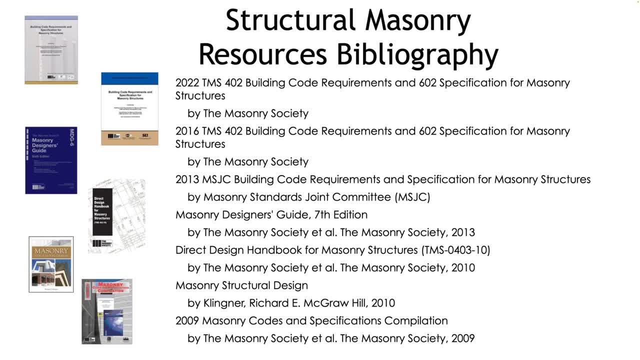 some of the primary ones that we'll focus on are the masonry codes that are referenced by international building code, by ibc. you know 2022 tms is going to be. the current codes is 2016, which is the current reference code. there's 2013 and then back and back we have different. 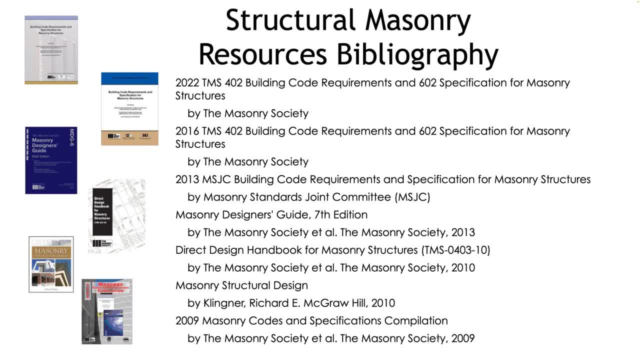 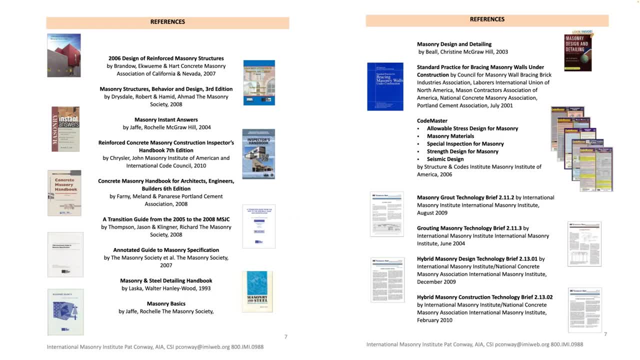 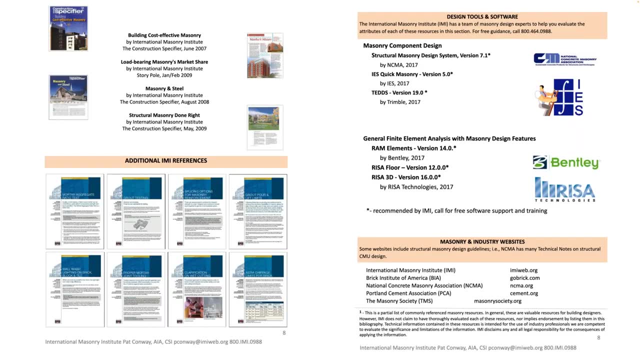 books and design guides. we have all kinds of different references here, so i just try to list a bunch of different references that i've used through the years and different types of- whether it's actual papers or books- that i think can be helpful. and then, lastly, you can see here: 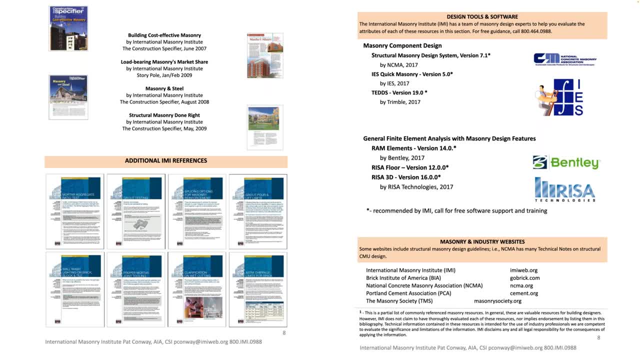 some elements from the international mainstream institute. they have a lot of different information and then, on the right, some of the different software programs that that i reference and look to. but we'll kind of reference those more during the program as we're kind of getting to some of the different options. so the first one: 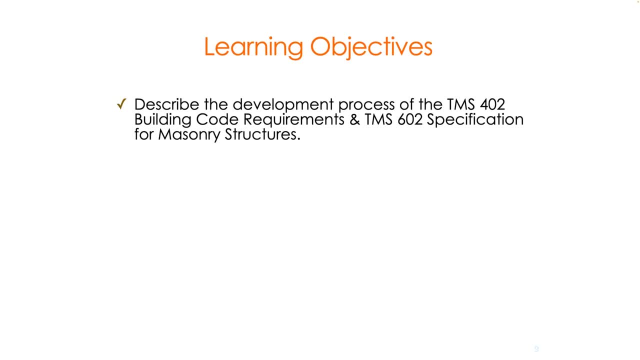 we're really going to be kind of focusing on code, so learning objectives for the code is just just kind of talk. through the development process of the tms 402 building code and the 602 specification for masonry structures, understand the relationship between ibc and tms. tms is the 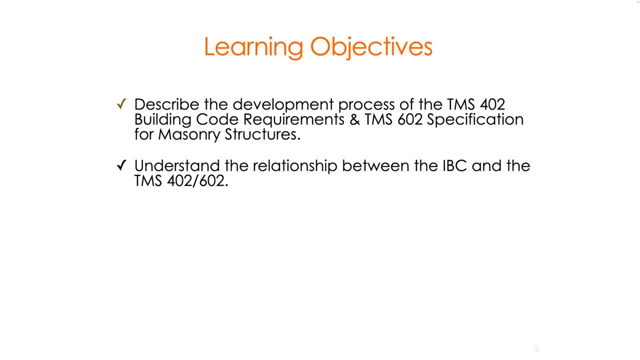 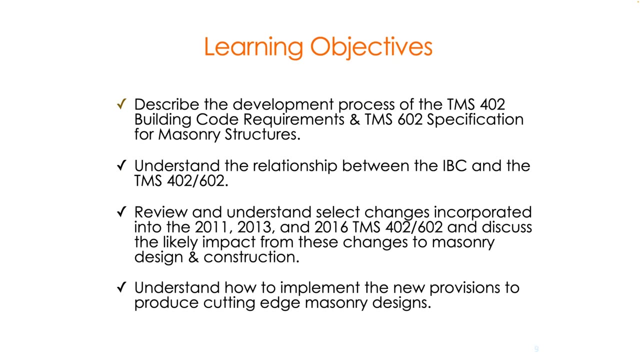 code that's going to be the code that's going to be the code that's going to be the code for masonry design review, and understand some select changes as they've been incorporated in the 2011, 2013 and 2016 code books, and then just understand how to implement the new provisions for design. 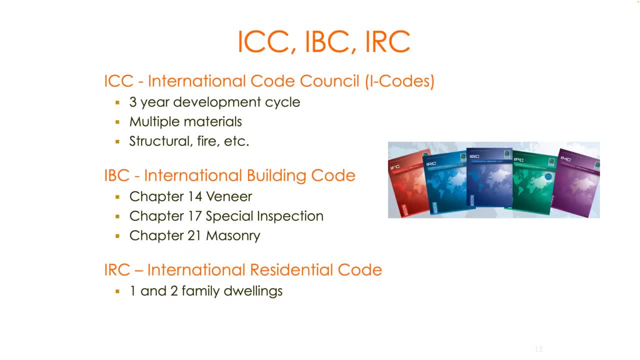 so some of the development process for masonry codes. hopefully everybody's aware of the different codes that are out there, international code count so they really are trying to go with a had been going with their three-year cycle for their codes. ibc international building code has several sections that are relevant for masonry chapter. 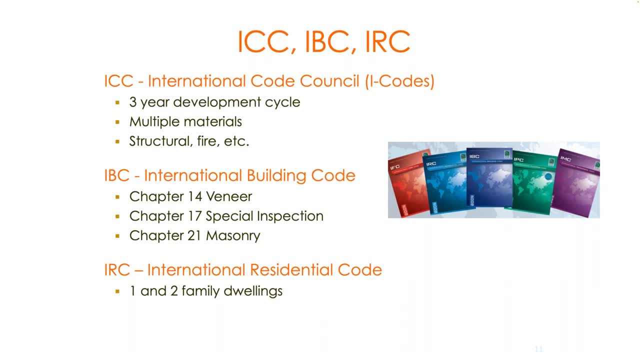 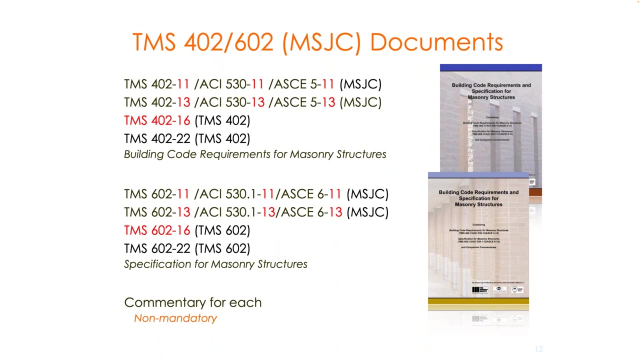 14, veneer, chapter 21, masonry, and then 17 for special inspection, and then you also have the international residential code. so that's the general codes that everybody is aware of, and then we get into the masonry specific codes. the codes for masonry used to be the msjc, the masonry standard joint committee, where we had 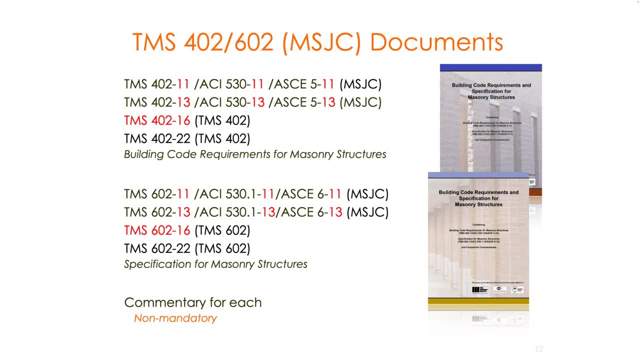 several different code bodies coming together to put out a masonry code, so that that's the msjc, the first two lines that you see there, where you had tms and you had aci and then you had asce. so as we look at those different code bodies, really most of the work was really being done by tms. 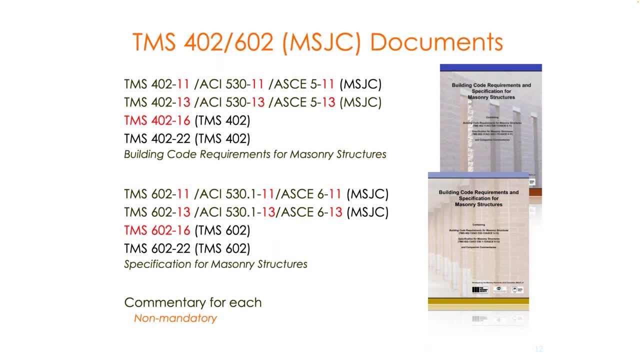 so in 2016, the masonry code just is now referenced as the tms code. tms 402- 602 are going to be the the building code requirements and the specification for masonry structures. that both come in that, that one book that you see highlighted there on the right. 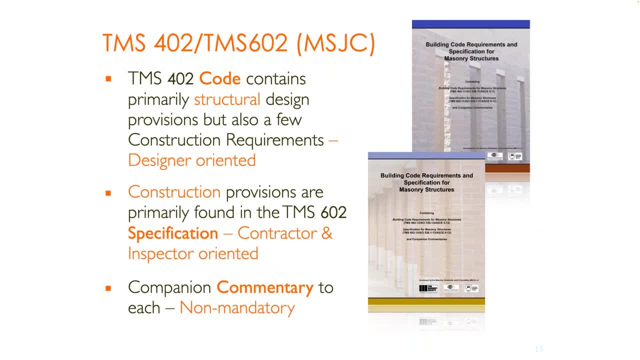 so 402 code is going to contain the primary structural design provisions. in this case the primary structural design. it's a general construction requirements. really it's kind of written for use, use in design, and it's really trying to help designers come up with different design equations and really trying to help everybody get get the masonry design. 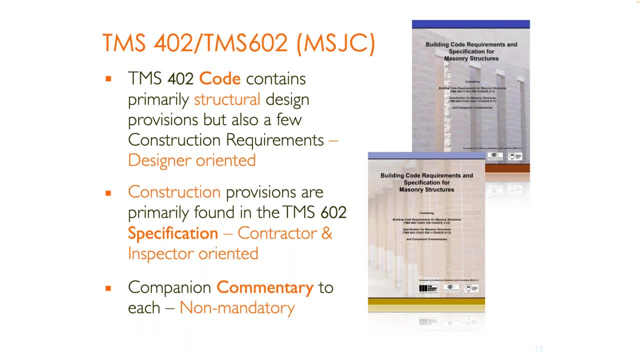 information out there. 602 is really a specification for, say, contractors and inspector oriented. certainly designers need to be aware of the different provisions in 602. there's a lot of things that are, too, that we want to be using as designers as well, but it's written just a little bit differently and 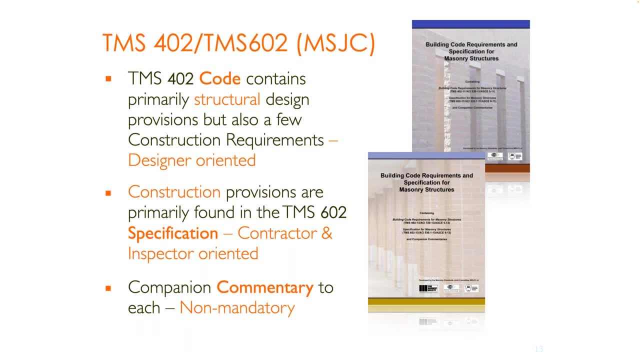 you know, like grout procedures and stuff like that is going to be, stuff that's going to be 602. so a designer might not need to think about all the different means and methods for grout, but certainly being aware of the different options that might be. 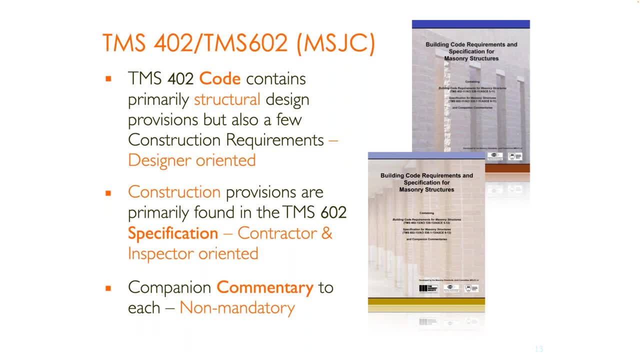 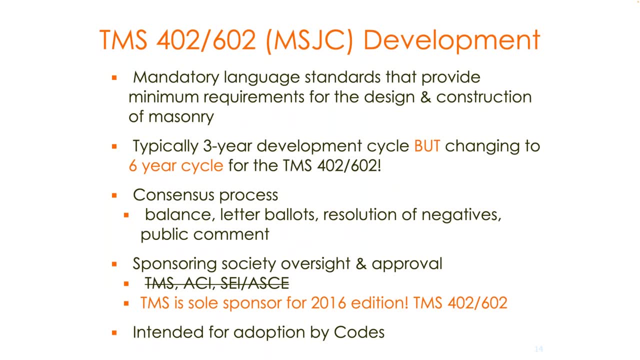 selected by designers or by contractors, and certainly there's a commentary which is non-mandatory. so in the development you have some mandatory language that provide minimum requirements for design. you know that that's certainly things that we have to stick with. it's been a three-year development cycle, but masonry is changing to a six-year cycle. 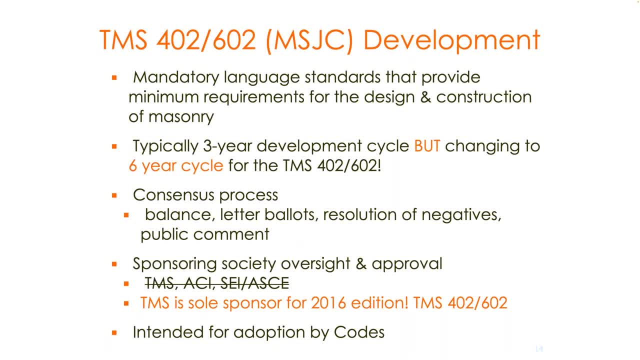 so just the 2022 code that just came out, that's been six years since the 2016 came out, and so that you know, obviously is you know we get a little bit exhausted with constantly buying reference manuals and and so on and so forth. we're trying to hopefully with the different 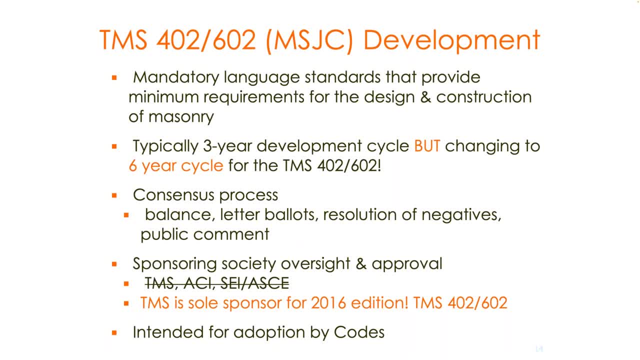 materials kind of settle down into a little bit less frequent code cycles. like i said, the the main sponsor now the main body that's going to be representing the code, is going to be the masonry society, so it's not going to be the collector of all the different bodies, it's just going to be. 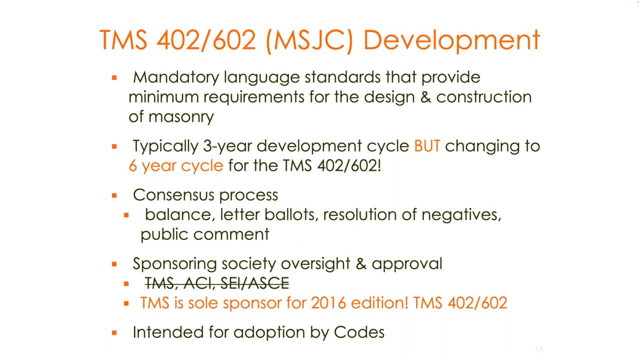 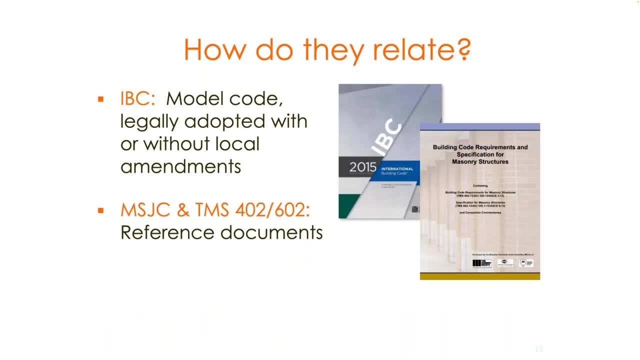 tms. so that's why we see the references to the codes being changed. so obviously there's going to be ibc is going to be the model code adopted, with or without local amendments, and then there's the, the masonry code. generally, you have to make sure that. 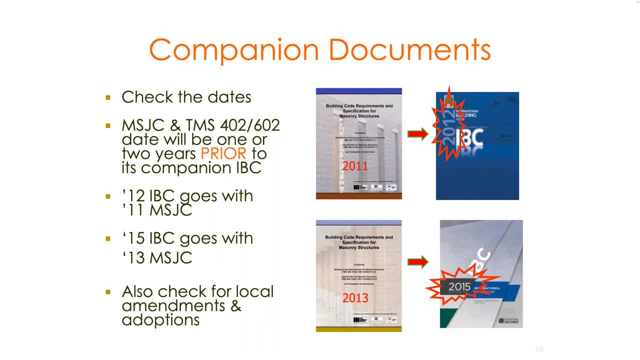 you check which masonry code is actually referenced by the different ibc codes. obviously that's always going to be important, the way the masonry codes are trying to be developed. now they're trying to be developed so they come out a year or two prior to the ibc, so that all the 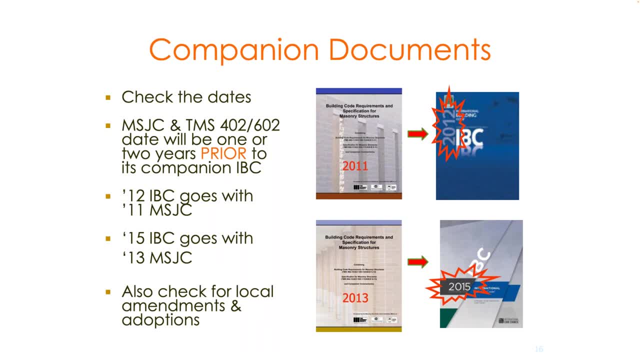 information in the masonry codes can be adopted into a similar year, maybe a year or two later, ibc code that can reference them. for the most part, ibc is referencing most of the information directly out of tms codes. that's going to be, i think, very useful in our designs to make sure. 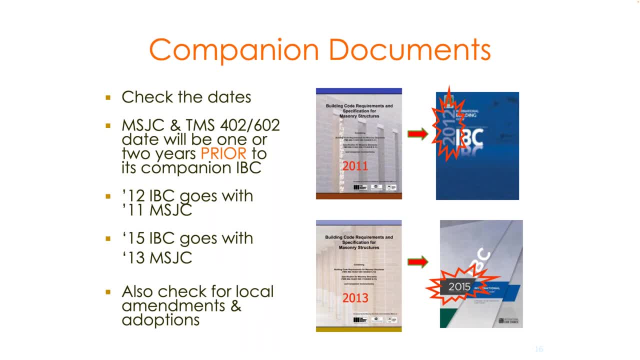 that we don't have multiple different codes, that we're trying to cross check and reference and make sure that we're not using something that's- um, you know, not working in the ibc when it says that it's working in tms. ibc is referencing more and more the mainstream code, as they do. 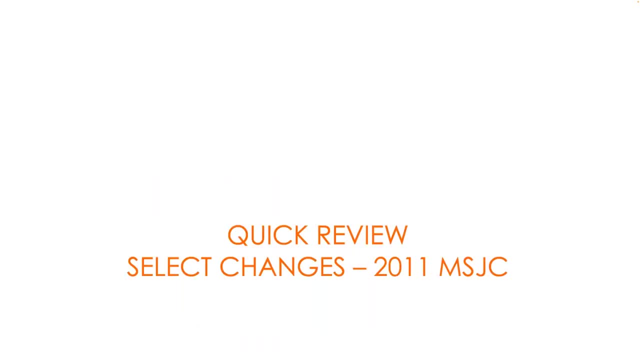 other machines to make sure that the masonry code is as good as it is in the ibc. so that's why we're trying to make sure that we're not using that stuff in the ibc. so that's why we're trying to make sure that. 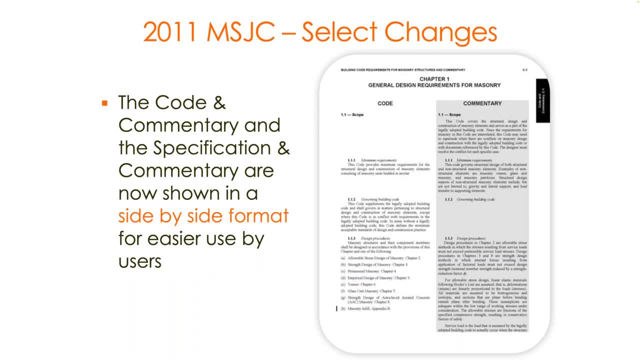 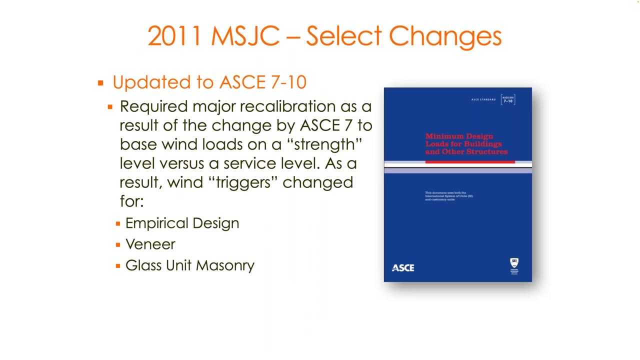 we're not using too many and too many materials. just as kind of a review, trying to walk through and look at some of the different changes that we have for the different codes. the code in the commentary are now kind of in a side-by-side format which is, i think, a little bit. 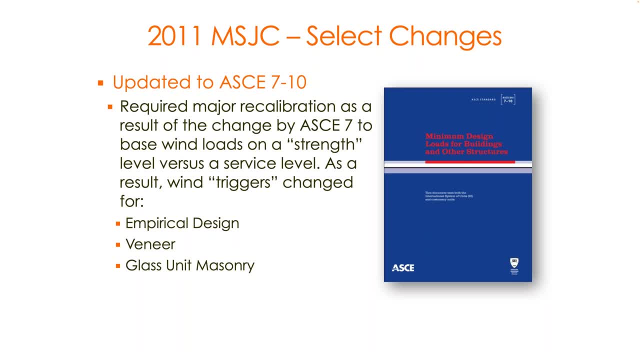 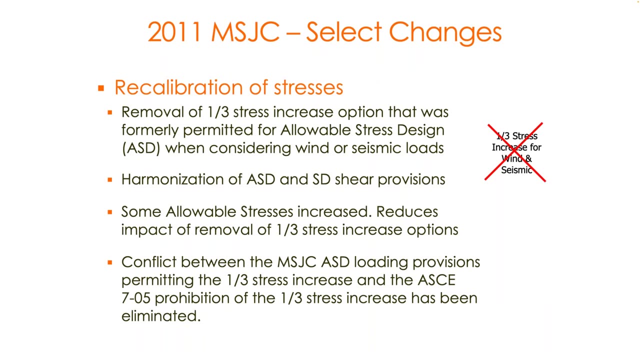 So that was kind of a major change, if you guys remember, for wind design and some of the different factors for wind design: empirical design, veneer and glass unit masonry, all updated to the newer design codes. We had a recalibration of stresses. 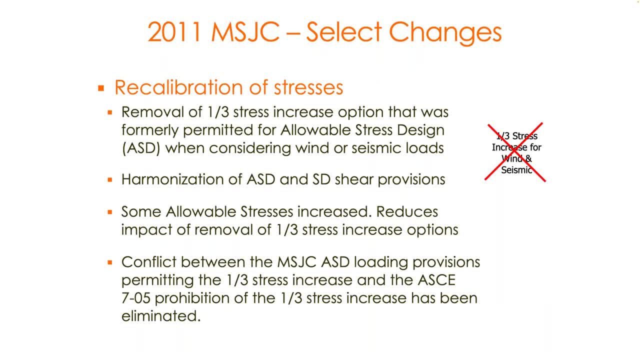 Anybody that's been doing masonry design for a while remembers the one-third increase option that was formally permitted for ASD when considering winter seismic loads. So that was taken out. We just want to make sure that we just have some simplicity there. 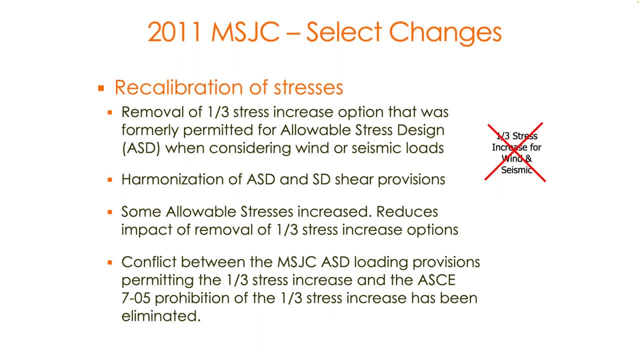 And so all of that stuff is still going to be there in terms of safety, but it's going to be more cooked into the capacities so that we don't have to worry about increasing stresses relative to those two different design modes. There's more harmonization of- and I see this- this certainly started back in 2011.. 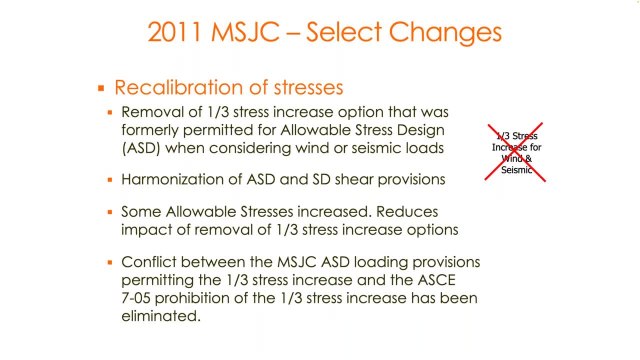 That goes all the way to the current 2022 codes, Trying to bring together the ASD and strength design provisions so that you have similar results between the two different code options. And boy, I see that a lot across different materials. We don't want to have design. I mean, certainly there's preferences. 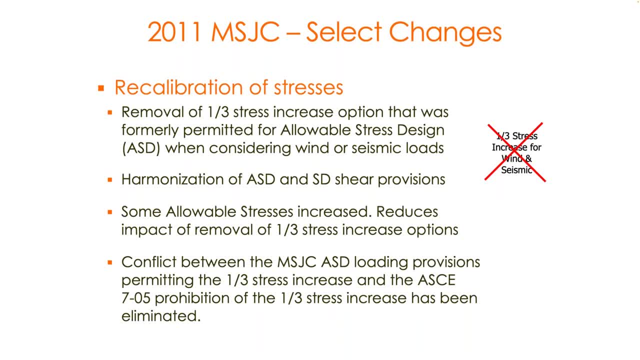 Designers have preferences in terms of, maybe, the way that they learn or understand materials and design provisions, between the level of stress and strength. design that really should come up with very equivalent results. just because you have a preference in design for procedures Doesn't mean that you should have a completely different capacity. that gets determined. 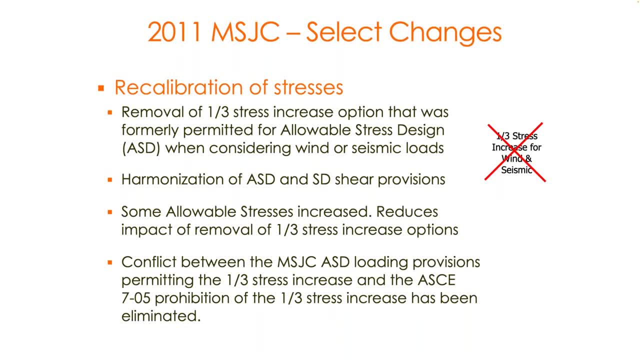 So when the codes, especially the mainstream code as it was developed- I mean it definitely had different parts of the code that were more current- strength design provisions tended to be more current than allowable stress design. So there'll be new things that would be added to strength design provisions that weren't 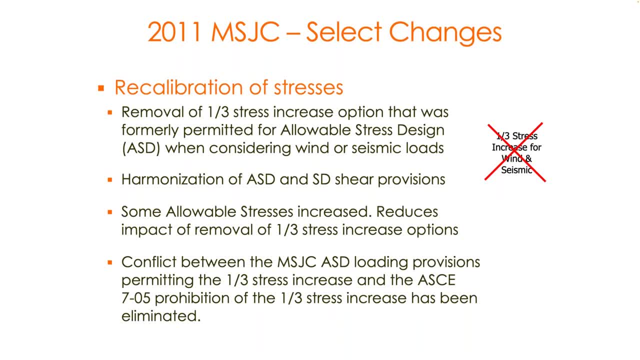 in the ASD provisions. So what that created was a pretty big difference, And sometimes in some of the capacities. But we really don't want to have that. I mean there's really no good reason for doing that. Just again, because of your preferences to the code doesn't mean that you should have. 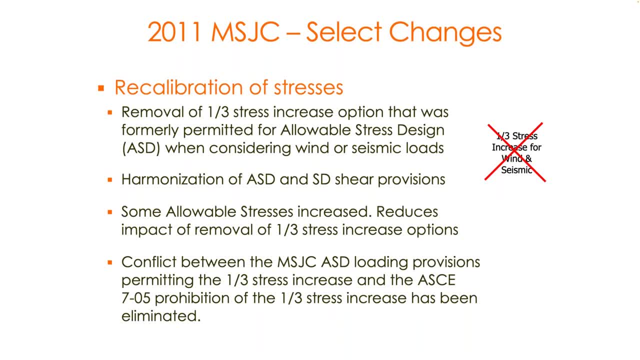 wildly different answers. Certainly there are different procedures, so you can have some small differences, but we want to make sure that that kind of is brought closer and closer together. Some allowable stresses were increased. Some of that- sometimes that was, you know- reduced the impact of the research. 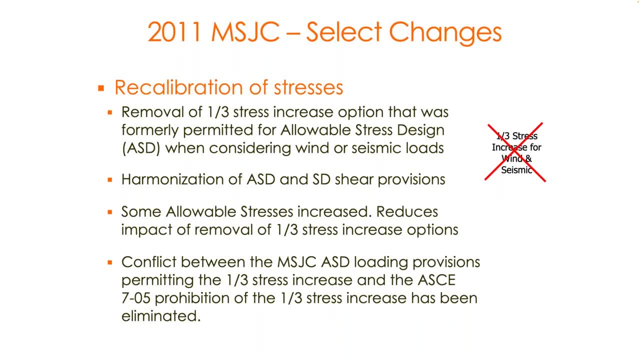 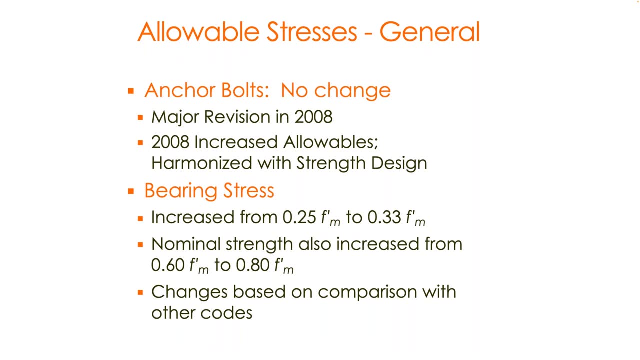 The one-third stress increase options. there was some conflicts between ASD loading provisions and the one-third stress increase in the ASD 7 prohibition of the one-third stress increase. So all of that stuff is certainly now been eliminated. For the anchor bolts, there was really no change in 2008.. 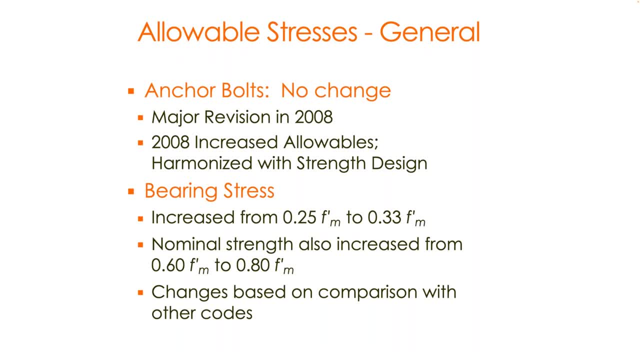 There was an increased allowables kind of some harmony with again more with strength design Bearing stresses increased from 25% to 33% of the strength of masonry, So giving a little bit more capacity there And again. sometimes, as these provisions change, it's maybe more testing was done to have a 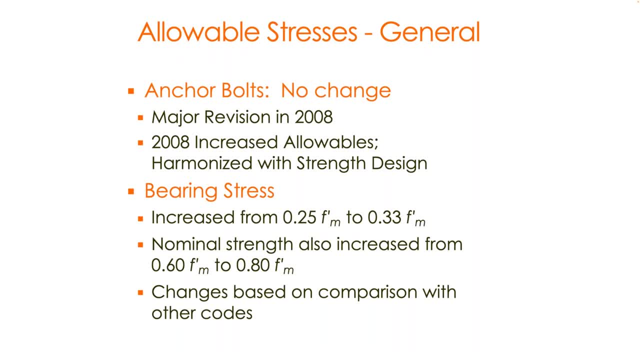 more, better comfort level with the overall capacities. It's not that masonry and bearing got stronger suddenly, but a lot of times that is what the code is. It's really just having a better understanding And the code writer is having more comfort in increasing capacities. So, as you can see there, So the nominal strength also increased from 0.6 to 0.8.. And then it also makes it similar to other materials, Unreinforced masonry. Yes, we can still design with unreinforced masonry. 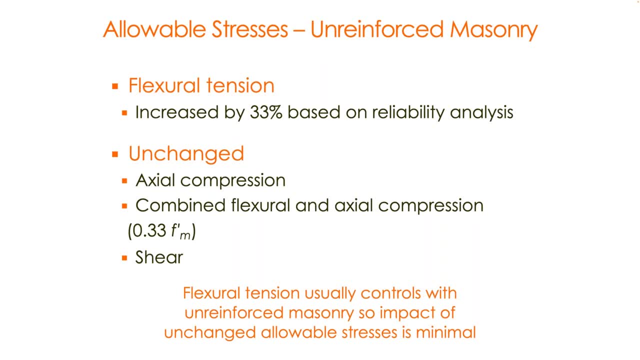 That is definitely something that you know I'll reference from time to time today. I think that's a pretty important aspect of masonry design- Certainly not a major strength, But it's definitely something that we can still use. I think structural elements aren't going to be unreinforced as we get into some large 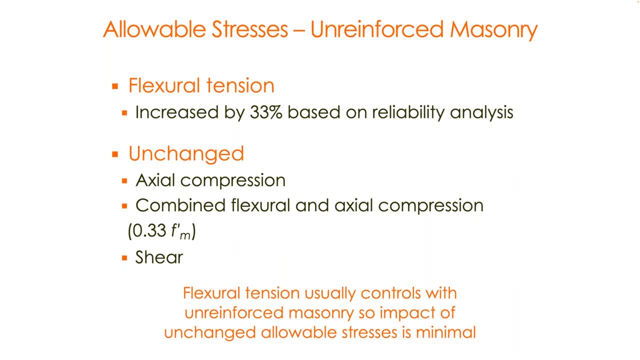 tall walls or sheer walls- Large elements are still going to be reinforced, But we do have plenty of options in times where an unreinforced partition wall or different parts of mainstream buildings can still be unreinforced mainstream. So that's a really important element for designers to remember in reference. 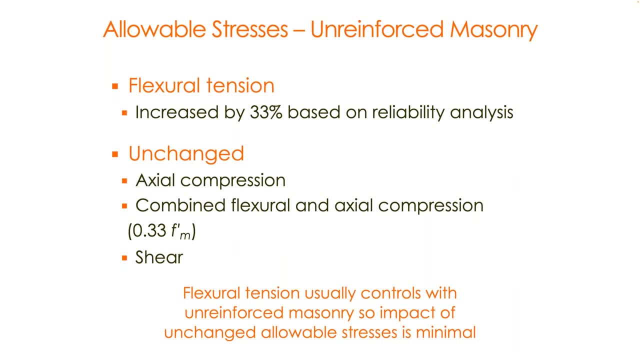 So we'll talk about that, Thank you, So we'll talk about that, certainly in different parts of the day, different sections as well. Flexural tension was increased by 33% And axial compression was unchanged. combined with flexural and axial compression, 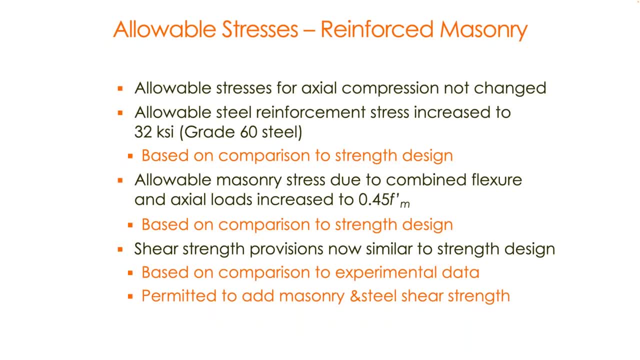 So just some of the different updates that were done there: Lovable stresses, Reinforced masonry. Lovable stresses for axial compression- not changed. Lovable steel was increased to 32 KSI for a grade 63.. Okay, Lovable steel, again more comparable to strength design. 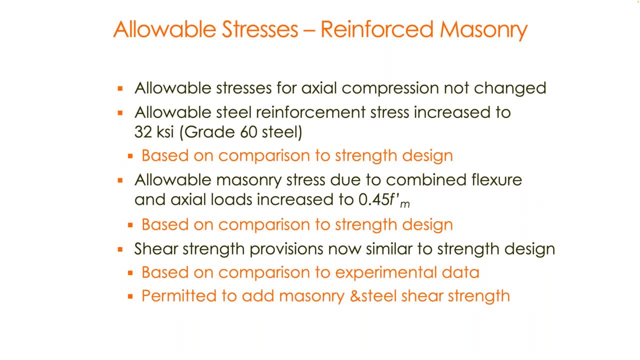 And then you have allowable masonry stress due to combined flexural and axial increase to 0.45. strength to base rate: again. to bring it in a little bit of harmony with strength design, Shear provisions now similar to strength design based on comparison to experimental data. 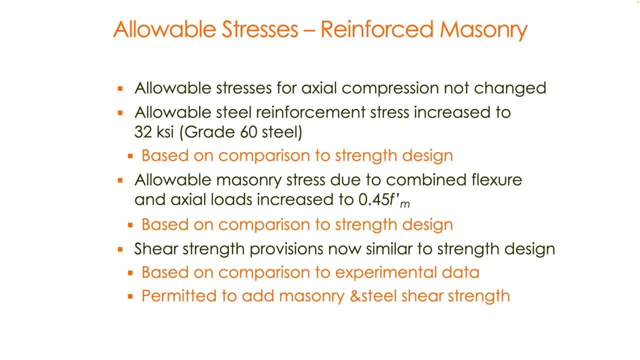 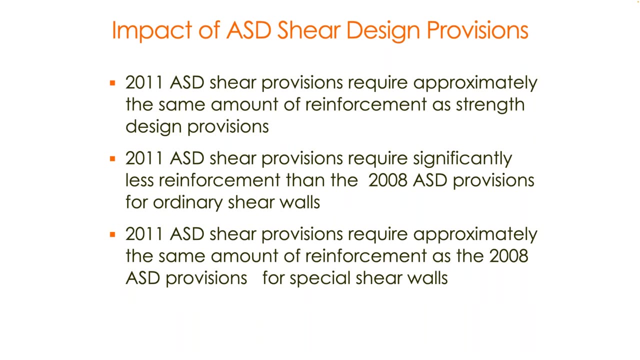 Again, strength design provisions were maybe created more currently, So just bringing allowable stress design closer to that. Okay, So with the impact of ASD strength design provisions. So you have approximately the same amount of reinforcement to strength design. Really, again two different procedures. 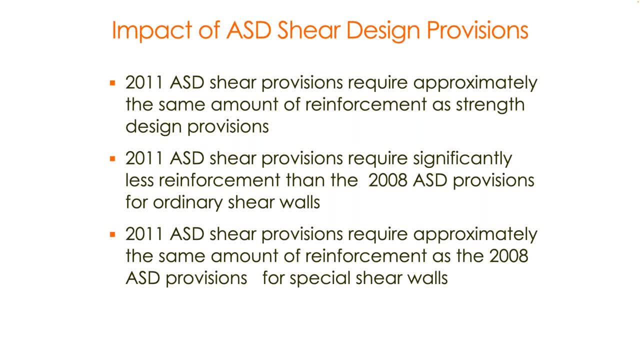 We don't want to have wildly different results. ASD shear provisions requires significantly less reinforcement. So again, that's going to be important for some of the typical common masonry walls, And the shear provision required approximately the same amount of reinforcement in 2008 for. 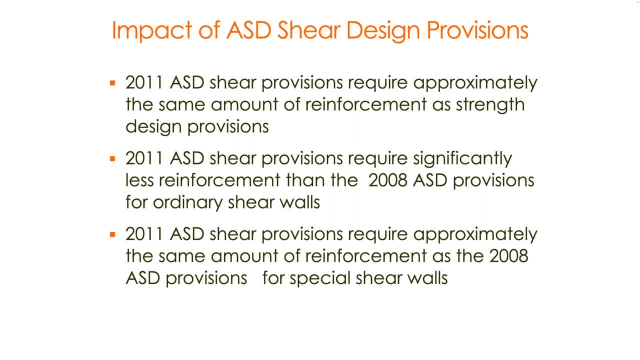 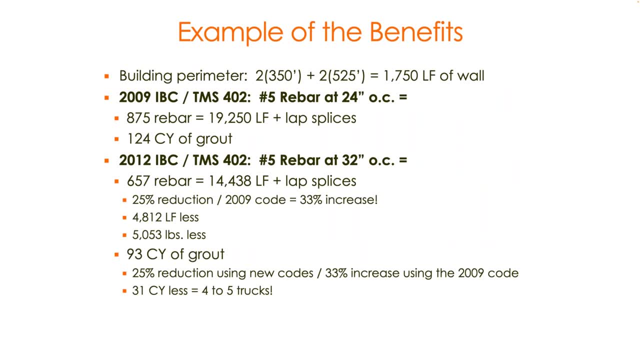 a special shear wall. So those things are certainly important as well. So just kind of an overall example of the benefits: If we look at a building perimeter, say, like a 350 by 500 foot building, 1,750 linear feet of wall. 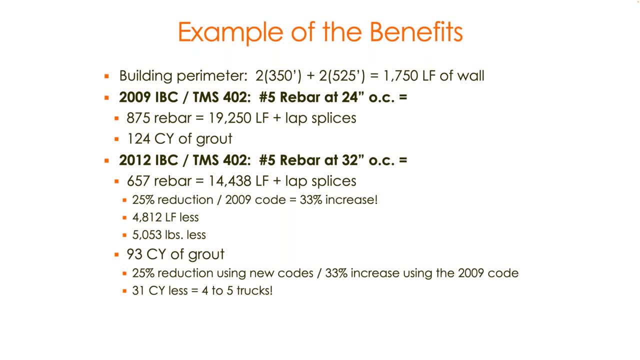 So if you look at 2009 in the masonry relative to that number five at 24, you have a certain amount of rebar, a certain amount of grout. That's a lot of reinforcement. You know, that certainly doesn't seem to be changing much if we go from a 24 to 32.. 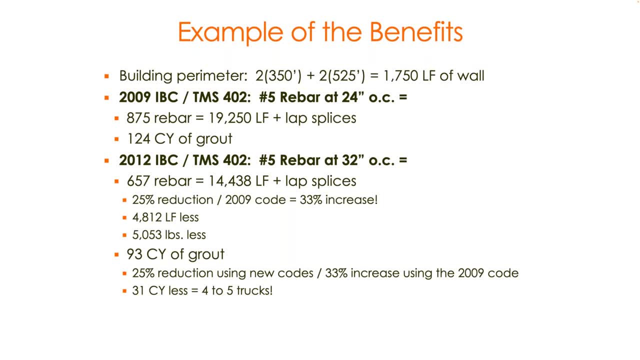 So with the current code, or with that more current code, it does require a lot less bars, a lot less grout. you know it's really going to be saving. you know, small changes in masonry designs. You know, as I talk about that in different times, being more efficient with masonry it. 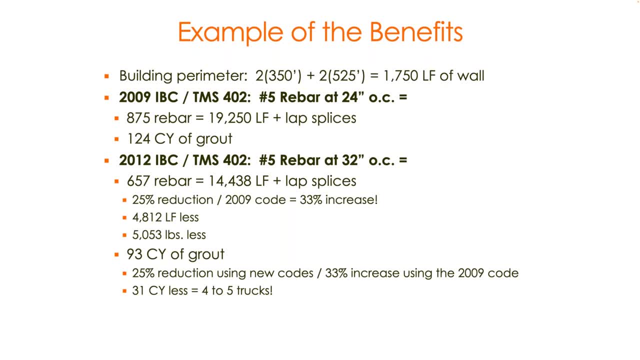 doesn't have to be much and you can really save quite a bit. You know going forward. You know saving 33% of the grout or something like that could be a pretty significant amount of material that you can save and placed within confined spaces. 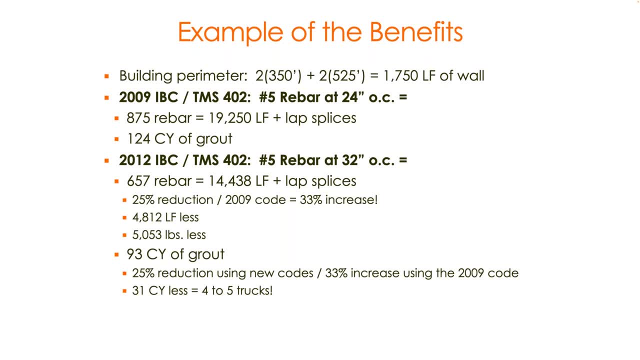 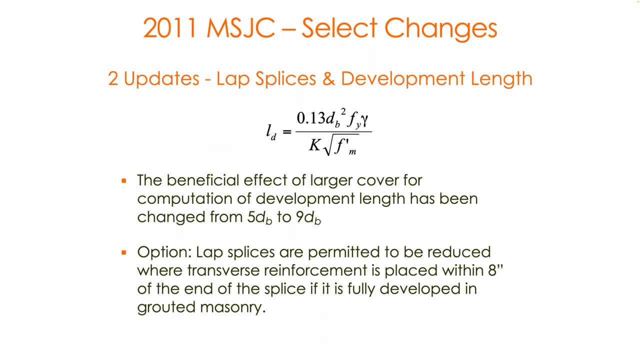 All that stuff makes a pretty big difference, So we want to make sure that we continue to go with that. You know, in 2011, really, the masonry code really got pretty specific about the lap lengths, and IBC has certainly been a big part of that. 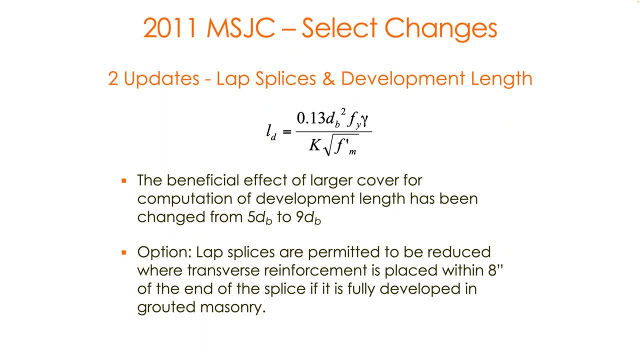 I mean, you know it's a lot of work. It's a lot of work. It's a lot of work. It's been getting us more and more information or giving us more and more leeway to use the TMS, the masonry codes, provisions for lap lengths. 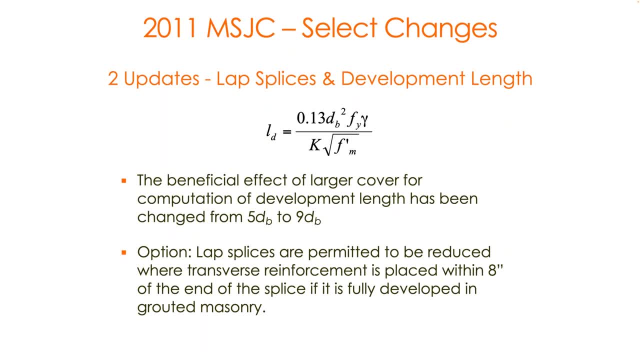 I still have people that will talk to me from time to time and using some of the old provisions based on IBC, but we don't want to use lap length provisions that were developed by the masonry people by the masonry code, and here you can see the equation for lap lengths. 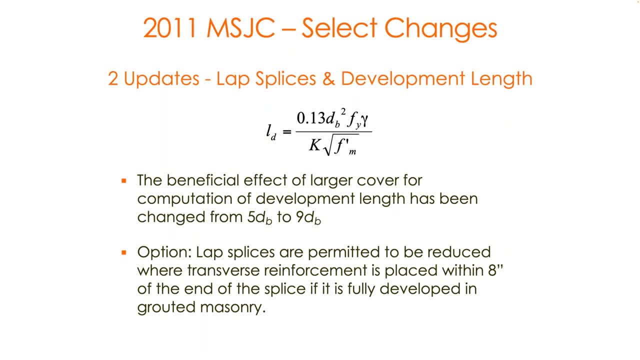 A larger cover. It's been Taking into account for the computation of lap length change from five to nine, So that certainly helps with lap length. Lap splices are permitted to be reduced within when transverse reinforcement. So what does that mean? 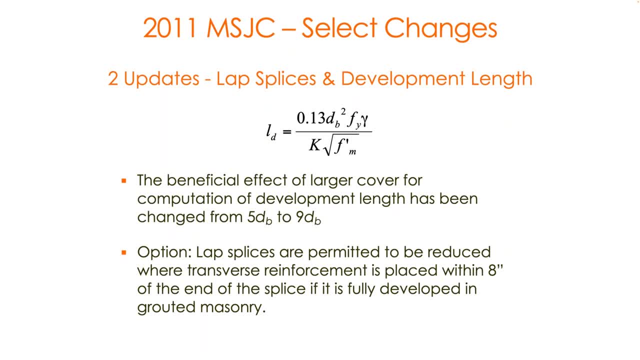 So any time that you have a wall, that you have vertical reinforcement, that you're trying to lap, if you have horizontal reinforcement within that wall, where the horizontal reinforcement occurs, where the bars are lapped, then we can reduce the overall lap lengths, Okay. 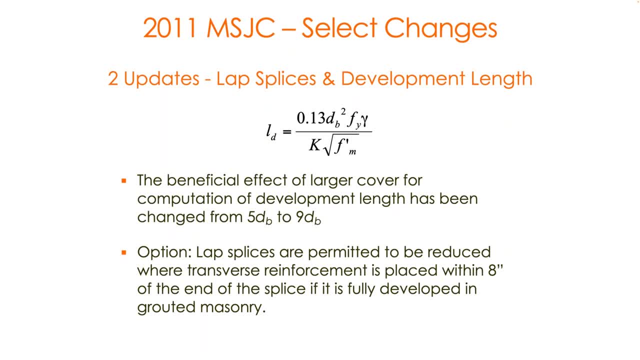 And so that can certainly help you know for different elements of the design. You know, if you have a wall that's got both horizontal and vertical reinforcement, just detailing that wall correctly can really save on some of the overall lap lengths and that. 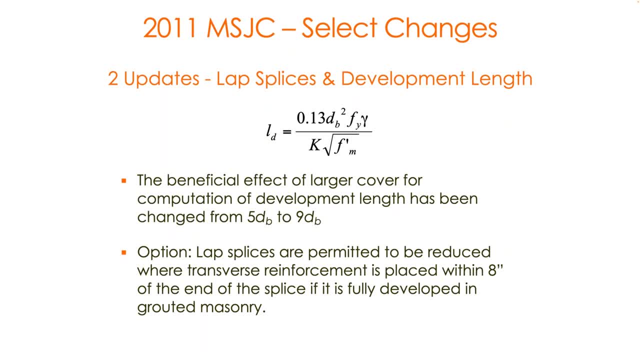 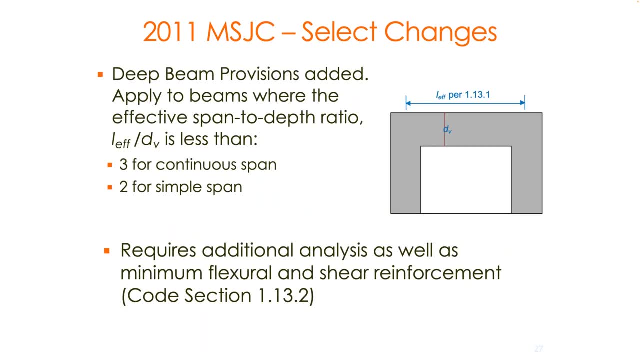 can make a pretty big difference, certainly as some of the bars get a little bit larger. So it was really nice to be able to see that get added to the code and have that help us design wise a little bit, Okay, Okay. 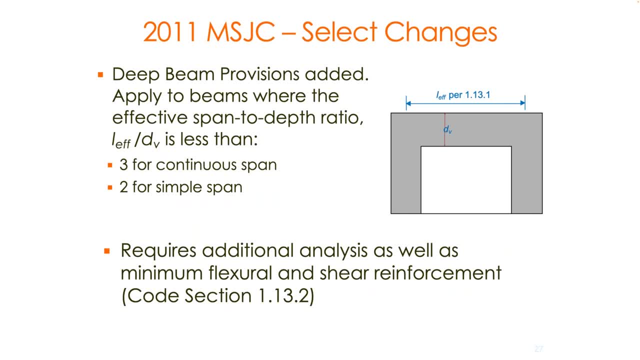 So in 2011,, there was some deep beam provisions that were added for masonry, and this can be very useful as well. We'll talk about masonry and masonry lintels here at different parts of the day today. You know, if we look at a masonry wall, you know one of the big misconceptions that I. 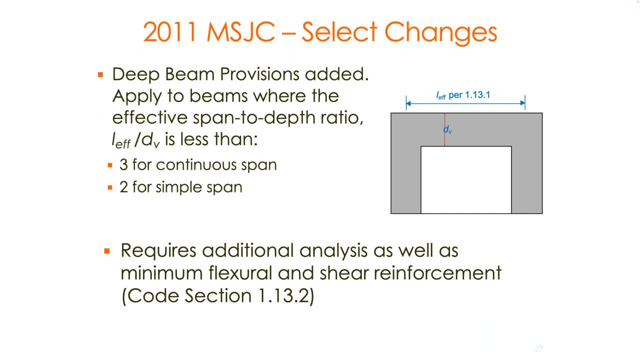 think people have is that we need some sort of different material to be added to a masonry wall to span an opening. Not only is that not true, there's a lot of different options for designing masonry walls, So the different provisions being added really kind of a couple different images, really. 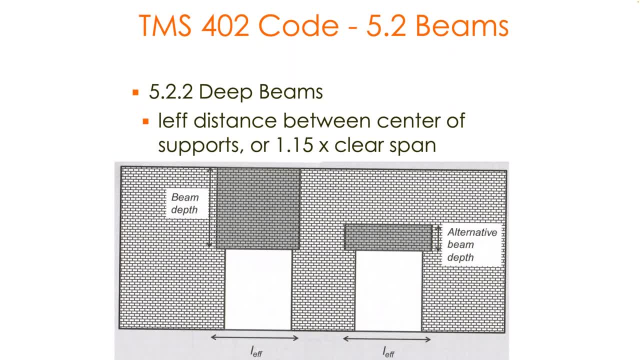 do help. You know deep beams could be added or looked at as the entire height of the wall above an opening. Really, when we have a masonry wall, we have everything that's staying interconnected there. Really you can utilize and you would utilize. the wall itself is going to be spanning that opening. 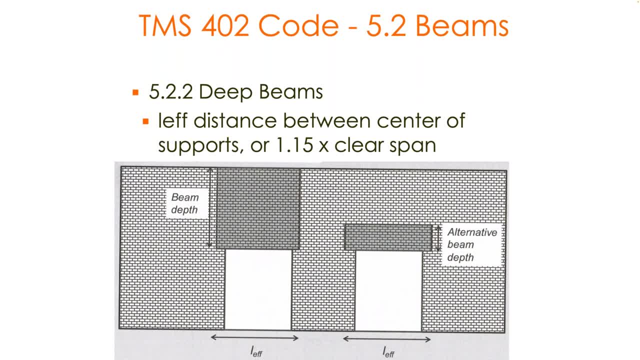 It's going to be working together to span that opening. There's no smaller parts of the wall that can fail and the rest of the wall is going to stay in place. I mean it's really going to be working together. So kind of giving us some deep beam options is really a nice way to look at the reinforcement. 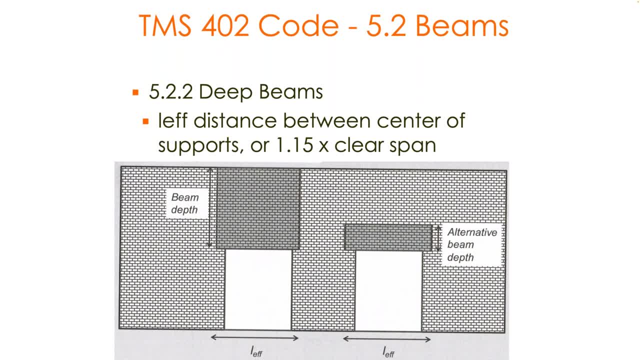 that you can add for a wall above an opening and not have some other different material that's going to be needed. You know there's an alternate beam depth which would be a lower height. We're not going to be using that But again, I like how the code writers developed this and pointed out. you know, if we do want. 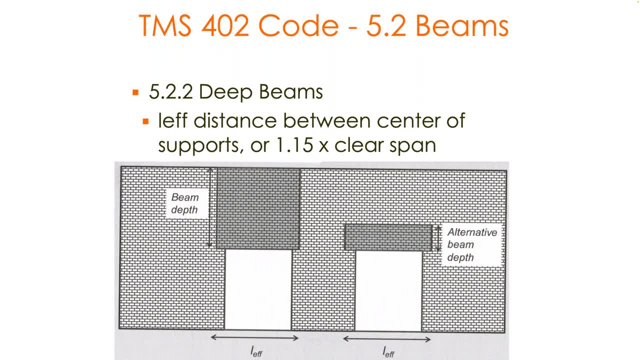 to look at the shallower depth, then maybe that's a little bit easier design-wise and a little bit less detailing requirements. That's the alternate, You know. again you have the whole wall that's going to be working to span that opening. 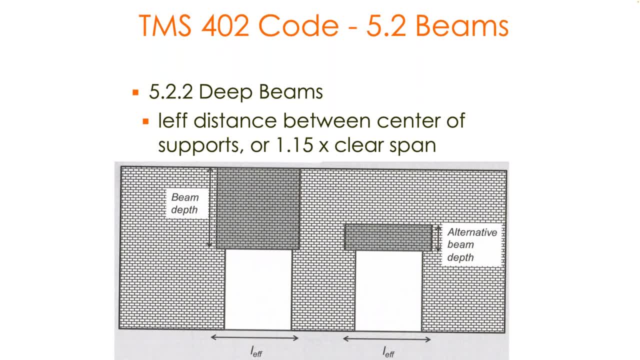 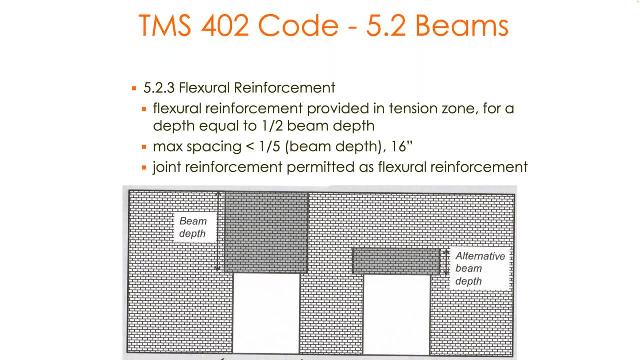 We might as well use that wall design-wise. So in those deep beams, you know, flexural reinforcement added in a tension area equal to half the beam depth maximum. The maximum spacing could be 20% of the beam depth or 16 inches. 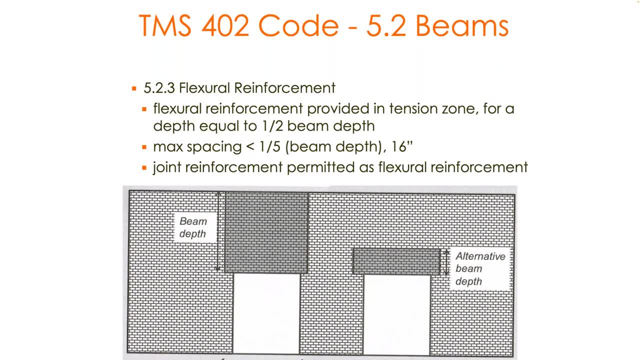 Joint reinforcement permitted as flexural reinforcement. I mean, certainly that's a very nice way to add some reinforcement in the deep beam areas. considering all of the joint reinforcement that's going to be added to our walls, We have shear reinforcement and different requirements for shear reinforcement, spacing for shear reinforcement and then the total reinforcement. 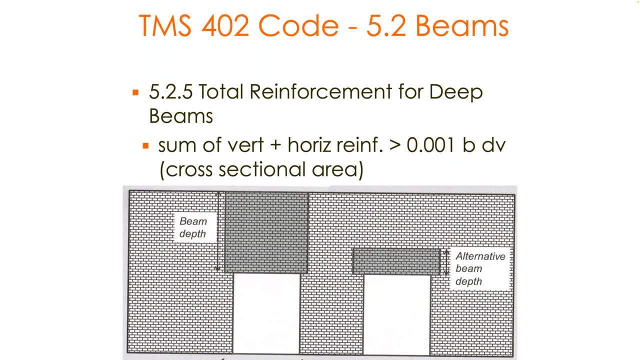 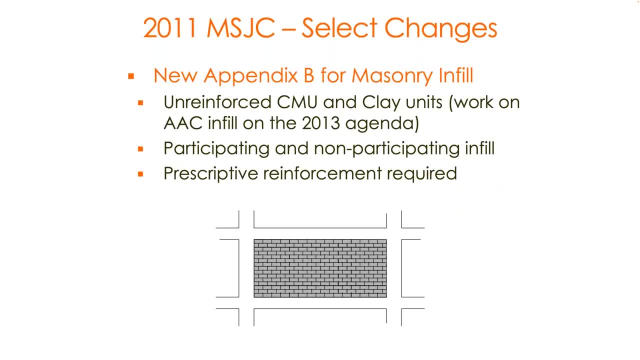 for the deep beam. So again, it's a very nice option for being able to look at the design of the wall above an opening and how it can span an opening. It's very nice to see they get added to the code. 2011 also looks at mastering infills, so unreinforced concrete or clay. 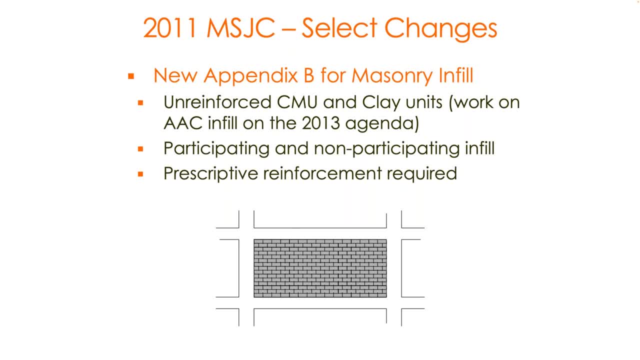 So this is going to be developed more in later codes and we'll kind of see some of that as we kind of review those as well. So you have participating and non-participating infills. So you have non-participating and non-participating infills. 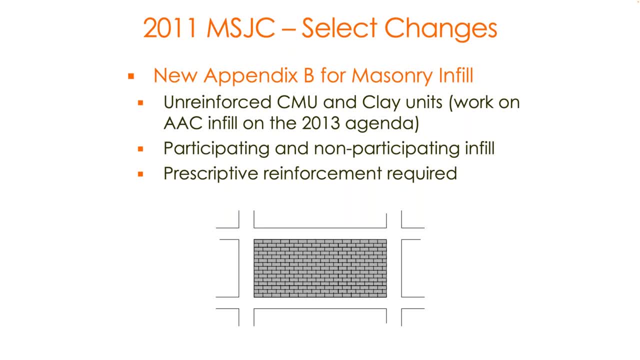 So you have non-participating and non-participating infills. So you have non-participating and non-participating infills. Really, the strength that you have in filling this elevation that you see below is really going to be looking at the elevation where you have, say, a concrete frame or you have 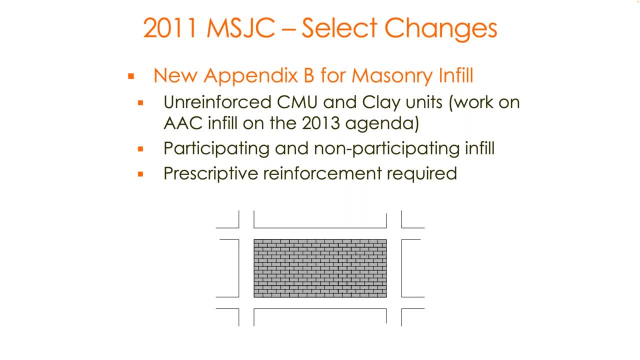 some sort of a frame and you're infilling it with masonry And a lot of times it's not going to necessarily be a structural reason for adding in that masonry. Maybe it's an architectural, probably an architectural reason for adding in the masonry. 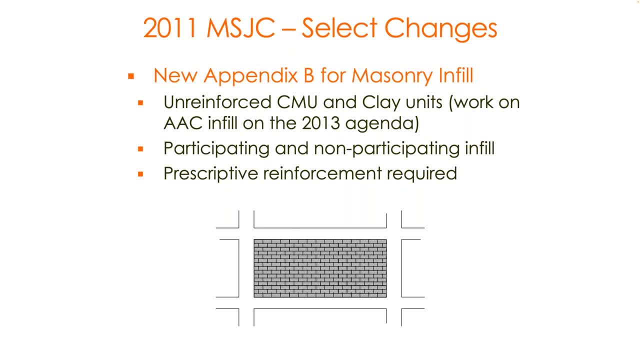 So when we do that, we can either utilize it and make it a masonry, or we can either a participating infill, and so then there's certainly design provisions that go along with designing it as a participating in resistant shear and maybe even axial loads, or a non-participating 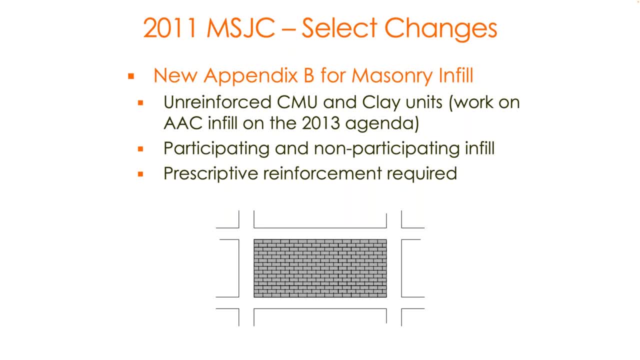 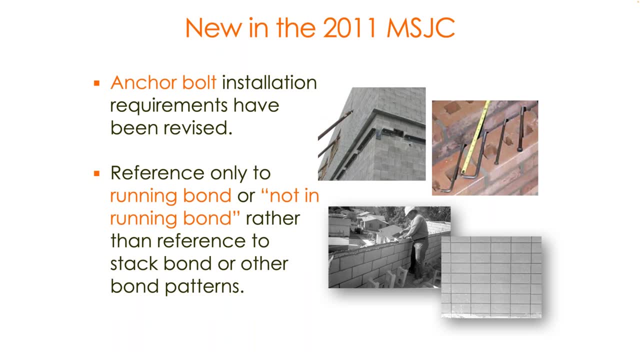 infill, where it's just going to be there architecturally, and then what some of the design checks for that are anchor bolt installation. so we see some different developments for anchor bolts and so, as we're attaching dimensioning, it's going to be important to utilize the current references for anchor bolts- references to running bond or not- in 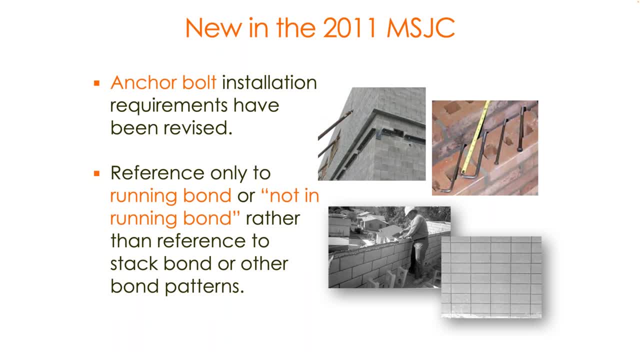 running bond. hopefully that takes out some of the misunderstandings between the different bond patterns. obviously there's, uh, the very direct stack bond and then there's the very direct running bond and then there's all the in-between. so running bond or not in, running bond is. 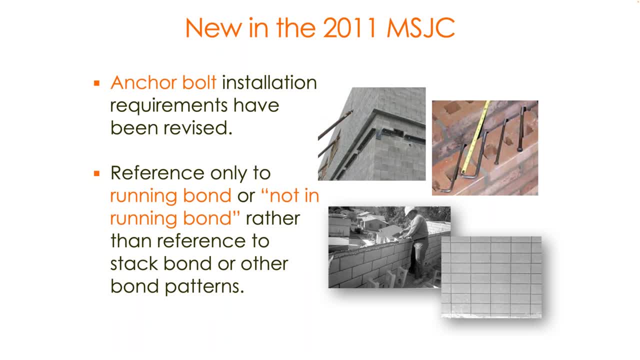 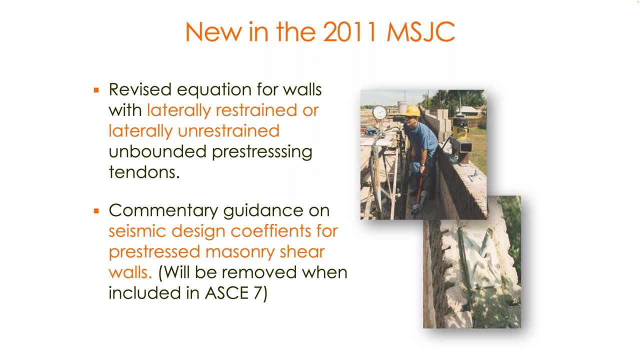 maybe a little bit easier way to reference and capture all the different options that are there. you know we don't see a lot of pre stressing for masonry. hopefully we see more and more as we go. I think there's a lot of different times for pre stressing. 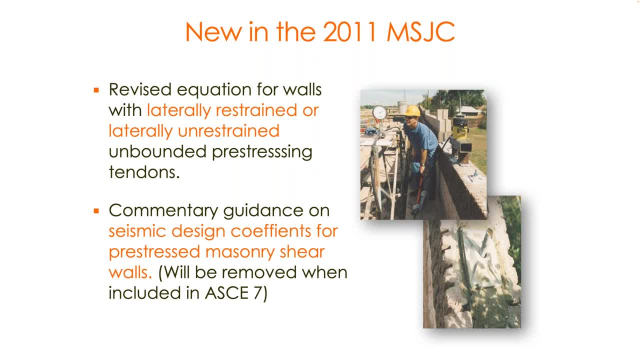 masonry is going to help. with masonry design we see more prefabrication, mainstream, which we'll talk about a little bit later, but that that certainly can help quite a bit, you know, as we're going to be maybe building and shipping mainstream panels. so having some provisions for pre stressing and having 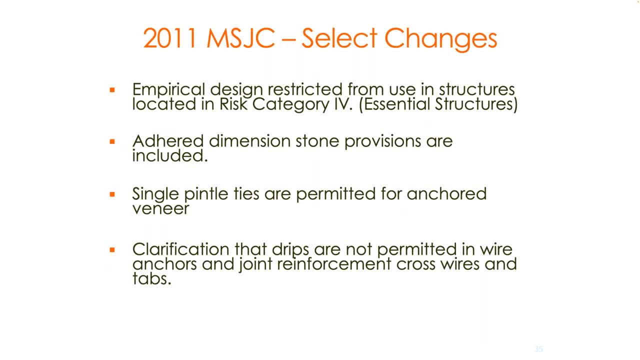 some of those updated as well. some of the other changes empirical design: empirical design is definitely something that I would love to see, love to see moved out of the code. I mean it's it's really doesn't have a good place in in structural design, whether it's concrete, steel. 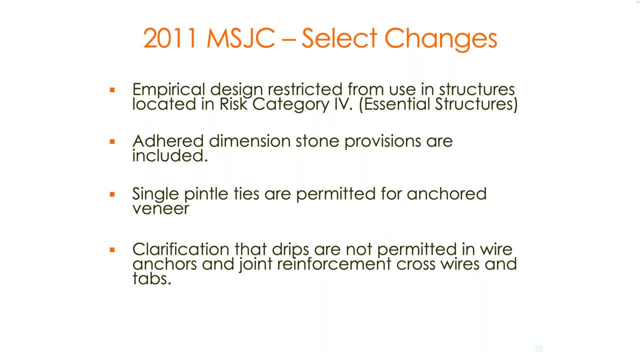 well then, the material you're looking at- empirical design is- is really something that we used to use, something that we should be moving away from, so it was restricted in its use all the way back to 2011. you can see it moving further and further out as we go. here we have some adhered dimensional stone. 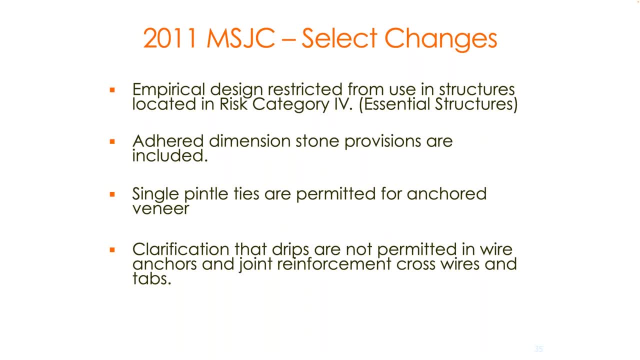 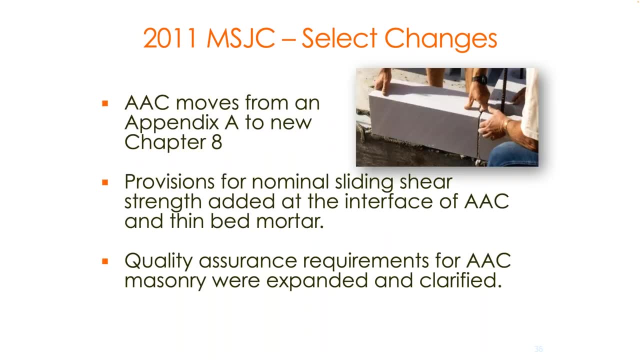 provisions added, ties permitted for anchoring veneer and so just other changes that we made in the 2011 code AEC. that is a material that I think we can explore more: autoclaved aerated concrete In the masonry code. it makes a lot of sense. it comes out as units. it certainly has joints. 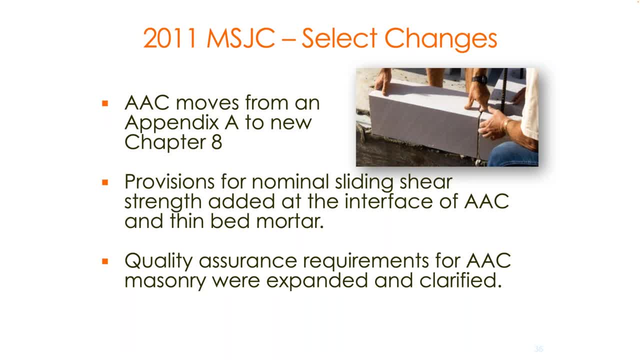 and they're solid blocks, so they're a little bit different than the standard masonry elements. They have a lot of great architectural reasons for using AEC. AEC is a material that we don't talk about nearly enough here in the United States, but 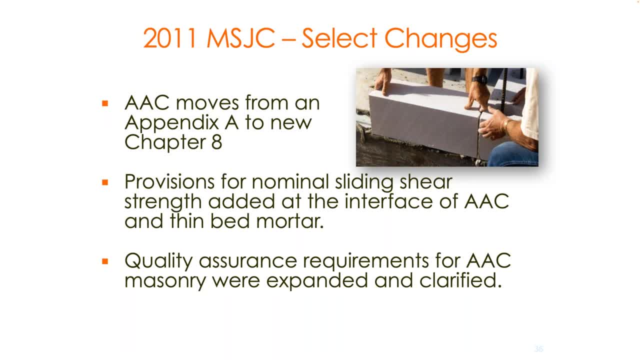 it's definitely a material that's got a lot of potential for meeting different energy codes, fire ratings. it's a really, really great material for a lot of different options in masonry. So having that moving to a standard chapter in the code and not just an appendix obviously. 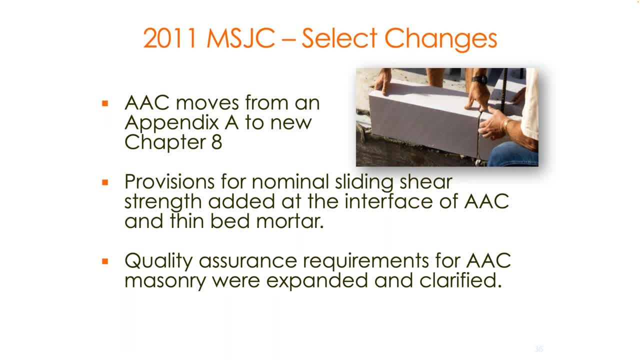 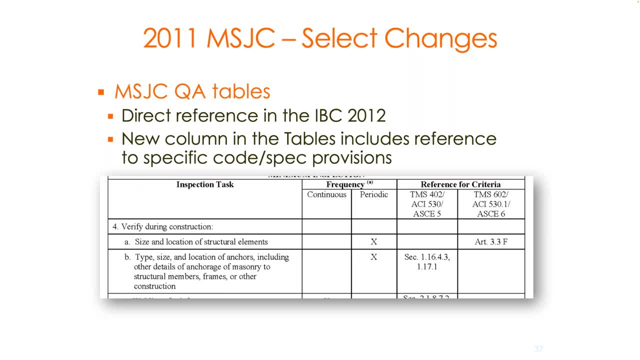 the code writer is giving more and more attention to that material as well, QA tables being added. certainly that's going to be more helpful as we get into having better and better reviewing of masonry design and hopefully helping more and more confidence in design. 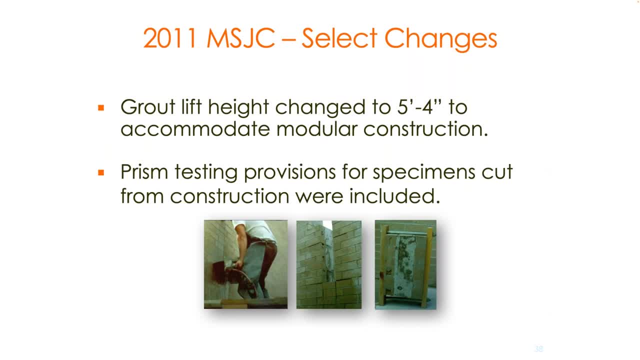 Just some very straightforward changes. grout height lift changed to five foot four. So anytime that we're writing a limitation for low lift grouting we have to make sure that we Reference that it's five foot. why five foot four instead of five foot? because five foot. 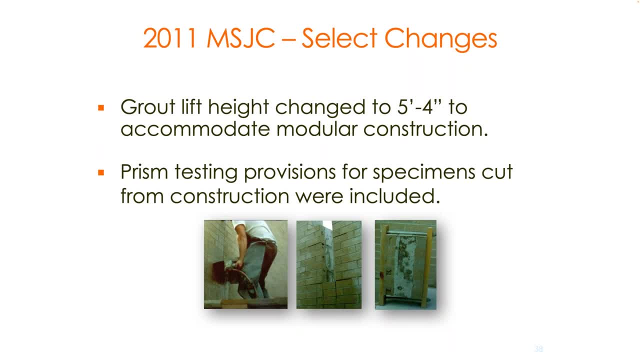 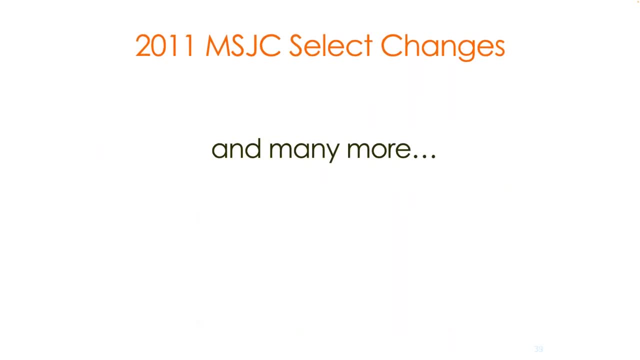 four is coursing. So instead of penalizing people and having them at four foot eight, then five foot four was certainly a more and more sense. So there's certainly more changes than that, but that was some of the highlights from the 2011, 2013 code. 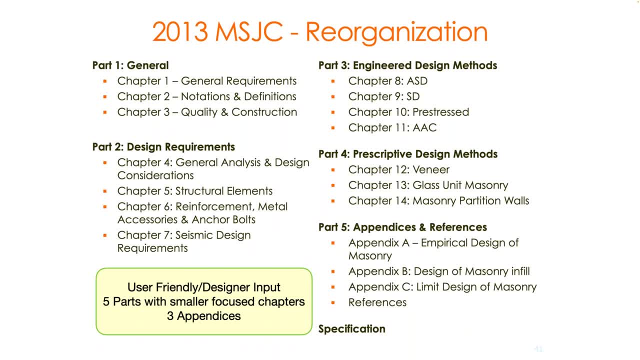 The major thing in 2013 is there's a pretty big reorganization of the code. If anybody had the 2011 code or used 2011 code, you see the 2013,, 16 and 22 or so They're organized a lot different, trying to break apart the code in different ways. 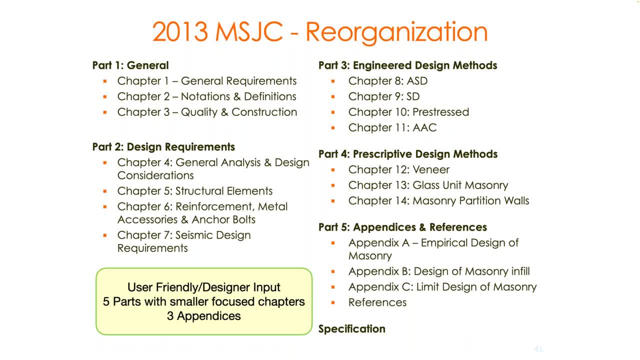 so that it makes a little bit more sense to general requirements. design requirements, engineered methods, ASD, strength design, pre-stressed and then AAC, all being different engineered methods. prescriptive methods for veneer glass unit masonry. masonry partition walls. 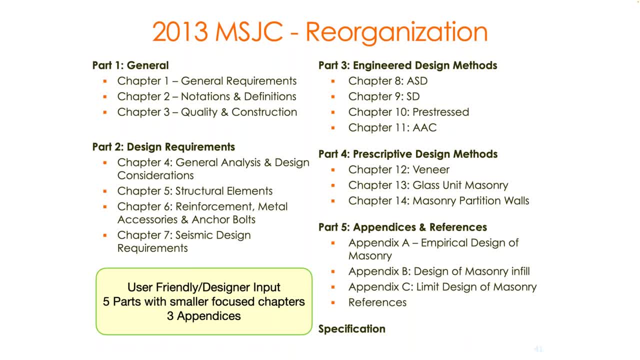 all different options that are added to the code, And then you can see some appendices that are added in there. Sometimes appendices are interesting: the stuff that's moving out of the code, like Appendix, A empirical design that's getting further and further out of the code. and then 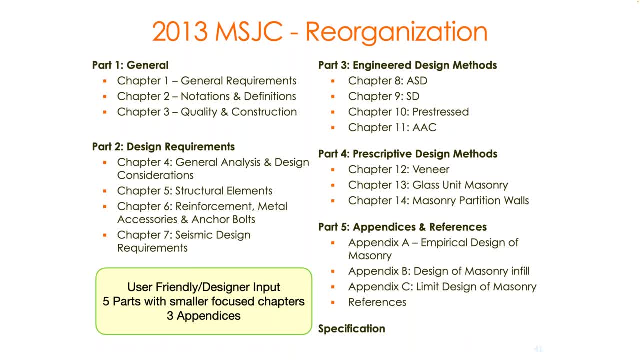 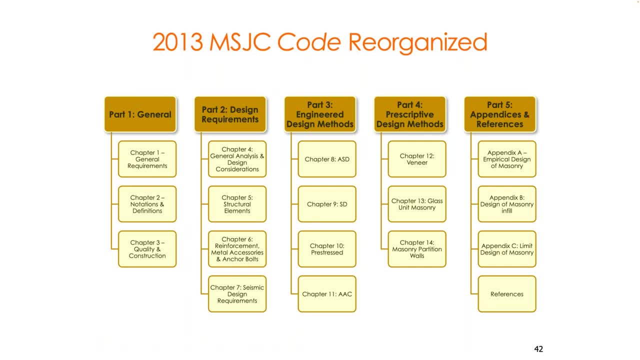 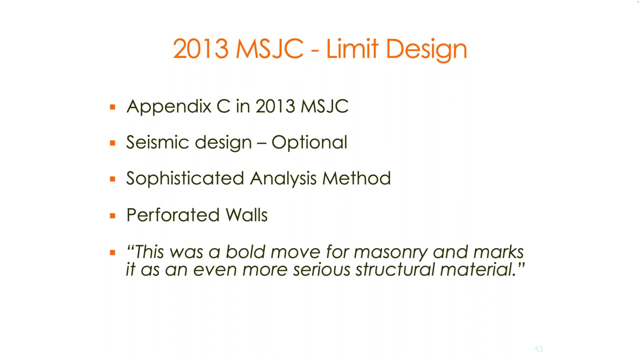 you have new things like design of infills or limit design of masonry being placed in appendices. So a little bit of a different look at kind of what the organization looks like. So 2013, again, it still references MSJC 2013 masonry code. we have Appendix C where 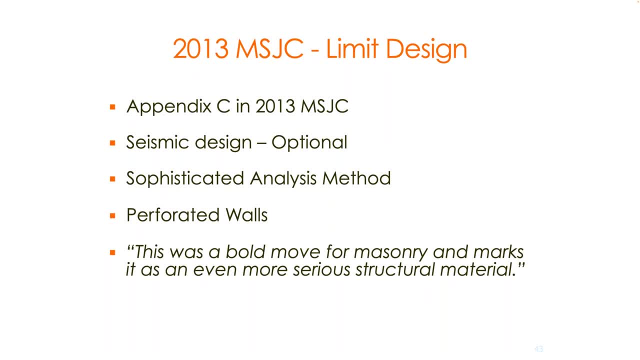 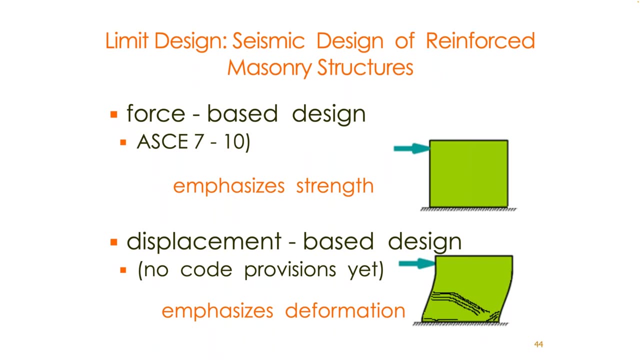 we add a limit design. it's a seismic design, optional. it's a sophisticated analysis method that certainly, I think, helps designers get a little bit more capacity out of their masonry designs Again. so limit design requirements for reinforced masonry structures in forest-based design. 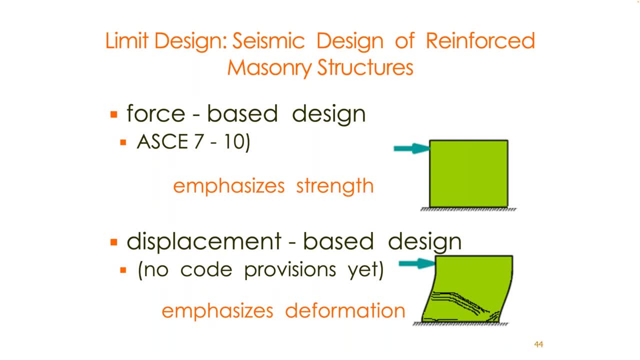 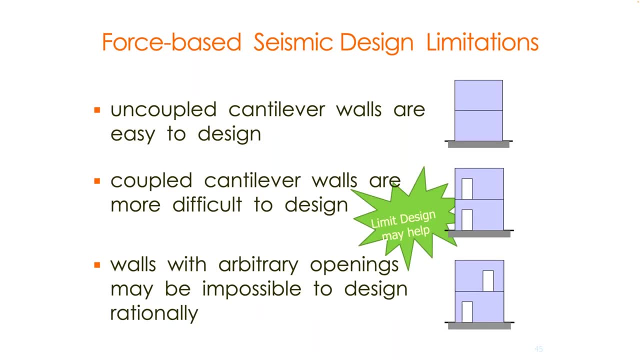 AAC 710 emphasizes strength. displacement design. emphasizes deformation, forest-based seismic design limitations. uncoupled cantilever walls are easy to design. coupled cantilever walls are more difficult to design. I think some of this stuff also comes into play as the more and more that we use software. 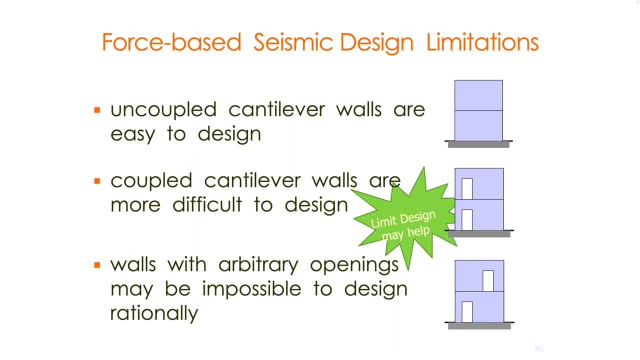 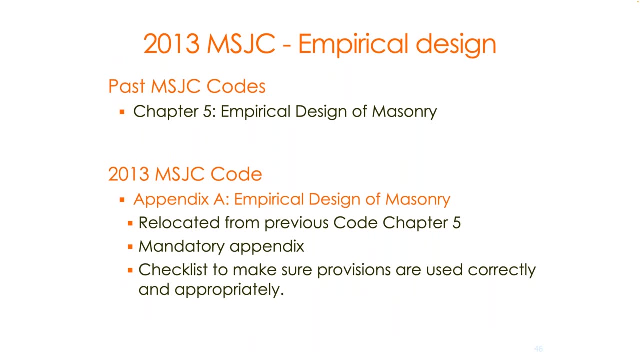 and software provisions. We have more options for looking at coupled walls or perforated shear walls. We have a lot more options that are being given there For empirical design. empirical design of mainstream 2013 appendix is going to be where the empirical design is now going to sit. 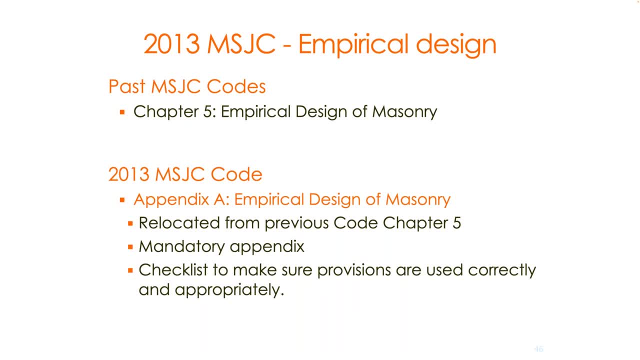 Maybe it's going to hang around for a little while. Like I said, it's definitely something that we should be moving away from and more into the more allowable stress design or strength design provisions, Things that can be maybe looked at as more like an empirical design partition walls. 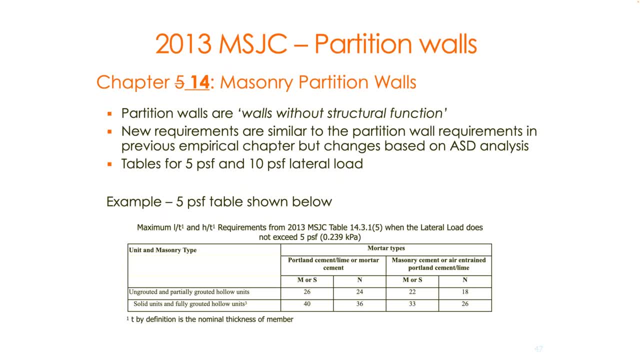 where you really do have pretty hard guides for what are the loads for an element, what are the different sizes of the elements. That's where partition wall chapter being added, not being part of the empirical design chapter but really being its own chapter itself. 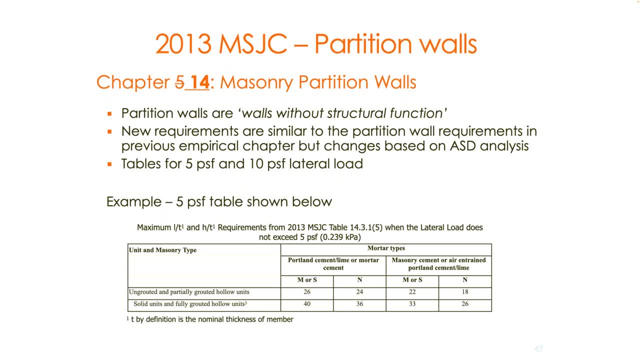 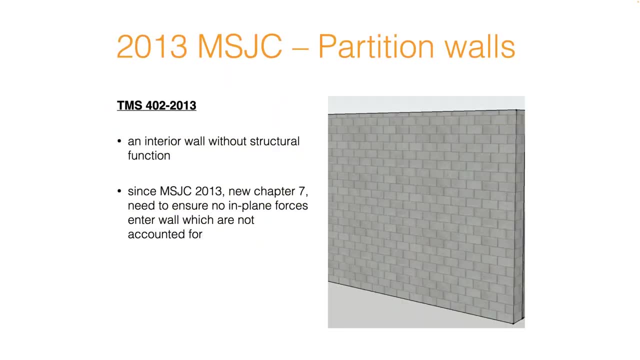 Tables for five pounds per square foot, 10 pounds per square foot. Just you see an example of what we have there. Just a little bit more about partition walls. Really, partition walls are an interior wall without structural function. They're really in there as dividing, demising wall to separate spaces. 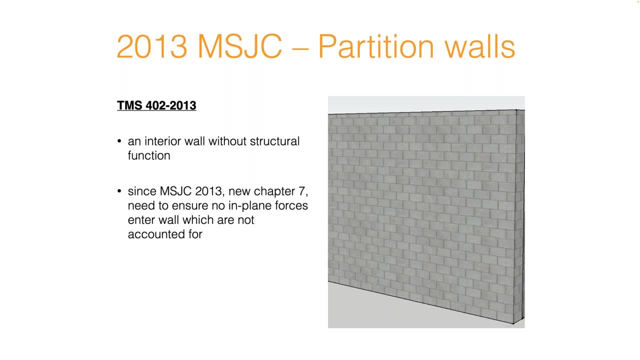 In the code in 2013,. it really did give it its new chapter. but then it also talks about how there's really no form, There's no forces that should be applied to a masonry partition wall that are not intended. Slipped connections at the top, no connections at the ends, really do help partition walls. 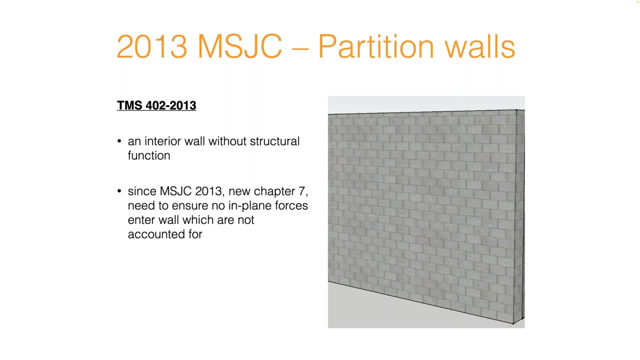 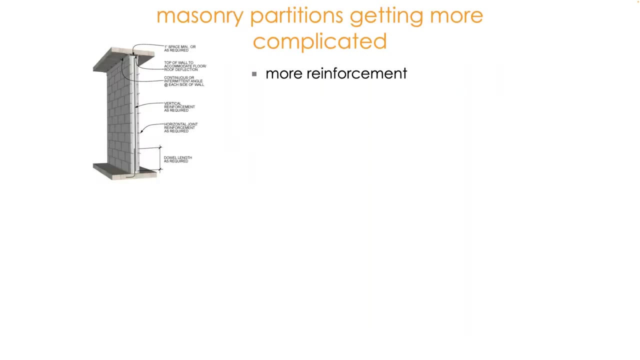 not see a lot of loads. This is important, I think, in the masonry world, because if we look at making sure that we have efficient designs, we want to make sure that we don't have any unintended forces, so that we can make these walls as simple as possible. 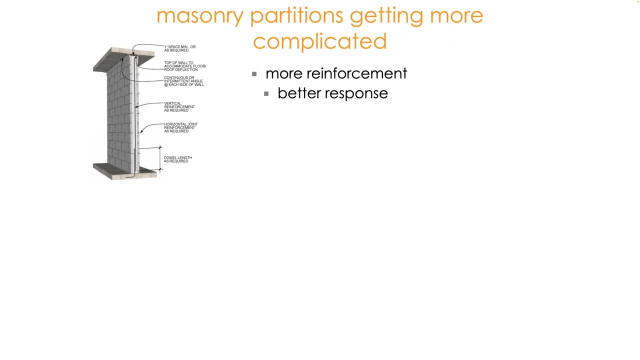 If they have more reinforcement There's, It's going to be a little bit better response, but it's going to be more costly. So making sure that we don't put too much in there. Smarter connections: We don't want an unintended loads. 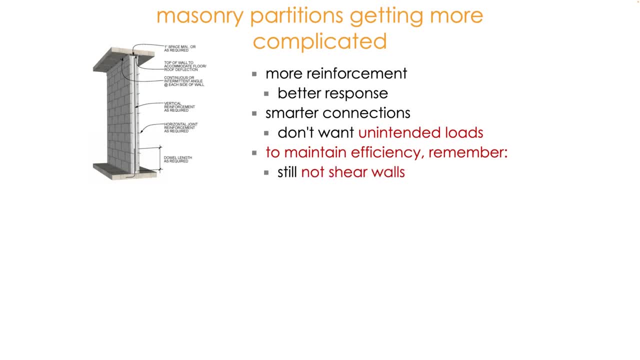 We want to maintain efficiency, though We want to make sure that we don't design them as sheer walls. If we do design them as sheer walls then it's going to get very expensive very quickly. Less grout equals less weight. Studies show a significant cost related to partition walls when more grout reinforcement 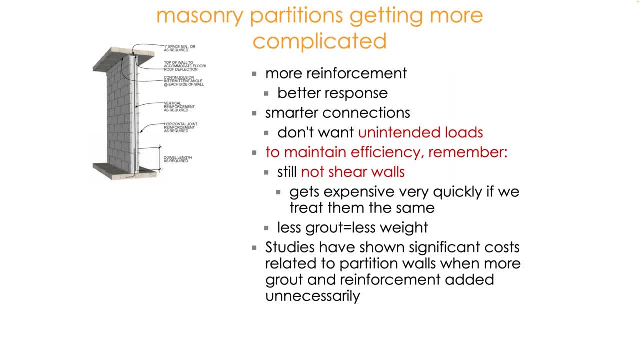 headed on this. really, Really, what we're looking at There is, you know, I talk about partition walls in the sense because you know we have mainstream partition walls that sometimes will get valued, engineered out of a project, And that can be unfortunate because sometimes those partition walls were not as efficient. 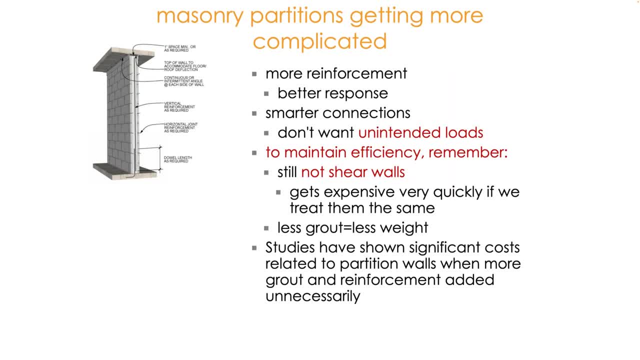 as possible. So really what I try to get people to look at partition walls as well. yes, if we had enough money and we had all the different options, we want to make the partition walls Maybe a little bit stronger, maybe be a little bit conservative. 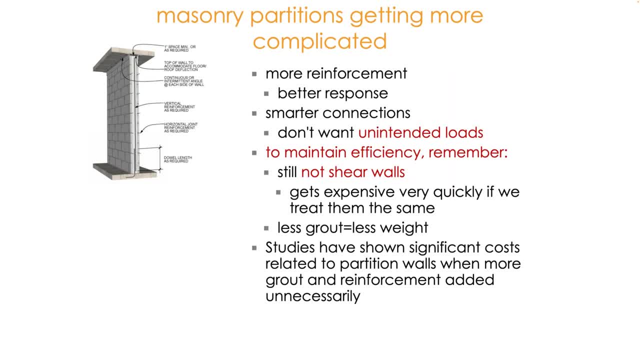 But we don't want to value engineer out a conservative partition wall for a stud wall with chipboard on each side. I mean, why not go to the most efficient partition wall as your value engineering option? So that, for me, is always the important step to take. 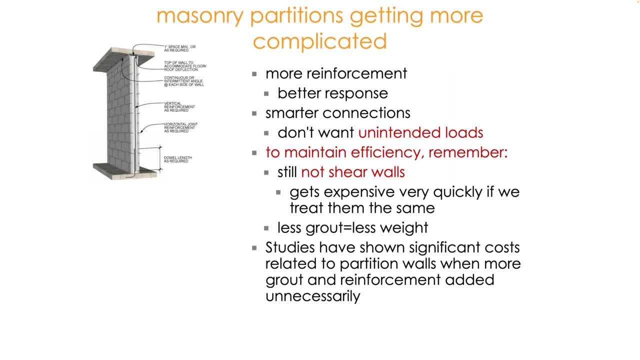 Make sure that we make partition walls as efficient as possible before we start valuing engineering things out. Looking at different seismic design characteristics that are in the code: You know. looking at different seismic design characteristics that are in the code: You know. looking at different seismic design characteristics that are in the code. 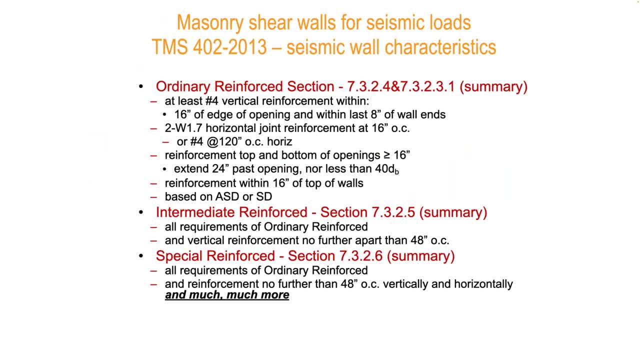 You know there's some really important ones that are in there. Reinforcement within the top of the walls- That's the second one from the bottom of the ordinary reinforced walls. That's a seismic requirement for a seismic shear wall. That's not something that we need for partition walls. 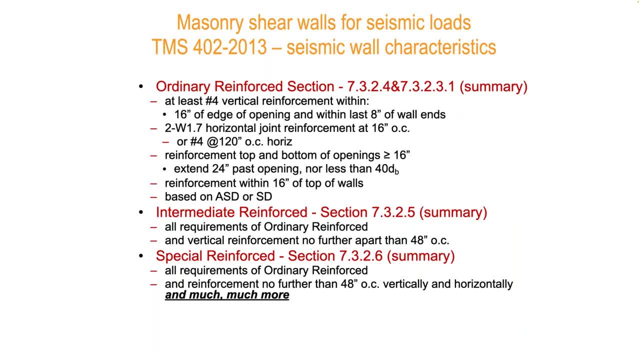 And then in the intermediate reinforced vertical reinforcement no further than 48, that provision is also for an intermediate reinforced wall. There's nothing in a main street wall that requires reinforcement to be at 48.. There's nothing in a main street wall that requires reinforcement to be at 48 inches on center. 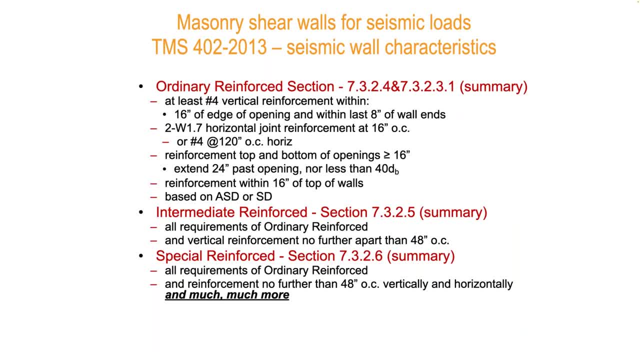 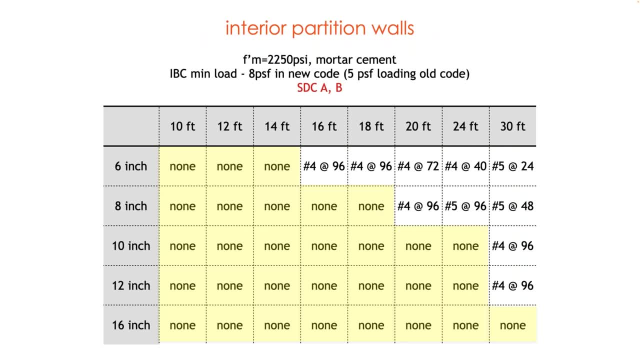 There's nothing in a main street wall that requires reinforcement to be at 48 inches on center, So we take some of that stuff into account, like recognizing these are shear walls, shear wall provisions. I can recognize that I really don't need a ton of reinforcement within partition walls. 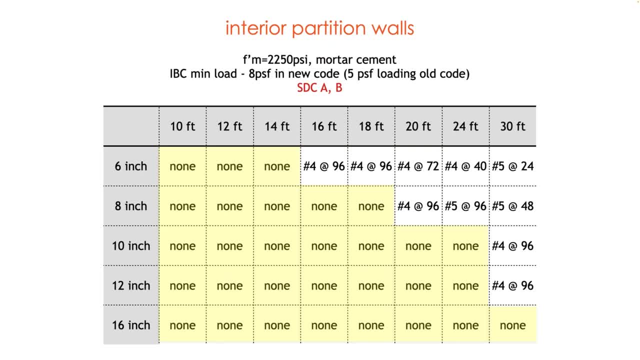 And so the code is going to give us, you know, some tables. We could also create our own tables where we have a lot of partition walls that can still be unreinforced. Seismic design- categories A and B- really do allow a partition walls to be relatively 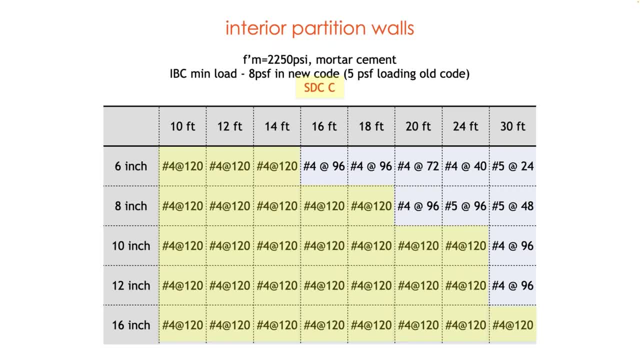 unreinforced. We get into seismic design, category C. we need some reinforcement. We still have many different partition walls and thicknesses that can be very lightly reinforced, And so that's going to be our efficient main street partition walls: making sure that we 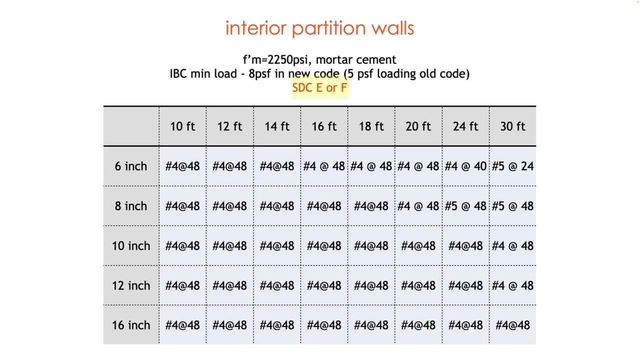 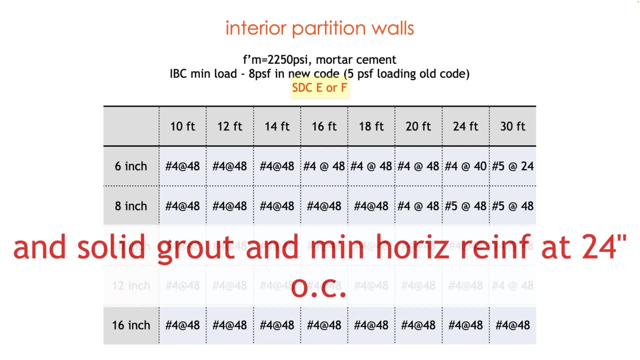 utilize those. We get into higher seismic design categories and more reinforcement is going to be needed and added, And certainly we need to go there because we're in a seismic area, but we want to be as efficient as possible in those places as well. 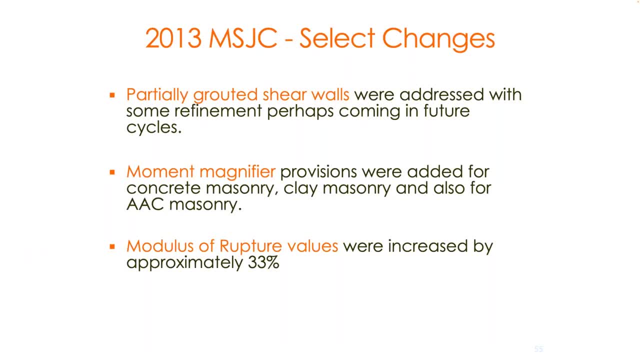 Okay, Thank you. In 2013, we have partially grouted shear walls that were addressed in some refinement coming in the future. Moment magnifiers modulus of rupture values were increased by approximately 33% again to help with some of the unreinforced masonry capacities. 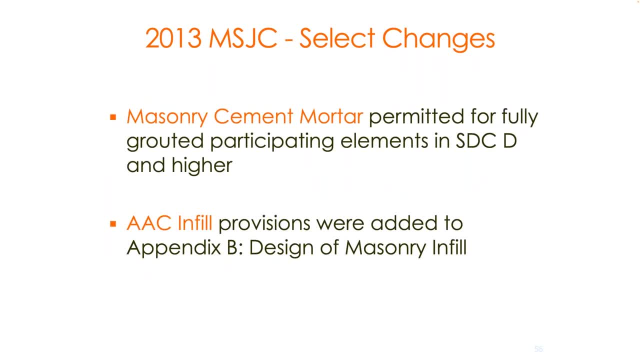 Masonry cement: Okay, Okay, Masonry cement mortar permitted for fully grouted. just a little bit of bookkeeping there. AAC infill provisions were added to Appendix B, design of masonry infill, AAC again being something that is. 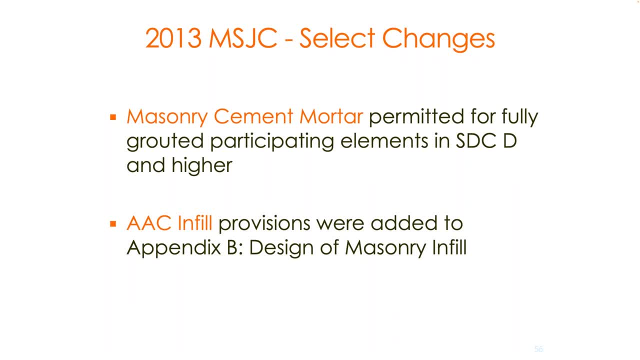 Hey, Sam, are you there? Yeah, I'm here. Yep, Can you hear me? It seems that your audio may be stopped here. I can't There you go. Can you hear me, Andrew? Yeah, Okay, Let me see. 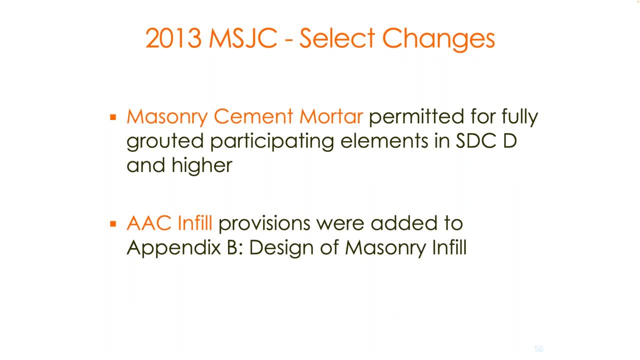 It looks like it's. I don't know If anyone else can still hear them. maybe they could say something in the chat. It could be my microphone, but I- Okay, Sounds like it's just me. I'll check my stuff. 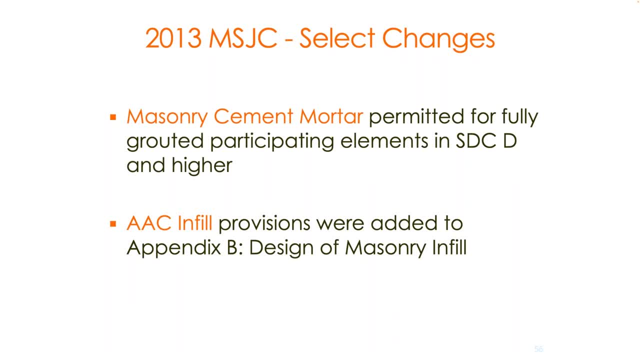 Okay, Sounds good. Yeah, If anybody can't. if you guys want to pop in and do any chat or questions, glad to see everybody can hear. okay, Let me see Other things that were in the 2013.. Yeah, Yeah. 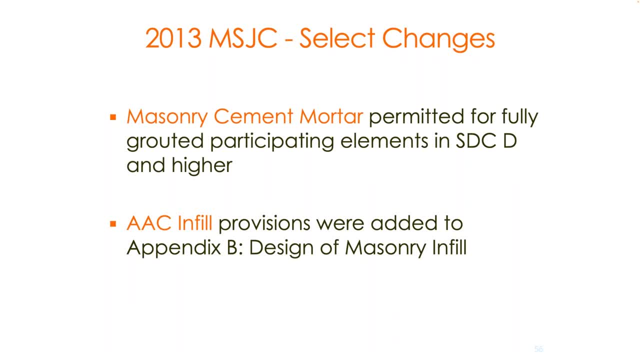 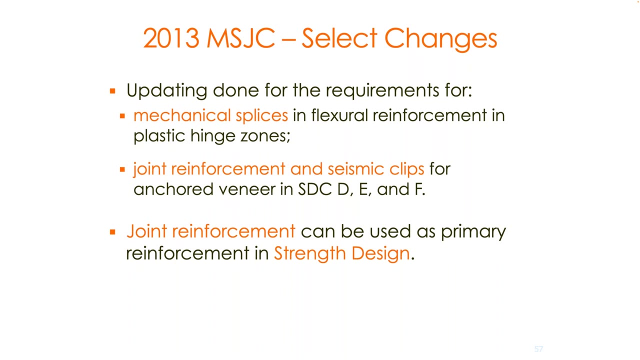 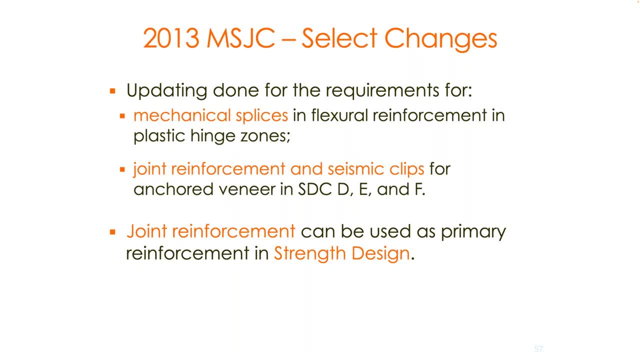 Joint reinforcement: seismic clips for inker, veneer And joint reinforcement can be used as primary reinforcement in the shrink design- Again, very, very helpful. Joint reinforcement is pretty common, pretty easy to add. It's gonna be something that we can很 often use. 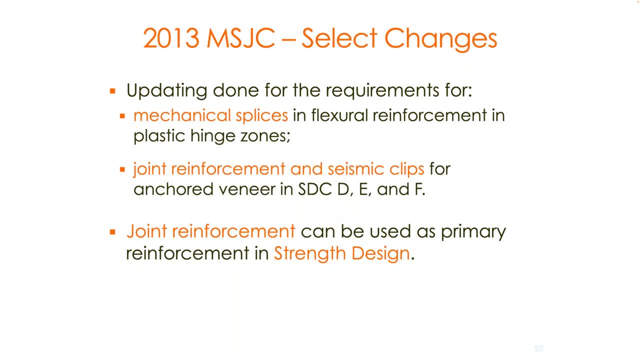 going to be something that we can get into those mortar bed joints and that can be very, very useful, so we'll cover that more. we'll get into the material section a little bit, one of the big things that happened in 2013 code and something that we can talk more and. 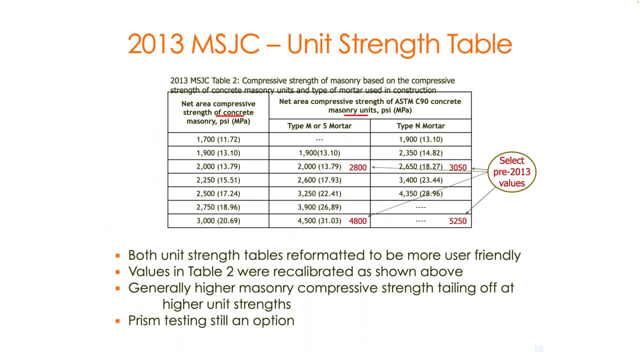 more about is there was a kind of recalibration on the overall strength of masonry, and this is something that's really, really important. we get into the design capacities of masonry. prior to the 2013 code, we had a lot of people designing to lower strengths for masonry. 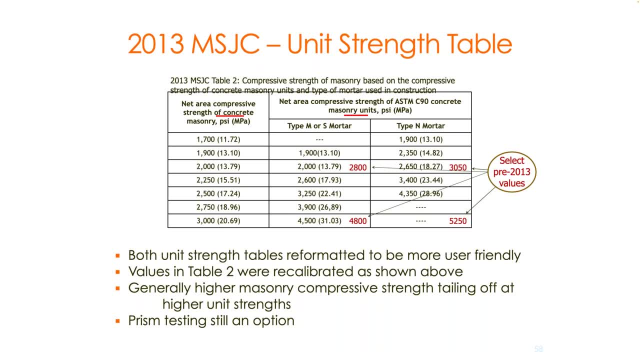 and so really a lot of that stuff was based on old test data that really kind of pointed to masonry taking a little bit of a hit when we took our units and we put them in mortar. really, what we found in kind of that recalibration is that really the block strengths. 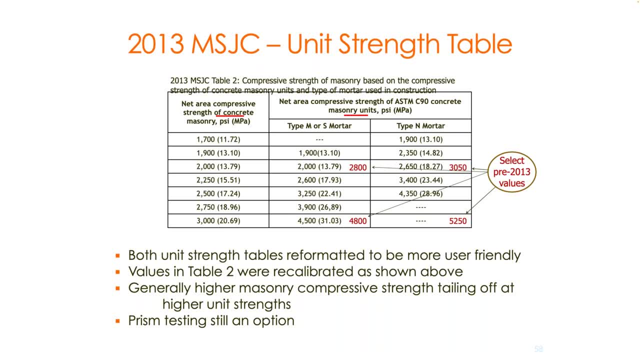 we're going to be the same as the design strengths or the lower end values of mainstream. so what i mean by that is, if i looked at the third- uh, the third- row up here in my table, the 2000 psi strength of mainstream, the far left column- all i would need is a 2000 psi. 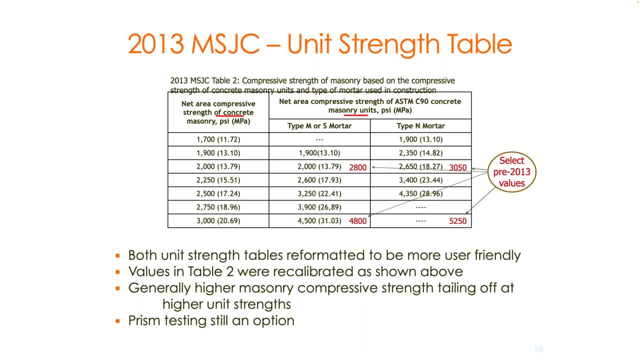 block strength with type mrs mortar. that's the second column. i have type mrs, i have 2000 psi block strength, then i can have my 2000 psi design strength. so there's no hit. there's no. i'm going to reduce the strength of the overall mainstream wall based on putting those blocks in. 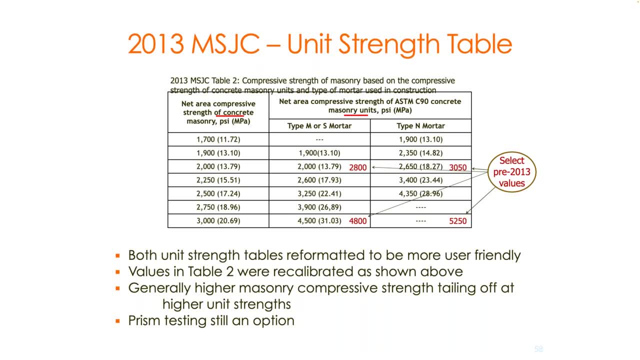 mortar prior to to 2013, i would need to have a block strength of 2800, so you can see those 2013 values shown up there. i had to have a block strength of 2800 uh in type s mortar to have a design strength of 2000.. so, again, very, very significant. um, it really does kind of put the. 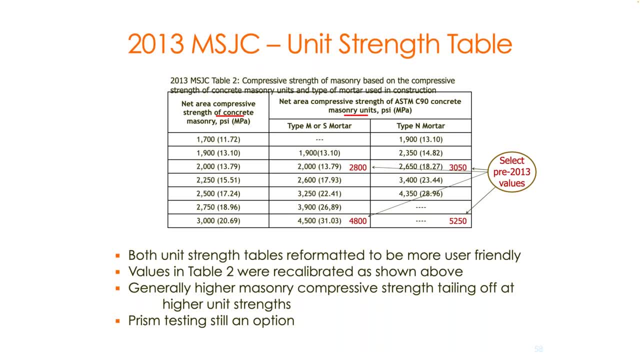 the floor on designs. actually at 2000. now you can see some revisions in the code, but certainly anything that was um, um. you know block strengths are had always been at 1900, so you can see 1900 to 1900. what they did was just eliminate that the uh current, current esdm are putting out. 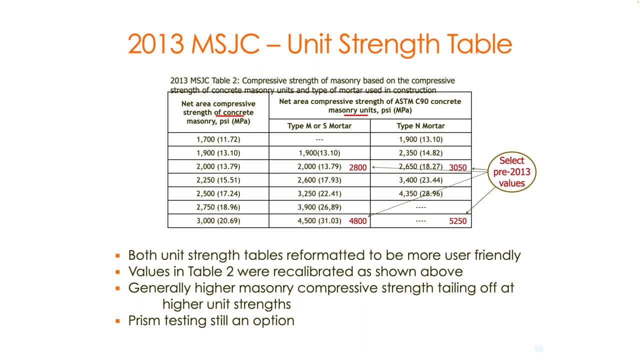 block strengths at 2000 is the minimum block strength. with that block in type s mortar we can have a design strength now at 2000.. so that's really a 33 increase in the typical uh minimum values that are used in design, and then achieving a meeting higher design strength has gotten easier. 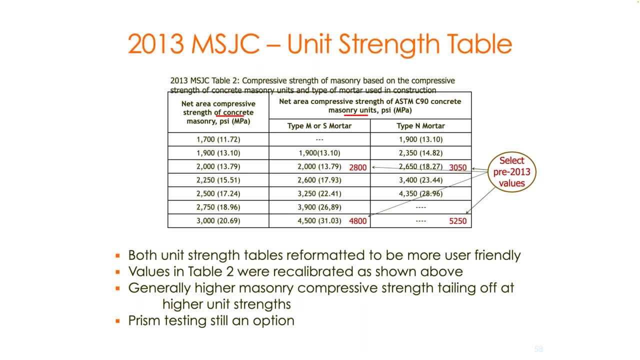 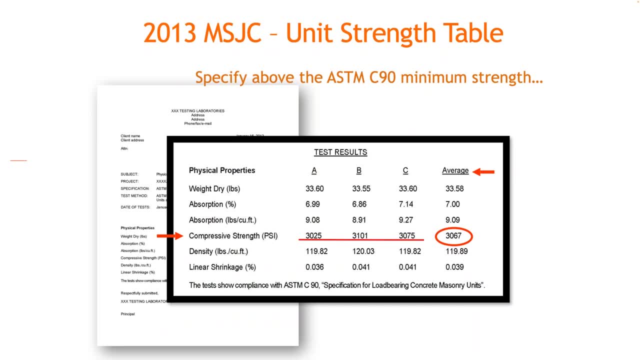 as well. um, so that that's going to be something that's pretty important. uh, for design. so, um, um, something that's really cool. we saw the uh 400 block for the early days. uh, there's an instance where people were actually using um- the block strength, but the block strength was. 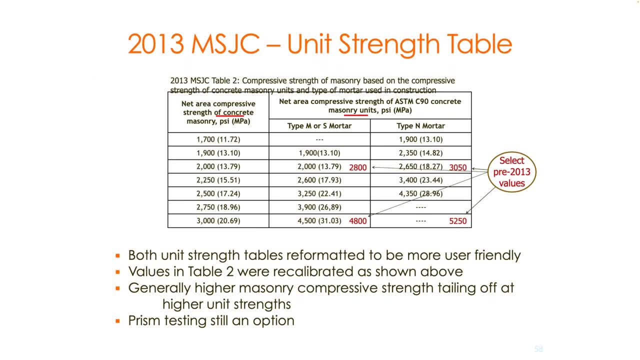 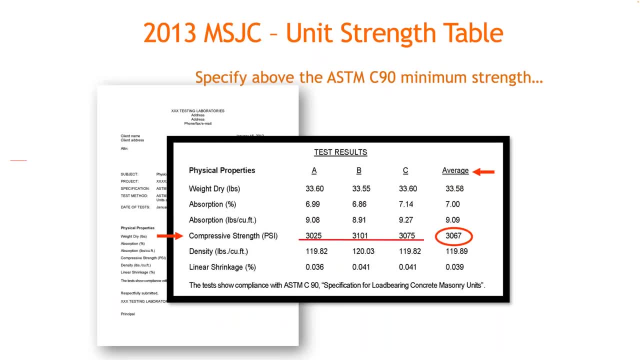 in the first place. so that's really looking at. uh, something that we've been seeing the uptick on um in the last couple years is that, uh, a lot of these blocks, the block strength are very high. uh, yeah, the block strength has been higher, but the block strength just doesn't. 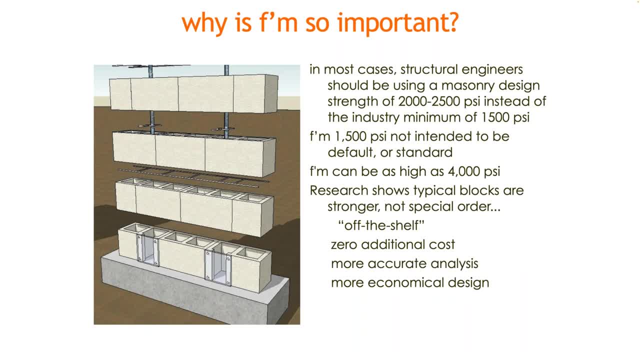 lower end of masonry, the 1500 as a default or standard strength of masonry, can be a lot higher. it can be as high as four thousand. in fact, we don't have to stop at two thousand now either. we can certainly keep going higher. really, the point is making sure that you understand. 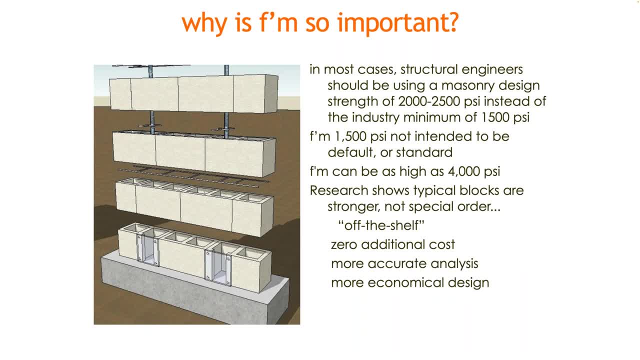 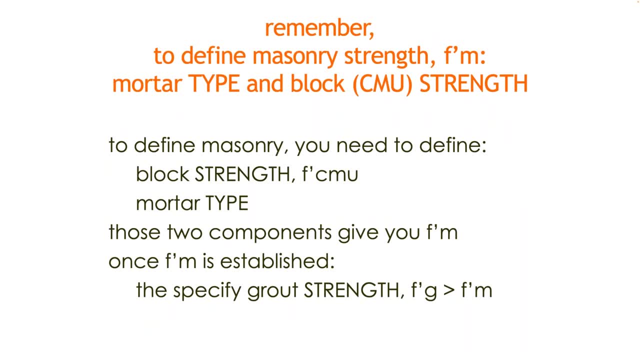 what the actual block strength are and then you can figure out what the overall design strength is. you know, for masonry, the two elements that you need to define the overall strength is the block strength in the mortar type. once you have those two components, then that gives you your strength, your f, prime, m, and then, once that's defined, then we actually 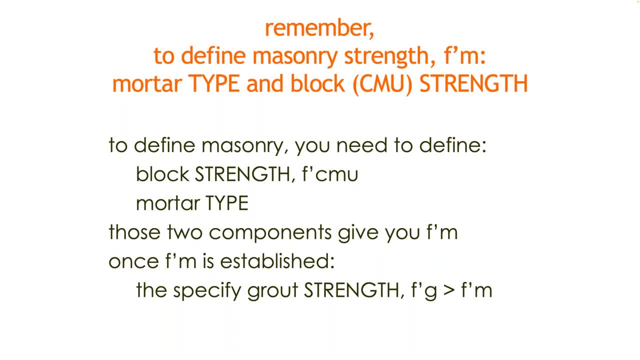 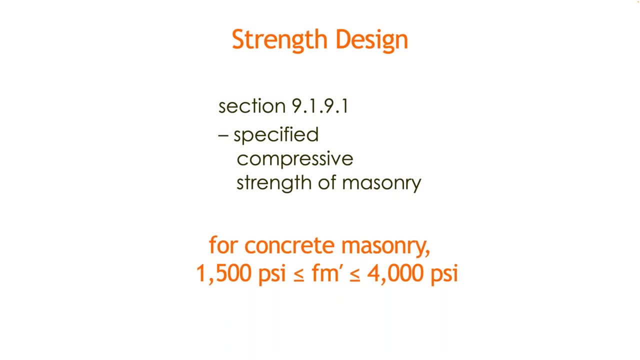 define the grout based on the other two elements that are there. strength design in the code gave us a range of 1500 to 4000. again, we can go up to 4000. we can move all the way up to that. what we do is we just ask for higher and higher strength. 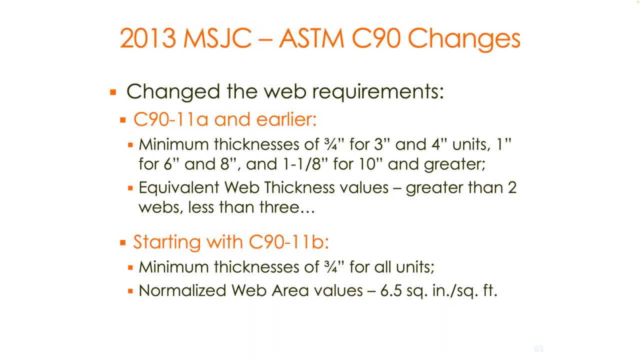 of blocks to be able to achieve that. other things that changed in ASTM: minimum thicknesses for units changed and that is going to give a lot better units for having better thermal performance if we can reduce the amount of grout and reinforcement masonry walls and we 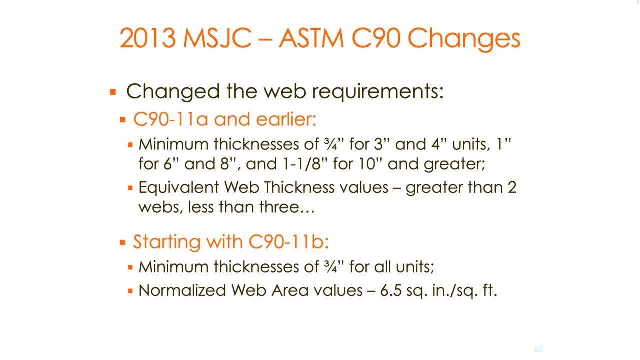 have relatively thin web elements when we have a lot smaller areas that are going to be creating these thermal bridges. so that's going to be something that was motivating the ASTM, the different code writers, to allow for smaller and smaller masonry elements so that those elements can then be have a lot better thermal performance. and so we can see. 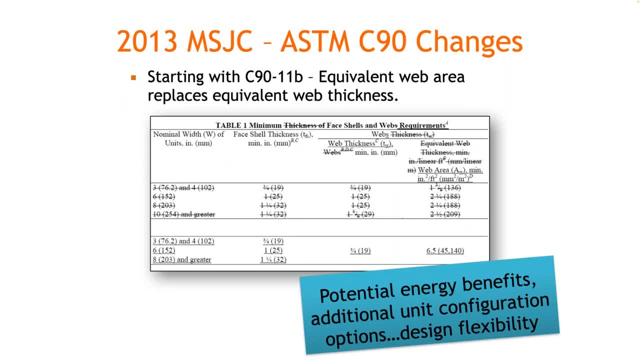 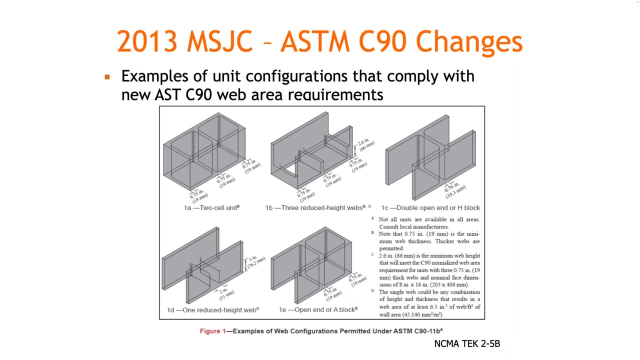 some of those changes as well. so within the table we have, you know, some of these different thicknesses and requirements changed in ASTM C90 and then from that we have a lot of different types of blocks that are created in the web. like I said, the primary elements there is going to be your web thicknesses that we're looking at for. 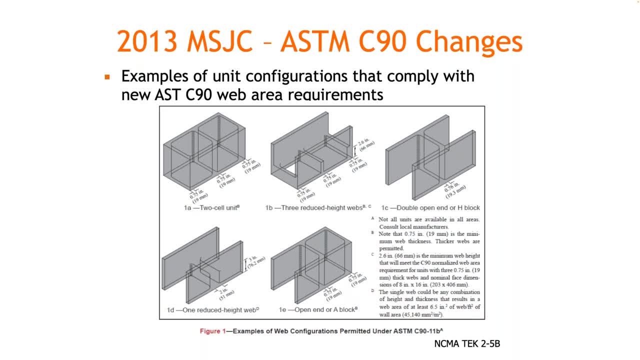 the different types of blocks that we have, whether it's a standard two-cell or it's a bond beam block or an H block. I mean that actually can have pretty, pretty minimal webs and eight blocks or something like that, going to be a block that we're going to be used when we have more grout and reinforcement. so 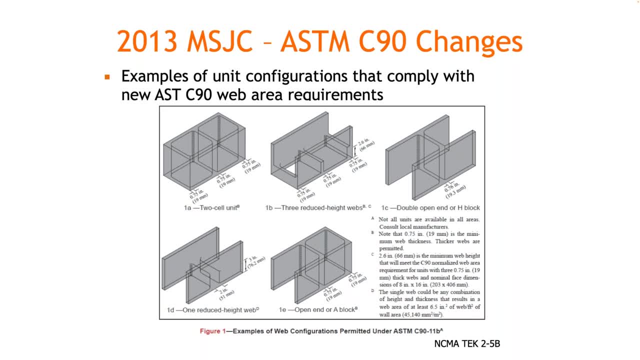 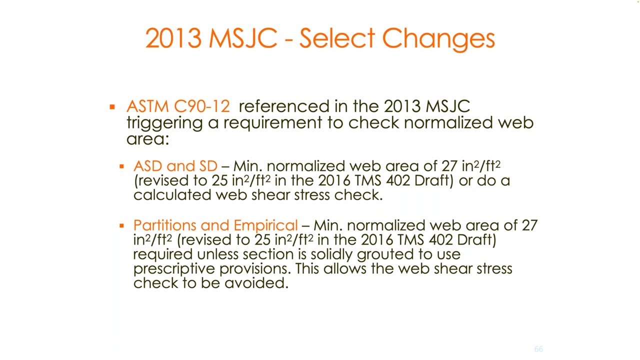 having a minimal web there maybe isn't super critical, but if it's an a-shaped block- there's some of the different blocks- can certainly have plenty of benefits in having a minimal web area. more and more on the changes and in some of the block requirements, partitions and empirical 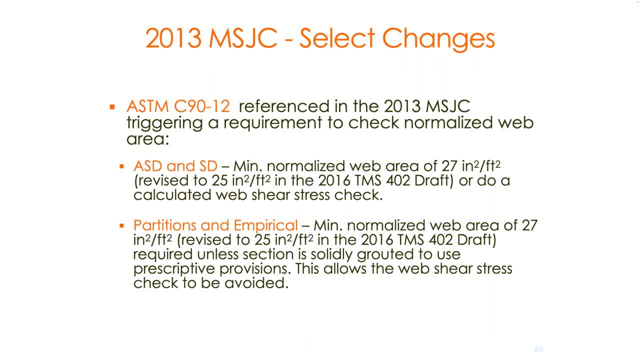 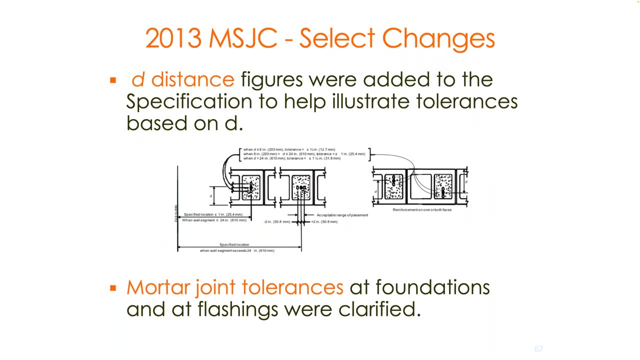 minimal normalized web area required, unless section is solidly grounded, to be used for prescriptive provisions allows the web shear stress to be avoided. other things that I think are really important in some of the clarifications that were made in a 2013 code. I really, really, really like these little images and guides that were. 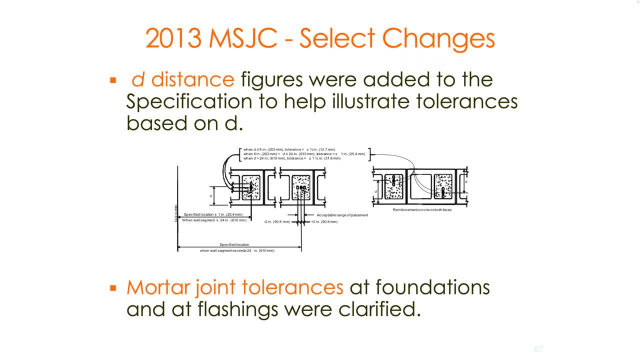 created. what this does is it helps designers see what the tolerances are for bar placement. the number of times that I've had people ask and have questions or have heartburn over bars not being exactly in the center of a grout itself, well, here the images really do give good, clear, clear. 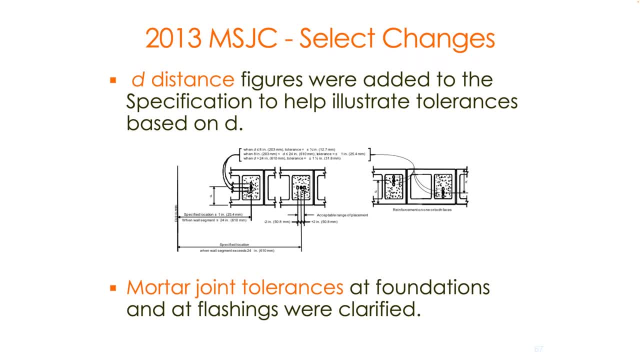 direction to the bar placement, and I think it's really important to have that in mind when you're doing a bar placement. and you're doing a bar placement and you're doing a bar placement and designers and contractors is to what the tolerances are. so, tolerances that are for the reinforcement. 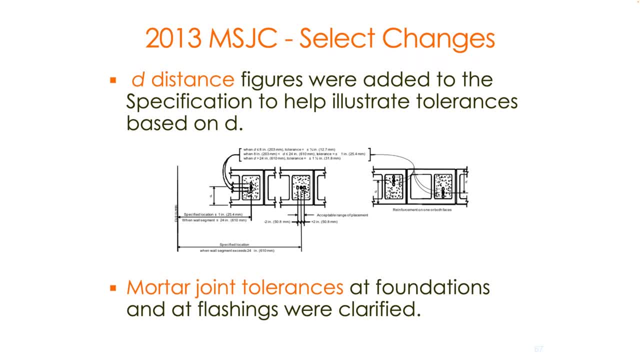 if the bar is not quite on center. we do have plus or minus an inch that you can have for the bar when you have like a 12 inch wall. if you have an 8 inch wall, you can have plus or minus a half inch, but that's a that's a huge number to be able to see. I still have plenty of capacity. 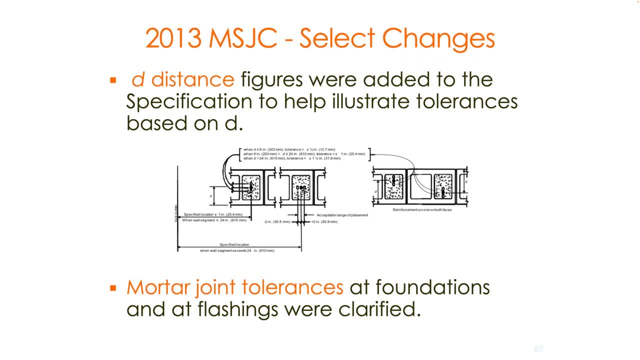 With a 12-inch wall. if my bar is a little bit off-center, if it's one inch off-center, that can be really, really helpful for designers to see that, to know that your wall is still going to have adequate capacity. 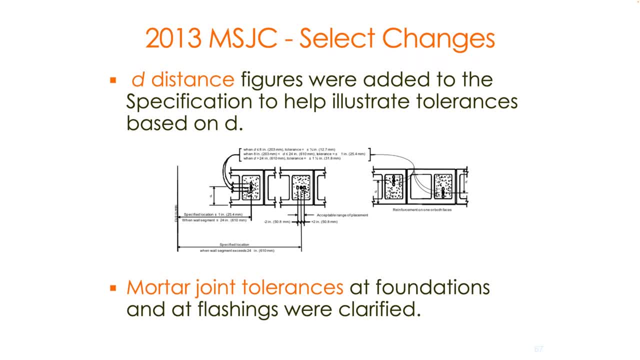 Your bar can be plus or minus two inches along the length of the wall. Again, very, very helpful when we look at the overall design of masonry and construction of masonry as we go ahead and review things on site, giving you more confidence in the overall design of masonry. 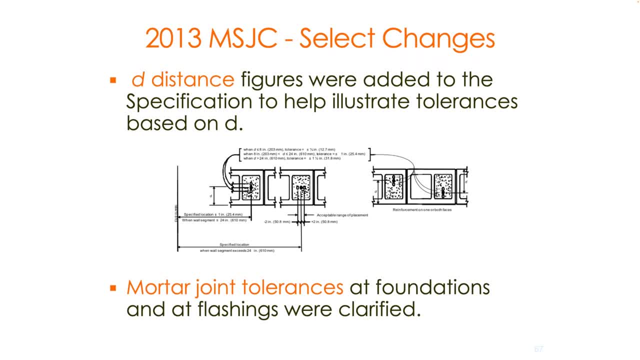 So knowing again, tolerances are for knowing that you still have the capacity. even if the bar isn't exactly where you detailed it, It does have some tolerance in terms of where it can go and your capacities are still going to be okay. 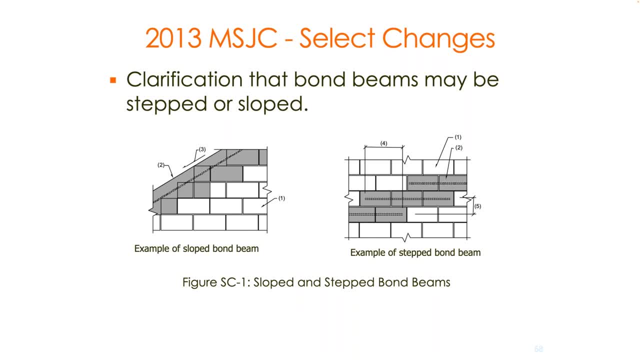 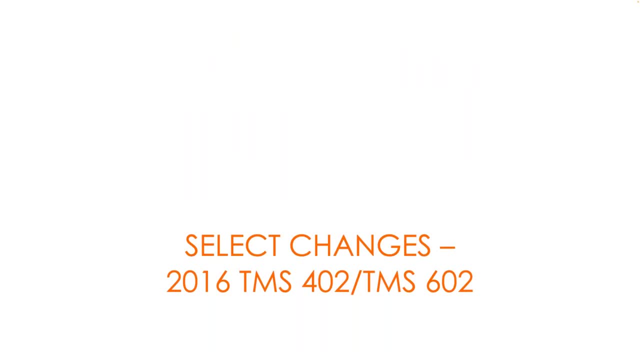 Step bond beams. just some details in terms of how we can step bond beams, So it's nice to have some of those details added as well. and then more and more changes. So, getting into 2016,, something that's more and more current. 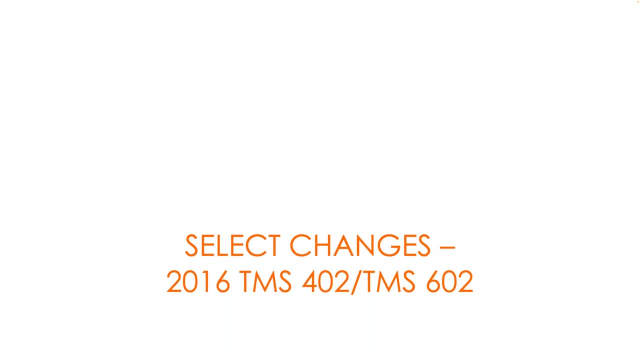 There were some really big changes there in 2011 and 2013.. I did want to kind of brush over it just because I think there's a lot of people that are still designed to some of the early provisions pre-2011.. 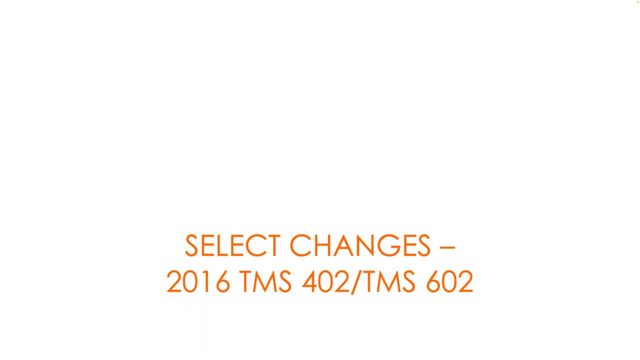 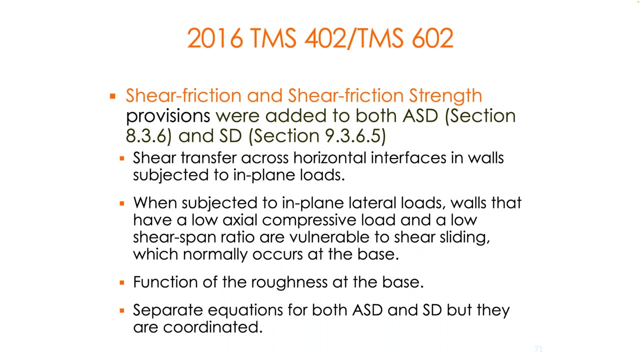 So covering some of the stuff that was covered in those two codes I think was really important 2016,. some of the highlights are going to be: shear friction: shear friction strength provisions were added to both ASD and strength design. shear transfer across horizontal interfaces. 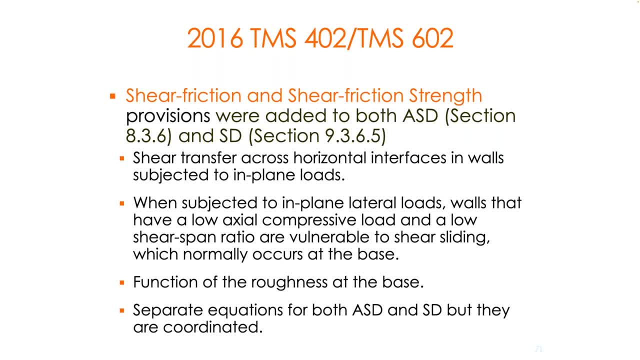 And wall subject to in-plane loads. Subject to in-plane lateral loads. walls that have a low axial compressive load and a low shear span ratio are vulnerable to shear sliding, which normally occurs at the base Function of the roughness of the base. you know all of the different things being added and confirmed in the 2016 code. 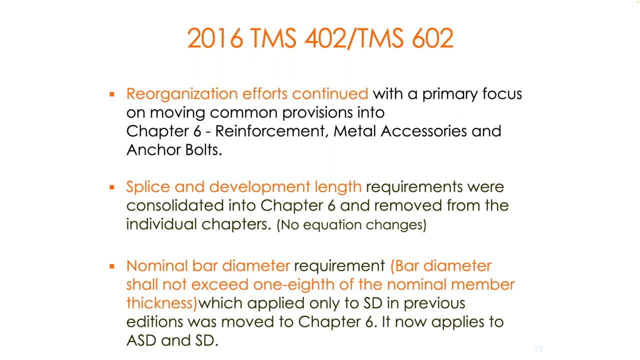 Other things. reorganization efforts continued Moving common provisions into Chapter 6.. 6 reinforcement, you know, accessories and bolts and stuff like that, all that stuff being added to Chapter 6 as well, into the design chapter. Splice and development length requirements were put into Chapter 6 and removed from individual. 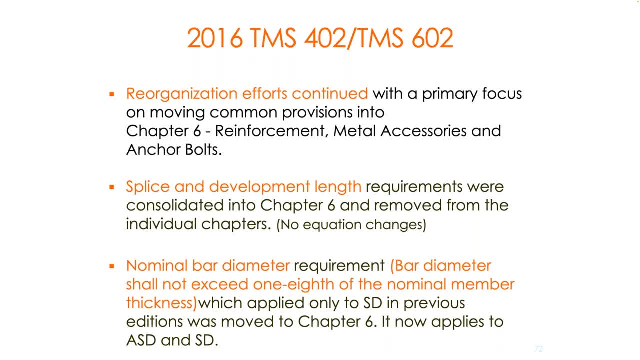 chapters- which is nice, you know, the more and more clear that it can be. Let me see nominal bar diameter requirements. bar diameter should not exceed one-eighth of the nominal member thickness. That could be really helpful in terms of understanding. you know, masonry having confined spaces. 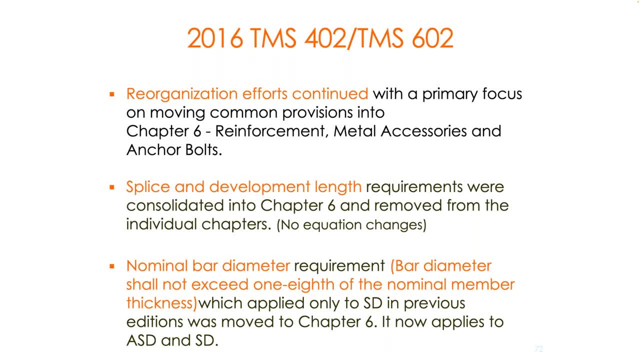 What the code writers are trying to do there is prevent really big bars from being added to really thin walls. Obviously that's not going to make a lot of sense, so it's just trying to give some guidelines to the overall maximum reinforcement that would be added to walls. 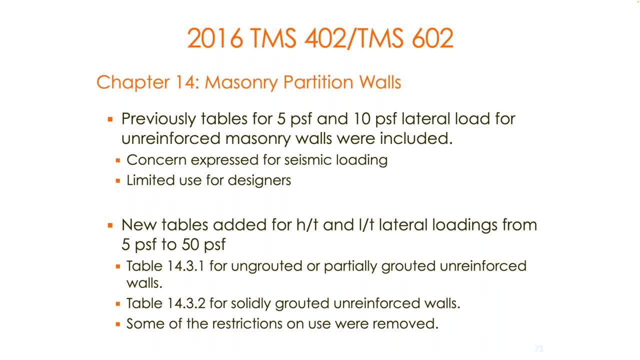 2016,. previous changes: Tables for 5 and 10 for unreinforced masonry walls were included. Concern expressed for seismic loading. limited use for designers. New tables have height to thickness and length to thickness. lateral loadings for 5 to 50. 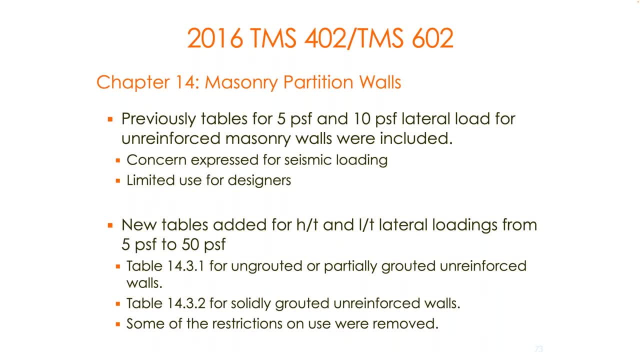 PSF, So kind of trying to expand upon some of the different loads. I mean you have all kinds of different types of buildings and structures and different loads that you maybe have. So some of the different tables Just as an example, Okay. 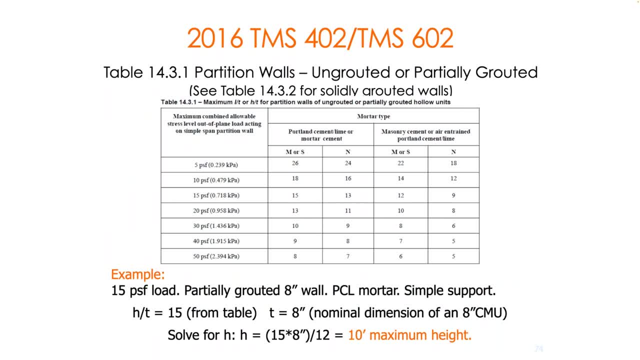 So, for example, in the new code, giving you the different pressures from 5 to 50 and then giving you again the LT or height to thickness ratio for ungrounded walls, really is going to be able to give us a pretty clear definition in terms of what we can do design-wise. 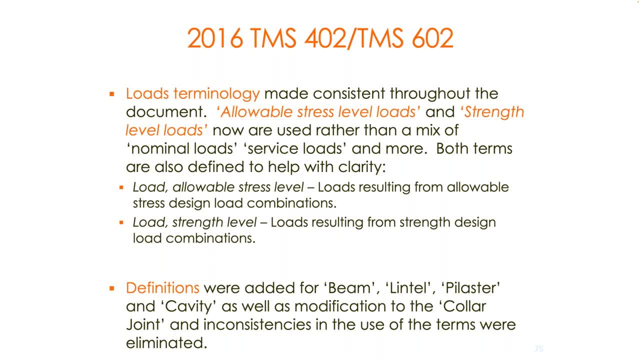 Load terminology, Make it more consistent. Obviously that's better of all the stress level loads, strength level loads. So just a little bit of clarity there. Definitions were added for beam, lintel, pilaster and cavity, As well as modification for collar joints. 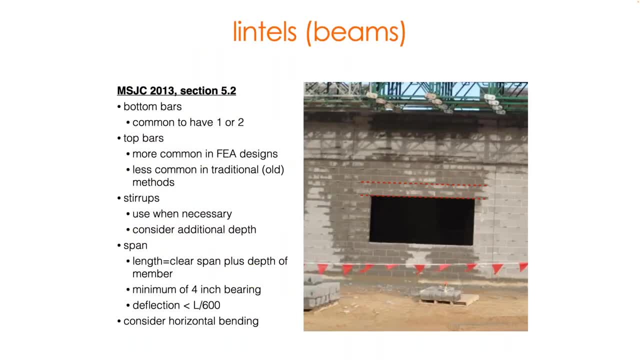 So just trying to help clarify some of those things, Just kind of pointing out some of the different elements that we have here, Lintels beams are really going to be, you know, the area that's going to be spanning and opening. 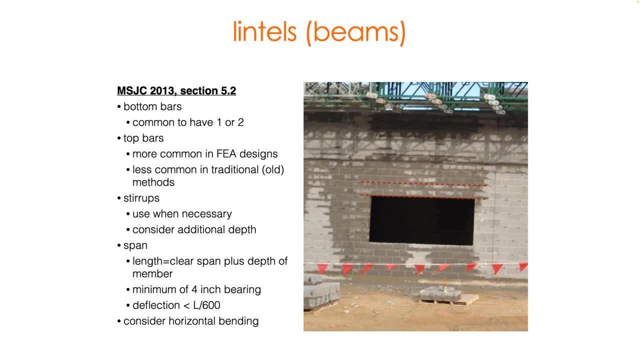 It's going to be the length, the clear span plus the depth of the member. Minimum four-inch bearing Deflection limited to L over 600.. Consider horizontal bending. You know, the thing with lintels is pretty common to have bottom bars. 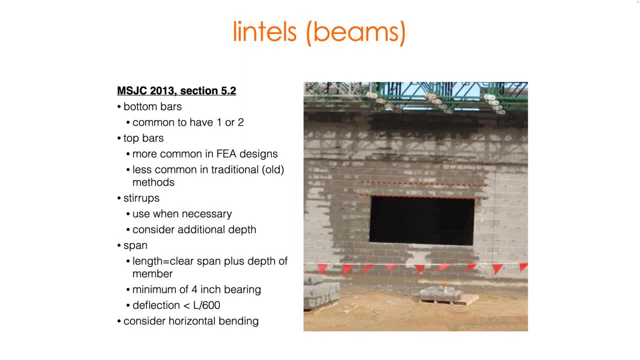 Top bars are, I think, things that we should be considering for lintel design. Again, it's the top of the lintel but it's, you know, well within the space of the wall itself. You know, If we're looking at horizontal bending, especially making sure that you have some balance. 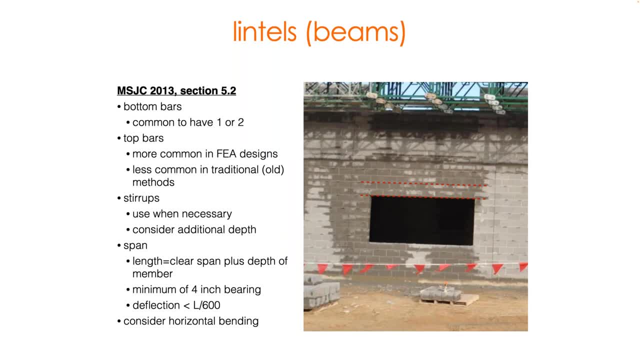 in this element that you have in there for having horizontal bending. Having top and bottom reinforcement certainly makes a lot of sense. Lintels also have both positive and negative moment regions. You know, when we have find an element, analysis designs which you'll see towards the end. 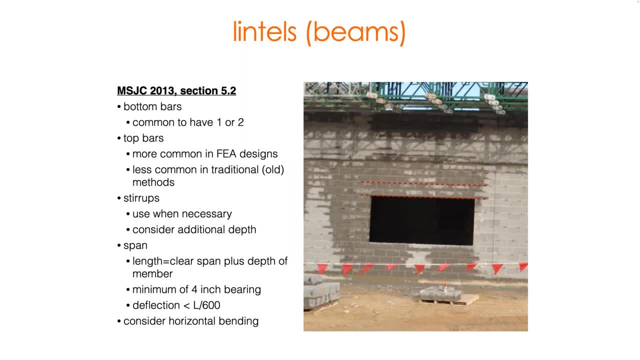 of today. you know some of the different loads and forces that you have there. Top and bottom reinforcement can be very helpful. stirrups: You can certainly add them When you had limited depth, but adding more depth to the overall lintel will be a much simpler way. 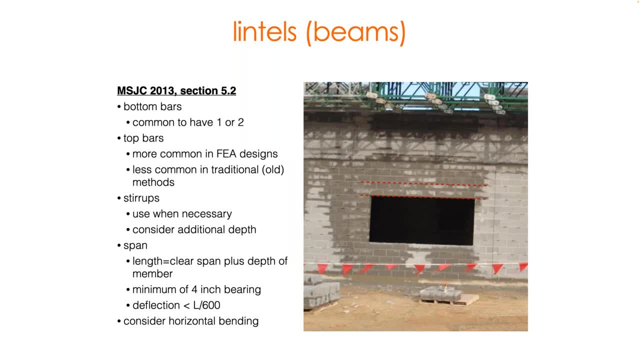 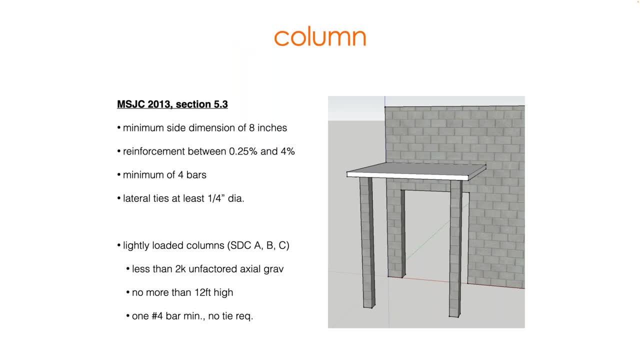 of solving that. So lintel beams are certainly those elements, Columns within the code. we have a minimum side dimension of eight inches. So yes, an eight by eight-inch item would be a masonry column Reinforcement between a quarter and 4%. 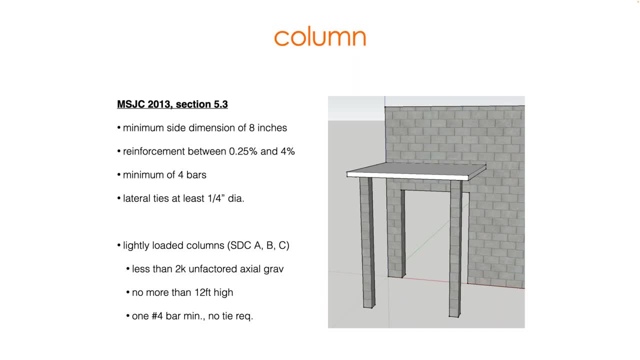 Minimum of four bars, lateral ties at least a quarter-inch diameter, So like a, And number two would be the tie that would be needed. So that's kind of the standard column provisions for masonry. So that's quite a bit of reinforcement, especially the minimum four bars. 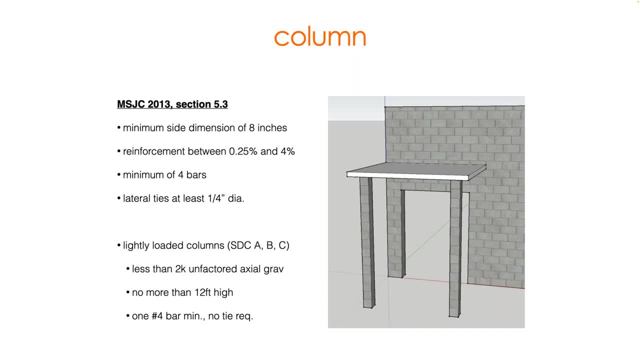 Within the code. they also have now lightly loaded column provisions, which are allowed in seismic design categories A, B and C Any time that you have less than 2,000 pounds of force no more than 12 feet high, the minimum reinforcement that you need. 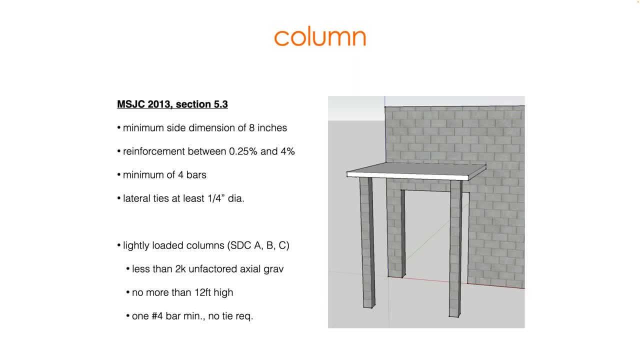 to add in that lightly loaded column is just one number four bar no ties, So that's certainly a very nice element. I always like to ask the question to designers. you know what is a column? A column is going to be that isolated element that's going to be away from the rest of the wall. 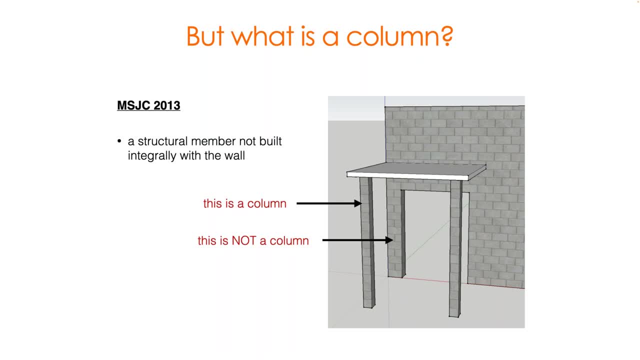 The wall. you know, if it's a section of wall next to an opening, that's not a column. The code writers did not define that as a column. it's certainly meant to be part of the overall structure, So that's a very nice element. 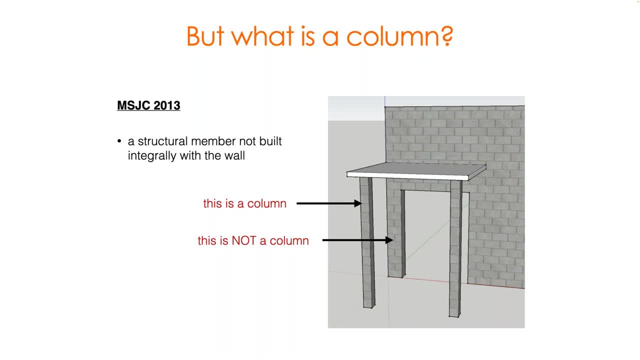 So that's a very nice element. So that's a very nice element for a wall and should be reinforced with wall provisions, not column provisions Could be considered a tier, I mean, it could be something like that. So really, what that does is get you know those isolated elements away from being 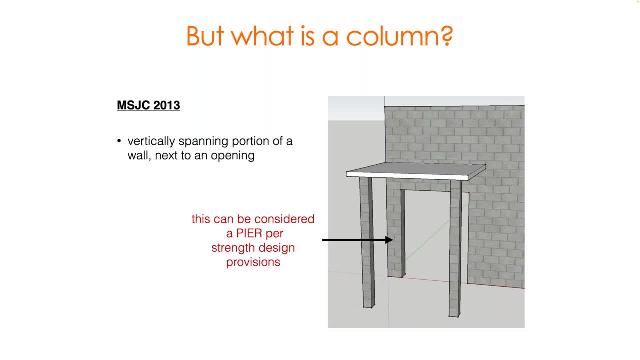 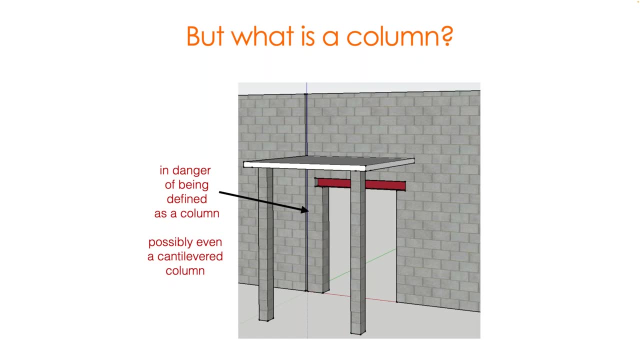 having all that stirrups and everything that you have to add to those elements. The one caveat that I make to that is if you would have some other material in there for a lintel design, then you could certainly be kicked back more to a column. 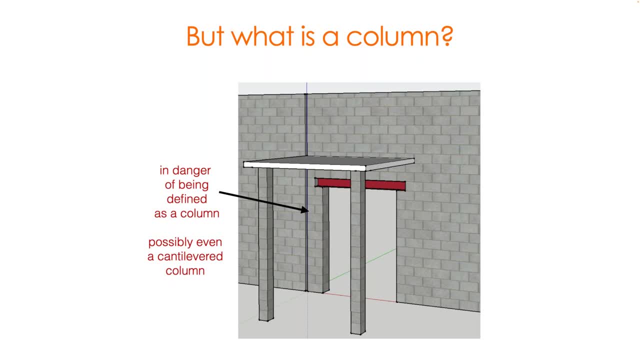 You could actually go back to a column. You could create a hinge in that wall where that element is actually, maybe even a cantilevered column, something to prevent that hinge from occurring. So what is a column? What is a lintel? 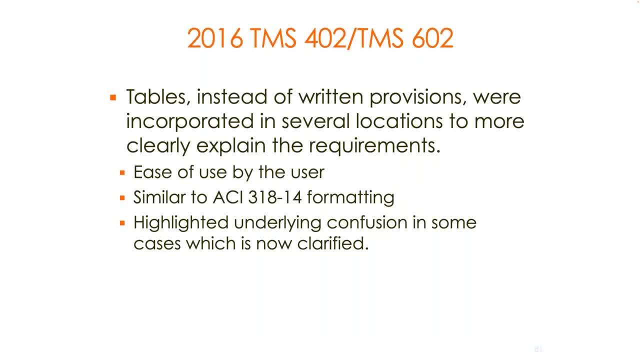 Some of those things are important to look at: design-wise Tables instead of written provisions incorporated in several locations to make it a little bit easier, Obviously trying to make using the code a little bit better. Just some examples. Just some examples of how that was being done. 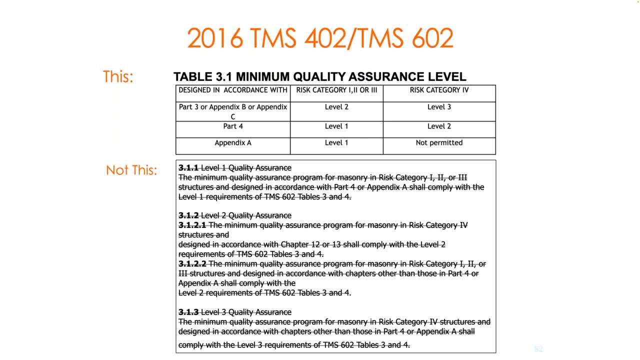 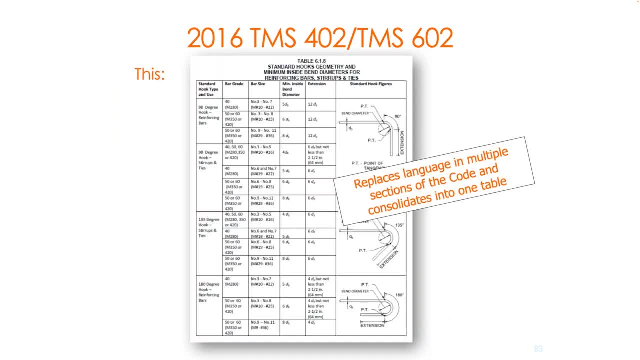 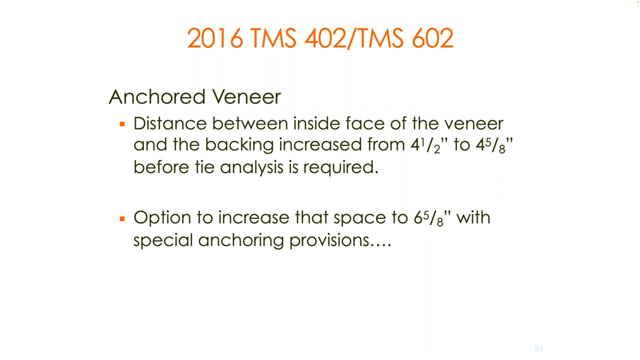 So again, just some cute little reference tables instead of long, long descriptions that are trying to explain the same thing. Hopefully that adds more clarity. Hopefully that gives designers a little bit better options for design. Distance between the inside face of the veneer and backing increased from 4 1⁄2 to 4 5⁄8.. 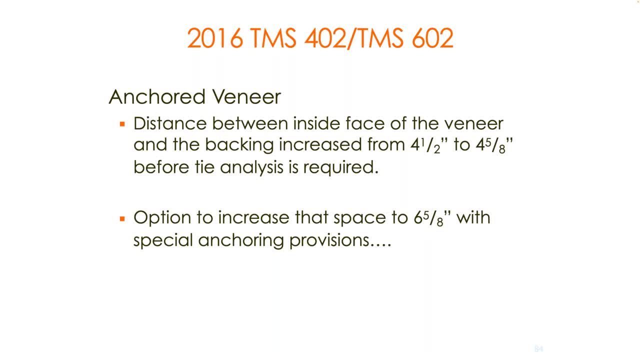 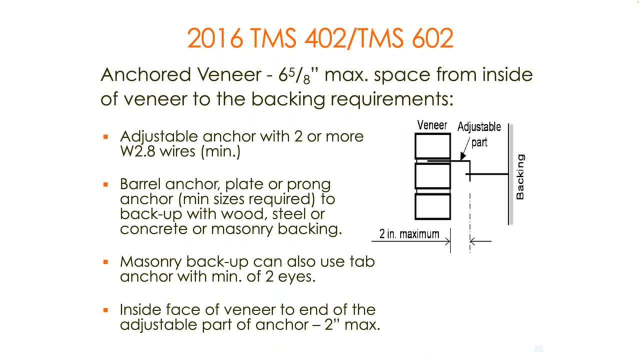 Look at that, Looking at going all the way to 6, 5⁄8 inches in later codes- Anchor veneer: 6, 5⁄8 inch maximum space from inside the veneer to the backing- What some of the different requirements are to be able to do that. 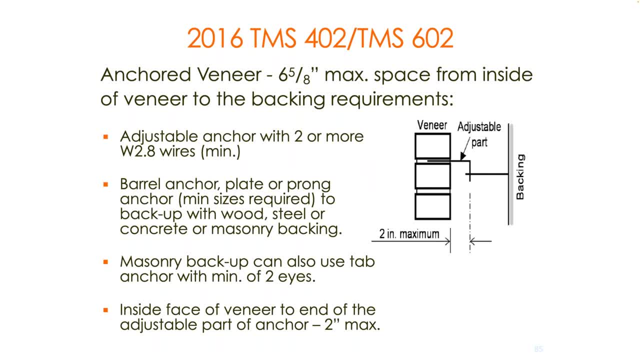 Adjustable anchors with two or more W 2.8 wires, kind of the minimum. So pretty heavy wire barrel anchors- Main history backup can also be used. Tab anchor with a minimum of two. I's Inside face of the veneer to end. 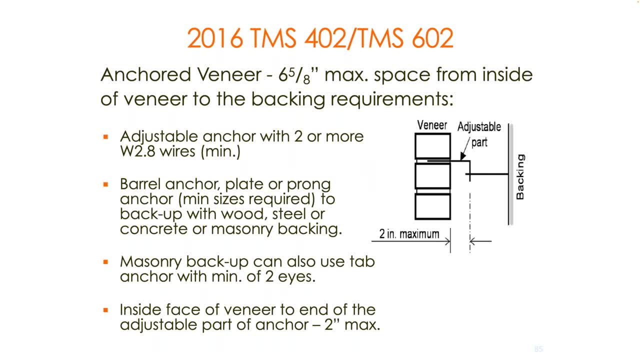 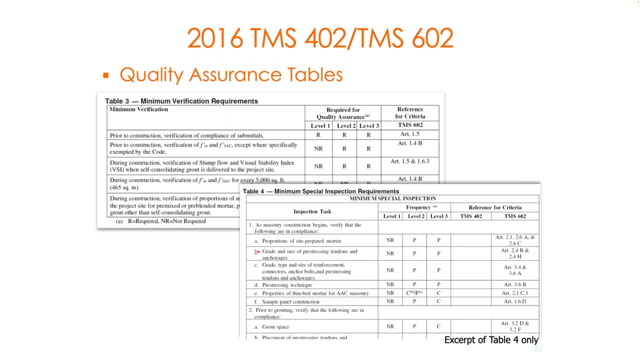 So giving it that larger space is certainly. as we have more and more insulation, we have thicker and thicker walls, having that larger space can certainly be very helpful. Quality assurance tables were rewritten and simplified. Some of those quality assurance tables that are there. 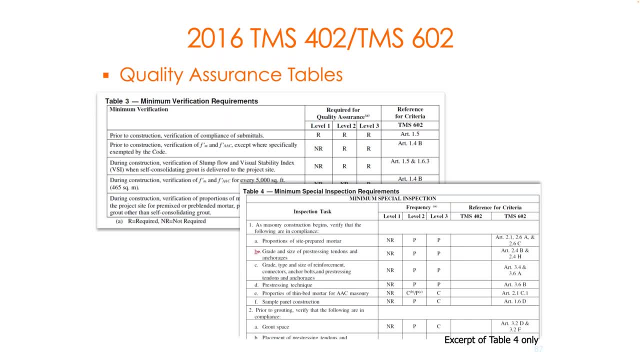 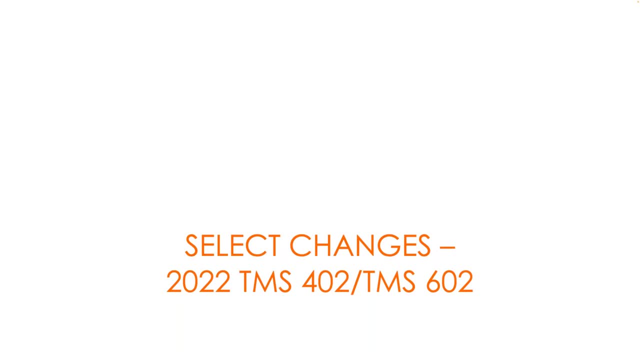 So hopefully the code getting a little bit easier to use, definitely getting thicker and more things being added, But hopefully that adds some clarity. Hopefully getting easier to use with some of those different tables being added- Kind of 2022, some of the major elements that are being added here. 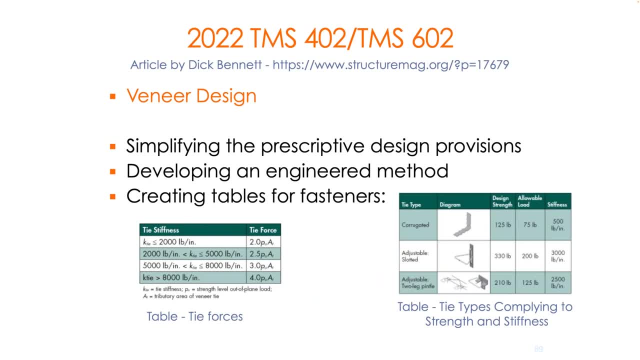 Now again, these aren't going to be showing up in most people's designs quite yet. They're going to be referenced in an IVC that's probably not quite referenced in too many places, But there's some veneer provisions giving some actual forces for those ties. 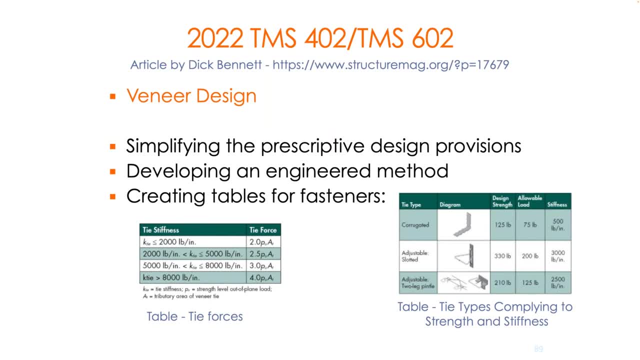 So, again, as we have more and more creative designs, we have more and more different options. We're tying veneers back to structures. So hopefully giving a little bit more of attention to what some of those design loads are and what some of the different ties that would be allowed for that would be. 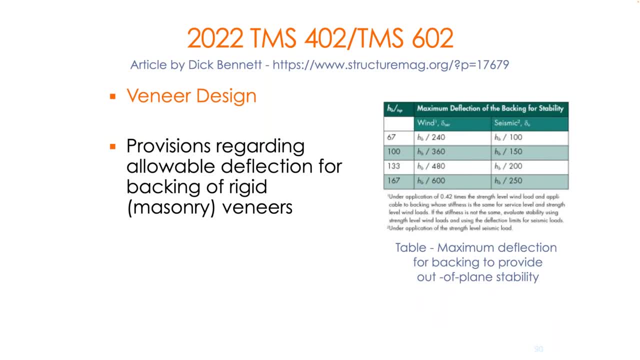 Also in the veneer design category, trying to point to having stiffer backups or actually giving what some maximum deflections that would be allowed for the backup when you have a rigid veneer. Obviously you don't want to have veneers. 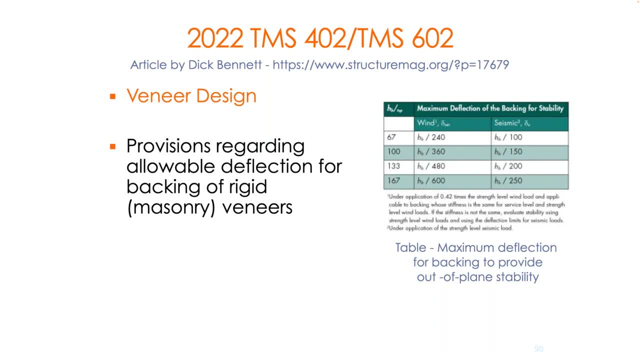 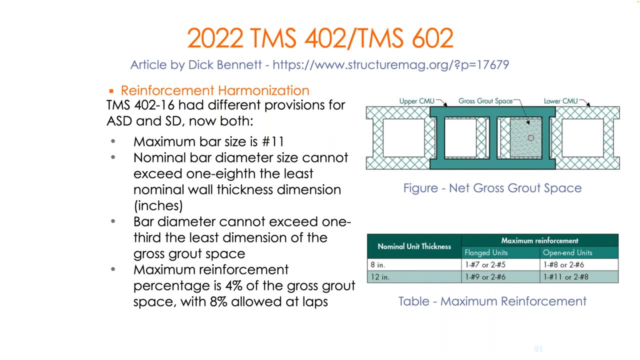 You don't want to have veneers that are cracking too much or are moving too much. So giving some references to what the actual backing should be for, stability-wise, for the veneer. Other clarifications that were made as you look at reinforcement: 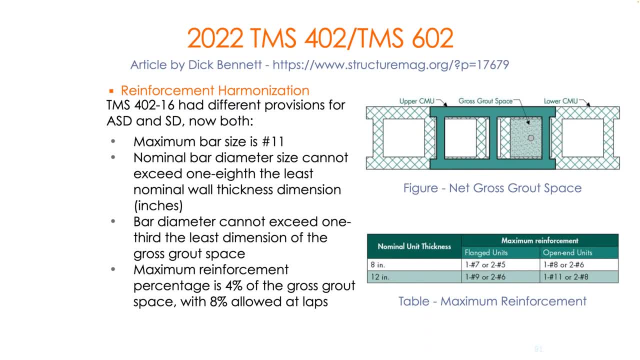 One. old codes had different bar sizes that were allowed within different sections of the code. So stretch Strength design, for example, had number nine as the maximum bar. A level stress design had number 11.. So now just giving one bar size as a maximum for either strength design or level stress design. 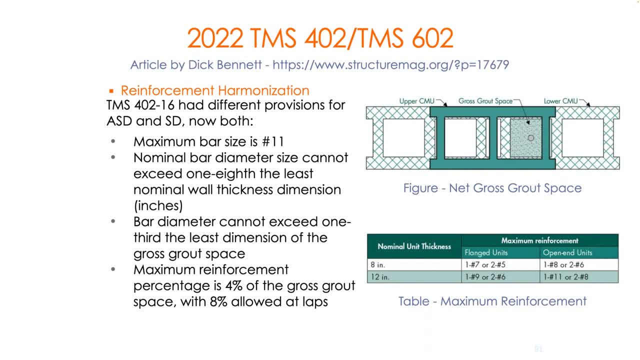 You know the reason for that, I think, was just the testing. Again, you know they didn't test strength design provisions for larger bars, So it just stopped at number nine. I don't think that we should be using 11s often within masonry walls. 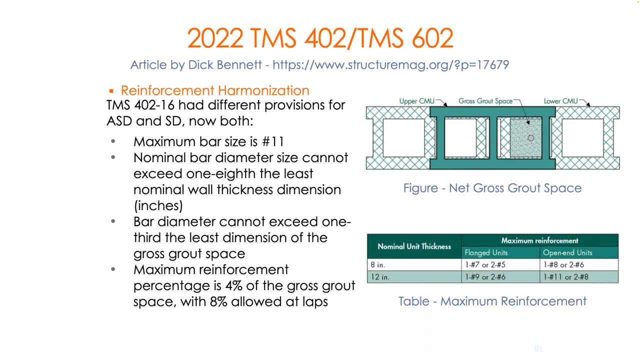 but it's nice to have that option. I guess I don't think you should be using number eights and nines for that. It doesn't matter, But anyway, and then giving a little bit more definition to the amount of reinforcement that's added. 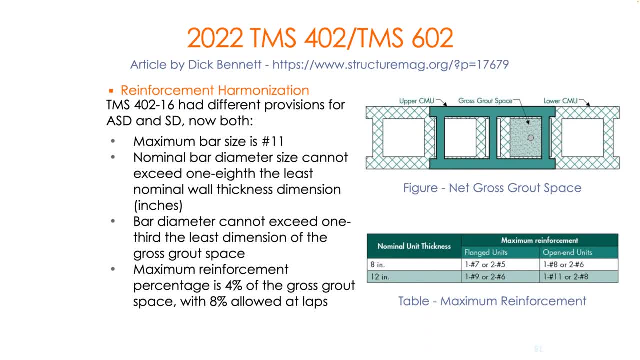 When you have H blocks or you have stretchers that are used where you have some flanges that extend past those cells, those do create a smaller actual net grout area. So different reinforcement maximums because of that reduced grout area. So you know you don't want to have a grout space, that would be common. 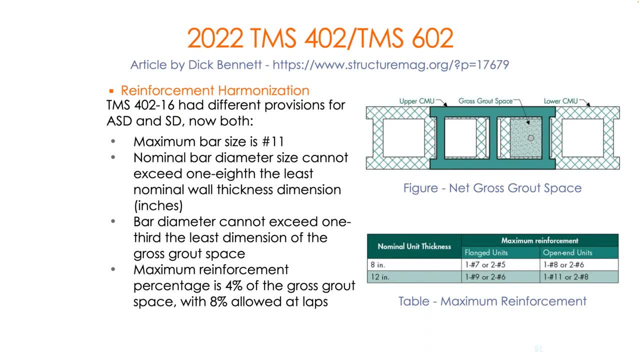 Again, all of that stuff, I think, is stuff that we can, as designers, exceed from time to time, But I think that we have to be careful when we do that. I think we have to really think about dealing with these confined spaces, and you know, 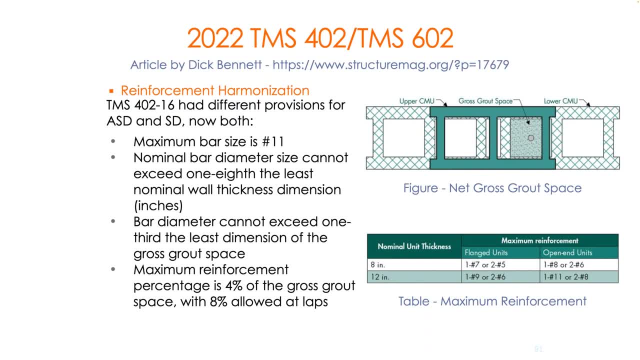 overlapping masonry elements and mortar fins that can be created. Anytime that you reinforce these masonry walls, you're dealing with these confined spaces that are moving around a little bit, So the codes really trying to give us some really good guidance as to the maximum reinforcement. 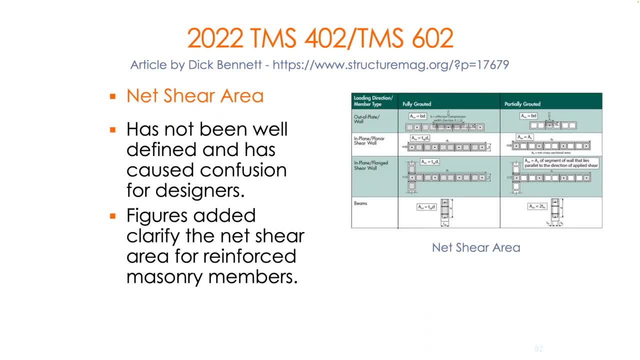 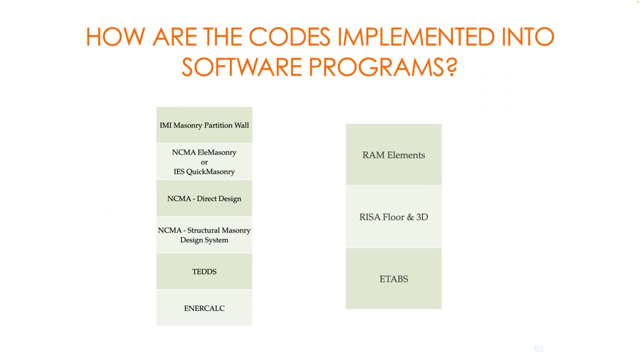 that would be used within these walls, Other things in terms of different provisions for net shear area, trying to define that more better as well. So a lot of different codes, a lot of different options, And then the last section of today is really going to be looking at some of the different softwares. 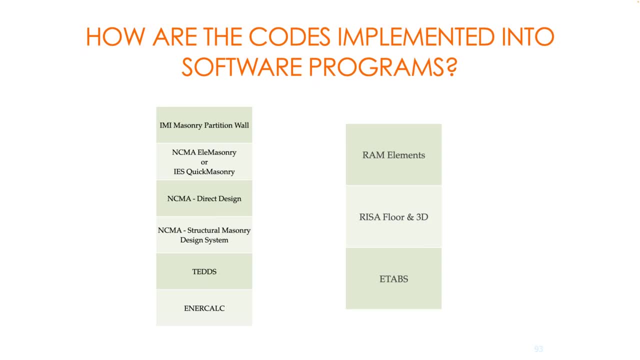 And really I think the rubber masonry. Okay, It meets the road in terms of you know the different software programs and what actual codes they actually have referenced. So we have a lot of different softwares and I'll cover these more later today. 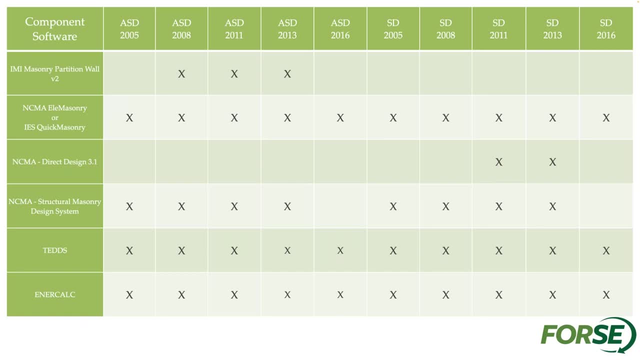 But just through these two tables in here and again. we have these in the sections later today, but this is really kind of pointing to different software programs have different code sections that are actually covered, So being careful with making sure that you use software. 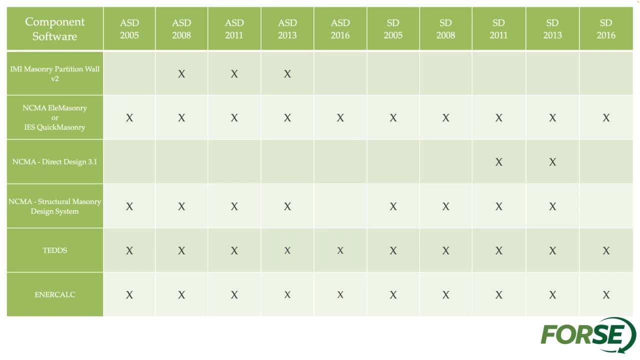 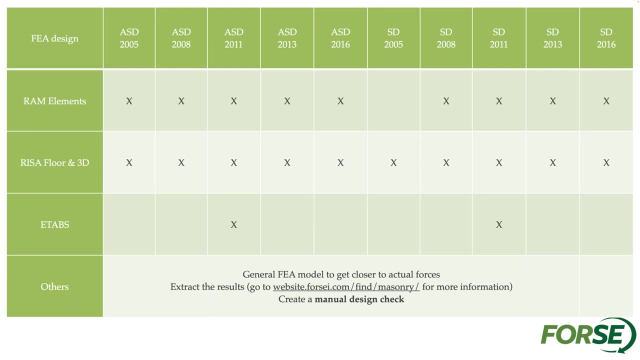 You use software programs that use the current code or use the code that you know. so this I will call these component design software, as we design one-off elements or some of the finite element analysis programs RESA and RAM. you know how they cover codes. 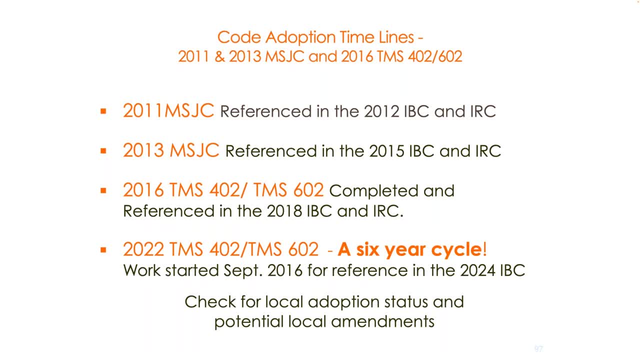 So just a really quick you know in conclusion. you know: 2011, masonry is in 2012,, IBC, 2013,, 2015.. You know, 2016 masonry is going to be in the future. 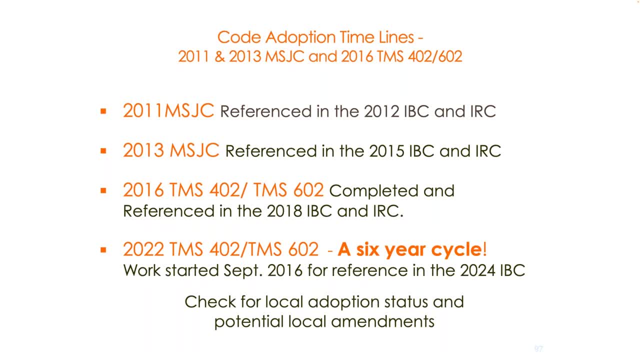 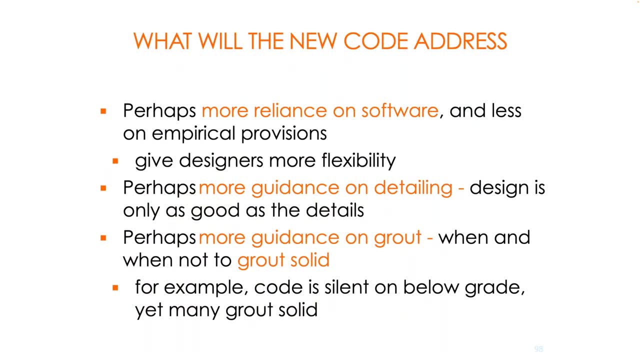 In the 2018 IBC and then the 2022 masonry code for reference in the 2024 IBC. So you know code. hopefully it continues to make things a little bit more clear. Obviously, they have more and more things that are added to the codes, but hopefully it's. 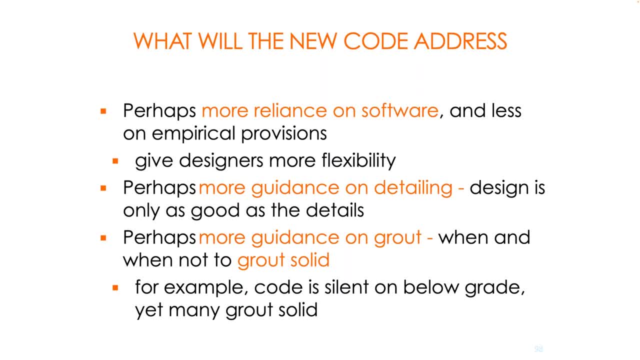 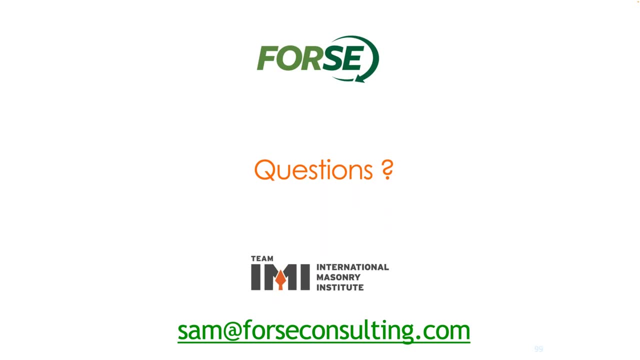 going to keep giving us more guidance, more harmonization between strength design, allowable stress design, Create some of the Reduce some of the confusion, stuff like that. But there's other things certainly that the code can go into, And so with that it kind of takes us to the end of that first section. 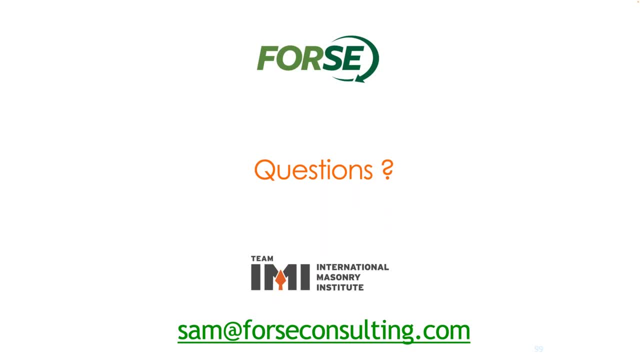 I don't know if you guys have any questions. It was just kind of a pretty big overview in terms of codes that are out there and then some of the recent changes for masonry codes. All right, So we'll take just a couple of minutes here. 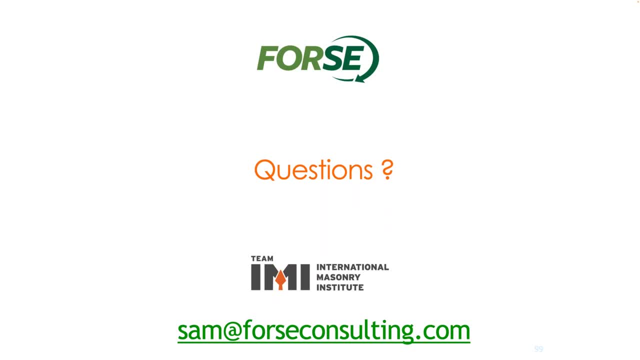 I'll just kind of keep a look at questions, Okay. So if you have any questions in the meantime, I'm going to switch over to a different presentation if I don't see too many questions in the next couple of minutes. And then just a quick make sure you guys are all still awake. 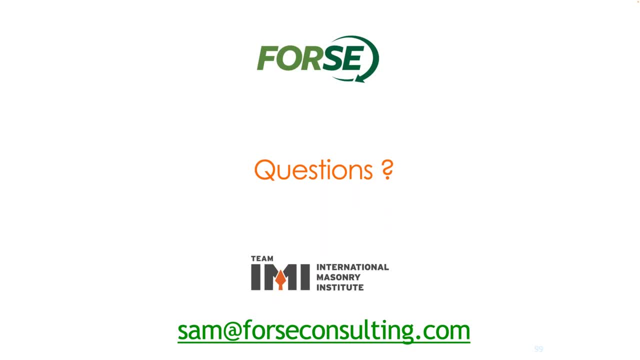 Can everybody still hear me? Okay, Audio is that. was that just Yeah? that was yeah, that was just mine. I think I bumped a mute button or something like that, So everybody else said they could hear the whole time. 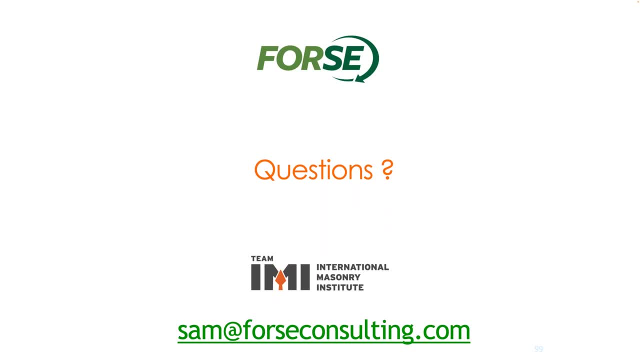 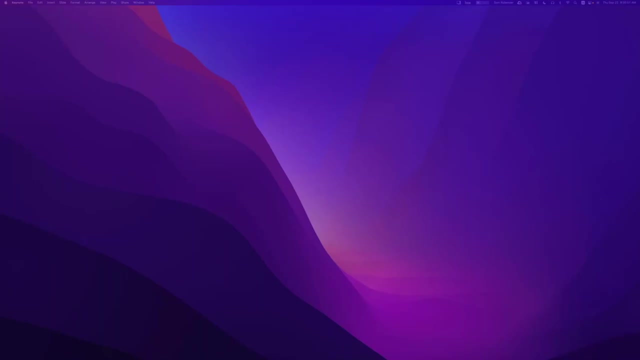 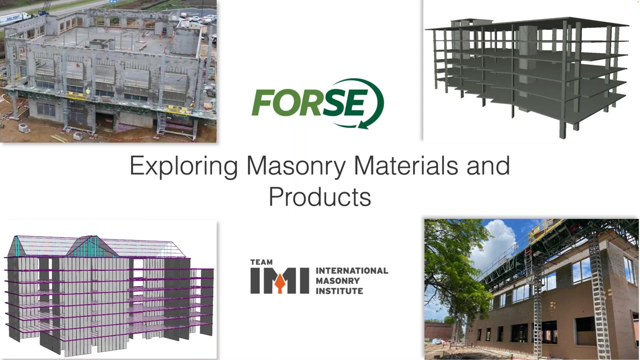 So, Okay, Very good, Very good, Yeah, Yeah, Sounds good. Okay, All right, Let me. it looks like there's too many questions, so we'll switch to different presentation. Okay, All right, so maybe we'll go through this section as well, and then we can take a five. 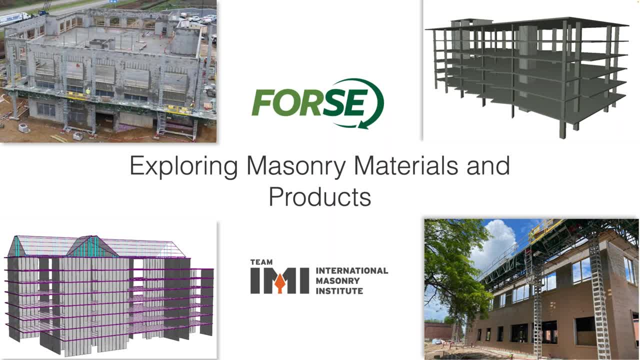 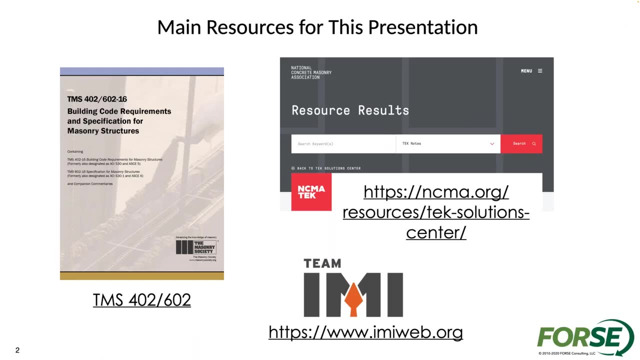 or 10 minute break, maybe after this section, for everybody to just to have a break, grab some water, do whatever we need to do. So All right, So exploring mainstream materials, kind of going beyond the codes. Okay, So the options and things that I looked at here for obviously most of the information. 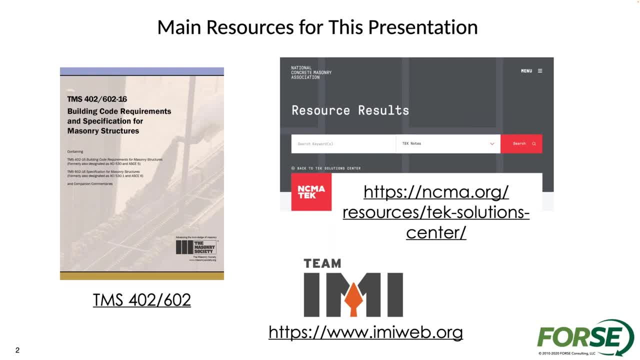 that I'm going to cover with the different materials and stuff is going to be either referenced in the mainstream code- Other really really great guides for mainstream design is not necessarily in the code, I'd say the elements in. you know some of the different papers that I have, you know. 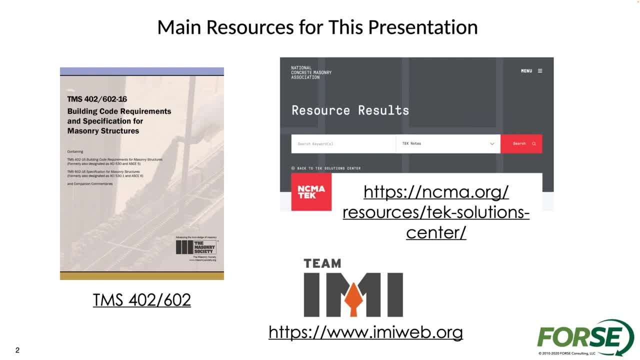 International Masonry Institute does have some information. but the NCMA tech guides are really great. They have a lot of great items for that are referenced throughout the day. There'll just be different times where you know the code doesn't quite cover something. 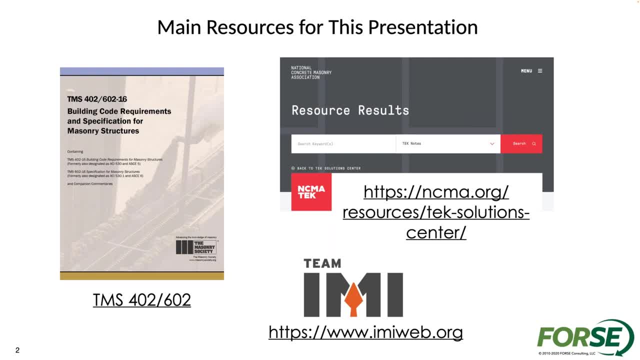 It doesn't go into the this in depth and you know, really we have to go to NCMA. So the National Concrete Masonry Association has a lot of different resources that would be papers and guides, and there's some spreadsheets and stuff that are out there that could really 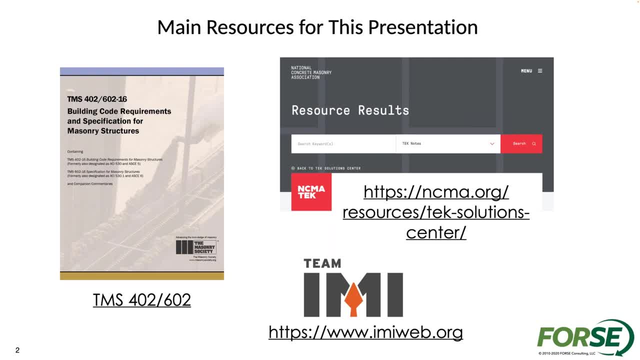 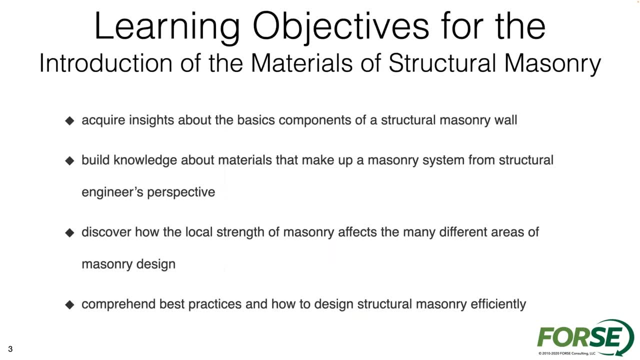 be very helpful for mainstream design. So I utilize those guys all the time. Okay, And if I point to a few different papers that they've written, really because we're trying to acquire some insights about the different components of masonry walls, build knowledge. 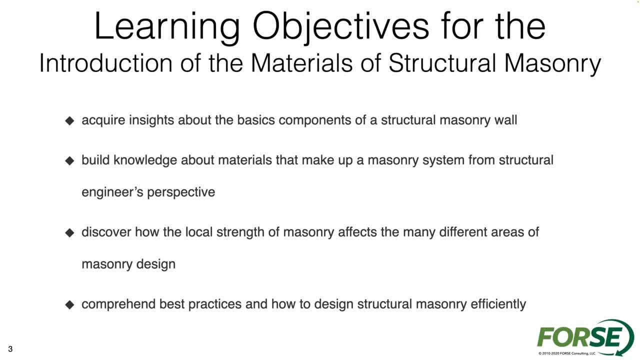 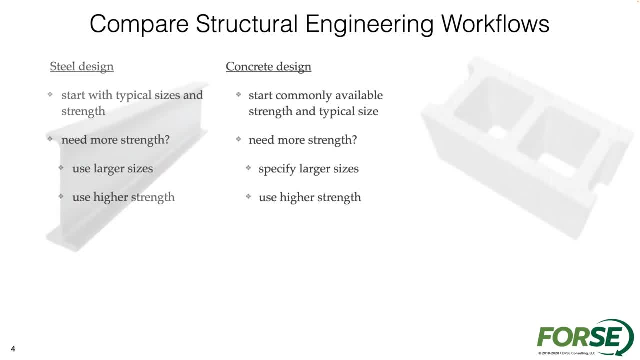 about the materials that make up the masonry system, learn how local strengths can affect masonry design and just look at some best practices. You know, when I talk about masonry, you know I like to compare to how masonry. how does 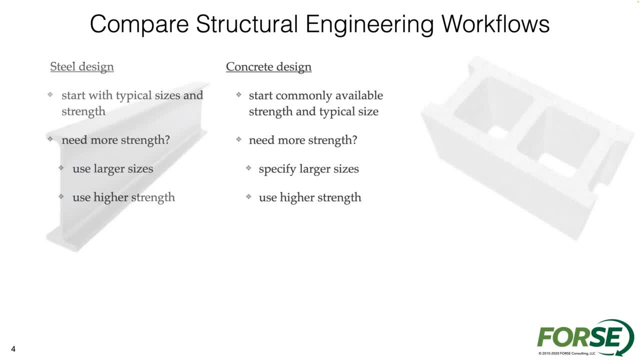 masonry stack up with steel and concrete design. You know we have some pretty typical Kind of design flows that we use for steel design or concrete design. We you know both of them. we just start with common sizes and strengths. 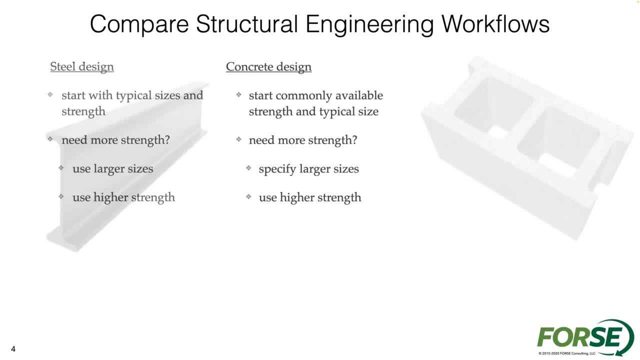 For steel. if we need more strength, we use larger sizes. Sometimes we use a higher strength, but that's kind of rare concrete design. We have typical strength sizes. We just you know, if we need more strength we can specify larger sizes, or often we can. 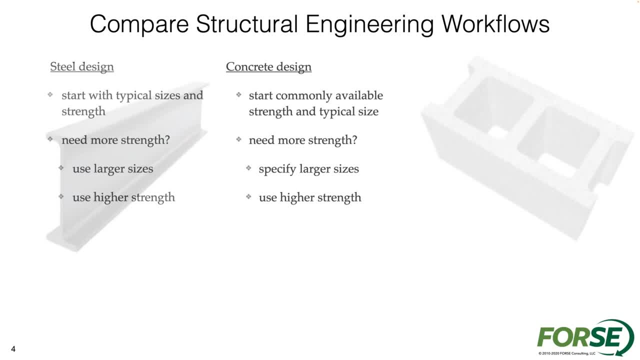 use higher strength. It's kind of fluid on both kind of both of those different parameters for masonry design. You know we start with a minimum strength, you know often, And then if we need more strength we just use thicker walls, larger blocks. 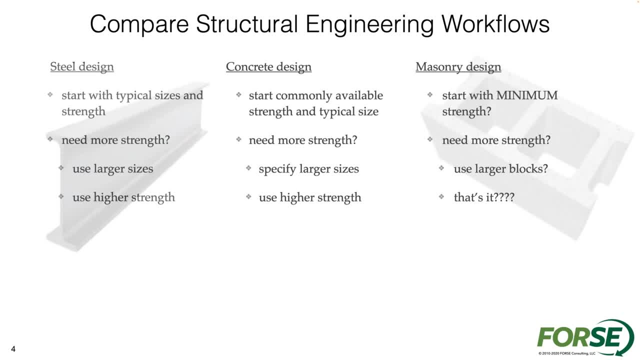 And so really what I want to do is I want to kind of eliminate, kind of the traditional way that we look at masonry design. I mean, masonry does have a lot more options than that. We can need more strength, We can use larger blocks. 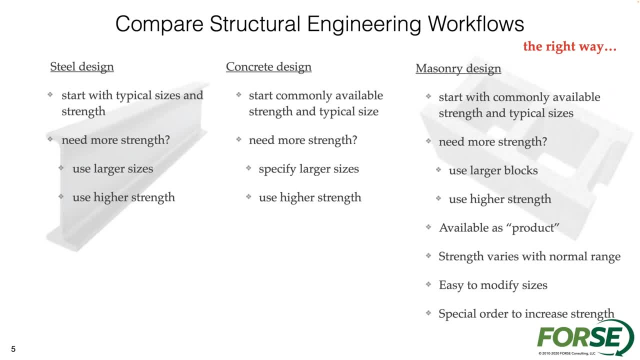 We can use higher strength. You know masonry is available as a product But Masonry product is made all the time in different block producers can specify. if you specify a higher strength block, block producers can make that block. Certainly I wouldn't ask for 10 of a higher strength block. 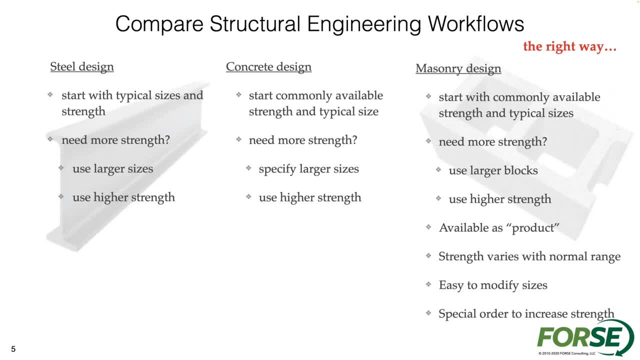 You want to have a lot of that material that you would need, But masonry is something that is easy to increase the strength. It doesn't be a special or it will be a little bit stronger, but so is concrete. So you have a FC of 8000. 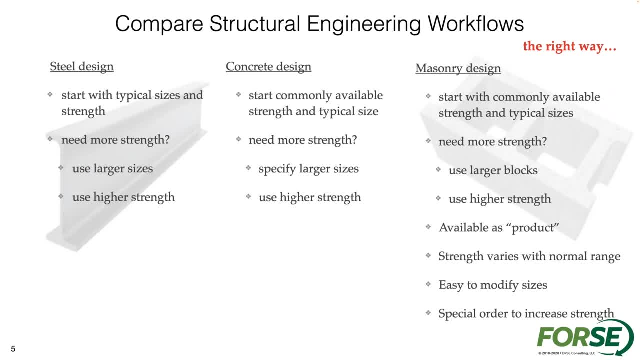 That's going to be something That's going to be a higher, higher cost of concrete. So just the same with masonry, if you need something that's a 5000 PSI block, that's something that they can make. It's probably going to cost a little bit more, but you can do that. 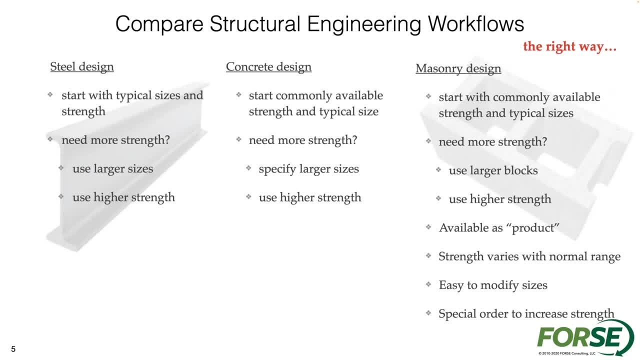 So I think that you know masonry does have some similarities between steel and that there are common strengths. We should know what those strengths are, but it's it's quite a bit different than steel. You know. I think a lot of times people put them in the same category, like it's a product. 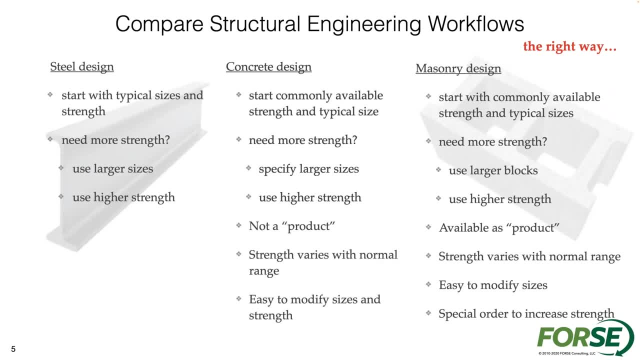 it's just something that's static and we really can't do anything else with that. So again, you know, as I kind of compare the two, it is available as a product. strength, you know, and steel is uniform. strength with concrete varies, strength with masonry varies. 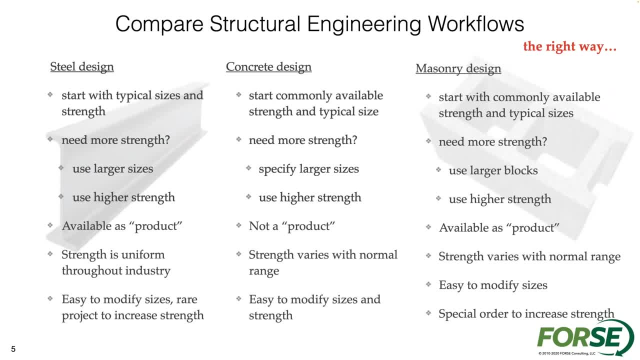 It's easy to modify sizes in steel. It's rare to increase strength with steel. easy to modify sizes and strength with concrete. I think masonry is the same Easy to modify sizes, But it's also easy To modify strength, especially if you need to get to a higher strength. 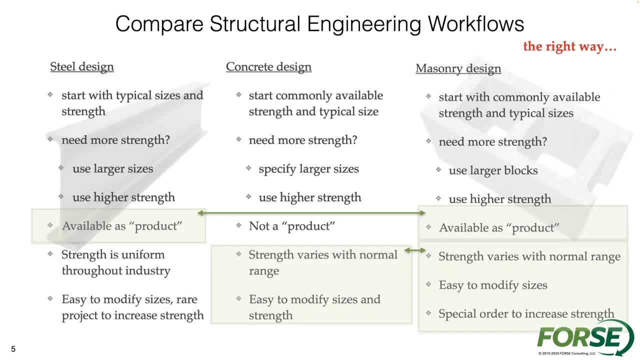 So I'd like to kind of show how masonry has got some similarities between both of them. It's not kind of this, this material that we just put on the side and and just designed to a minimum strength, and so on and so forth. 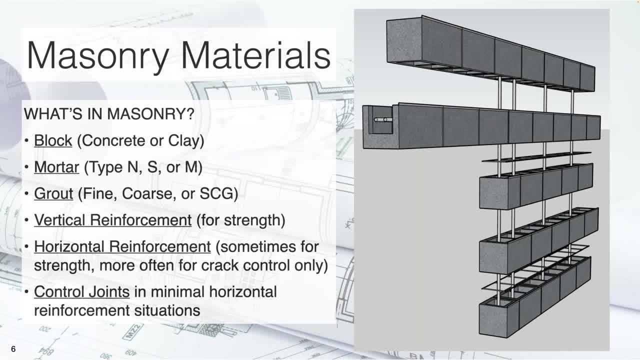 You know what's in masonry. there's, you know, quite a few different components that go into masonry design. you know blocks you know are going to be your primary element. Concrete or clay could be even a different material, but those are going to be the most. 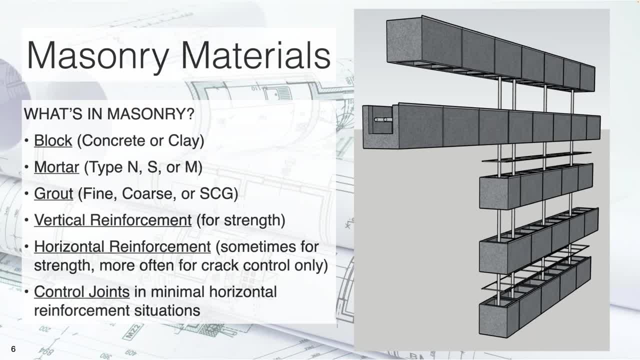 common. We have different mortar types: Type N mortar type S or type M. All of those have different pluses and minuses in different times that you would maybe use different types of mortar For grout. we have different types of grout. 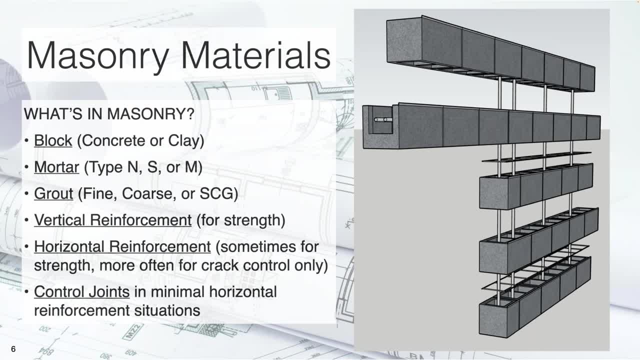 We have fine grout, coarse grout or SCG, which would be self-consolidating grout. We have vertical reinforcement. that we have in the design. Certainly you know we've got a lot of different types of grout. We have fine grout, coarse grout or SCG, which would be self-consolidating grout. We have fine grout, coarse grout or SCG, which would be self-consolidating grout. We have fine grout, coarse grout or SCG, which would be self-consolidating grout. 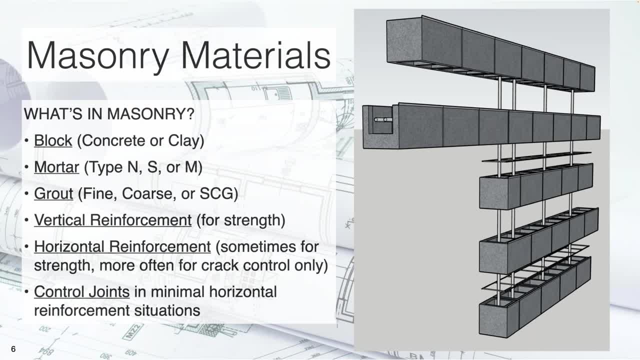 Any place that we put those we're going to add grout. We have horizontal reinforcement that can be used for strength design, Often used for crack control. We have control joints that are in minimum locations so that we can keep the horizontal stress in the wall as minimal as possible. 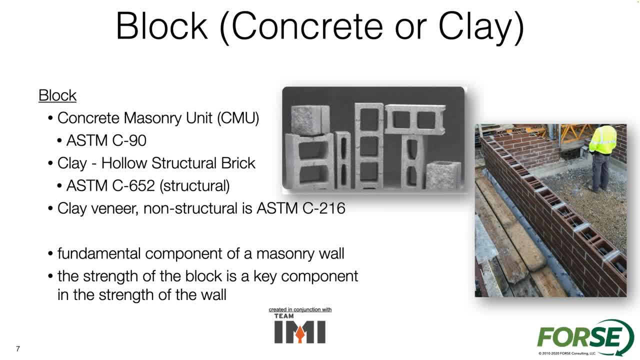 So a little bit more about the blocks. Again, we have concrete masonry units, ASDM C90.. That's going to be your common, That's going to be your common masonry element. that's out there. We see more and more provisions for clay, hollow structural brick. 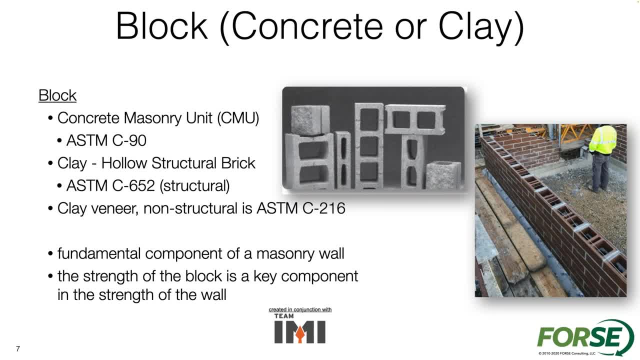 ASTM C652.. This is different than your standard veneers, your standard clay veneers, which is going to be ASTM C216.. The hollow structural brick or the concrete masonry units, both of those are going to be structural elements. You can see the two images on the screen. Both of them have. 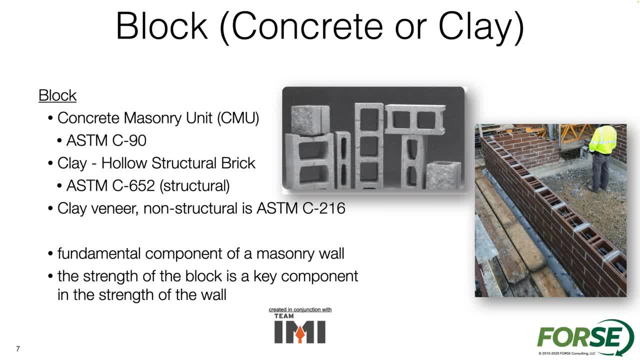 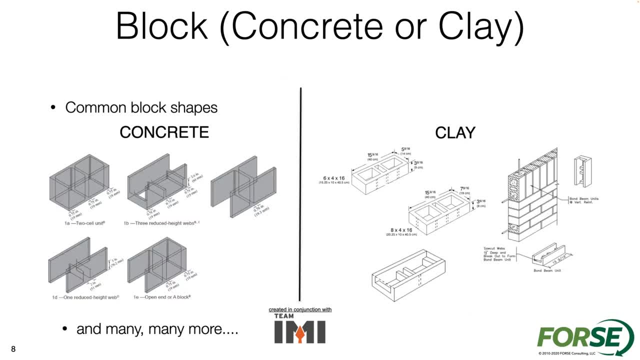 large cavities for reinforcement and obviously meant to be reinforced in that way. We have different types of elements that are available. Again, hopefully, that image looks familiar to the 2013 code- The different minimum thicknesses of the different flanges, webs- but it also points to the different types of blocks that are available for concrete. 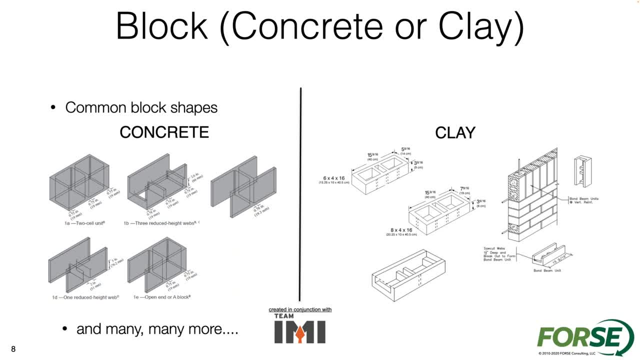 Really concrete can be formed, So then you can form all kinds of different shapes relatively easily. I would say clay I mean. so it's a hollow structural brick. The one thing about that is referencing the fact that it really is going to be one unit. I mean, they're going to extrude one unit. 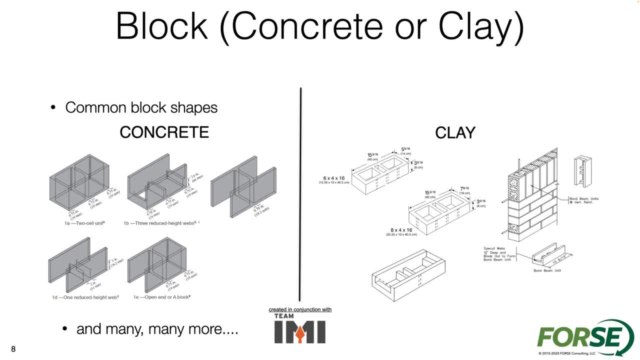 and then they can modify it. But really, as you look at reinforcing a hollow structural clay wall, you'd really want to look at, you know, detailing that, making sure the right different block shapes are used in different locations so that we can reinforce the wall the way that we want to. You don't have all the different shapes. 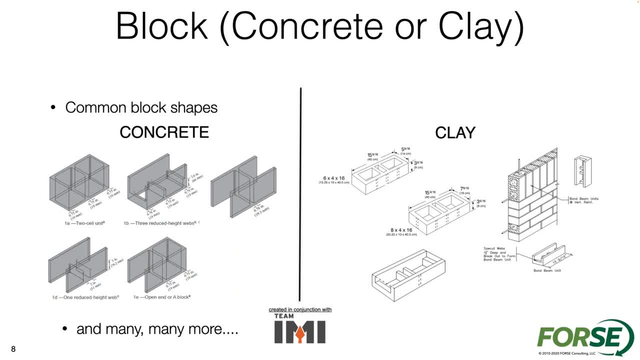 that are made coming out of the plant. You really have one shape that gets modified to create your flow through bond beam. so you're going to see that there's no U-shaped block, There's no lintel blocks for clay, It's just going to be pretty standard. just a little bit more information, because this is 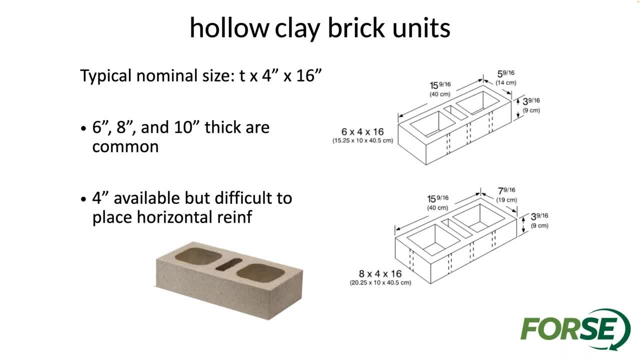 still new to some people. looks like this is a hollow structural brick right, A fitted piece of board. very well, So if you guys were thinking about…. structural brick units are going to be typically four inches tall, and then they can six, eight or 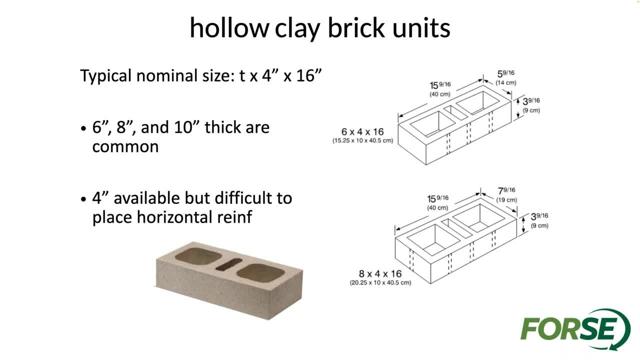 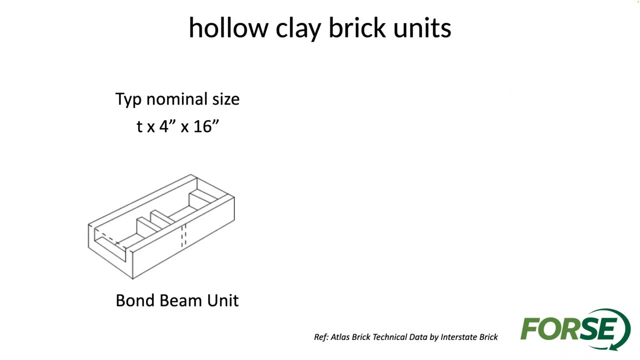 ten inches wide, but it could be shallower than that. it doesn't have to be four inches, it can be actually the, the two and five eighths or whatever that it could be similar to, similar to the common clay elements, and then for using it as a bond beam block, that's going to be something that again is going to take. 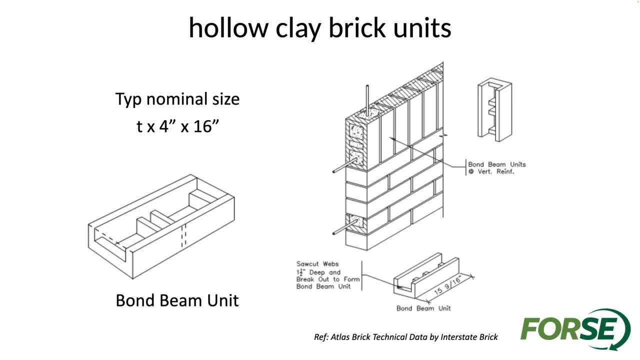 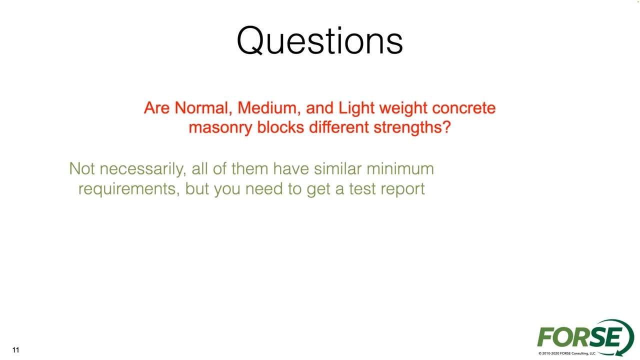 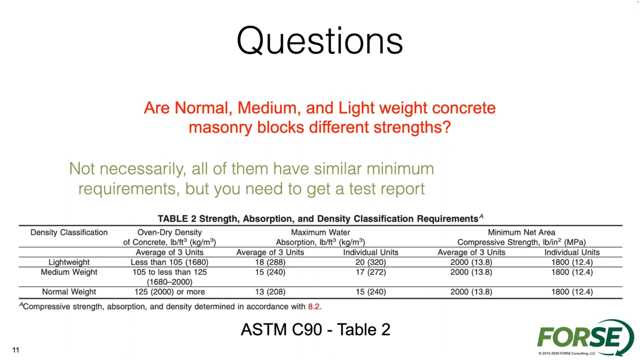 that standard unit and then they're going to be cutting the webs down so that you can place that horizontal reinforcement a little bit more straightforward design-wise. so just a quick question about concrete masonry units. are normal medium and lightweight blocks, all different strengths, not necessarily within the actual estm table. it points to the same minimums. 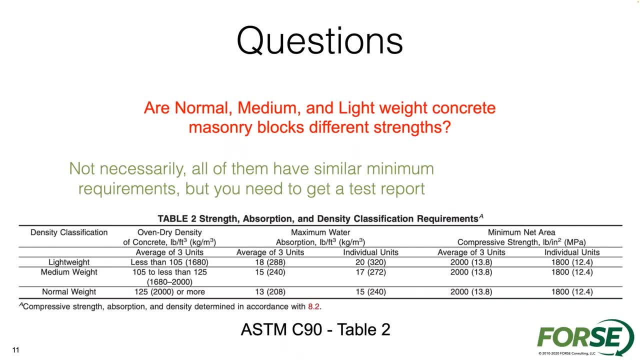 all the same requirements for the different weight materials. obviously lightweight is going to be a different aggregate likely than what you would have with a normal weight. different agigets going to lead to probably different strengths but all of them do start with that minimum standard of 2000. oftentimes i see normal weight probably being the stronger. 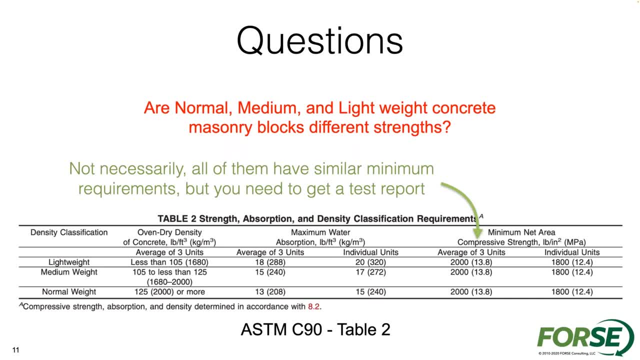 design strength. but i have seen lightweight blocks that are made that break out over 4,000, 4500. so it's really good to get the the test results uh to see you know what the different concrete uh um being added to the different uh normal weight, medium weight, lightweight options are. see what, the see what. 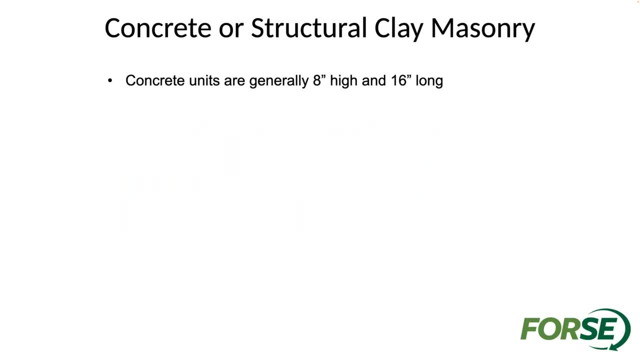 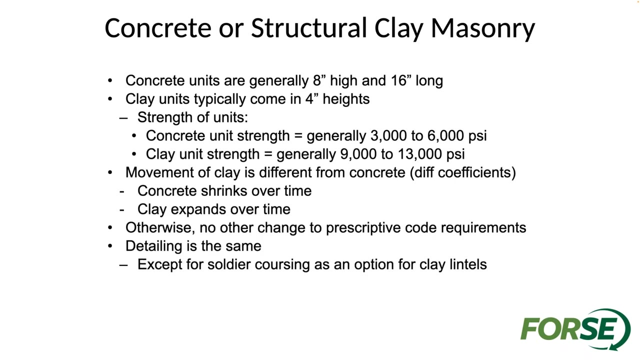 the data points to. um, you know, concrete units are typically eight inches high and 16 inches long. clay units typically come in four inches high. uh, concrete units are usually three to six thousand. clay is going to be somewhere in the 9 to 13 000.. um, the movement of the different, the different. 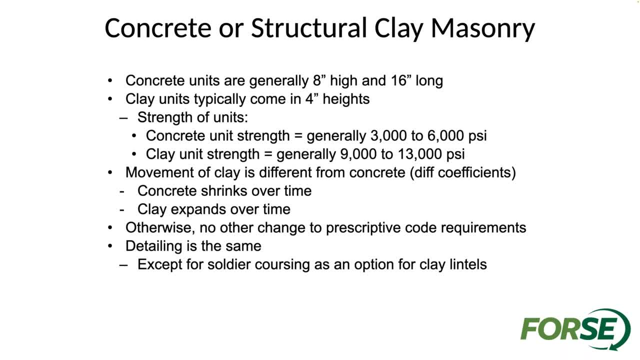 clay is going to be different than concrete. concrete is going to shrink, kind of have a tendency to shrink over time. clay is going to have a tendency to expand over time. otherwise, there really isn't any prescriptive changes to prescriptive code requirements really. they're going to be designed in the same way. you're going to be designing concrete and clay really with the 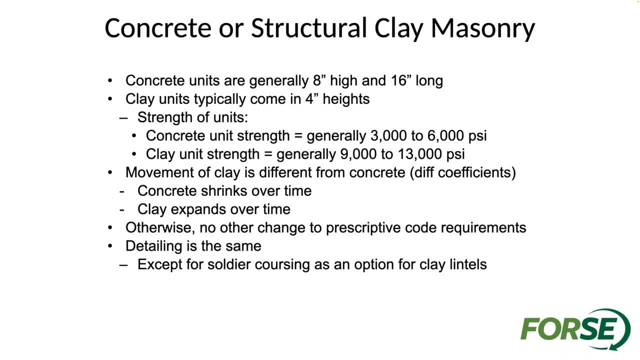 exact same equations, the exact same uh things as we're going through, and really detailing is going to be very similar. obviously you have more options for concrete. you can have more different types of elements that are going to be extruded, but you know, clay really can be used in some of the same ways, some of the different. 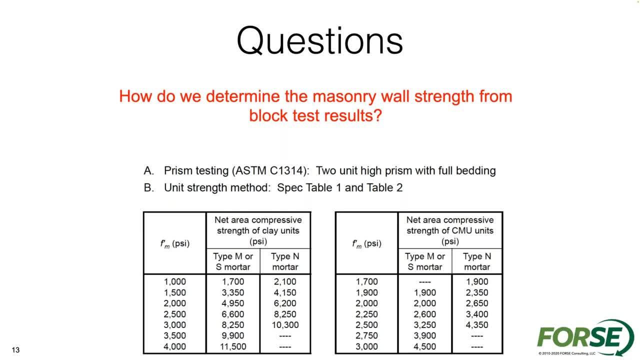 differences that you have between the two different materials. how do you determine the overall strength? the first way, prism testing, is going to be very straightforward. you take sam pls, you test them. the limitation to doing prism testing is the fact that you're usually doing prism testing close to when you're actually building a structure. that can add a little bit. 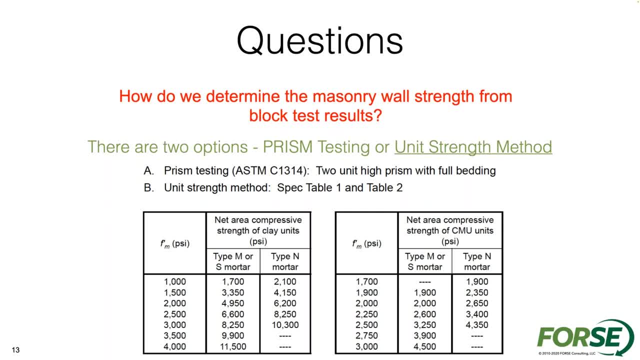 of a stress to the designers in terms of um. you know, how do we make sure that we have the right, how do we make sure that we have the right strength in our designs? so, unit strength methods. that's why those are created. and then you can see the two tables. 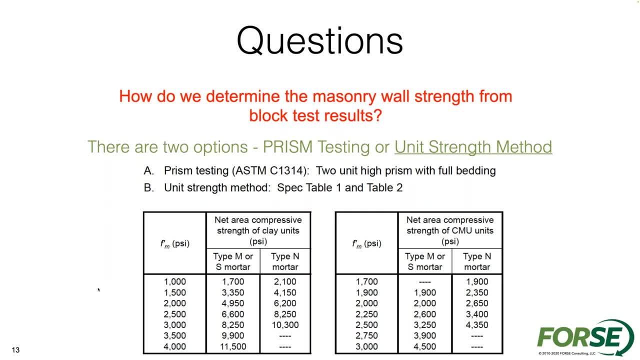 that are at the bottom. that's going to be unit strength tables, so you lost recently- sorry, i forgot- um. ambulances can support this, which is one thing where i want to play around with one thing called inflation. but what inflation means is inflation, and what inflation means is inflation in two different 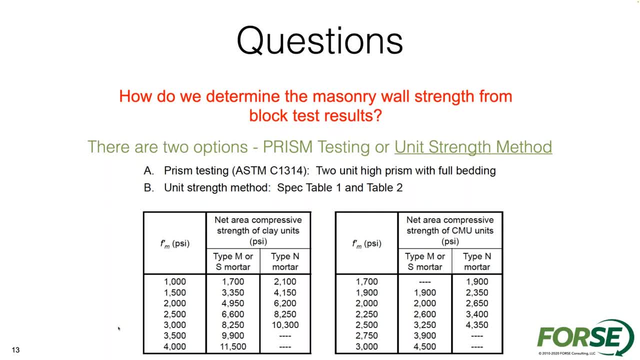 ways you're not going to have the same unemployment rate anymore. so inflation will give you the same rate of downward trend. inflation will give you a relative when the price of the starting望 rate way up to in the end of the year and that tion should divide into обязательно. 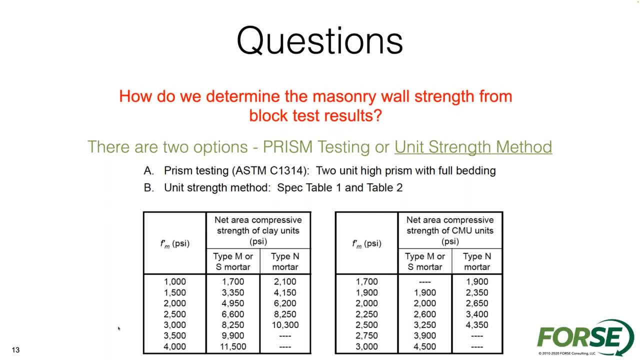 psi, so you have the same rate as you would if it's the strength you comes from. one boom, How heavy a pearl is reflected in terms of death weight for each square meter, and so itidos, in terms of such a力, somewhere in the 8,000 to 12,000,, 9,000 to 13,000,. 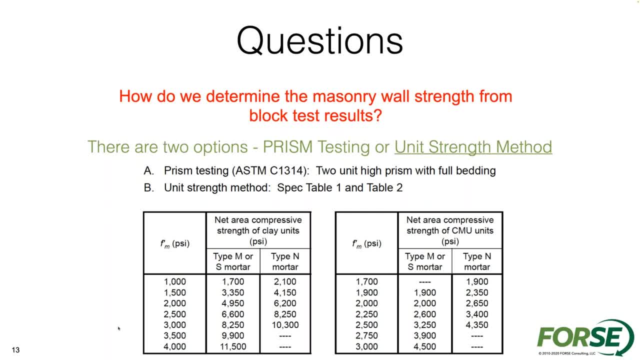 I think it was in the previous slide- in terms of the overall strength, We typically put structural clay units with type S mortar, so that's why I'm sticking to the center column for matching that with the to get the overall FRI mount. 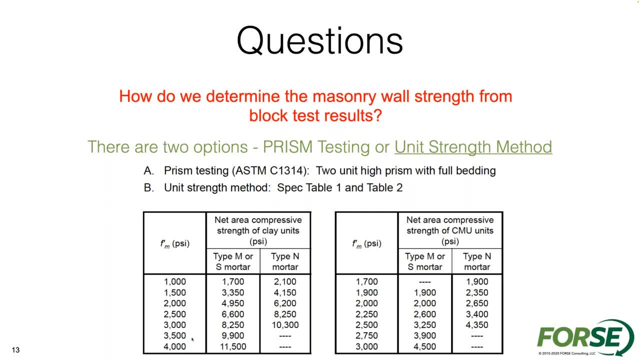 So the concrete strength you can see are a little bit smaller, but the actual, the difference between the overall unit strength and the design strength could be a little bit closer. You have a little bit more uniformity between the actual element strength and design strength. 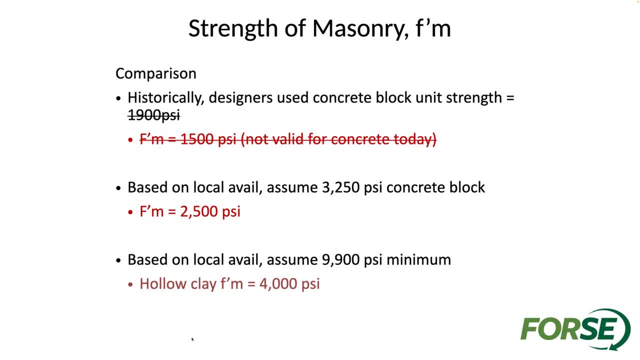 So the strength of masonry. historically, designers with concrete masonry have designed with blocks at 1,900 and then F prime M of 1,500. And that's just not valid for masonry. today We don't have blocks that are that weak. 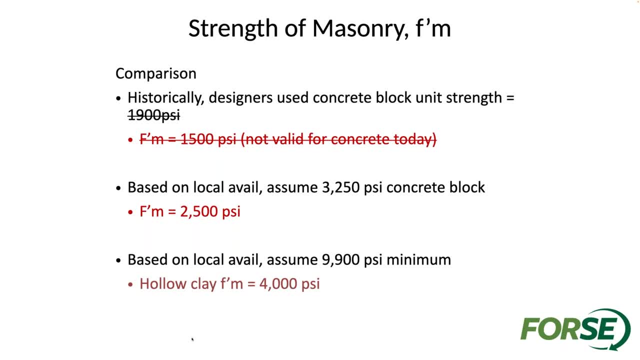 and with the updated code as of 2013,, we typically have a higher design strength. In fact, I typically point designers to using design strengths for concrete masonry with block of usually 3,250 or greater. Why 3,250?? 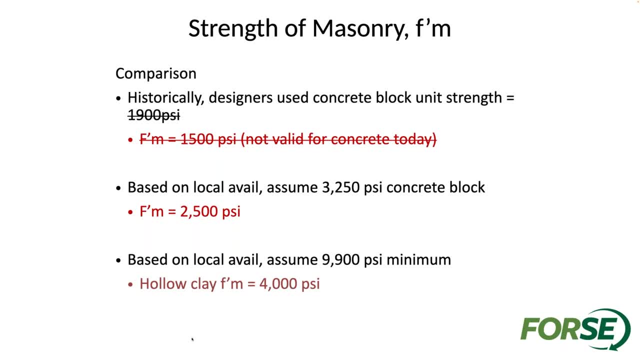 That's just a very nice round number that points to a design strength of 2,500.. So that's typically where we can start with concrete, with clay, We can start a little bit higher. We can go all the way up to 4,000.. 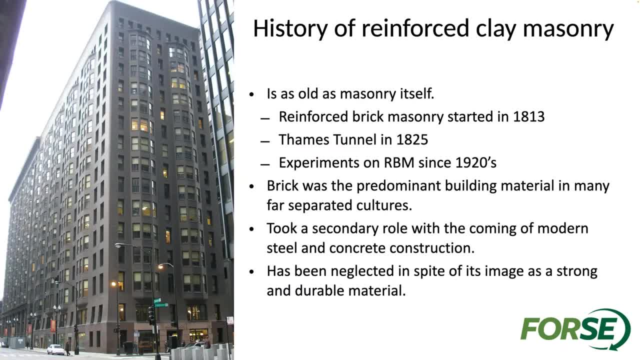 So there's just a little bit more about a clay masonry, just because it's something that we haven't seen a lot of, or I don't see a lot of designers using it, So I'm going to just give a little bit more reference here. 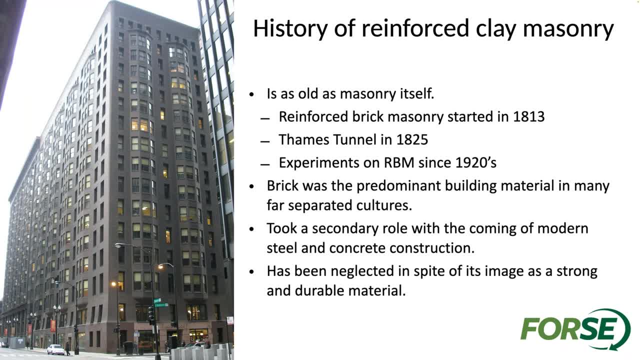 You know, reinforced clay is as old as masonry itself. I think that's fair to say. We've had reinforced brick masonry since the 1920s, So it's definitely going to be something that's been around for a long time. 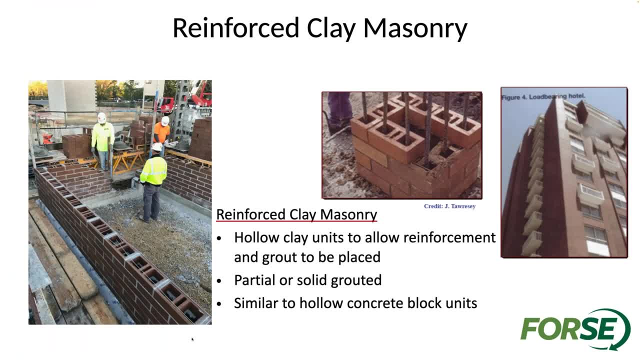 The units are going to be placed very similarly to how, you know, concrete units are going to be placed, you know, And so that's why the overall detailing and everything can be pretty similar. You know, what I try to point people to is sometimes people. 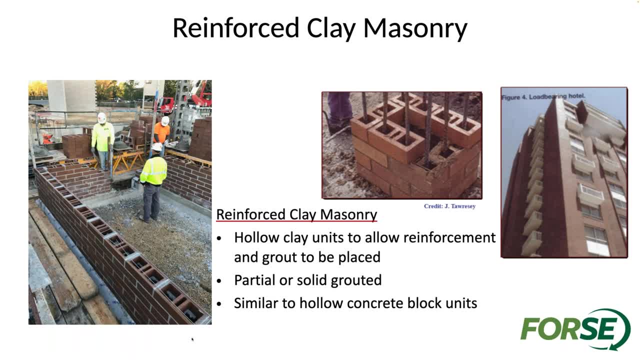 want to look like clay, but you know why don't they just use reinforced clay units? There's fewer manufacturers, There's less supply for this product than there is going to be for the common. Common bricks are available all over the place. 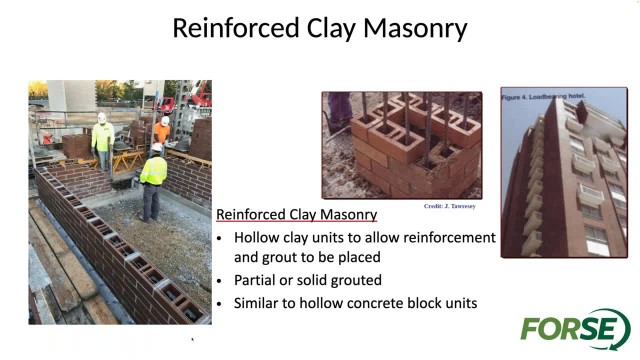 So I would say it usually comes down to a supply side. You know, if you're going to use reinforced clay, you want to make sure that you can get the material. That being said, there's some very large projects that have been done in reinforced clay masonry. 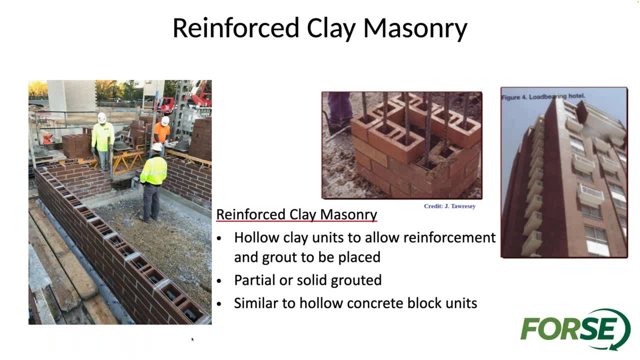 So it's something that is definitely worth looking into. if you want something to look like brick Instead of putting you know like a sign, I think that's interesting, Like if you wanted a brick sign to be designed. I see designers out there putting common brick. 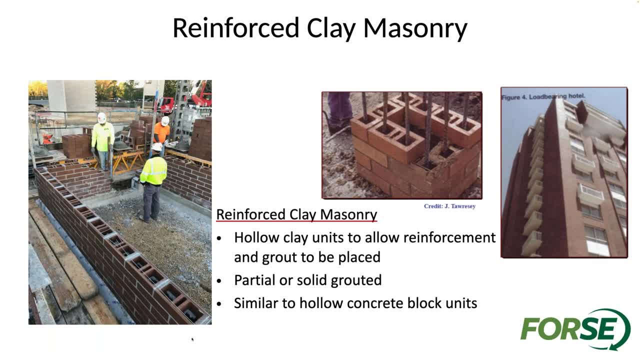 and then a reinforced concrete masonry and then a common brick. So it looks like brick from both sides, but it's got the three different layers- three different layers- to it instead of what could be one. It really could be a reinforced brick design. 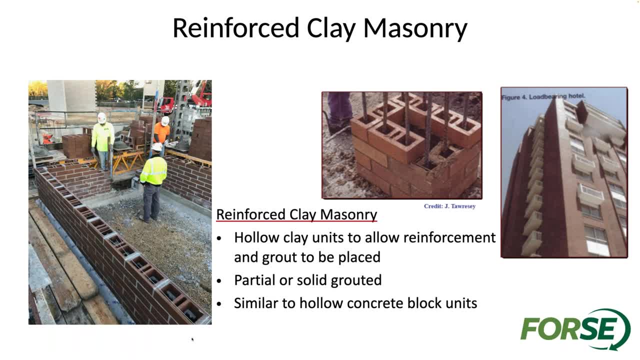 that has one material. You have no layers, you have no different, differing material there. That could be something that works really well. Or if you wanted to have a single white project, you have something that you can do with structure if you want it to look like brick on each side. 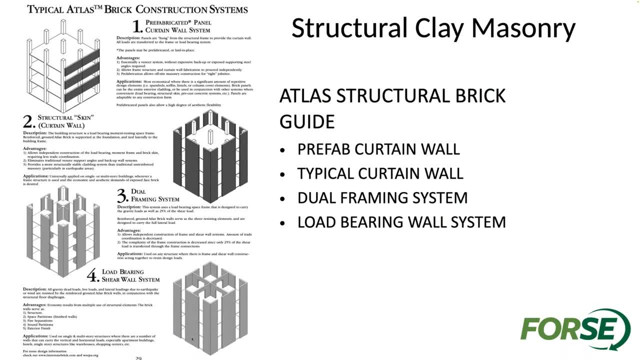 Really there's with the structural clay. I think there's a lot of different options. Atlas is gonna be one of the main manufacturers, There's Belden. there's certainly many others that are available for doing structural brick. But it does, it gives possibilities. 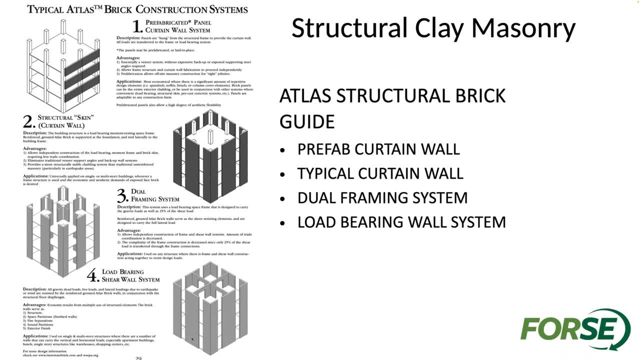 to a lot of different things like prefabbing a curtain wall or curtain walls that go past structures. They point to the different types of options that you have with different designs that are coming out again. architecturally, It really does have, you know, a lot of different options. 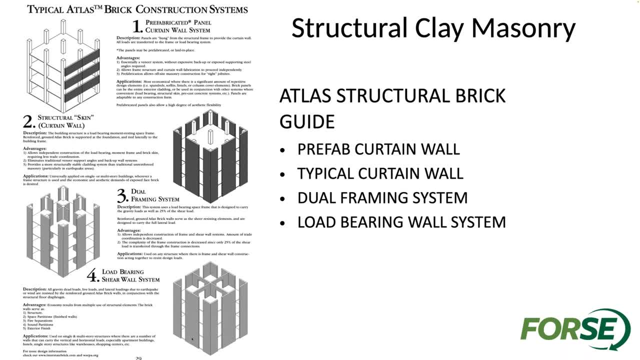 A lot of potential for a lot of projects to be material that we could use to do a variety of different things structurally. So if I just wanted to tie the veneer back just at the floor lines, I did that on a project where we really 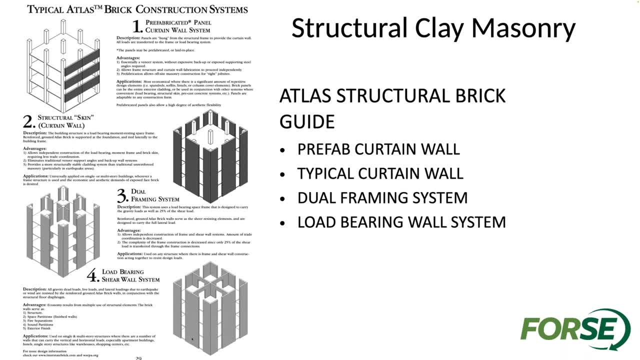 the brick's gonna be kind of self-supporting, self-sustaining. it just ties back the floors. I don't need all the tie backs everywhere, And so that's a very nice option. Sometimes you could use it as structure. You can use it as load bearing or shear walls. 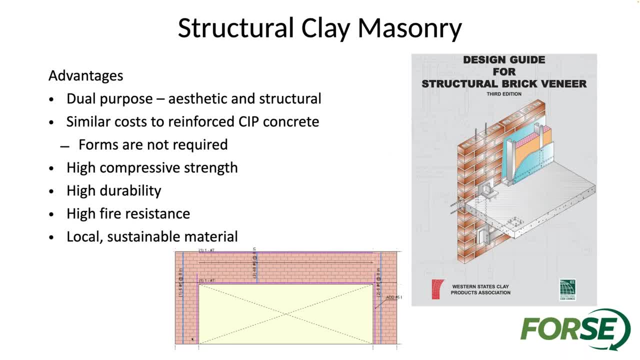 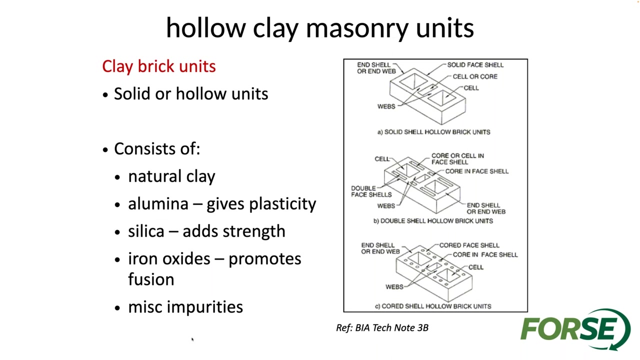 all the different options, You can use it as a. So that's something that's a very nice option for structural clay, Again, they have this design guide for structural brick veneer, which is very nice to be able to use. So again, clay units are gonna be, you know. 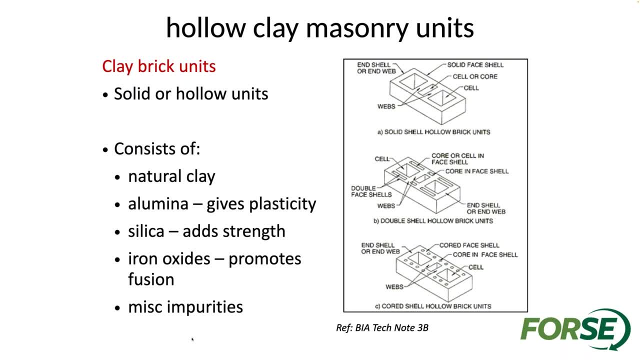 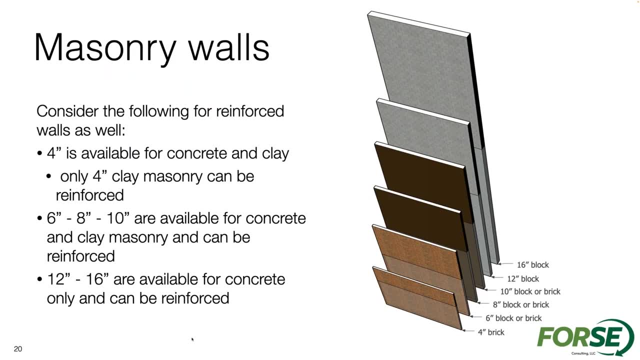 different manufacturers are gonna have again different ways that they're gonna create those elements And obviously it's gonna be starting with clay. So if I looked at masonry walls, I would have the different options that you can see here: Four inch walls that could be reinforced. 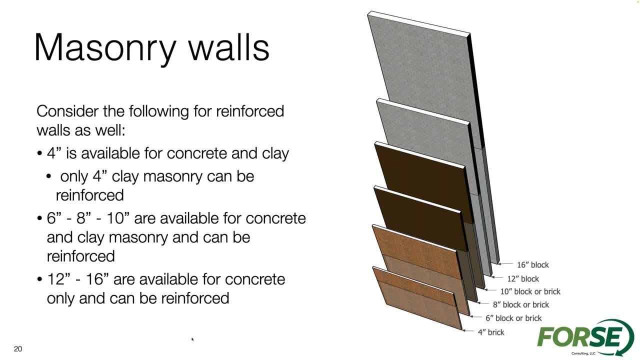 would only be with clay. You could have a four inch concrete masonry, but it doesn't have the space for adding reinforcement. 6H and 10s are really both concrete and clay can be designed. You get into 12s and 16s. really, you can get into 12s and 16s. 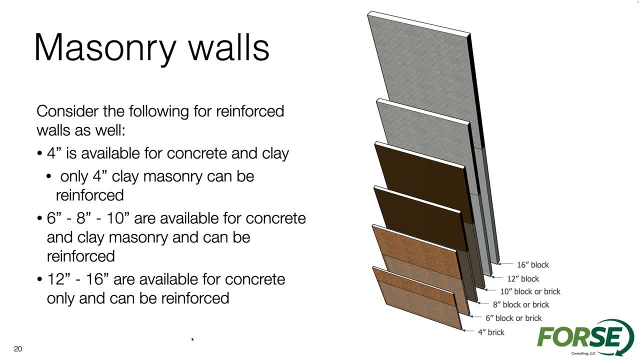 Really you don't have clay units that are that large. It's really then you're gonna be into concrete design And then obviously different heights that are available from there as well. So masonry walls and thicknesses certainly really come down to the unit sizes. 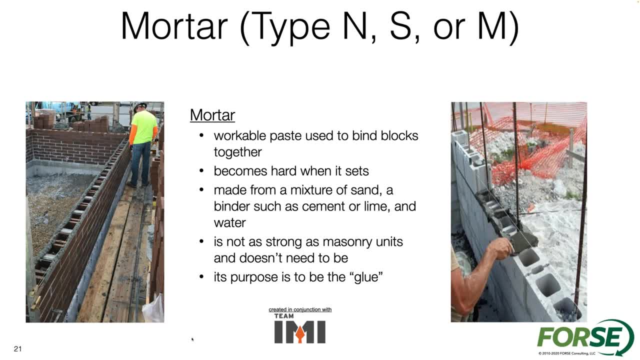 Other material. mortar is gonna be the other material that you can see. right, You have most of the wall. you know 90% of the wall is gonna be the units. What you're gonna see between the units is gonna be the mortar. 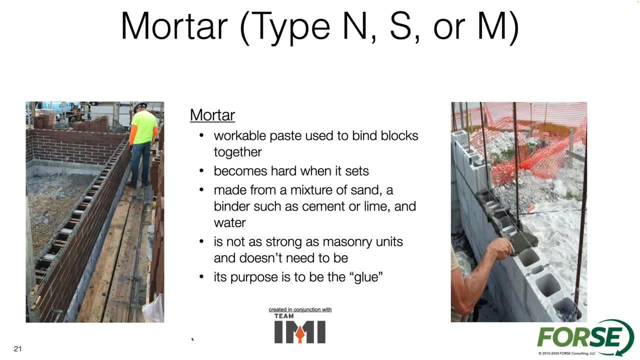 It's really meant to be a glue, something that binds the different blocks together, So it's a mixture of sand, cement and lime and water. It's not as strong as masonry and it really doesn't need to be. It's something that's just in these confined spaces. 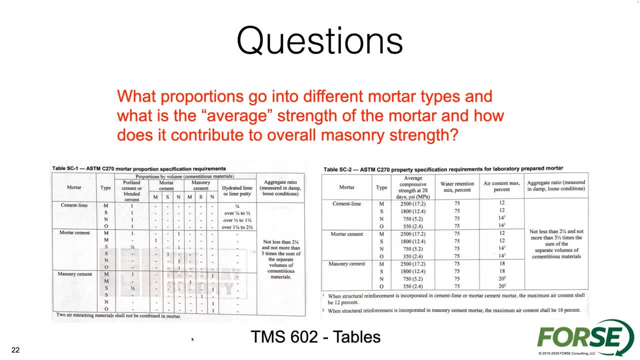 What are some of the different proportions that go into the different types of mortar? So again, you have the cement line, you have mortar cement, masonry cement, all the different types of- you know- concrete that's gonna be added to the different mixes. 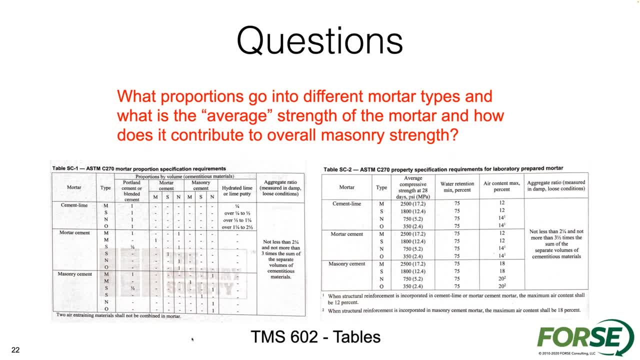 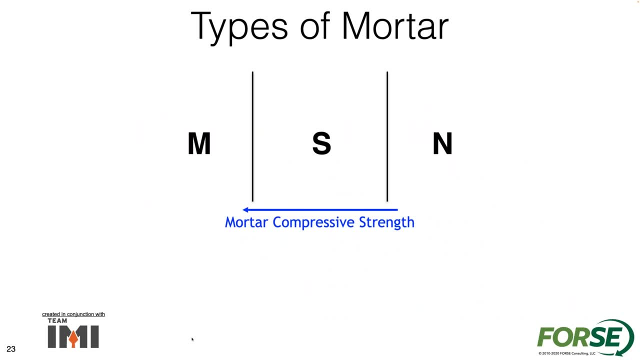 mortar, cement and then, like I said, water. So just some of the different values there. But really, when it comes down to design, we really wanna look at again the type M, S and N. You know, as a designer, you know. 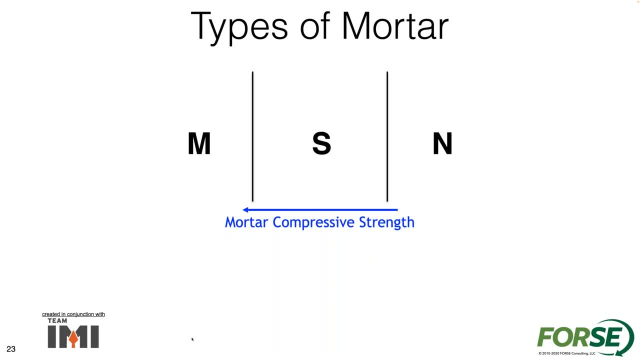 I tend to gravitate towards the left, right. I like the mortar compressive strength to be higher. Really, that's gonna be a value that maybe is overplayed a little bit because the overall assembly strength really, if I look at the unit strength method, 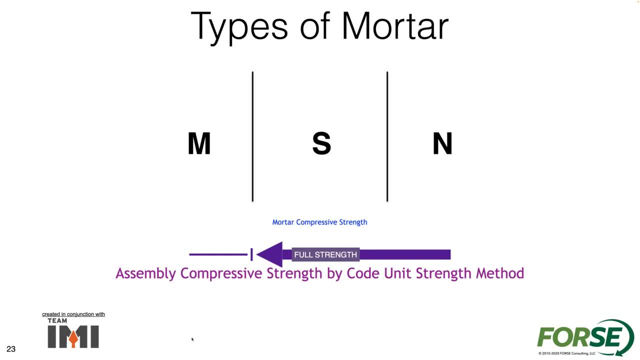 the method that's in the code for determining the overall strength of the walls. type N is weaker. type M and S are really the same, So we come to full strength with type S mortar. Really, what that does is it really says, you know? 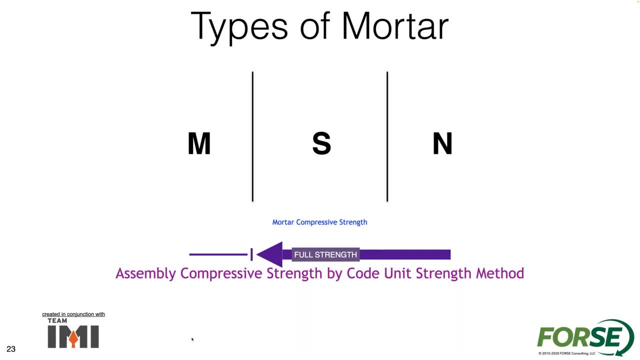 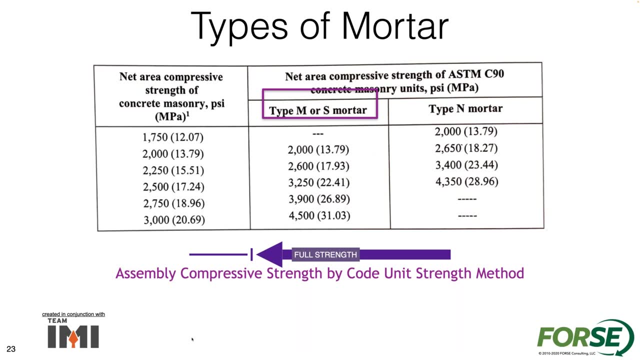 you can use type M, but it's really not gonna help you with your overall strength, or so marginally that we're not gonna give you any more credit for doing it. So those two are really gonna be kind of equivalent. That's why they're together in the tables. 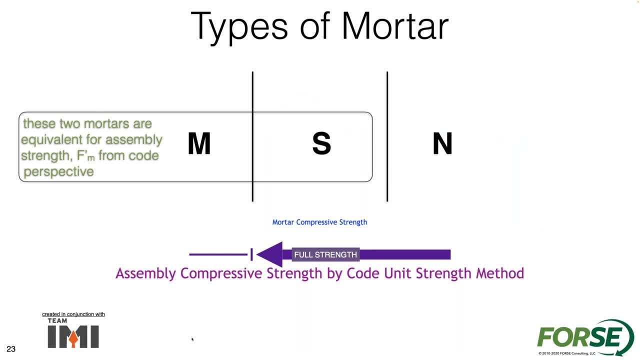 So those two are gonna be kind of lumped together. If I look from a construction perspective- workability, ease of construction- that actually the further I go to the right. So if I put these three mortars up in front of a contractor, 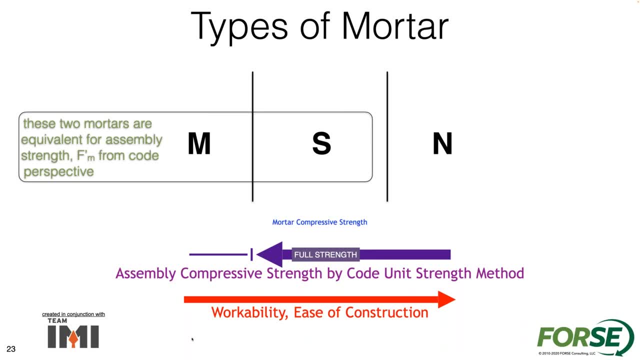 which one would you want to use? They would always choose type N. They would gravitate towards the right. So really, I think it comes down to you know types of mortar, probably what's in the middle. S is a good compromise. 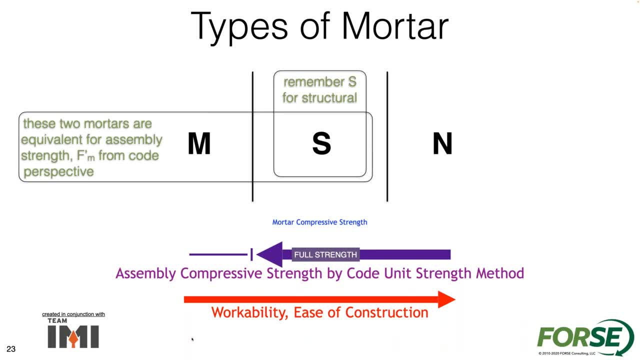 We want more strength. They want more workability. Type S is really gonna give us our full strength in terms of the unit strength method. So I think that's a nice kind of happy medium to live in. We have different, you know, in terms of mortar, you know. 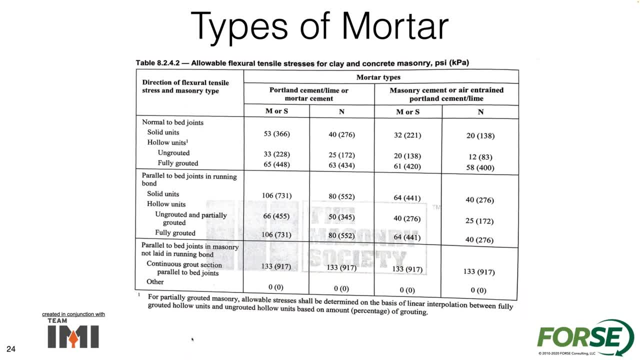 what are the different types of capacities that we have: Tensile stresses for clay and concrete masonry- This if you're designing an unreinforced wall, then you certainly want to get into maybe the different types and the different whether it's a Portland cement or masonry cement. 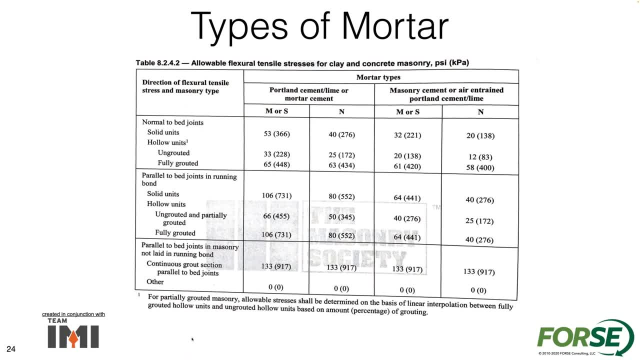 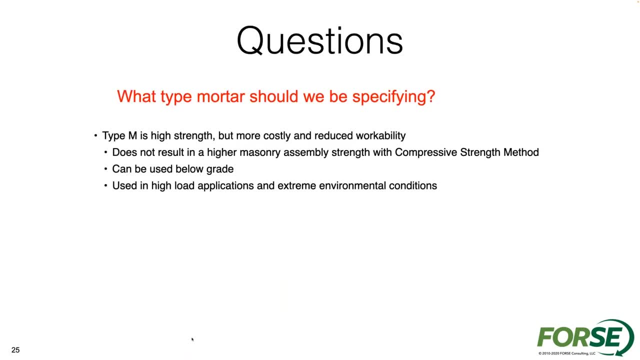 you want to make sure that we have those different types in mind as we're designing, with something that could have tensile stresses, which would be an unreinforced wall. So what should we be specifying? Again, type M is more strength, but usually more costly. 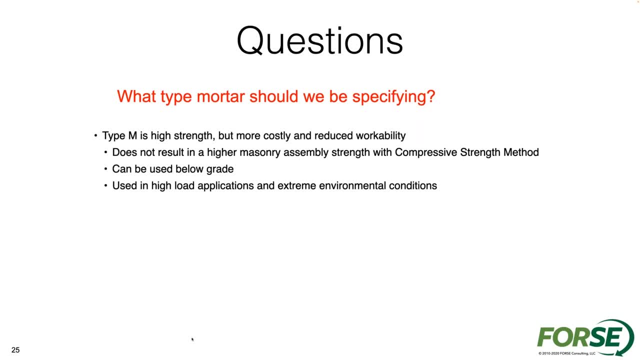 reduced workability doesn't result in a higher strength, unit strength or compressive strength method. It can be used below grade but it's used in higher strength and it's used in high load application extreme environments. I recommend type S for structure walls. 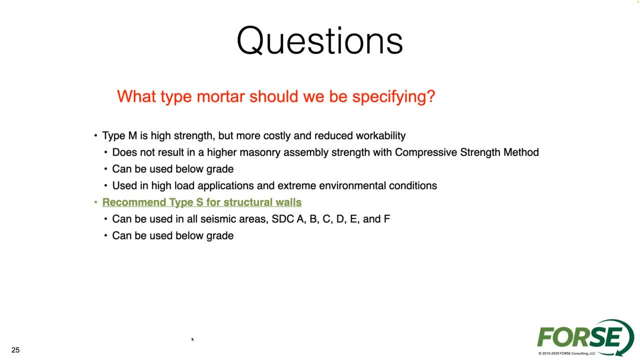 It can used in all of the different seismic areas. can be used below grade as well. That's something that is really really really important to remember. Type N for non structural walls. Veneers usually use type N unless it's a structural. 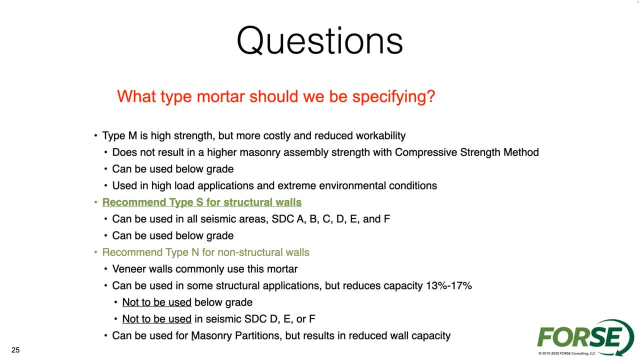 reinforced structural veneer, then maybe we again go back to type S- Can be used in some different applications. It's not Type N, is not to be used below grade and it's not to be used in the higher seismic design categories. 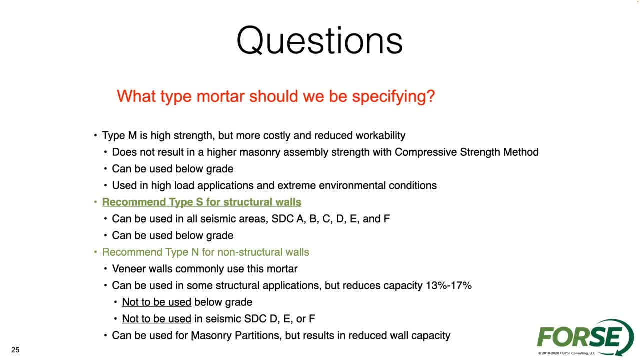 So again, it can be used in mainstream partitions but it results in reduced wall capacity Again. so the three different types. Type S is probably the most common place for most structural designers to sit. Grout is gonna be something that the strength of the grout 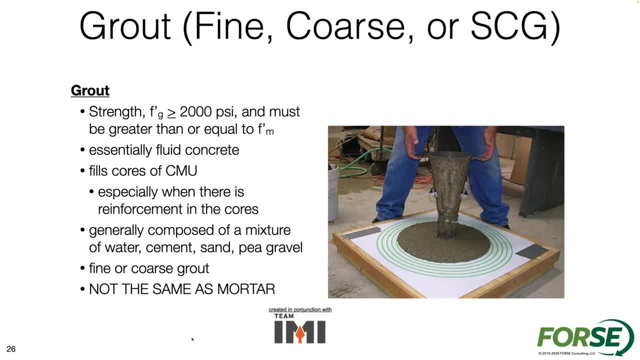 is gonna be an important component to the overall material, but just as important as the strength is gonna be the flowability, because really we want this to be very liquid to flow into all the different confined spaces that you have within a masonry wall. 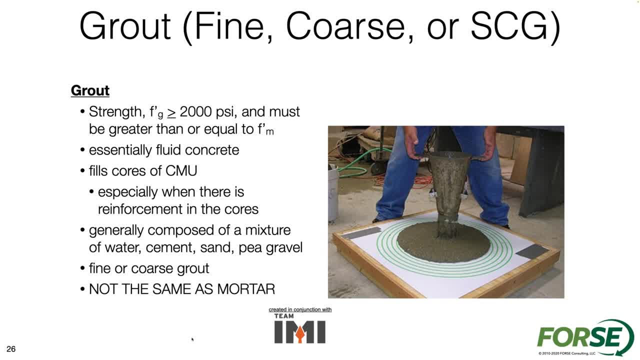 So it's gonna be different than mortar. It's definitely gonna be fundamentally different. Mortar is meant to be a little bit stickier, something that binds to something very quickly, and certainly grout is meant to bind. but you certainly need the flowability. 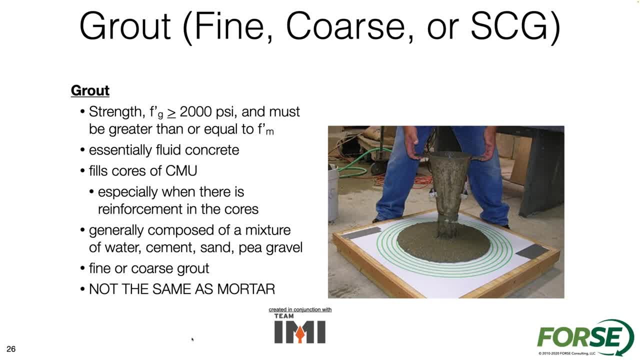 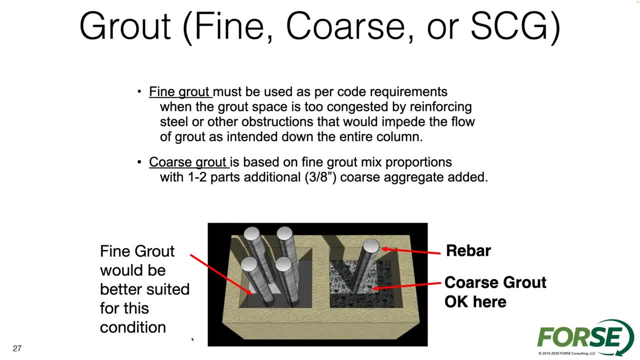 to be one of the primary functions of the grout as it's flowing in these spaces. Looking at the different types of things- I mean just looking at the spaces here- you can see fine grout would be something that you'd want to use anytime that you have. 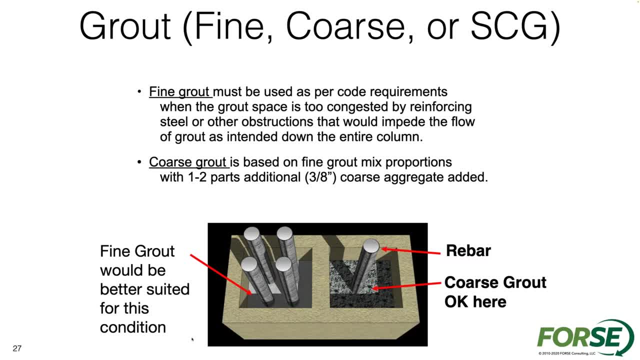 a fair amount of reinforcement within a confined area. Fine grout would be something, and there's certainly there's different requirements as to when you can use fine and coarse grout, based on clearances. Coarse grout is probably gonna be the more common. 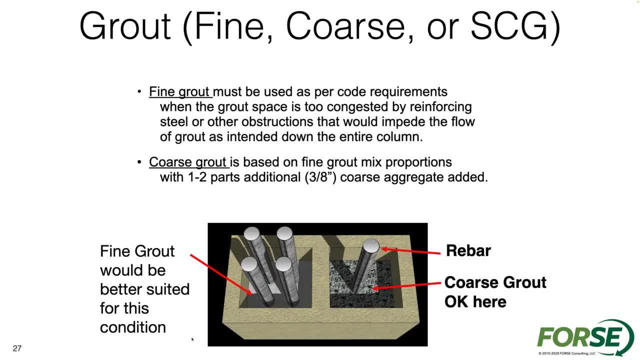 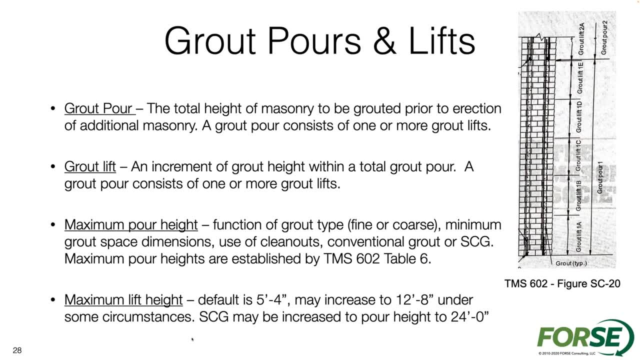 Hopefully we have typically a single bar reinforced designs Within the cohort. there's a number of different types Within the cohort. it also points to grout pours and grout lifts. making sure that we have. maybe the lift is gonna be what we define. 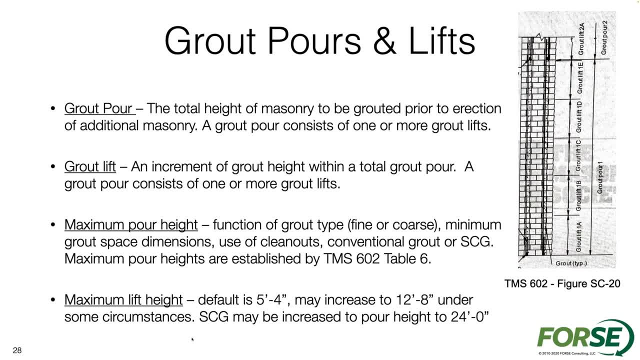 as low lift grouting five foot four, You can get it increased to 12 foot eight under certain circumstances with clean outs and a lot of space to use, and self-consolidating grout could increase your pour height to 24 feet. 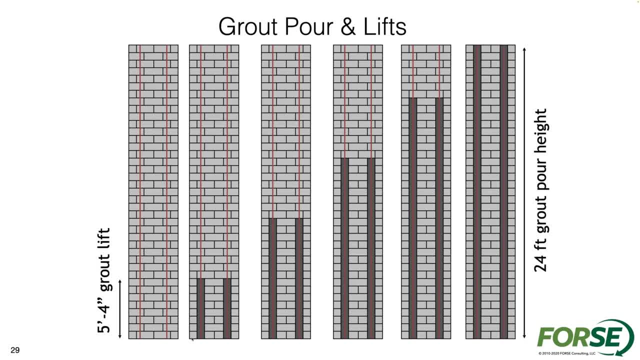 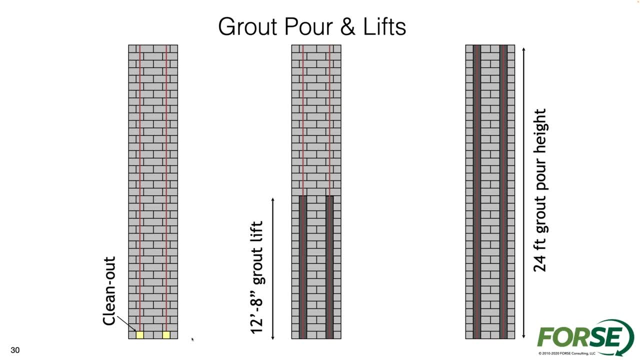 All this pour height, pour lift. a lot of this stuff is really meant for contractors to be reviewing the different pours pour heights that we can consider. Adding clean outs certainly adds a lot more ability to add more and more to the lift and, like I said, self-consolidating grout. 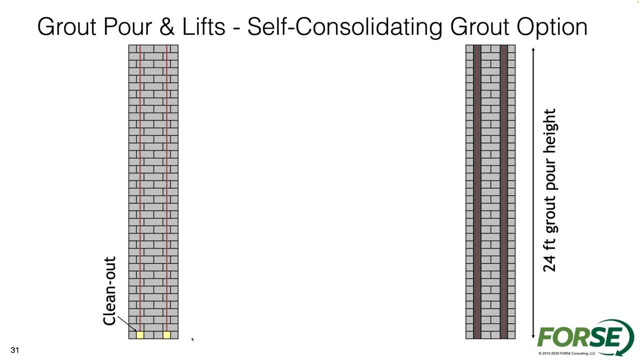 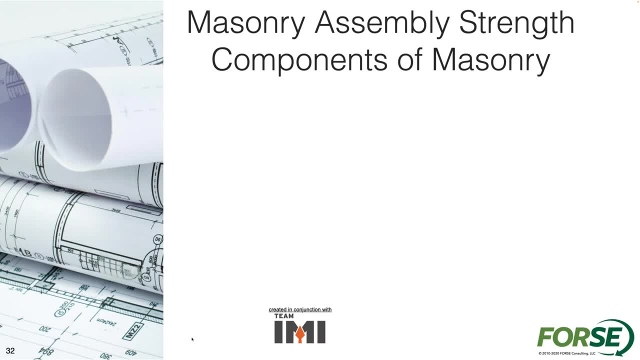 being the one that can go all the way to 24 feet with just a clean out at the bottom, So that might be a really, really nice option for contractors. So if you look at all the different materials- the block, the mortar, the grout- 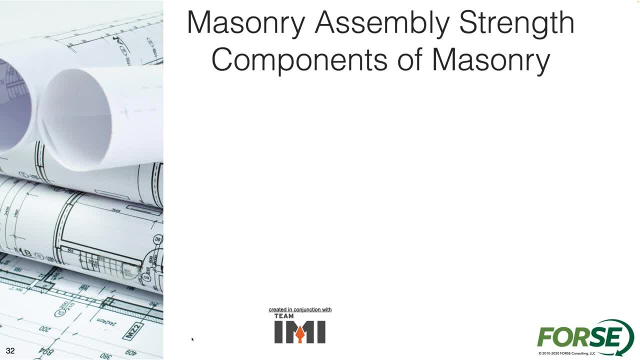 one of the things that I try to point to is: you know, people are specifying these different materials for projects. is I recommend not just saying F prime, M is equal to a certain value? Really, what we want to do is we want to call out. 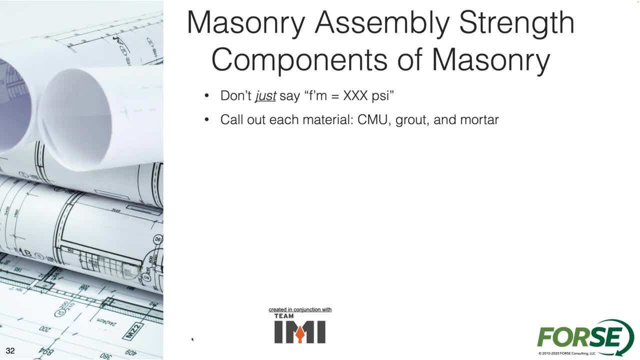 each material, the different properties of each material and the different strengths of each material. So, as an example, what I would point to people is putting an overall assembly strength F, prime M of 2,500, but then specifying your block strength to be 3,250 or greater. 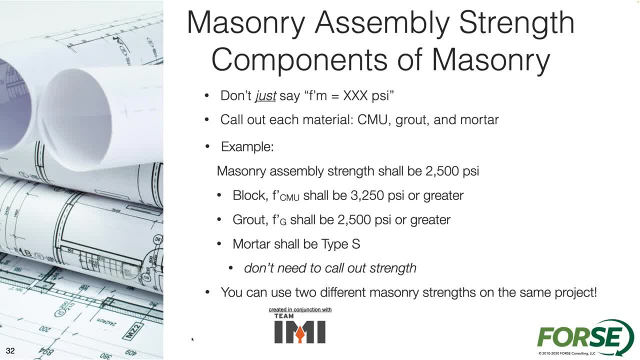 and then your grout strength to be 2,500, because that's your F prime, M or greater- and then your type S mortar, And once you define your type of your mortar, you don't have to define your strength. So that's gonna be the two different. 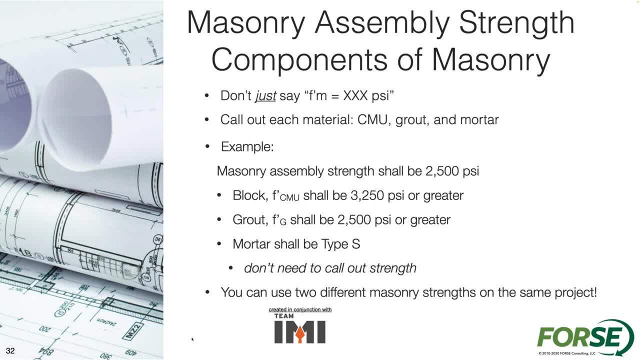 So, and then you can also have different strengths in our same project. I mean, that's something that we certainly can do. We do that all the time for concrete. But, just like for concrete, we want to be careful as how we store material, so on and so forth. 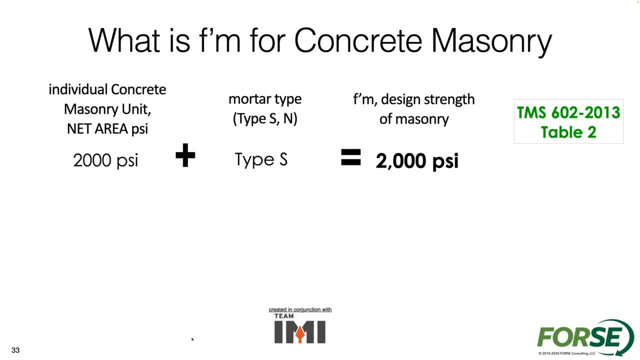 when we, if we, would do something like that. So for F prime M, the D is equal to 2,500, and D is equal to 2,500. So for F prime M, we want to be careful for a concrete masonry. again, if I boil down all the tables into a really simple chart here. 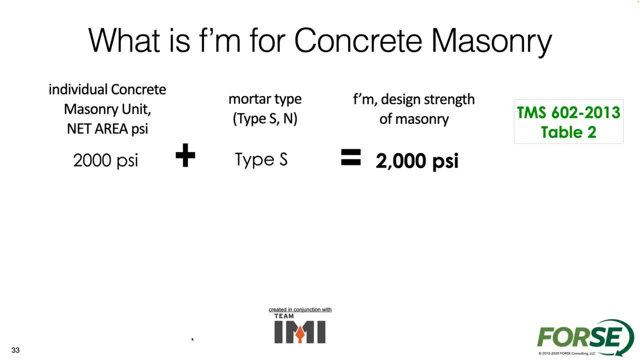 if I put 2,000 PSI blocks with type S mortar, I get an F prime M of 2,000.. So again, that's our minimum With the 2013 code and beyond. that's our minimum design If I have blocks of 3,250. 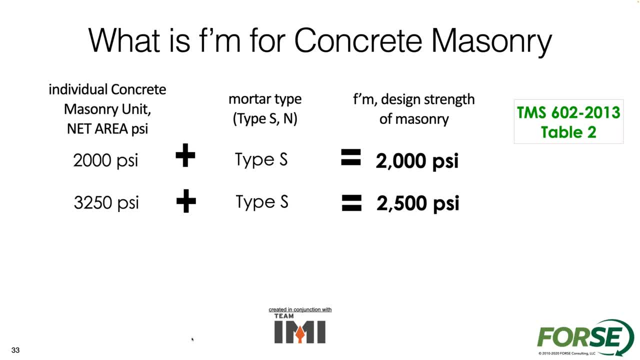 type S mortar and 2,500, then I have a strength of, like I said, 2,500, 4,500 PSI for the block to get to type S, to get to 3,000.. Really, it's the one in the middle That's going to be our. 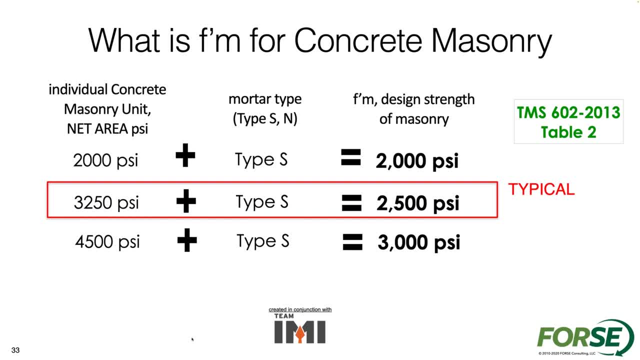 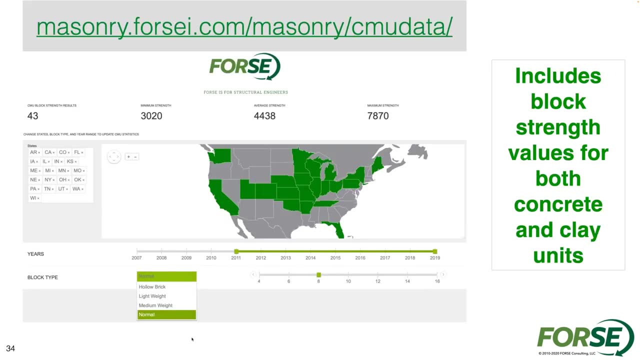 typical design strength across the country. And so when I started talking about masonry design 10, 12 years ago, really kind of pointing people to this fact that people really wanted to see some data, So what I did was I created a website. I actually started crowdsourcing some of the 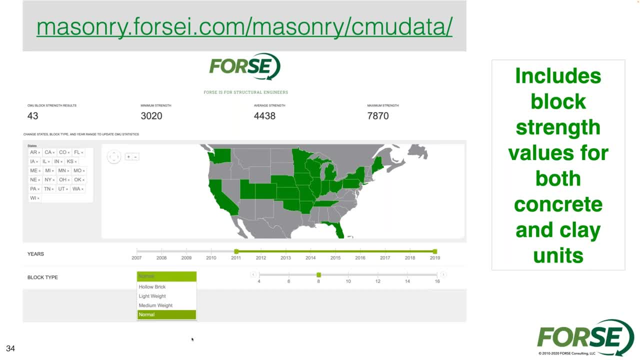 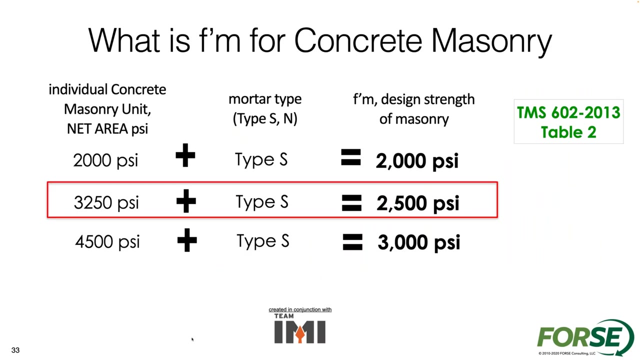 different strength that I was getting for blocks. So this is a normal weight block, eight-inch block, And these different states. you can see the minimum strength of 30-20,, the average strength of 44-38, maximum of 78-70.. So again, if I go back to 2,500, that 3,250, that's something that's met. 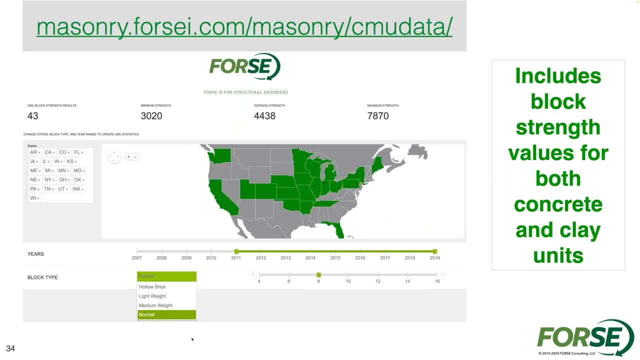 most of the country with normal weight block. That's something that we can achieve pretty easily across the country. You get into medium weight, light weights, You get into different thicknesses, all those different things. you can check on this website Or you can just call the different block suppliers that are going to be used on your 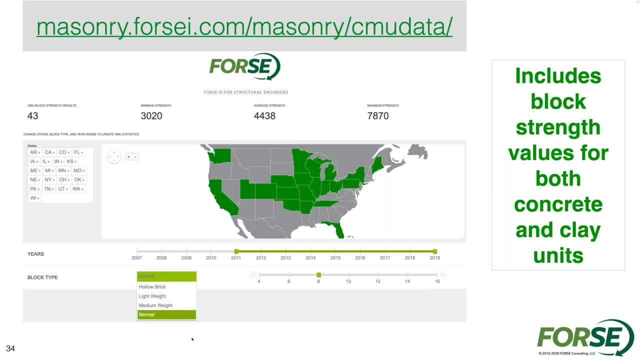 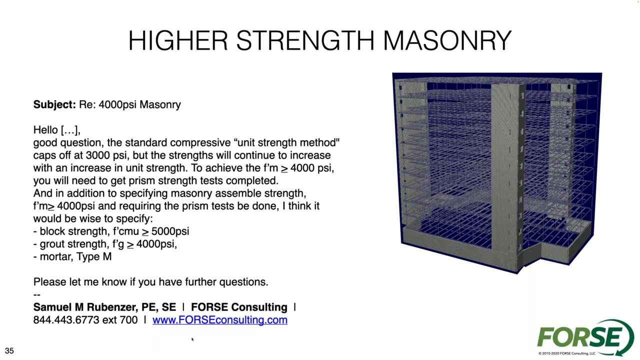 project or the different block suppliers in the area to see what the actual strengths are. Anytime that we want to go to a higher strength, I think that we can go beyond what was even a unit strength method. We could get to that frame of 4,000.. But to do that we certainly need 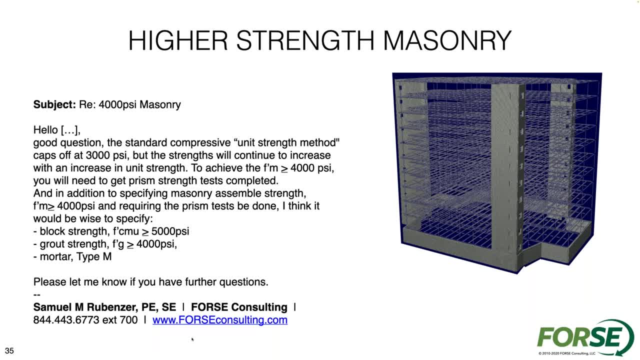 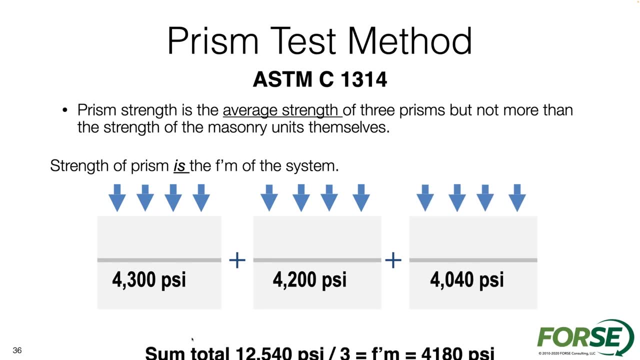 to use higher strength block, maybe type M mortar. Really, you're going to have to to define higher strength elements, But more than anything, you're gonna have to then specify a prism test method to make sure that we have three different samples and the test between those. 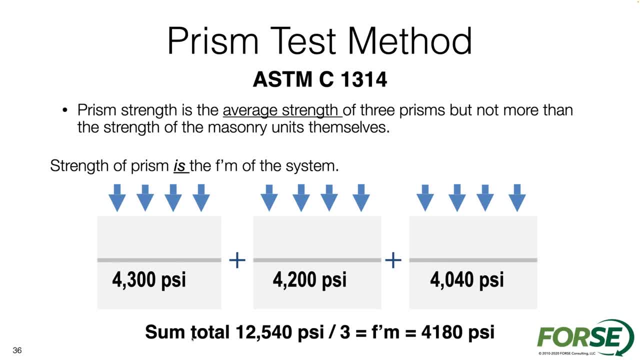 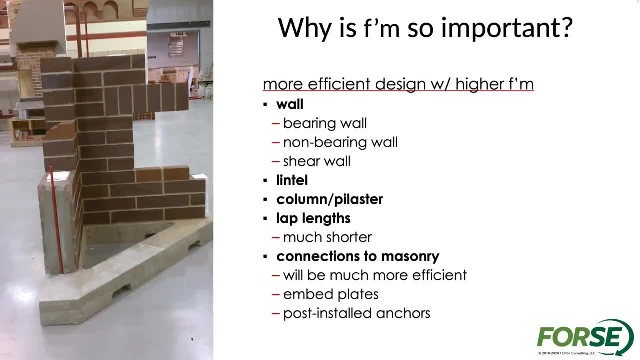 three different samples. we average them out to make sure that we get a higher F prime M. that could be up to, like I said, 4,000 for our strength design provisions. Why is F prime M so important? It's important not just for the wall design. 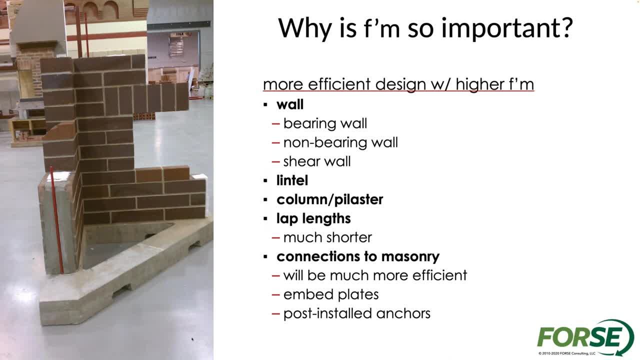 You know the small differences in wall reinforcement can make a huge difference in materials and stuff that you'd use throughout our design. But lintel designs the depths of lintel, sizes of lintels, columns and pilasters reinforcement that you would need. 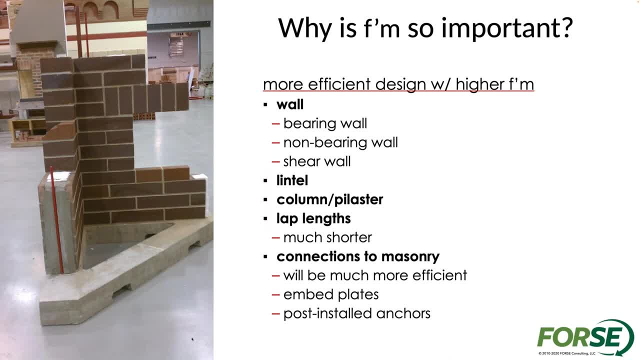 Lap lengths are a lot shorter when you have a higher strength- F, prime, M- And then connection to masonry. Anytime you connect to a masonry wall, usually the controlling parameter in the connections to masonry walls is gonna be the actual masonry strength. 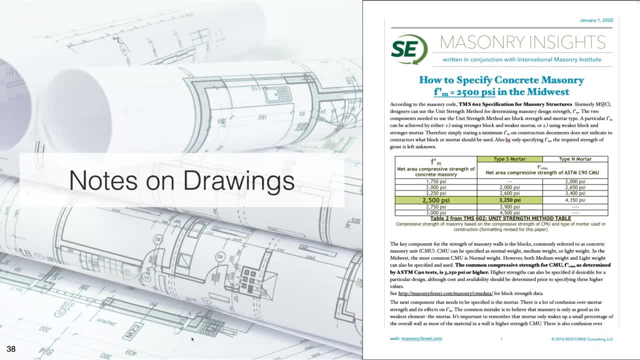 So I actually put together a little white paper a couple years ago and I think this could be kind of useful. It really kind of spells out all of that stuff, This stuff, all these papers that I've put up here. by the way, I'm not selling any of these. 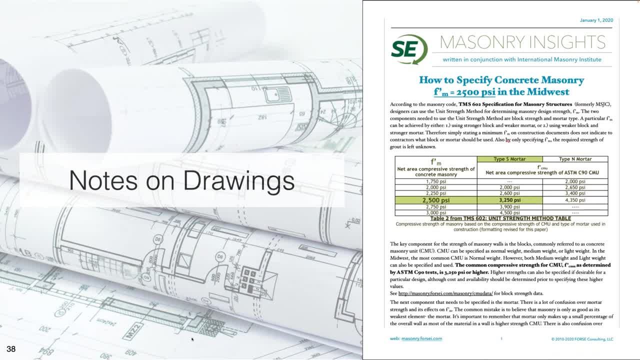 These are all free to download. You can certainly grab those. I could actually send some of these PDFs as kind of a follow-up to the presentation today. So this is one for concrete masonry In the Midwest. it's kind of what I typically see. 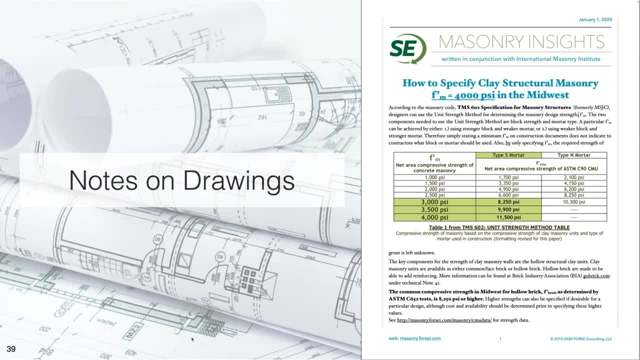 how to get to the F prime M of 2,500.. And then for clay, also pointing to the fact that it could be three to 4,000 pretty easily with most of the common clay elements that are out there. The other materials that we want to point to: 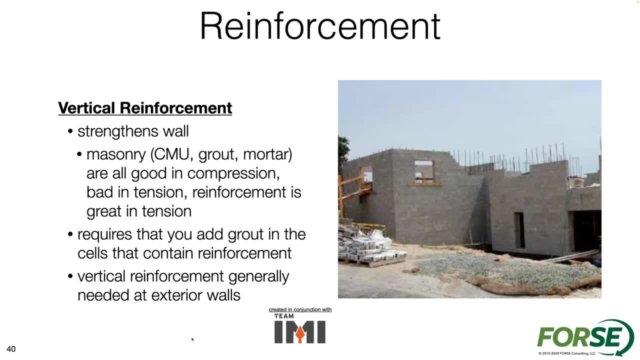 with the materials in masonry. So reinforcement, obviously reinforcement's gonna be added. It's gonna strengthen your wall quite a bit. You have the blocks, the grout, the mortars, all that are all creating compression but not so good in tension. 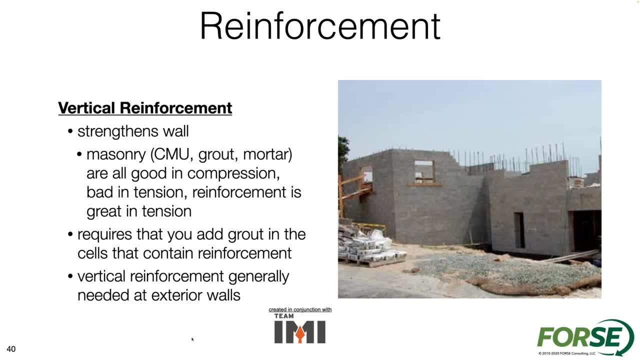 So obviously reinforcement's what makes your wall quite a bit longer, stronger, because it has that tensile, high tensile strength. Every place you put reinforcement, obviously you need to put grout, Grout's kind of that mechanism to create that internal moment arm between your compression block. 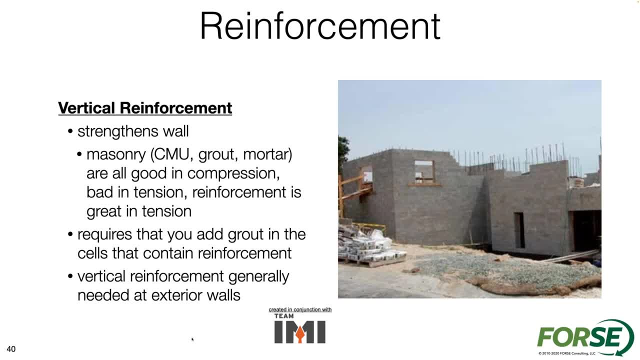 in the masonry and your tensile force in your bar, So grout. that's why grout's obviously, obviously really important to be consolidated, to make sure that we can find, contain and bond to the reinforcement and the masonry as well. 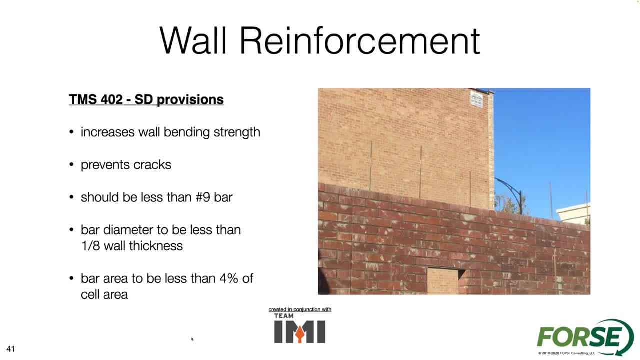 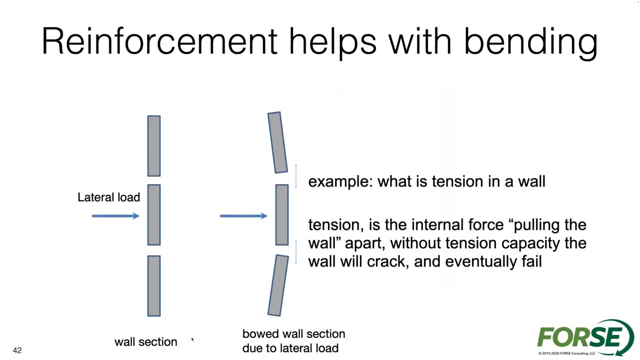 Again the strength design provisions pointing to number nine, bar the number 11 in the new code, but then also some bar diameter to wall thickness limitations and then a bar area to be less than 4% of the cell area- Right, because we're adding the reinforcements. 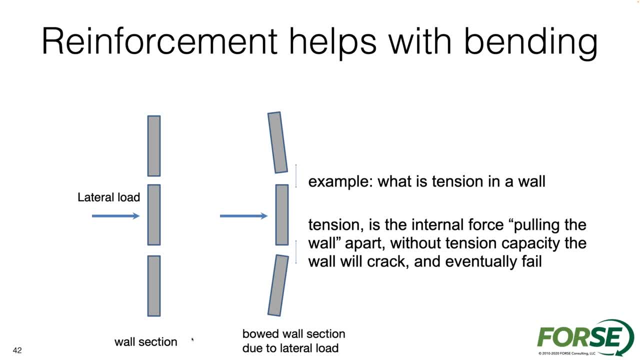 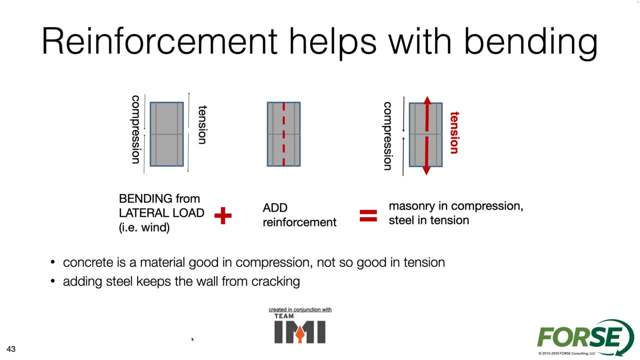 so that when you put a lateral load on the wall, that tensile force that you have due to the bending in the wall is taken by the reinforcement right- Kind of some pretty rudimentary illustrations for why reinforcement's important. And then what I wanted to do next is I wanted to put together 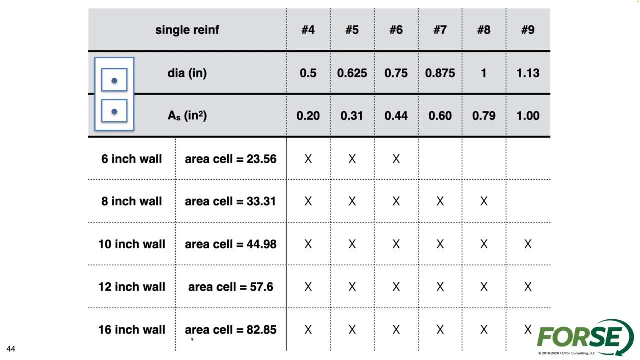 a couple different tables. You know when we had some of the different reinforcement provisions, what does that look like? So I'm an engineer. I like to throw together spreadsheets, The different wall thicknesses and the different reinforcement options at the top. 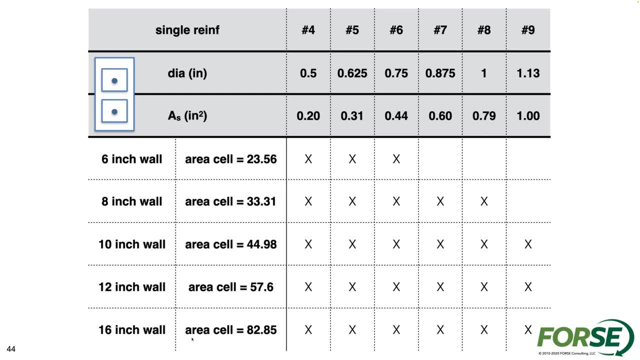 all the way from fours to number nines. You can see where I can use those in different walls. I think it gets a little more interesting when we put in doubly reinforced walls. Really, again, we're dealing with confined spaces. Doubly reinforcing a masonry wall should be done. 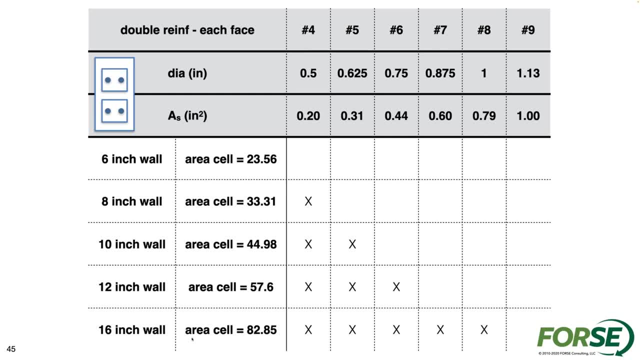 you know, carefully, And we want to make sure that we're not adding too much, too much reinforcement so that it's hard to build. So that's what's shown by the code. The other side of this is: you know, what do contractors prefer? 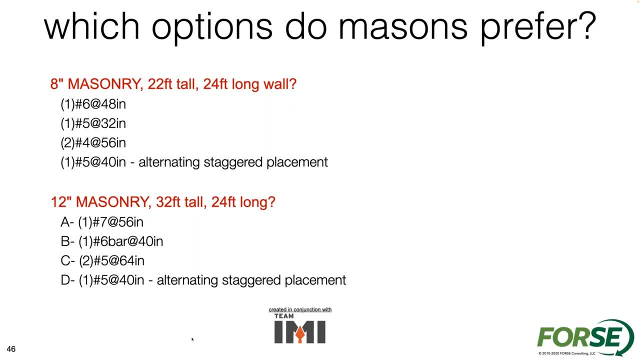 You know, what do masons prefer? So what I actually did was I created a little survey to try to see what different masons would prefer If I had an eight-foot or eight-inch masonry wall, 22 feet high, 24 feet long. 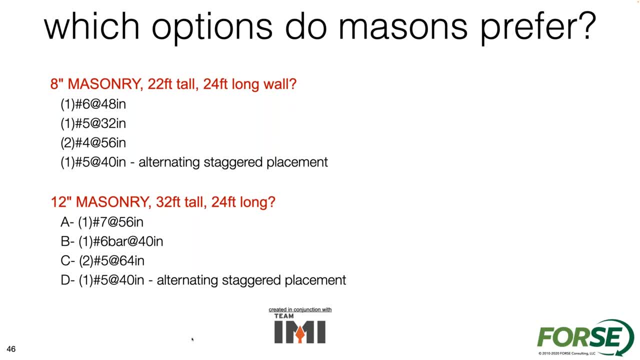 I have four different reinforcing options that have very similar capacities. Which would they rather do? What are they going to build? A six at 48,, a five at 32, so a smaller bar closer together, Two even smaller bars, but this time even maybe a little bit more spacing. 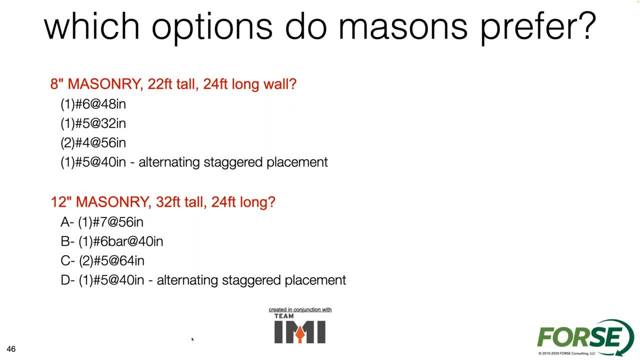 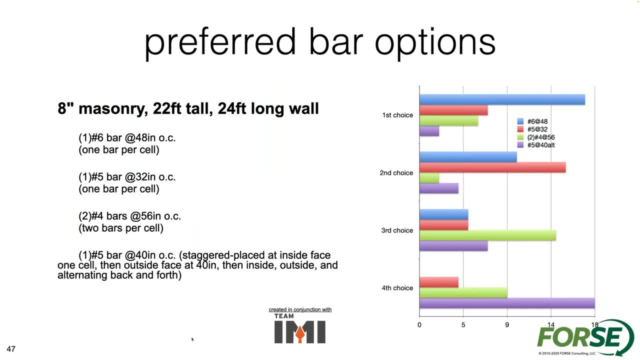 Or a number five alternate staggered reinforcement placement, which is kind of unique, Or a 12-inch masonry wall with the different reinforcement options. So if I look at the survey results I think it's kind of interesting. You know, for masons you know that eight-inch wall. 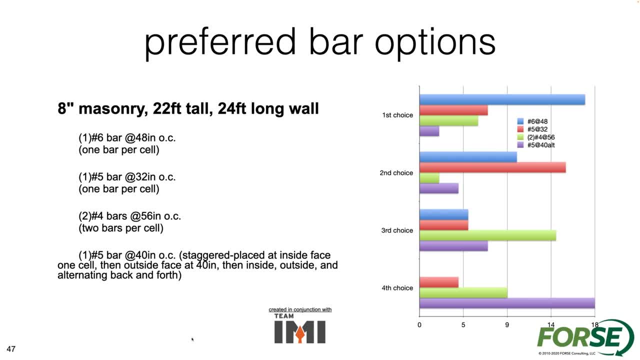 you know the larger bar at 48 inches on the center was their preference, kind of a strong preference. They prefer that much more over the two number four bars, even though that two number four bars would be less grout. They prefer that over the smaller bar. 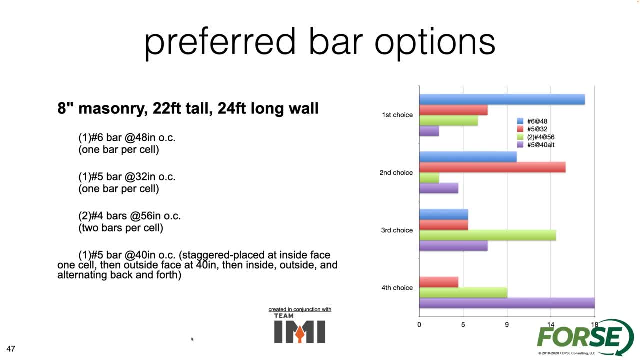 because there would be a lot more grout with the smaller bar. So again, I think that that's interesting. You can see the strong preference in an eight-inch wall for the single bar. for their part, It gets a little bit more interesting if I look at the results for the 12-inch masonry. 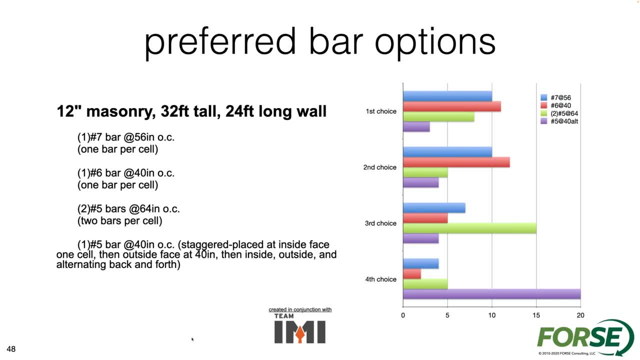 One number seven bar at 56. So again, smaller bars. Number six is at 40, is what's required. Two number fives at 64, something that you know would be even less grout. So kind of similar options, right. 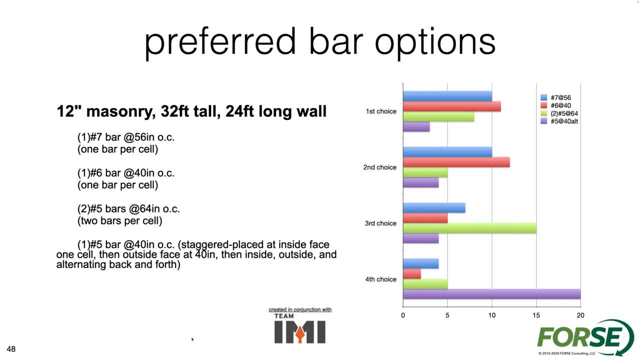 Here you can see a slight preference for the number six at 40, which I thought was really interesting, you know. So they are looking at this and saying: you know, number six bar is really the largest bar that I want to deal with. 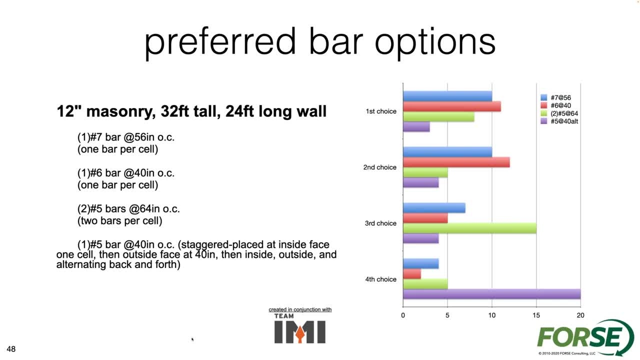 I get into sevens and I start to shy away from it. Even if it's less material, less grout, at the end of the day they would prefer to use a number six Again, cost-wise, maybe cost the seven at 56. 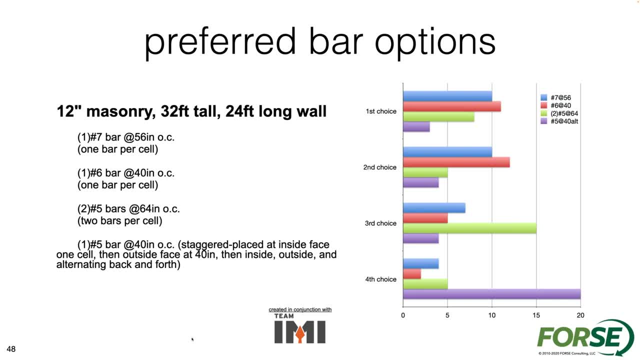 is what costs a little bit less, So maybe that's what they go with. But I think that that's interesting. You know, when you deal with what masons want to build, four, fives and sixes are the preference. You get into sevens and they start to get. 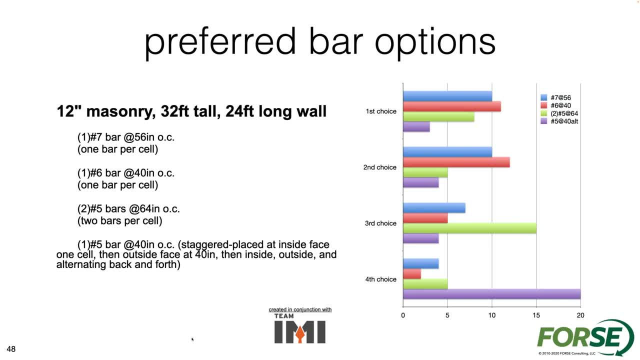 a little bit gun-shy, Get into eights, nines and, like I said, all the way up to a number 11.. Obviously, they're going to have some concerns with placing some of those very large bars within a masonry wall. 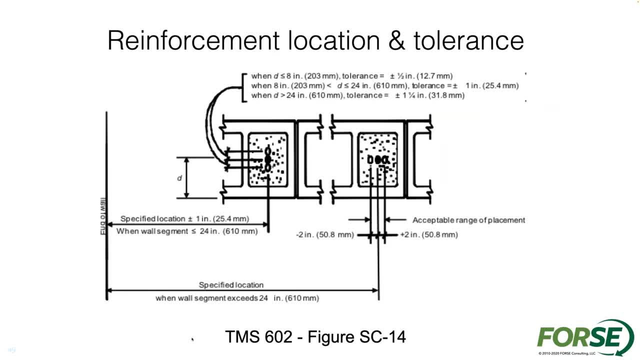 This is that little image that I pointed to before when it was added to the code. This is a great little detail to add to your standard notes and details specifying where the reinforcement can be. Again, when it's eight inches thick, the bar can be a half inch off-center. 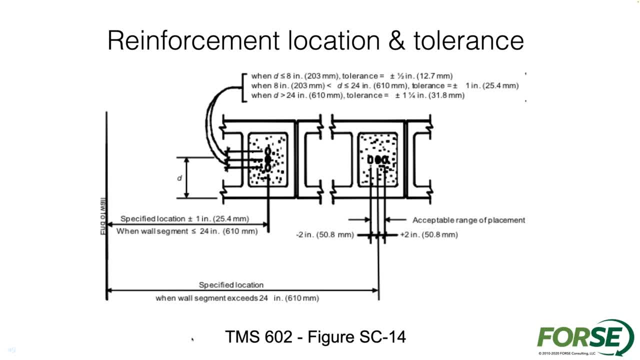 It can be plus or minus a half inch. If it's a 12-inch wall, it really can be plus or minus one inch. So that's a really great information to have that your bar doesn't have to be exactly at the center. 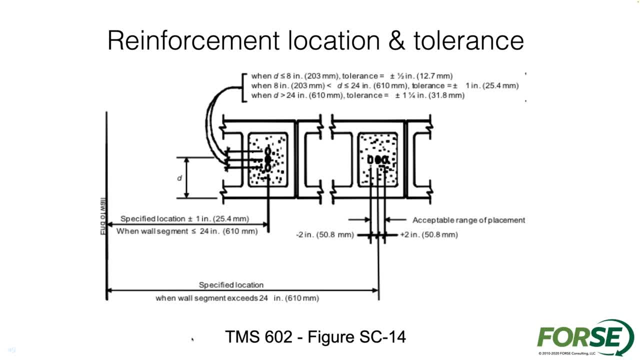 and you'll still have the same capacity for your wall. So that's really important to realize, kind of where the bars can be placed within a masonry wall. So it's a very nice detail. You get into a little bit more about the lapse. 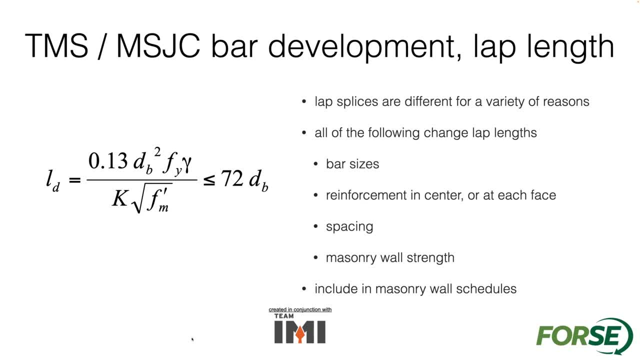 of reinforcement. Again, I said, different things make the lapse shorter or longer. So that's a really great information to have. So that's a really great information to have. So they are different. Obviously, they're going to be longer the larger the bar is. 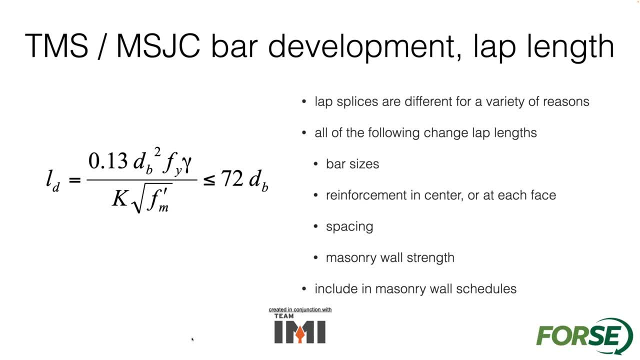 But if we have a higher strength of masonry that we're considering, that's going to make the strengths lower. Really, I think it's pretty easy to take this equation, drop it into a table. We can see pretty quickly where the number three's. 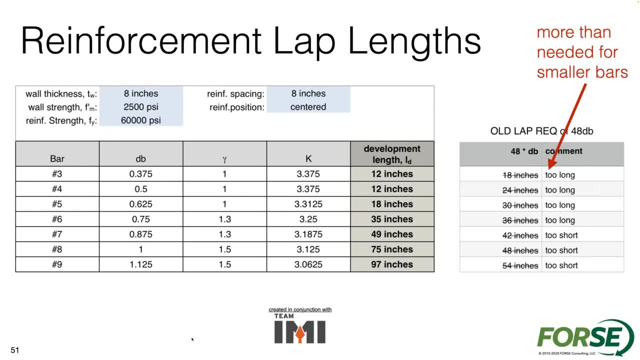 number four bars have pretty short lapse. This is an eight-inch wall, 2,500 psi. You can see what some of the different lap lengths are. So I also want to point to the old reference of 40 bar diameters, Certainly for the smaller bars you 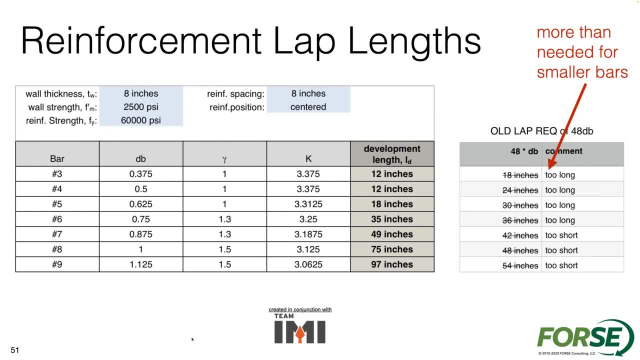 have too long of a lap, that's required, But some of the larger bars you have too short of a lap. that's referenced. So it's not necessarily the just save material but to make sure that we're more accurate based on current test information, where 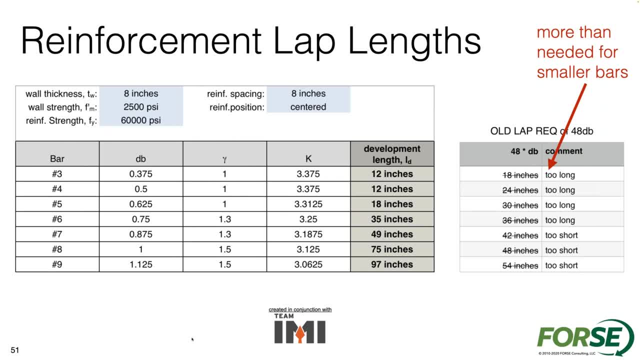 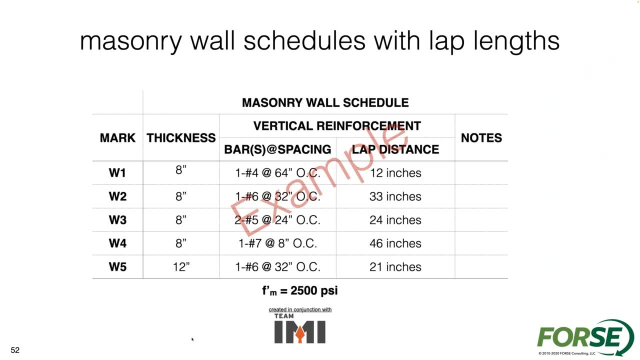 we are with lapse design-wise. The other thing about lap lengths is- I think it's something that could be added to schedules- Reinforcement. lap lengths can actually be different for the same size bars. So here you can see the W2 with the one number six. 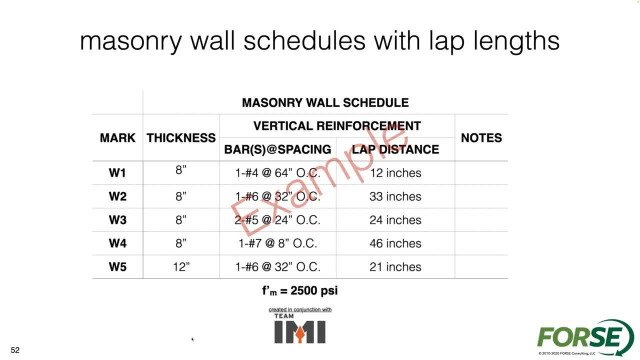 at 32 inches on center, that's a 33-inch lap because it's in an eight-inch wall. One number six at 32 inches on center in a 12-inch wall would be 21 inches, I think if W5 is the most common wall. 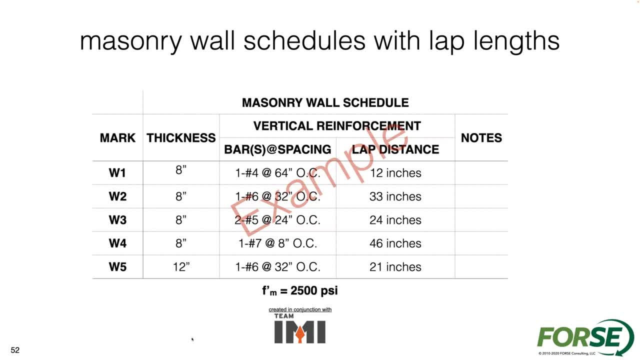 making your lap at 33 inches is probably not that's a lot of you know- 21 inches But 12 inches of extra bar every place that you have a bar. So I think a schedule is just really good and it helps create a lot of clarity. 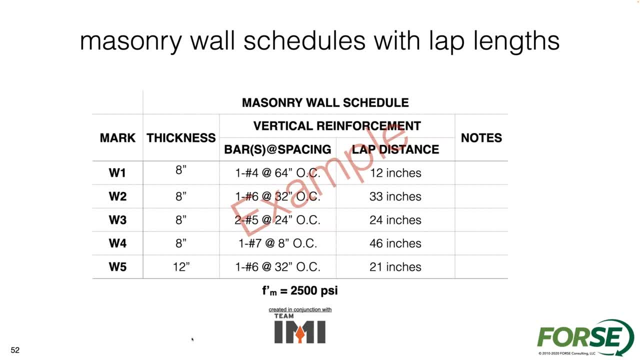 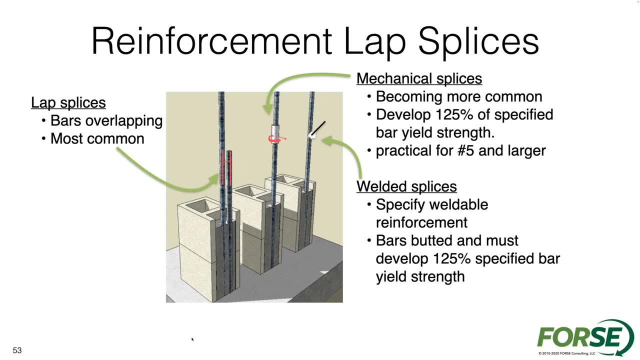 over what the actual laps that are going to be required for different areas. Other things about reinforcement lap splices can be achieved in different ways. I've had mason contractors that have preferred lapping bars over mechanical couplers. I've had some of them prefer mechanical couplers. 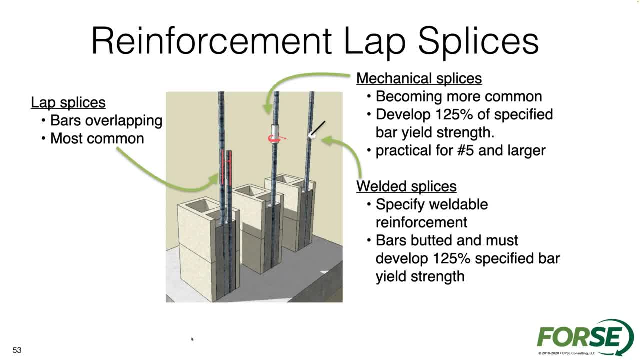 Recently I've had a few. I've had mason contractors that said: hey, we know how to weld, Let's just weld the reinforcement. So obviously you have to have weldable reinforcement, But that's a very nice option for lapping reinforcement. 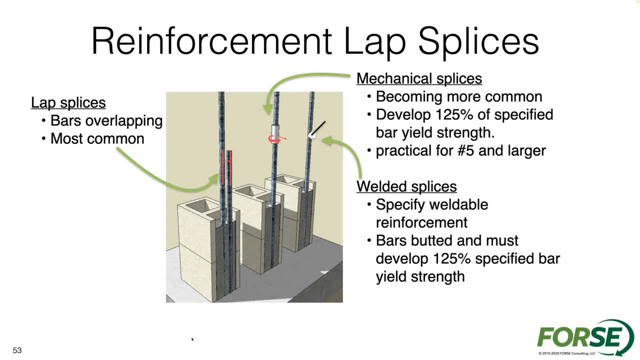 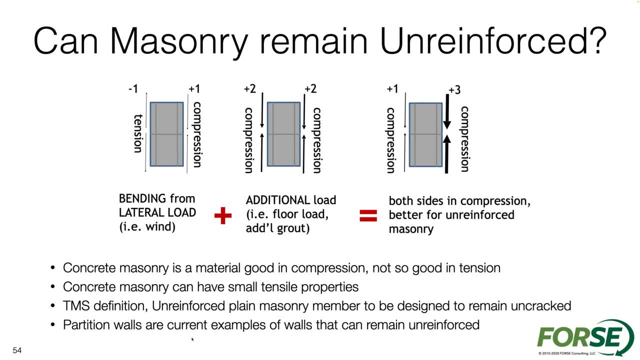 You have different options that can be selected there. If I get into reinforcement, you know, I always like to step back here and say: you know, hey, you can have an unreinforced masonry wall. Masonry can be a little bit heavy. 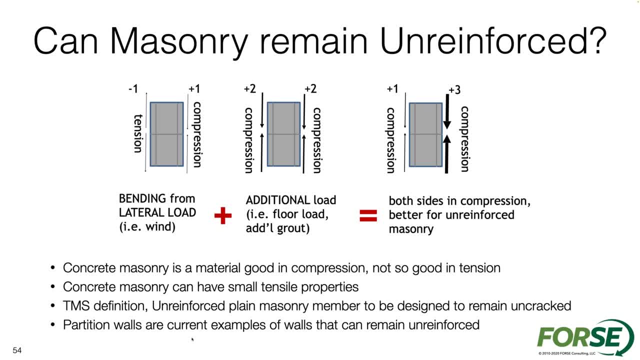 So that's one thing that really does help it, Because if you look at the different bending loads, certainly any time you put a pressure load on a wall, you have a negative side, that's in tension, You have a positive side, that's in compression. 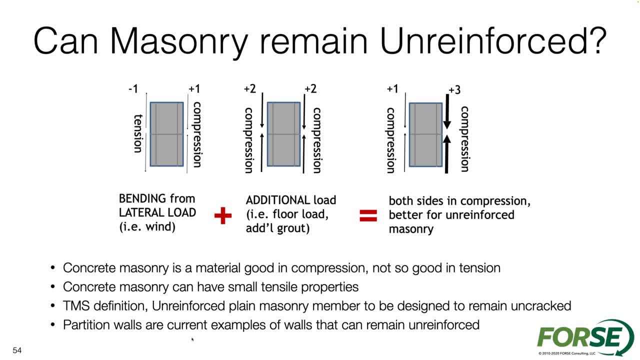 from the bending force. But if my wall weight is actually sufficient that I actually keep both sides in net compression, one's going to be more compression than the other. certainly you can have an unreinforced wall, Or if it's in mostly compression and then very minor tension. 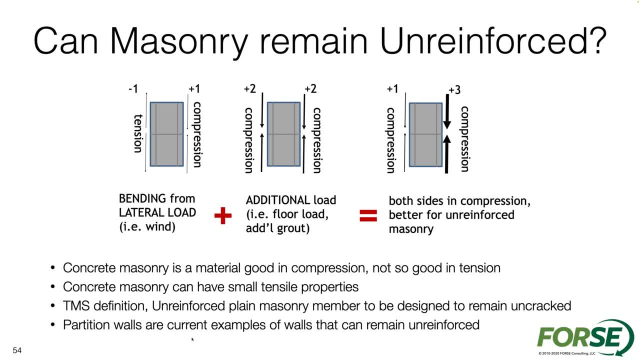 you can still have an unreinforced wall. So it's really important to remember- And this is, like I said, important for partition walls, walls that really don't have a lot of load demand or lateral load demand. A lot of times it's pretty easy to keep both faces. 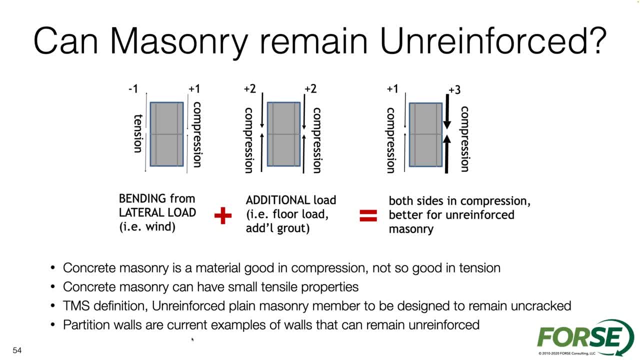 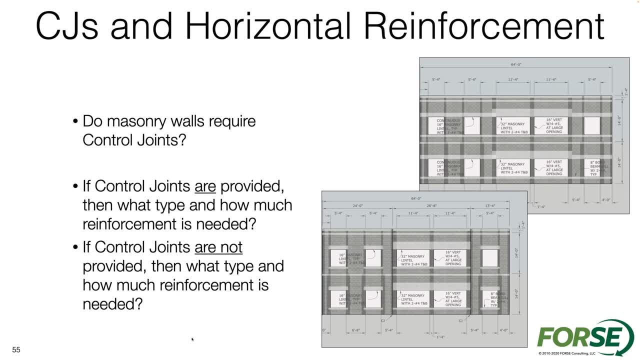 in compression and have that design still be valid. The other thing about reinforcement: so you don't have to have reinforcement. When you do have reinforcement, horizontal reinforcement is reinforcement that we like to add to walls. Horizontal reinforcement really does keep the horizontal stresses from getting too high. 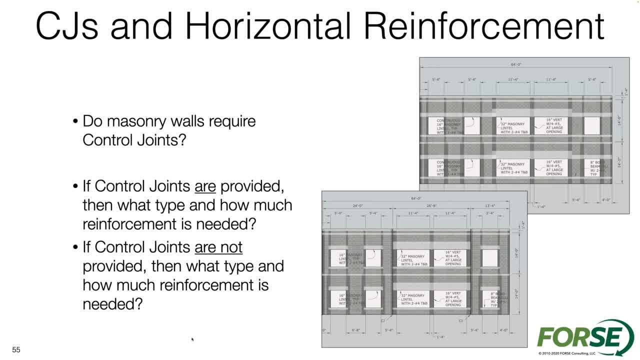 due to temperature changes or shrinkage in concrete Could be different reasons why you have horizontal reinforcement to prevent some of those cracks from occurring. There's different levels of horizontal reinforcement that you'd want to add. You can add a minimum amount of horizontal reinforcement. 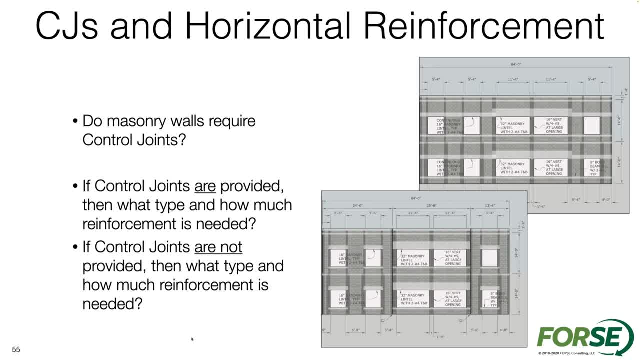 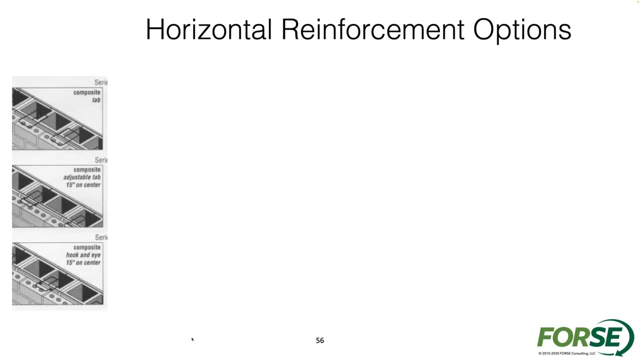 and add control joints. Control joints are joints that are placed within major walls to relieve some of the stresses that might be accumulating due to, again, shrinkage in temperature forces in a wall. You could also add enough reinforcement so that you don't have to have control joints. 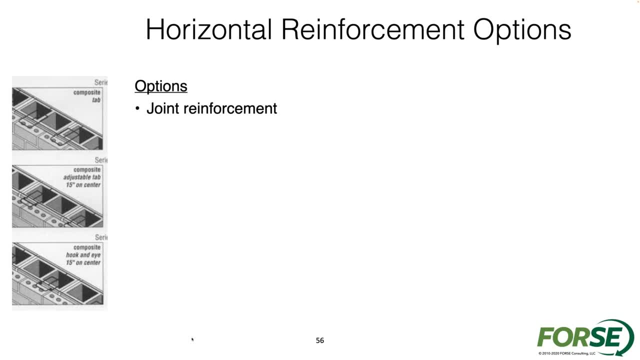 So what are some of the different options here? Options, joint reinforcement. we commonly have nine gauge, which is what all masons are going to bring, So you can add a minimum amount of horizontal reinforcement and add control joints, And then you have the other option that you're going to prefer. 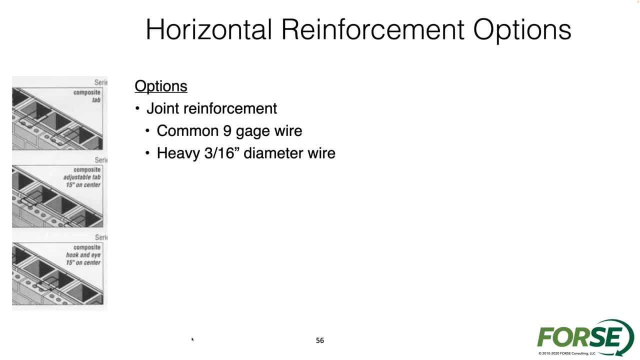 You have an option to have a heavy 316-centimeter diameter wire that could be added, which could be added in rare situations for certain reasons. You could have bar reinforcement. You don't have to have horizontal joint reinforcement. You could actually have horizontal bar reinforcement. 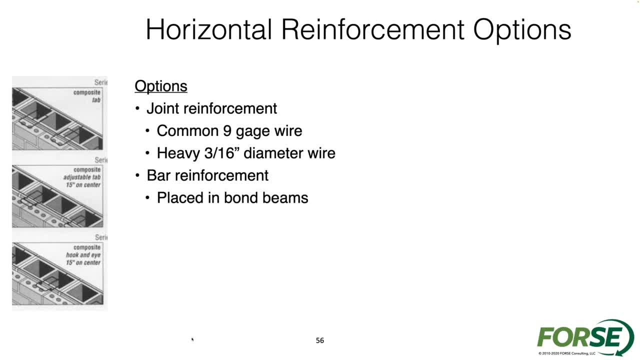 instead of joint reinforcement. So bar reinforcement is going to be obviously placed in bond beams, which again could be common for concrete and structural clay masonry. You know, from the code's perspective, reinforcement is not allowed to be more than half. 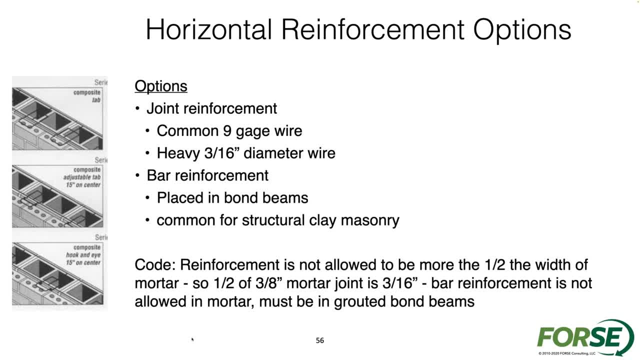 the width of the mortar. So half of a common 3-eighths-inch mortar joint is 3-sixteenths. So that's why the 3-sixteenths-inch wire is the maximum wire that you can place within a bed joint. 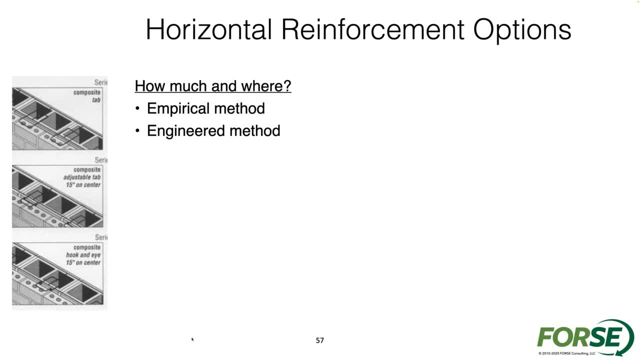 and still have that be horizontal reinforcement, How much and where? Empirical method, engineered method, two different methods for how we place reinforcement From the joint reinforcement- closer spacing, then bar reinforcement, which could be nice. Bar reinforcement option is larger spacing. 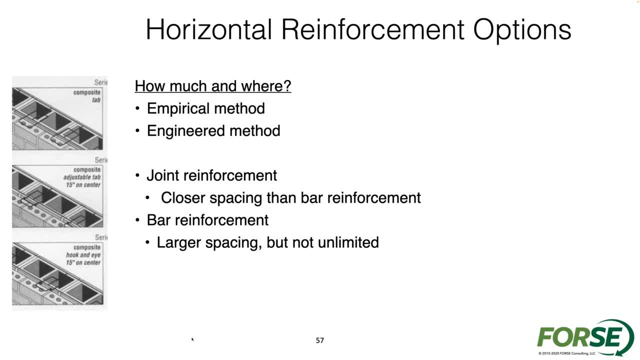 but it's not unlimited. We only can go so far with bar reinforcement. You got to remember we're trying to control the stresses in that masonry wall due to shrinkage in temperature. putting bar reinforcement too far apart and maybe we'd have some localized cracking that. 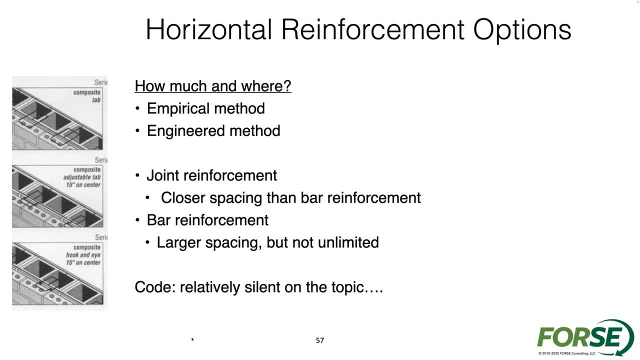 would be undesirable. The big thing about horizontal reinforcement is that the code itself is relatively simple. It's not silent on the topic. It doesn't give a lot of provisions for what is needed for horizontal reinforcement within a wall. So that's where I go, to those NCMA tech guides 10-2D and 10-3. 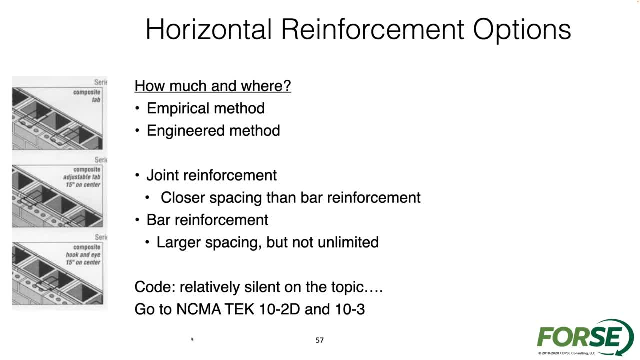 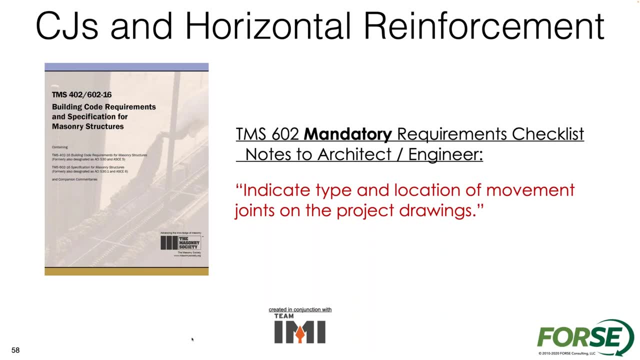 That's really going to be my main references for horizontal reinforcement within masonry walls. The one thing the code does say a mandatory checklist. in the specification 602 section, Designers have to indicate the type and location of movement joints. So if you're going to locate the movement joints, 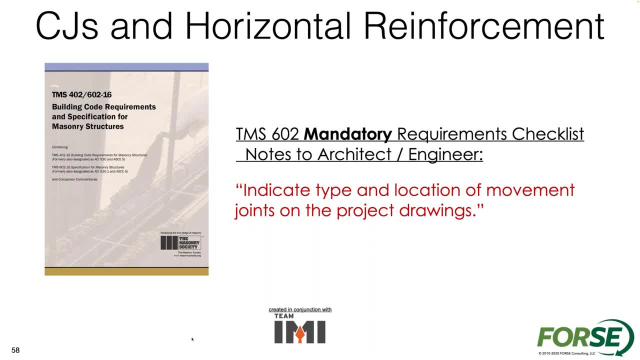 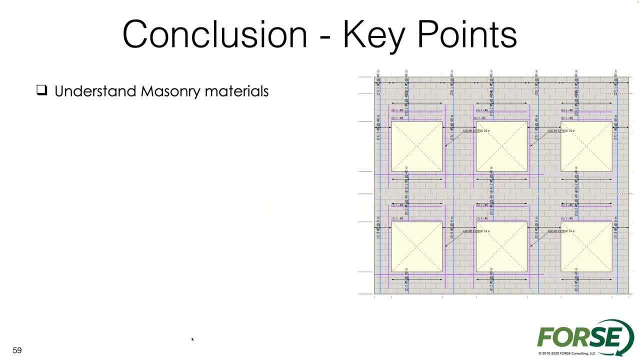 you better know where the horizontal reinforcement is, so that we can understand what movement joints we even need to add. So just some, really quick some, and we'll cover more on movement joints and control joints and horizontal reinforcement a little bit later. Some of the main parts of this section: 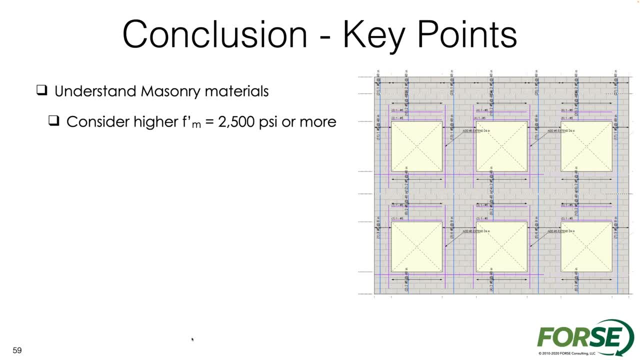 just understanding materials. consider that strength can be- from my own experience- a little bit more powerful: 2,500 or higher. If it's clay it's even higher. Locate, control joints and horizontal reinforcement. Understand different wall options. Consider unreinforced partitions. 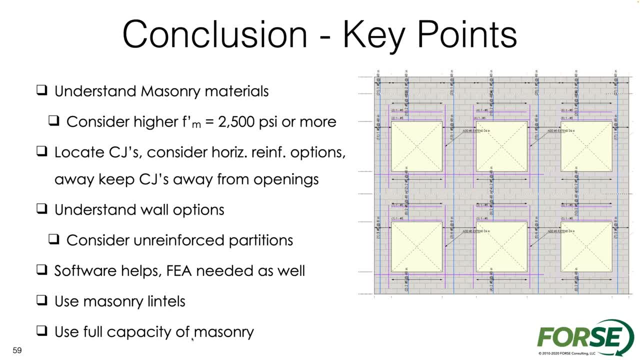 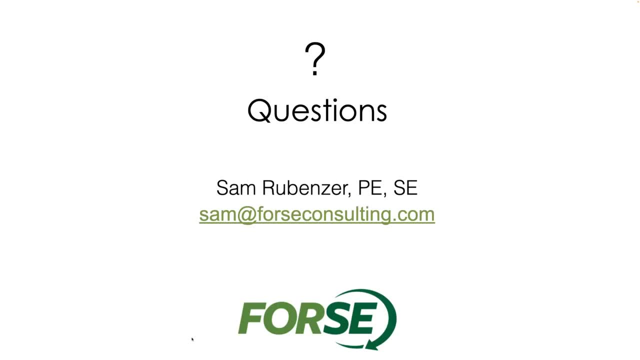 And then we can get into a little bit later today software and how that can help lentils and stuff like that. So that's going to take us to the end of this section. I'm not sure if anybody has any questions, but I think we can. 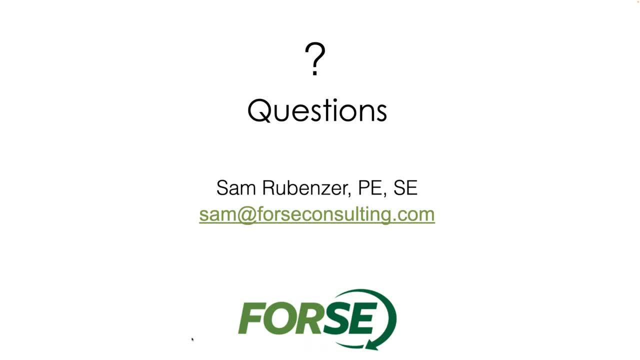 take a five-minute break or so. So if anybody has any questions, certainly throw them up there. in the next five minutes We can take a little bit of a break. I'm going to switch to another section And let's see why don't we say so? it's 10, 10,, 12.. 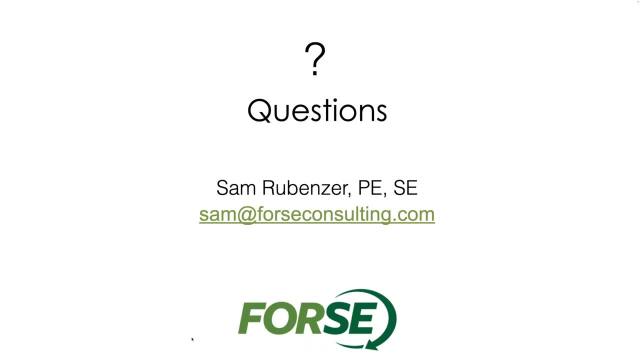 Let's say 10, 20.. We get restarted with the next section of the presentation. Does that sound OK with everybody? Yeah, that sounds good, Sam, We can definitely do that, And We'll all be back at 10, 20 then. 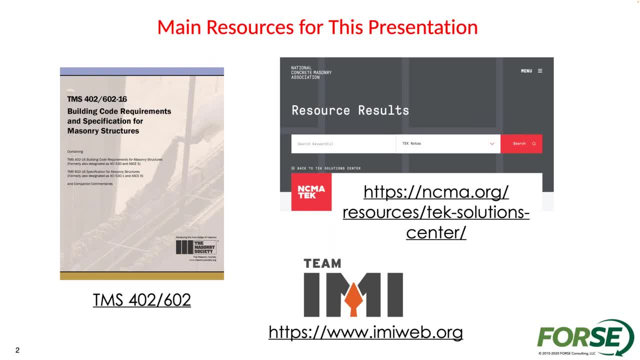 i don't think i missed anything here. did you? um? you might have already caught it, but someone asked about: uh, could you please comment on the different mortars? ms and n? i don't know if you caught that one yet or not. oh, i see it there. yeah, um, yeah, so different types of mortars. um, yeah, gregory, i don't. 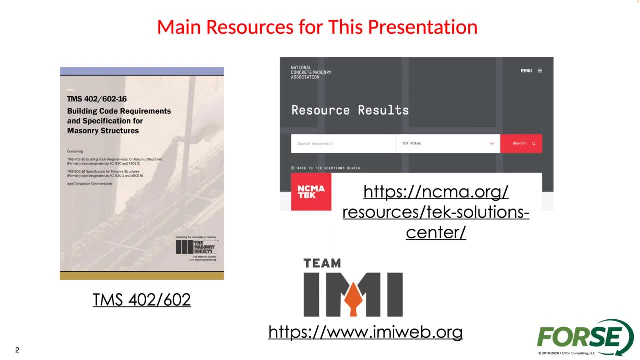 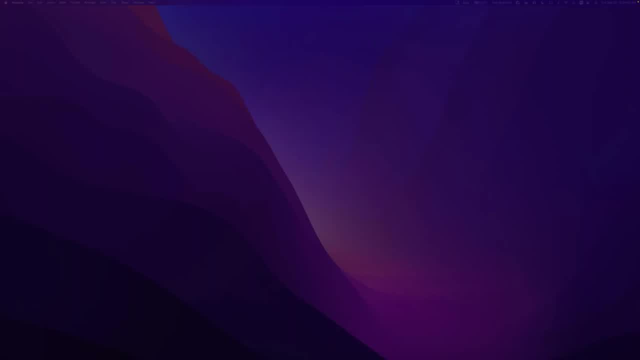 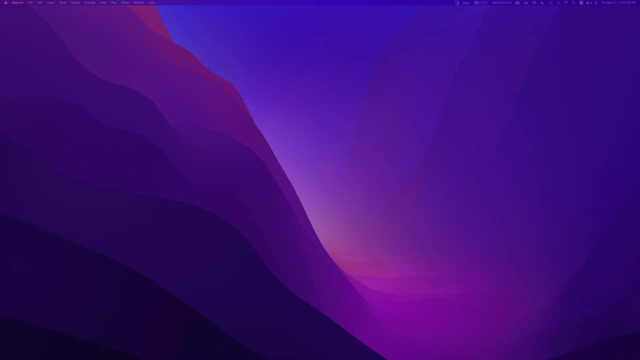 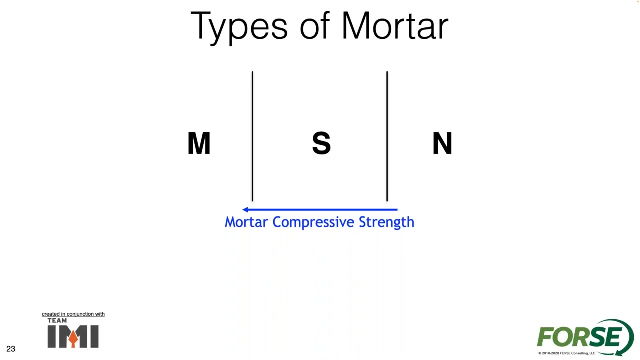 know if you have any specific uh questions about the different types of mortars that you've caught. but type m is going to be um. why don't i go back to a couple slides here? all right, so hopefully everybody can see that different types of mortar, ms or n? um really i. 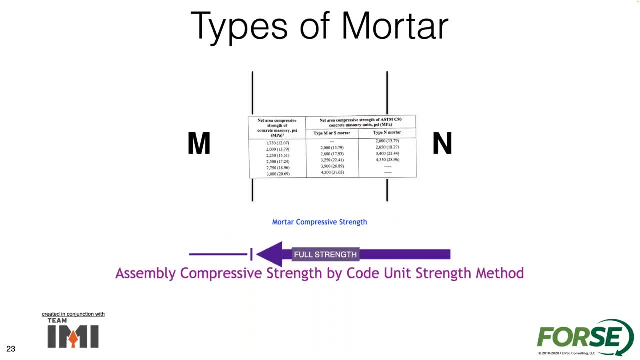 kind of put this uh slide together to really kind of show that uh, really type m and s are going to be similar in terms of uh the code perspective when it gets a unit strength method. in a sense, the code is basically saying you don't get a lot more strength uh from the overall design strength of the wall. 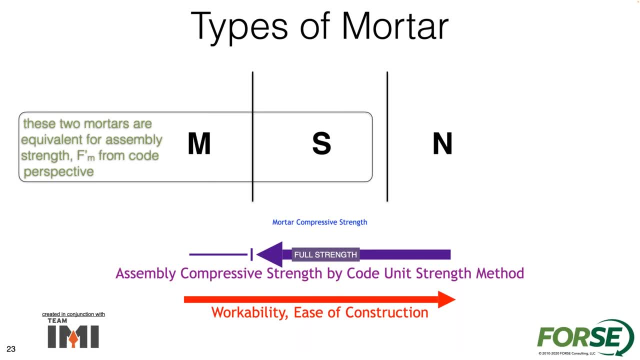 between the different types of mortar. it's really kind of similar. type n, you would, it's going to be a weaker wall, uh, it's a weaker mortar. um workability, you know that's going to be a lot easier when you go from uh, from left to right. so type n is going to be: uh, it's going to be the most workable ease of. 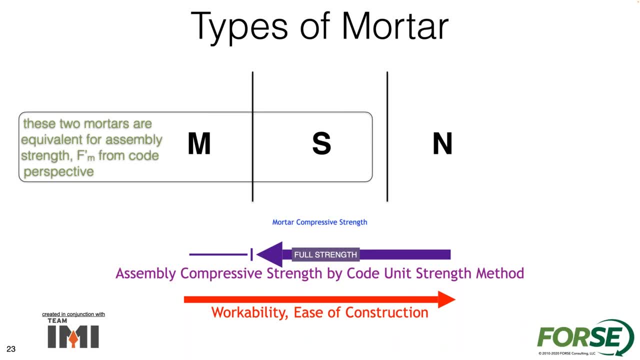 construction contractors prefer n, uh, engineers tend to prefer m, and i'm trying to say: is type s is actually the best mortar to use for most applications? uh, for the structural wall, if you get into a veneer or like an architectural wall, sometimes partitions type n can be, uh, the one that 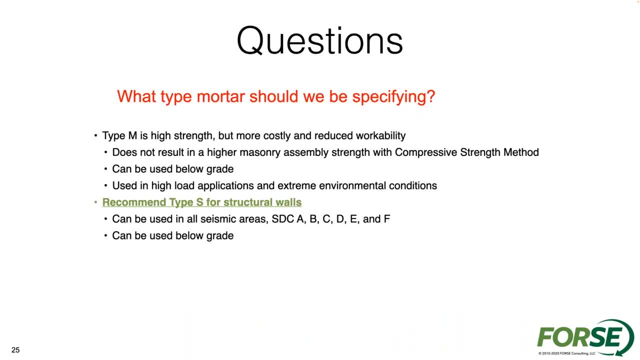 that that is the best. so i just go here, let me see. yeah, so this is kind of a summary slide on uh mortars type s is going to be uh, the most, the best for the most um people, you know, engineers are going to like it, contractors are going to like. 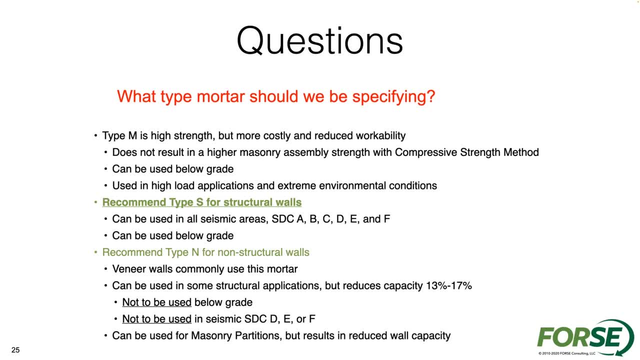 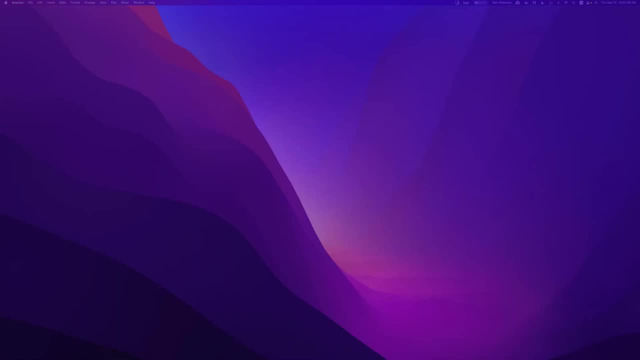 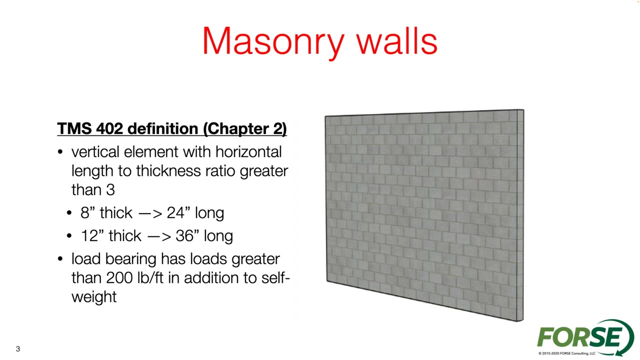 it, the very common water. so, hopefully, gregory, hopefully, that's, that's everything you were looking for. all right, let's go ahead and skip ahead to design. yeah, um, all right. so the design of masonry, design of masonry walls? um, really, what we're? 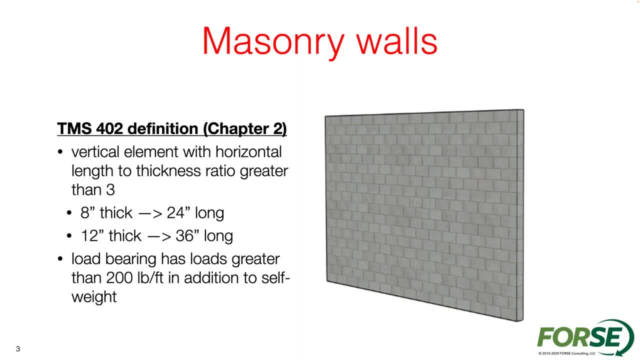 going to be looking at here is the TMS 402 is going to point to a wall being something that's three times longer than it is thick. so you know, if it's 18 inches thick wall, then 24 inches, 12 inch, 36 un inches long. on youtubers, you extremely please don't talk about walls for the purpose ofunch you don't really want to say. just well, you don't kind of sound like you expect me just say: okay, you know. 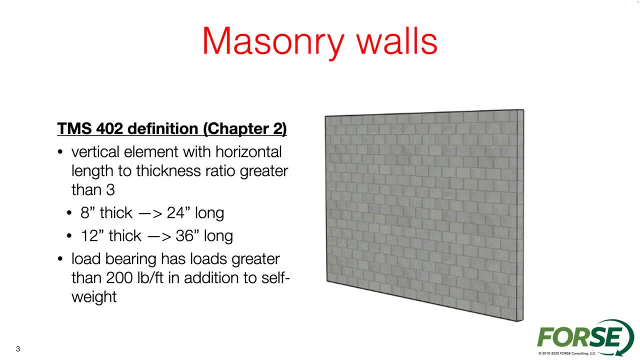 orbeift what we'll you know, in the long run you getting more than double. what do you want to say about just theunted wall? now, x10 is going to be something that's three times longer than it is thick. so you know, if it's eight inch thick wall, then 24 inches, 12 inch, 36 mSq. 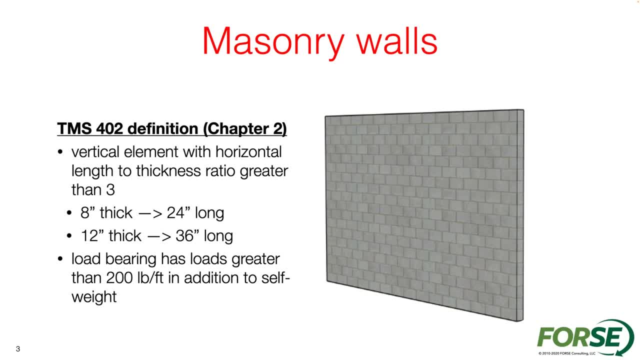 if it's eight inch thick wall, then 24 inches, 12 inches, 36 mSq long, load bearing loads greater than 200 pounds per foot, in addition to cell plate. so all different things that make something. a measuring wall, a shear wall is going to be things in the code. 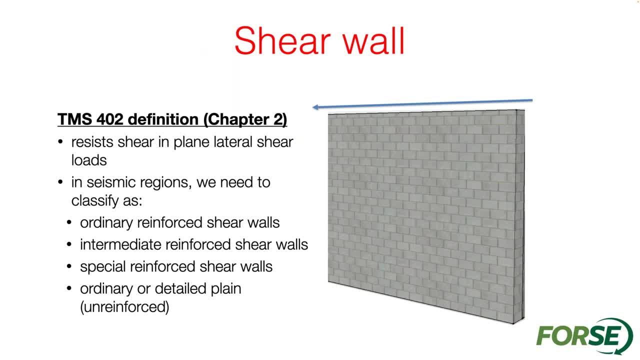 where we're obviously taking on some lateral force different than a partition wall. it's going to be taking some in-plane forces and then the different seismic design regions. ordinary reinforced shear walls are going to be pretty lightly reinforced or the requirements for them are pretty light. you have boundary reinforcement, top reinforcement, reinforcement at each end it's. 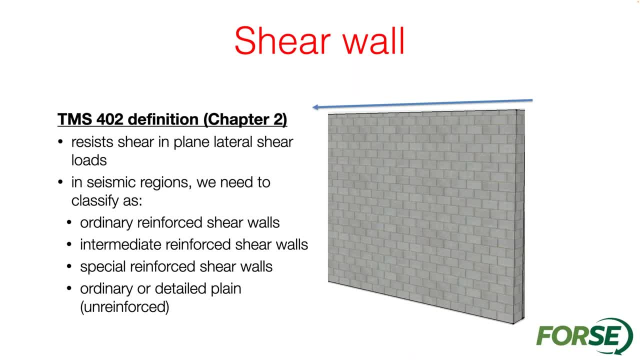 really when you get into the intermediate reinforced shear walls. intermediate reinforced shear walls have reinforcement requirements at 48 inches on center each way. obviously, the more complicated, the more ductile the wall needs to be, so like if you get into specially reinforced shear walls, it's even more and more reinforcement requirements for higher seismic areas. 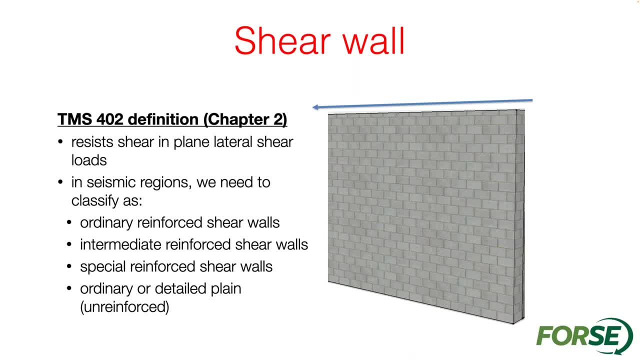 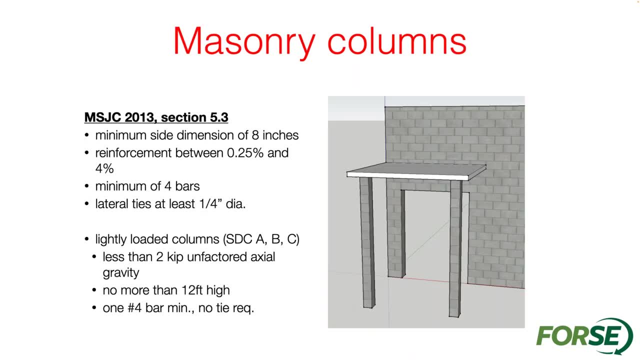 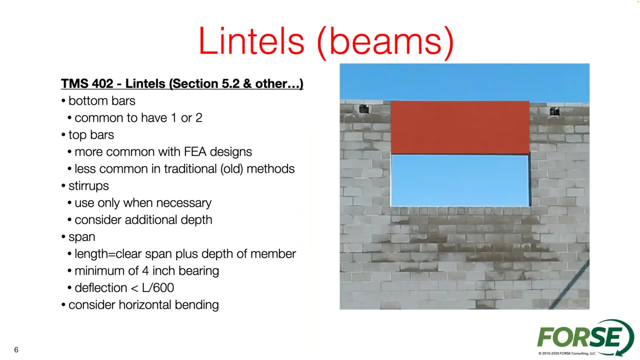 that really demand the walls go through, you know, more of a ductile response as it has the higher seismic forces on them. we talked about columns, we talked about beams. so those are going to be the two different, two different main elements for walls. so lintels are going to be, obviously 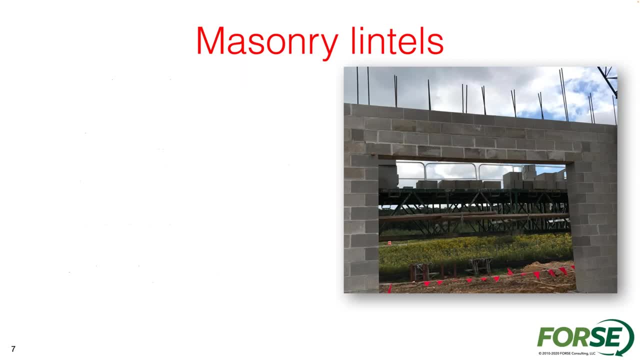 this area. that spans an opening. we'll go a little bit deeper with lintels. we're actually i have a little bit more information on how the lintels are going to be built and how the lintels will be moved. we're going to talk about them in a little bit more detail, but for now i want to make sure. 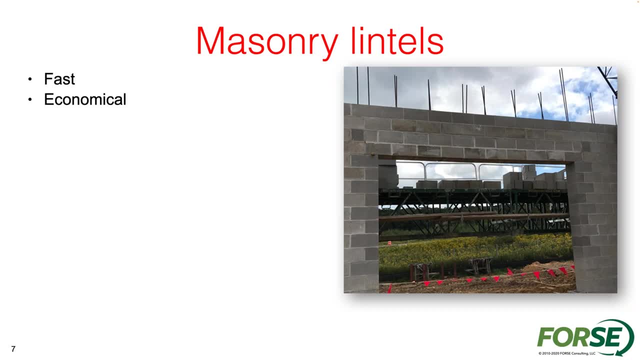 that we are getting back to the point where we were talking about the lintels, just because masonry and lintels are going to be something that is going to be a preference from the overall masonry perspective. it's going to be fast, economical matching of wall moves at the 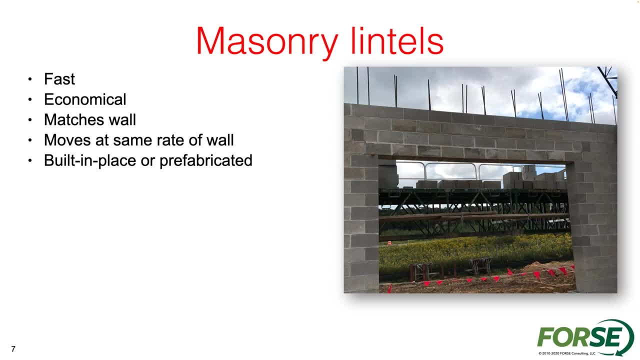 same rate of the wall, which is going to be important from an engineering perspective, built in place or prefabricated. a lot of times shoring was complicated back in the day. Shoring has gotten a lot less complicated and a lot of masons actually don't mind at all. 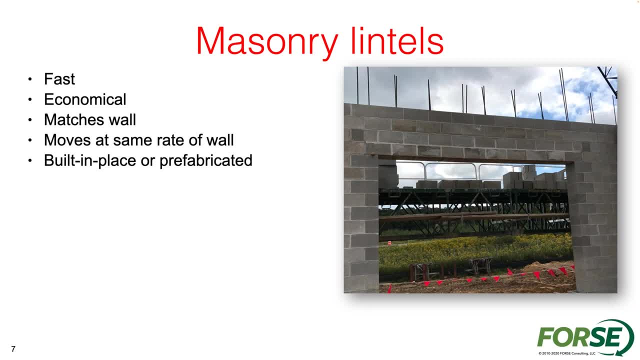 shoring up an opening, But prefabrication is gonna be as we get into more and more prefabricated elements. prefabricating masonry, lintels is gonna be something that's pretty straightforward, pretty easy to do, any length really being possible. 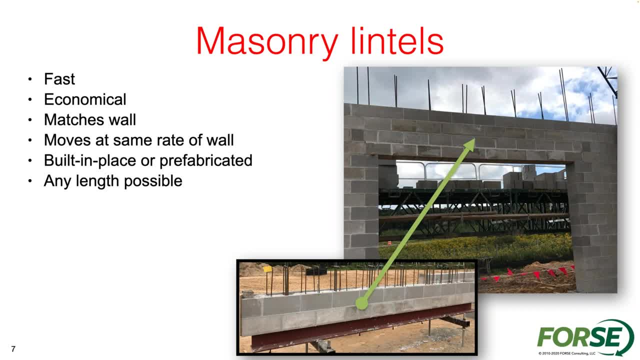 So here you can see the actual lintel in this wall is something that was prefabricated. You can see the shim on one end. that kind of points to it. Really, there's any length that's possible. There's not a lot of length restrictions. 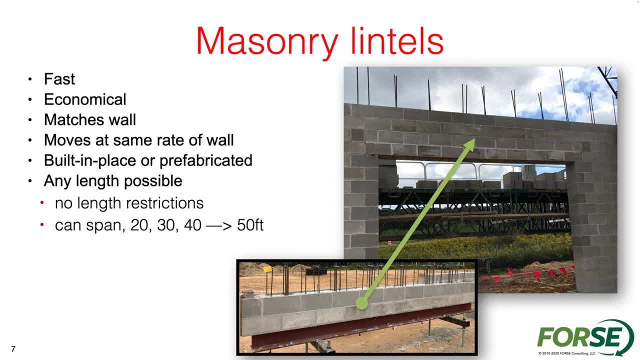 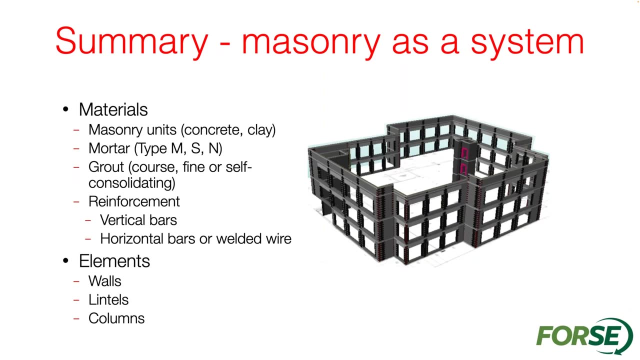 20,, 30,, 40, even 50 feet. 50 foot masonry lintel is certainly something that is possible and doable and really does, like I said, have a lot of benefits for the overall wall. So again, a lot of different types of elements. 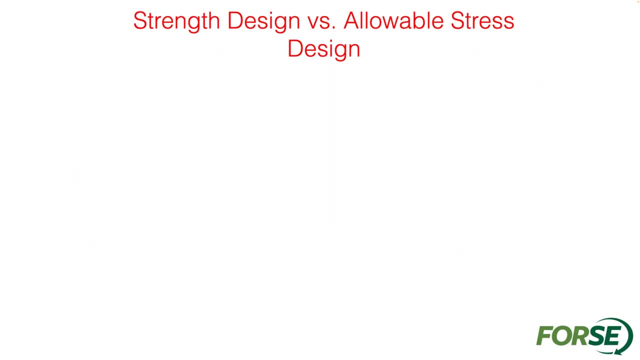 that we're gonna look at. We wanna get into the actual design provisions: strength design versus allowable stress design. I know a lot of people in masonry are allowable stress design, so I'm gonna kind of take the opposite perspective in strength design and why it makes sense. 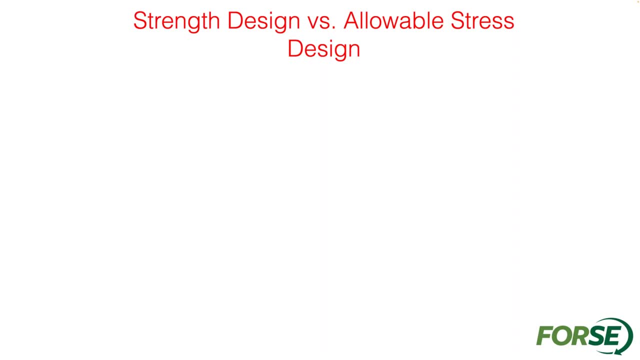 and why it maybe is worth a look. Like I said in the first section, today there's a lot the code designers are trying to do to drive to bring allowable stress design closer to some of the strength design provisions. to be honest, 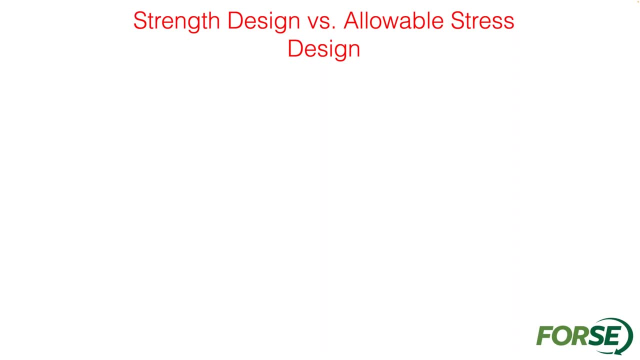 So harmonization of the code is really kind of that effort. Really. the most common code that we're looking at are again sacral and structural loads are based on strength design because it gives more uniform factor of safety against a structural failure Loads on a building area that are permanent. 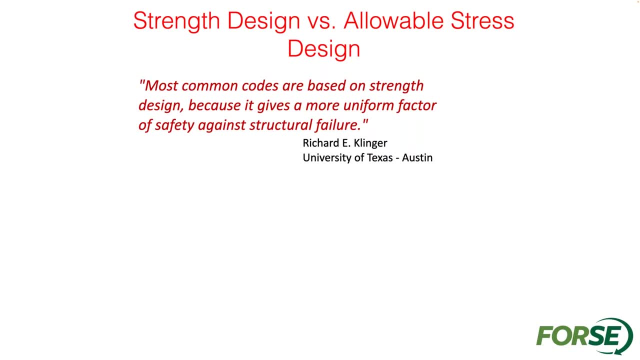 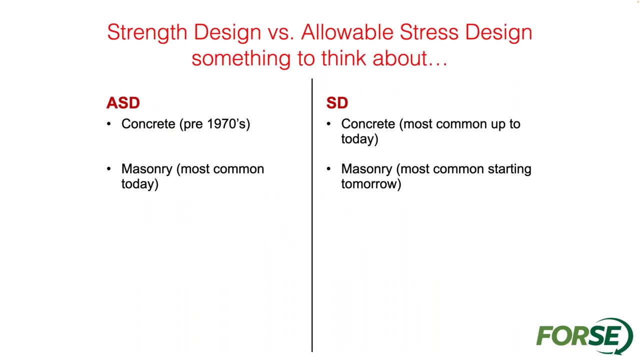 or transient or moving. changing Strength design puts a higher factor of safety on less predictable transient loads. So I think that that's something that's important to think about and recognize. I mean, strength design doesn't make a lot of sense, Just a quick comparison. 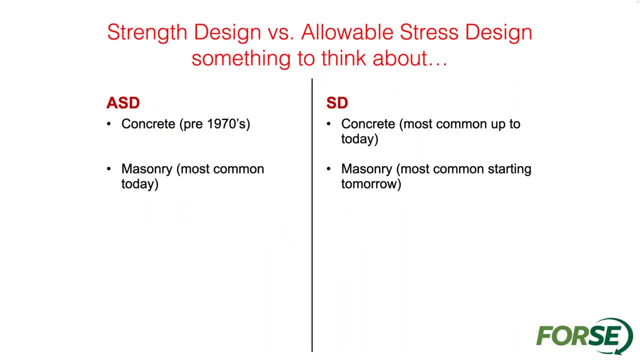 Let me do this between the codes and different timeframes: ASD. there was ASD in concrete, believe it or not. It wasn't always strength design, but that was pre-1970s And I would say most masonry design today is ASD. 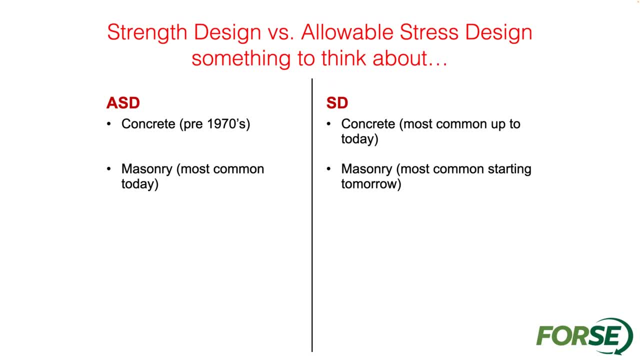 So strength design for concrete been very common. Most people learned in strength design, basically in concrete, and then hopefully masonry. maybe that's starting tomorrow for all of you. I think it makes a lot more sense And that's where a lot of the efforts go into. 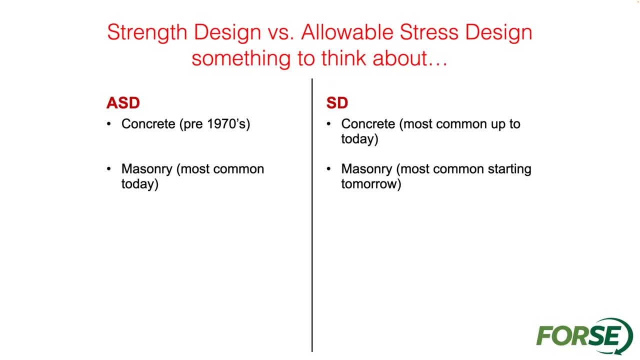 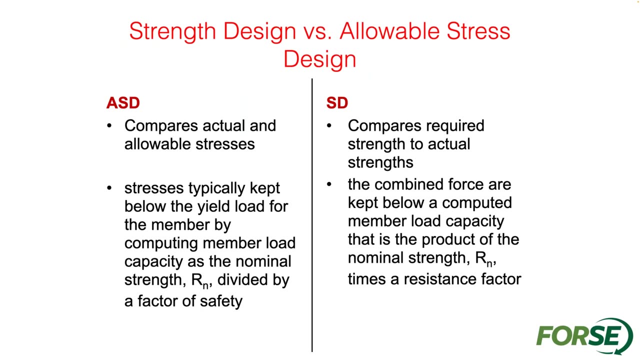 in terms of the codes and the testing. it's more in the strength design And, like I said, the harmonization is really kind of bringing allowable stress design up to the strength design parameters. ASD compares actual and allowable stresses. Stresses typically cut below the yield. 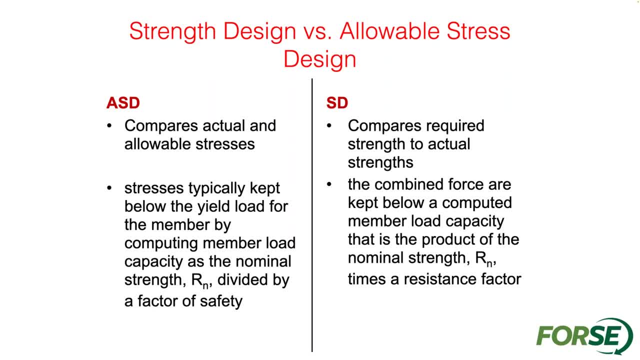 for a member computing the load capacity, By the way. in fact, there's a lot more in terms of the load factor, safety, And then again strength. design obviously looks at different strength provisions to try to keep it with an actual and then the combined forces. 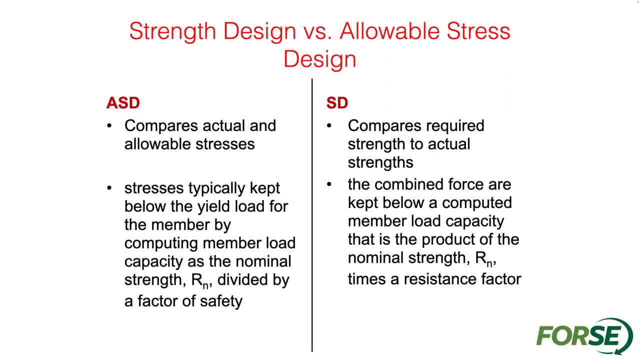 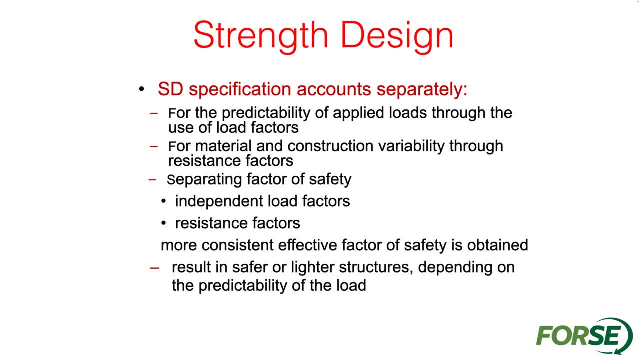 are kept below computing member capacity for resistance times. resistance factor: resistance factor: Again, strength design specification accounts for the separation of the different predictability of the different loads to the different load factors. Again, allowable stress design has made some efforts in kind of moving towards that direction. 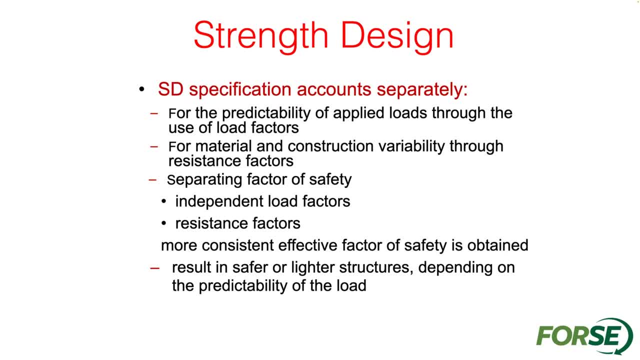 For material and constructability variability through resistance factors, separating factor of safety, independent load factors or system factors. more consistent effective factor of safety is obtained, resultant in safer, lighter structures depending on predictability of the load. So obviously you get into more of the wind loads, seismic. 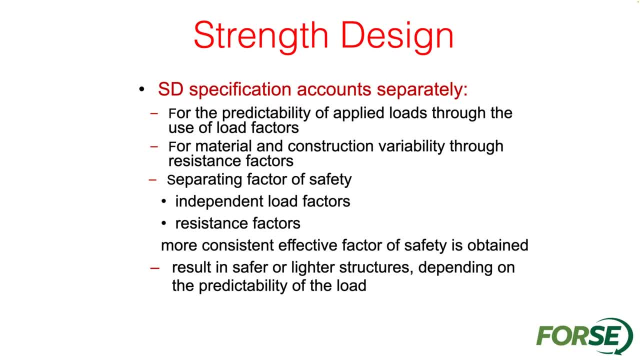 loads. Those are things that we're looking at. When those are dominating the demand, then you're going to have maybe a little bit more conservative designs. When it's more of the gravity loads- dead loads, live loads- then strength design would probably 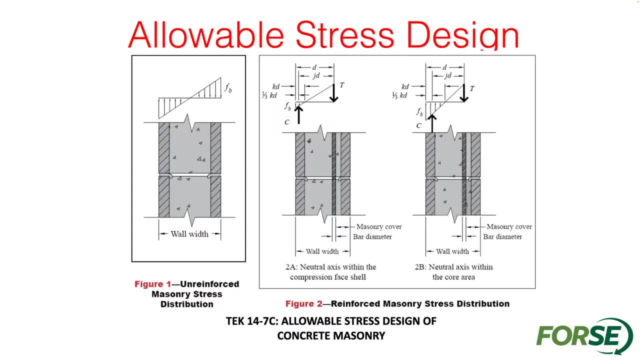 be more favorable of a design. Just looking at the overall stress distributions here, obviously, masonry being able to be unreinforced, you have tension Tension equal to compression And obviously we have to stay within the tensile limits. 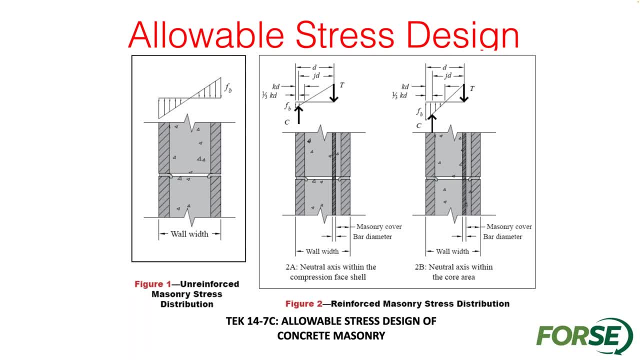 Obviously, if you have more compression on the wall, then you could actually maybe reduce or almost eliminate some of the tension on an unreinforced wall. Otherwise, we have some different variables that we look at in terms of tensile force And then strength design obviously. 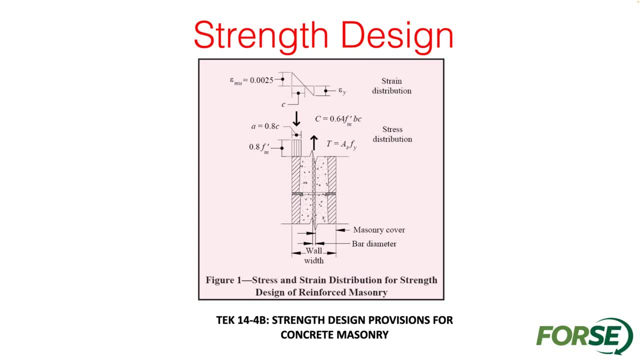 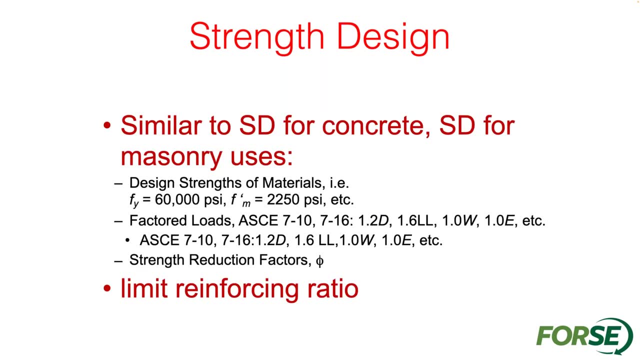 has a compression block and tensile force. So some of the similar diagrams, just a little bit different ways of coming to the same thing. OK, Same conclusion, hopefully Similar to strength design. strength design uses for masonry design of materials. FY of 60, KSI. 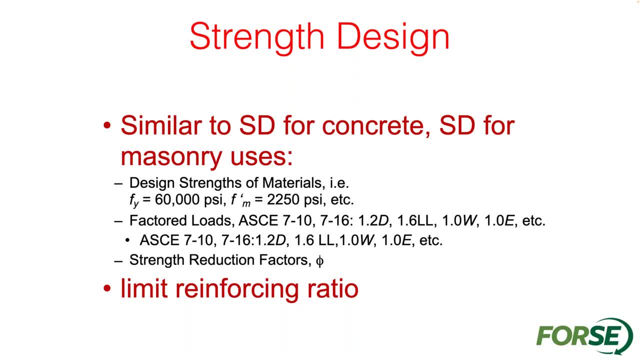 F, prime m of whatever the masonry is here: 2250.. Factor loads come from ASE 7, 1.2 DES, 1.6 live, 1.0 wind and 1.0 times seismic, And then you have the strength reduction factors phi. 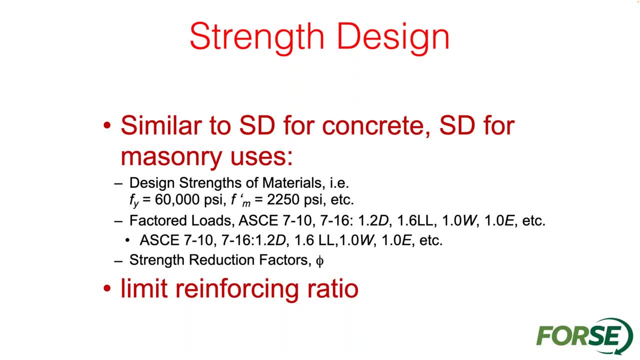 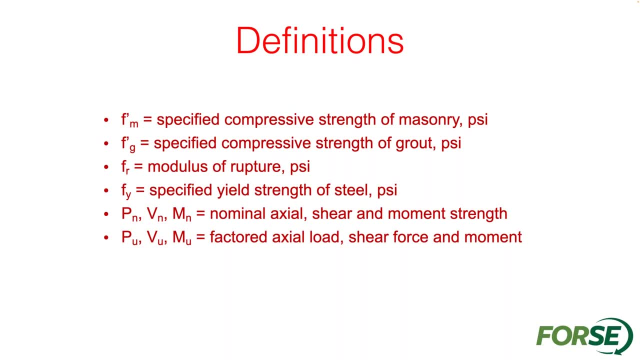 Limiting reinforcing ratios, I think are also really good to make sure that we stay into a ductile area. Here are some of the different variables: F, prime, m is specified compressive strength of masonry. That's the overall assembly right. 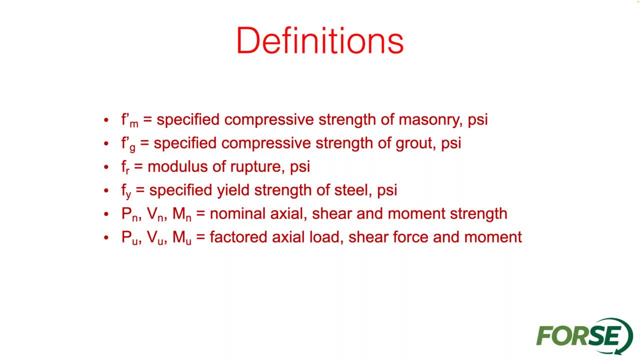 That's not block strength, That's not mortar strength, That's the overall assembly strength. The grout FG is going to be the specified compression of the grout itself. Grout is not one of the variables. And determining F, prime, m, that's always something. 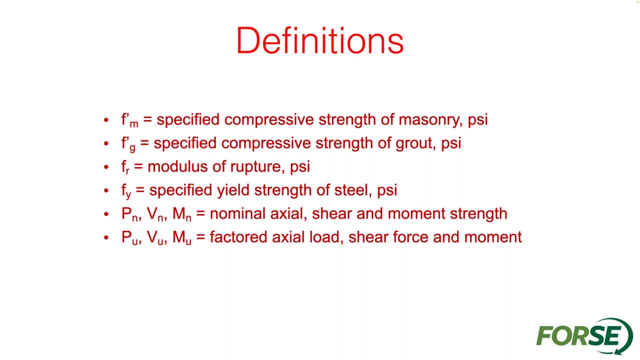 that we have to remember. That's why it's kind of held separately here. FR and modulus of rupture is really going to be looked at as the kind of that tensile capacity, the tensile stress that's allowed for our masonry wall. 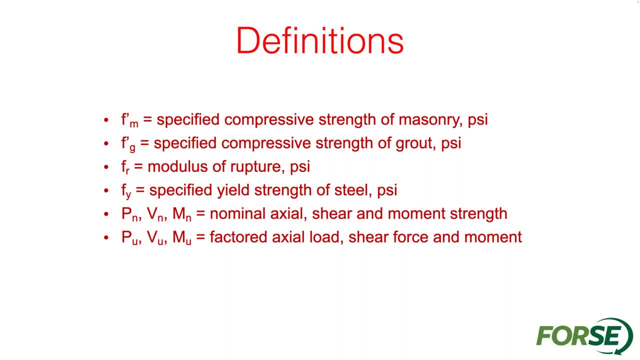 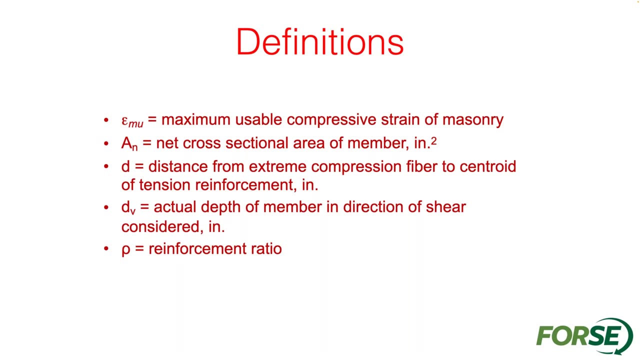 FY specified yield strength of the steel. The PNVMN is going to be the nominal axial shear moment strength. PUVMU is going to be the factored axial load shear force. It's going to be a moment. You have strain variables. 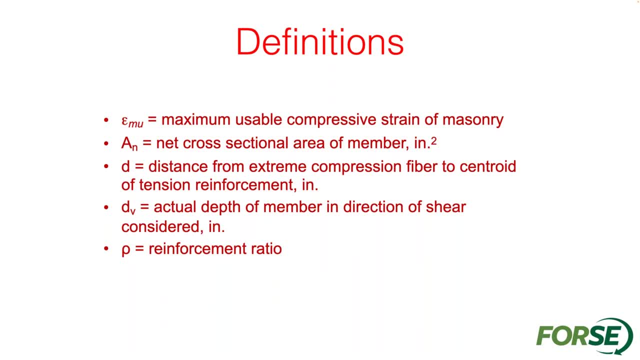 We have net cross section areas, So all the different variables that are going to be used throughout some of the different code equations specified here. Rho is going to be your reinforcement ratio. the distance between stream compression fiber to the centroid of the tensile element. 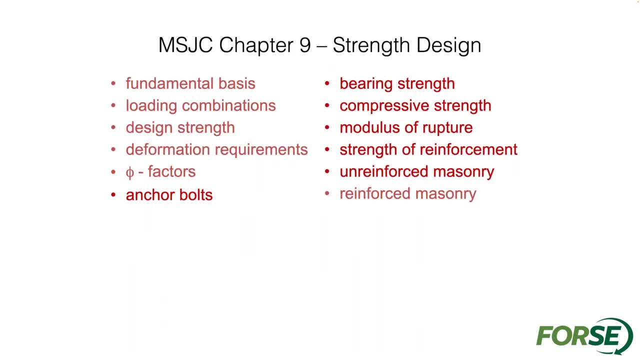 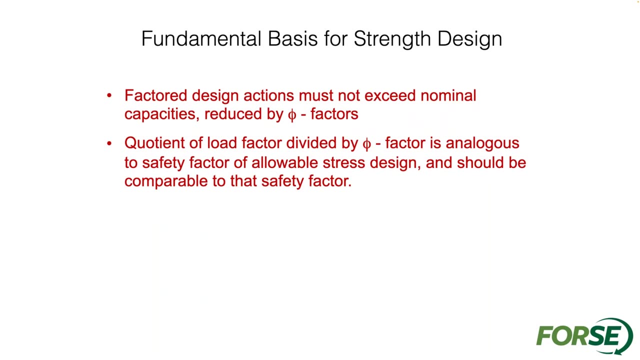 PV: actual depth of member. So chapter 9 strength provisions. we have the all the different again sections of the code that we're going to be looking at. So, factors: design actions must not exceed the nominal capacities reduced by our fee factors. 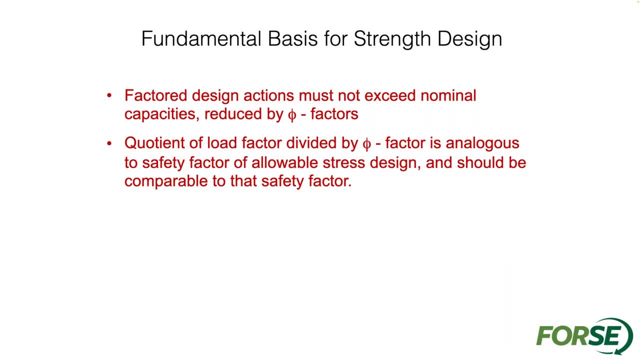 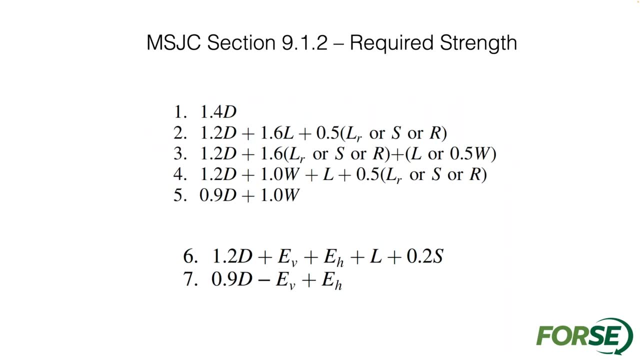 Quotient of the load factor divided by fee is similar to the factor of safety of a long stress. that should be comparable to that safety factor, So obviously something that's good to think about compare. Let's hear some of the again, some of the load equations. 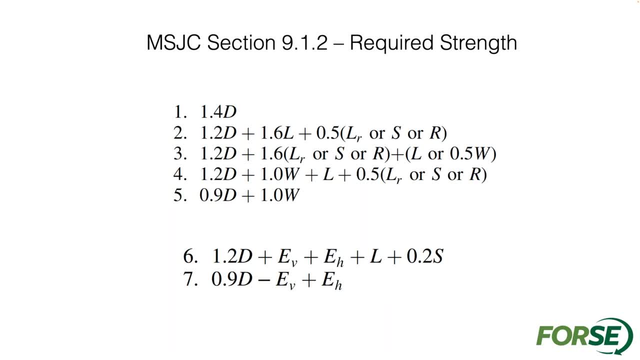 Okay, So the load equations that we have with strength design. the other thing that I do appreciate at the codes: this isn't just masonry code, but we look at the masonry and concrete and steel, all of them using similar strength design provisions. 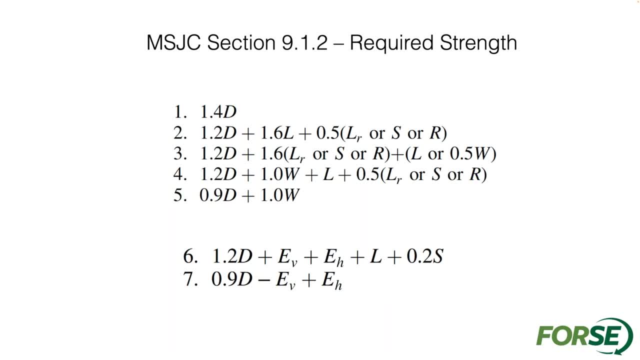 strength design: 1.4 times dead, 1.2 times dead, 1.6 live, like all of those things, instead of the concrete code having the 1.4 dead, 1.7 live, so on and so forth. 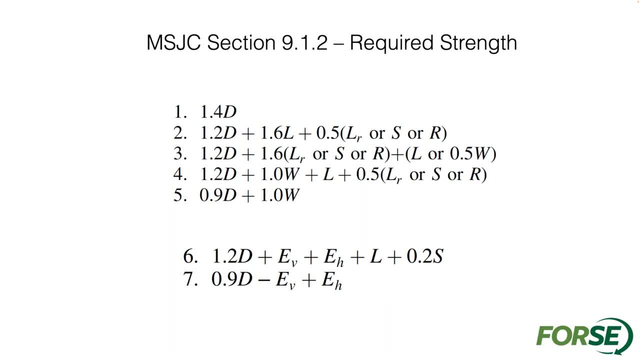 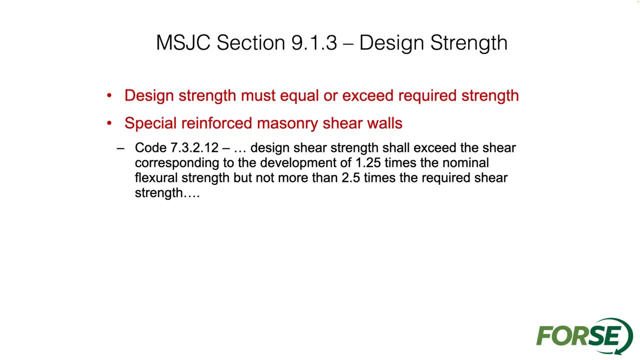 So having all that uniformity obviously helps a lot with the different material designs. So within the code design strength must equal or exceed the required strength, especially reinforce masonry. shear walls do have design strengths. they'll exceed the shear corresponding to development of 1.5 times. 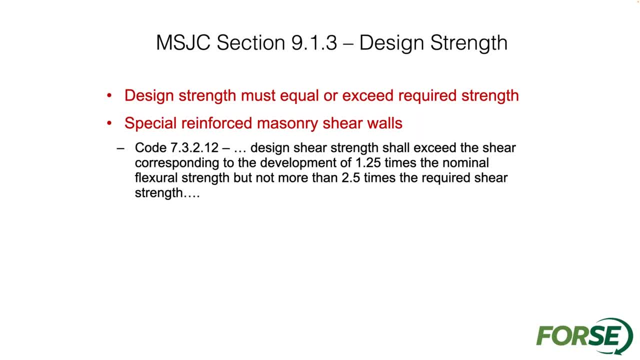 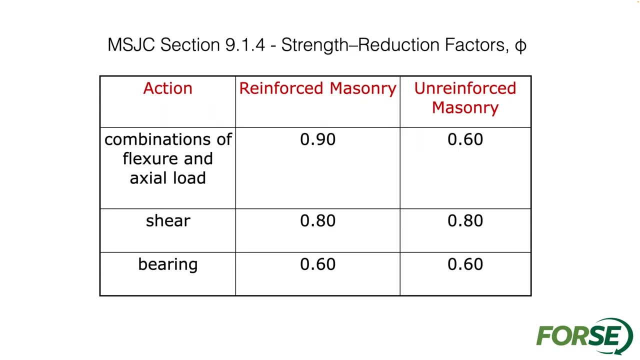 1.25 times the nominal electrical shrink was not more than 2.5 times is required shear strength. so not just meeting uh, the required shrink but actually staying within a range of range of values. especially reinforced walls, obviously a higher seismic area. so strength reduction factors. you can see unreinforced masonry having lower fee factors. 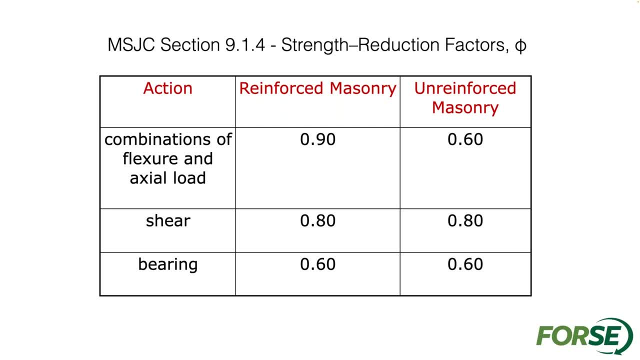 for the combinations of flexure and axial load, so basically giving us higher factor of safety, right we it's less predictable with unreinforced masonry, so we have a 0.6 for the fee factor instead of reinforced, which is at 0.9. 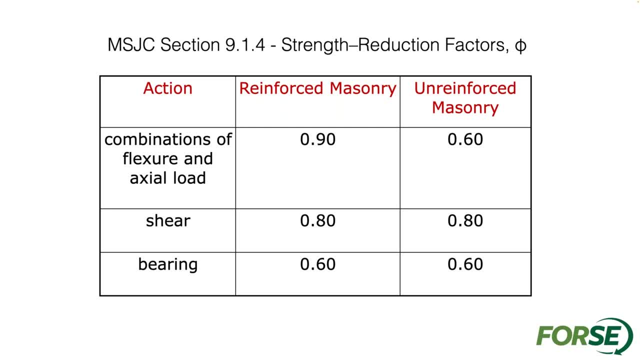 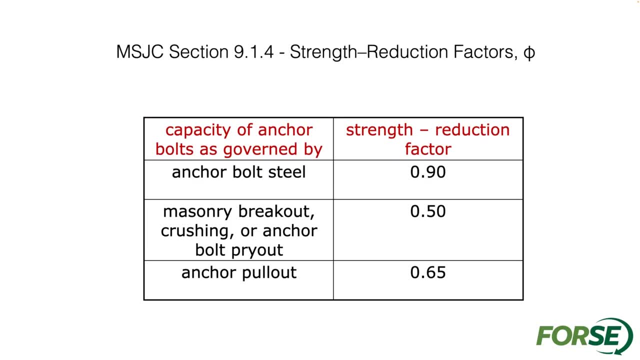 we have similarities between shear and bearing at 0.8 for shear and 0.6 for bearing. fee factors again for the connections to masonry: we have 0.9 for the actual steel- uh, anchor bolt steel. we have 0.5 for a masonry breakout, crushing, or so we look. looking at the 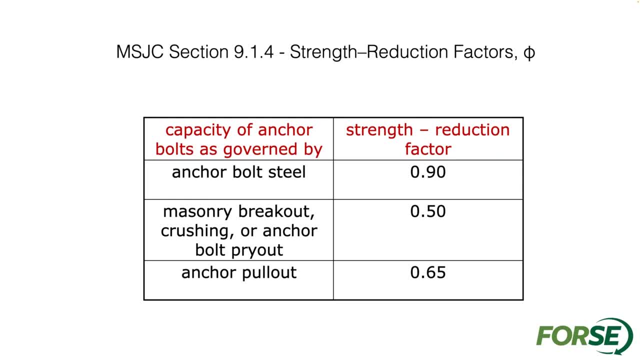 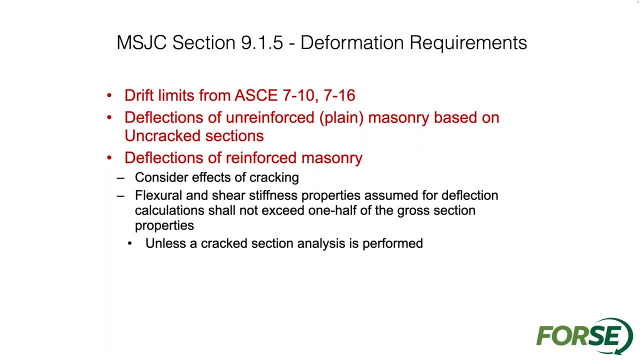 actual kind of tensile strength out of out of masonry itself. that fee factor at 0.5 and you can pull all of that 0.65. we have deformation requirements, ase 7, 10 and 16.. uh, deflections of unreinforced masonry are. 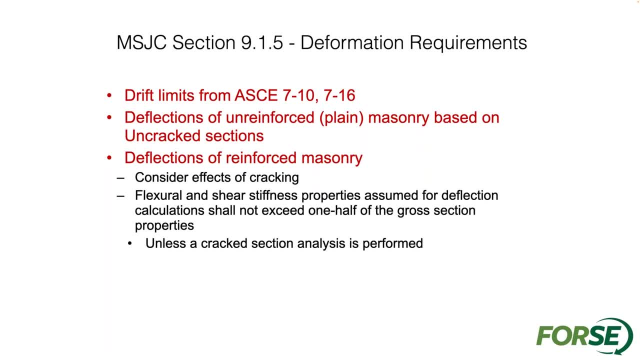 based on uncracked sections. uh, obviously, obviously we can't have cracking occurring. uh. deflections for reinforced masonry consider the effects of cracking. uh flexure and shear stiffness properties assumed for deflection calculations is not to exceed one half of gross section properties, unless a crack section analysis form. so basically, you know, when we have a reinforced masonry, we have 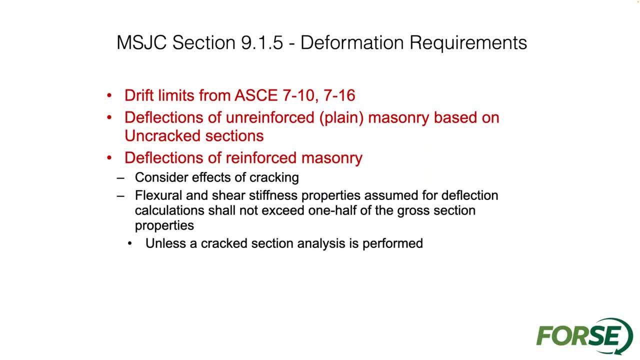 to take into account that the actual section properties are going to be less. there's going to be uh section properties are going to be reduced once the section goes from uncracked to crack. then, once we have cracking occurring, we have something that's going to have less stiffness. so 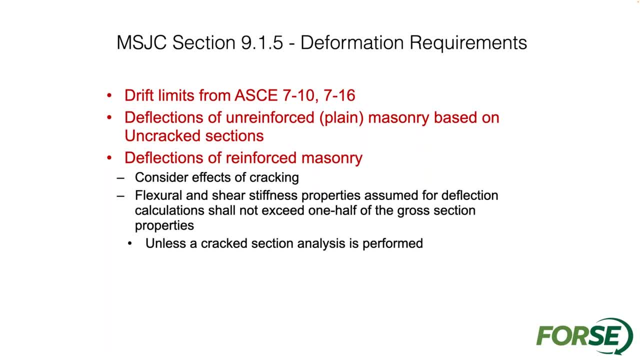 that 0.5 times the uh stiffness of the wall, uh, giving accounting for the crack factor. but you certainly can come into, um you know, having a more, a better analysis. we actually wrote a couple papers, uh on cracked sections, uh for masonry, kind of coming up with a better value certainly. 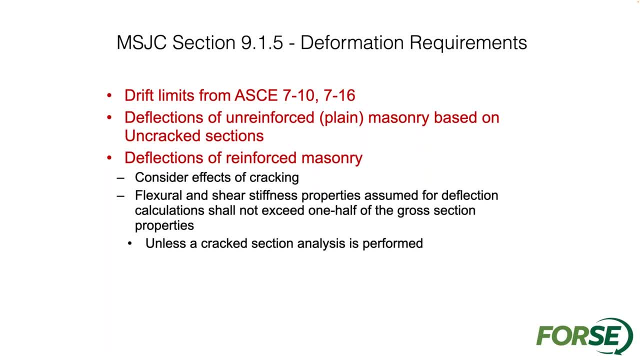 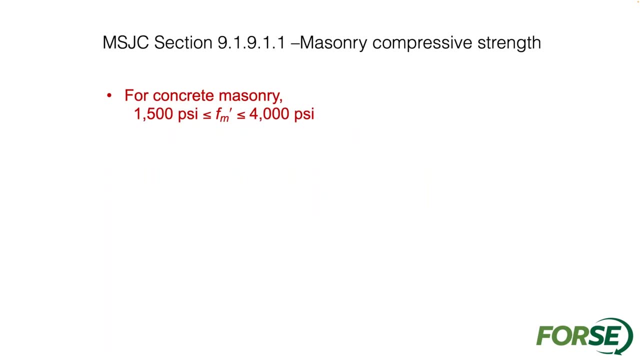 the 0.5 is a nice place to start, but we can certainly get into something that's more um. there's more relevant to the section uh. within the sections of the code, we keep the 1500 in there, but all the way up to 4 000 for. 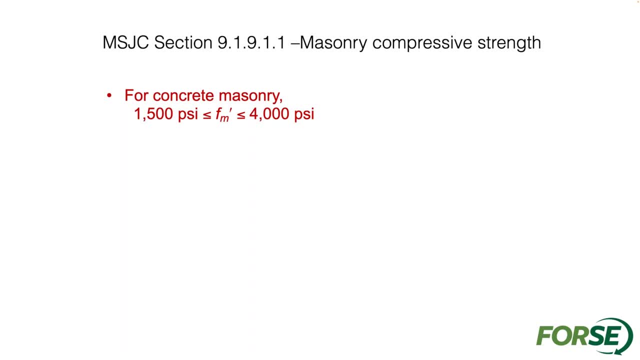 the masonry compressive strength. uh, we have grout which is going to be greater than f prime m, so that that's going to be important, but then less than 5 000 psi uh for the overall uh growth strength. so we want to make sure that we stay uh within those values. we don't want growth, that's. 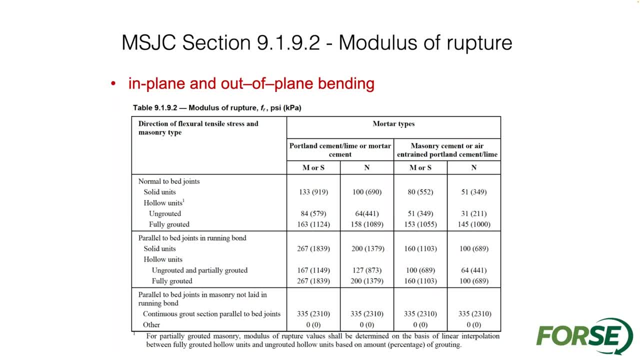 overly strong or that's overly high. so we want to make sure that we stay within that value. um, in plane, out of plane bending, we have different types of mortar and modulus of rupture, so different tensile capacities that you have. you know, with those different um, different options for. 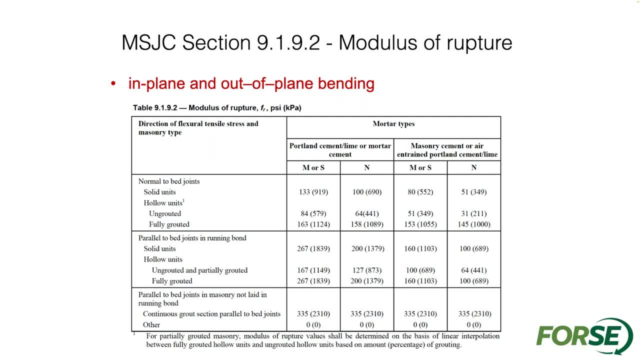 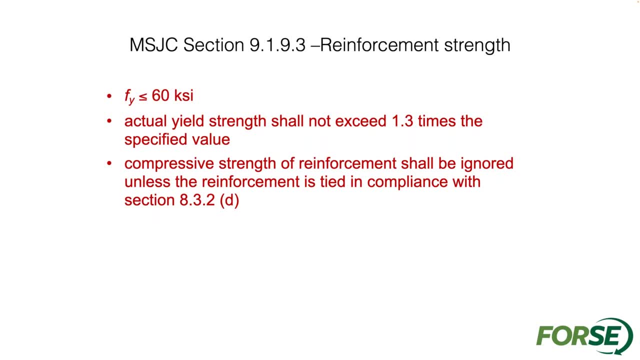 an unreinforced masonry section: uh reinforcement strength. we have fy of uh less than or equal to 60 ksi. yield strength still not exceed 1.3 times specified value. uh compressive strength and reinforcement should be ignored unless the reinforcement is tied by a certain section. so unless you get into some of the higher detailing requirements of the 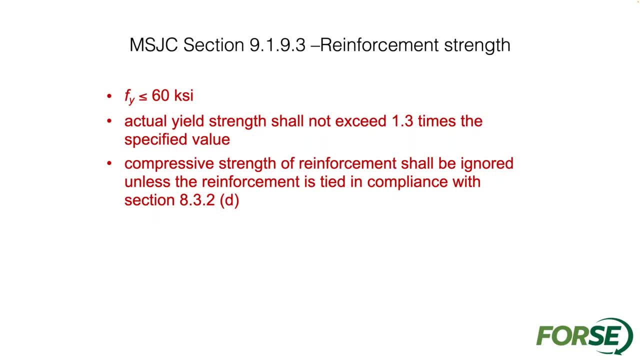 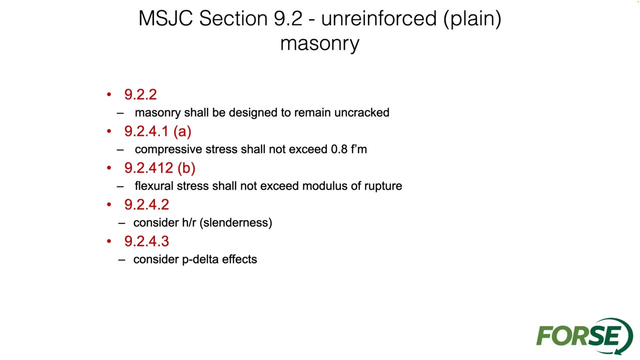 code. you really are going to be ignoring any compressive capacities of the reinforcement which would be very common with concrete and concrete masonry design. uh, unreinforced, obviously, masonry shall remain uncracked. compressive stress will not exceed 0.8 times f prime m flexor stress will not. 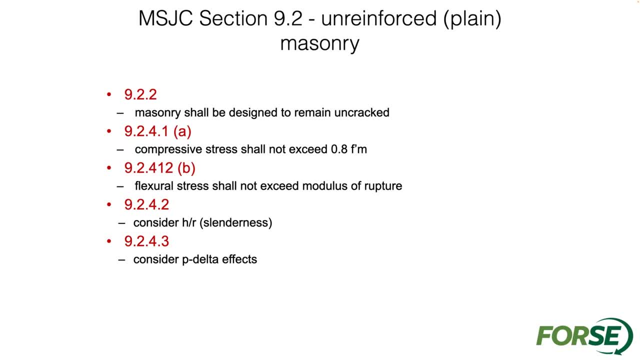 exceed those moduluses of rupture. uh. consider the h, h over r slenderness ratios and consider the p delta effects on on crack section. obviously if you have something that's low bearing, it can be good in terms of it's going to keep the section in compression. but 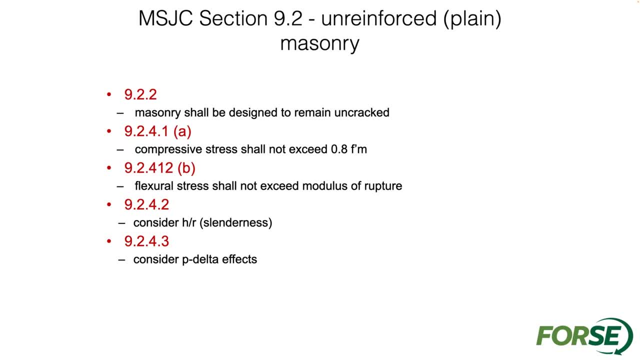 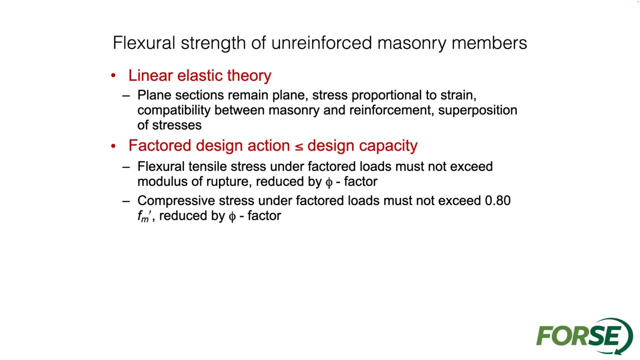 it's something that we need to be careful of to make sure that we don't exceed some p delta effects making and accentuating the actual moment on that wall. so linear elastic theory, plane sections, remember, remain plane stress, proportionate strain, compatibility between major reinforcement and superposition of forces. so um factored design. 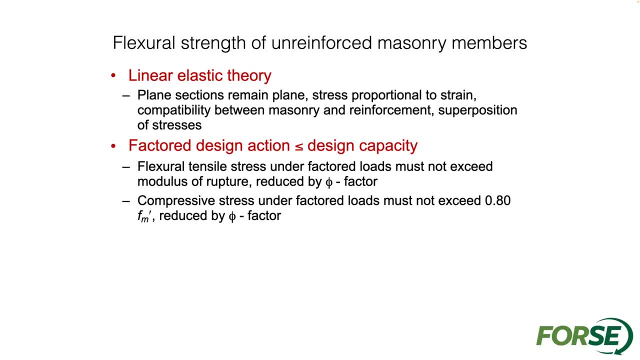 is less than the design capacity, so our fluctuant stress is less than the unfactor modes must not exceed the modules, the rupture reduced by the p factor. so obviously we we can't get into any uh crack sections or anything that's going to cause that price of the structure. but it doesn't just be. 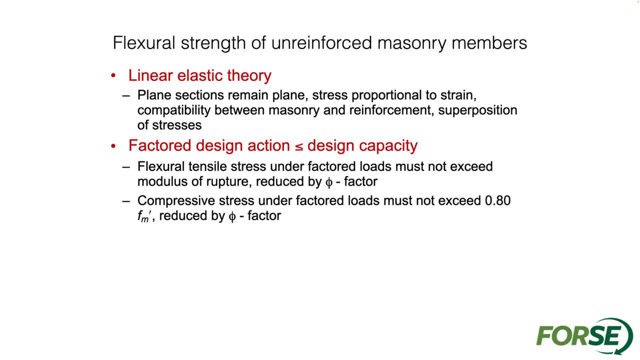 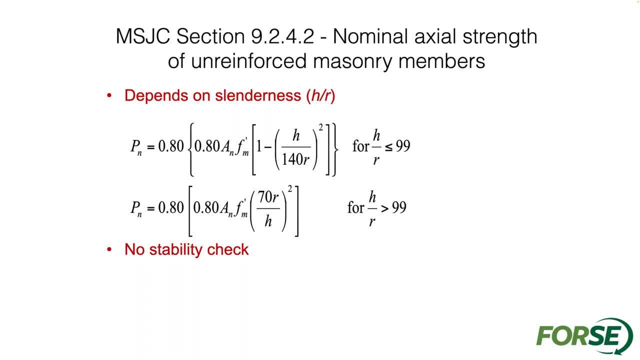 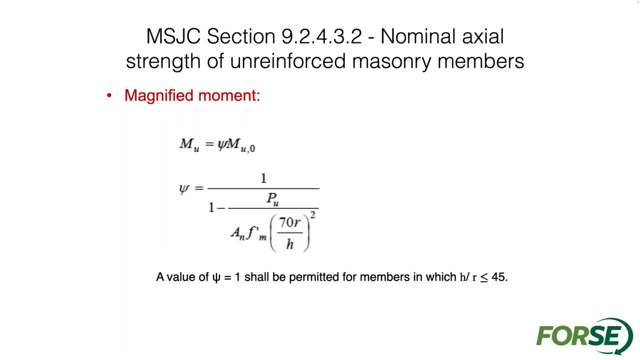 the structure of, uh, any of these structures anymore. it's not an rainy day. we don't want to go into the anything like that for a mainstream wall. we have some pretty specific equations for axial strength for our walls, for unreinforced mainstream members, and then a moment magnifying for the unreinforced mainstream members as well. 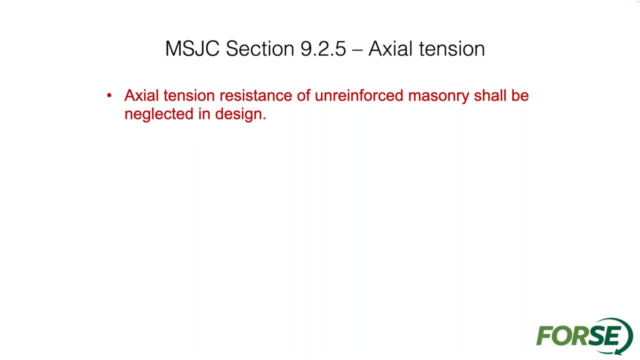 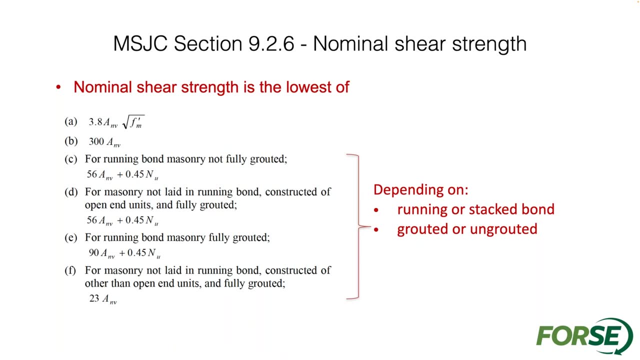 axial tension resistance and unreinforced masonry should be neglected in design. and then we have nominal shear strength. based on these different equations, depending on running bond or stacked bond, grouted or ungrouted, we can have different types of capacities that can be determined for our shear strength of masonry. 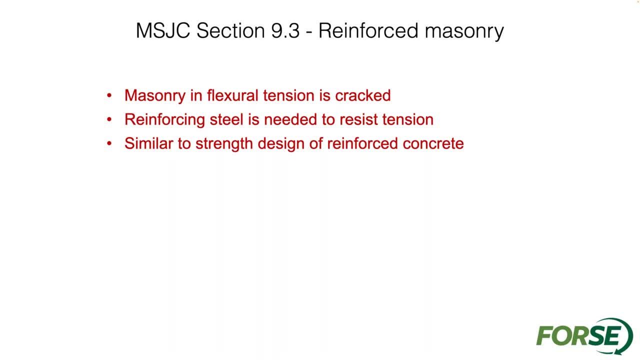 so we get into reinforced masonry. obviously it's going to be quite a bit different. reinforced masonry is cracked. reinforcing is needed to resist tension, similar to the design of reinforced concrete. and reinforced masonry is not the main reason why reinforced masonry is not the main reason why reinforced masonry is not. 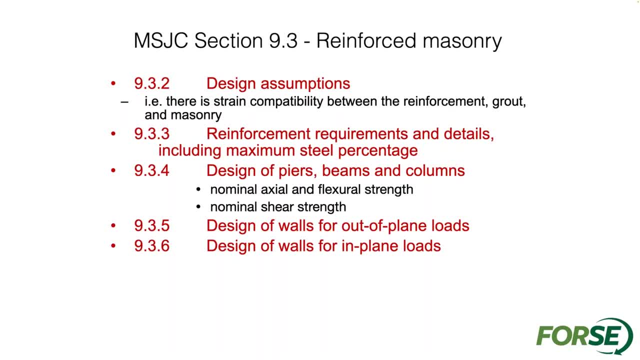 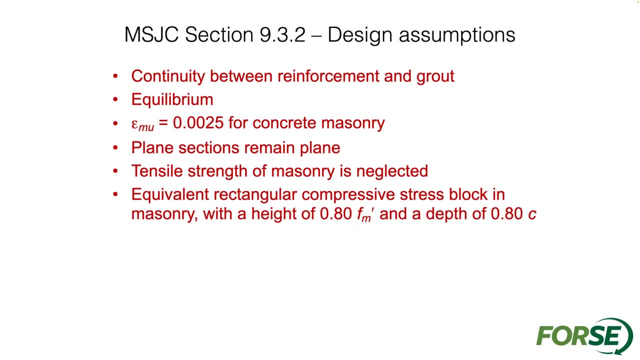 again design assumptions. there's strain, compatibility between reinforcement, grout, masonry. you know, reinforcement requirements, details, all those different sections for design of reinforced masonry, the continuity between reinforcement and grout. we have some equilibrium for concrete masonry. plain sections remain plain. tensile strength of masonry is neglected. equivalent rectangular compressive block in masonry. 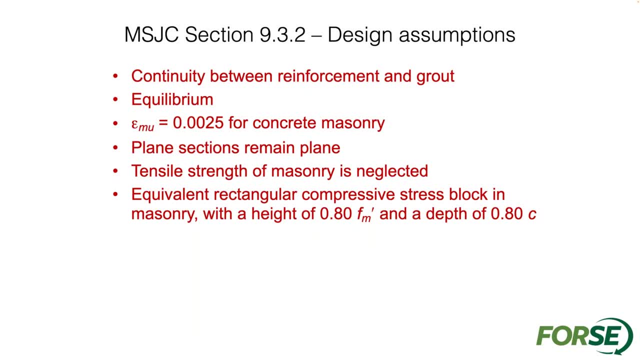 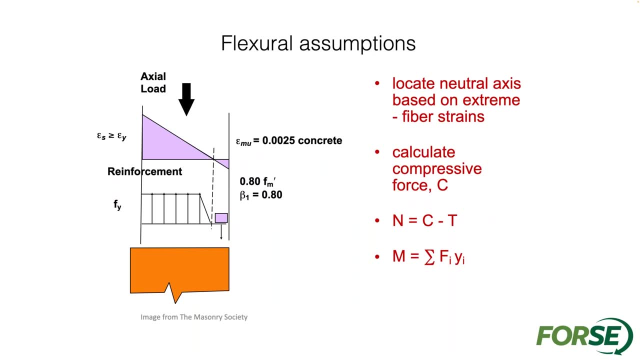 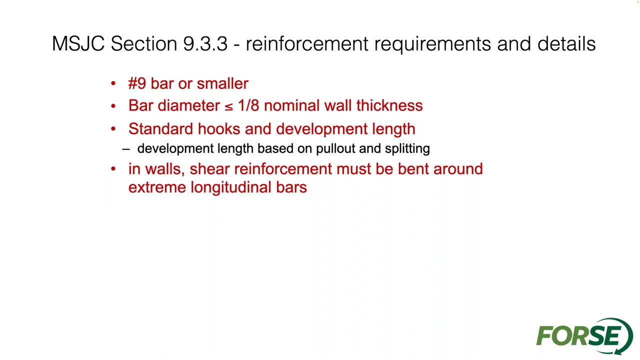 with a height of 0.8 times f, prime m and 0.8 times c. so we look at the overall stress strain force diagram that you have, so obviously you can see that tensile force be there for reinforcement. go back into the reinforcement section. we again see the provisions in there for number nine bar. 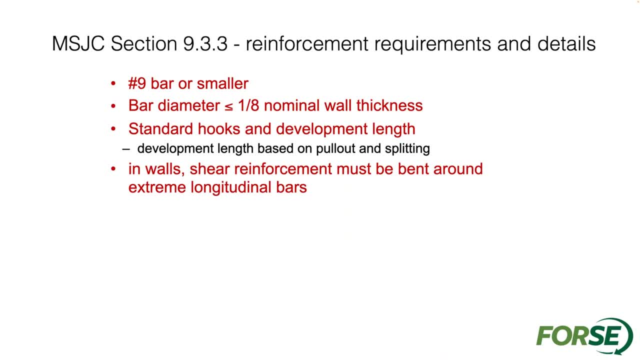 or smaller bar diameter, less than the overall wall thickness which we talked about. and then we have hooks that we can use within mainstream walls. hooks obviously need to be detailed very carefully within a major wall. again, we're dealing with confined spaces, so how can the hooks be? 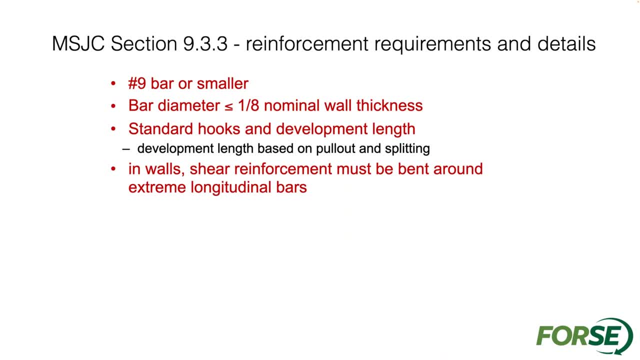 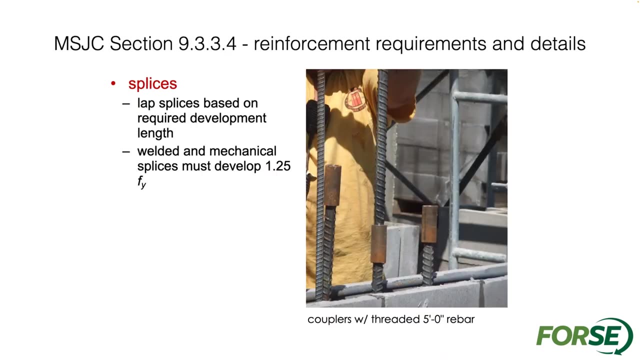 placed and located? do we have bond beams and do we have right types of blocks that allow for hooks to be utilized? development length and wall shear reinforcement must be bent around extreme longitudinal bars. um, good detailing requirements. uh, if we do get into splices, we have welded or mechanical splices. 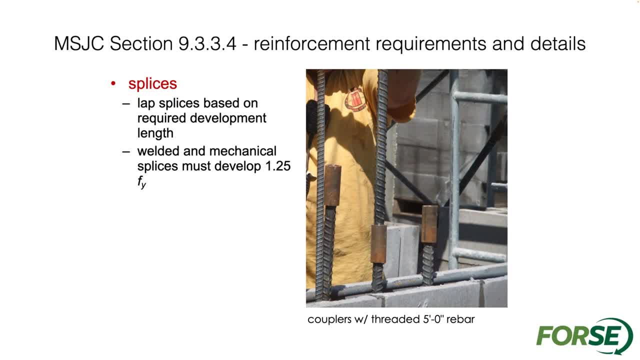 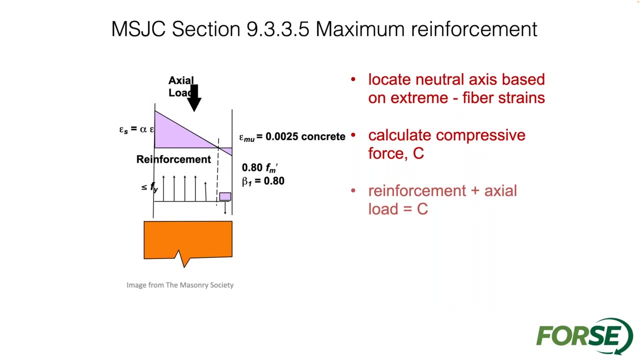 have to develop 25 more capacity than the overall bar itself. so making sure that we have good force transfer from one bar to the next is obviously going to be very important. we have maximum reinforcement provisions for reinforcement within a wall. we can't just add a wall after a stop. 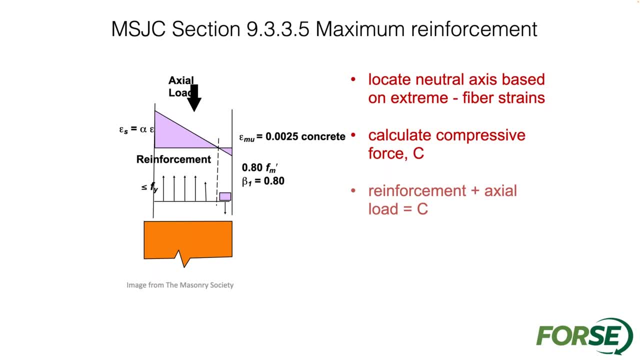 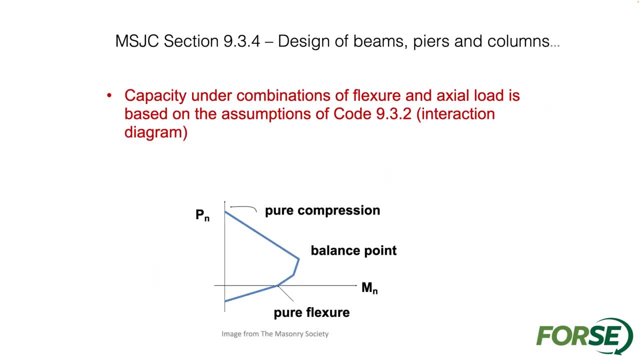 add number 11 bars to a six-inch wall. you're probably gonna have too much reinforcement in that wall, so there is some maximum reinforcement. there's your axial moment curve. we have balance, compression, we have tension, and so we obviously need to stay within that capacity curve. 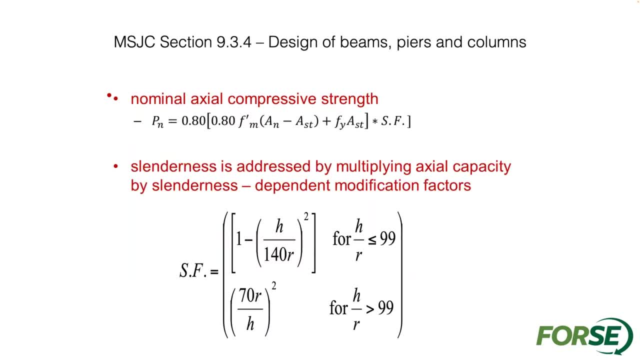 design of beams, peers and columns. we have nominal axial compressive strength. we have axial force, point eight. point ten, strength of masonry, different variables in there for areas of steel. we have a slenderness factor that we have to determine for different height walls, making sure that we have basically a 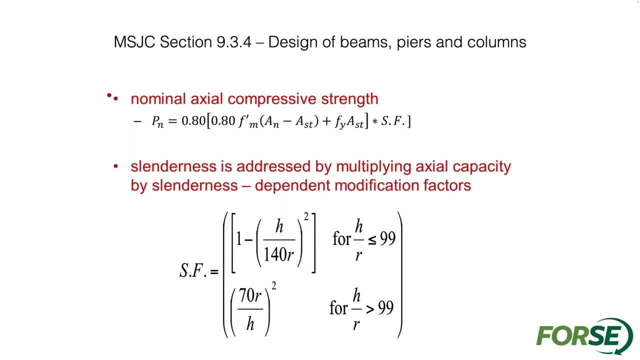 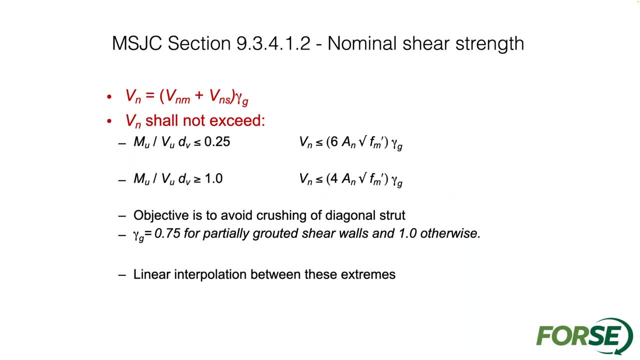 p-delta effect that we're taking into account of and make sure that we consider that with a in our design we have different shear capacities depending on the different moment to shear ratio that we have for the member. the lower moment to shear ratios we have B? n times six times a? n over square root of f, prime M versus the. 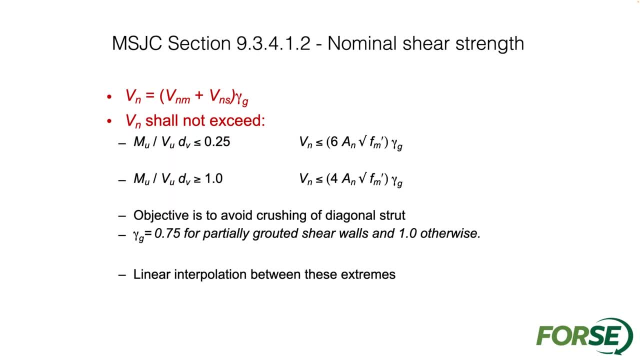 higher moment ones, we have a little bit less capacity. there's three percent less capacity. objective is to avoid crushing of the diagram of the beam, and then we're going to have to determine what the, the signal strut, so on and so forth. we linear interpolation between the 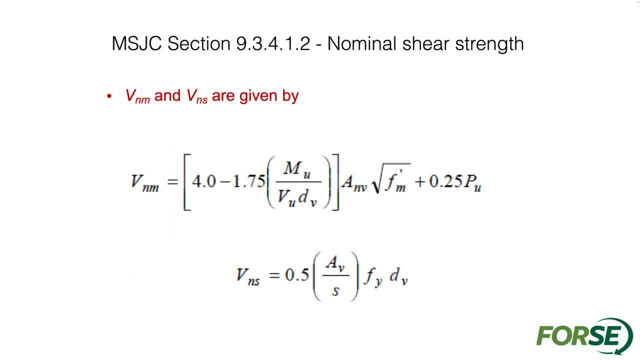 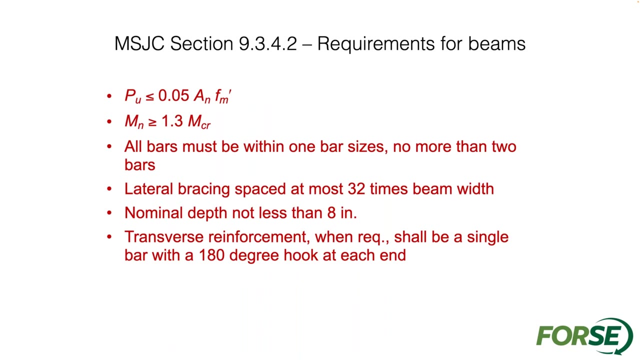 extreme values, then obviously there's more capacity that you can develop. if you wanted to add in some steel for shear strength, you have the shear strength provisions and then shear capacities with steel axial moment capacities for beams. all bars must be within one bar size, no more than two bars. 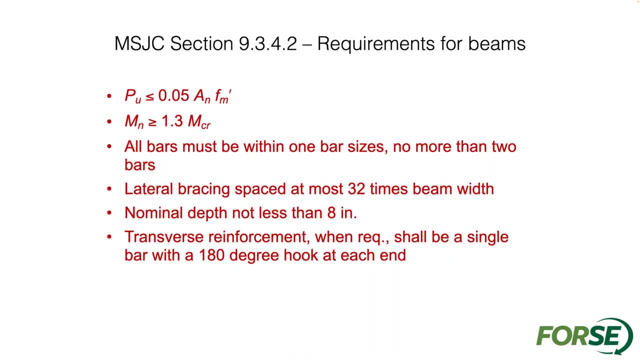 lateral spacing space more than 32 times the beam width. nominal momentum depth not less than eight inches. I think it'd be hard to have something that would be that shallow transverse reinforcement when required shall be a single bar with 180 degree hook at each end. 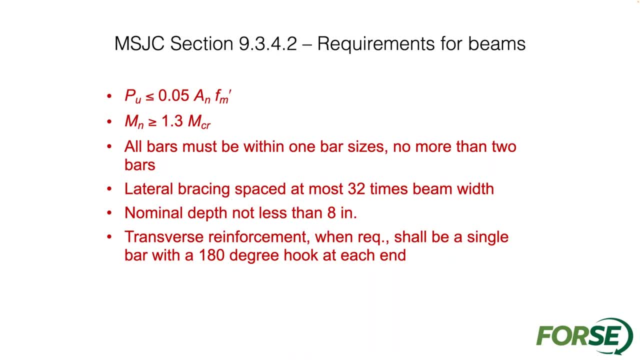 I mean, it's really kind of looking at. you know, anytime that you have sheer reinforcement, transverse reinforcement for beams lentils within a wall, you have to make sure that it fits in and works within the wall itself. reinforcement for piers, isolated elements, got a different. 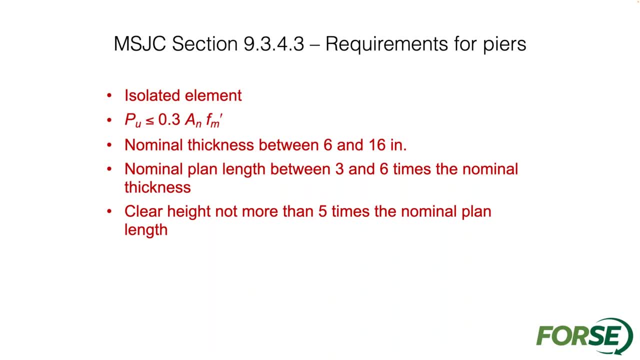 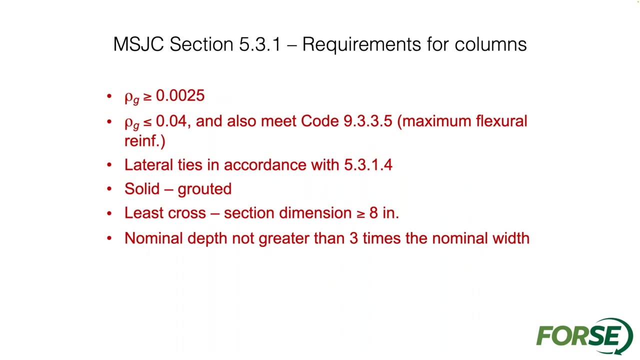 axial equation: thicknesses between six and sixteen inches. nominal plan length between three to six times the nominal thickness. clear height: not more than five times the nominal plan length. again, we have reinforced requirements for columns. we have different ratios for reinforcement that we want to add. we have lateral ties that we can include. remember that we do also have. 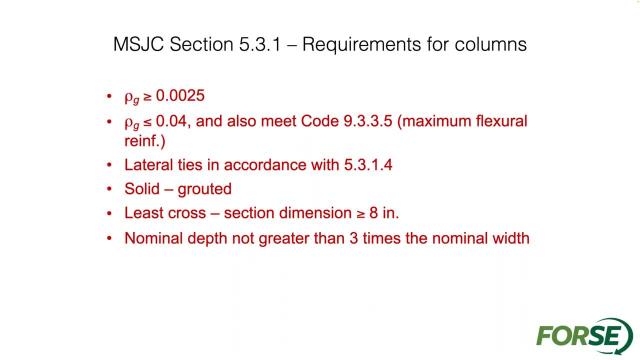 the ability to have a lightly loaded column that we can consider. we have a least cross-sectional dimension which is eight inches by eight inches. that's a pretty nice little small kind of masonry column that we can consider. nominal depth: not greater than three times the nominal width for different walls. we have all kinds of different forces that we have. 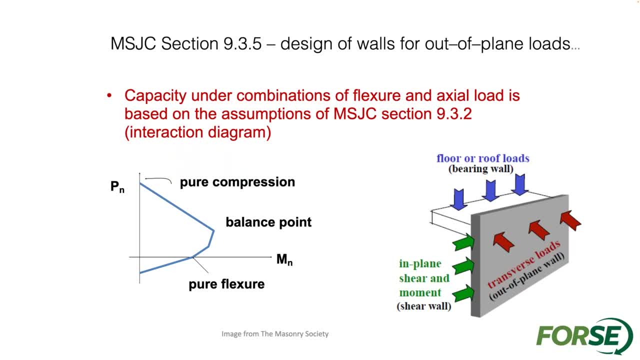 to consider capacity into the combinations of flexor and axial load is based on the code nine, point three. point two: you know we have out of plane forces, we have in plane forces and then obviously we have axial forces, that we have axial load and moments. so all things that we want to. 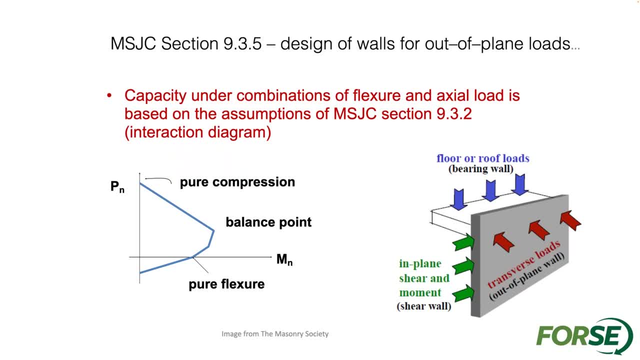 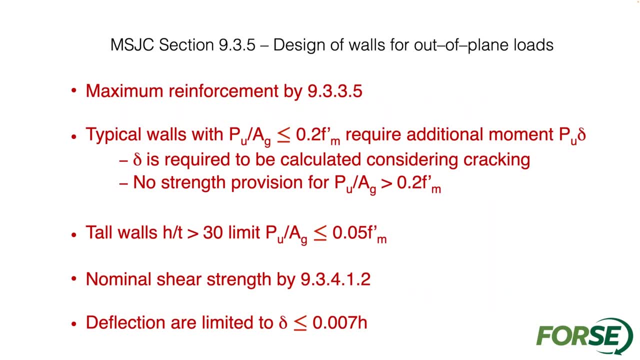 consider when we are checking the capacities of these walls and different sections for maximum reinforcement: typical walls, the, the tall walls. height, the thickness ratio of 30, we have a limiting value of the axial load to the growth section area and then we have deflections are limited to Delta. 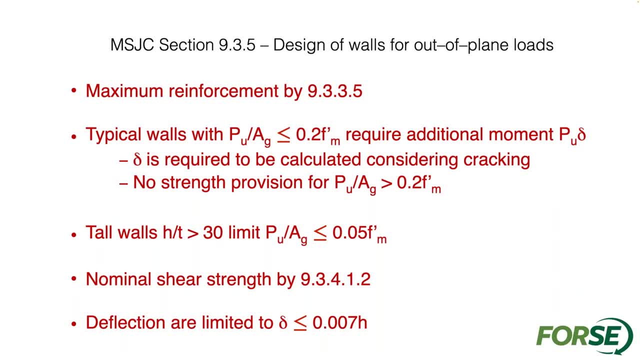 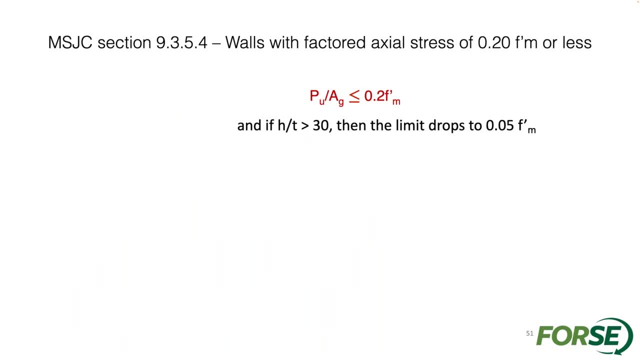 times the height, So that's something that creates a deflection that I think is probably more than what most people are used to, but making sure that we stay within that code requirement would lead to a safe design wall And anytime that you can be less than axial. 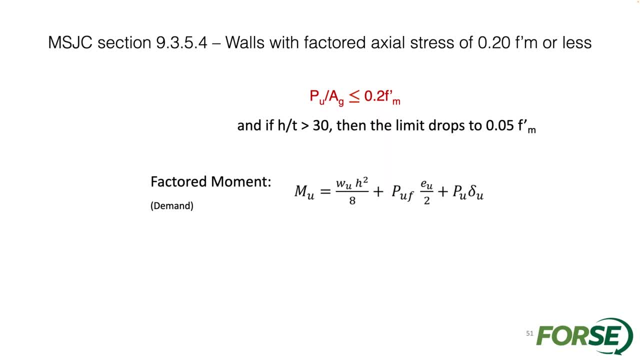 to the gross area less than 20% of F prime M. then we have a factor moment that we can utilize Taller walls. if the thickness is greater than 30, then the limit to the axial force on a wall drops to 5% of F prime M. So again we have all these different equations and 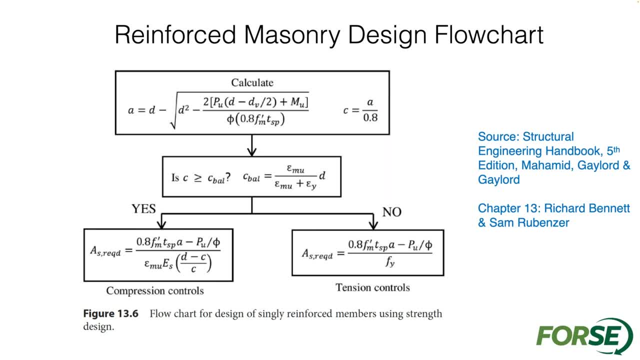 I'm obviously not going through each one of them. We have tension controlled compression, controlled designs. We have a nice little handbook that we can see, with the chart in there, to help us make some design decisions A lot of times. I mean, you know, I'm going through this stuff pretty quickly because 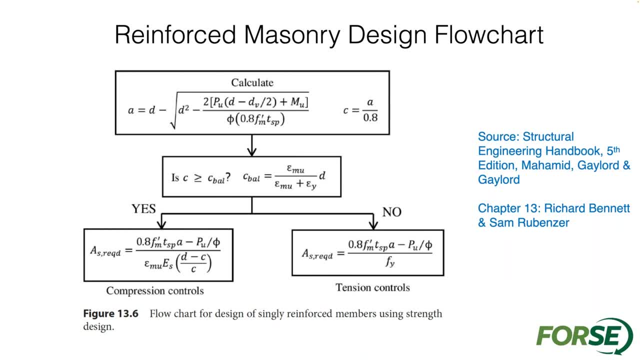 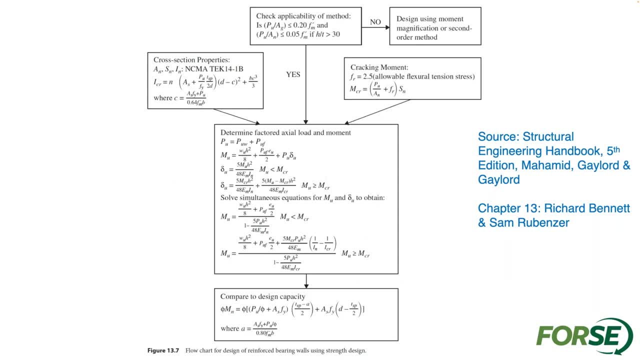 a lot of times our designs are going to be based on a computer or a spreadsheet or something like that that we're designing, So I'm not going to go through these really in depth. Another flow chart, more and more in depth to determine the overall capacities for moment. 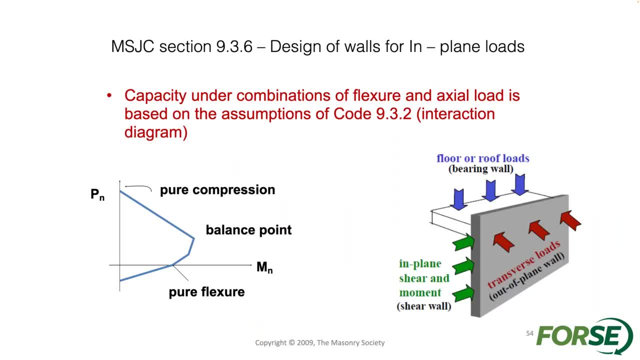 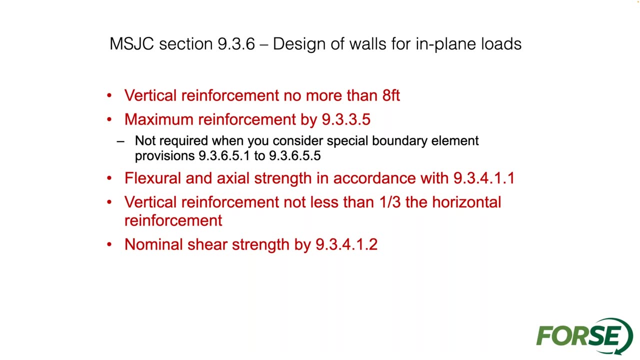 and shear for our designs. Then the in-plane forces, obviously having a lot of the similar requirements, a lot of these similar Bending and shear capacities that you would have Other things about in-plane designs: vertical reinforcement not more than eight feet. so 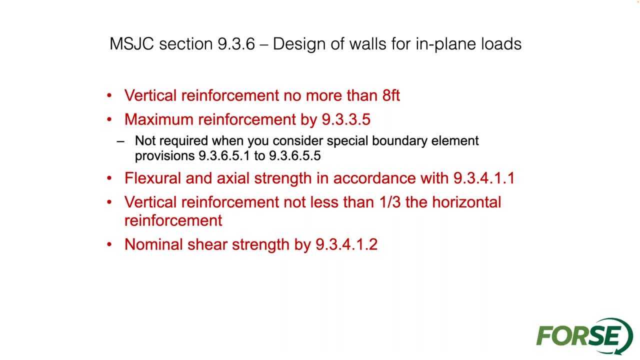 not more than 96 inches on center. I think that might be a little bit of a surprise to people. A lot of times people put a lot more reinforcement in walls than every eight feet. So really it's not until you get into looking at the wall for in-plane loads for the wall. 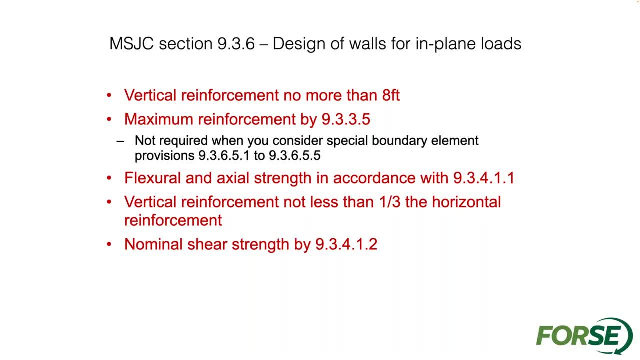 being a shear wall could be an ordinary reinforcement, But if you get into a reinforced wall, that's when we have to start putting some reinforcement in there, not more than eight feet apart. So again, that's when some minimum reinforcement provisions start to kick in. 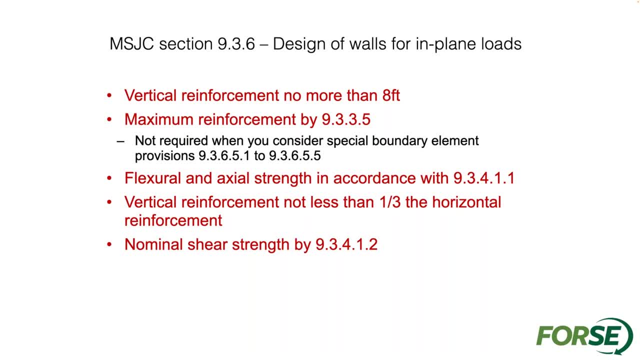 But, like I said, I think that would be a surprise to a lot of people. A lot of people would put in reinforcement a lot closer than eight feet on center to start. So flexure and actual strength based on 934.1.1 vertical reinforcement, not less than one-third of the wall. 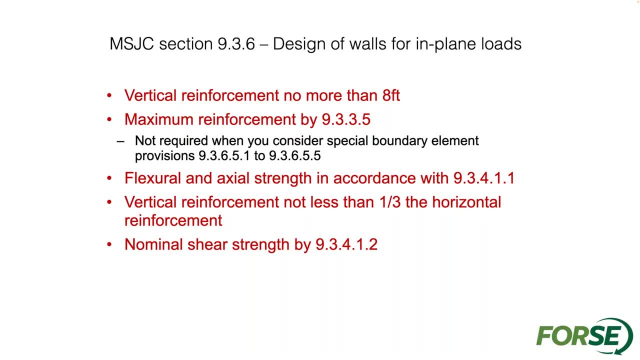 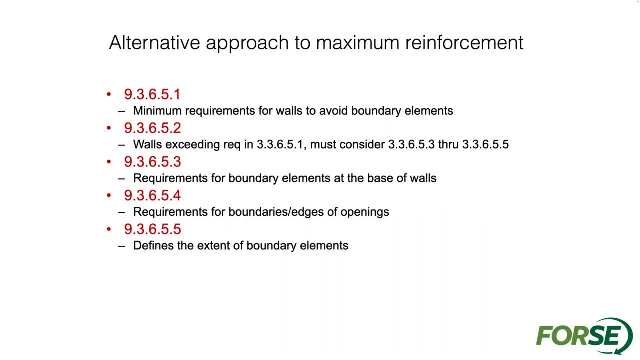 The horizontal reinforcement. so we want to make sure that we have a decent amount of vertical reinforcement. in the wall Nominal shear strength provisions There's an alternate approach to maximum reinforcement. I mean you have minimum requirements for walls to avoid boundary elements based on 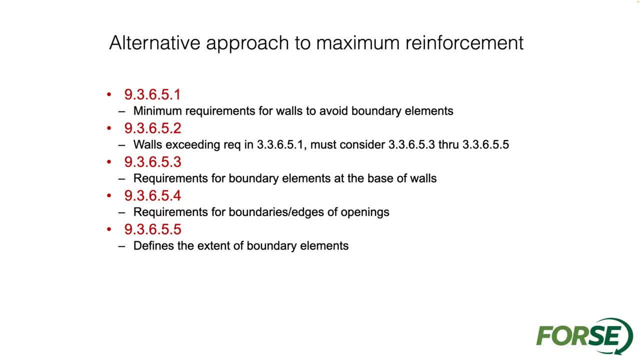 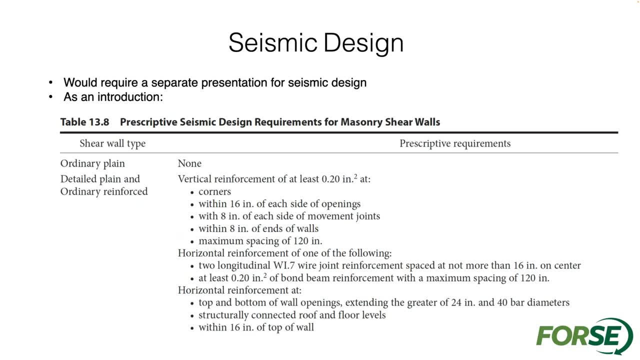 certain provisions within the wall, All kinds of things that we get into when we get into kind of special design of the masonry walls And a couple of different charts here that we can with a separate for a separate seismic design, just kind of with some pretty straightforward information. 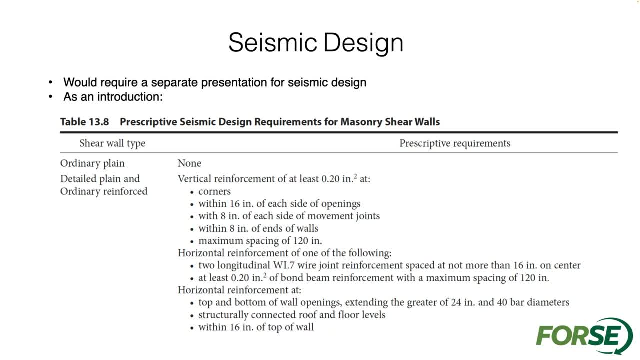 An ordinary masonry wall doesn't have any prescriptive requirements for seismic design. You get into the detailed plane and ordinary walls. That's when we start to get into some design provisions. here We have basically a number four bar that needs to be placed in the corners within 16 inches. 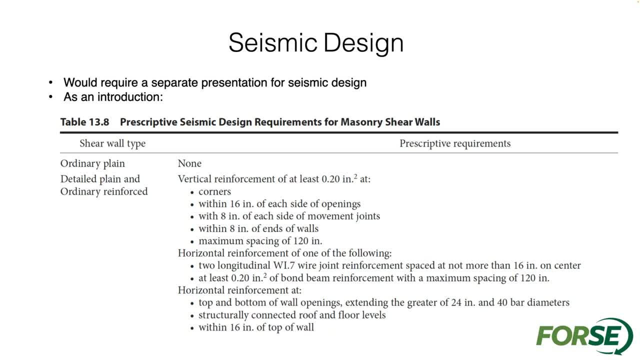 of the side of the openings, within eight inches of the each side of movement joints, within eight inches of the ends of the walls and then a maximum spacing of 10 feet on center. So detailed, ordinary reinforced walls just don't have a lot of requirements. 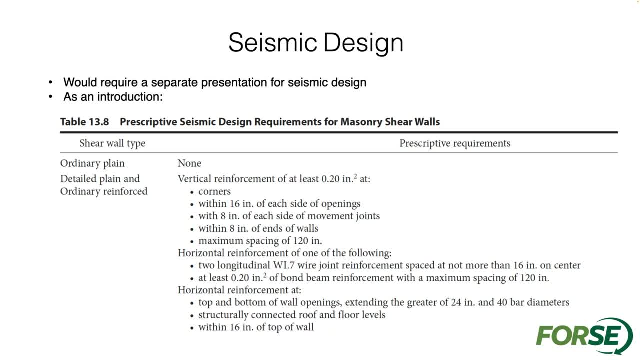 Two longitudinal, basically nine gauge wires at 16 inches on center, or a number four bar with a maximum horizontal spacing of 10 feet. All right, So again pretty, pretty minimal requirements: Horizontal reinforcement at the top and bottom, basically boundary reinforcement, and within 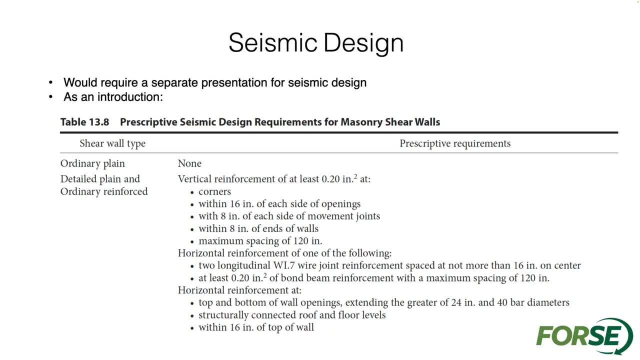 a wall within 24 inches or 40 bar diameters, structurally connected to roofs and floors and within 16 inches of the top of the wall. So an ordinary reinforcement just doesn't have. it's not that much that it demands and requires for your design. 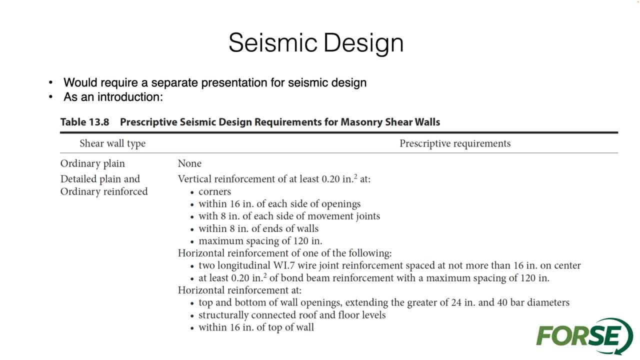 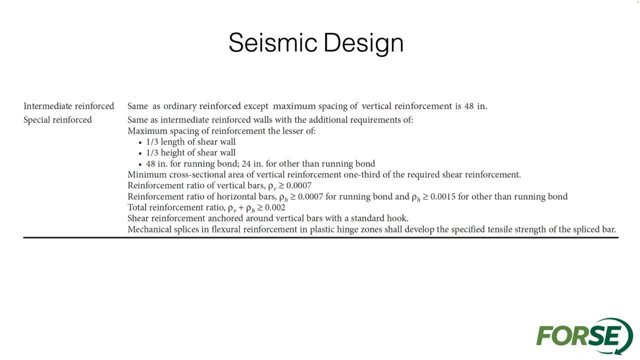 We really do have. It's really the intermediate reinforced walls. If we skip to that, that's when we really have all the same requirements that we had for the intermediate. it's going to be the same as the ordinary reinforced, except for the vertical spacing is limited to 48 inches on center. 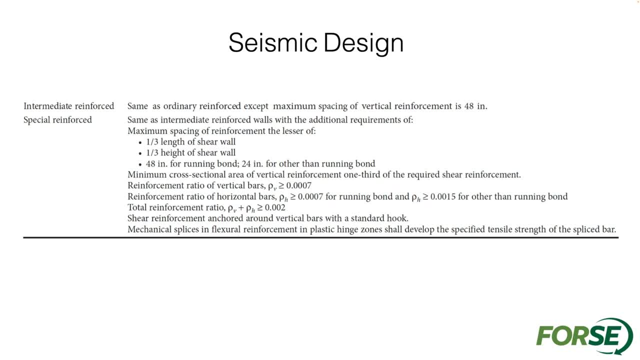 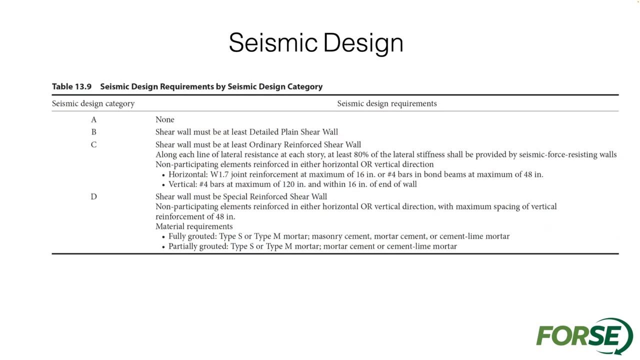 Even especially reinforced. then you have all kinds of other consideration to look at. You have reinforcement, that's tighter together. You have reinforcement ratios- Really, really Really kind of looking at more and more of a ductile response for the wall. If we looked at again size, design category, it doesn't really have any A, doesn't have. 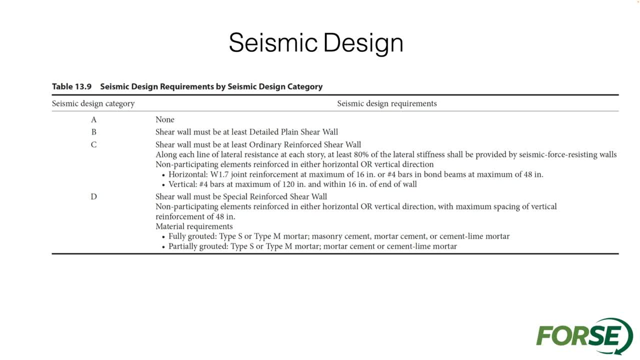 any size and design requirements. B- you get into, shear walls must be a detailed plain shear wall. C- you can get into still having an ordinary reinforced shear wall When you get into. D, when you have to have a shear wall designed to be especially reinforced. 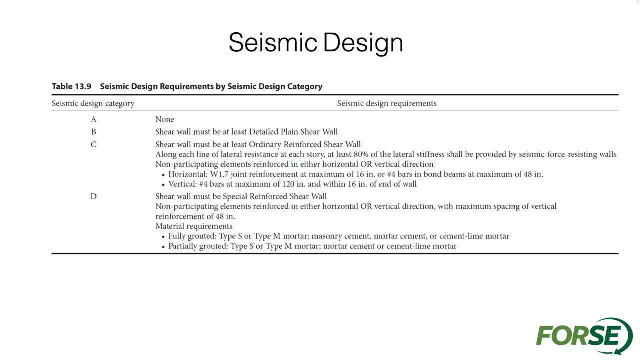 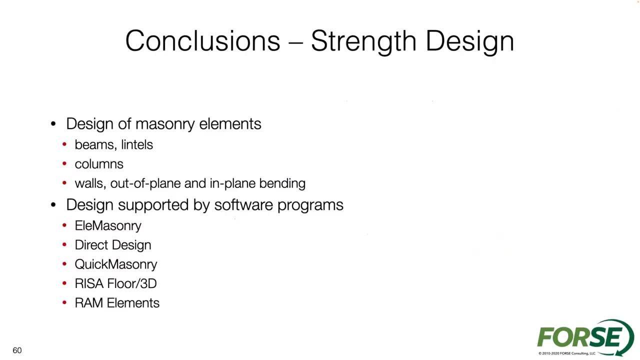 So that's the first thing. Okay, So, in terms of our seismic design, really looking at strength design and- and you know whether it's going to be beams or lintels, columns and walls out of plane and in-plane bending, all kinds of different provisions. 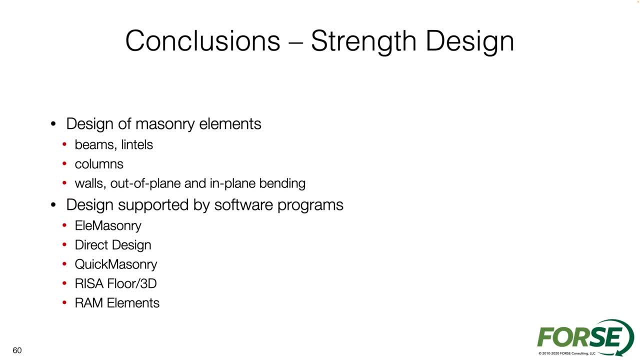 And then where is it going to be used. So the strength design is going to be also in the different software programs. Again, it's going to be the last section today but obviously going to be able to use that within all the different Softwares that we have, all right. 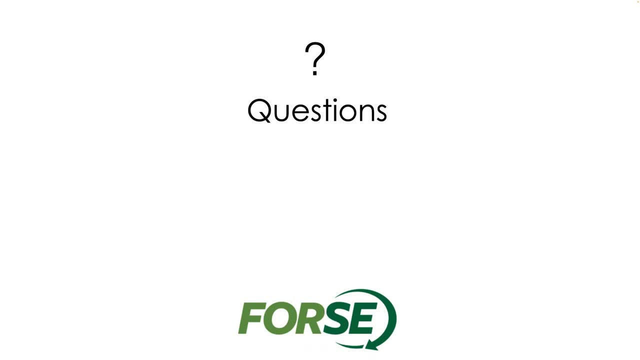 So that was a little bit of a brief section that there's a lot of equations, a lot of stuff that I didn't want to spend too much time on today. I don't want to put anybody to sleep, So we wanted to move through that section a little bit quicker. 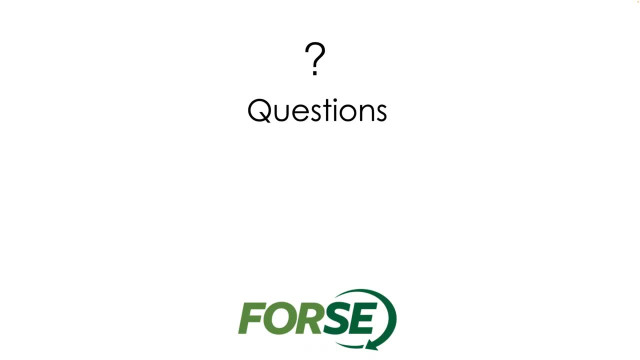 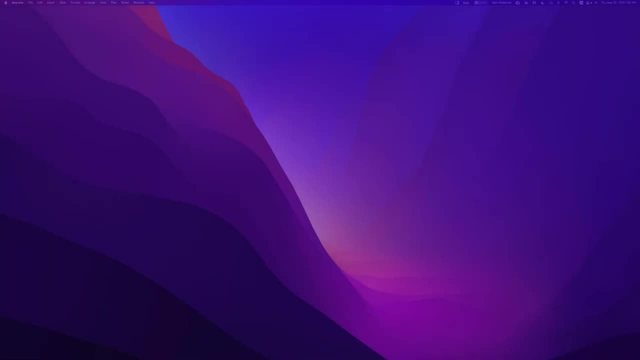 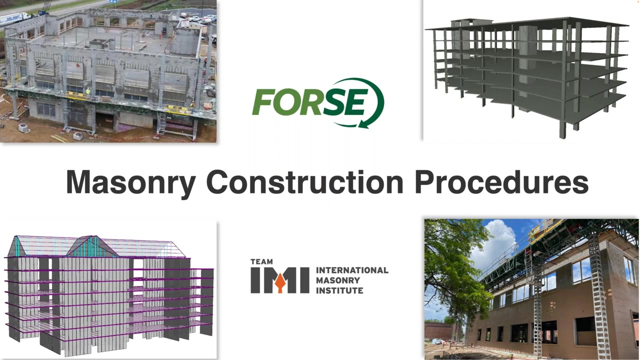 But again, if anybody has any questions, like I said, a lot of design equations. take a second here to switch between this and the next section. Okay, it doesn't look like we have any questions that popped up there. I'm just going to give it another minute just in case anybody's writing something and wants. 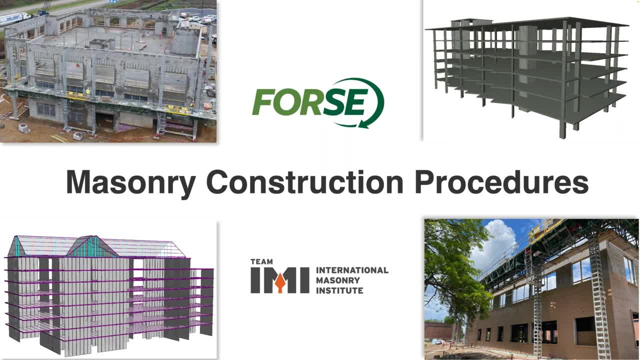 to take a moment to ask a question, but I'm going to give it another minute just in case anybody has any questions. Okay, so the next section here is going to be maybe a little bit more on the practical side of masonry, the different topics and what I would call the wall construction procedures. 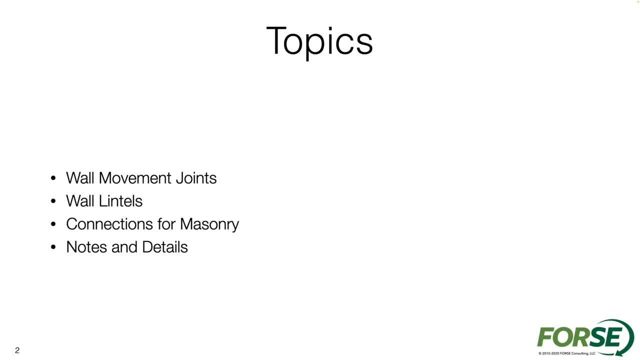 would be wall movement joints, wall lintels, connections for masonry and then notes and detailing. So I would say, if we get through the first two parts of this section- wall movement joints and wall lintels- hopefully we can move through a couple of those before the lunch hour. 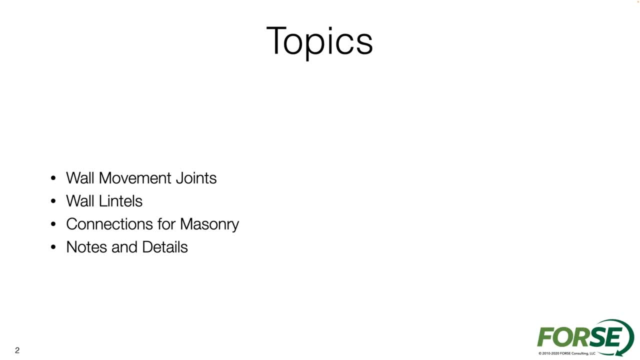 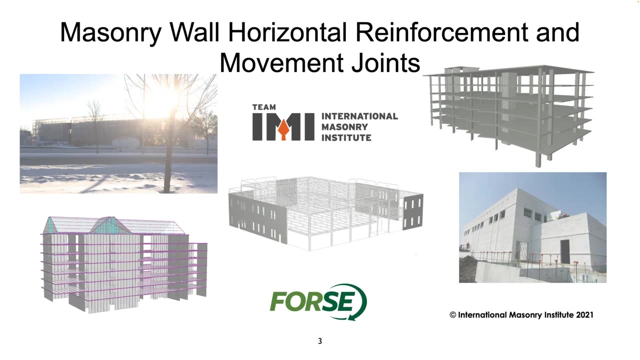 That would be good. Let's see how long those take, and then we can kind of see where we are before we take some time for lunch. All right, still no questions. All right, let's keep moving forward. All right, so the wall, masonry wall, horizontal reinforcement and movement joints. 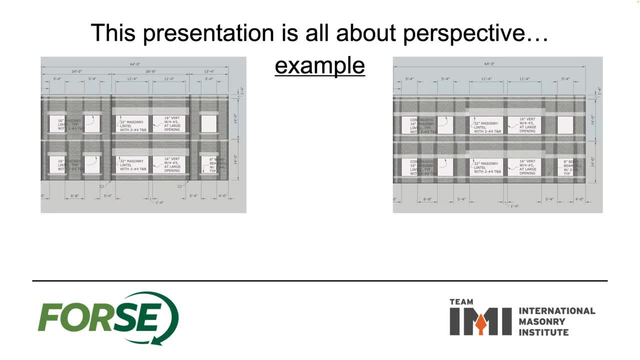 If I looked at a wall like this kind of a common wall, I really have a couple different options. or we have a lot of different options for this wall movement joints. you know how much horizontal reinforcement with or without a control joint. you know that really. 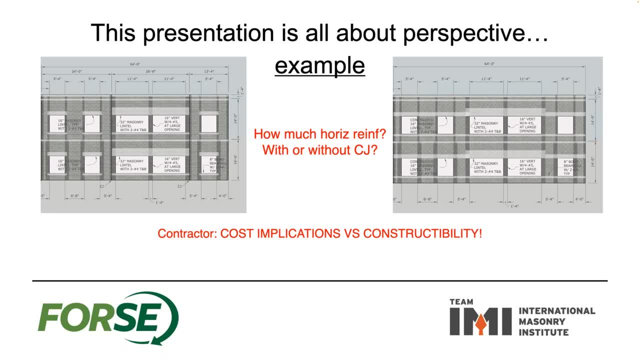 has implications, obviously: cost implications and constructability. You know two different things. you know, if I'm looking at these different options for these walls, you know architects might say: you know how does it look? Will this crack? 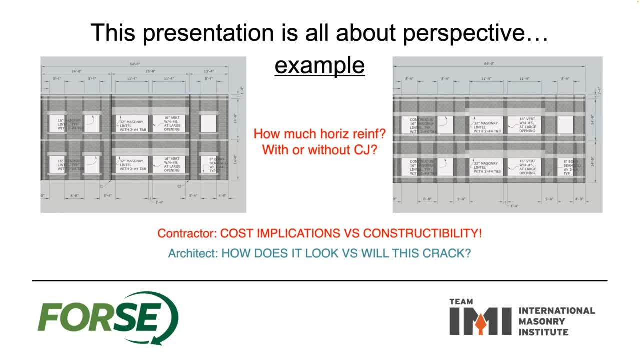 I mean, obviously those are going to be things you know designers will look at And then if you're located in Wisconsin or in the Midwest, people, engineers, might ask you know who designs without a control joint? you know, in certain areas of the country. 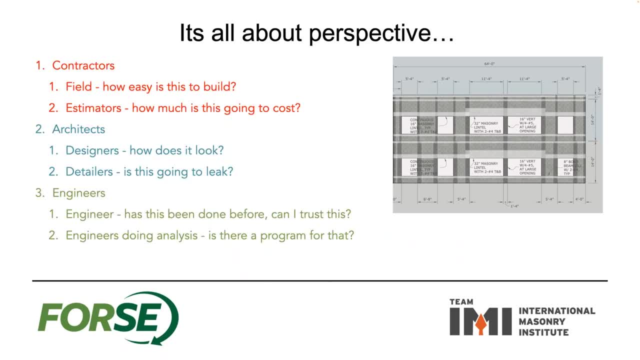 I mean, you know how easy is this going to be to build if I took out, you know, control joints? How easy is it to design this wall with no control joints? you know how much is it going to cost? It's all kinds of different questions. 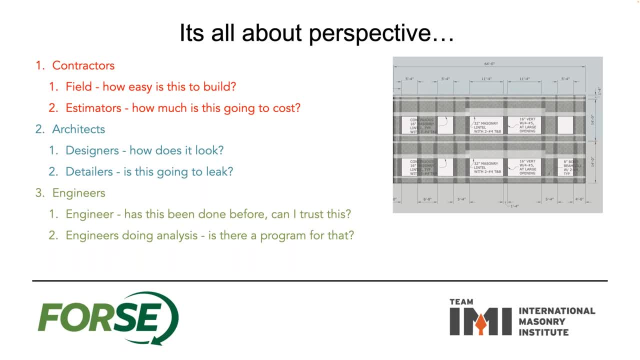 So really what we try to do is we try to come up with different options for contractors so that they can price out different options. Obviously, this is just one little example, one elevation, you know. and then you know if I do take out control joints and stuff like that, you know I'm making the design. 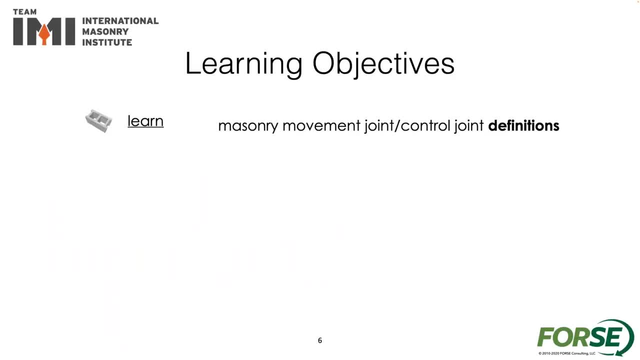 more complicated. Designers need to be able to design this thing. So let's talk a little bit. Let's talk a little bit about movement, joints, control, joint definitions, horizontal reinforcement options. We talked about what horizontal reinforcement we have, but what are some of the different? 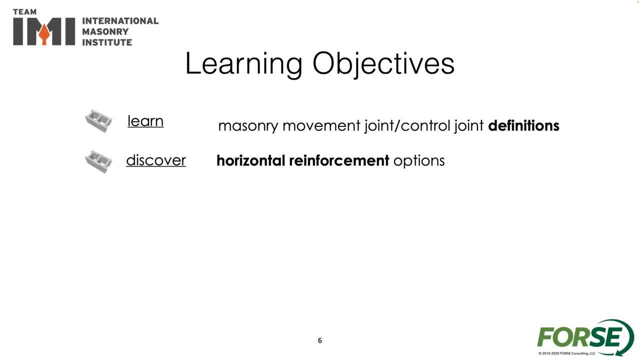 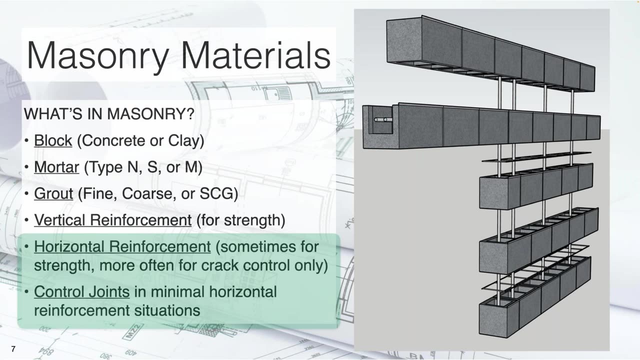 options that we can utilize, understand the balance between control, joints and reinforcement, And then the structural impact of the various options. So this is a slide that we looked at before right, The different materials of masonry. really, we're going to kind of focus in on the last. 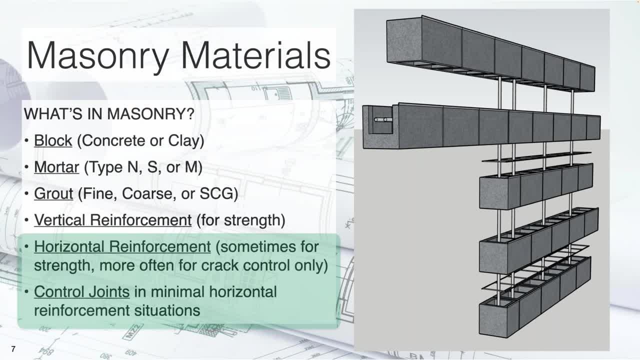 two here: Horizontal reinforcement. Like I said, the horizontal reinforcement can be used for strength design. you know whether it's shear for the wall or if it's horizontal bending. Most often horizontal reinforcement is going to be there for some respect of crack control. 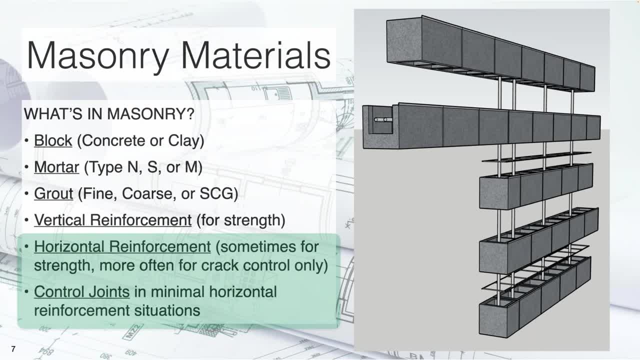 as we go through the different shrinkage in temperature, stresses and forces that are on the wall And then control joints and horizontal reinforcement situations. We're going to look at that And then control joints, And then control joints And then horizontal reinforcement situations. 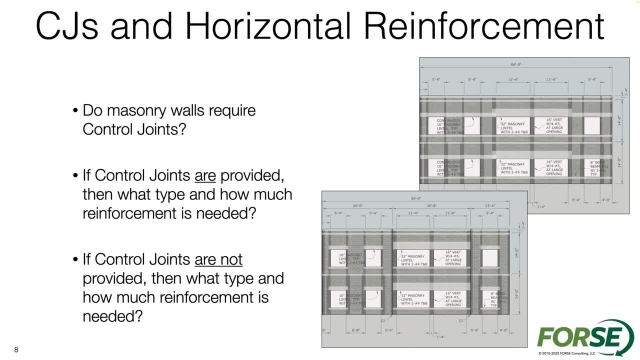 We're going to look at that. We're going to look at where we want to put control joints. One of the first questions that I like to ask is: do all masonry walls require control joints? And then, if control joints are provided, then what type and how much reinforcement is needed? 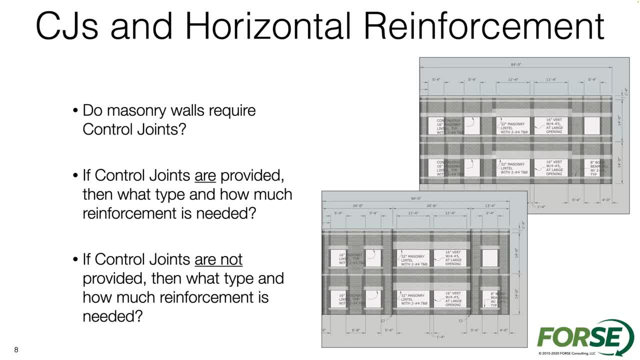 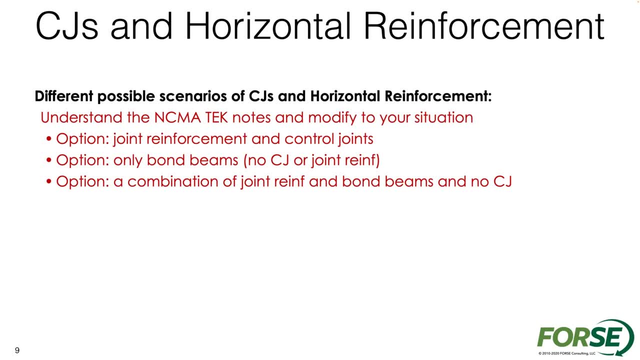 If control joints are not provided, then what type and how much reinforcement is needed. So again, within the code it's kind of silent in some of these topics. so I think that that's good to understand. You know different possible scenarios of control joints, because there's kind of this: 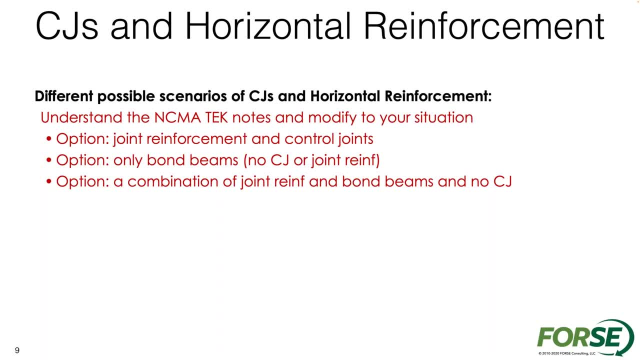 balance. The more control joints you have, the less reinforcement that you need. If you don't have any control joints, then you have to have much more horizontal reinforcement. So the different NCMA tech notes are going to be where we come to for getting some of. 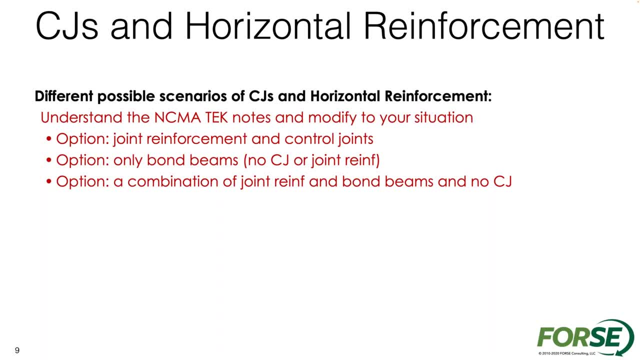 the guidance here. One option can be joint reinforcement and control joints. Another option could be just bond beams with no control joints or joint reinforcements. So we're going to look at that And then control joints, Joint reinforcement, And then another option might be a combination of joint reinforcement and bond beams in minimal 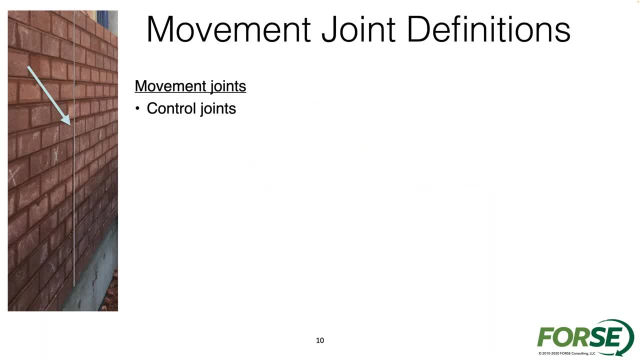 or no control joints. So movement joints within a masonry wall, often within a structural wall, are going to be called control joints. We just label them as CJs, which is going to be common for structural masonry design. Expansion joints are going to be things that are obviously a little bit different. 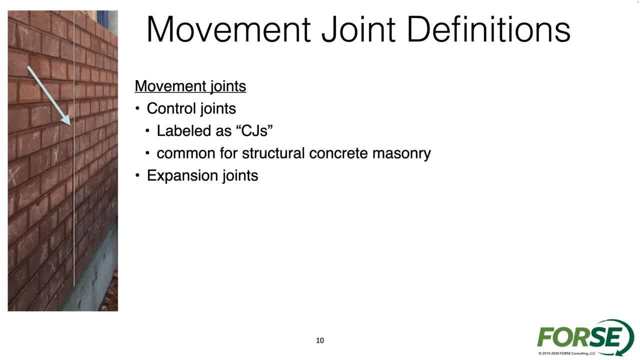 They're going to be a little bit of a different. They're going to be a little bit different, Different reasons for putting in expansion joints. We label those as maybe EJs. They're going to be common for the structural clay masonry or just common clay masonry. 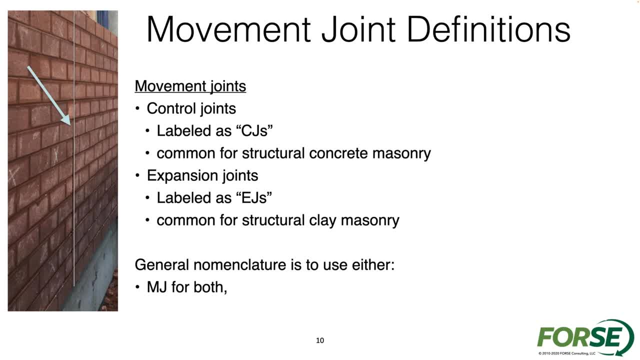 So today we're just going to kind of maybe do nomenclature. I mean, when people put these on plans, it's either EJs and CJs or you could just call everything an EJ. It's basically like a block for M&J or M&J-movement joint for now. 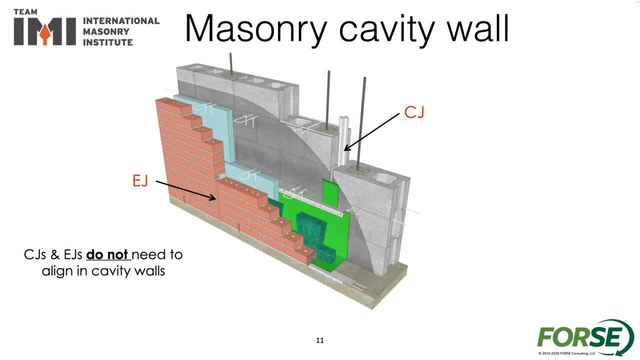 One of the very important things to remember with it, especially if you have a cavity wall. any time that you're looking at differences between masonry walls, an unreinforced wall has different requirements for movement joints than a reinforced wall, So an unreinforced wall might have expansion joints at certain locations. 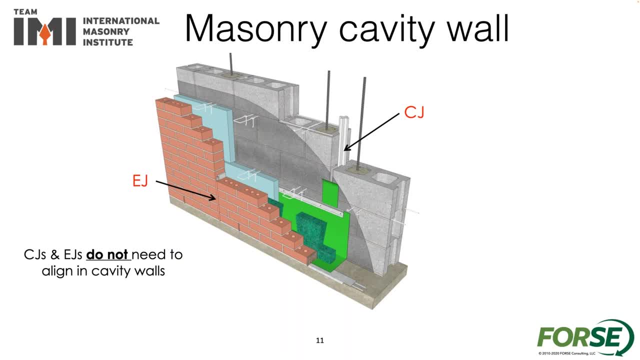 You might want various kinds of expansion joints. You might want to be really careful certain locations, because the wall is unreinforced. When you have a reinforced wall you're going to have again different requirements and those maybe are going to be called control joints. 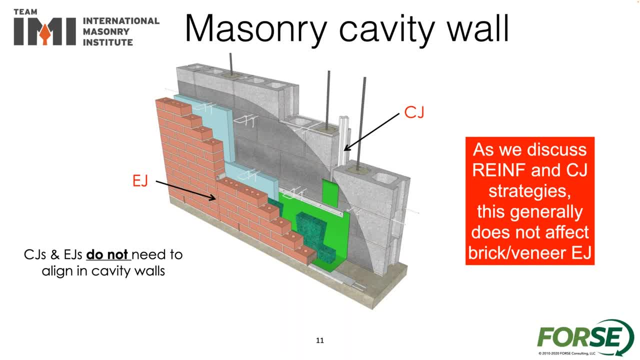 So they're very likely not going to be at the same location within a wall And there's really no requirements for having those joints aligning within a wall. The veneer ties that we use today if you have a cavity wall allow for the different movements to be occurring within the walls. 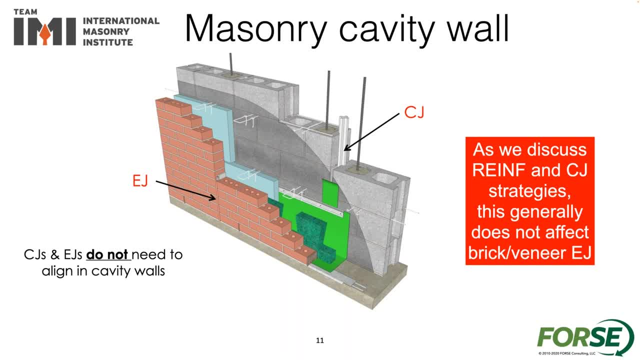 And so it really does allow for those joints to be in different locations and really those walls to be acting independently, And so that's going to be something that's pretty important to remember: If we have those joints, they're going to be in unreinforced and reinforced walls. 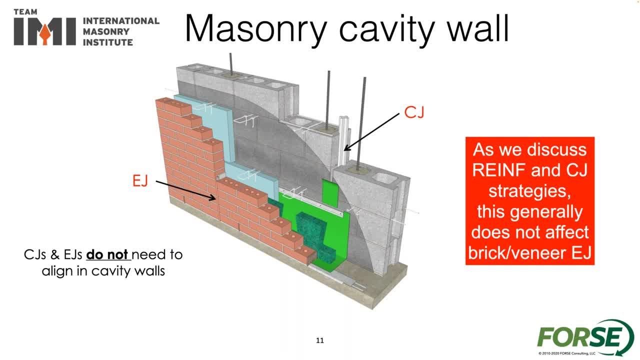 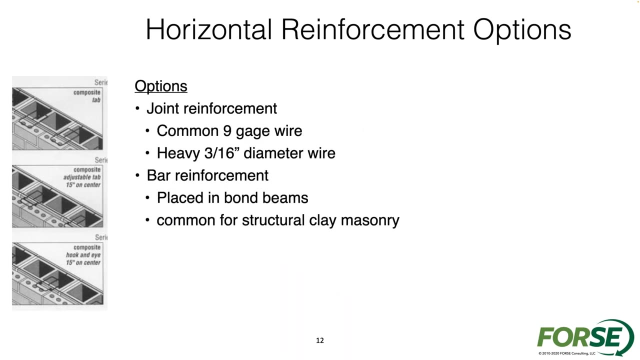 in completely different strategies, different locations, and they do not need to align. In fact, I would probably say that they should not align. I think you'd want them to not align in your designs. So again, our different options for our horizontal reinforcement. we have joint and bar reinforcement. 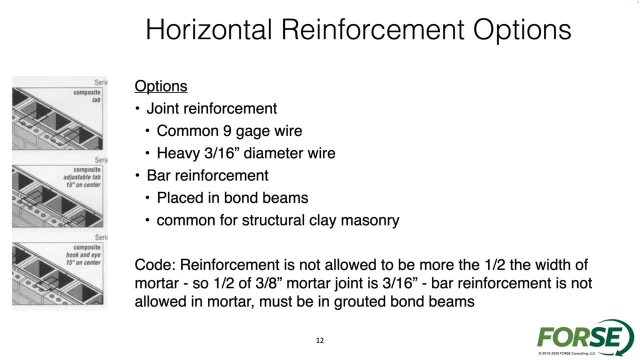 that we can add. Code says the reinforcement is not allowed to be more than half the width. So that's why we have a three-sixteenths inch reinforcement that's allowed. And so how much and where? So we have these different options for where we're going to have the reinforcement. So 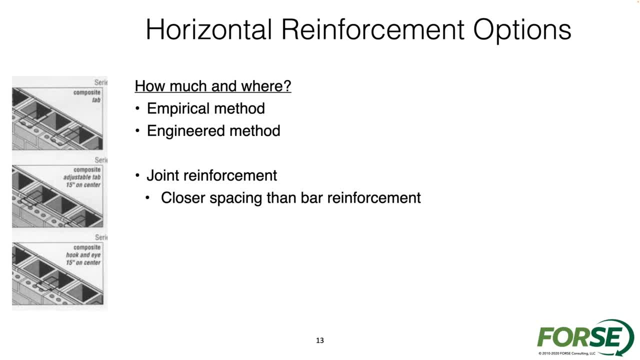 we're going to put the reinforcement. we have empirical engineered method, joint reinforcement. Joint reinforcement is going to be a lot less area of steel, So that's why it's going to be closer than bar reinforcement. Now, bar reinforcement we can put quite a bit of steel, say within a 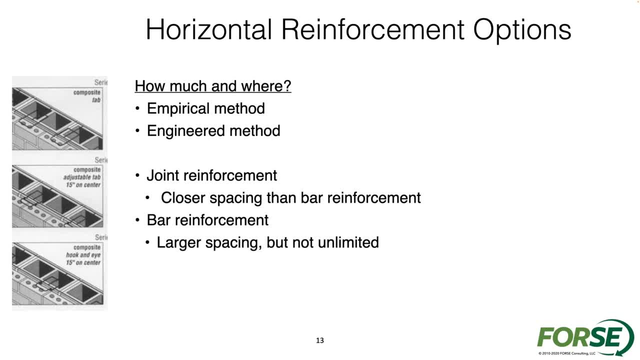 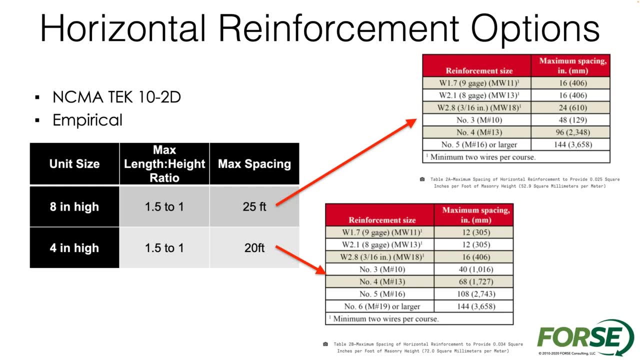 bond beam, but it's not unlimited. the spacing that we, like I've said before, code can be kind of silent, which is why we turned to the tech guides. Within the tech guides, what it does is it points to horizontal reinforcement options. If I have eight-inch high, 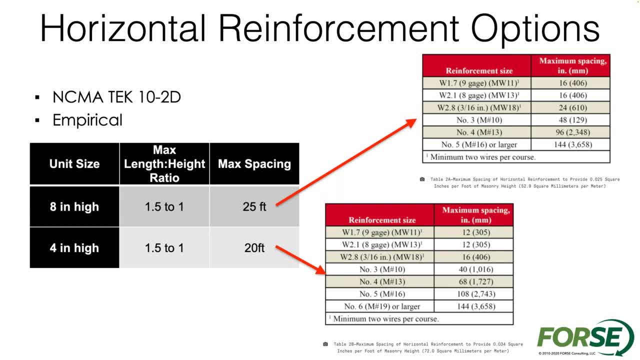 eight units. NCMA tech guide 10-2,- this is an empirical method- says that we have a length a wall to height of the wall ratio that can be 1.5 to 1, with a maximum spacing of 25 feet for. 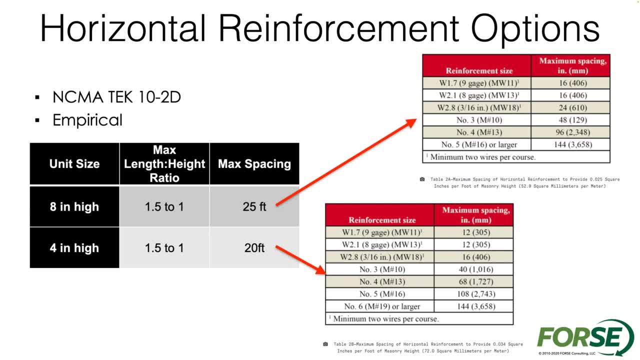 eight-inch high. So a common concrete masonry design is going to give us that joint reinforcement at that spacing. So that's why we can see nine gauge at 16 inches on center. That's the very, very common. So that's why we can see nine gauge at 16 inches on center. That's the very, very common. 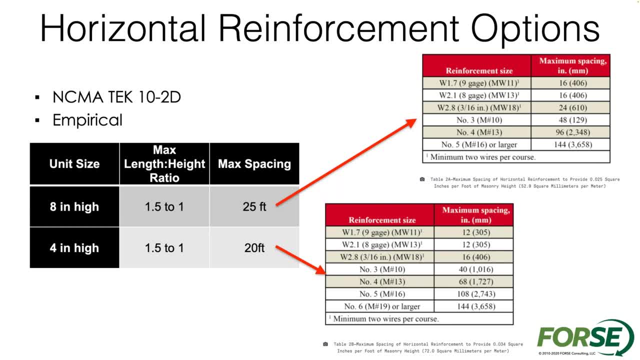 So that's why we can see nine gauge at 16 inches on center. That's the very, very common way to put in horizontal reinforcement. We can also see within that table, though, if I put one number four bar every eight feet or number five bar every 12 feet. 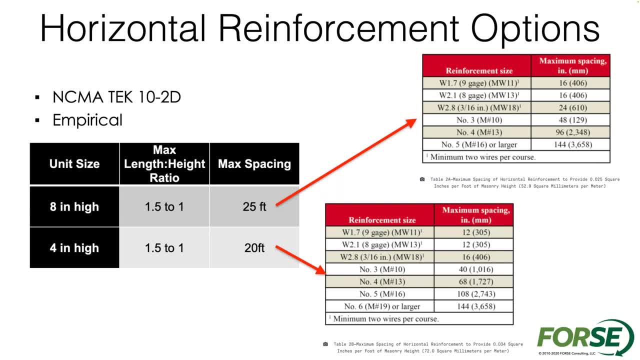 that's sufficient amount of horizontal reinforcement. You don't need to have both. If we decide that we're going with horizontal bar reinforcement, then I just use the number five. I don't have to put in joint reinforcement. If I just want to have joint reinforcement, then obviously 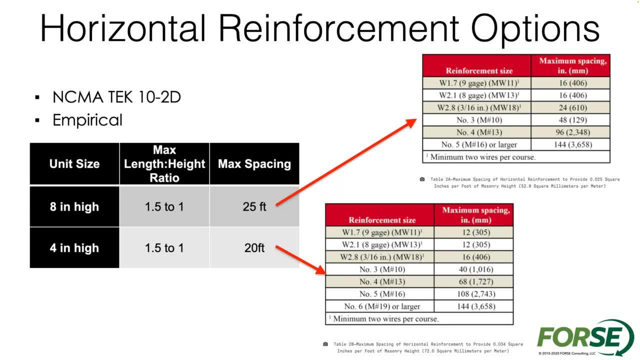 I don't have to have bar reinforcement. I've seen designs, I've reviewed designs, where people tend to put in both- maybe kind of a belt and suspenders, which just isn't necessary design-wise, And then anytime you have a four-inch high. so obviously we're getting more into a clay. 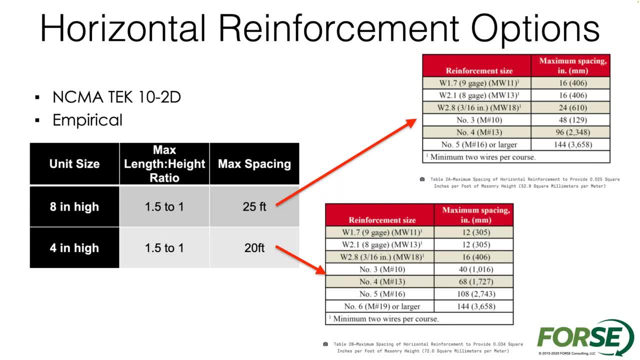 reinforced clay, masonry or half-high concrete units. then we have slightly different maximum spacings that we would want to use for the different reinforcement requirements. So that's the empirical design method. This is kind of independent of anything. So that's the empirical design method. This is kind of independent of anything. 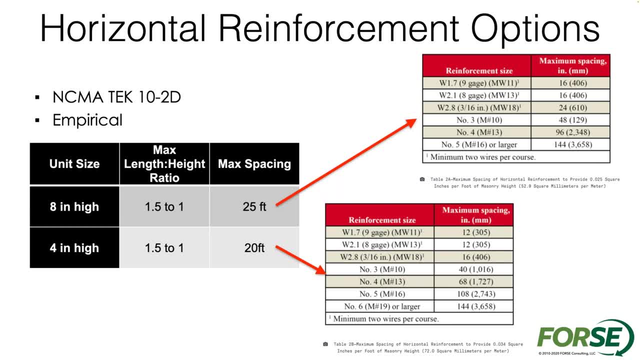 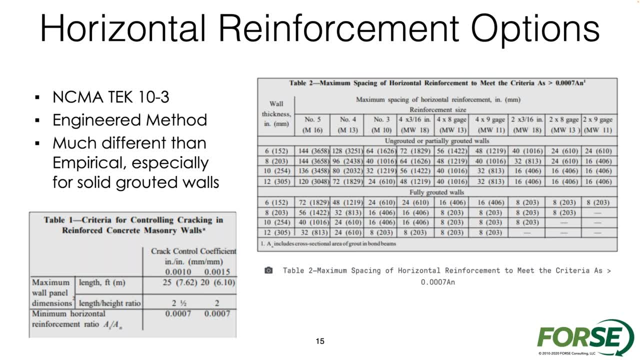 other than the thickness of the wall. You know, this is the just- I'm sorry, the height of the unit. That's really the only variable here. Getting into the NCMA tech guide 10-3, similar provisions, This is going to be: 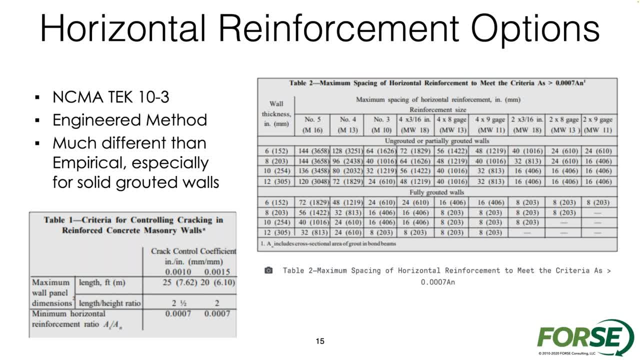 again looking at the requirements for horizontal reinforcement when we have control joints. So table one at the bottom is going to be showing us our maximum length of wall and length to height ratio. so 25 feet high of two and a half times length for the height ratio. 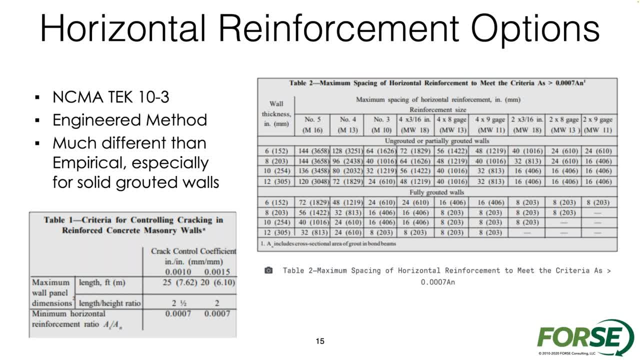 for a crack coefficient, a minimal horizontal point zero zero zero seven. so what is point zero zero seven? that's going to come to giving us uh for different wall thicknesses. so now what we're doing at the engineer method is we're looking at the actual area of concrete. you know, back here. 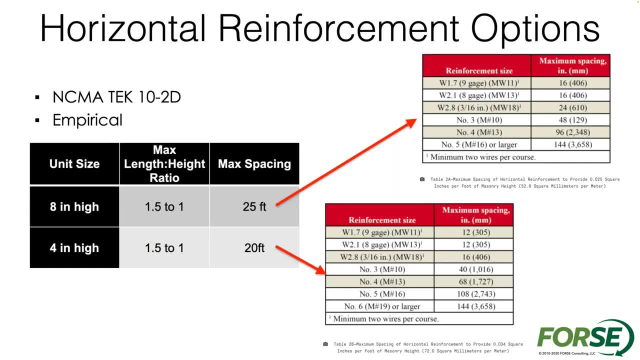 when we did the empirical method. that really wasn't. we're just looking at. empirical is really looking at what has worked in the past. what do we see success with? we don't necessarily have a lot of engineering number crunching to back this up, but this is what's worked well on the past here. 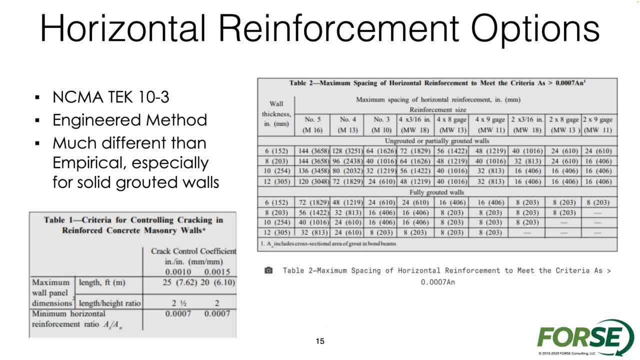 this is why, engineered method we're actually getting into, kind of the nuts and bolts of area of concrete that's, you know, shrinking, uh, you know, due to shrinkage in temperature. you know it's the actual. what is our demand going to be on our horizontal reinforcement? because 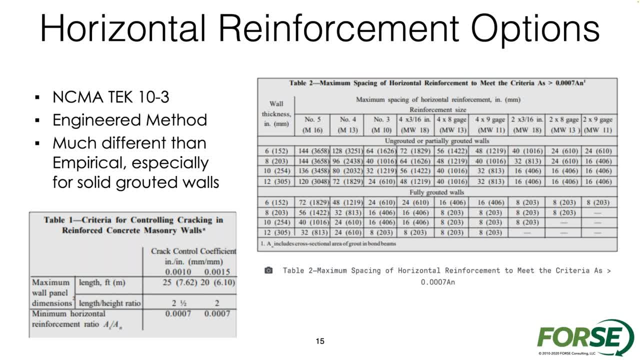 all kinds of concrete is going to crack. all concrete masonry is going to crack. really, the reinforcement that we're adding in here is going to be preventing those cracks from actually opening up where you'd have any water or any type of things that are going to be infiltrating in the design. so again, 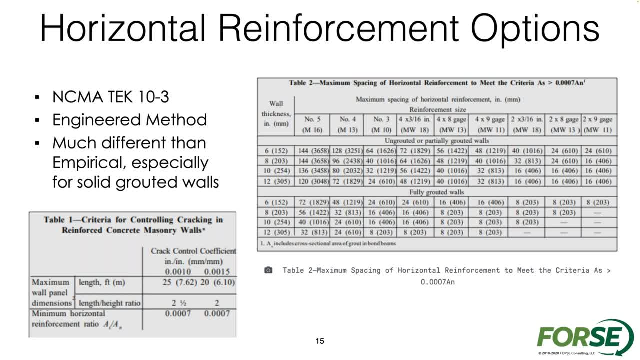 so now we have all kinds of different thick, because thicknesses have different wall thicknesses have different um face shells. that you have so a six inch, you have thinner face shells than a 12 inch. so even if it's a ungrouted or partially grouted, the continuous concrete is going to be a certain value. and then 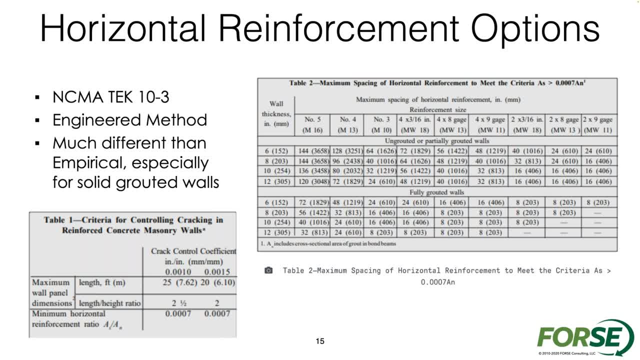 fully grouted, actually has not just the face shells, but obviously then it's a full concrete wall. what i think is really interesting here is when we have, um, the engineered method, we look at the actual designs, we can see that there's quite a bit of a difference between empirical and engineered method. 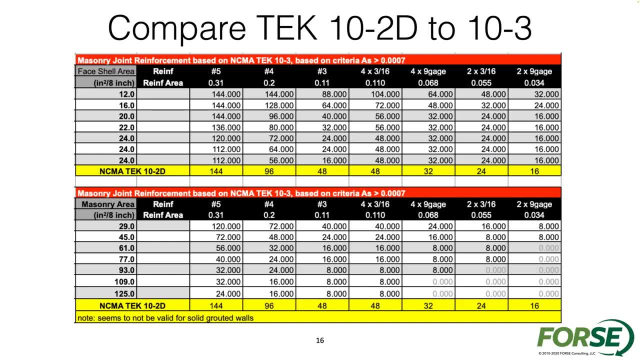 in fact what i thought was so interesting. i actually created a comparison. i did a table that looked at, uh, the joint reinforcement based on ncma tech, the engineered method, versus what i had from 10-2d. so if i have a partially grouted or ungrouted masonry wall, 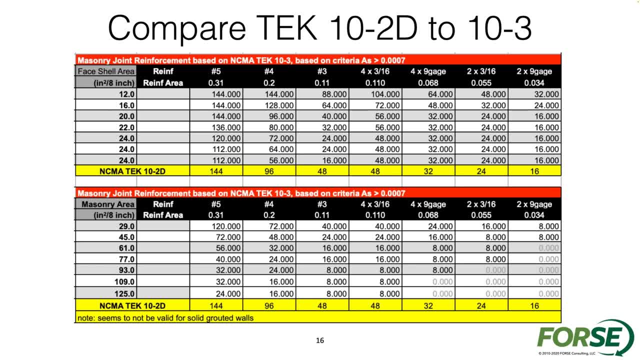 it's going to be the top table that i see at the top of the screen and you can see it compares pretty well. there's areas of the chart that are going to be unconservative. you know if i have, um, you know a design here. you know where i have a different thickness of walls. you know the, the thicker the walls, the. 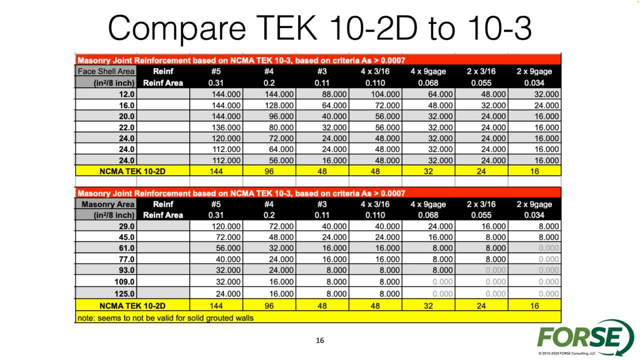 the the less conservative i am, but it compares pretty well. it does actually compare pretty well to the overall um what? what matches up here it's? when i get into the fully grouted walls i can see that i'm very, very unconservative. by using the empirical method, i have far too little, uh, joint reinforcement, uh, in here, design-wise, the. 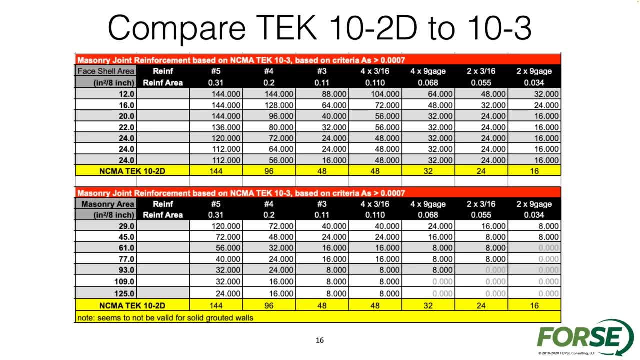 two, nine wires don't work for any wall grouted solid, whether it's a six to a 16, all of them are going to be very unconservative and certainly, as i get to, uh, some of the thicker walls, um, it's going to be worse and worse. 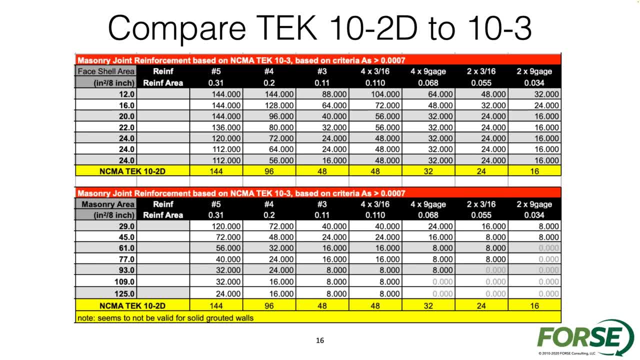 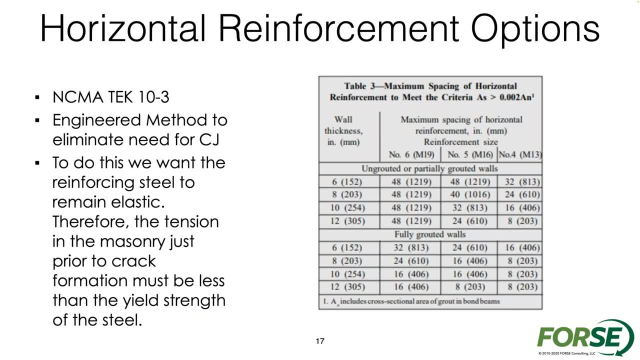 i have that much concrete so, like the bottom row, is this 16 inches concrete? so it that's um. that's something that's very important to remember. if we look at the tech guide 10-3, there's also a provision in there for moving beyond um moving. 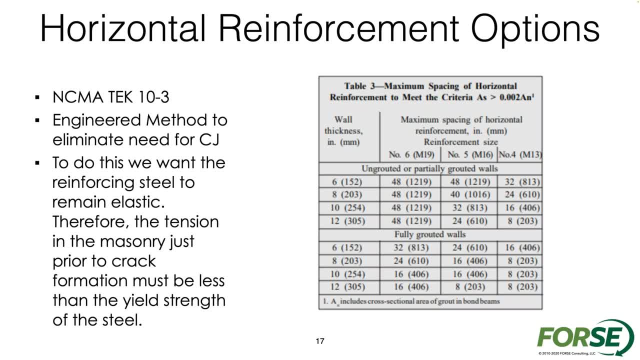 adding control joints. 10-3 also gives us an option for providing enough horizontal reinforcement so that i don't have to have any control joints that are prescribed within a wall. i can design a wall without control joints at specific locations and that's just a. it's a higher level of reinforcement. if you look at the chart, the reinforcement ratio that you see- 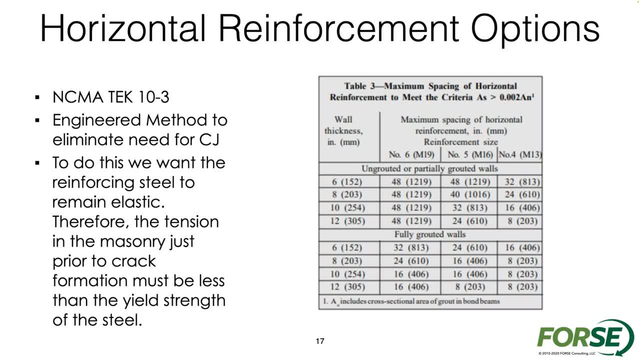 at the top uh in the top title it's point two percent uh of the overall net area of concrete is what's needed for the area of steel, 0.002. it should be very it should look very familiar to everyone because the essentially the same area that's. 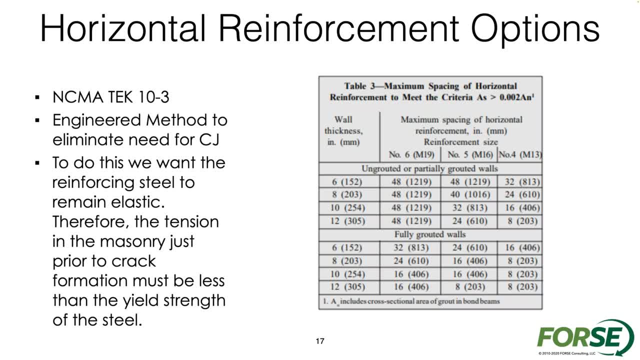 required for the horizontal reinforcement needed for concrete. so it's really we're not doing anything different. we're really kind of looking at making sure that we have enough reinforcement in there to prevent any shrinkage or temperature cracks from uh opening up, and so we have this. 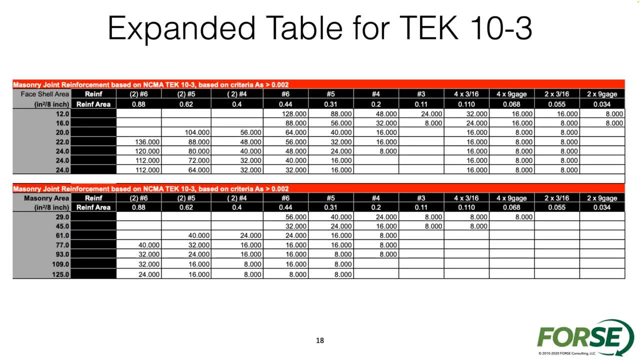 it's a quite- that's the really important thing to look at- to provide enough reinforcement. so again, if this is a floor, you can have it there and then you can add that on a concrete to kind of give a bit of a twist on this. the other thing that can help us determine what kind of 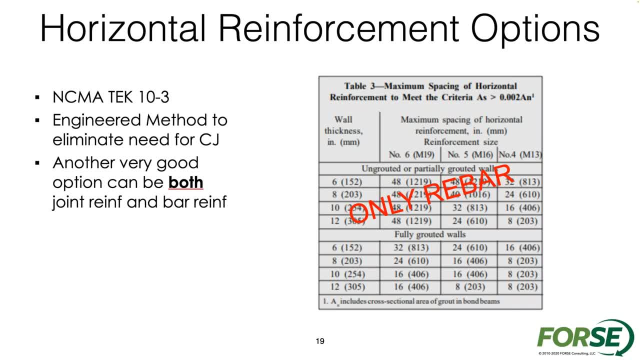 but I'm trying to see if I have a combination. So sometimes I have a design of a wall where I'm gonna put in some horizontal reinforcement, but I still gonna have joint reinforcement. Joint reinforcement might be in there for adding in joint reinforcement, for maybe it's a brick tie and stuff like that. 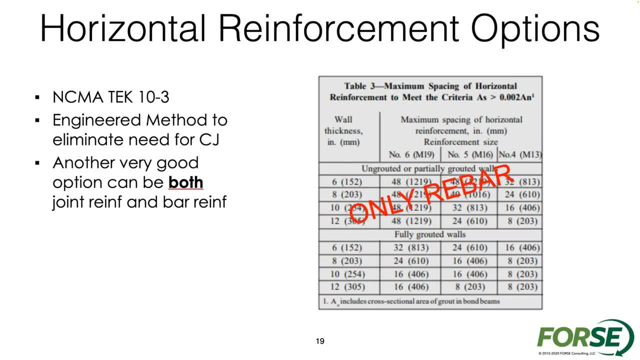 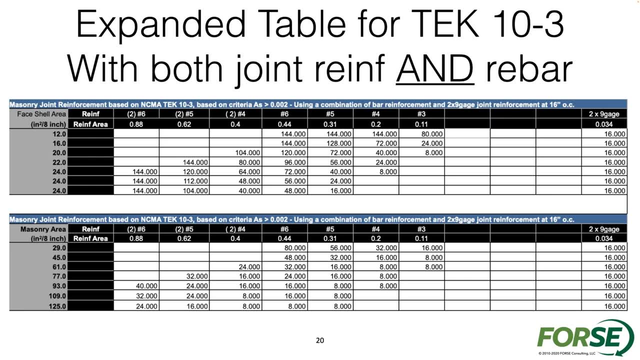 So I'm gonna have the joint reinforcement, I'm gonna add some bar reinforcement. So what I did was I created some tables here, for if I have both joint reinforcement and bar reinforcement, the actual bar reinforcement requirements are gonna be pretty minimal. So for a six inch wall, for example, 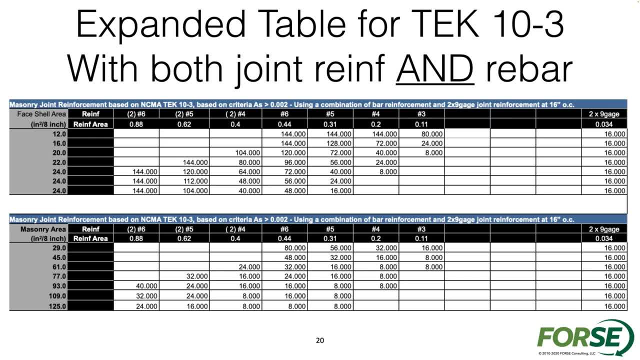 I could put a number four bar every 12 feet and joint reinforcement and not have to put in any control joints. That's a pretty straightforward design. You'll get into eight inch. maybe it's a number six: bar every 12 feet and joint reinforcement. 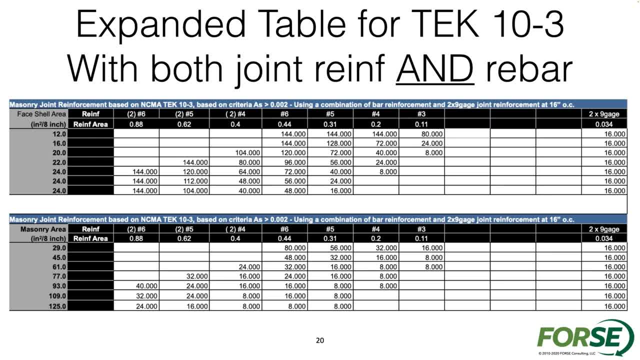 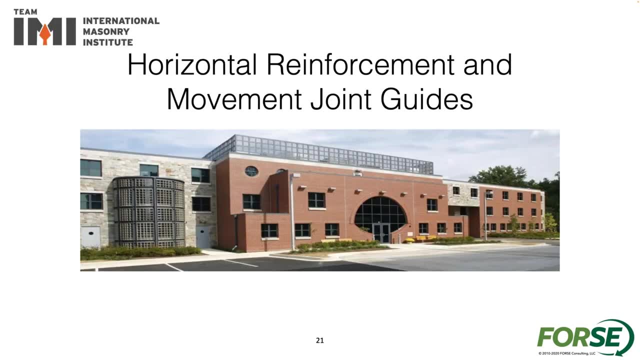 and I don't need to put in any control joints. So that's a pretty nice options for being able to look at the minimum amount of horizontal reinforcement that you would need to not have to put in control joints. So horizontal reinforcement movement joint guides. 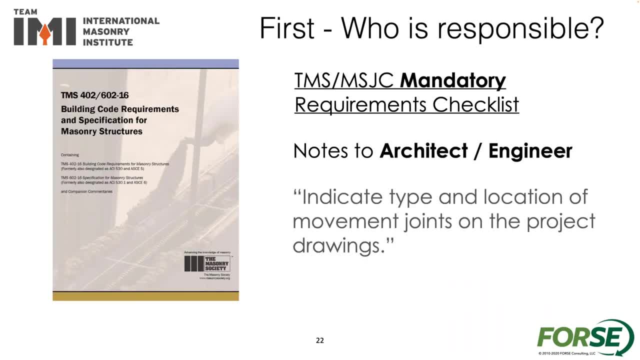 Again going back to the code. the code does require that, as designers, that we do locate them. We have to locate the type and location of movement joints on project drawings. Way too often I see this being delegated to contractors. We can't just list the requirements. 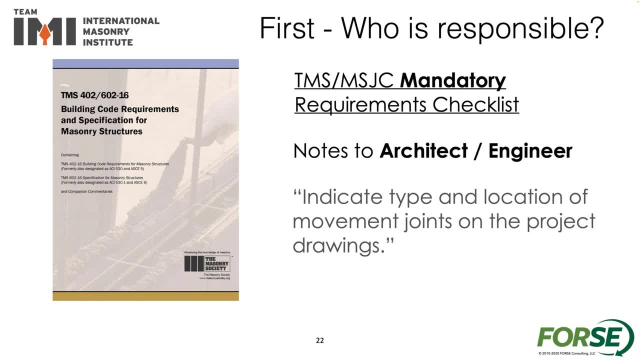 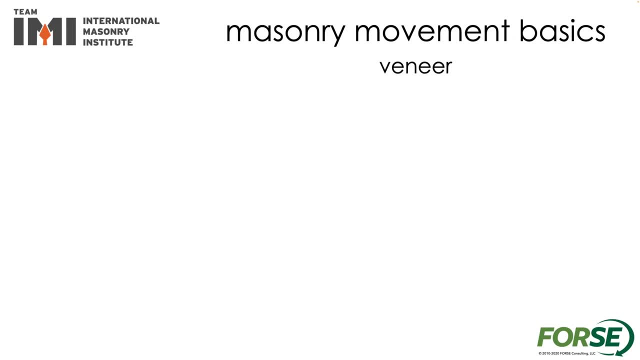 for where the joints go. We actually have to be specific to the type and location of movement joints on the drawings If I look at different types of joints for veneers, for movement joint basics. So a veneer unreinforced masonry is what we need to be thinking here. 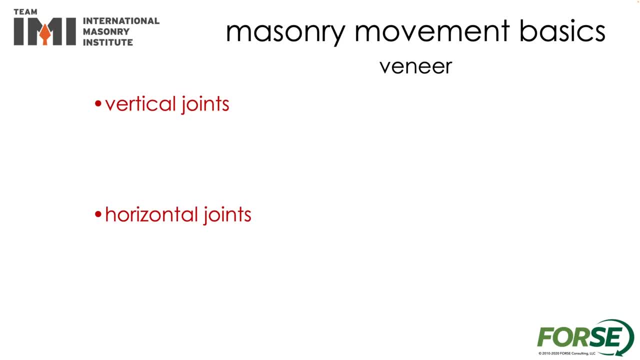 We have vertical joints that we add. We have horizontal joints that we add. What are some of the reasons that we add vertical joints? Needed to prevent cracking. We talked about that a little bit. We also need to add vertical joints when there's differential support. 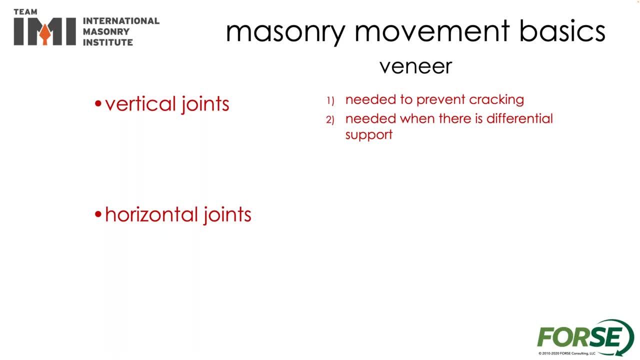 Anytime that we might have a wall that could be supported on different types of support systems. one might be a roof, one might be a foundation. There could be, it's just gonna be stresses that are gonna be created there. It's pretty rare that you would eliminate vertical joints. 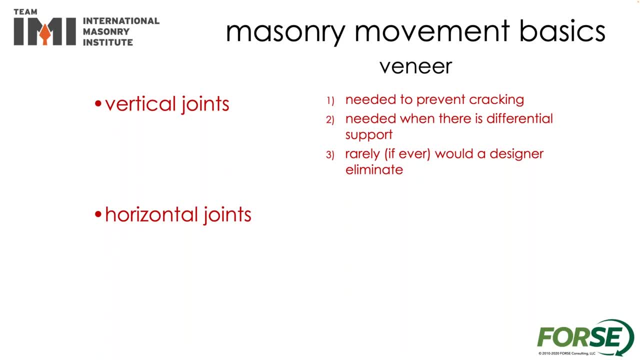 in a veneer. I mean, you'd have to add a fair amount of joint reinforcement in a veneer to eliminate those which maybe for certain projects would be desirable. But it'd be pretty rare to eliminate vertical joints For horizontal joints again. 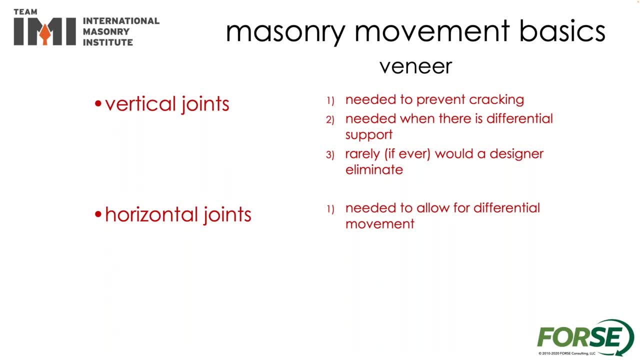 you need to allow for differential movement. This is a movement between the support structure and the veneer itself. We'll talk about that in a little bit. Horizontal joints is not to relieve. So anytime we look at masonry we look at like even or say, a brick veneer. 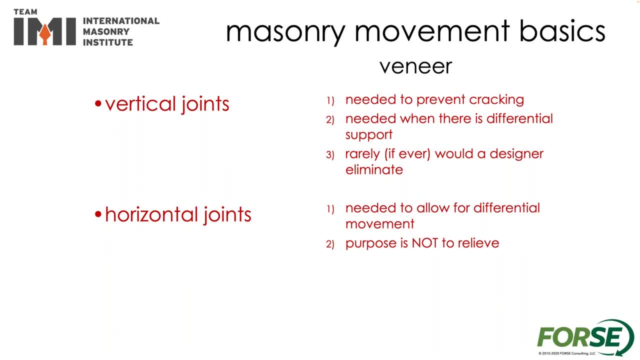 the capacity of brick is very, very high. We do not ever need to relieve the stresses that bricks are gonna accumulate. Masonry is gonna have plenty of capacity to support itself. Really, the horizontal joints is just trying to create some break between the veneer and the backup. 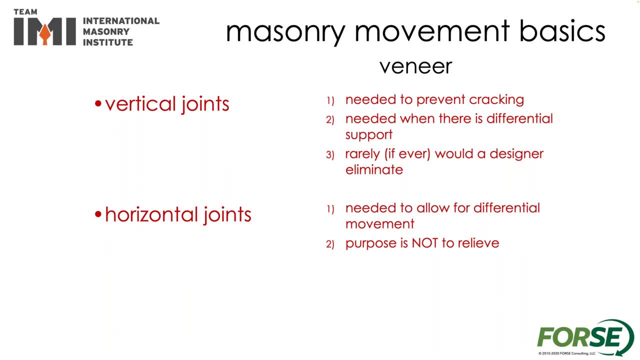 so that movement can be different between the two different spaces, And we'll talk about that in a little bit. There's some cases where you could eliminate the horizontal joints. In fact you could in quite a few cases, And we can talk about those as well. 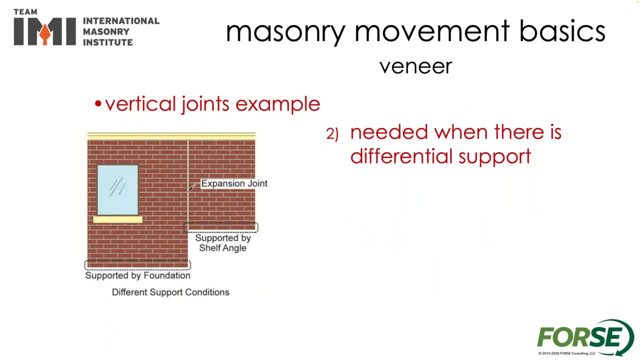 So again the vertical joint example, the differential support, again, if you have parts of your veneer that's supported on the foundation and then you have part of your veneer that might be on a shelf angle or on a lintel angle, 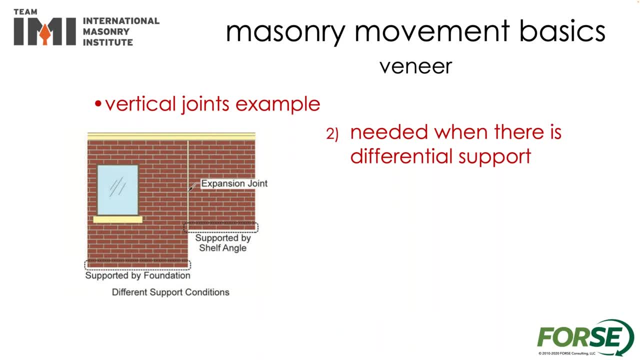 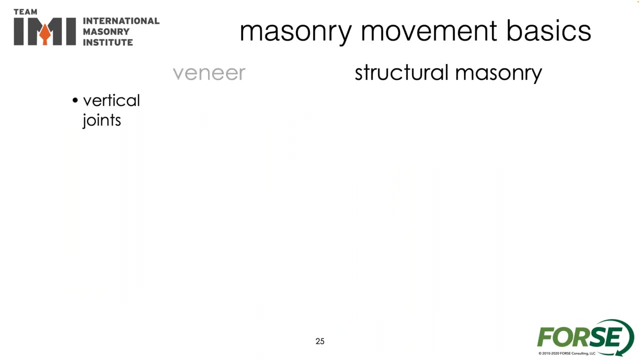 that those are gonna be locations where you have a differential support, The supported by a shelf angle. that angle can move a little bit, So that's why we do put those joints in those locations. That will be a common place for cracking. So that's differential support from the veneer perspective. 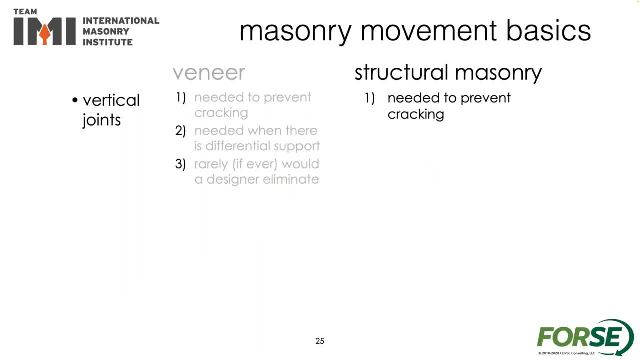 If I looked at a structural masonry. so veneer is gonna be unreinforced. Structural masonry is gonna be reinforced. Vertical joints: we still need to put those in to prevent cracking if we don't put an up horizontal reinforcement in. 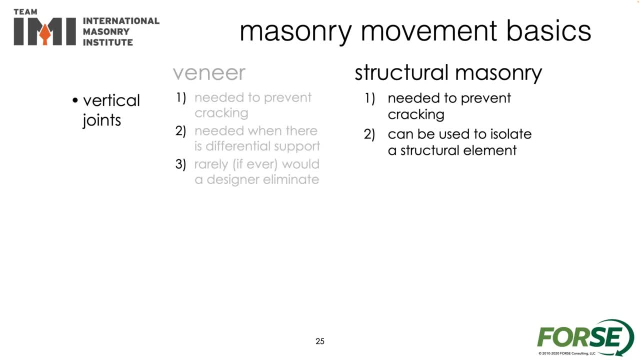 You can use vertical joints also to isolate structural elements, Structural design, where we maybe wanna have sheer walls just in a certain area And so we maybe wanna add in joints to isolate the sheer walls that are gonna have a lot of reinforcement versus other joints. 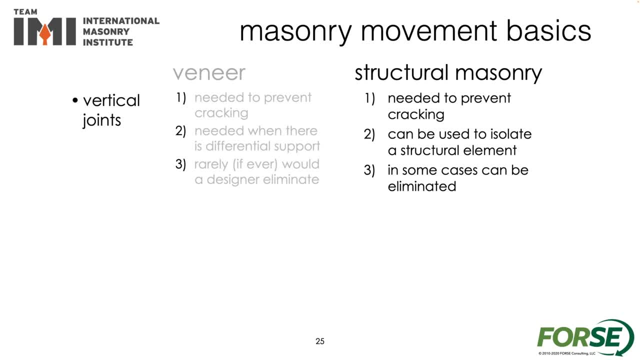 And then vertical joints we can eliminate in the structural masonry by having sufficient horizontal reinforcement, which isn't that hard to add. So horizontal joints in veneers. again we have those options. When do we put a horizontal joint in structural masonry? 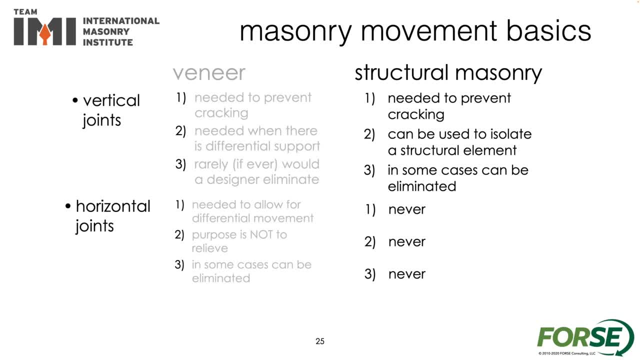 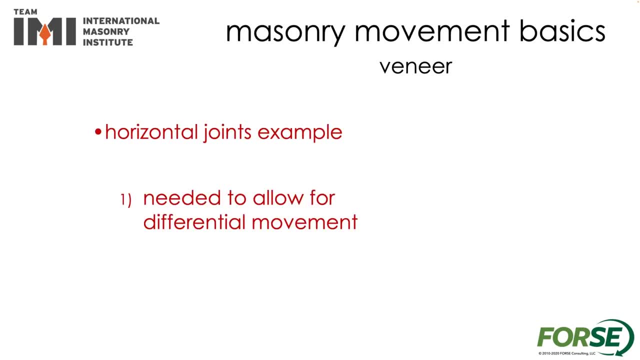 And the three times would be never, never and never. I mean there's just no time that we actually need to put in those horizontal joints in a structural masonry wall that's got plenty of capacity to support itself. So the horizontal joint needed for differential movement. 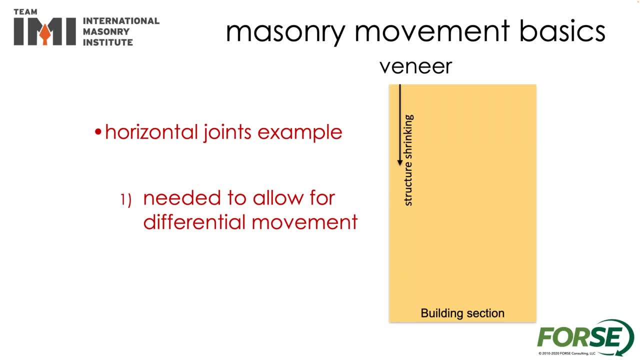 this really kind of comes to: the structure which is gonna be moving tends to be shrinking, especially if it's gonna be something that would be like a wood structure. it's definitely gonna be shrinking The things about the masonry and the veneers. it's gonna be very strong. 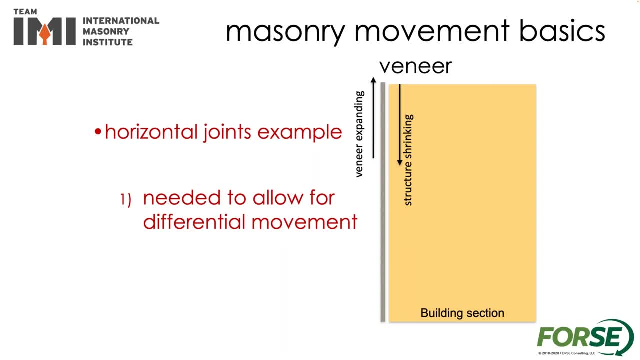 So that's probably gonna be expanding. So that differential movement. that's why our veneers need to be separated. quite often We have something going on with the structure behind that's moving quite a bit, whether laterally, vertically, so on and so forth. 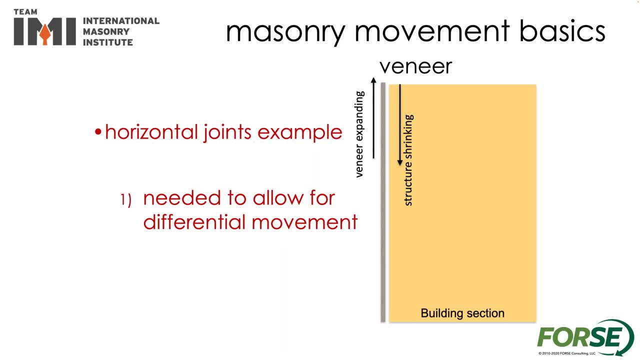 So the joints that are needed there horizontally, you really have to account for the different movement. If we have the multiple story structure, the reason why we typically add joints there is because we don't want that differential to accumulate over the height of the building. 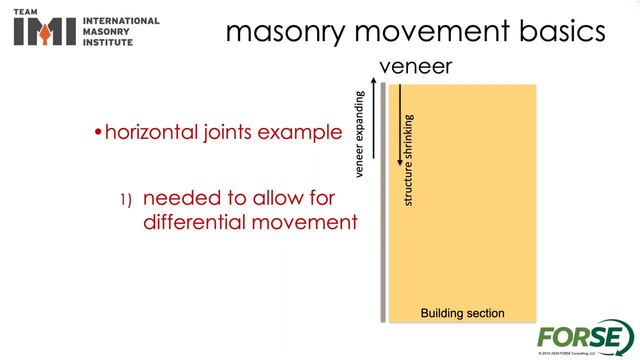 So that's why they're shelf angles and not relief angles. The shelf angle is just there to panelize the wall so that our differential movement isn't too high. It's not to relieve the brick beneath. So what are some of the structural elements? 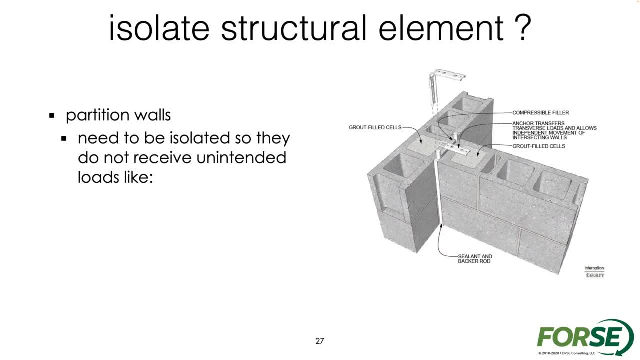 that you might wanna isolate. Partition walls could be an element that you wanna isolate So you put in a vertical joint to make sure that it doesn't get into gravity or lateral forces that you don't wanna have. It could be a shear wall. 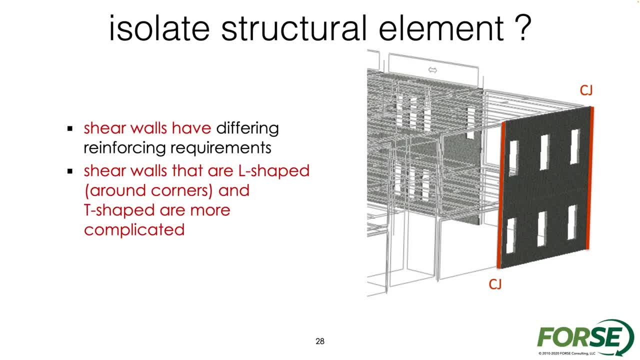 Maybe again that shear wall that you don't wanna have too many other forces stresses, or you want to simplify the behavior of the shear wall so that it stays in one plane. That might be a nice reason to put in some vertical joints. 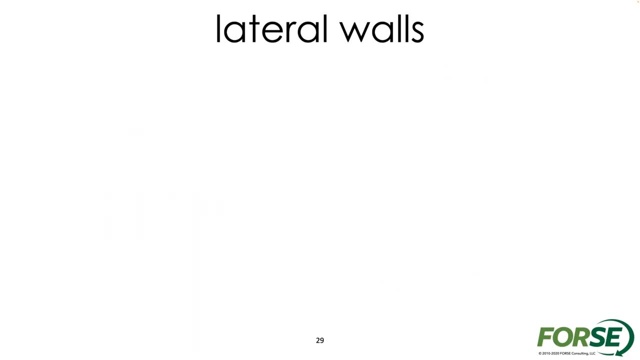 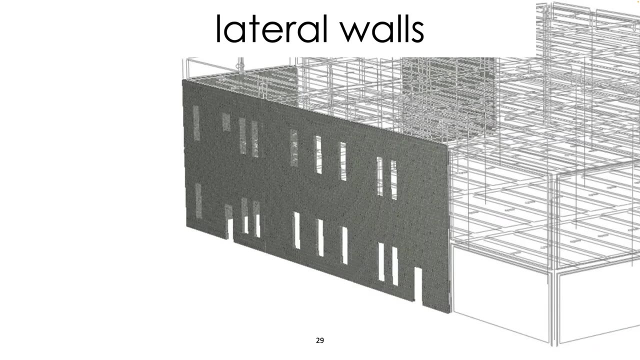 in a reinforced masonry wall. To talk a little bit more about lateral walls, one of the things that I look at for lateral design is looking at the elevation like this Typically. you know, in the past, without some better tools to design, 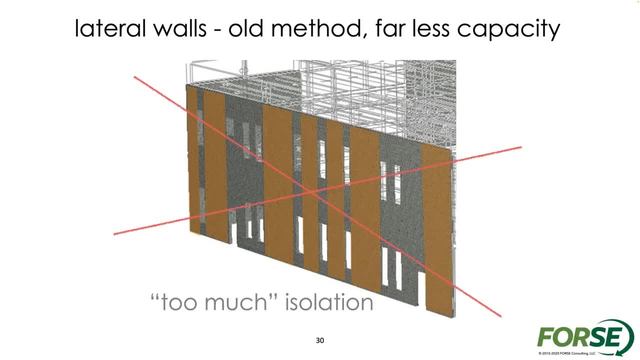 what I might have to do is I might have to look at individual areas between openings, because maybe that's where I put in joints, Maybe I put in joints at most, or many of the openings within a wall, And so what I ended up having was a lot of smaller. 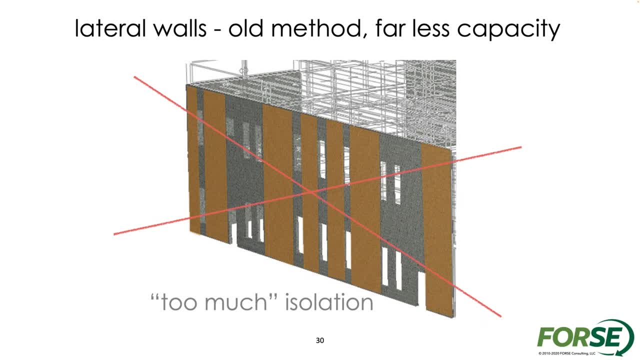 shorter shear walls, which are less effective design, And the reason for not making it include the opening is it just gets pretty complicated. It gets pretty complicated to design a perforated shear wall, a wall with an opening in the middle as a shear element. 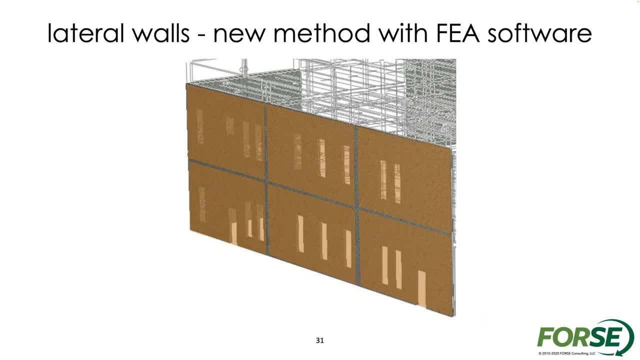 And so that's really you know we talk about software. A lot of my background is in software. Now, having a finite element analysis software to look at a masonry wall with openings that can be all over the place is really not that complicated. 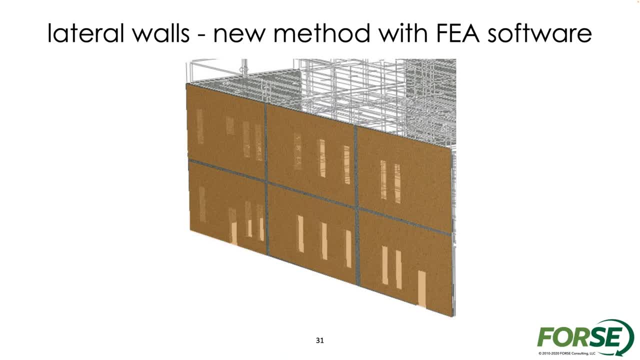 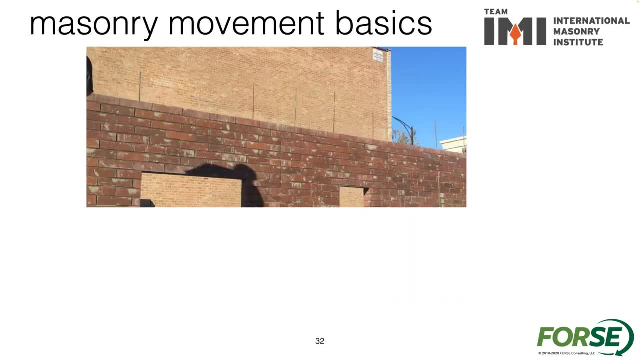 And then you have a system for actually looking at a wall. like this We can look at a lot longer wall, which again is gonna be a lot more effective. So again some, basically some masonry movement basics. all buildings move, concrete masonry shrinks. 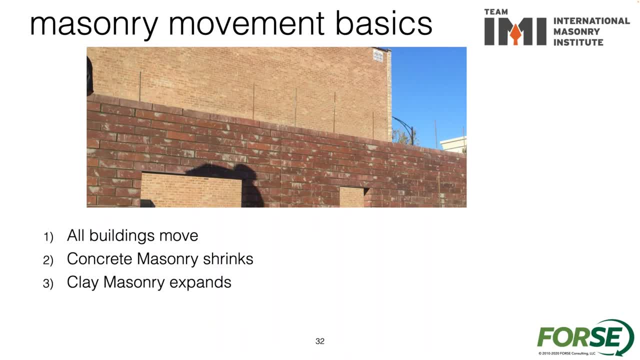 clay masonry expands- Two things that we have to think about If we have the two of them in the same wall. you know, if we have a cavity wall we definitely have to think about it, But just knowing that they move, you know. 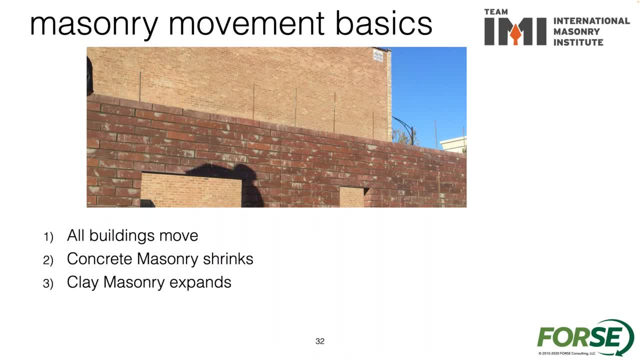 concrete tends to shrink over time. As it cures it tends to shrink. Clay is gonna expand over time as it takes on more moisture and the actual bricks grow a little bit. That's why you have the shrinking and expanding. I mean both of them, both shrink and expand. 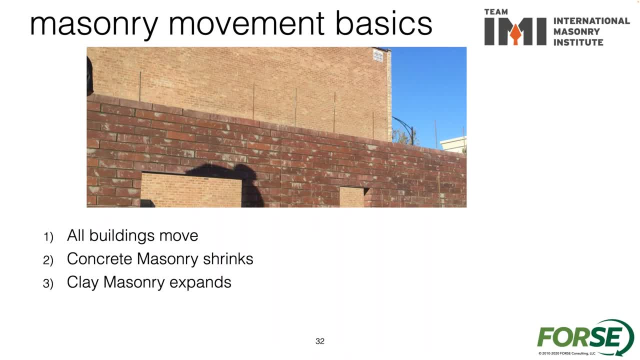 due to temperature loads, if that is variable. So the best thing to do with those is either accommodate some of the movement or restrain the movement. So we have to have some way to restrain the movement so that it doesn't Have negative effects in the overall building. 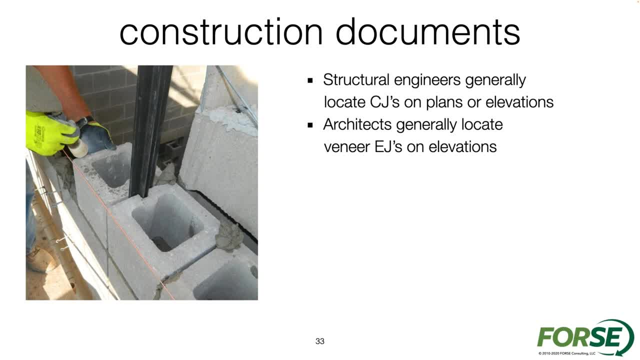 In terms of the actual construction documents, we typically have structural engineers locating control joints on plans, sometimes on elevations, and architects usually locate expansion joints on elevations. I would just say again: you cannot locate movement joints with a single sentence in the specification. 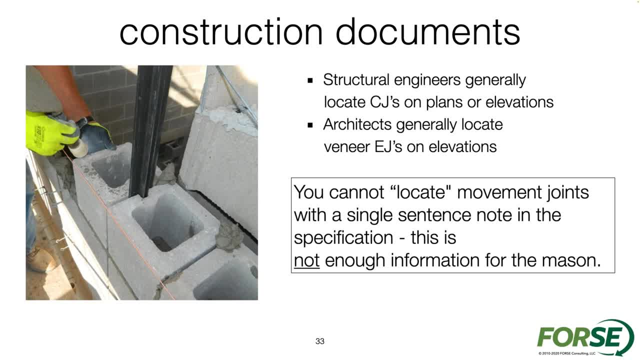 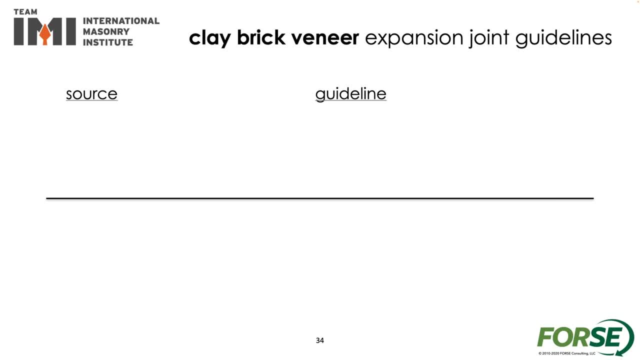 It's not enough information. We have to be specific, We have to make sure that we have those plans or elevations, that we're putting those joints on. In terms of some references, some guides that you might want to use for again: clay, brick, veneer- BIA is a good reference. 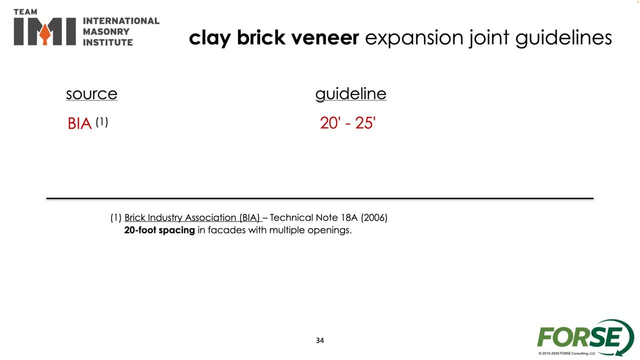 Brick Industry Association. They have a 20 foot spacing, that 20 to 25 feet that they allow for clay brick, and National Masonry Institute, IMI, has 18 to 25 feet. So somewhere in there 20 feet It's probably a good maximum length of wall. 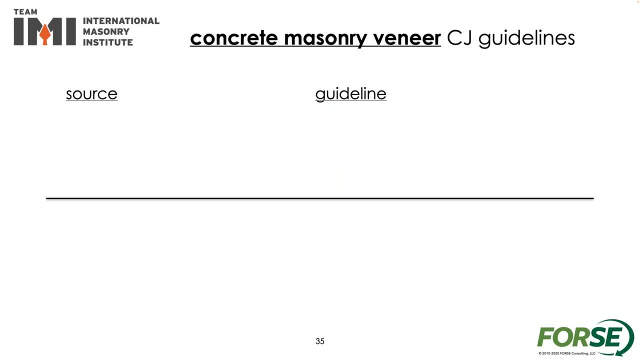 before you put a control joint, You have a concrete masonry veneer. Again, NCMA is going to say 1.5 times the wall height, not to exceed 20 feet. That's within NCMA tech 10-4.. If I have a concrete masonry design, 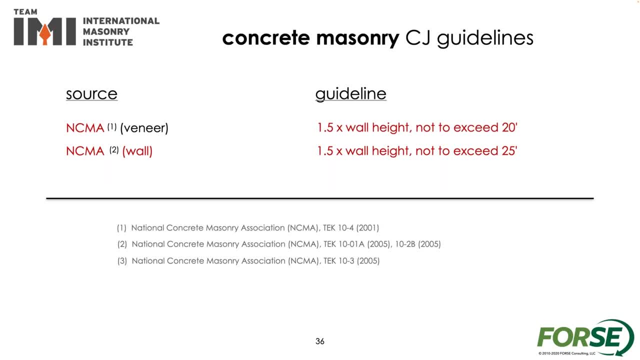 where it's a reinforced wall. then again I have similar 1.5 times the height, not to exceed 25 feet. That's one reference. But then I also have the reinforced wall options. where I can have no limitations, I have a movement joints that I can put. 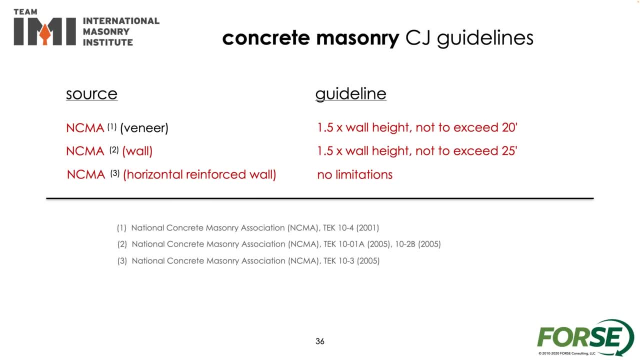 wherever would make sense for the overall design. I don't have to put them regularly. So you really have three different types of walls here. You have a veneer, you have a mostly vertically reinforced wall with the second option And then you have a vertical. 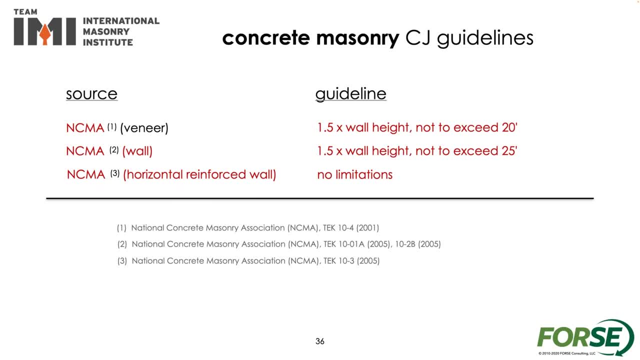 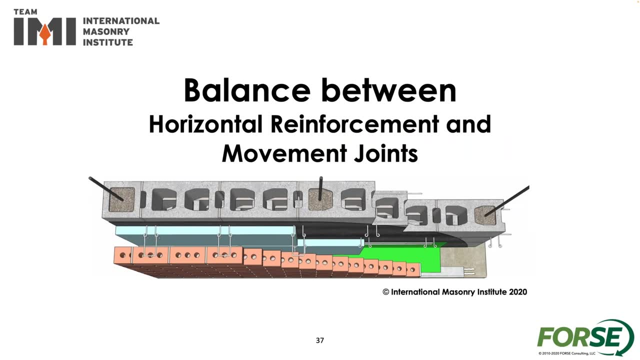 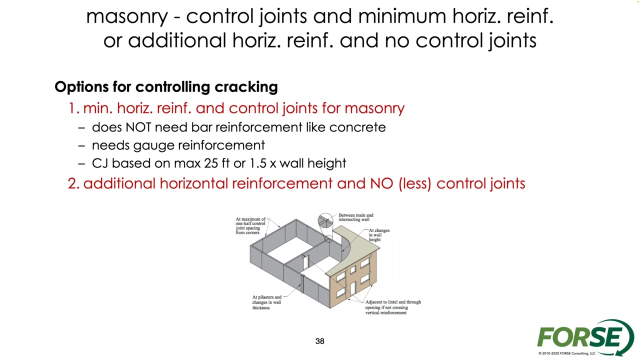 and horizontal reinforced wall, And that's it where our limitations are very minimal. so i would say there really should be somewhat of a balance between the horizontal reinforcement and movement joints. take into design consideration what different things that we have in. here again, our options are one or two, one minimum horizontal reinforcement and control joints. 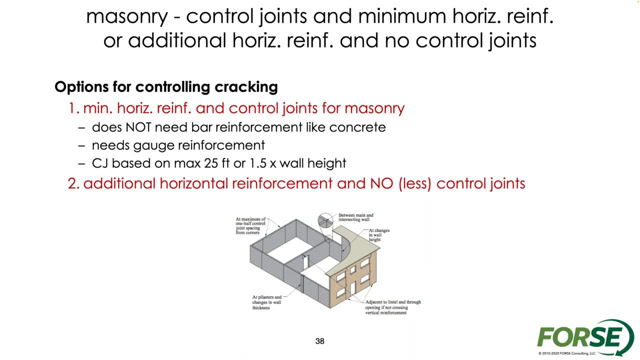 and then the control joints are the ones that we have in the control joints. you know, if we go with this option- just recognizing that you don't have to have as much horizontal reinforcement as concrete- that's why you can get away with just the light gauge reinforcement and that's why we put the control joints pretty regularly. 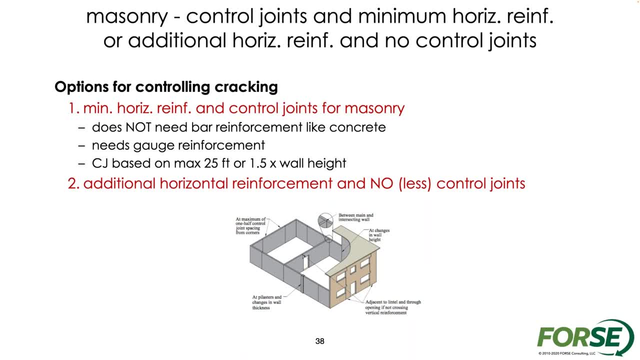 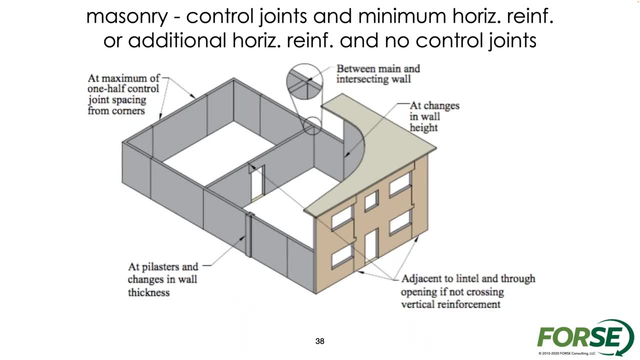 and then the second option, really getting into the additional reinforcement: being more like concrete and having no- which is practical terms less- joints. the ncma tech guide also gives some a nice little diagram here to kind of point to you know: anytime that you have a change of wall height, that's a good place for a control joint. 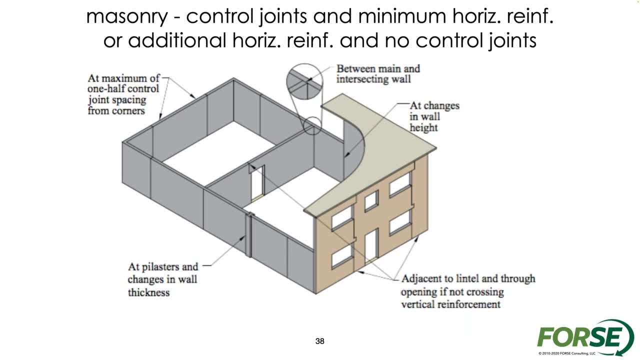 anytime that you have intersecting walls, that's a nice place for a control gym pilasters. uh, just because the change of the overall capacity or maybe change of load demand might be a good place for a control joint. and then you know, as you kind of go around corners, maybe there's a 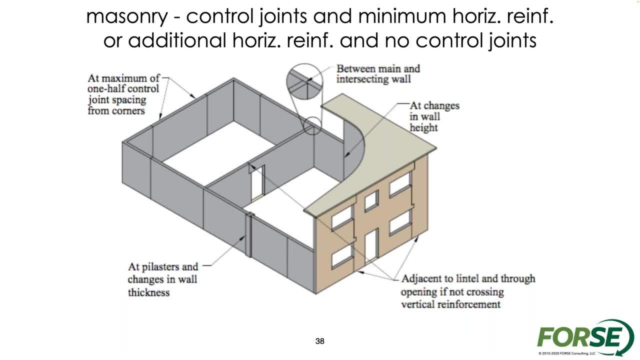 good place for a lead-in for a contract. there's another good places for control joints. if you look at the diagram a little bit closer, you can see maybe partition walls or exterior walls. you can see the different color right. it's a maybe shaded a little bit red to. 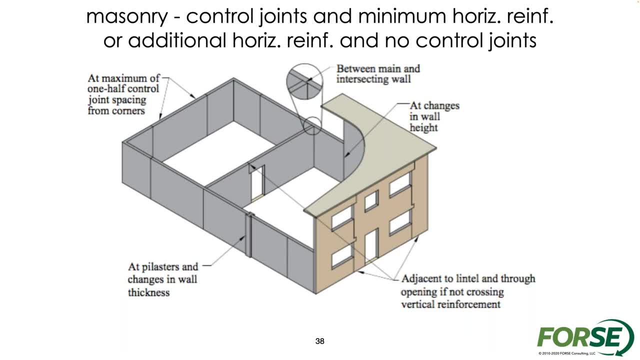 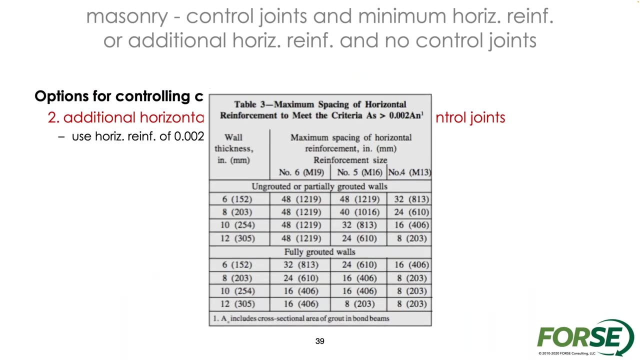 show a brick veneer, those kind of showing unreinforced options where you'd have next to lintels, where you would want to have some joints. so a nice little diagram pointing you to some common locations for joints within a building. then, like i said, we went to the table. 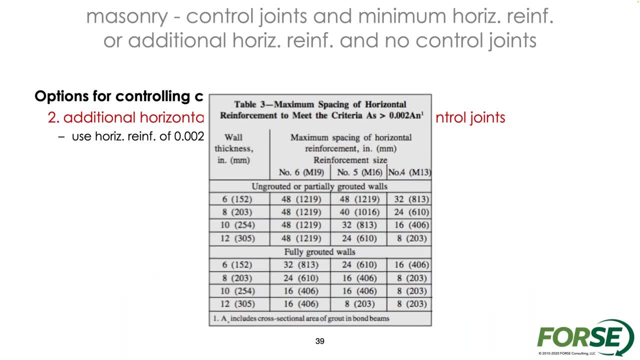 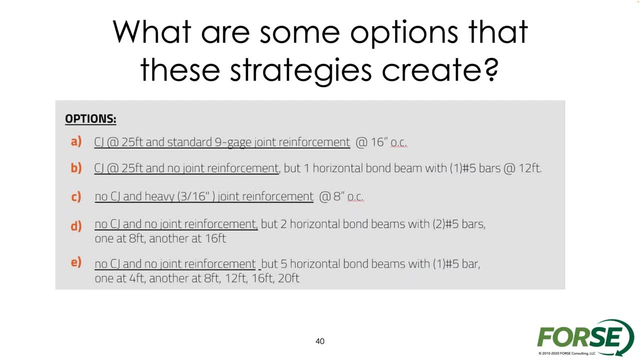 a little bit kind of looking at what are some of the different horizontal reinforcement options to have reinforcement. so again, we look at again different strategies. we have different options, we have different designs that might look at you know what, what would be the best for this option. so this is something where i- you know, i actually created this survey and reached out to several. 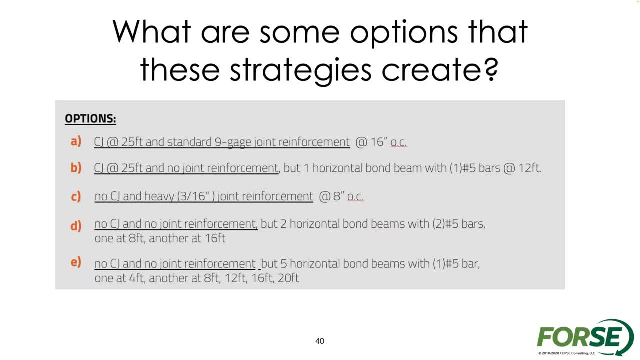 different contractors to look at. you know what their preference would be, what they would want to do, uh, design wise. so, looking at option a, where we have a standard joint, standard reinforcement. option b, where we have standard joints, no joint reinforcement but horizontal bond beams, not a bad. 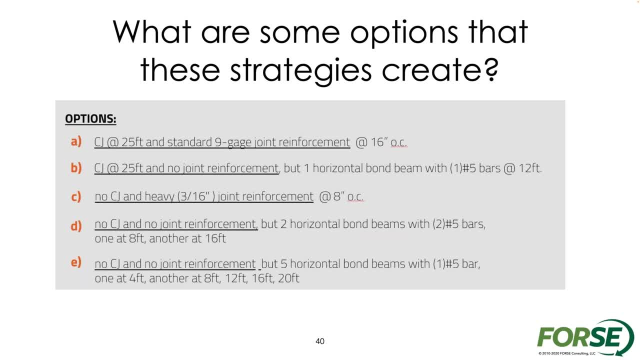 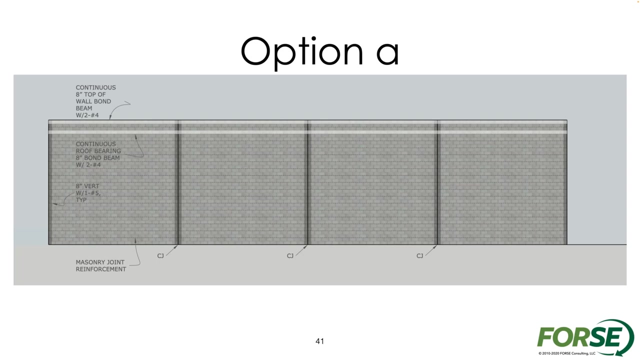 not a bad option. and then c, where we have no control joints, heavy joint reinforcement, that's another option. and then no control joints and no joint reinforcement, but two bars throughout a wall. and then no control joints, no joint reinforcement, but even more bars more regularly. so just kind of: what do those elevations look like? so this is again a pretty common 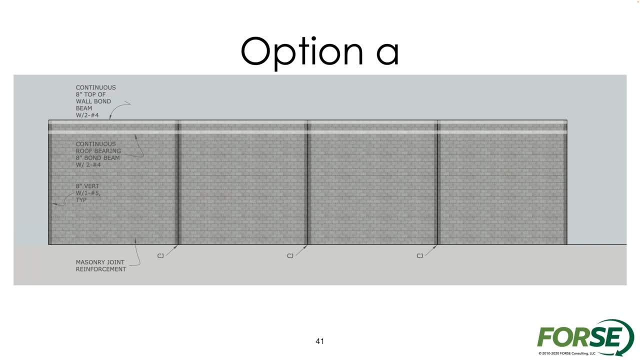 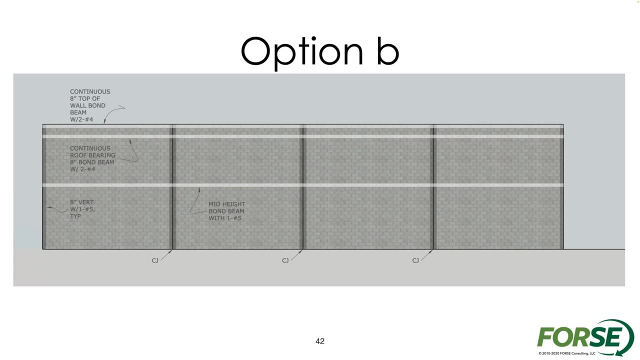 masonry wall with a lot of joints throughout the wall and joint reinforcement kind of everywhere. this just looking at the wall. obviously it's a lot cleaner. there's not all the horizontal wire that you have to add. you can put in these mid-height bond beams. that can be a really nice. 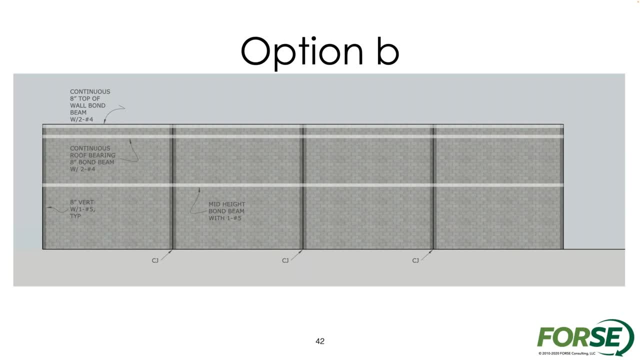 option preventing uh cracks. maybe this is a nice option. you know anytime that you have a cavity wall. if there's some minor cracks that would occur in in some of these bigger panels, then then maybe it's not that big of a deal if you get into. you start to get into some of the options that look. 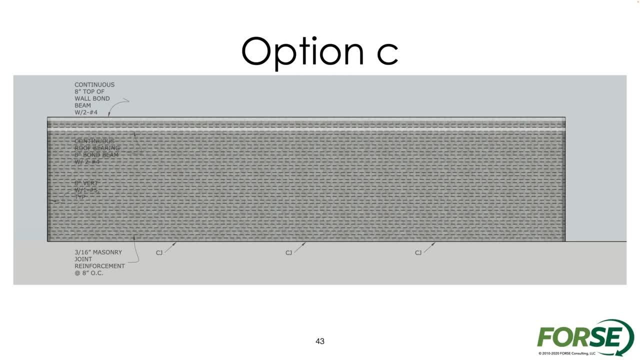 at eliminating the need for regular control joints. you know this option is one that contractors did not like at all. uh, it's putting this heavy joint reinforcement uh, every eight inches. yeah, you can eliminate control joints, but it's that heavier three 16 inch joint reinforcement is not one that. 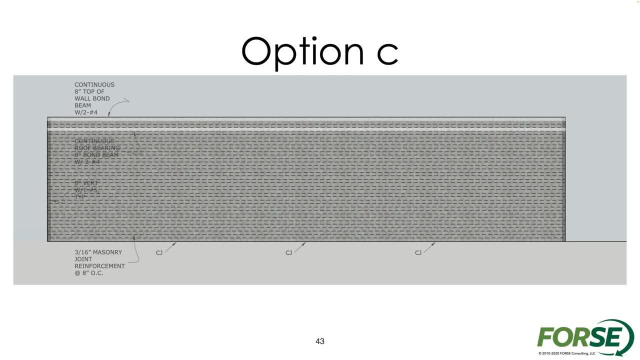 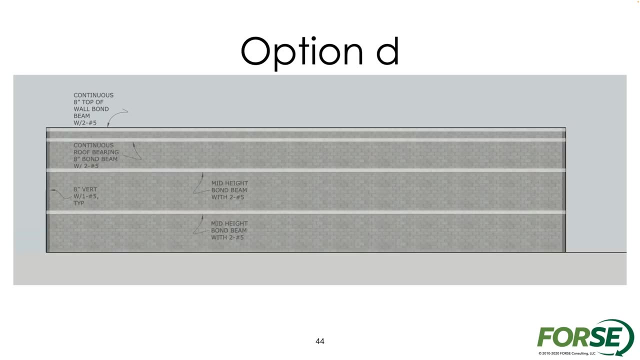 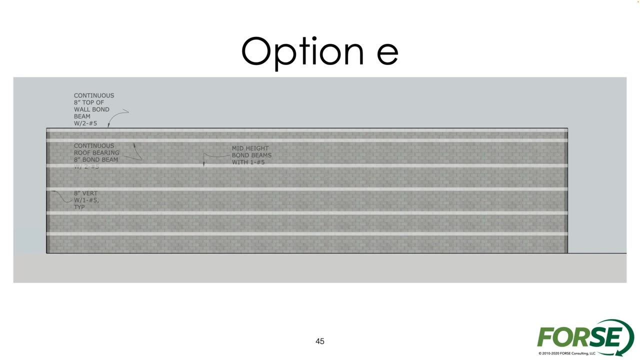 contractors enjoy using. so having to do that regularly throughout every level of the building or every level every course of the construction is not something that's desirable. option d: less bond beams, more reinforcement. or option e: more bond beams with one bar. so different options that you have that would satisfy some of those control joints. versus minimum reinforcement, i think it gets. 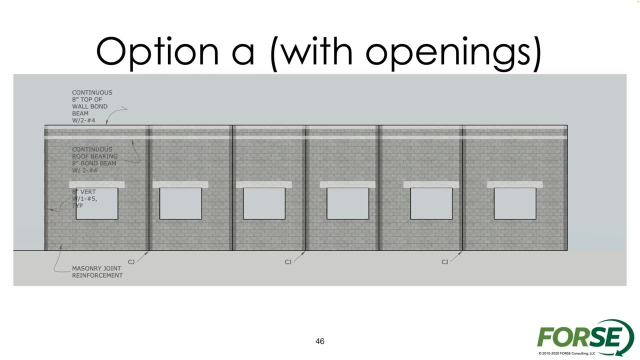 a little bit more interesting when we start to add in some openings, putting in openings, you know, just because of the location of the openings, reinforced- uh, you know, masonry walls don't want to have control joints at the openings, it's unreinforced ones that do. so. now we're maybe even adding in some control joints because of the openings. 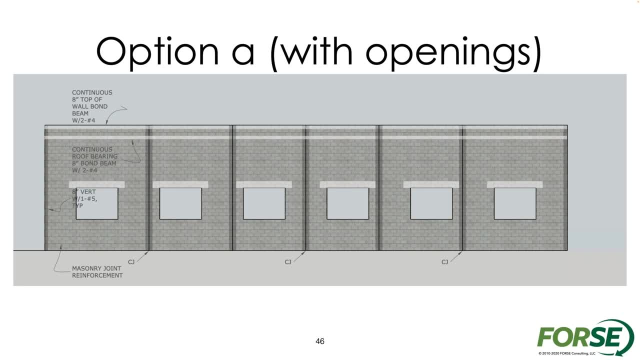 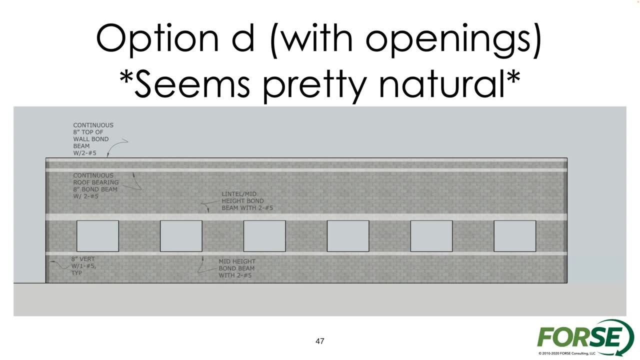 we have joint reinforcement. we have lintels. you know it might be simpler to put in: uh, just have the lintel reinforcement be continuous, have the sill reinforcement be continuous, and maybe that seems better than just adding them in. we're seeingoring the lintel reinforcement that you. 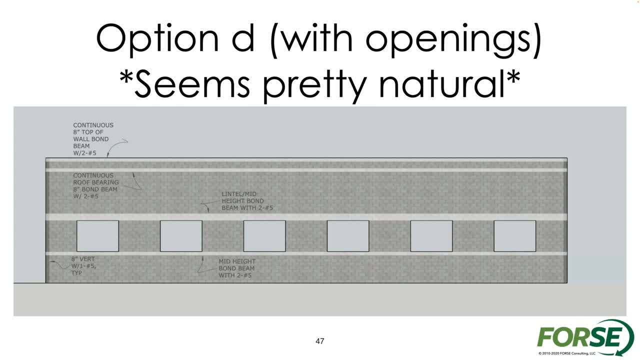 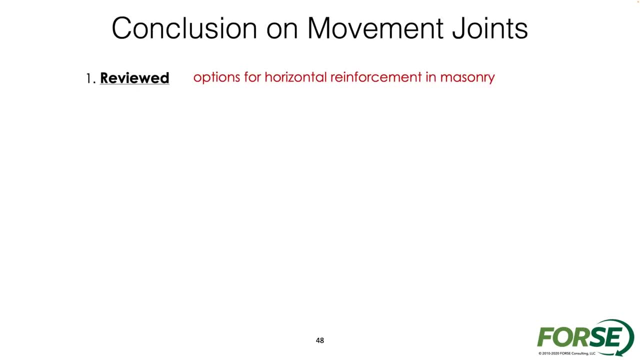 might see coming for most blockARR packs. so we're seeing, were we discussed, that there's some significant like a very nice little option for our control joints and movement joints. so for the movement joints, we looked at horizontal reinforcement in the masonry walls. movement joints, purpose and location requirements. we looked at different reinforcement and movement. 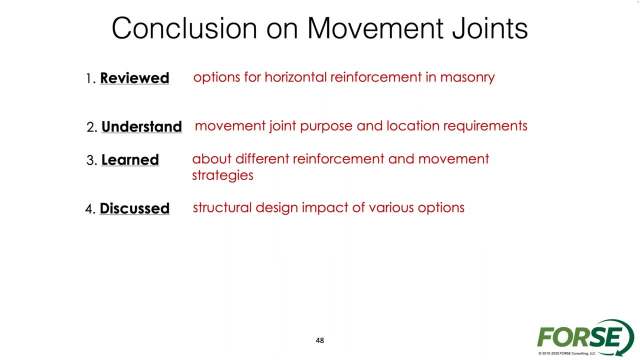 joint strategies and then some of the structural design impacts the resources. there are a lot of different resources that i referenced here. a lot of them are going to be ncma tech guides. there's a bia and obviously the, the masonry code, is also utilized here as well. 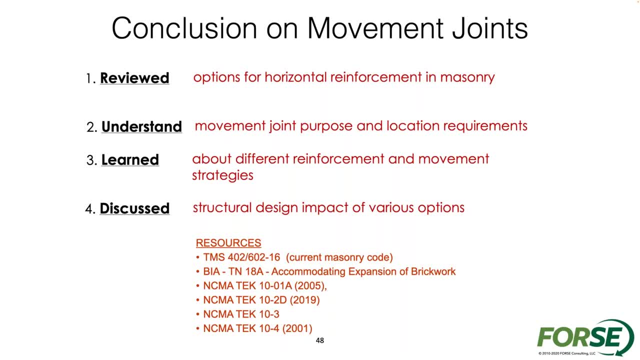 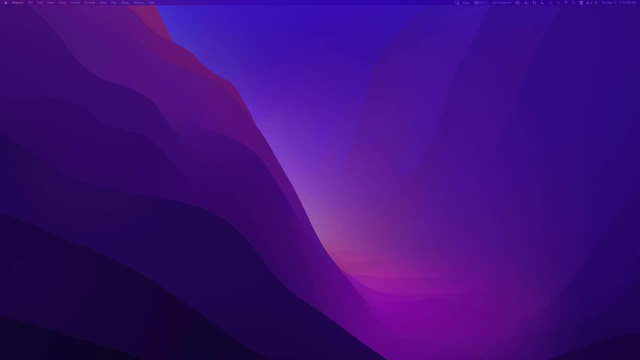 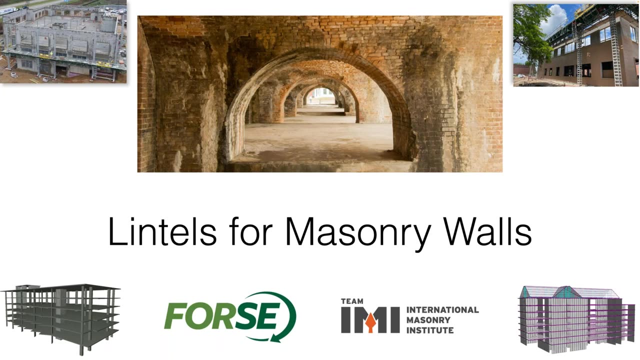 all right, so that's going to take us to the next section, where we're going to look at lentils for masonry walls. all right, gregory, it looks like you were looking for some designing questions about the masonry walls, so we're going to take a look at some of the masonry. 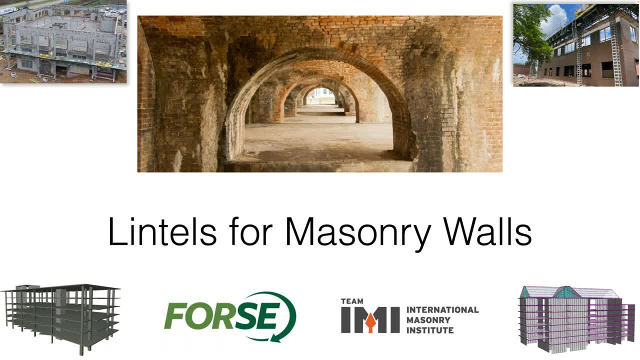 walls, and then we're going to take a look at some of the masonry walls and then we're going to take a look at some of the masonry blocks below masonryoft, of an of the masonry blocks below the wall, we're going to play bernard. 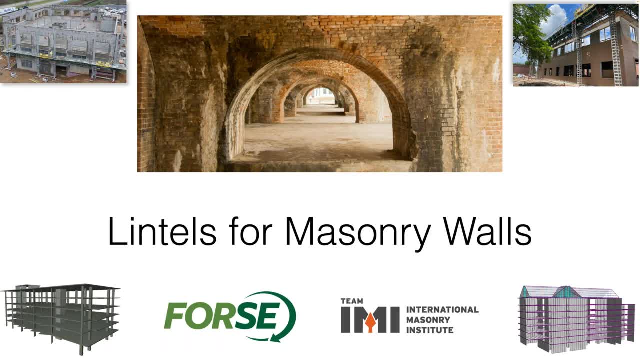 sorry that's not a double click: linos każos stories of masonry et cetera that you could possibly think of doing for masonry design. so again, that's the masonry designer's guide that's available from the masonry society. okay, lintels for masonry walls. this section is maybe a little bit longer. 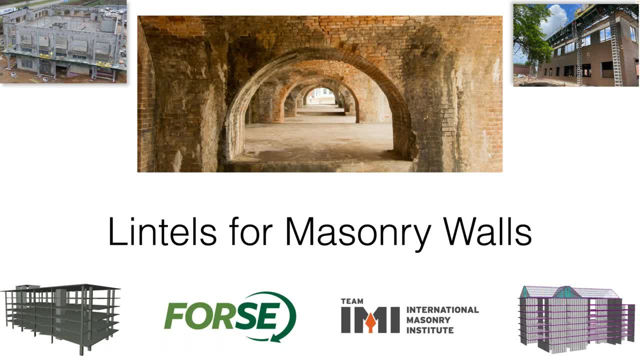 so we're going to try to get through the whole section before we take lunch. uh, lintel for masonry walls. i think the uh things that we're looking at here is maybe a kind of a proposed change to what the typical uh, you know, the way that we've typically did. 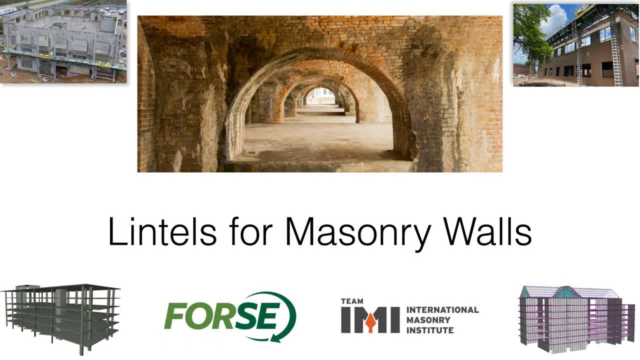 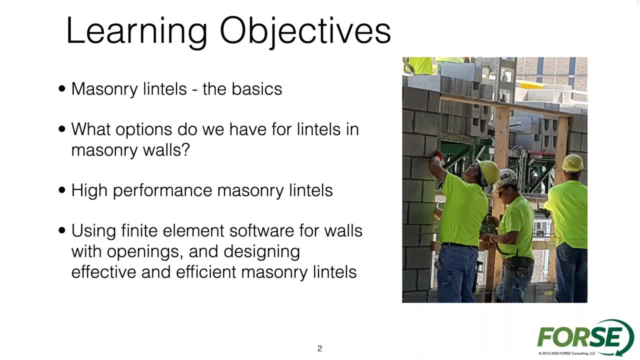 uh, lintels for masonry walls. so that's why we're going to spend a little bit more time, um, on masonry lintels. today we're going to look at the basics for lintels. what options do we have for lintels and masonry walls- what i'll call high performing masonry lintels- and then how to use. 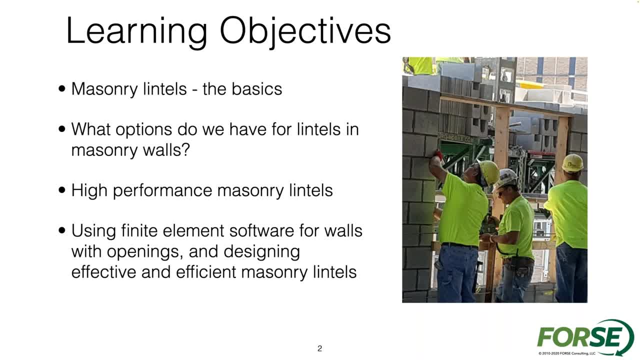 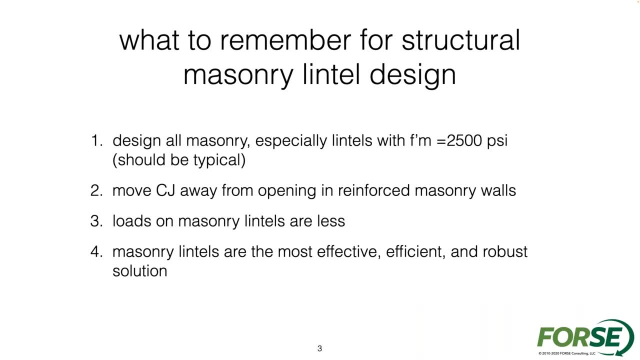 software for the lintel design. you know, i think there's definitely things that we want to remember, maybe things that we've talked about a little bit already. uh, designing all masonry, special lintels for that higher strength, a premium of 2500, moving control joints away from openings. uh, for a reinforced 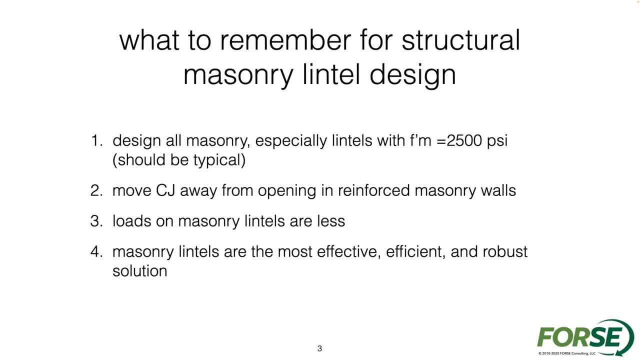 masonry wall is very, very important and we'll see why. uh, here within the lintel section, um, those on masonry lintels are a lot less. we'll talk about why that is versus some of the other materials that we're going to be using for the lintel design. 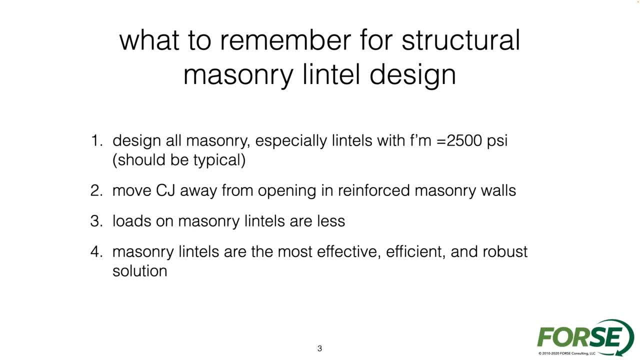 that you could have. and then masonry lintels are going to be the most effective, efficient and robust, and we'll kind of talk about why and how and kind of why that's important. so really, lintel is just going to be the area above an opening right. 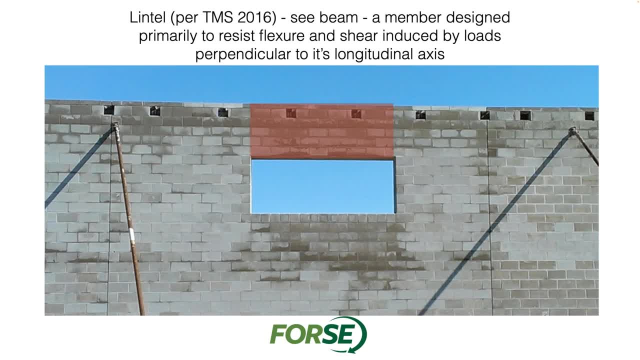 for tms 2016, c beam a member designed primarily to resist flexure and shear induced by lows perpendicular to its longitudinal axis. so it could be um, could be a vertical load, could be horizontal load, either. one of those could be uh options that we can look at there, and you know when i look at. 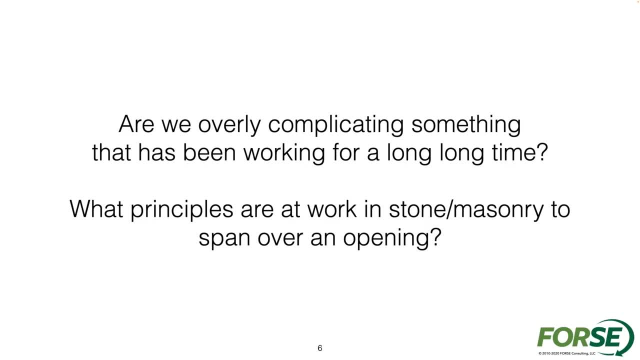 something like this. you know, sometimes i want to step back a little bit and say: you know, are we over complicating something? i mean, we have this concrete masonry wall. um, you know, have we been over complicating it? have we making this more than we need to? you know, what are the principles that work in stone and masonry? 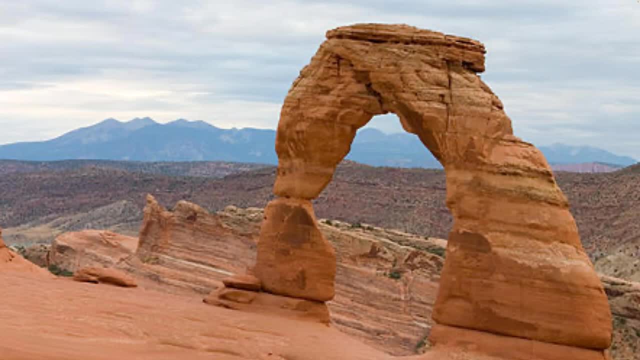 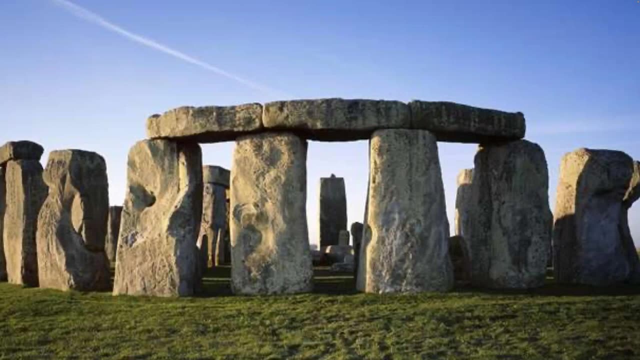 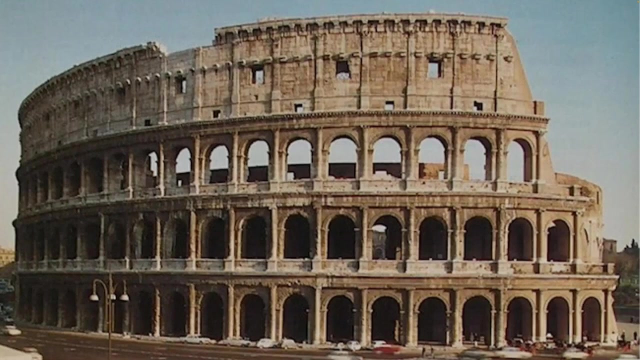 to spanning an opening. and so i just i mean i look at some of the pictures and images of stone and masonry that have spanned openings. i mean you can see that we don't need to add reinforcement, we don't need to add steel, we don't need to add a different material. we look at some of these. 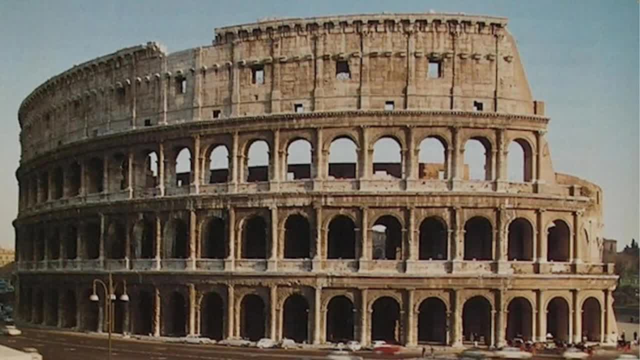 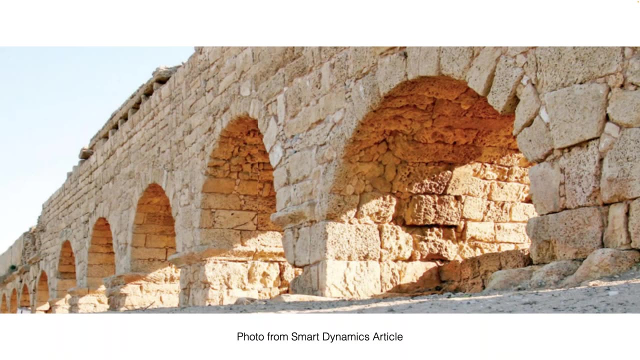 historical structures and buildings. we have the principles in place of these również buildings. these materials that are compression-based materials for spanning openings can be pretty large openings. We can span those openings pretty easily by just recognizing the compression-friendly materials that we're dealing with right. There's not a lot of tensile steel that needs to be added. 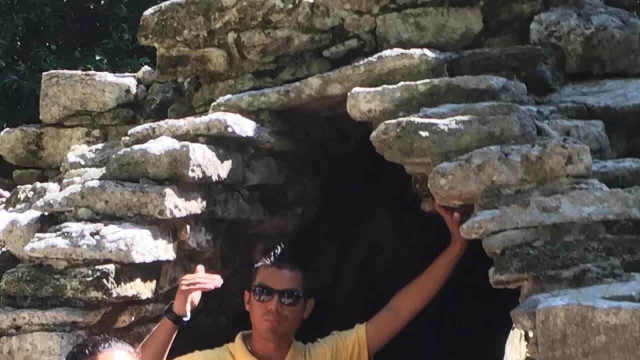 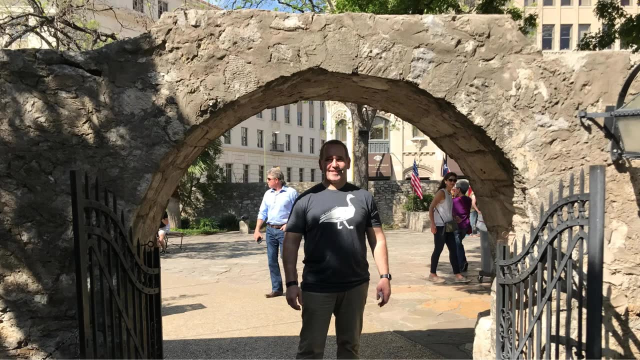 to these openings And so I think that's really good to recognize. I mean, these are just different archways that we've seen. that I've seen- This is me way back in the day down at the Alamo- Just you can see compression arches all over the place, And so when I look at doing a masonry- 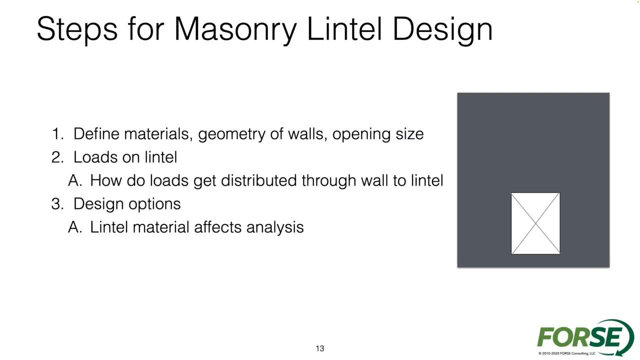 design. lintel design. there's several different things that I want to look at: Definition of materials, geometry of the openings, opening sizes, lintel, loads on the lintel. How do the loads actually get to a lintel? How does it get distributed through the wall? What are some? 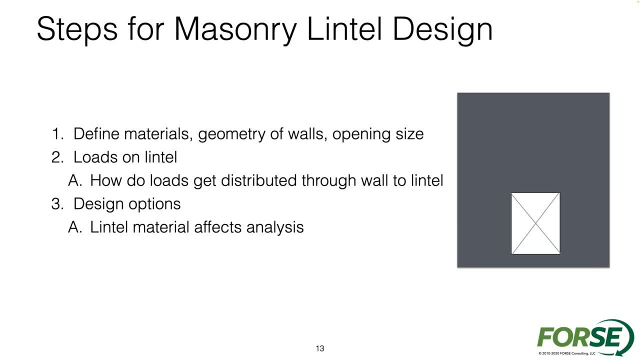 of the different options that I have to look at there, And then design options. the different lintel material affects the analysis because it has different demands on you know. back to number one: geometry of the walls, opening size, so on and so forth. 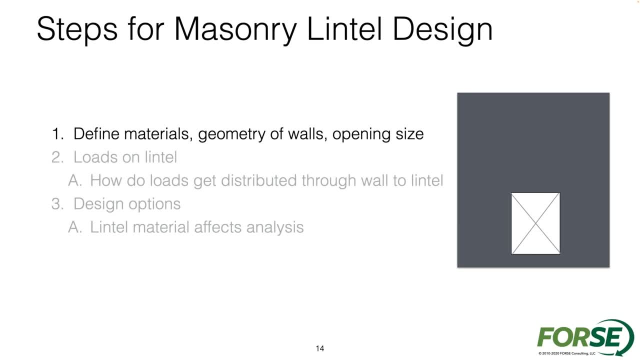 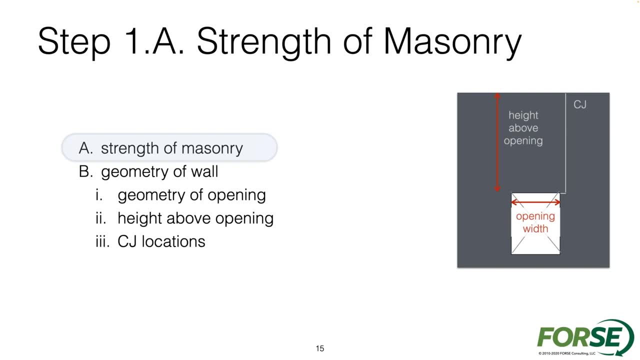 So let's go ahead and look at defined materials, geometry of walls, you know. strength of masonry Again, if we look at the area that you have, that we're dealing with, the strength of masonry is going to be, you know, looking at that, right above the opening. 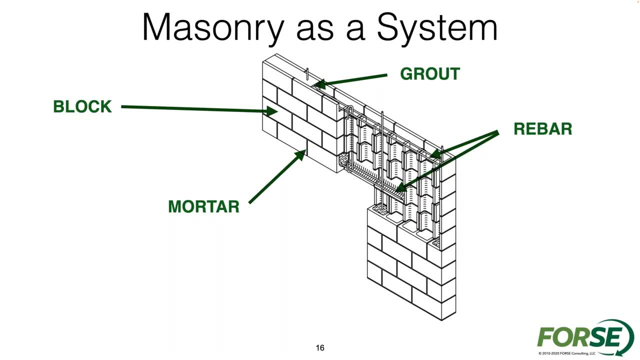 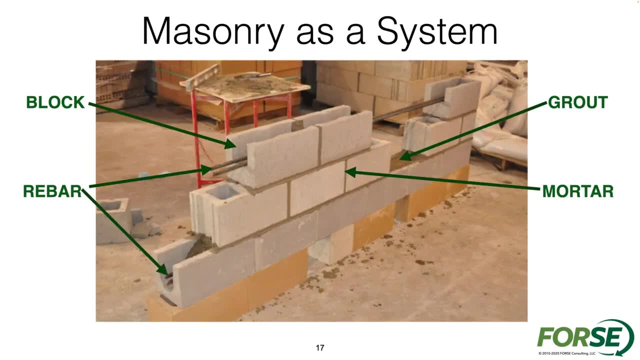 It's going to have, you know, the same block mortar, grout rebar that we've talked about in previous sections A lot of times. if I looked at masonry lintel, it's going to have the same materials, just utilized in a little bit of a different way. Obviously, you're going to have 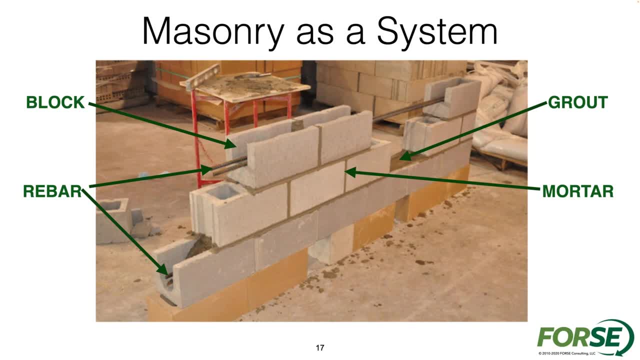 horizontal reinforcement, not just vertical reinforcement in this lintel, So it's going to be common materials. We have a little bit different blocks that we want to look at. We can have all kinds of different blocks that are used throughout the lintel, though We have the 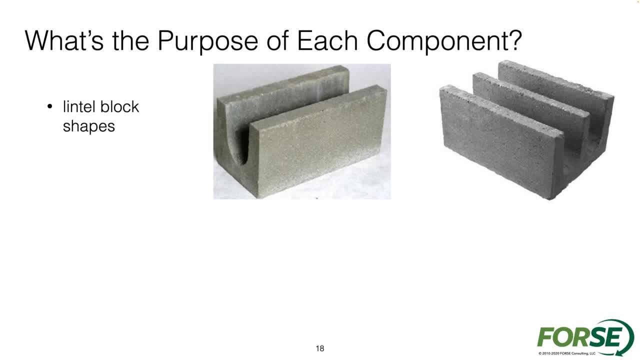 lintel-shaped blocks, which are going to be the standard kind of UW-shaped blocks that are going to be used because it's got a solid, flat bottom right And that's going to be important for lintels because when we span an opening, especially if it's architecturally exposed, 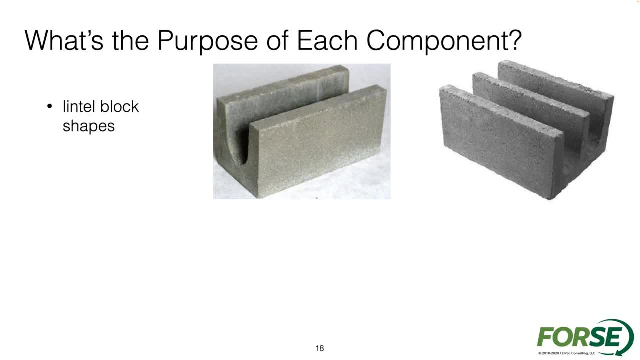 obviously you don't want to see anything there but a solid masonry bottom. So it also contains the grout. It works good construction-wise. Other lintel blocks are going to be just your standard stretcher blocks. You know, if you have several. 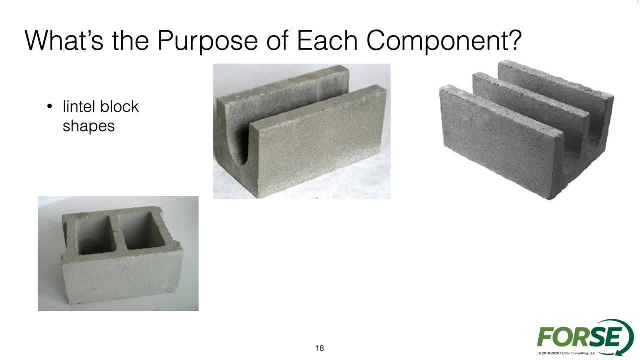 course, masonry lintel, your standard stretcher blocks are going to be just fine. Then you get to the blocks that could probably form the top course. So you're going to have a flow-through. It's going to be a bonding block where you can actually remove the webs of the block and you 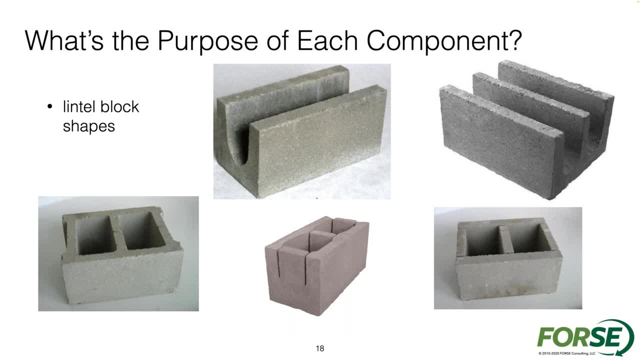 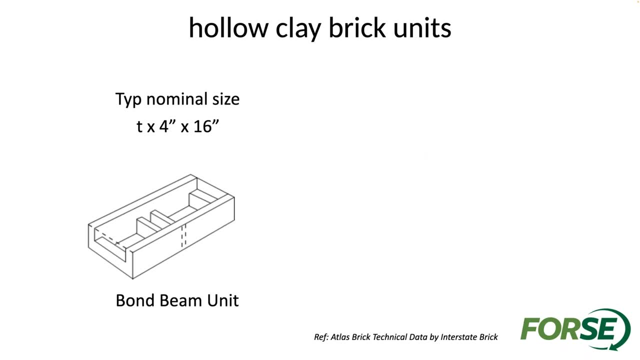 can run the reinforcement kind of through. So that's your concrete masonry options. If you get into the clay masonry again, we have pretty similar blocks that are going to be used throughout a reinforced clay masonry design. But those blocks would be modified right If we had a bond. beam block would need to be. 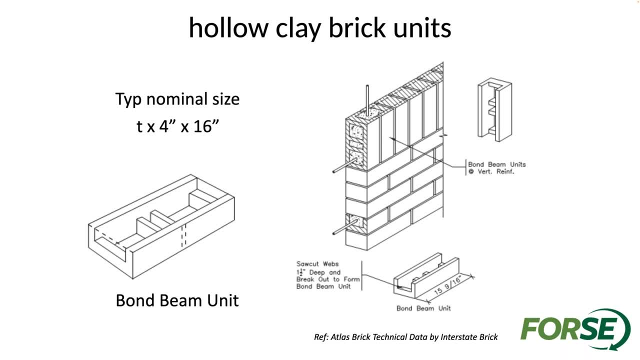 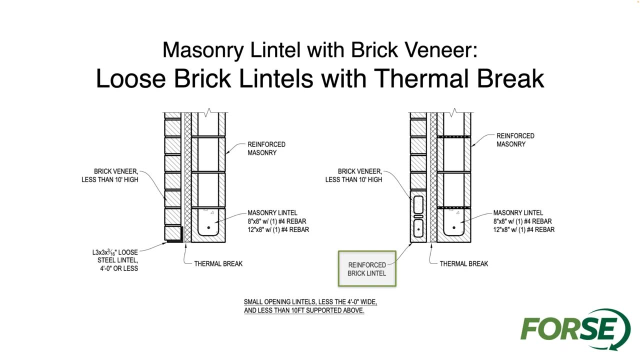 created, or something would have to be created design-wise If you wanted to have reinforced masonry both in the backup wall and the veneer. the only way to kind of do that with a clay masonry is you have to have soldier courses. You actually have to turn the. 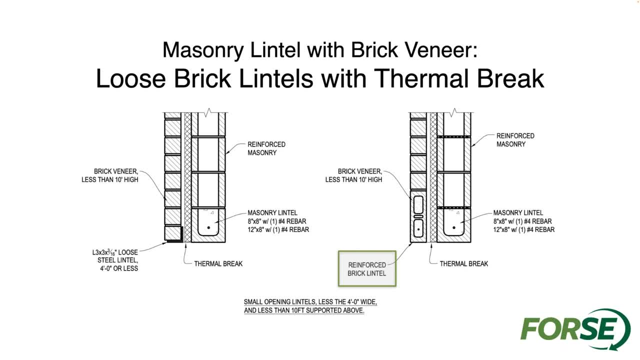 block on its side. Now, it doesn't have to be a full soldier course, It could be a half-high or it could be a third, But it does have to have a soldier course. that would be So. then you could have both masonry and weiss. that could be reinforced masonry lintels. 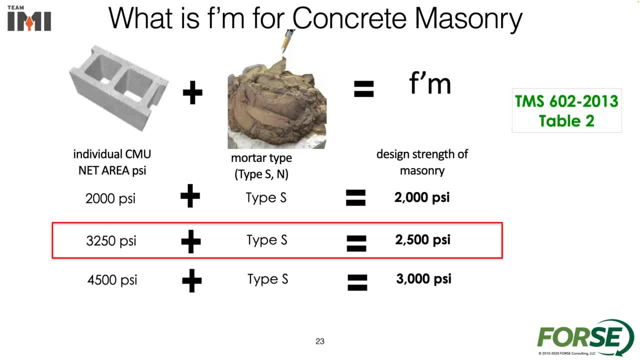 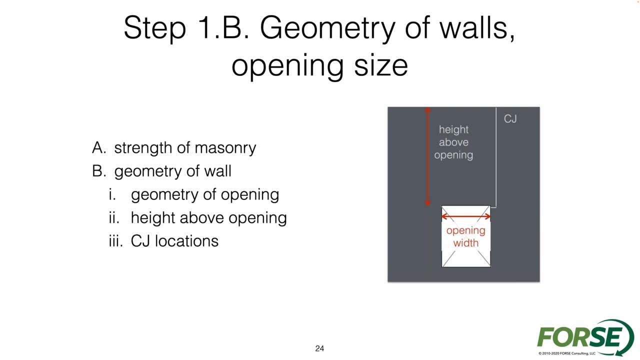 So F prime m of masonry. again, this is…. we keep going back to this, but this is a good reminder. 2500 is really going to be our typical design strength for a masonry wall, that's for, obviously, for our concrete masonry. so the next thing to look at: 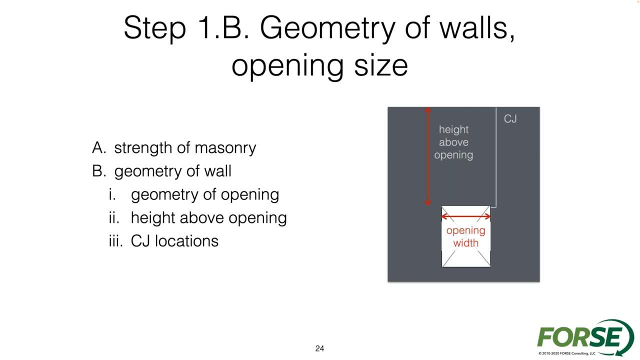 strength of masonry is what it is. uh, the geometry of the wall. um, you know what do we have in terms of the geometry above the opening, the height above the opening? uh, control joint locations, two things that are going to be pretty important to. to look at control joint locations is going 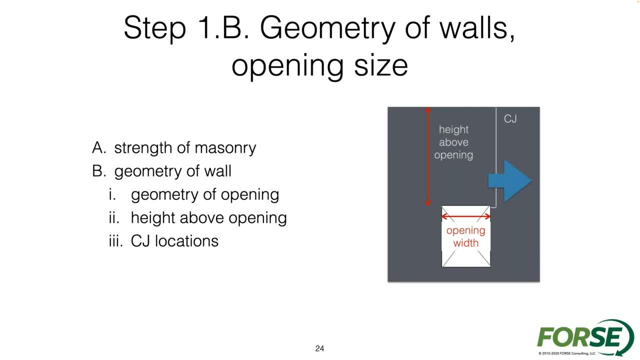 to be something where, again, if i have an unreinforced masonry wall- which again isn't too common for a structural wall, but an unreinforced wall- that's when i have a control joint that's going to be at the opening, but when i have a, when i have a reinforced masonry wall, 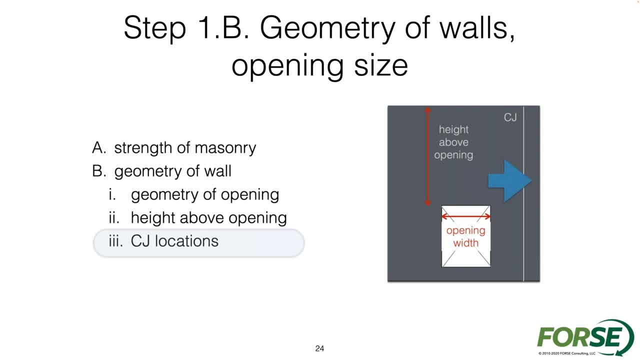 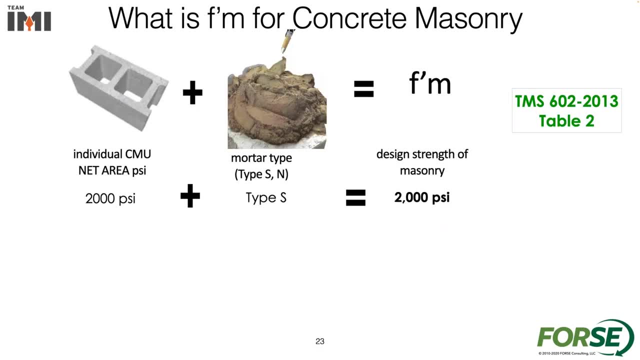 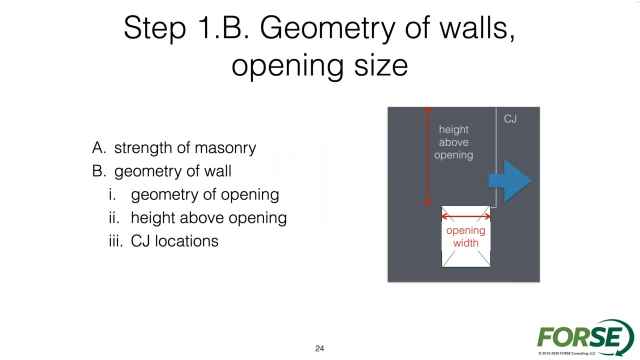 again. let's see one second. yeah, there we go. sorry, when i have a reinforced masonry wall, that's where we're going to get into the control joint. uh, wanting to be away from the opening? uh, the reason for that is i don't need the control joint at the opening because i have reinforcement on each side. i have reinforcement. 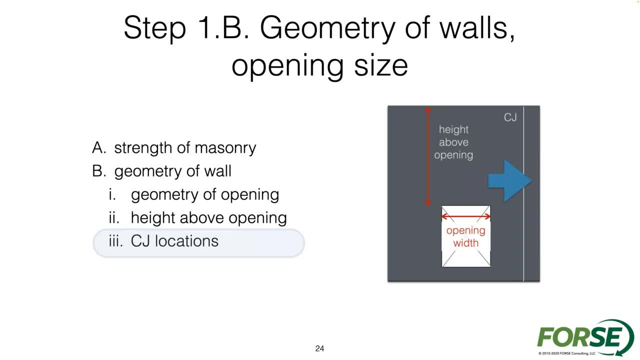 that's going to be vertically on each side in the jams and i have reinforcement in the actual lintel and sill itself. so i don't really have the ability for cracks to occur at the opening corners. so i'm going to be able to get into the control joint wanting to be away from the opening. 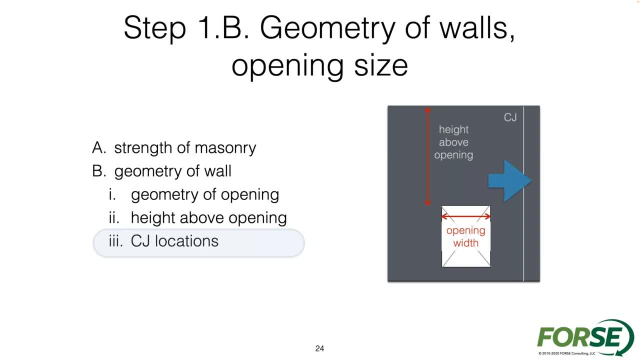 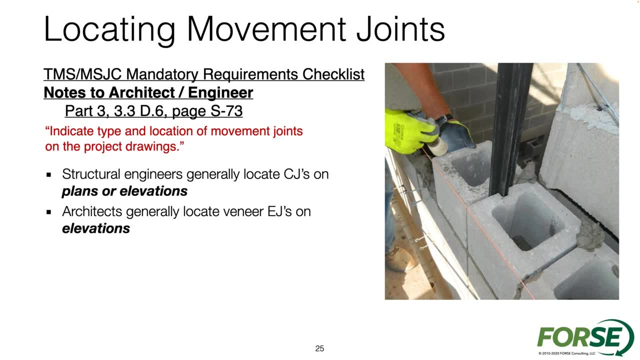 so that's why control joints are going to be important again. locating the movement joints, just like we just talked about uh plans or elevations. this might be a really good point to putting them in on elevations, but making sure that we remember that it's not okay to just put. 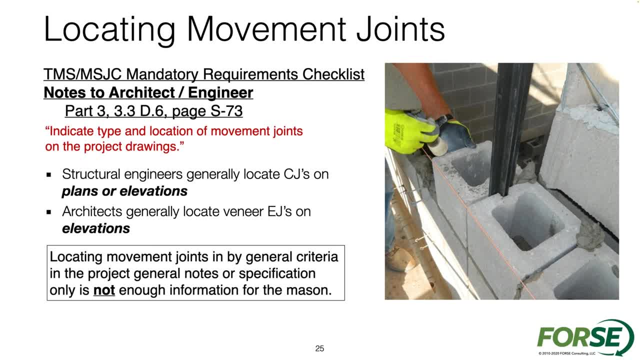 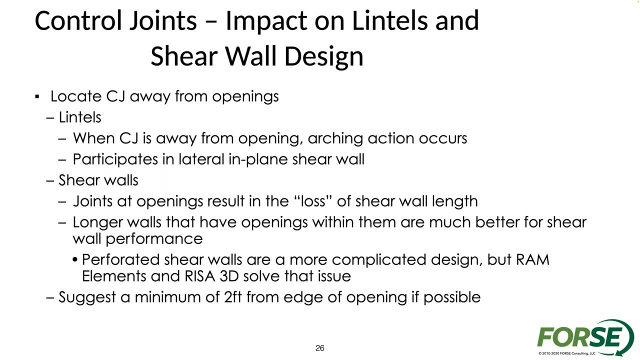 the movement joints. um, in notes, just because of, like, the lintels that i'm talking about here, moving the lintel away is actually going to change the overall design capacity. so locating control joints away from openings it's going to be something that you know. control joints away from the opening, you actually can have arching action. you can actually 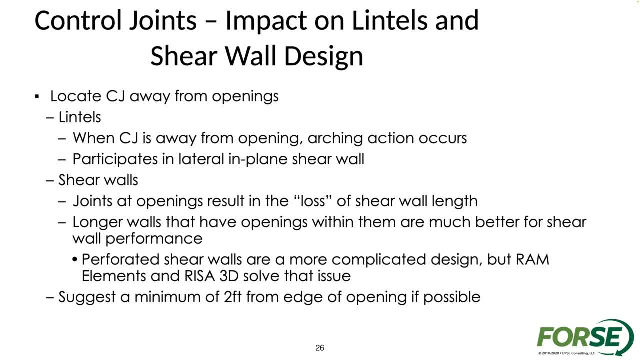 have the mainstream wall, that can. that can form the arch over the opening. if i put a control joint there then i don't have the ability to have arching action. so that really does change the overall performance of the lintel. uh, the wall itself, the, the lateral in plane shear force. 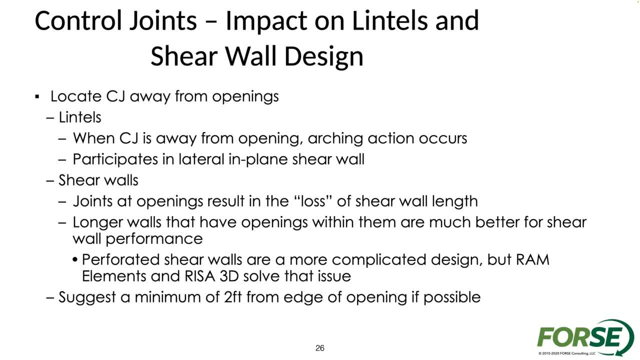 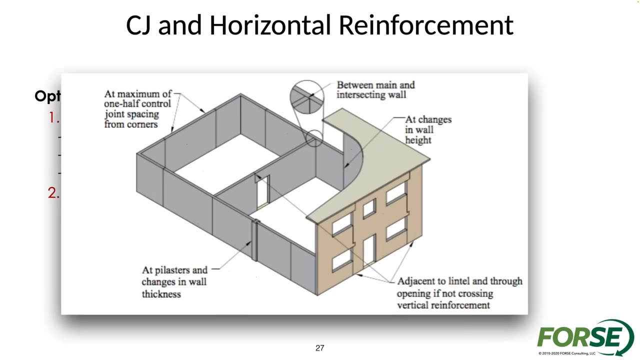 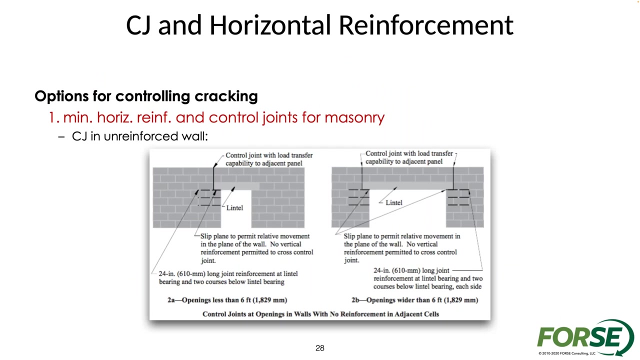 the perforated shear wall is not able to happen when i have a control joint next to the opening. so a lot of different things that change. so what i suggest is at least two feet from the edge of the wall, so that's how we can determine the support of the wall. and then another thing to note is that the lintel joints are built on. their own leading post in place. they're not clipped on the lower part of the wall and they are quite high and high, so that's why the lintels will move a little bit after they're placed, so they're not creating their first uh lintel location. 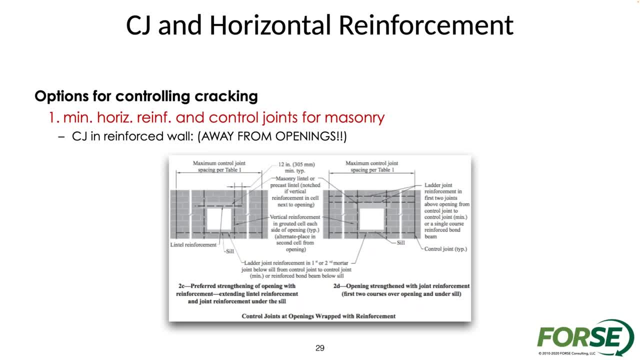 anytime that I have reinforced masonry, Anytime that I've reinforced masonry, lintel and jams, then I wanna make sure that I move those control joints away from the openings And so obviously it's gonna affect the overall lintel capacity quite a bit. 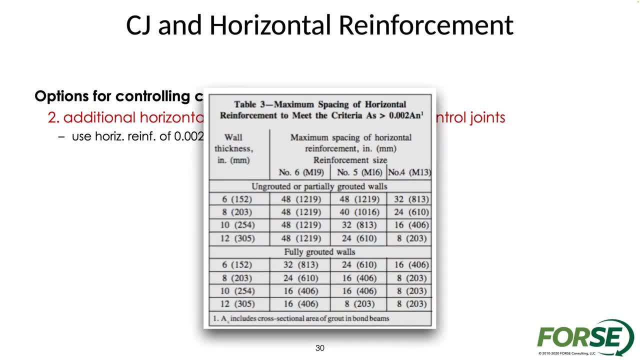 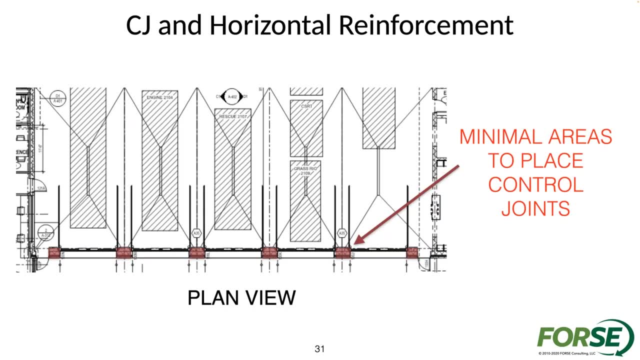 And then again we have the maximum reinforcement. that or the reinforcement that you need to eliminate control joints and how that affects lintels. Let's just say area like this: I'd have very limited locations for control joints anyway, but if I don't have a control joint, 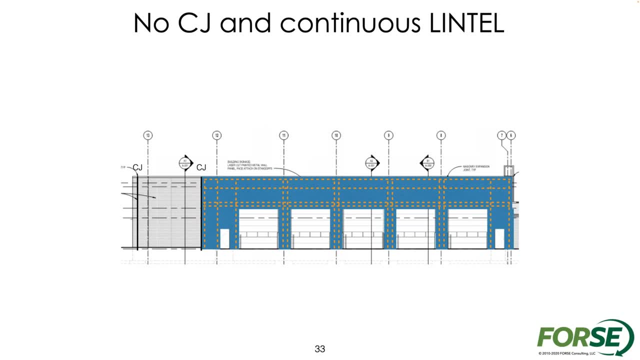 then I have a continuous lintel. You know, I have an area of wall that I can design as one monolithic kind of piece of wall. I have the lintel that's gonna be continuous. I don't have any control joints interrupting. 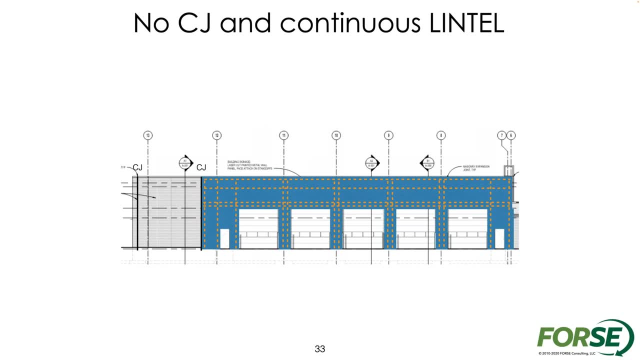 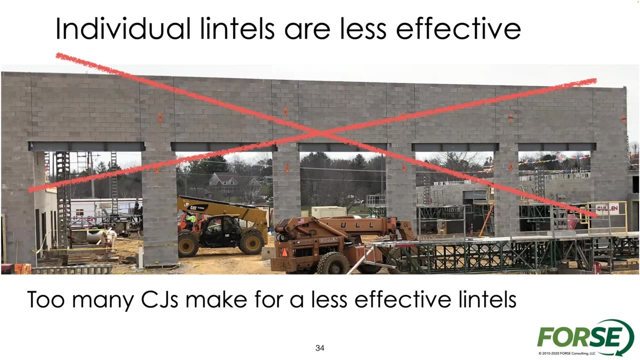 and breaking up that continuity with the lintel that I have beyond the openings. I mean it would be obvious, right? A continuous beam is obviously gonna be more effective Then a bunch of simply supported beams, And that's why we really wanna get away. 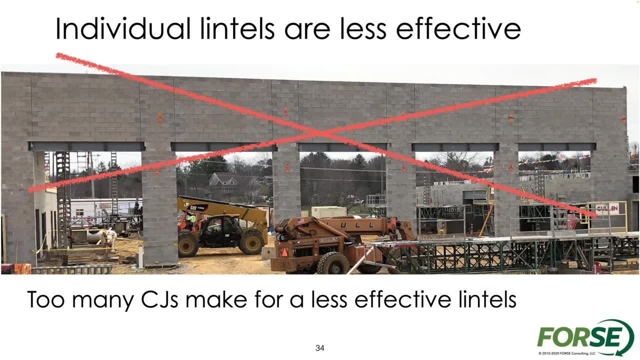 from having control joints at openings. Those individual beam lintels are gonna be a lot less effective. It's gonna make the overall wall performance a lot worse, You know, just because you're gonna have those piers that are gonna be the only lateral resisting element. 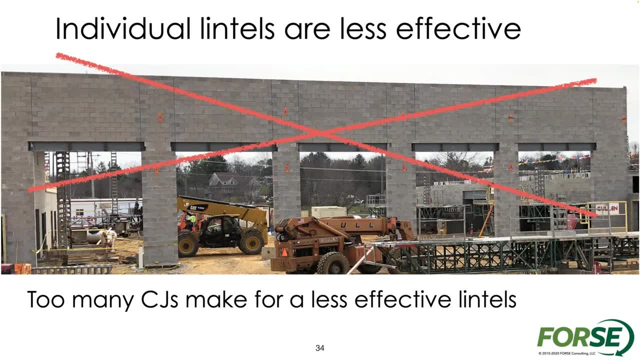 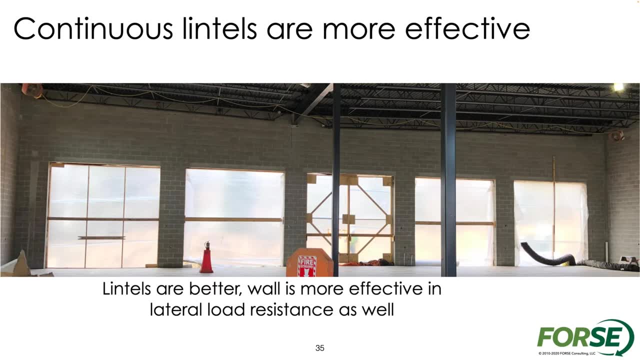 We're gonna have those lintels that are gonna interrupt those piers quite a bit by having some bearing area. Anything. that time that you can have this continuous lintel, this continuous wall span, is gonna be more effective. It's gonna be a lot better performing design. 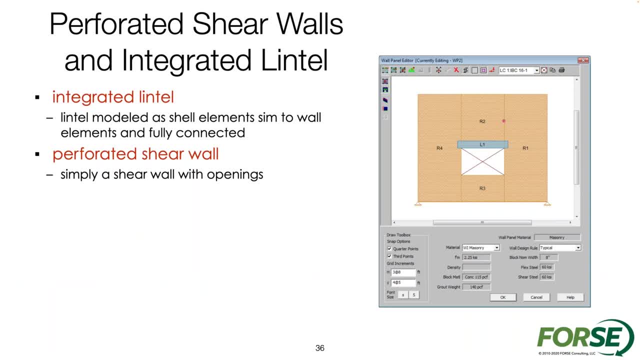 And then, obviously, like I said, with the shear walls, you have an integrated lintel, you have a perforated shear wall. You're gonna have a lot more shear wall capacity. So again having that integrated lintel. you know if I look at a historically detailed wall. 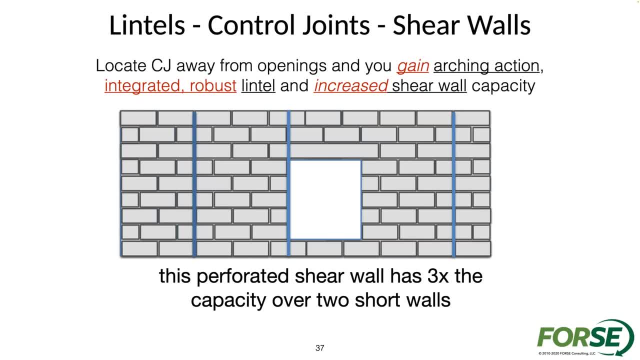 I would have a wall like this where I'd have a control joint at the edge. You know I really have a third of the capacity with the two small walls versus if I eliminate that joint and just have the one really long, short wall, that's gonna have about three times the capacity. 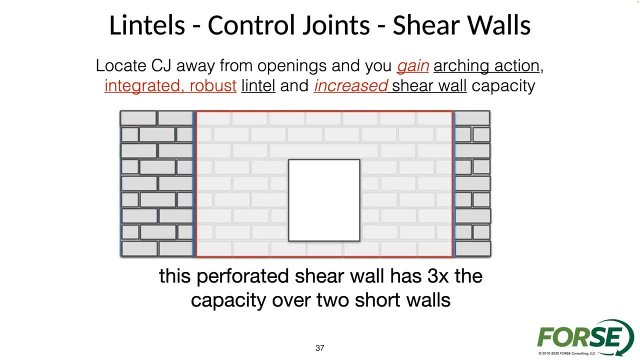 over those two short walls. So that's gonna be kind of a pretty big difference on the overall lintels, control joints, everything that you wanna consider there, shear wall capacity, all of that stuff kind of working together, coming together with those few things. 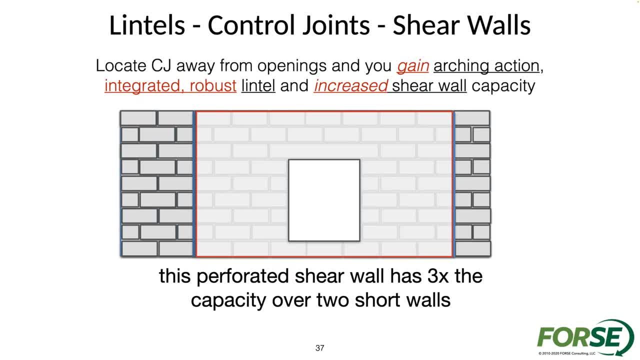 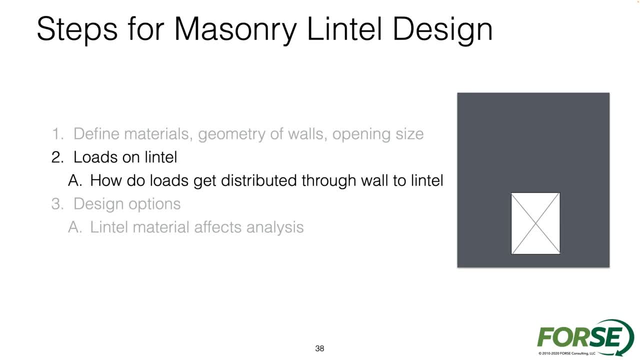 just a few simple things with the control joints And then loads on the lintel. How do the loads get distributed through a wall? You know that's gonna be a little bit more complicated. It's gonna be something that's really important. 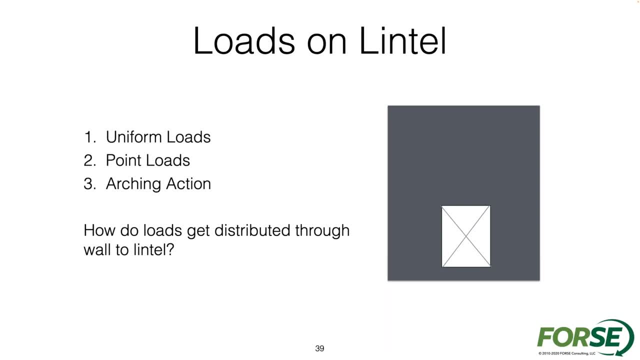 you know, looking at different types of loads that you have on the wall- uniform loads, point loads and arching action- three different topics that we wanna look at. How do the loads get distributed through the wall? I mean just not so much quantitatively but qualitatively. 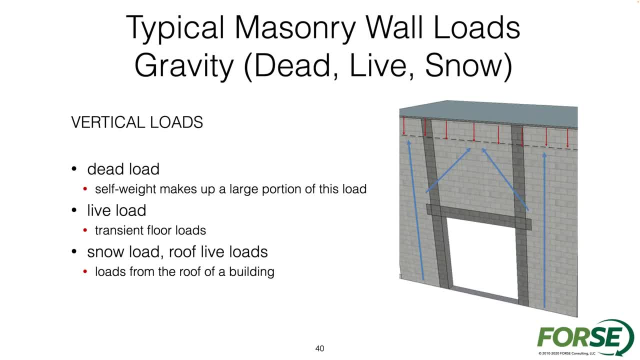 If I looked at a wall, I put on the gravity load that would be on the wall. those are gonna be my red arrows at the top. If I just look at the wall, how do you think it's gonna respond? You know, how is it gonna get to the demand. 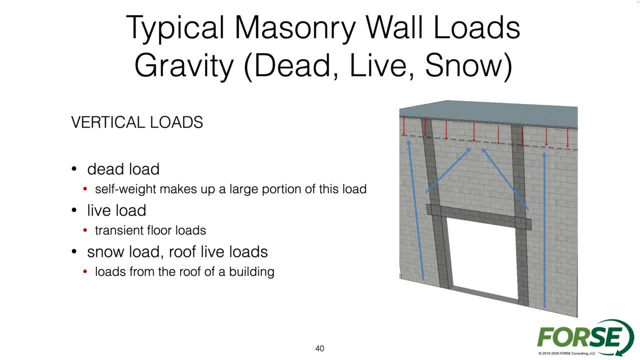 Mostly it's gonna be those blue arrows, It's gonna be vertical compression capacity. that's really gonna create most of the support. You know what's gonna happen to that area below those blue arrows, above the opening. Well, really, that's gonna be what's covered. 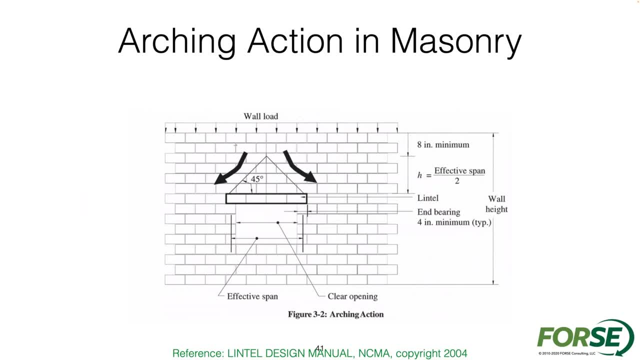 in another NCMA tech guide or another NCMA lintel design manual- arching action- So that goes all the way back to those first few slides of this section- is looking at arching action. You know arching is really gonna be how the wall's gonna. 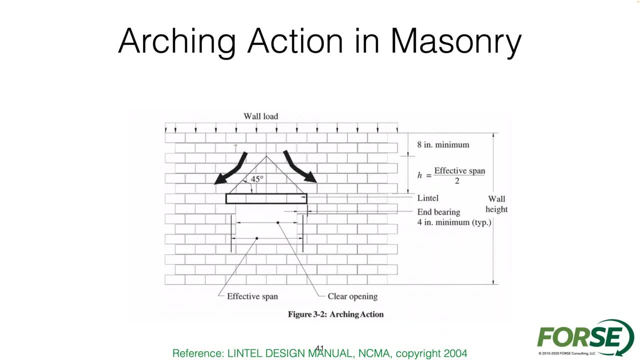 respond to the loads on the wall. The compression, stiff compression elements that are part of masonry are really gonna do most of the load supporting for the masonry design. It's just gonna be kind of that small area below the arch That's really gonna be the only load. 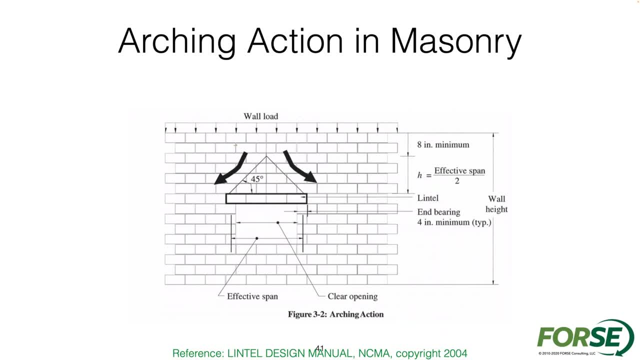 that you're gonna see on the lintel itself. The wall itself is gonna really support most of the wall load, the roof loads, so on and so forth. You know, looking at an arch design, you know what are some of the key components for an arch. 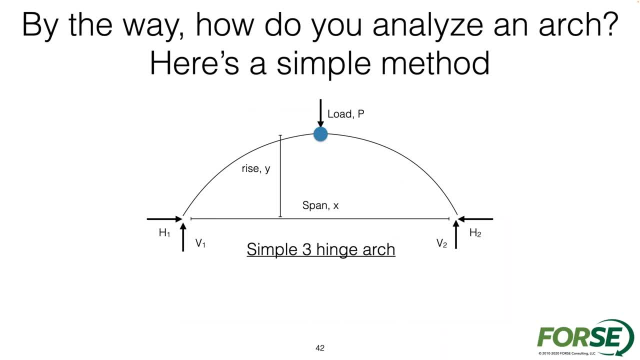 Anytime. just looking at a simple three hinge arch is probably the best way to kind of get a handle on some of the forces that you would have or reactions that you would have Really, if you have a load at the top of the arch right. 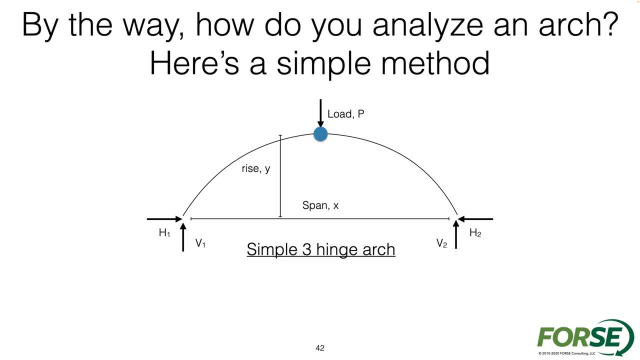 it gets resolved by having vertical loads at the bottom, but because it's an arch, you really have some horizontal loads that you know the arch is gonna be, you know, creating or forcing load into the abutments on each side of it. 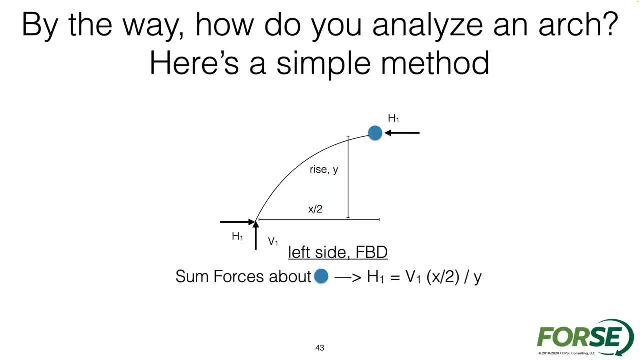 So if I just looked at a free body diagram, you know, looking at some of those forces that you would have in there, the horizontal force is gonna equal to kind of that vertical force. it's gonna be kind of equal and opposite if it would have a really simple three hinge arch. 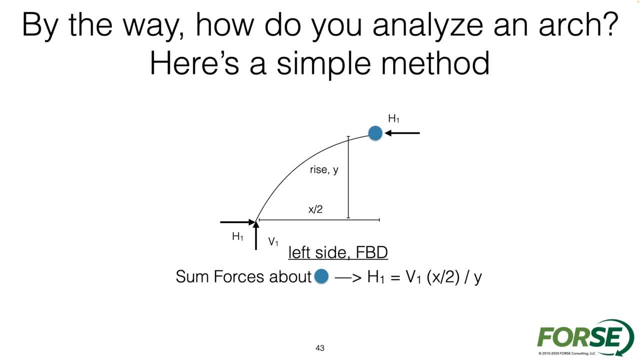 Obviously we don't have that, but that's kind of a really nice simple way to kind of look and see what the forces would be design-wise So thrust being half of the load of the arch. I mean, I think that's what sometimes can scare people away. 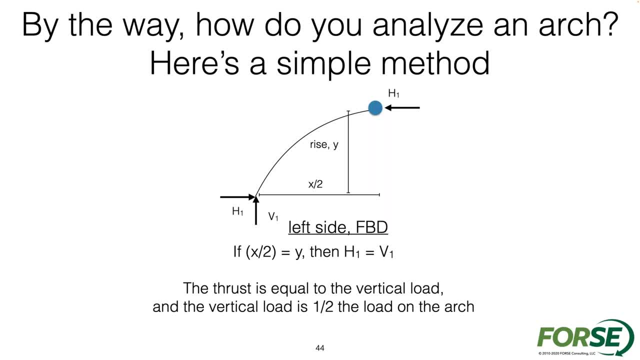 from looking at arching action, just kind of recognizing that there is all these new forces that we have to consider. But again, masonry is good in shear. Those, any areas outside of the openings, are gonna be very good at resisting any of those thrust loads. 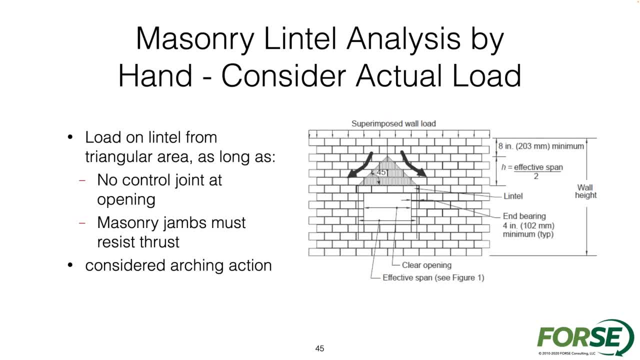 So load on the lintel is really gonna be just kind of a triangular area. The NCMA guide does a really nice job of showing you know again, if a wall is taking care of itself, it's taking care of those roof loads. 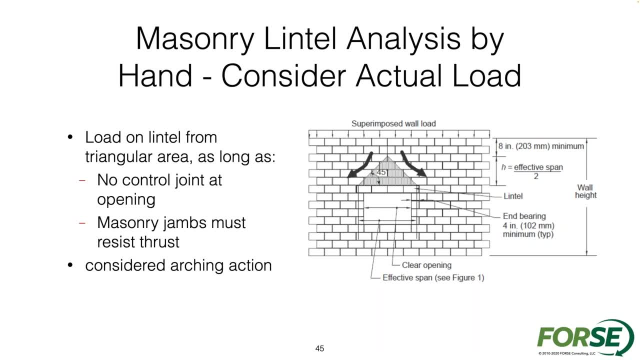 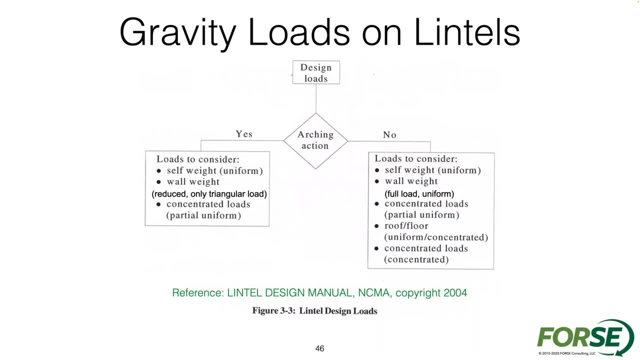 you know, really the load on the lintel is a pretty minimal self-weight plus the weight of the wall in that triangular area below the arch. Within that lintel design manual it actually has a nice little flow chart If we can consider arching action. 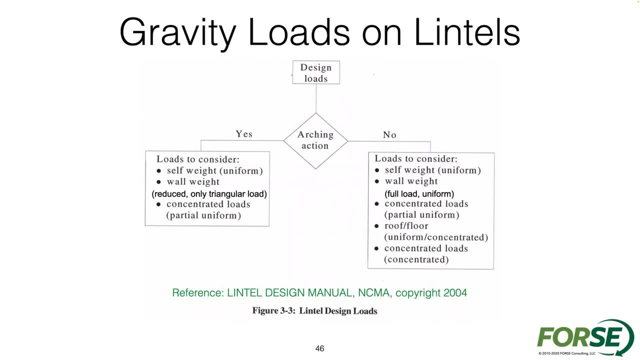 then the very small loads that you have to consider for design, or if you can't consider arching action, that's when really a lot more load starts to kick in. We have to not only take into account the self-weight but the full weight of the wall above. 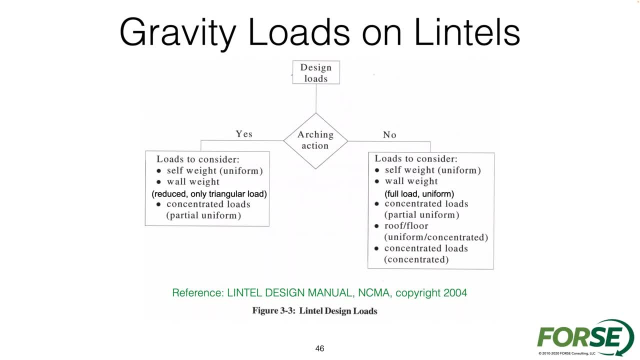 We have to take the full weight of the roof loads. We have to take, you know, all of the concentrated loads. So we're really now demanding a lot more load on that lintel. once I can't use arch, and why wouldn't I be able to use arching action? 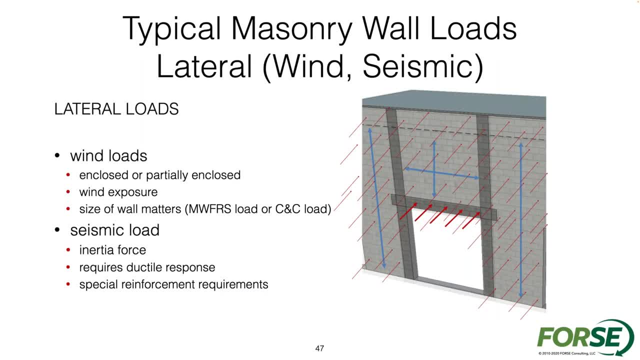 Again, that gets into. if I have control joints on each side, then I'm gonna really lose the ability to do that. The other load that we wanna think about again is lateral loads, Pressure loads. you know kind of how does masonry respond? 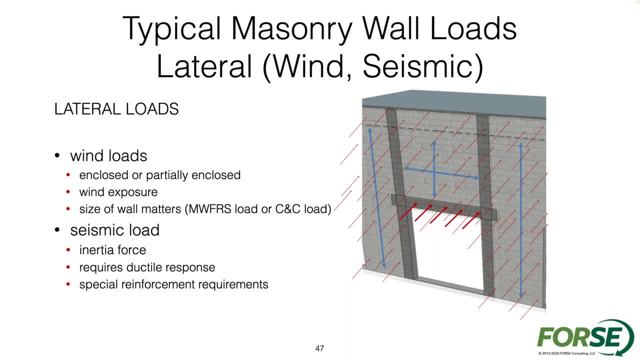 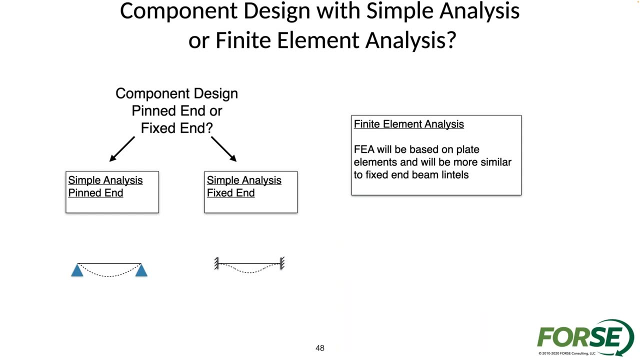 You know where are some of those forces. You know the red pressure forces, wind loads or inertia forces from seismic. where do those forces go and how does the masonry wall respond? So, again, if I would look at some of the different tools, 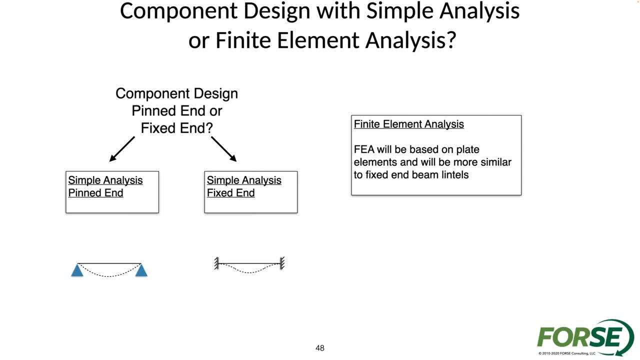 that are gonna be available. so this will start introducing some of the software pieces because I think that's a very, very relevant and necessary for understanding overall masonry. lintel design is: what tools do we have and what those tools are? Again, we'll talk about software a little bit more later. 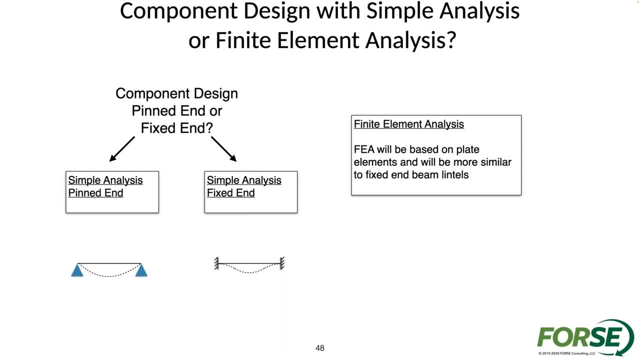 and we'll kind of complete the whole picture in terms of why software is important for masonry design. But we're gonna start a little bit with it here because, just because helping us understand what some of the forces are in these lintels- 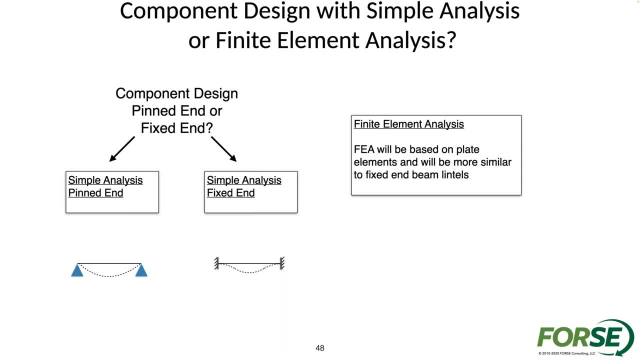 So if I would look at the lintels and the analysis options that I would have available: simple analysis and pinned end. that's how a lot of people have been designing masonry lintels or lintels within masonry walls- if it's a steel lintel- for a very, very long time. 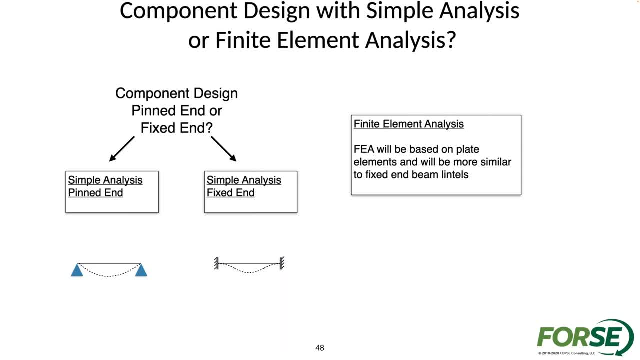 That's one option. I can look at a simple analysis with fixed ends that would change the forces to be a positive bending moment and then negative bending moment at the supports. And then this third option that I'm introducing is find an element analysis option. 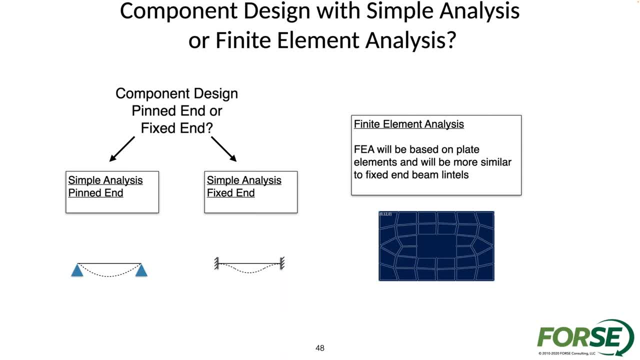 where I would actually have plate elements. I would model the opening with all of these different plate elements so that I can have an understanding for what some of the stresses and forces would be in those plates design wise, Practically. I mean, you can see lintels are gonna be. 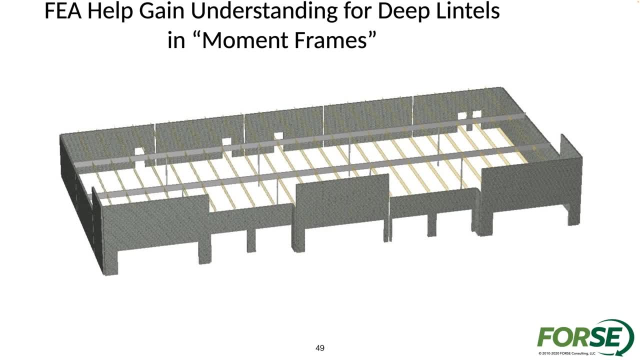 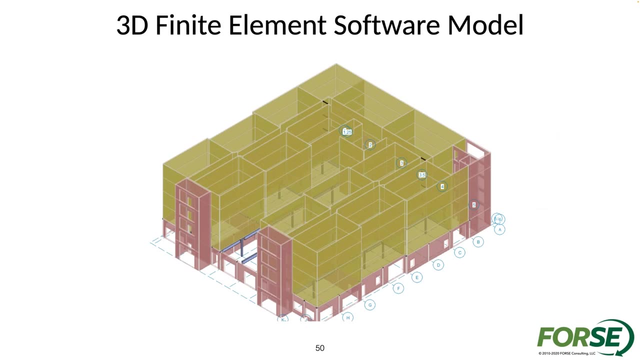 all over the place in these walls. They're gonna be in buildings like this that maybe have a very long span openings, Or I could have a lot of lintels kind of spread throughout the whole building. Looking at it with software is gonna be able to help us. 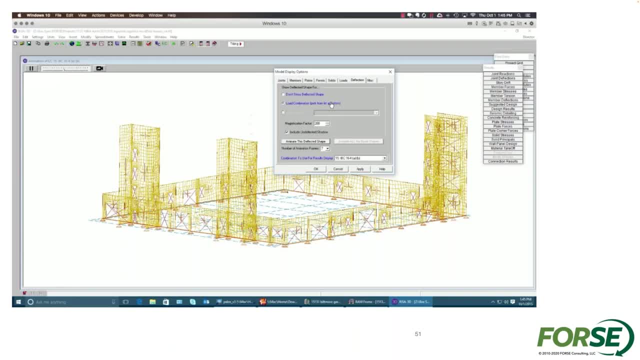 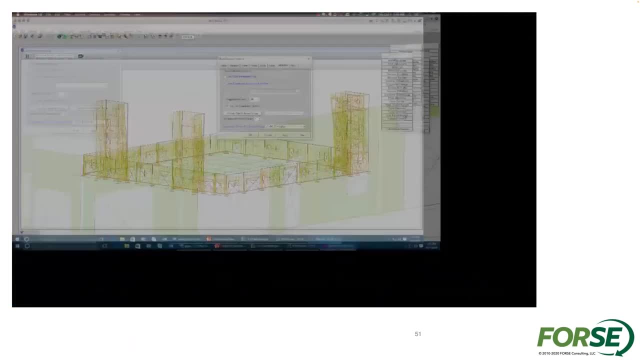 really understand that behavior. I can understand the overall building movement, but really with software I can also tunnel into and look at a kind of a specific area. I can look at how lintels are gonna behave and interact with piers and so on and so forth. 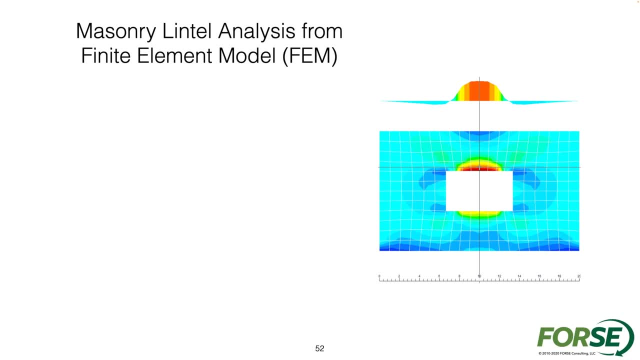 So again, software find an element. analysis software really can help me understand, I think, of the stresses and forces in the wall itself. Again, more on that later. But if we're kind of tunneling in on lintels here a little bit, 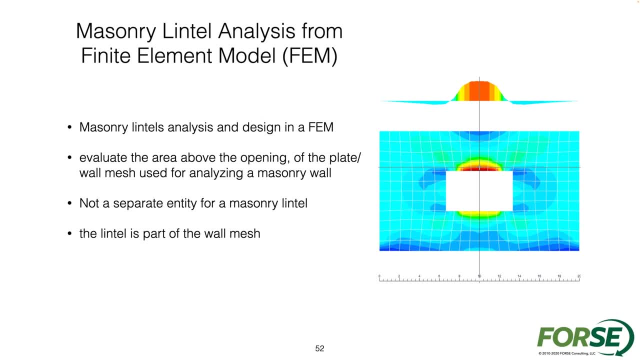 we can see a whole lintel is gonna be integral with the wall itself. It's not a separate entity. for a lintel little is part of the overall wall mesh. If I really wanted to see what some of the forces and stresses are on lintels and demand for lintels. 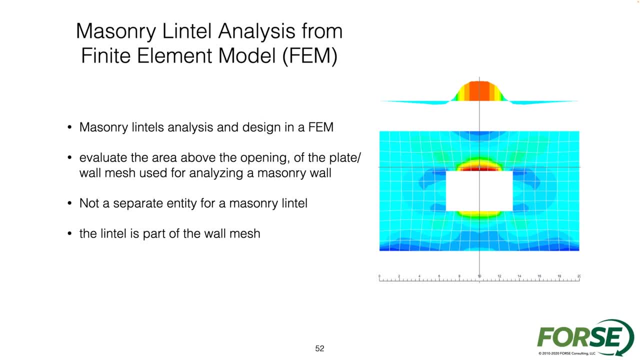 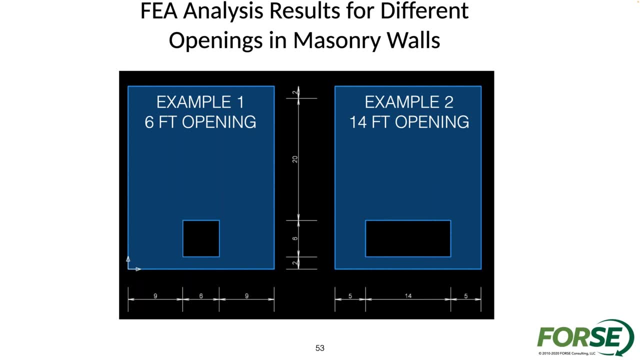 looking at it with a finite element. analysis is gonna help we understand these forces pretty clearly. So if I have- let's just look at a couple of different examples- If I have- a smaller opening, a six foot wide opening, a six feet tall or a 14 foot wide opening, 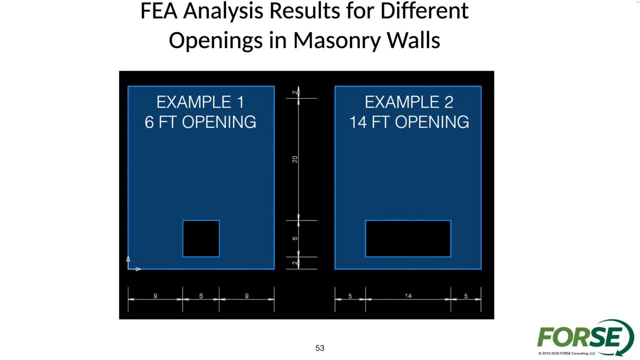 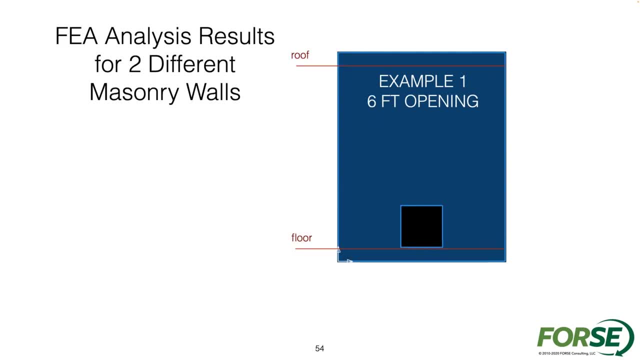 maybe this is a big window again, six foot tall. You know what are some of the stresses and forces. Because of the finite element analysis I can really do, you know, evaluate this and kind of slice and dice this thing in a few different directions. 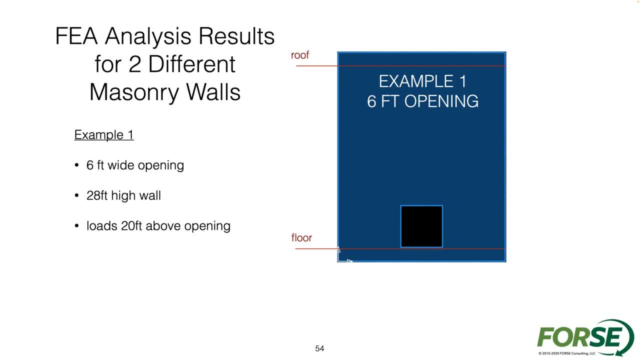 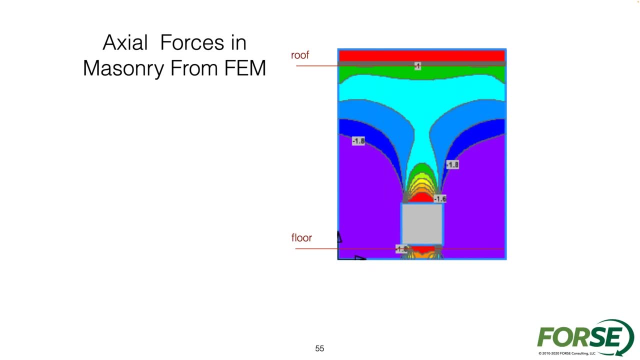 and kind of see what some of the forces are. So again, six foot wide, 28 foot high wall, 20 feet of load above the opening. If I would look at the axial forces on the masonry wall from the finite element analysis, 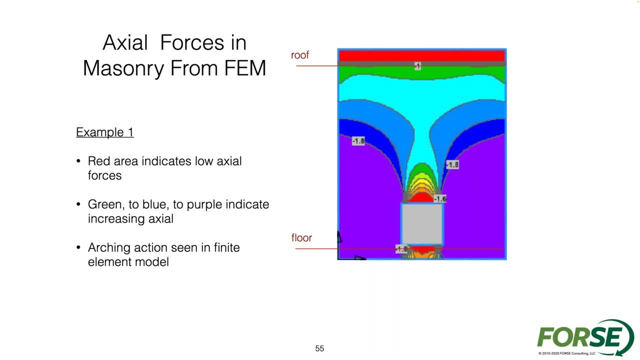 now, red color here is gonna indicate low axial stress. So at the top of the wall obviously is gonna be a low axial stress, But then you can see the area right above the opening. the axial stresses is essentially gone. You know the wall. 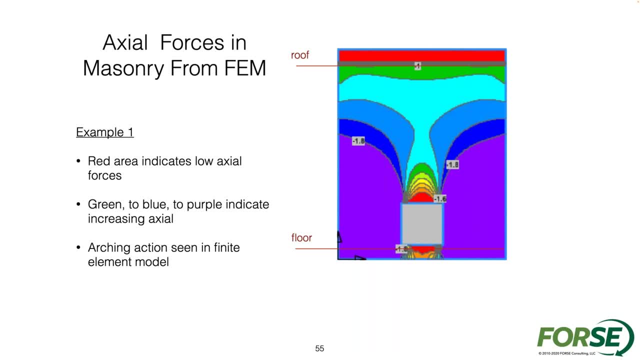 itself again is bridged, the opening. It's got a lot of compressive capacity. The axial forces are getting shed from the wall area, So it's a low axial stress at the top and then low right above the opening, Then obviously low right below the opening as well. 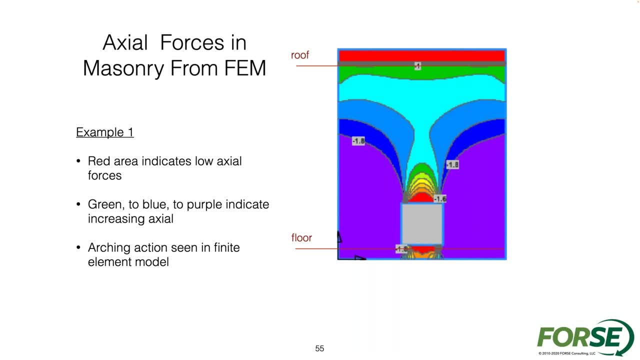 And then you can see the green to blue, to purple, indicating higher and higher axial forces, And that never really gets into the actual area above the opening. So you can see the arching action Actually occurring in the stresses that we look at for the wall. 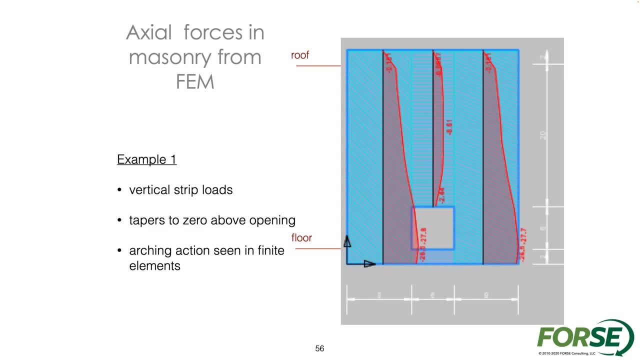 If we actually again look at the sections that we have here, look at the actual forces, you can see the forces and how they're accumulating. If I look a little bit closer at the area right above the opening, you can actually see the axial stresses kind of increasing. 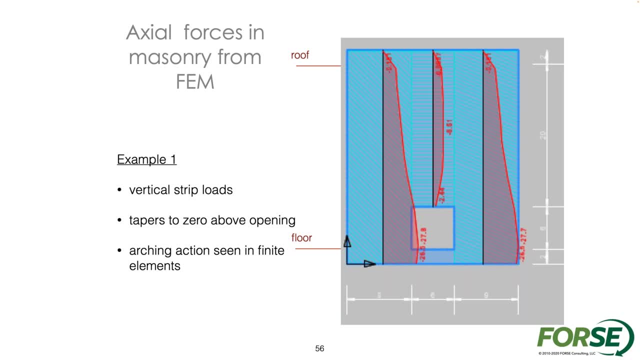 then kind of stabilize and then actually decrease as we get to right at the edge of the opening, which obviously I don't have any axial stiffness right above an opening, It's just an open area, So the axial forces have to go someplace. 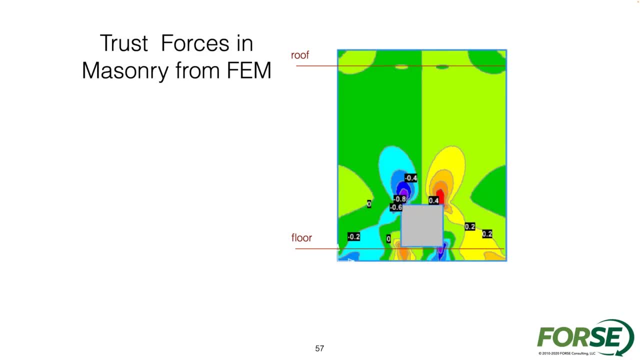 So you can see that arching action, The other main part of arching action is I have the axial forces, but then I have the horizontal thrust loads as well. So again, looking at what those would be, looking at the horizontal forces with finite element analysis. 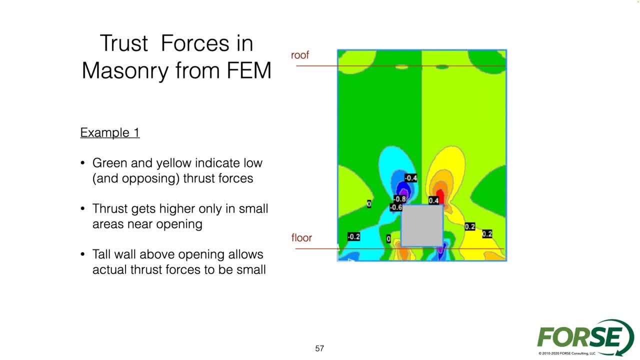 I can see again green and yellow kind of opposing opposite forces. obviously for the most part it's kind of nil, It's pretty low. It's kind of nil, It's pretty low, but then you can see those stresses kind of getting higher. 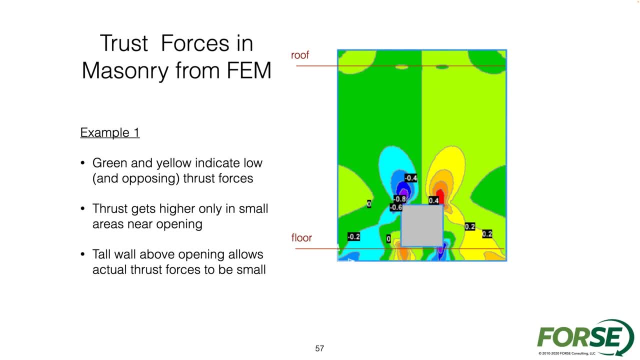 and the thrust forces being the highest right, at the corners of the opening. It doesn't necessarily carry through the whole wall, though, right. I mean it's just right there, kind of at the corners of the opening, and then it kind of dissipates. 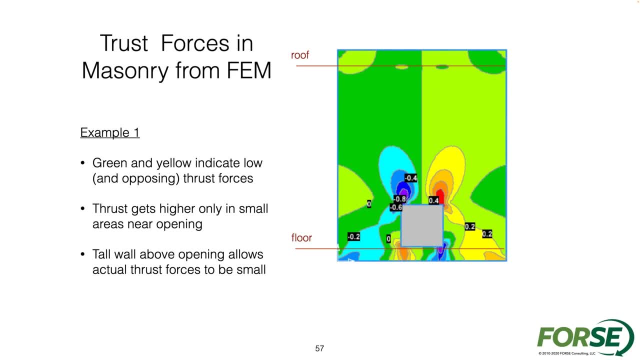 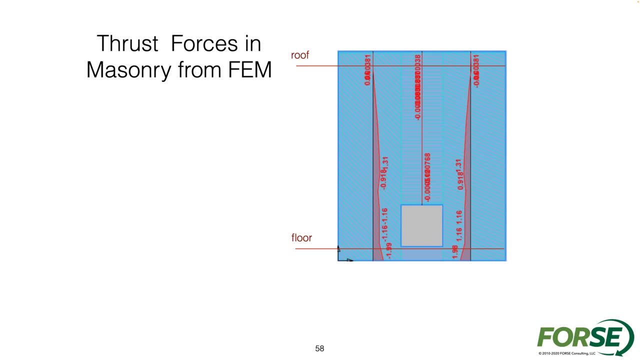 as we go out further with the wall, which I think is kind of interesting right. And then the overall thrust loads are pretty small. I mean, the thrust loads are about 10 to one, the thrust being the one, the axial forces being the 10,. 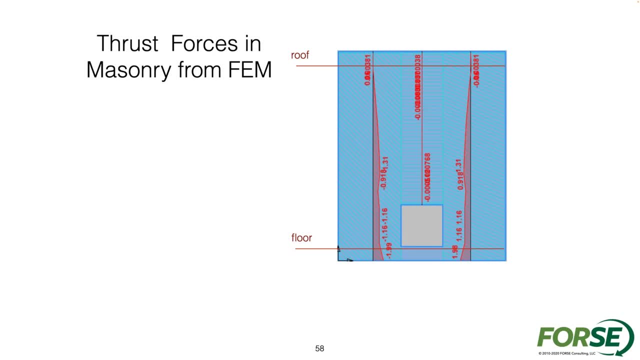 it's like a 10 to one ratio between axial and thrust loads. And so, again, if we think back to the empirical arching action guide where we looked at that simple arch, where it was one to one, that's a very conservative way to look at it. 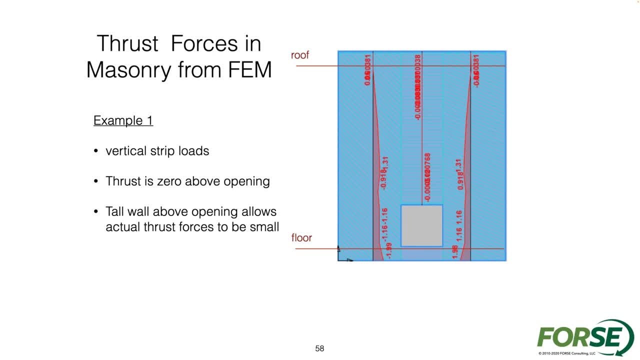 Really, the actual arching action is gonna be able to dissipate the loads quite a bit. We have a very deep arch here. We have very deep arches. that can be occurring. There's arches within arches, within this wall, right. 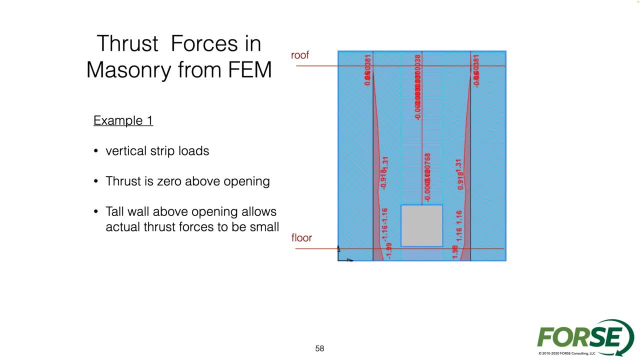 It's not just a singular arch. The wall doesn't just arch in one nice little uniform arch above the opening. It actually can arch the entire height. So that's why the actual thrust loads are very, very low, kind of that 10 to one ratio for thrust loads in the wall. 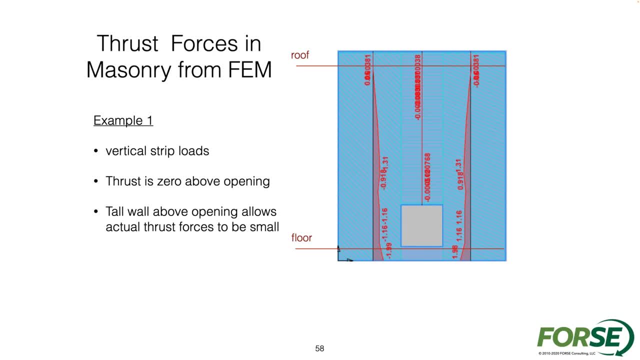 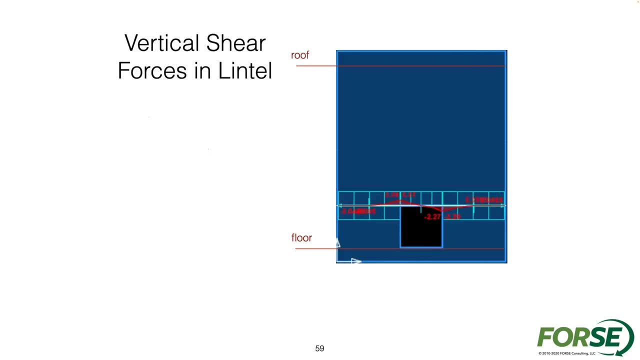 So you can see them. you can see that they're there and once they accumulate and kind of stabilize, then they don't really change throughout the rest of the wall. So I think very interesting. Other things that I'm interested in is I'm looking at the actual lintel itself. 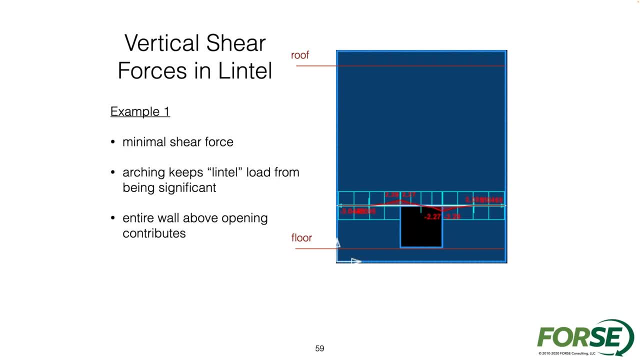 If I kind of slice and dice some of the different forces, the minimal shear forces again, I don't have a lot of load that's gonna be local to that opening if the wall is arching throughout the height of the wall. So again, the lintel load. 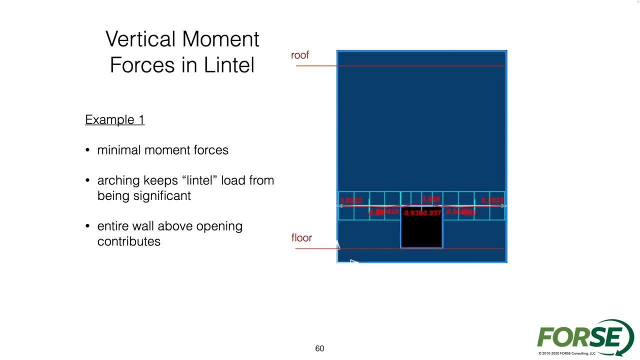 the shear loads are gonna be relatively small. If I look at the moment, demand also gonna be very minimal. I can see some negative moment area. I can see some positive moment area, So all of that stuff makes sense. It's really tied in. 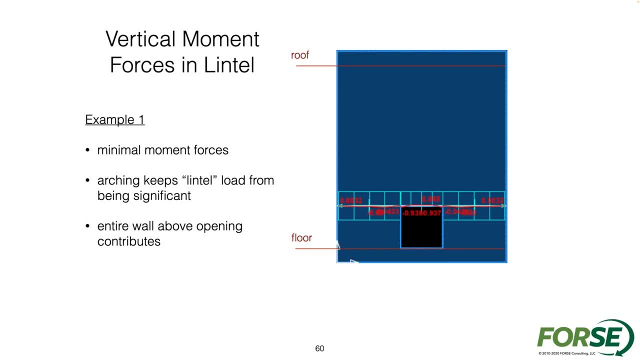 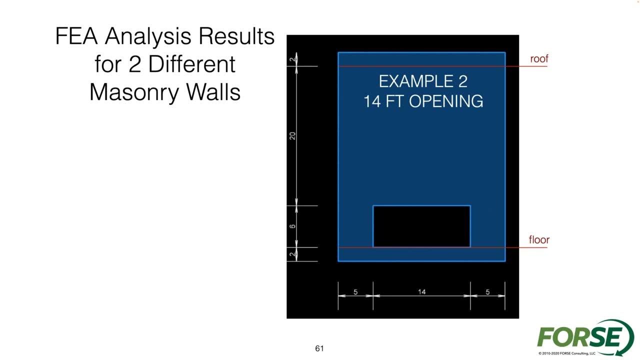 It's kind of the fixed end member condition that I was thinking about, And so that was the smaller opening. What about the bigger opening? So if I go to the bigger opening, does it fundamentally change? Do I have some really radical differences here? 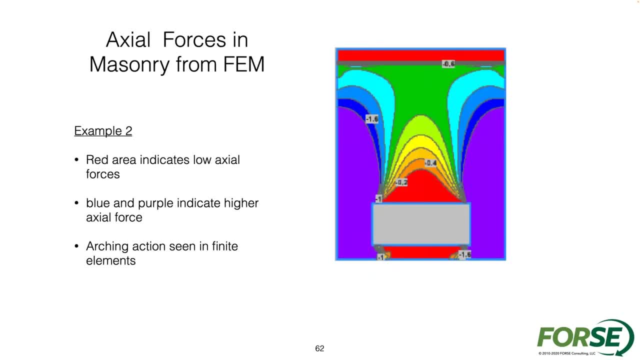 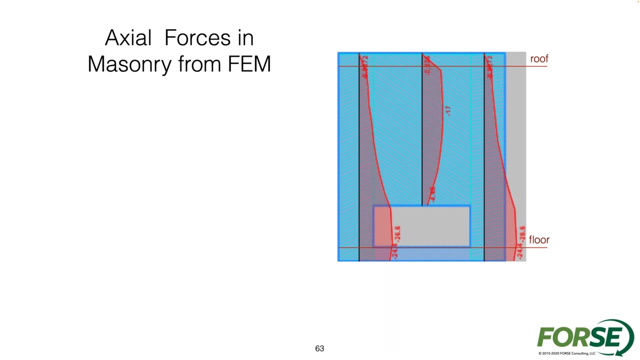 14 foot wide opening. Again you can see the axial stresses. You can see the red being the low axial stresses. Very similar behavior, It's just on a larger scale. So axial forces you can see again get higher. 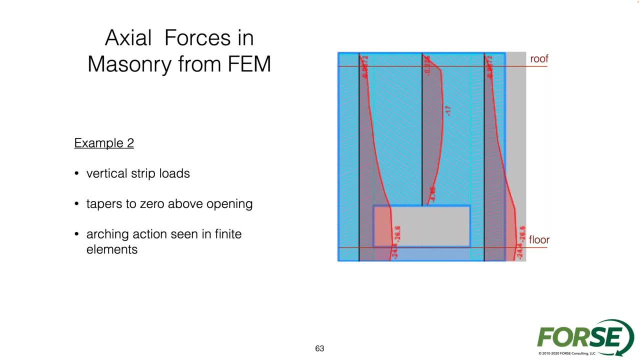 and then they start to drop off. in that area above the opening You can see the axial forces get, not just linearly, but you can see that on each jam it's actually accumulating forces quite a bit faster once we get closer to the opening. 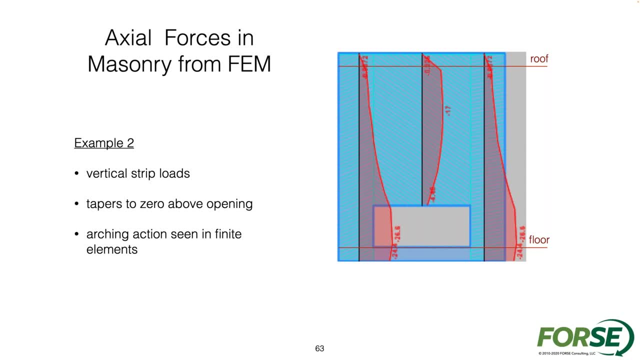 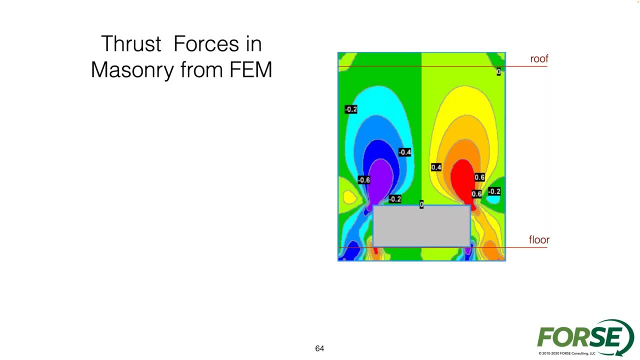 So you can see that the load's getting shed and dissipated to the outside, which again makes a lot of sense. You can see that arch occurring Again. the thrust forces- the thing about the thrust forces: you can see them occurring higher within the wall. 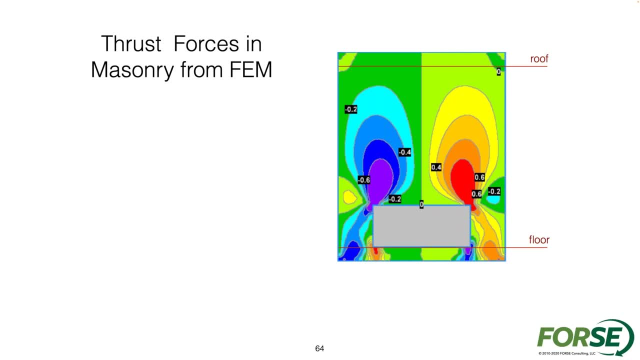 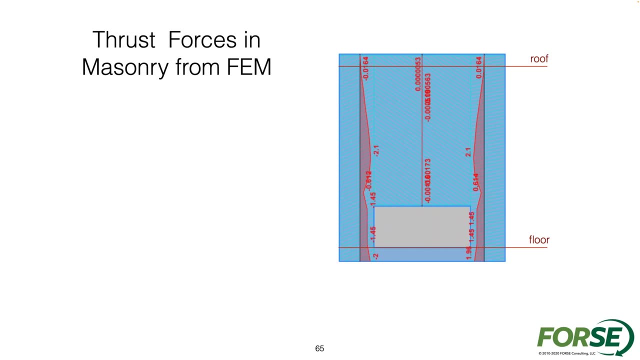 So it's like it's a deeper arch that gets created. It's not so much just local to the opening. So I think that that's very interesting. I think the thrust forces, you know, this is maybe a little bit higher, but it's not that much higher. 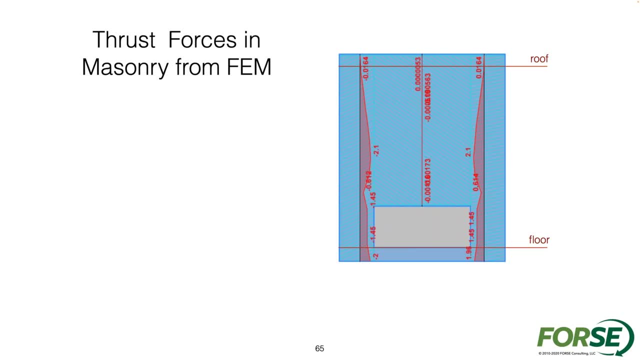 We have still a very tall arch, very tall arch that are able to accumulate within this wall area and so that the thrust loads are still relatively small relative to the size of the opening. It's not a one-to-one ratio, It's still, you know, six, eight to one. 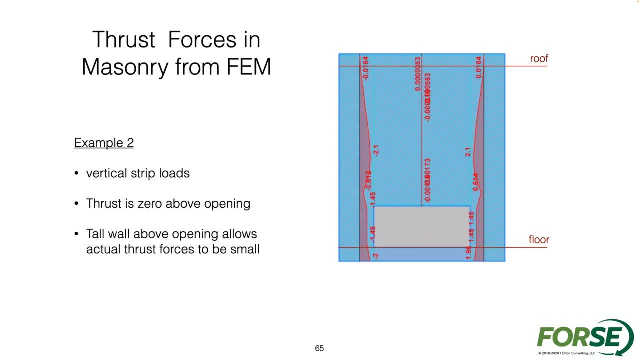 in terms of the axial force to the thrust load that we have occurring. So again, the axial forces are good to understand, The thrust loads are really good to understand with the tools that we have here. Oh, we also want to look at the shear. 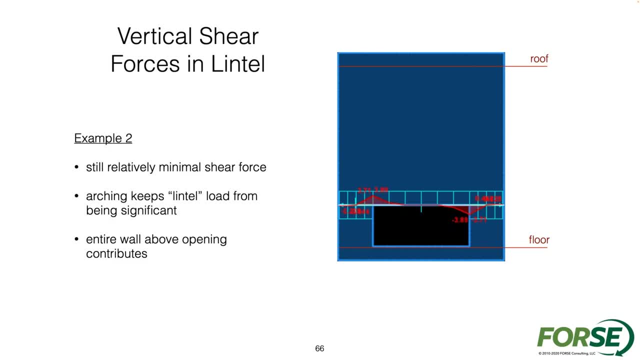 The shear force is still relatively low, Relatively small. You know the things about a finite element analysis programs is it accumulates the forces It shows me. you know some of this information based on the sections that I cut Here. I cut a relatively shallow section. 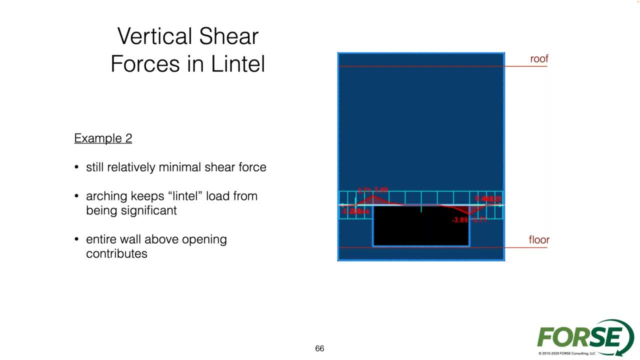 And so you can see some of the forces. If I cut a taller section, if I actually say this larger area is the area of the lintel, then you can see my forces go up. Well, I'm cutting a larger section And so there's some practical experience that's needed. 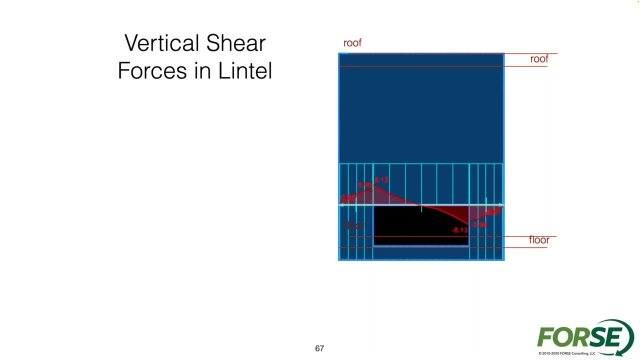 to say: I'm designing a lintel, I'm going to design this area of the opening, this height of the lintel for this span of the opening, And so, as you change the different depths of a lintel within a finite element, analysis. 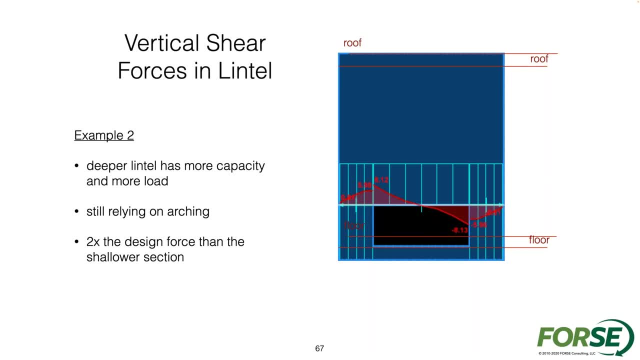 you can see the different forces that would be needed to be designed for in that local area. So that's where you can see the shear force here. Moment forces: These are relatively nil Again with the smaller section if I do go to the larger section. 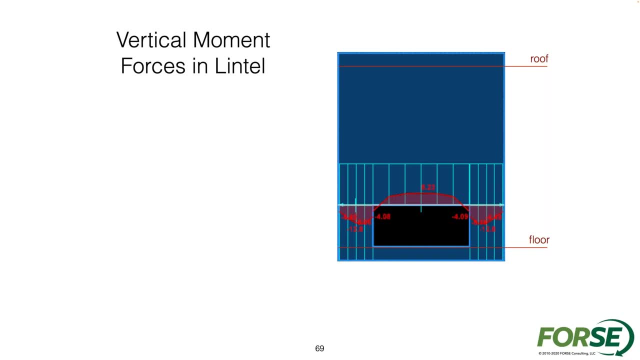 you can see more relevant positive and negative moments that are being created here and shown on the diagram. So again, finite element analysis. we haven't touched on it too much, but just realizing the software really gave us a much, much better understanding, I think. 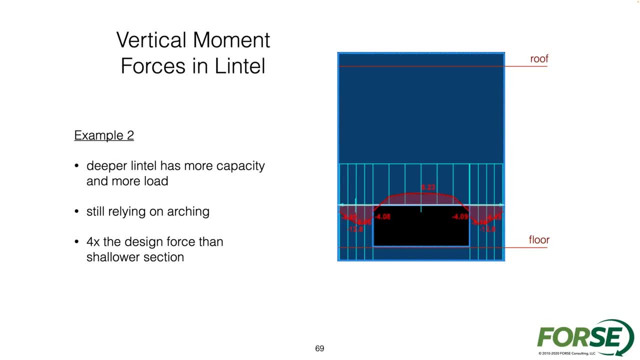 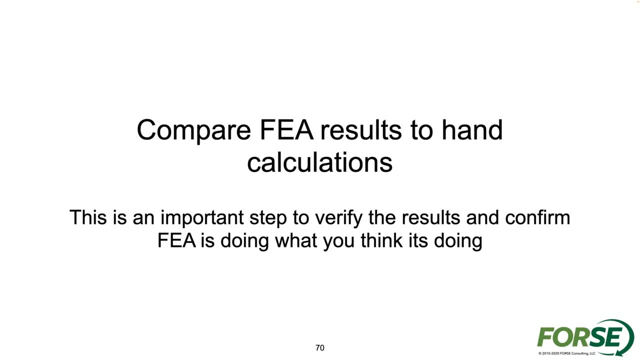 of the forces that you have with a lintel, that's going to be, that's going to grow with the wall around it. So I think one of the really important steps of doing software analysis is being able to actually verify it, kind of back check it. 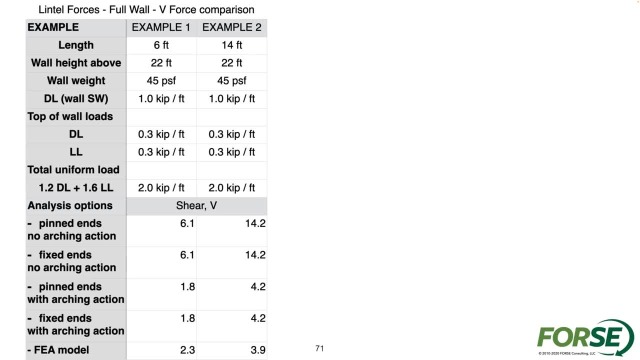 And so that's what the next few slides are going to be. First, I'm going to start with the hand calculations, we'll call it. We'll look at the different spreadsheet numbers, just kind of going through these kind of one line at a time. 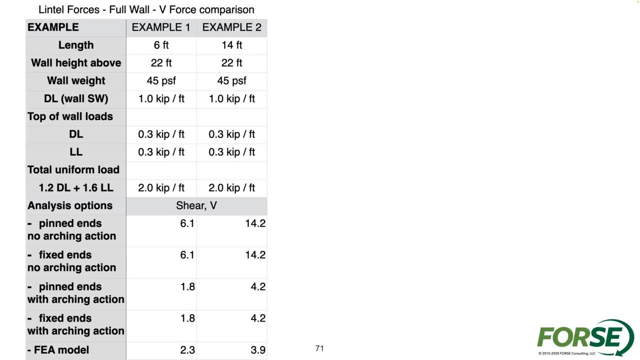 We look at the two different examples Again. we have the length of six feet versus 14.. We have the height of all. the opening is 22 feet. in both cases a wall weight, a dead load from a self weight. We have the loads that we have in the top of the wall. 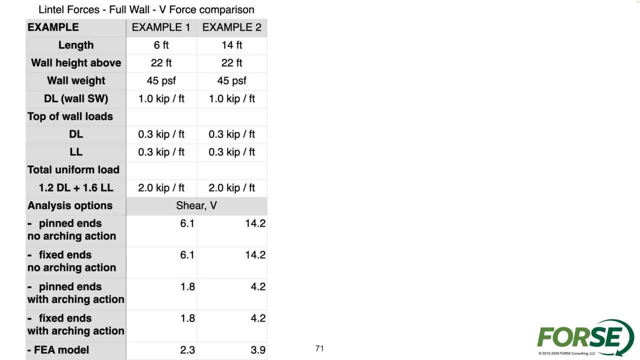 dead and live load And then we have the combination that we used. So the different analysis options that I looked at is: I looked at pinned ends- no arching action. So that's looking at it as a pinned end. lintel- no arching action available. 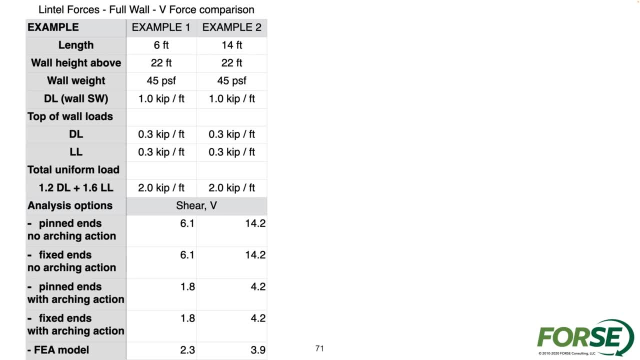 So it's just going to be a positive moment. in the center I look at fixed ends, no arching action. I look at pinned ends with arching action. So pinned ends with arching action is going to be looking at most of the load going outside of the lintel area. 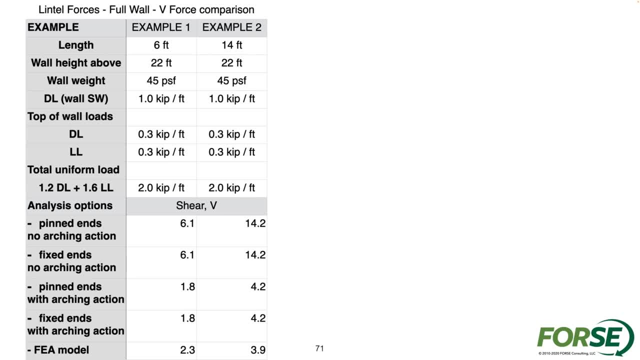 So the load is going to drop down to just that triangular area, the empirical kind of arch that we were thinking about. So pinned ends is going to be the same shear as fixed ends with arching action. It's just going to be a lot less load. 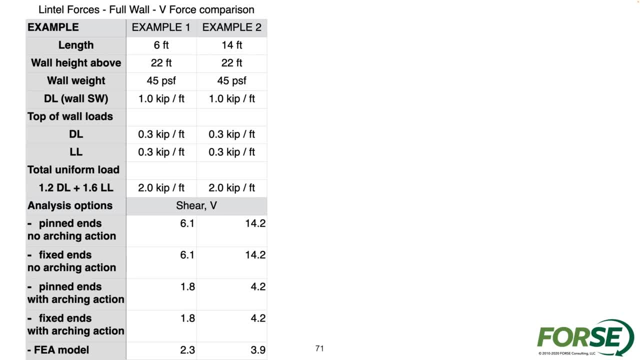 And then what I do is I compare those different simple hand calculations to the actual results that I got from the finite element analysis. So I think that's pretty interesting. You can see that the finite element analysis confirms similar to the hand calcs for both examples. 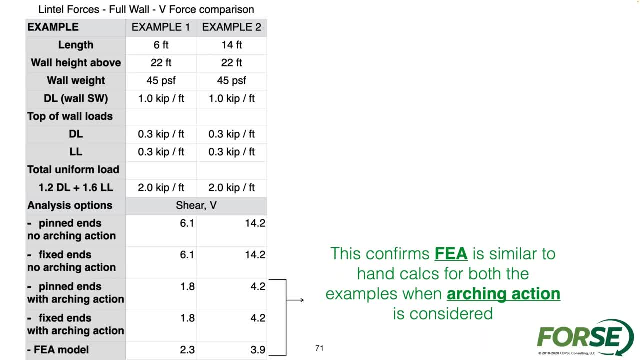 when considering arching action, which makes a ton of sense. I mean they should be very similar. It's really saying that, Yeah, You know that load is just going to be the load local to the opening, which is going to be similar. 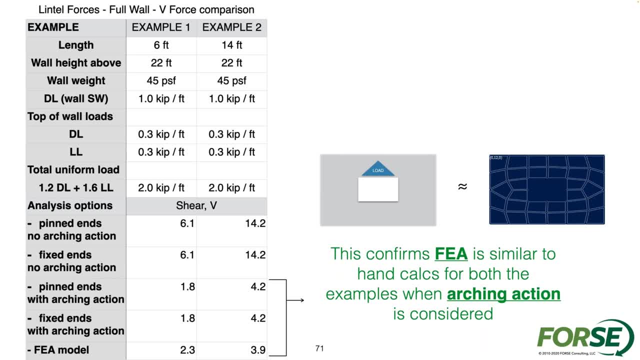 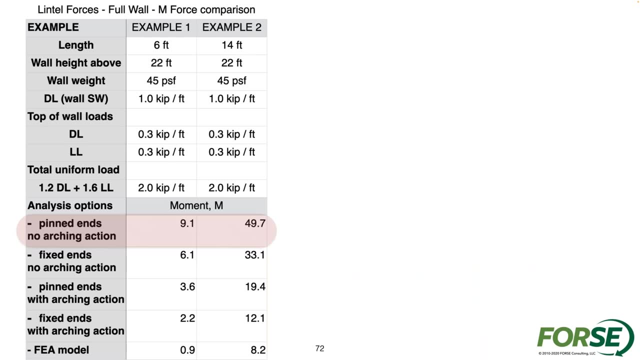 to the finite element analysis result. A stark contrast between that pinned end and the finite element analysis, right? Well, we have far higher forces at the end. So that was looking at the shear, If I switch over to looking at the moment. 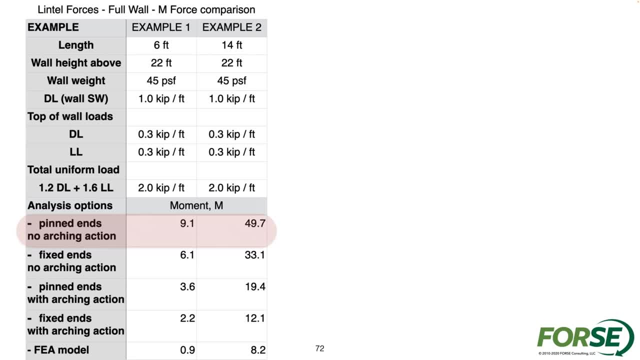 kind of the similar things. if I have a pinned ends and fixed ends, it's going to change the moment demand. It's going to be similar to the finite element analysis model And then obviously, the longer span you know, the finite element analysis model really does. 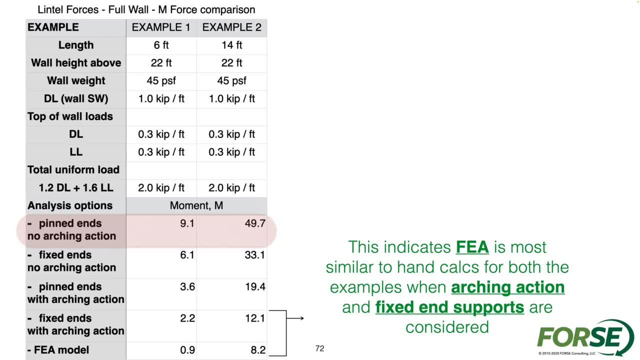 again compare very well to the fixed ends with arching action. So now we're kind of tumbling down to: yeah, that makes sense, That's going to be similar to the finite element analysis model And when you have a lintel, that's going to be integral. 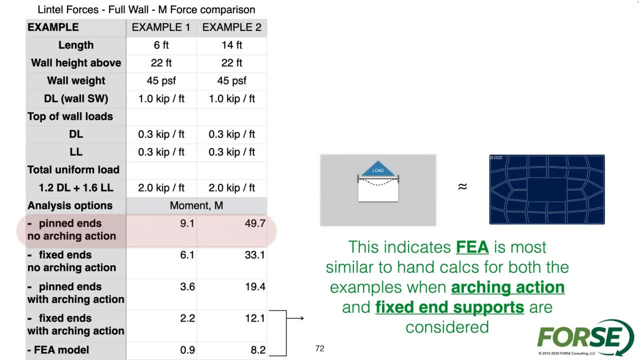 with the wall around it. you know it's going to have reduced load It's going to have. it's going to be tied to the wall around it. It's going to be tied into the wall on each side. It's really going to be kind of in that arena at the bottom. 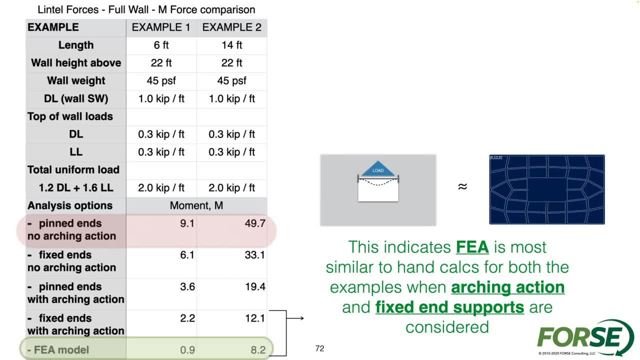 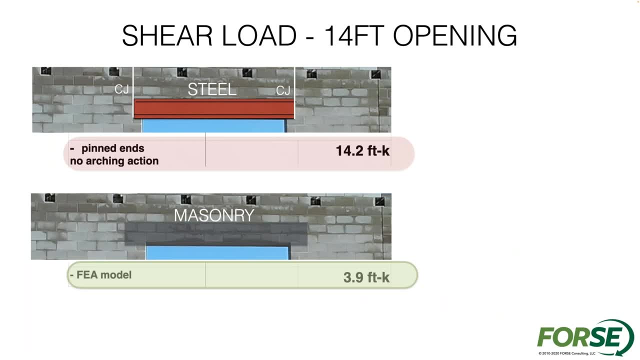 And I keep highlighting the pinned ends: no arching action to the finite element analysis model. Really, the reason that I want to point to this is the fact that this is why the different types of lintels that you use can make a huge difference. 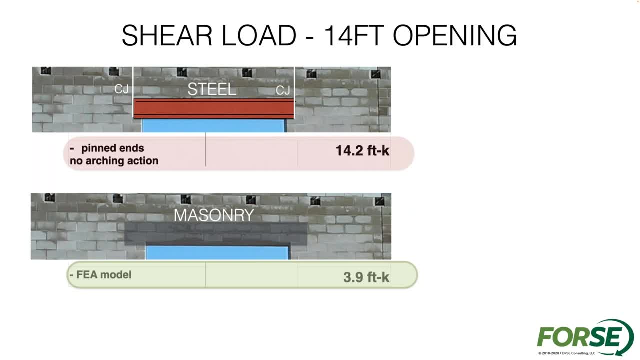 If I have to put in a different type of material, then I usually have to have control joints at each end because that material might move differently or that material is going to be set in there in a way that I might have to allow for some differential movement. 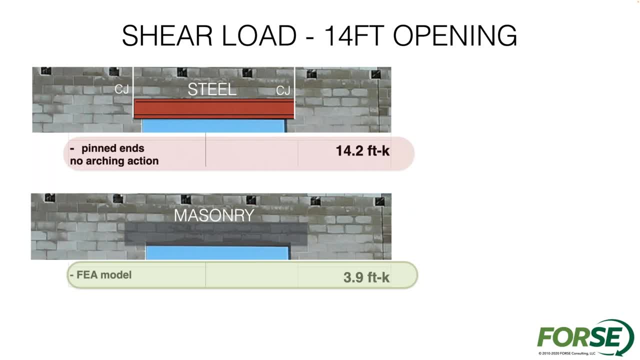 for that element. Just putting those control joints in there really fundamentally changes the load demand that you have the shear and the moment that you have on the lintel. So that's why masonry lintels can generally be designed for a lot less loads. 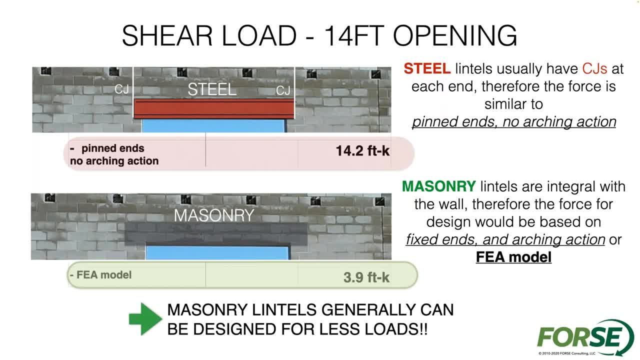 They can really make a lot more sense for the overall design. Yeah, Yeah, structural design of the lintels. So kind of going all the way from software through software to understanding the forces, understanding how those forces compare with hand calculations, and then really kind of seeing why any lintel 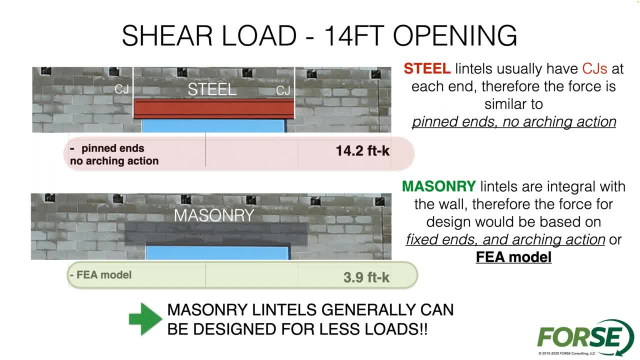 that you can provide. that's gonna be integral with the masonry wall system, is gonna be something that allows for the wall to actually do a lot of the work and it not just all fall on to the lintel for spanning the openings, Which I think is gonna be pretty important. 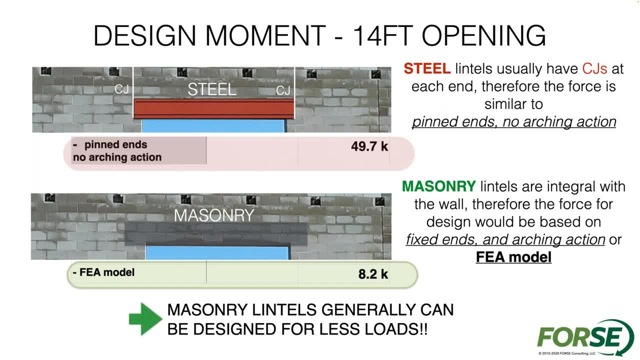 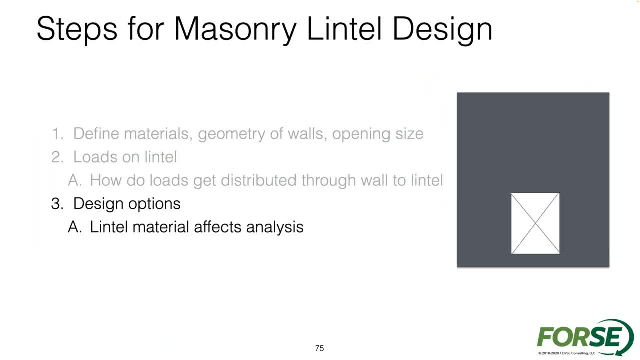 So that leads to looking at different design options, right? So we kind of kicked it off there. I kind of pointed to steel versus masonry, different design options that we have for lintels. The lintel material does affect the analysis, just because it gives you different options. 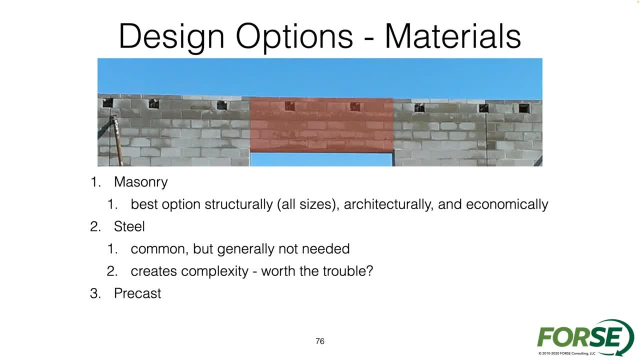 for how you can detail what you have to do with those areas next to the openings. Steel masonry is gonna be, I think, the best option: structurally, architecturally, economically, I mean from like a building maintenance perspective. it really doesn't require any further maintenance. 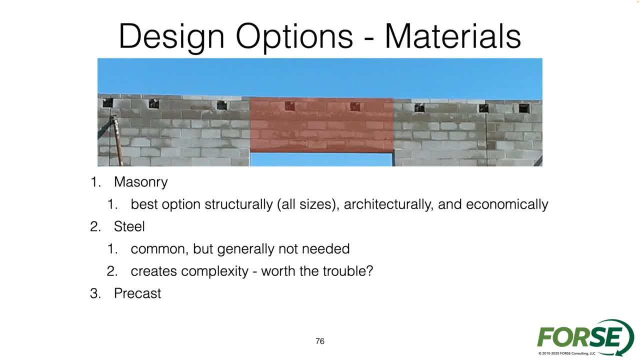 when you have a masonry lintel, When you have a steel lintel. those are common, which we recognize, but they are something that was added to a masonry wall at a different time and different age, when we had maybe a lot of unreinforced masonry. 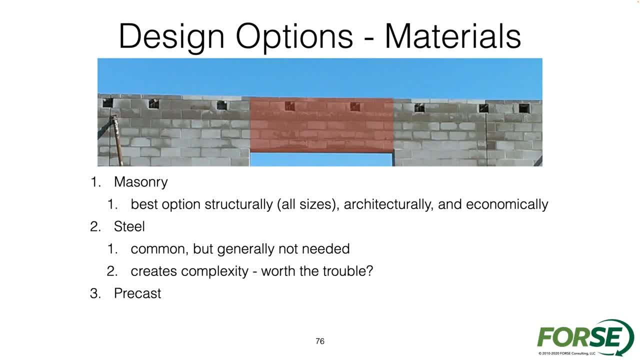 that we were considering. So steel and some of the demands of putting a steel lintel led to similar details that you would have with an unreinforced masonry wall. Right now, with a reinforced walls being more common, I think steel just creates complexity. 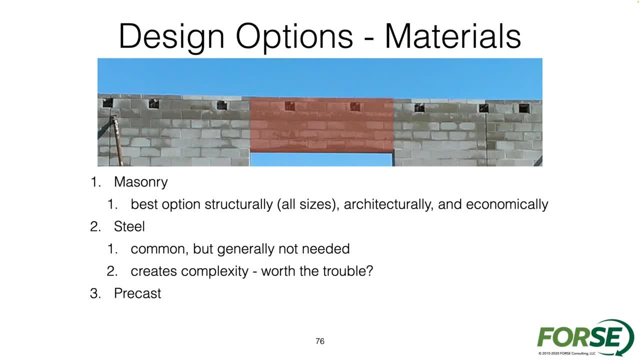 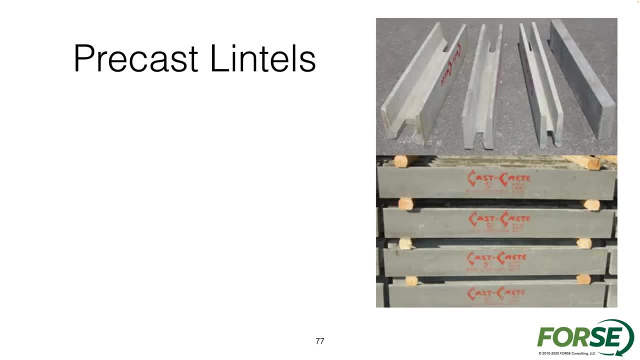 and I don't think it's worth the trouble. I think it really does cause a lot of problems that we don't necessarily want to have with a masonry design. Now, third option: there a precast, and maybe we'll start with that in terms of looking. 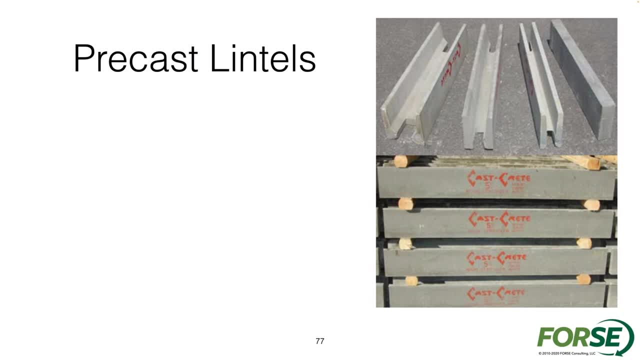 at these different options. Precast lintels: these are lintels that just prefabricated concrete. They can be in the shape of a U, which, and you know. precast lintels: these are lintels that just prefabricated concrete. 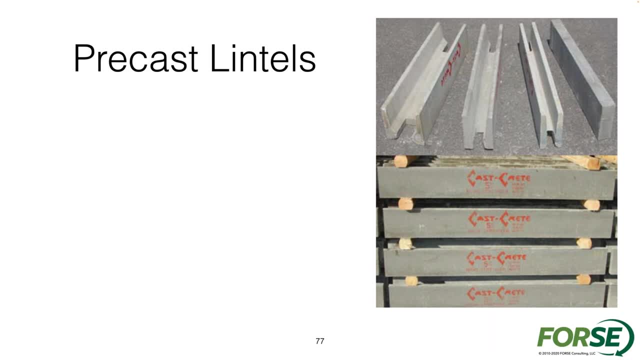 They can be in the shape of a U, which, and you know, you can see the end reliefs being in there, So you can reinforce the masonry the same way that you would if it was a masonry. So these precast lintels, I think, are like extended. 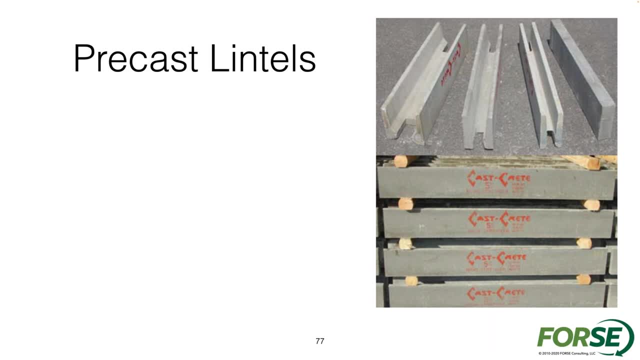 or stretched out U blocks is the way that I used to usually describe them. You know they can be a little bit heavier and you gotta lift them into place- The compatible aesthetic with masonry- but you know they're gonna look a little bit different. 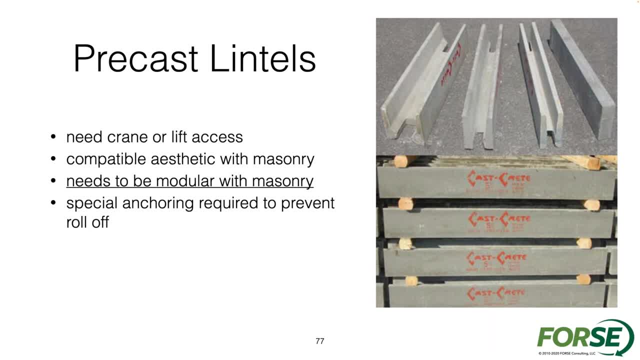 You know it should be modular with masonry. They maybe have to anchor them to prevent them from rolling off. You have a additional coordination item Sometimes. I think there's some mason contractors that have pallets of these like they're just another masonry block. 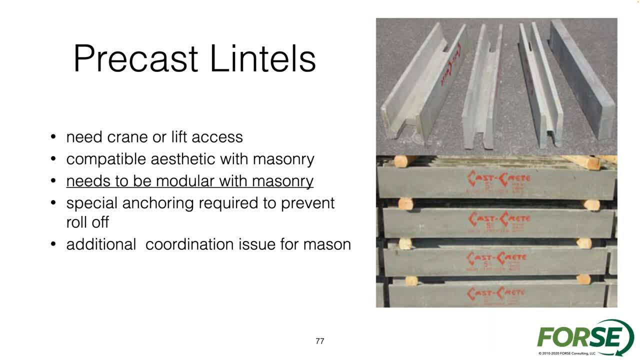 They're just a U block or a very long U block. So precast lintels, I think, are a really really good option, as long as you get the right ones. They're resistant to fire. Could be a potential scheduling issue if they don't have a lot in place. 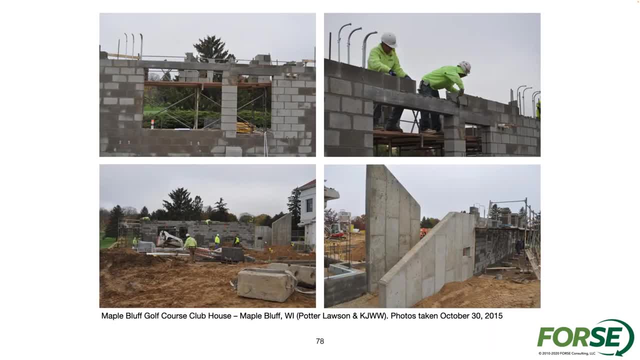 And then here you can see some in a job that I use. They work really, really well. So again, precast can be kind of the similar to masonry, as long as you have the right types of precast masonry lintel. 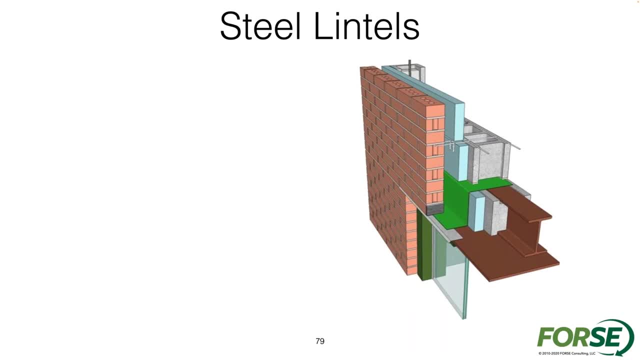 Steel is gonna be the one that I pick on today And again I do a lot of steel design. I like steel. steel is a fantastic material. It's just using the different materials within the same wall plane can create a lot of potential problems. 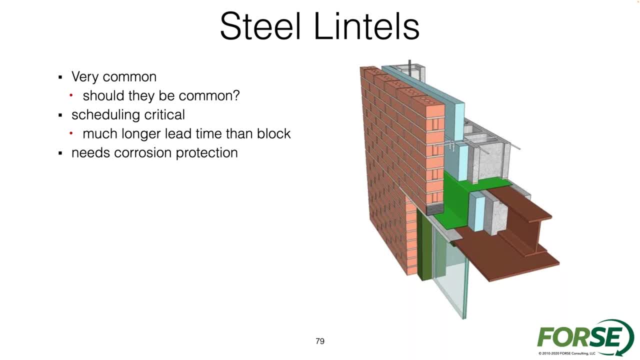 So they're very common. Should they be. they're scheduling critical. There's usually gonna be a lot more lead time than a block. They need some corrosion protection, flashing treatment. There's bearing plates that are often required. Steel is not resistant to fire. 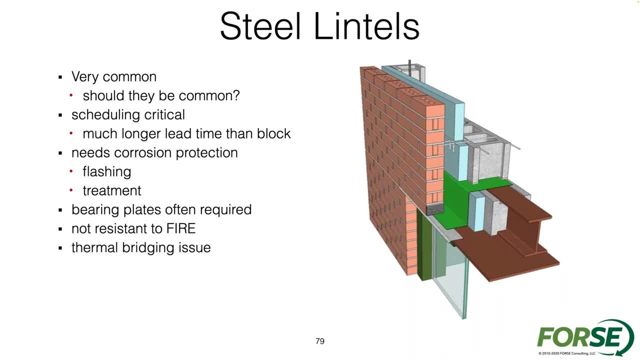 Obviously we need to somehow protect it in some way. We have a thermal bridging issue that we create when we use steel lintels. It's used as shoring, but it's usually more common. When I talk about thermal bridging, a lot of times people want to talk about the architecture. 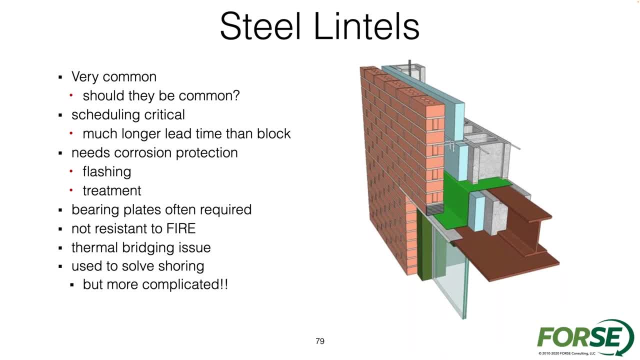 The architectural issue of thermal bridging and how the cold from the outside gets to the inside. We have that thermal bridge. When I think about thermal bridging, I think about, well, if the cold can get from the outside to the end. 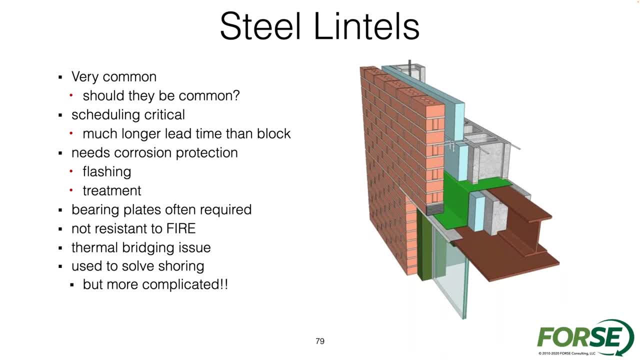 then it's going through a material that changes temperature more quickly than everything around it. So when I put in a steel lintel like this and I have a thermal bridge, I have a steel lintel that's gonna be shrinking much more quickly than the wall around it. 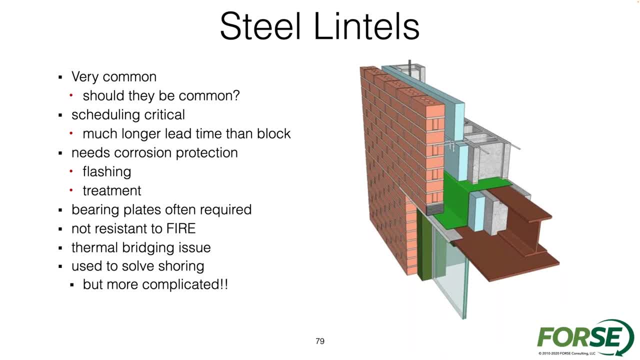 So that's gonna put some- I don't know, I don't know Some internal forces into that wall that are gonna be forces that I don't necessarily want on that wall. that can cause a lot of problems for that wall. So steel lintels- sometimes the way that people 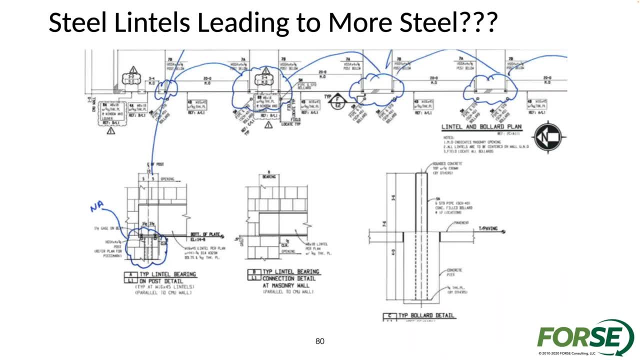 are resolving them is put in steel lintels and then, instead of having to deal with it, putting in steel columns. now we're cutting masonry everywhere. Now we're creating more problems, not less. So steel columns to support steel lintels is not a good solution. 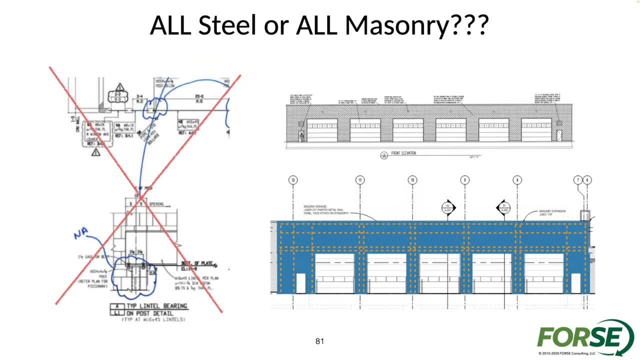 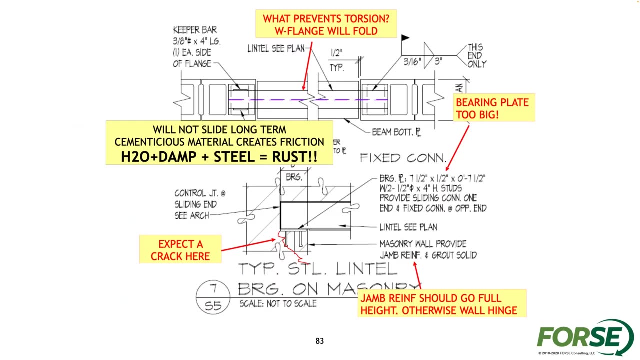 Similar. instead of the steel lintels and steel columns and all masonry, a kind of continuous lintel option is gonna be much better structurally, architecturally and again from a building maintenance perspective. So other things that we wanna point to with steel. 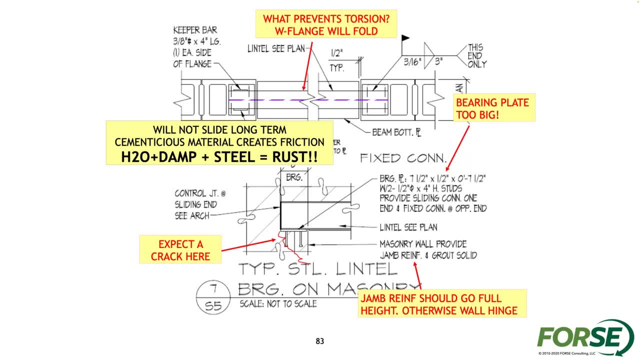 looking at, where are you gonna expect cracks? The most common cracks that I see within masonry are gonna be when steel lintels are used and the bearing, that compromise bearing crack, which doesn't sound good, It sounds concerning and it is concerning. 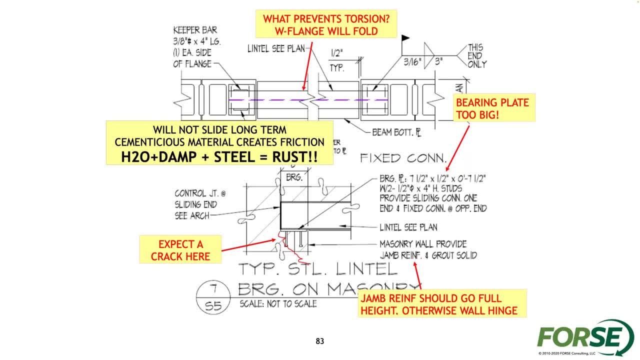 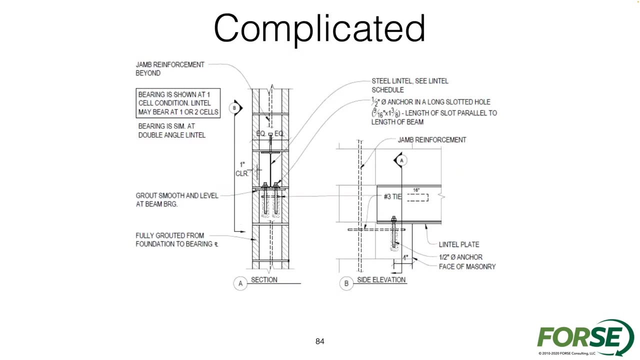 This is gonna be the most common crack that I see within masonry Bearing plates being too large and being exposed and rust can be an issue. Wide flanges twisting and having some rotational movement is also gonna be a concern. So all the things that we have to really kind of think about. 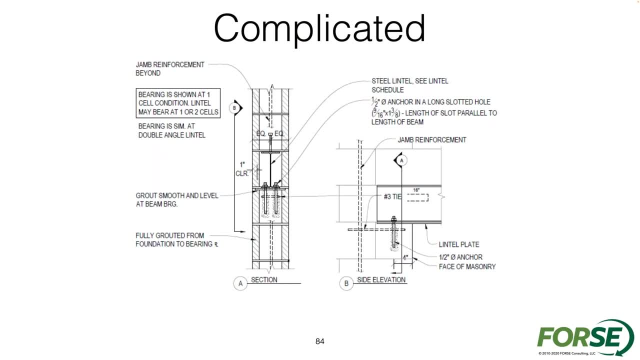 We can put in horizontal reinforcement. So if you look at the steel, the lintel that's in there, hairpin horizontal reinforcement bar is something that can be used and I've used it before to prevent cracks from occurring In a situation like this. 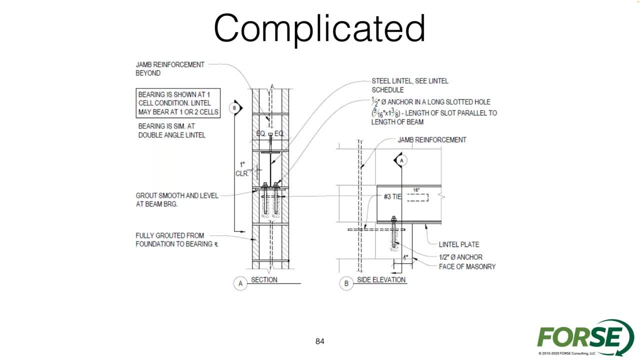 sometimes steel is needed as this floor beam and it's landing on a wall. You have a bearing condition on a masonry wall with a steel beam sitting on it. A variety of times when we have steel that interacts with masonry, we need to think about some of these things. 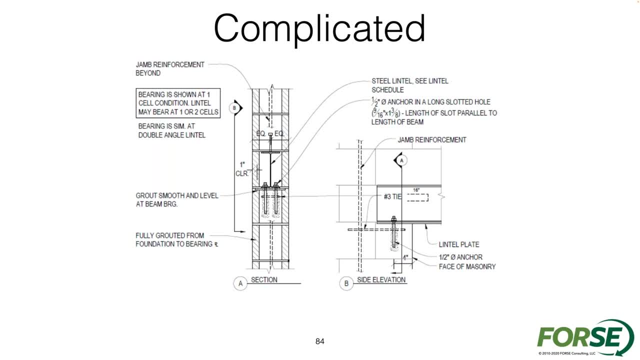 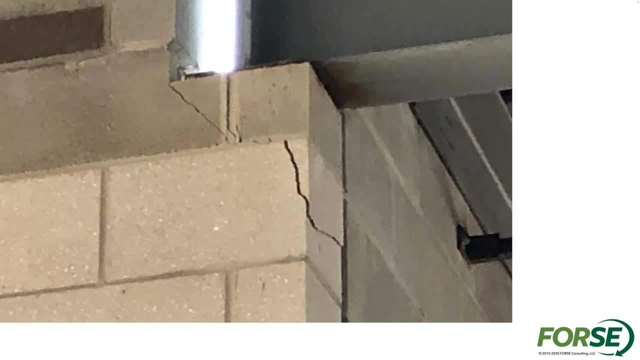 making sure that that steel can move relative to the masonry and not cause further issues, Because otherwise we just have this crack or this crack or this crack. I mean it's just those compromised bearing cracks. They're certainly concerning when we see them. 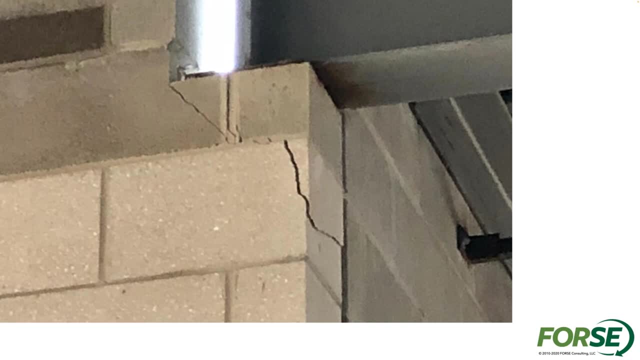 and we definitely know that there's things that are moving there and we have a lot of structural concerns. So now we have to shore it up somehow. We have to replace that masonry, We have to maybe break it out, make it solid. 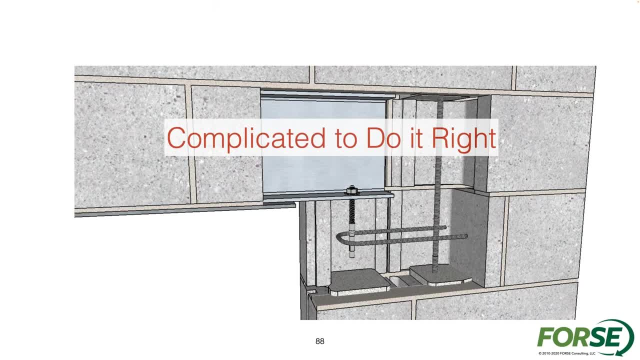 We have to do something with it. It's complicated to do it right. I mean, those hairpins are something that do solve the problem. They prevent that crack from occurring. But again, why do we have the steel? there Is the steel necessary. 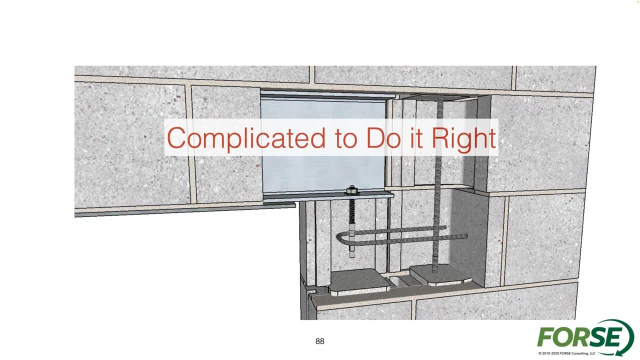 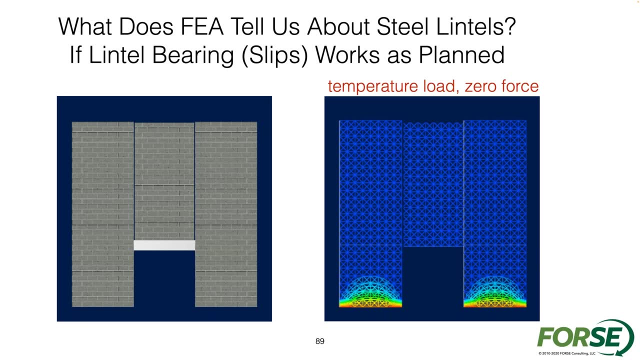 And so on and so forth, Other things that we look about, like why we have that again. maybe a software is a really nice little tool here to see that if I put in a steel lintel so I just model all the different elements. 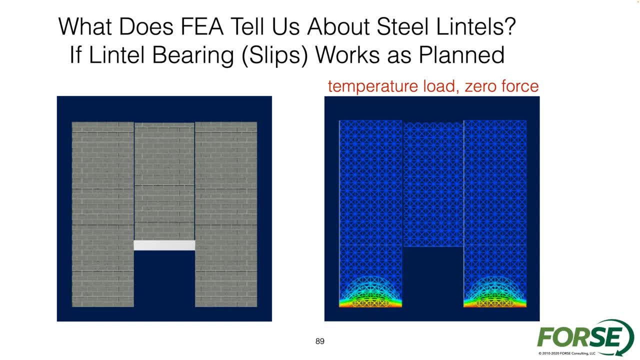 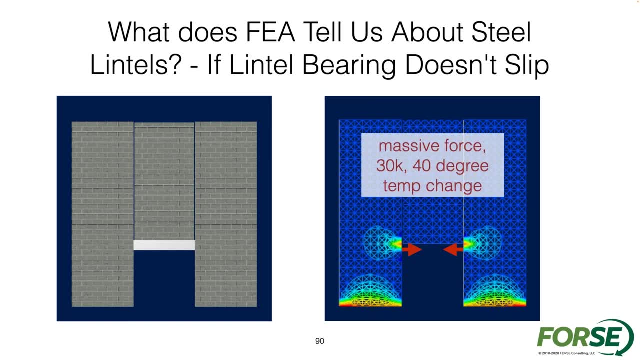 concrete masonry we model in the steel. If I put in a temperature load and everything slips, then it's just fine. If I put in a very simple steel beam, you know, a 40 degree temperature change can cause a 30 kip force to be on those masonry walls. 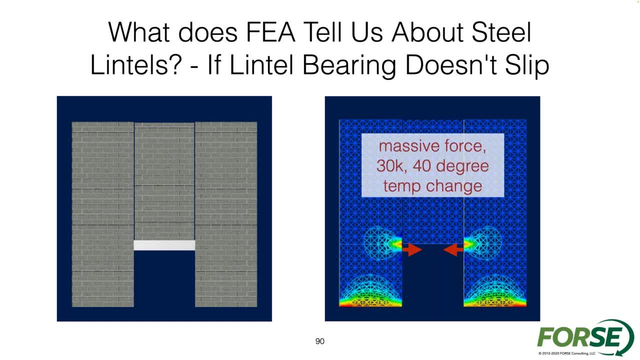 So that's why you can see why those cracks occur. I mean, it's a large force. It's not a lot of movement, but it's a large force because of the stiffness of masonry that's not moving. You know people will ask me well, 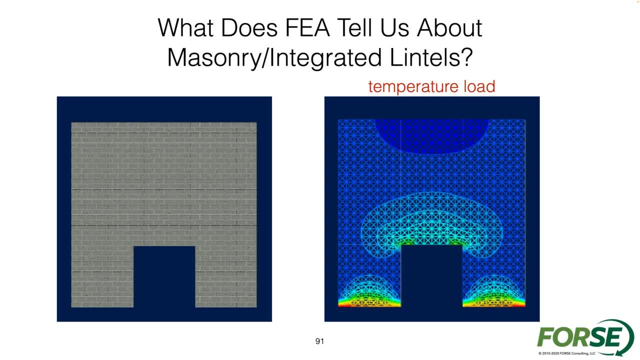 if you have the temperature load and you have masonry, doesn't that also create stresses? Well, absolutely. But those are much more distributed, not nearly the same magnitude, so on and so forth. The other thing is just thinking about the common axial forces. 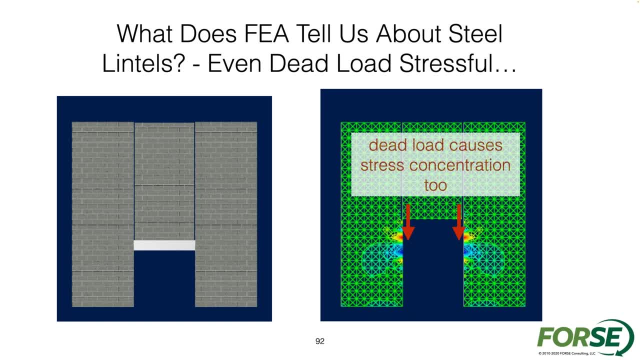 that you have in a wall. when you have a steel lintel, you have limited bearing capacity, which again creates stress or concentrations, which is not necessarily gonna lead to a crack. It's not necessarily gonna be, but you can already see that. 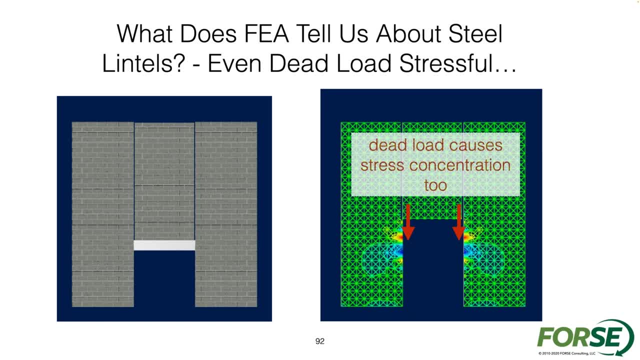 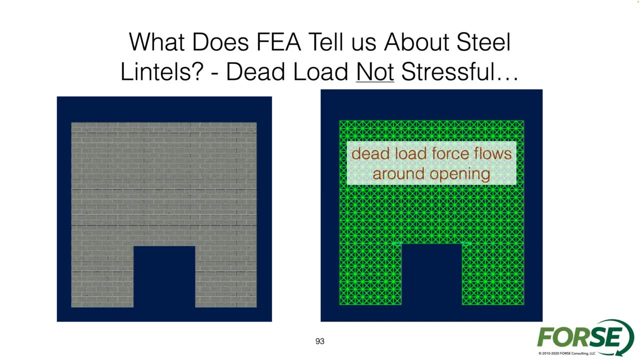 the masonry is stressed in that area. Add a temperature load and you're gonna have a recipe for a problem. So again, dead load really doesn't change the stress flow just minimally around those openings. So other things to think about when we have steel. 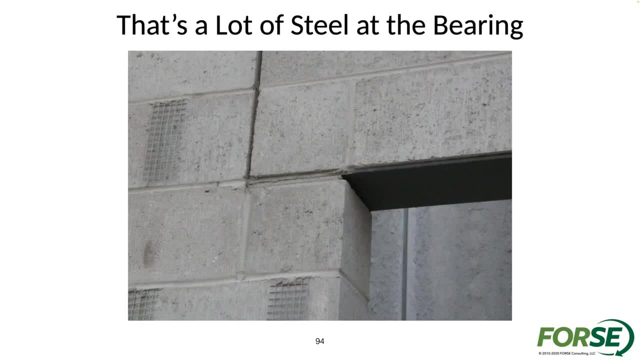 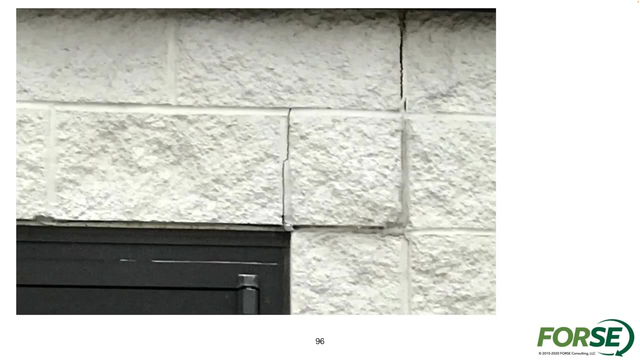 and masonry is making sure that those bearing plates are okay. We're gonna talk about that a little bit in one of the next sections when we look at connecting connections within masonry or to masonry. Bearing plates that can get too large can also cause plenty of cracks and rust cracking to occur. 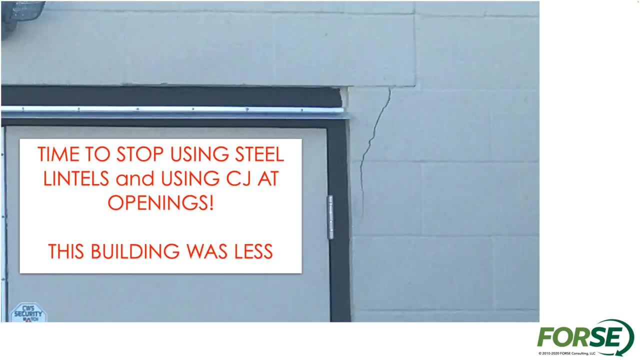 We wanna make sure that we avoid those things at all costs. So, again, let's stop using different material within a masonry wall. You know, this building was, yeah, like I said, less than a few months old, and we already saw that crack occurring. 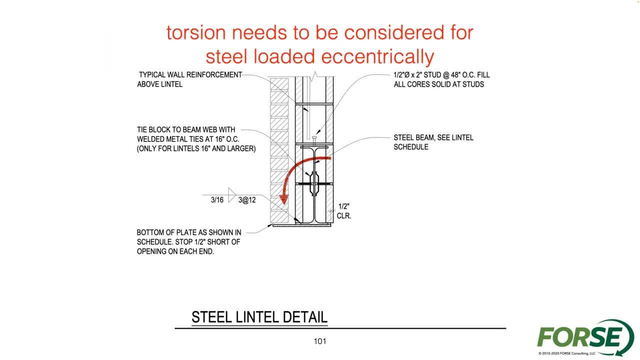 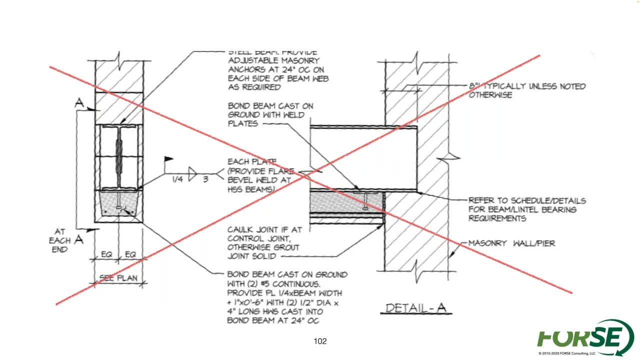 Yeah, we talked about rotational stiffness. We talked about a lot of different options that cause problems here. One of the other things that I've seen people do is trying to resolve some of these issues, but trying to be creative. They want it to look like masonry underneath. 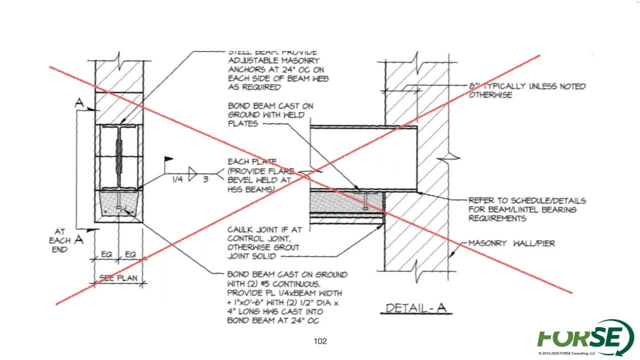 but they wanna use the steel. Maybe, again, they're just thinking about this in terms of like prefabrication and not having. so they'll prefabricate like a masonry and then they'll put a steel beam on top of it. 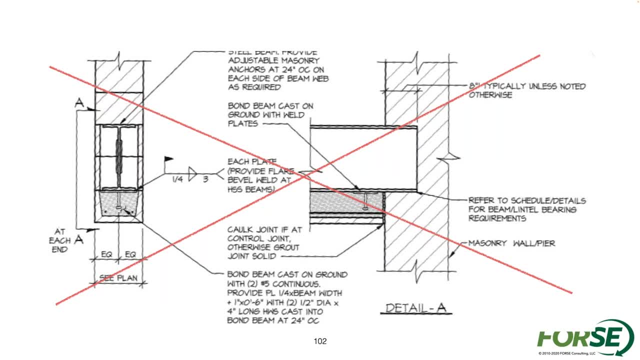 span the opening Again. that's cute but it's not needed. You could prefabricate that- all The masonry, lintel. if you have limited depth, think about stirrups that you can use and add to be able to span that opening. 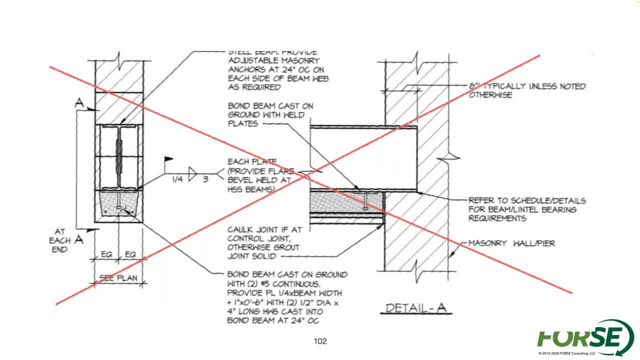 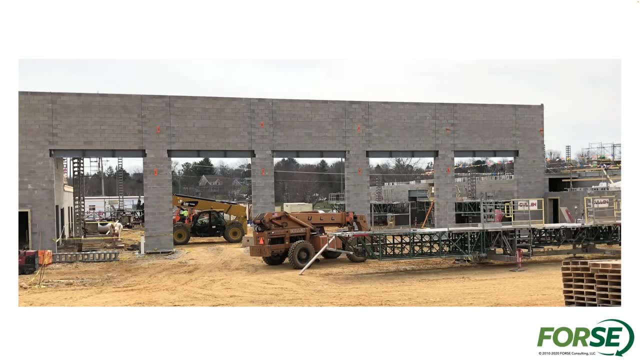 which can work very, very well. So other complications that we have here with the masonry steel beams that are used, what to do with the jam reinforcement Sometimes when we have these walls, when we have these jams that we are trying to look at, 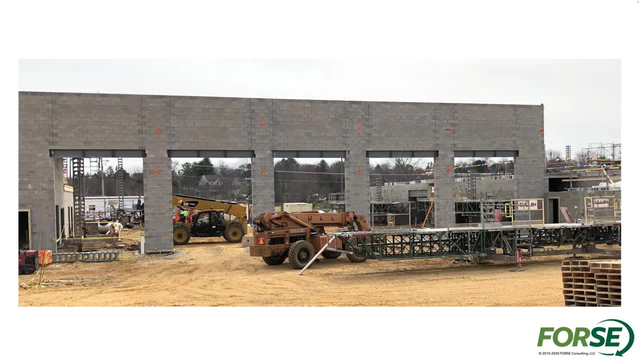 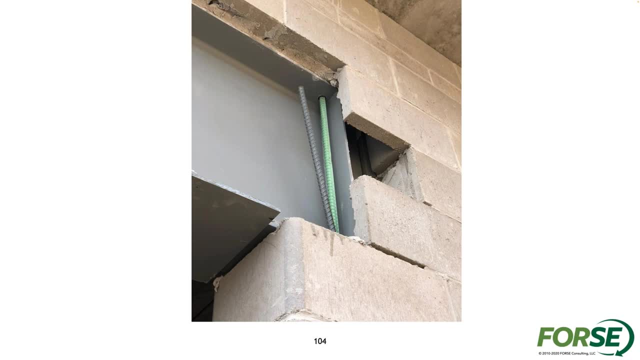 and think about trying to make sure that we don't lose too much of the section due to the lintels If I look a little bit closer at some of the bearing seats of the steel lintels trying to keep the reinforcement continuous at this location. 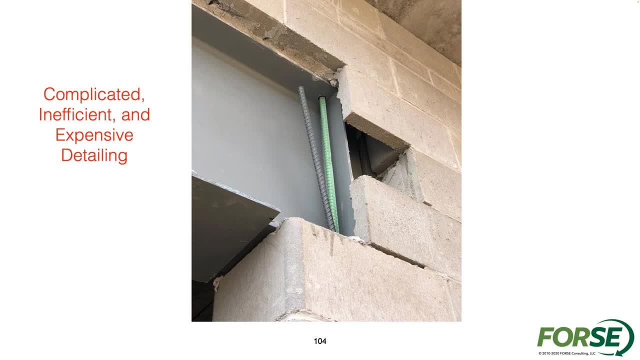 so that we don't lose all the depth of it can be really really complicated. Putting all these parts and pieces together again is something that the masons will do, contractors can do, but it does really, really, really really. 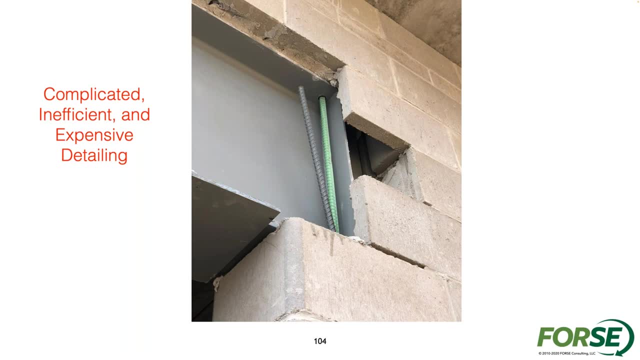 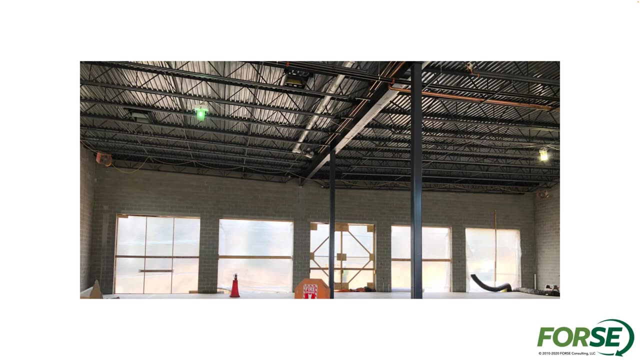 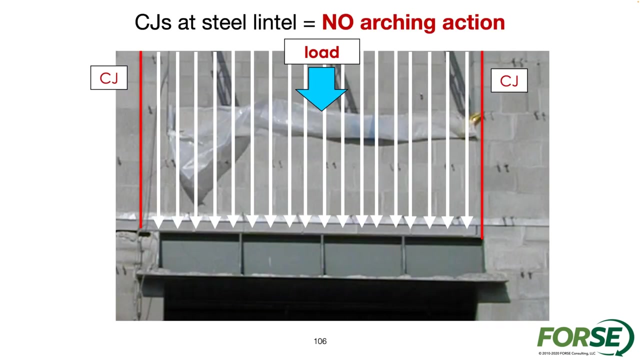 add a lot of complication to this design. So, again, if we have something that's continuous, we have no control joints. we have much cleaner joints. we have a very clean and better performing design. You know. the other thing about steel is again: 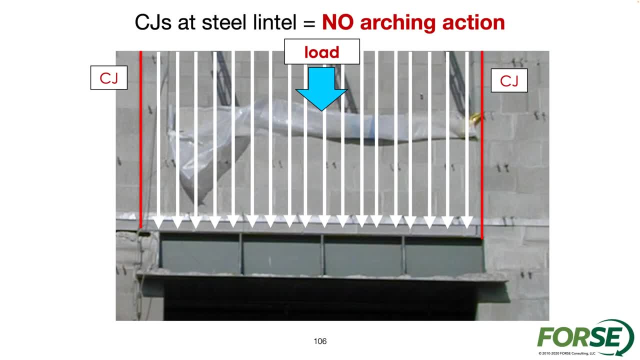 I pointed to this a little bit earlier when I looked at verifying the forces that we have within masonry lintels, but then talking about if I did have no arching action and I don't have the continuity between the lintel. you know that's what steel is. 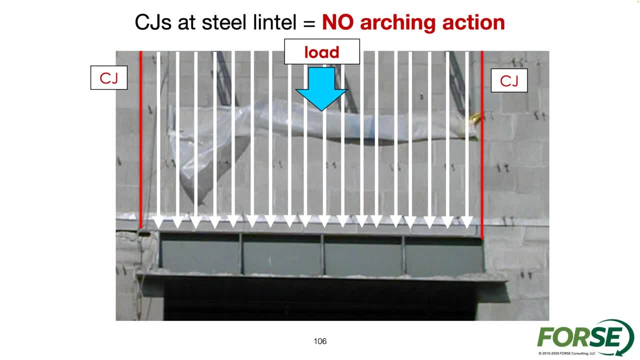 You know, we really do have a steel that we probably are putting control joints on one or probably both sides of the opening, And so then that steel lintel has to take a lot of load, It has to take all the load of the masonry. 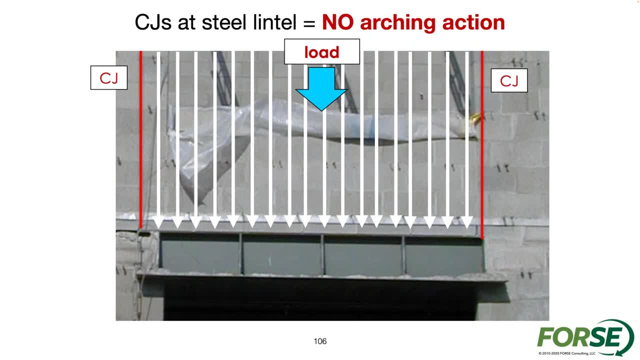 and the roof above it, And it has no positive, negative moment. There's no, really no relief from the for the design of it. You know why. so then I'm going to go back to again: why do we start? 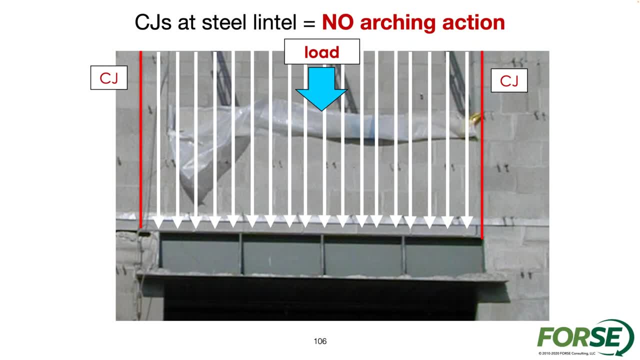 start putting steel in there. if it didn't make sense, Well, control joints in this location in an unreinforced masonry wall. that made sense When we did a lot of walls unreinforced, which again 30,, 40 years ago. 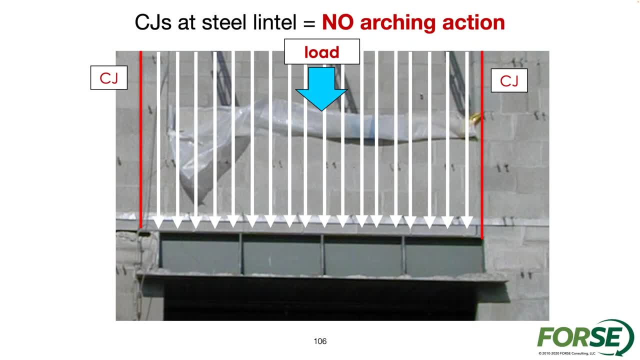 I think we did a lot more of that. this all kind of fit together, Putting those control joints in there, having the thing be unreinforced other than maybe the reinforcement and grout that you'd have below the beam- that would be a very common design. 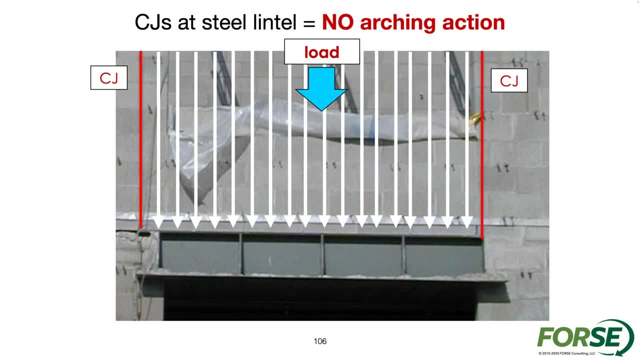 That would be a very common way to do the design. So we put the steel in. we didn't have to deal with the shoring. Contractors were shying away from it anyway. This is kind of what our design was looking at anyway. 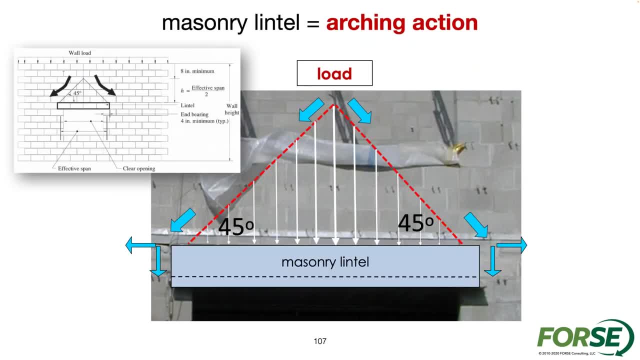 Versus now when we're moving those control joints away. the load on that masonry lintel is pretty minimal. The wall arches around that opening. it really does allow for quite a bit more capacity in the overall system. The masonry lintel doesn't have more capacity. 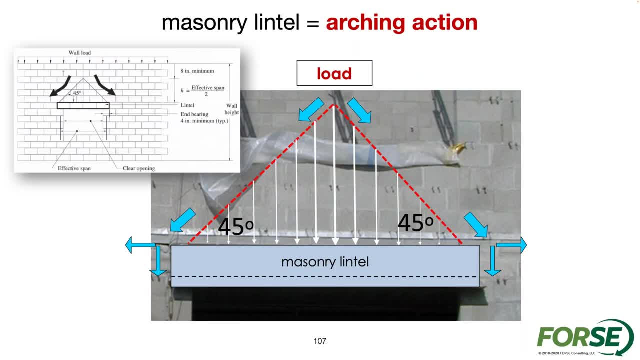 than the steel lintel, The masonry lintel. it just has less demand right, Because of everything that can stay continuous and stay all together, we have a lot less demand. So our demand to capacity ratio, our masonry lintel can do a lot better. 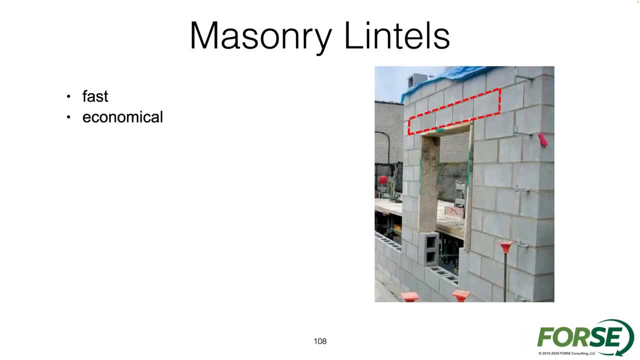 stacked up against the steel. So again, masonry lintels are fast, economical match. the wall moves at the same rate of the wall built in place or prefabricated. Six to 10 feet pretty easily. Longer spans are possible. 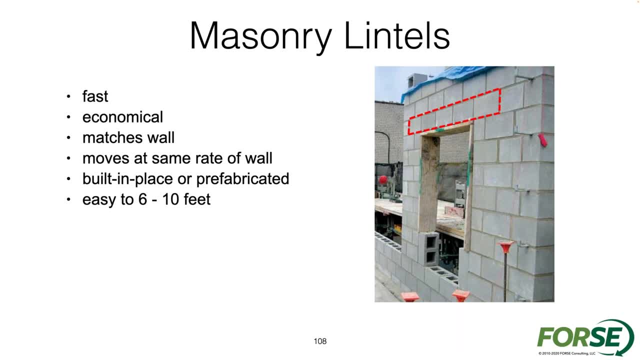 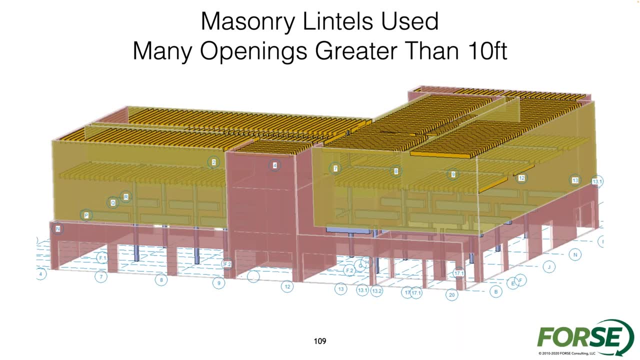 12 feet can be pretty common, But there's really no length restrictions. 20,, 30,, 40, even 50 feet. Design-wise masonry lintels can be used In buildings like this. this is something that with that. 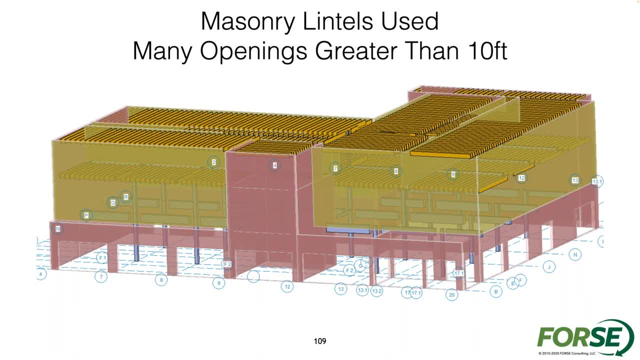 especially with the mixed use buildings. you have some pretty long span open spaces at the first floor of a lot of these structures. Having these long continuous masonry lintels can work really well versus adding in other elements. We really do have to break up that elevation. 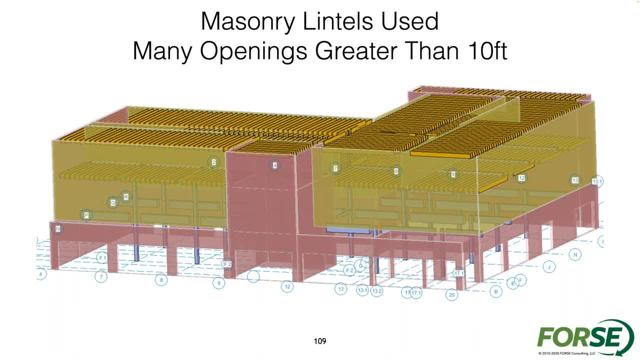 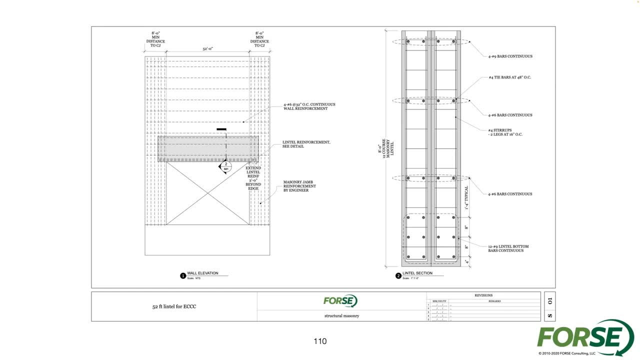 Think about what you're doing. Think about control joints and it really gets pretty complicated pretty quickly. Again, this is a 52-foot long masonry lintel. You look at the cross section. there's a lot of reinforcement in it. 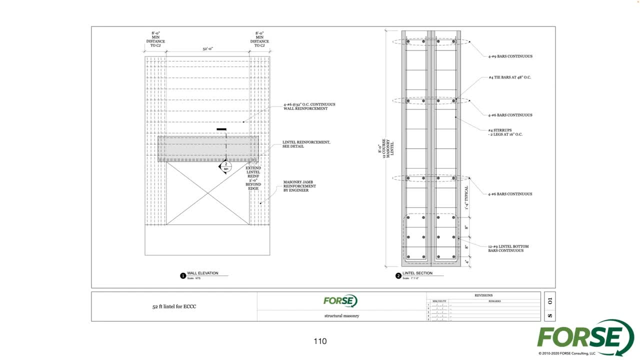 There's a lot that was going on within this lintel. It looked pretty similar to what a concrete beam would look like, And so that it was pretty similar to the concrete beam design. It was kind of the same thing design-wise. So making sure that we think about you know. 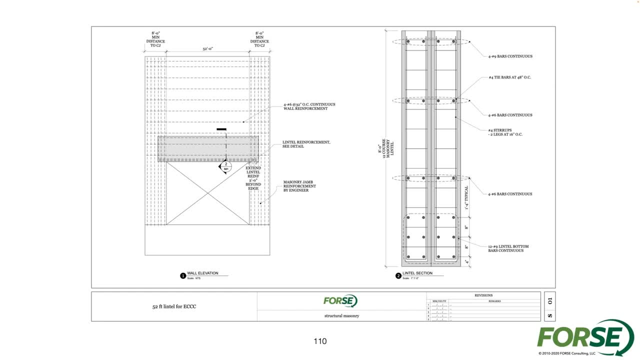 what we're doing with this lintel, So making sure that we think about you know what the potential is. The thing that I think is interesting about this is sometimes people will point to the bigger the opening, the more it makes sense to go to say steel. 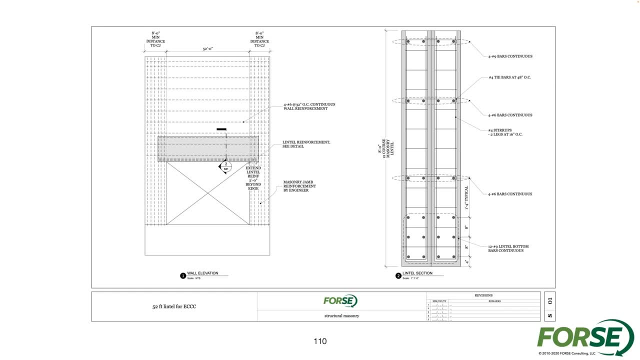 or something with more capacity, It actually makes less sense. The larger the steel section, the more force it's going to put on those bearing seats. The longer the span is, the higher the stress concentration is gonna be. from the gravity, though, When you have the lintel. 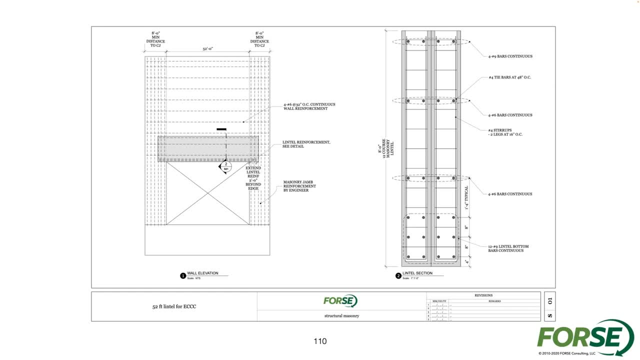 that can be the same material as the wall, that the ability to dissipate the forces you know and have arching action and have the ability for the wall to participate and not just be in an isolated element in an isolated bearing seats. that actually makes more sense the bigger the opening. so things to think about and consider. 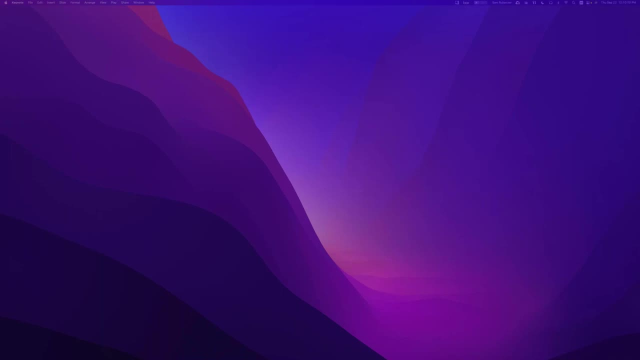 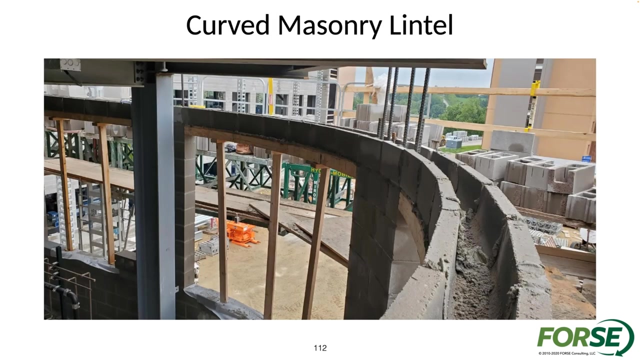 design-wise. oops, sorry about that. if this is what you want to represent with um, we just implemented our mediaге with a size nine zero, that is. uh, you know, suppose we, we, we, we basically just want to say that if things go at your Meredith. 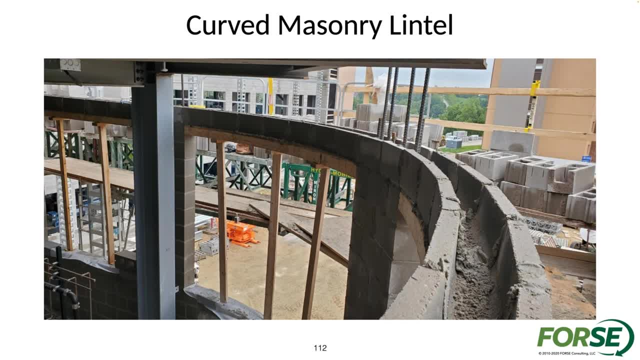 length of five percent. it's a caustic charge, but that becomes a high area of discovery. it's also sorry design-wise. um, it's especially when you reverse carburetion- and this is not so easy at all- can be like concrete, kind of something that you can form. 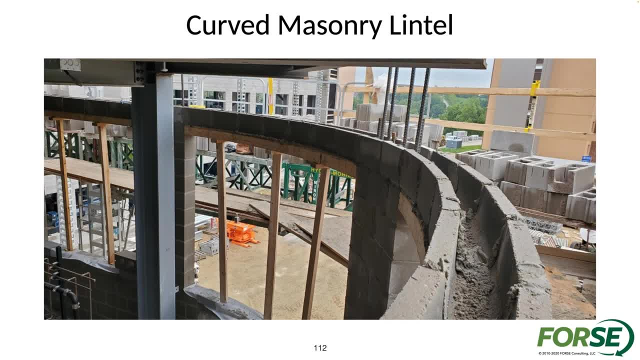 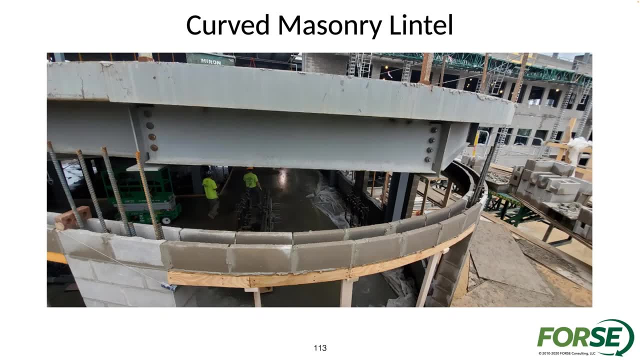 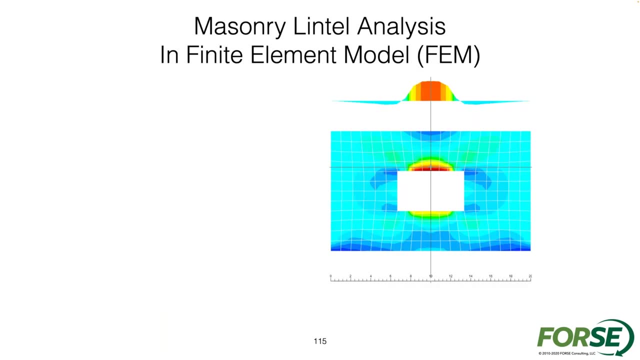 you can reinforce, you can put in a torsional reinforcement into a masonry lintel, be able to have a little more capacity there. So you can see what the masonry lintel looks like here and then here. So again, finite element analysis. 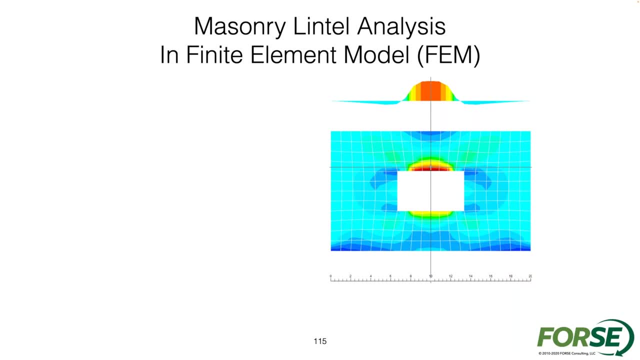 is kind of a pretty big part of this section. We're gonna talk about that more this afternoon for a couple hours on different software programs that are available. Just ability to have the lintel be parts of the overall finite element analysis mesh, not separate entities for the lintel. 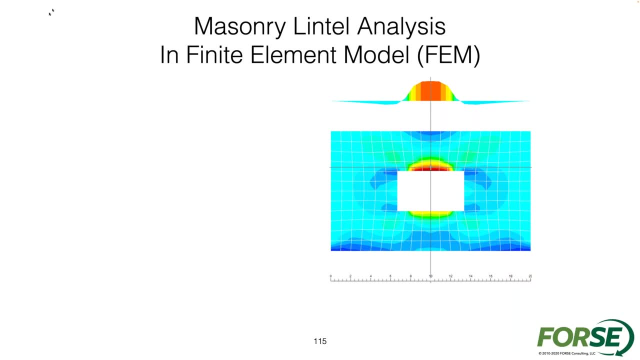 we're not putting in separate pieces, we're actually kind of keeping them in together. So with the finite element analysis it's gonna be comparing pretty closely to the fixed end the beam with arching action. So do you have to have finite element analysis? 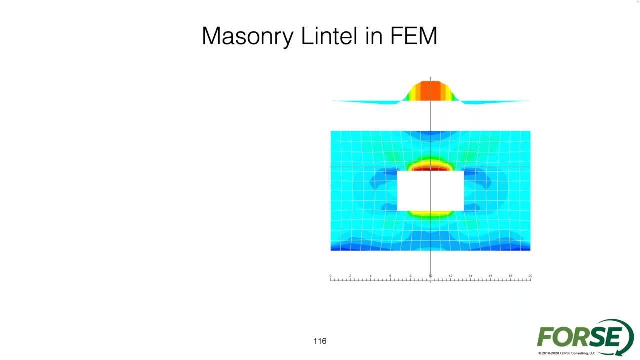 to utilize some of the things that you've learned? Well, you definitely don't. I mean the spreadsheet that I did. the fixed end arching action is really gonna be what we would need in terms of the forces and the stresses that it would need to design. 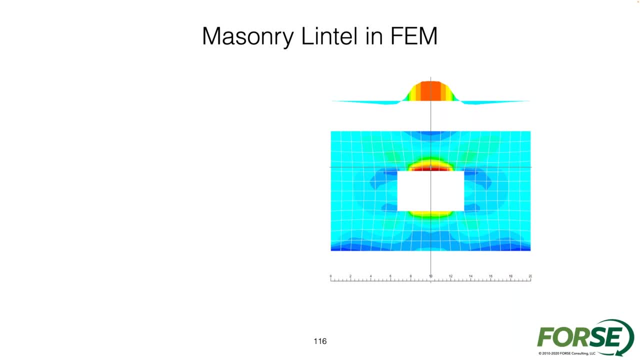 for that masonry lintel. I don't need to have a finite element analysis program but it certainly is helpful. You know shear walls. we really can look at the area above the opening as a coupling beam. It really does pull into our perforated shear wall. 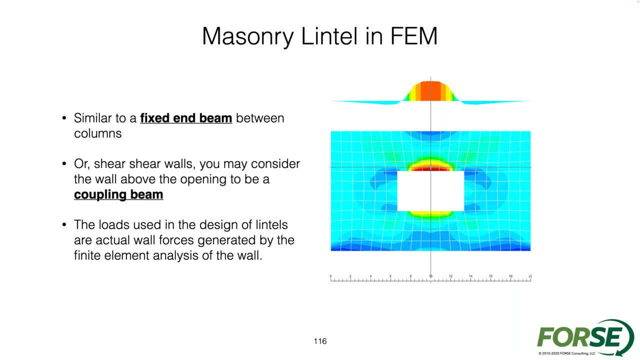 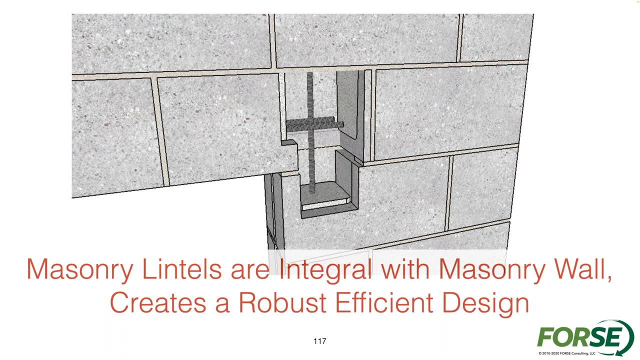 It really does pull into the walls on both sides. So that really is gonna be a very nice design, You know. so masonry and lintels are just gonna be that integral with the rest of the wall, creating what I would call a robust, efficient design condition. 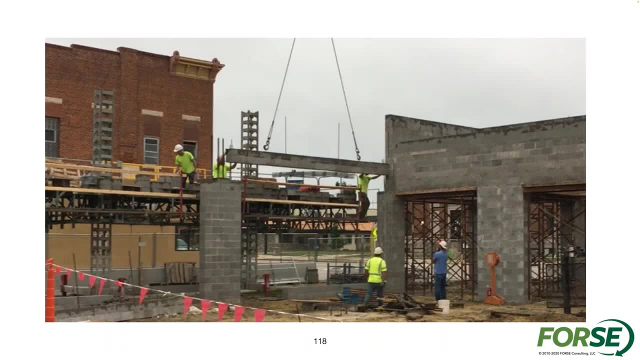 You know, again, shoring can be solved with a head, but having prefabricated masonry lintels that can be lifted and set into place, we need to make sure that we have areas for that vertical steel to be still be continuous. 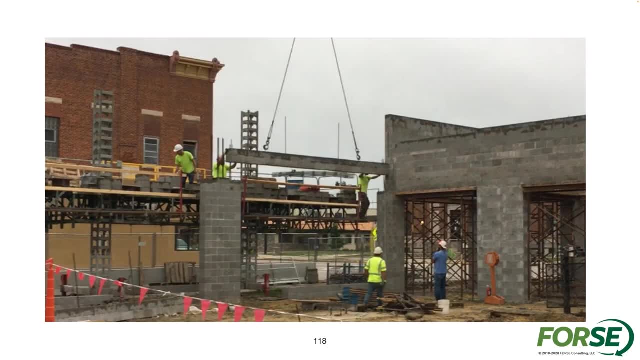 but still something that we can utilize prefabricating. And if I say I have a four or five course lintel, it doesn't mean that I have to prefabricate the whole thing. I can certainly just prefabricate the lower sections of that. lintel set that into place. 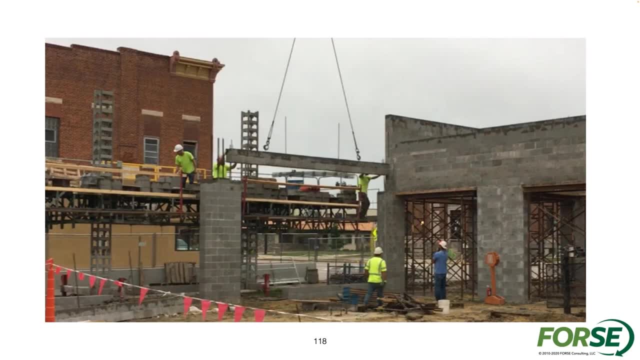 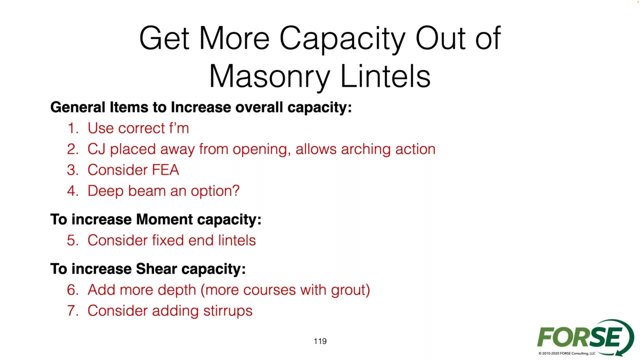 and add the later courses on as we build the rest of the wall. You know, if I look at lintels and how to increase capacity using the right F prime, M is certainly one way to do it. If I wanted to say prefabricate. 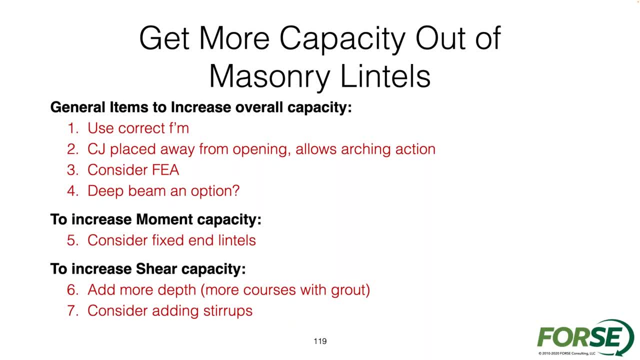 and I wanted to get more design strength. you could certainly even specify a higher strength of masonry for our lintels and then use a higher strength grout. if we needed to do that, That's certainly something that could be placing those control joints away from the openings. 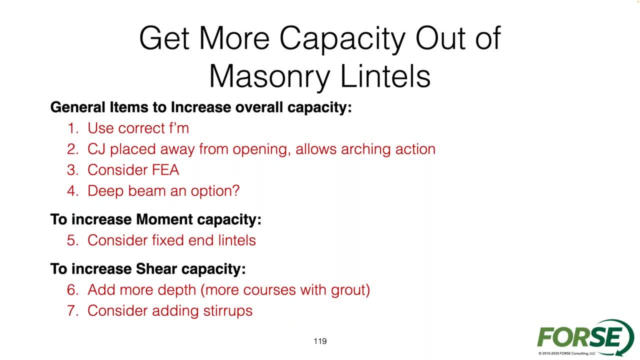 allowing arching action. that's just gonna be a much, much better way of detailing masonry, making sure those control joints are away. Consider finding element analysis, If nothing else just to understand behavior, not much better, but maybe even utilizing it as a tool. 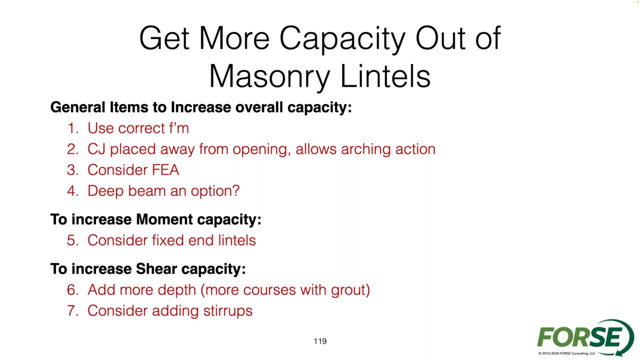 Deep beams could be an option. We talked about that code provision from 2013 where they started looking at deep beam provisions. That's certainly something that works really well to get more capacity for the area of wall that you already do have To increase the moment capacity. 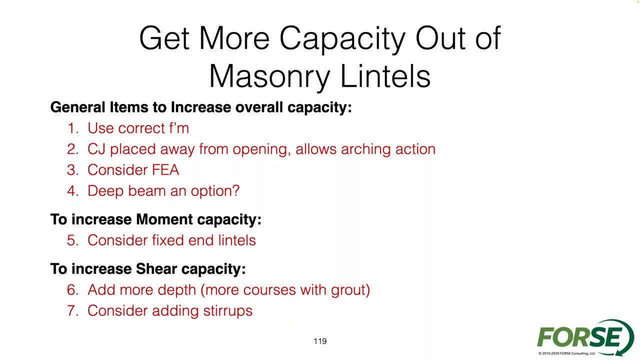 if you had some problems there, considering making sure that you have the fixed end condition. we have top and bottom reinforcement that's utilized for our lintels To increase shear capacity. really adding more depth is gonna be the best way to do it. 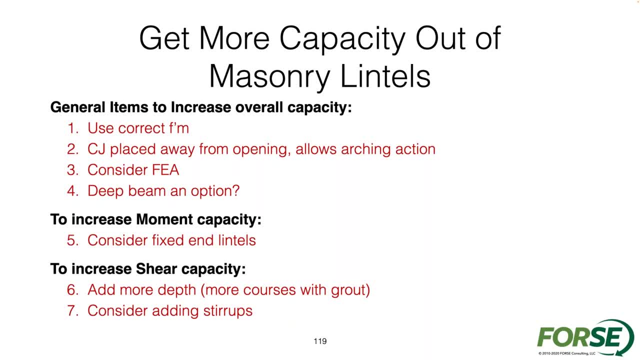 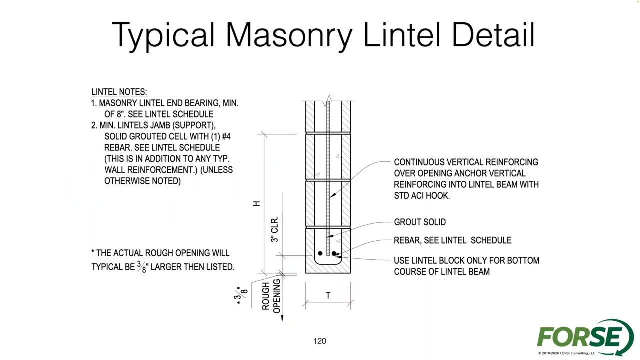 Adding more courses to be included in the shear into the overall lintel depth is gonna be the best way to do it. You can add stirrups. Adding stirrups to masonry should be done with caution, though, You know. our detail could look something like this: 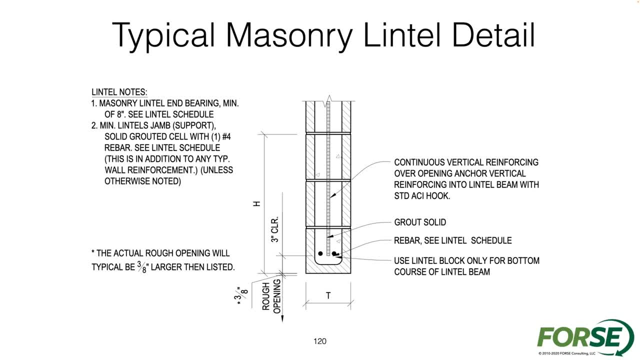 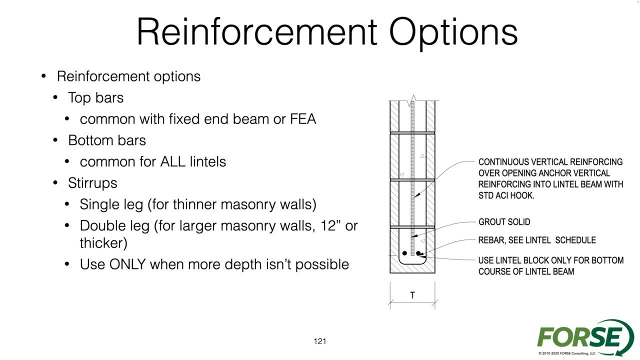 making sure that our reinforcements off of the bottom- you know, maybe this is a pretty straightforward lintel, Like I said: top bars, bottom bars, single leg for thinner masonry walls. double leg stirrups could be added for walls that are 12 inches or thicker. 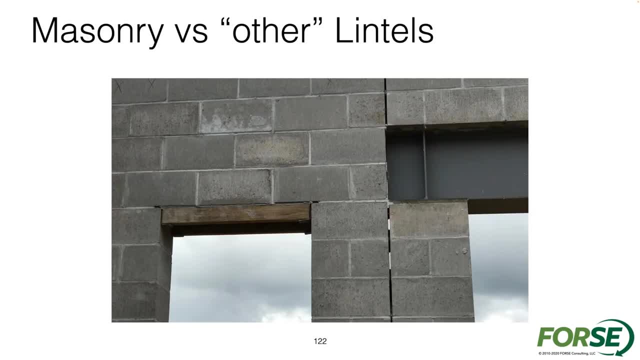 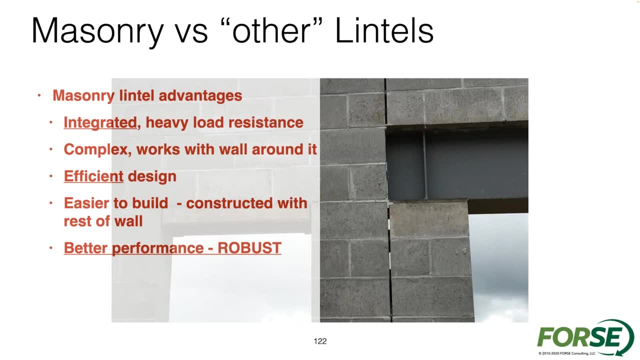 but only use one. more depth is impossible. So the last little bit here on lintels: again, masonry and lintels, the advantages: they're integrated, They have heavy load resistance because they're working with the whole wall. It's complicated in the sense, some senses. 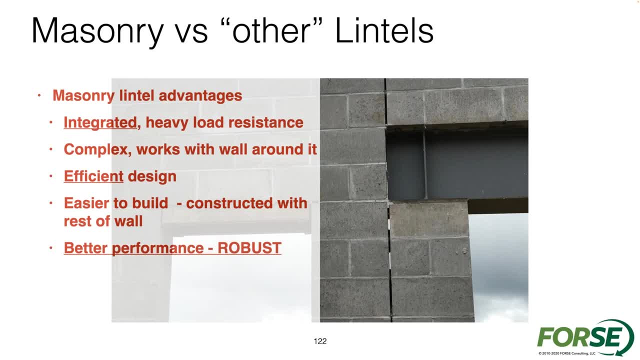 you know, as it works together with the wall around it. So a tool like finite element analysis does help. It's a very efficient design. You can have the best use of materials. if you do allow it to be complex and integrated, It's usually gonna be easier to build, in the sense that it's 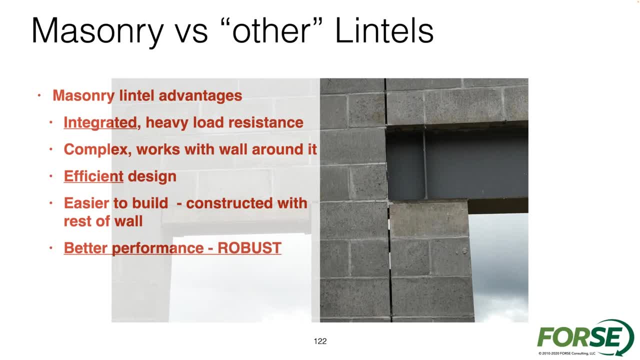 all assembly materials. it's going to be one contractor. It's going to be a lot better performance. It's going to be a lot more robust. It does have a challenge of requiring either prefabbing it or shoring it. You know the other lintel options. 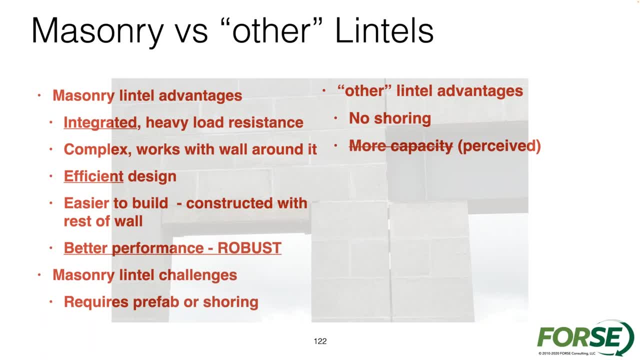 you know it doesn't involve shoring. There's something that you can apply in, but the more capacity is really just perceived. It's not a reality. The actual lintel themselves have a lot higher demands. If I have isolated lintels, 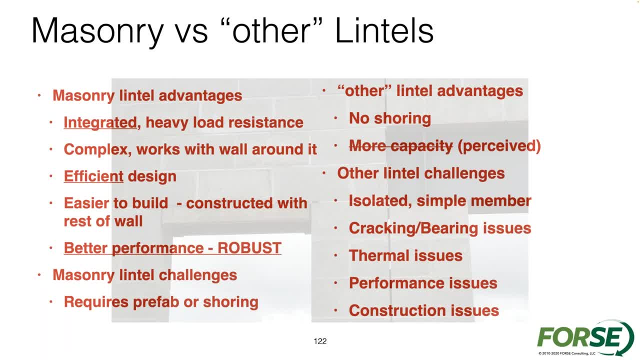 that have a control joint at each end, and I have performance issues, construction issues, thermal issues, a lot of things that I have to think about and consider there. So that kind of wraps up that section. different types of materials that you can use. 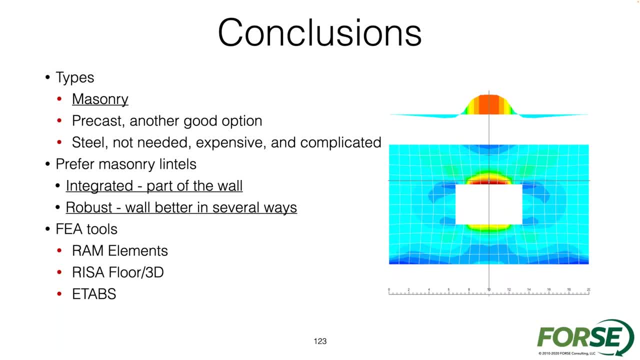 why masonry lintels make more sense, and then some of the different finite element analysis tools that do utilize and design masonry lintels. So that, I think, would wrap it up for the morning. We have several more sections for the afternoon, including the software one. 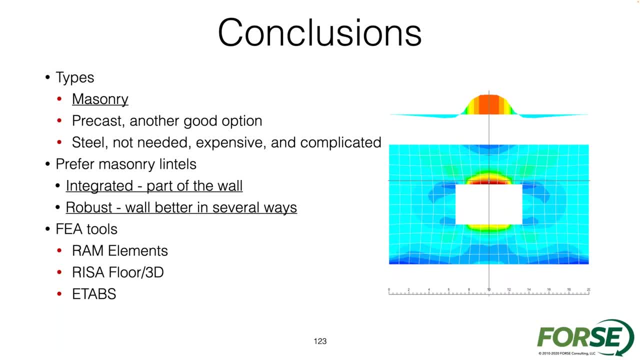 that I've kind of been tipping my hand towards here. We can certainly answer any questions. if you guys have any questions for the next five or 10 minutes- And I don't know if we want to come back at one o'clock or I think one o'clock would certainly be- 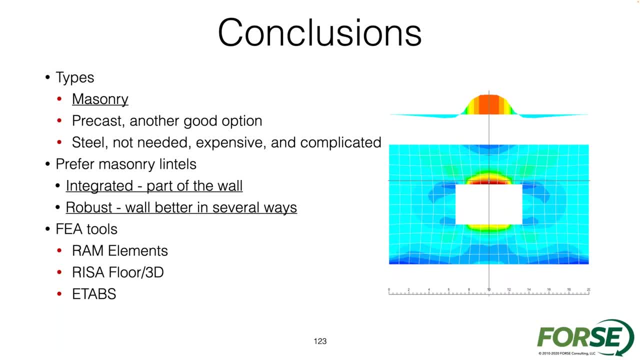 that would make sense. One to four should be plenty of time to get through the rest of the material. So I'm going to hang out here. I'm going to hang out here. I'm going to hang out here for the next five 10 minutes. 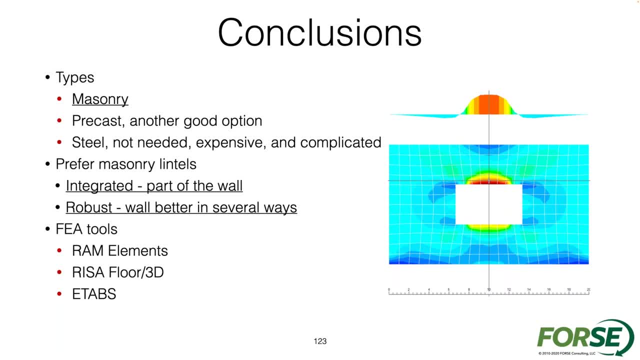 and see if there's any questions that anybody does have. And, Sam, I'm almost positive I heard you answer the question, but there was that. Mr Shaikas asked again: are there the design examples that could be provided? But you did answer that one, right. 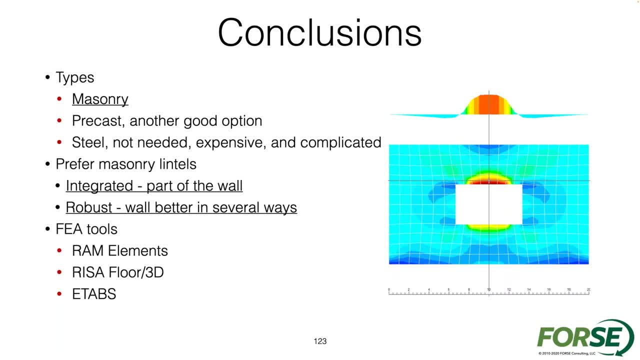 Yeah, so design examples, Yep, yep, yep. I mean again, it's the masonry. designer's guide is really going to be the best tool for that. There's tons of examples that are in there. Certainly had a few examples that are in here. 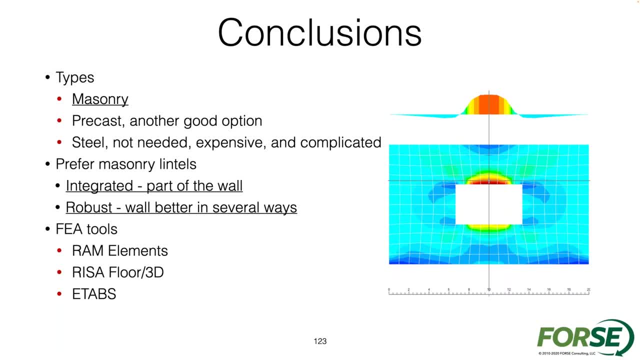 but I didn't want to spend too much time on examples, just trying to cover all the material today. So, yeah, good comment. Like I said, I'm going to go ahead and put my mic on mute. I'll hang out here for the next five, 10 minutes. 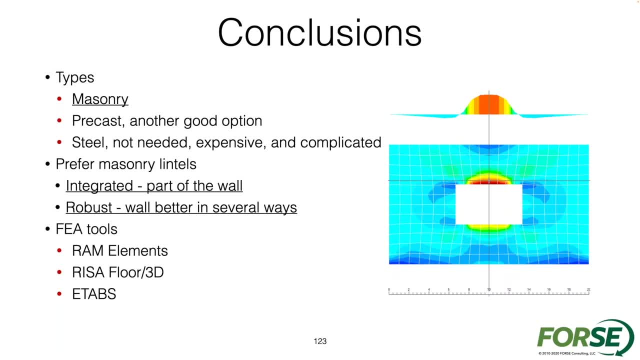 if I see any questions come in. Otherwise, if that's okay, we'll get started back at one o'clock. Yep, that's definitely okay And I'm going to do the same thing. I'll be at my computer If anyone's got any technical questions or issues or something. 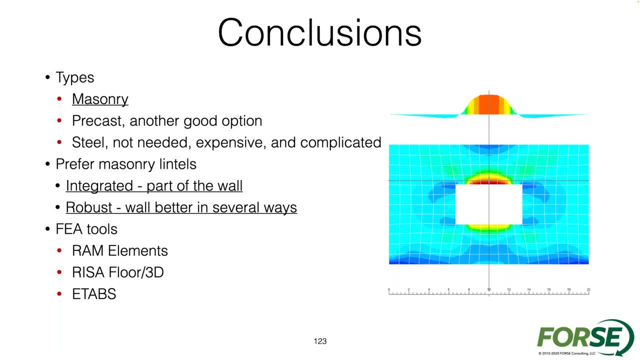 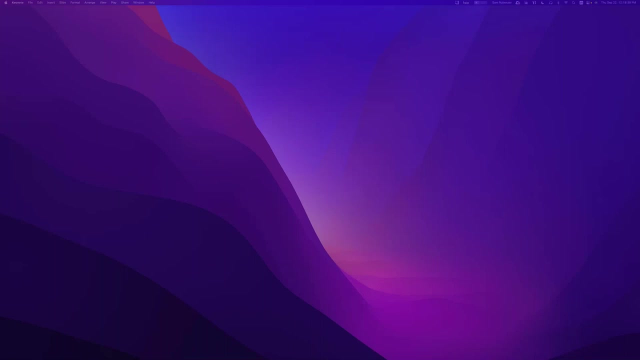 but I'm also going to mute myself and I'll be back at one with everybody else. So thank you so much. I appreciate it. Thank you for listening to this. I hope you had a great day. I hope you enjoyed the video. 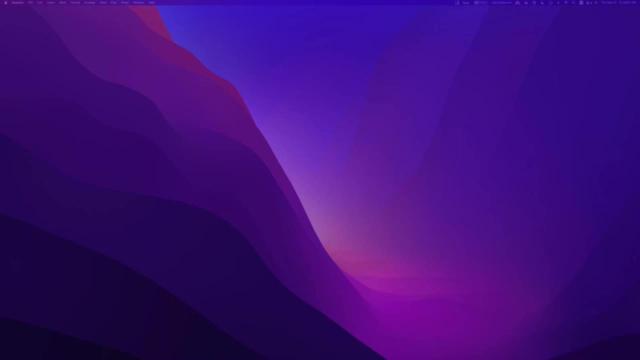 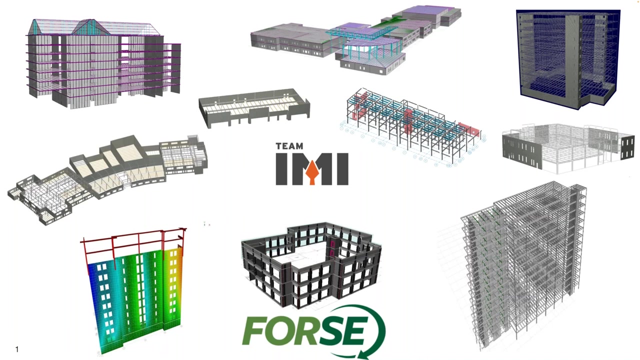 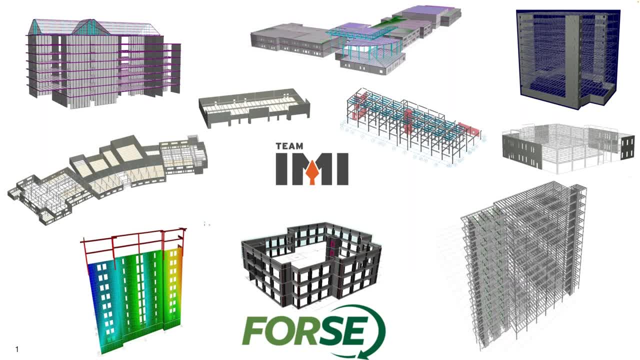 steel plates used at the bottom of the mainstream lentils. it would be um just mainstream. so the lentil blocks, the u blocks, that would be there, um would be the bottom of what you would see. um there's differently, uh detailing, that would have to be considered for how to. 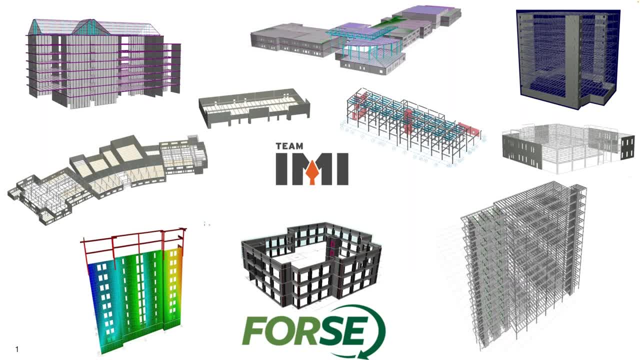 say, especially if you had a cavity wall, how to bridge that gap, um- and we have some information on that- um, bridging that gap with a masonry lintel and, uh, bridging the gap between that and say a veneer, it's something that's certainly you can use. a. 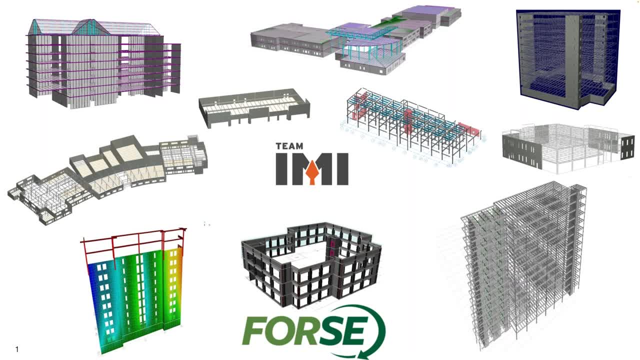 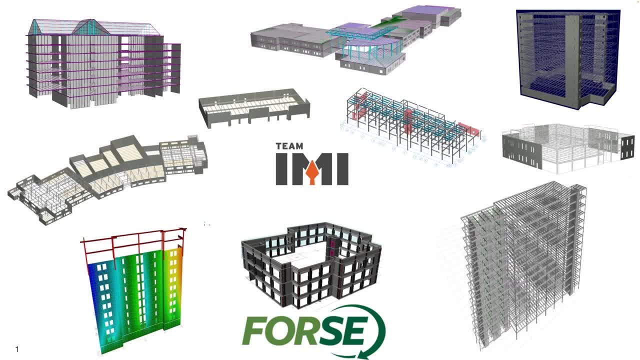 uh, uh, hopefully he's not too loud. so is everybody with us this afternoon? um, i believe so. i know i'm back here, so let me see if it looks like everybody is so excellent, excellent, okay, so why don't i go ahead and get started? um, i did want to just answer the the question that gregory asked right at the end. 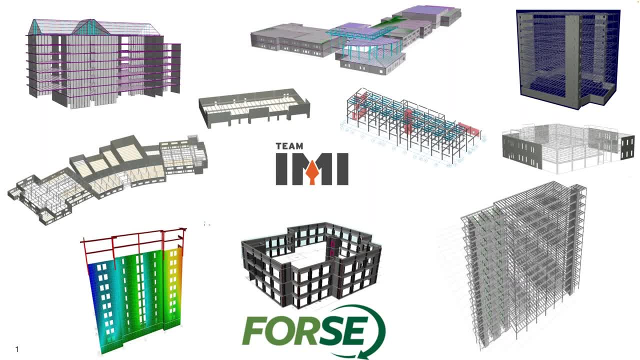 and uh, uh, um, before we ended, um, he asked if there are no steel plates used on the bottom of masonry lintels, and that is correct. there would not be a need to put a steel plate at the bottom of the mainstream until you would have the, the u-shaped block that would be at the bottom of the bottom. 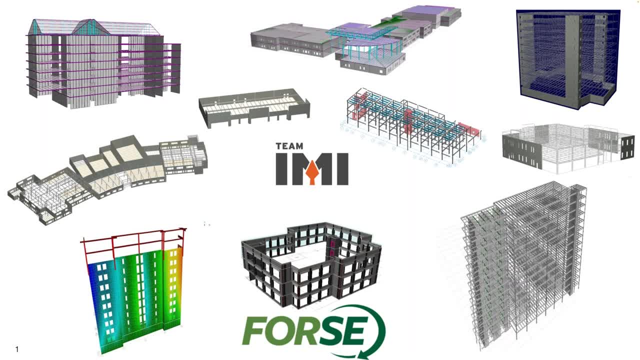 course of the lintel, which would be enough closure for, you know, for the single white wall or something like that. and you know obviously, how does all the door window frame? where does that? does that bridge a cavity wall? does it bridge the gap between um, or does a light gauge plate need to be added? 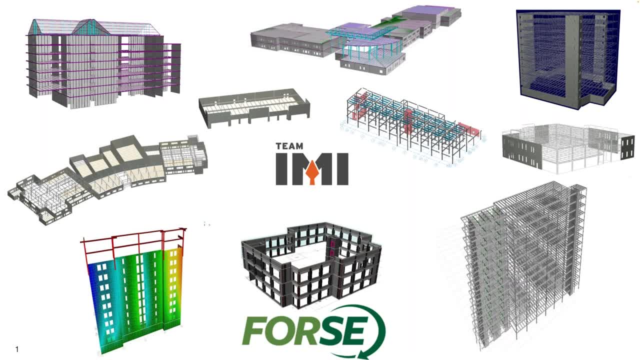 to fill that gap. um, you know there's a few questions there, but i don't know if that's where the question was leading or if you had further questions to that. but with the mainstream lintel there would not be a need for a steel plate at the bottom of the lintel. and then certainly 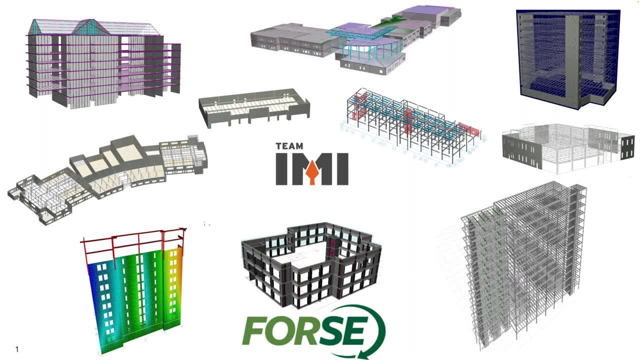 there wouldn't be a steel plate there to close that gap either, so it would need to be a different detail not used to close the gap in the cavity wall, if that's what you're asking. so thanks for the question. appreciate that. all right, if there isn't anything else. 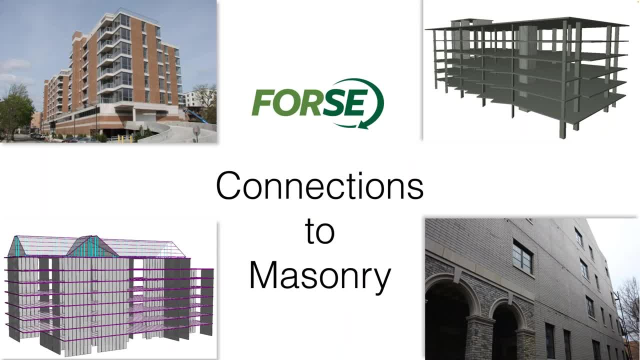 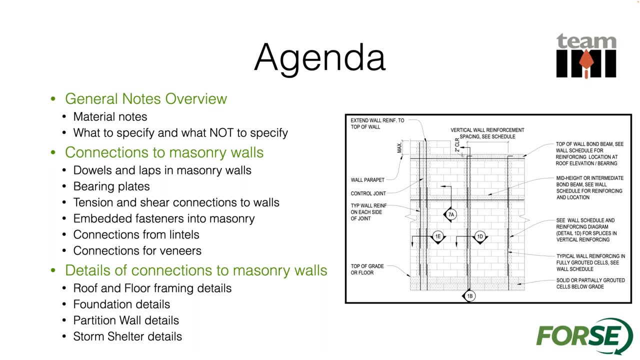 uh, we'll go ahead and get started with the second half. um, we're gonna go into uh connections to masonry and a little bit about uh details to masonry. um, you know, we just kind of want to start to cover beyond the design. you know kind of how do we start to tie some of this? 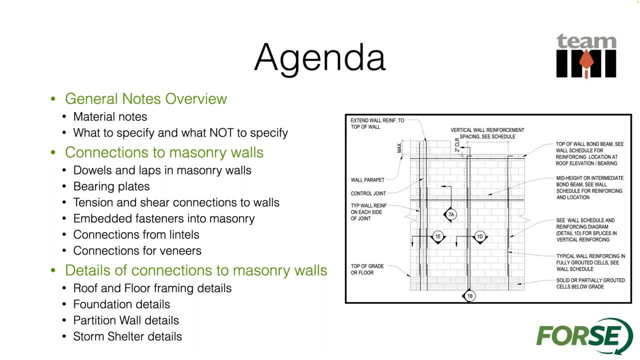 stuff together. uh, what are some of the details, what do they look like for our masonry designs? and then, uh, so we'll have a couple more sections, this one on connections, next one on details, and then we'll go into, uh, some software for masonry design and, hopefully, 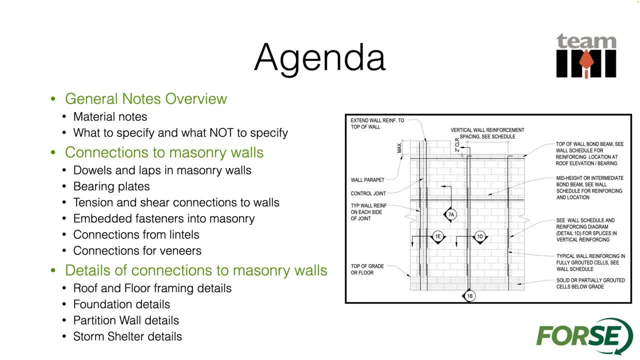 um, hopefully help you guys with uh learning about some tools that are available, and so we'll talk about that a little bit more and we'll go right over here to the next slide, all right, so, uh, so, just a really quick overview against just connections to masonry. we just kind. 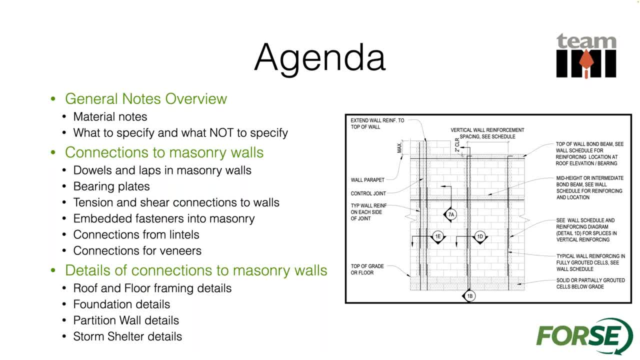 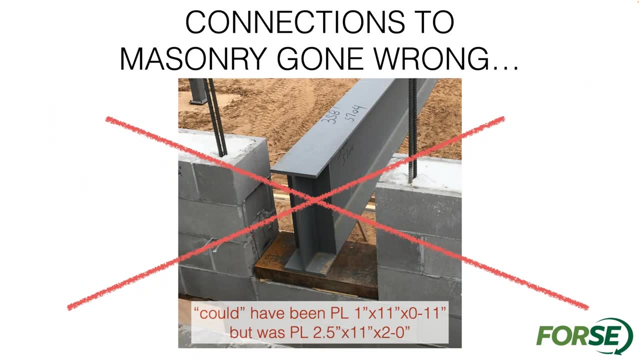 of look at some of the different elements that are used there, um bearing plates and bed plates, um connections from lintel veneers, so on and so forth, and then it looks like a few details that'll be used um roofs and foundations. You know some of the things with masonry design is. you know, we have from time to time, as I help out with different masonry coalitions, design coalitions, we encounter some things that slip through the cracks, some designs that get out the door and just don't make a lot of sense. 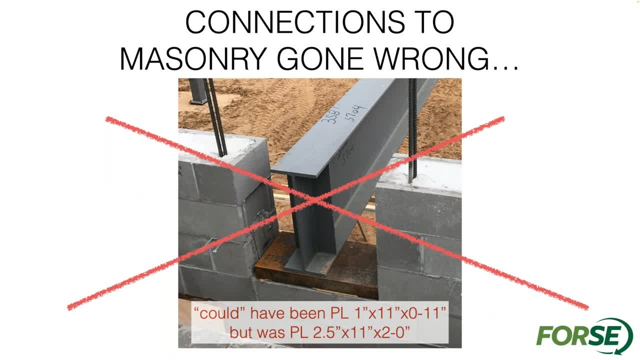 You know this is a design for a steel beam sitting on a masonry wall that was almost 500 pounds. It was a very, very, very heavy steel plate that was used for a bearing, for a beam bearing, And it just wasn't necessary. If it was necessary that'd be one thing, but it wasn't necessary And it just. you know, the number of problems that that massive plate is going to create in the future can be difficult. 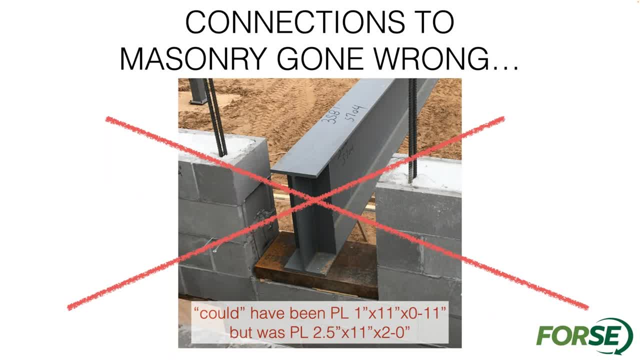 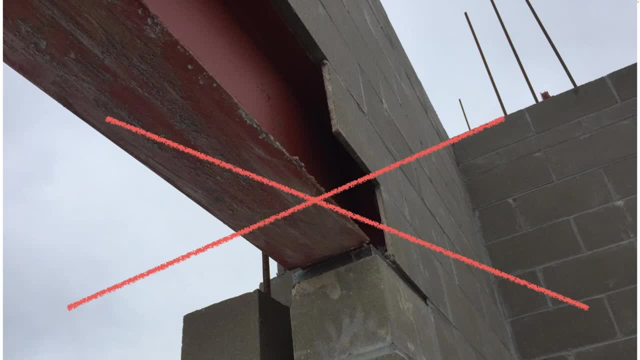 So we can do everything right design wise, But if we land with something like that, it's just not going to be something that's going to service well over time. You know other things. you know big bearing plate here. but the other thing that you know, as we detail in some different elements into masonry walls, you know thin soaps and stuff to conceal different steel pieces can really lead to a lot of issues and problems down the road as well. 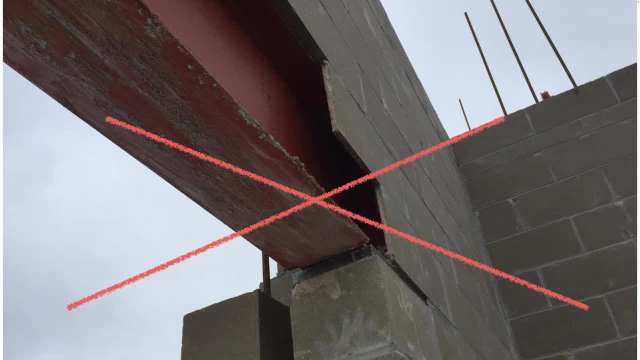 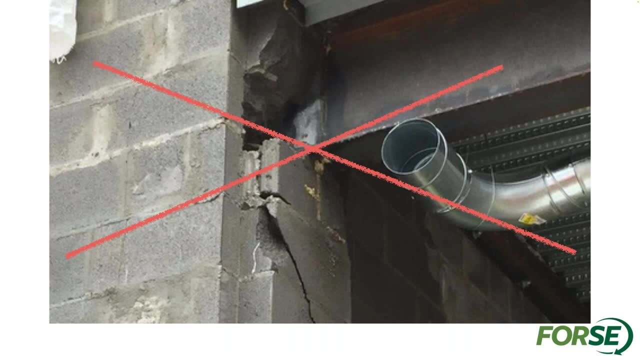 So again, we just try to head some of that off with a little bit better detailing and a little bit better designs. This is a very large steel beam. It's not necessarily a high end to a masonry wall, not necessarily steel into like I like to pick on. 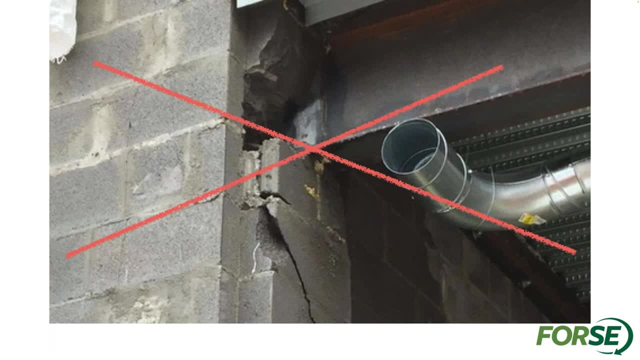 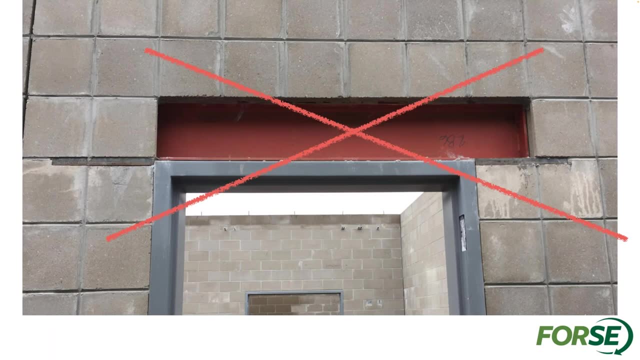 But this is just another one of those compromised bearing conditions that really required a very extensive and costly retrofit. So you know this is probably headed in that direction. It's a large steel beam, massive bearing plates. You know, and again, this is something that definitely could have been done with just masonry. 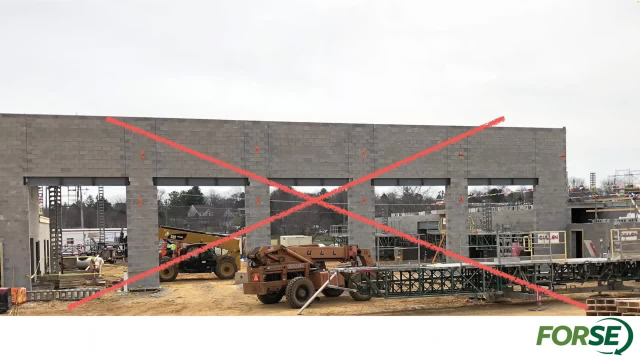 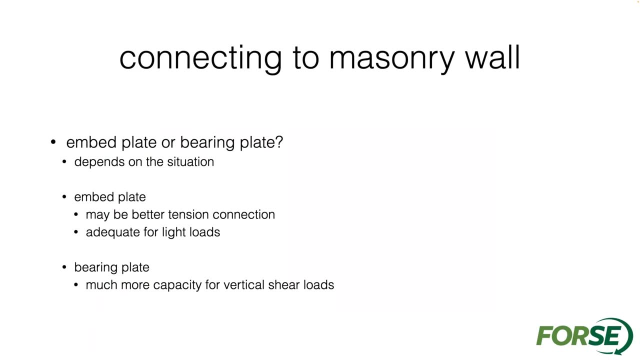 So, and we have a lot of little details like that. So connections to masonry, You know getting some of that stuff right, You know those could be certainly where a lot of problems exist for masonry. I think concrete masonry, clay masonry, concrete walls, a lot of those things perform very well. 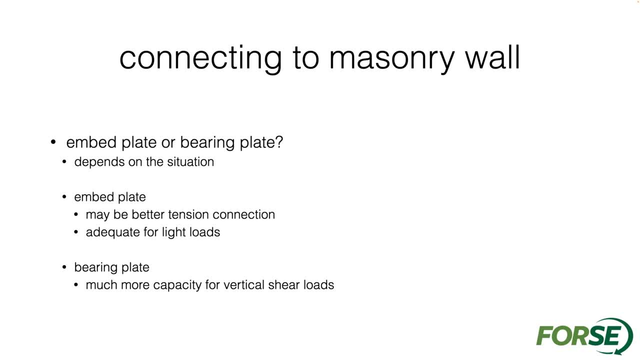 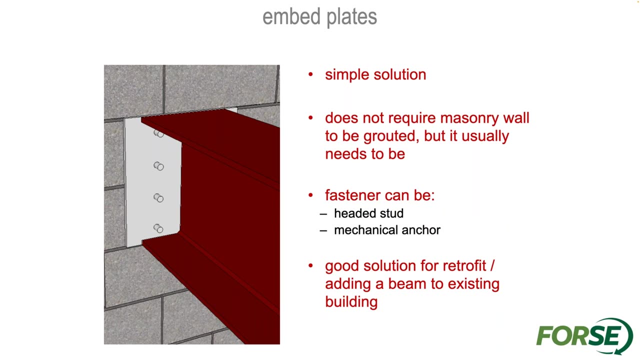 It's usually the connections to them or within them that can cause most of the issues. So you know, some of the common connections to masonry would be an embed plate or a bearing plate. You know, like tying in a steel beam into the side of a wall. you know an embed plate is something that we would. 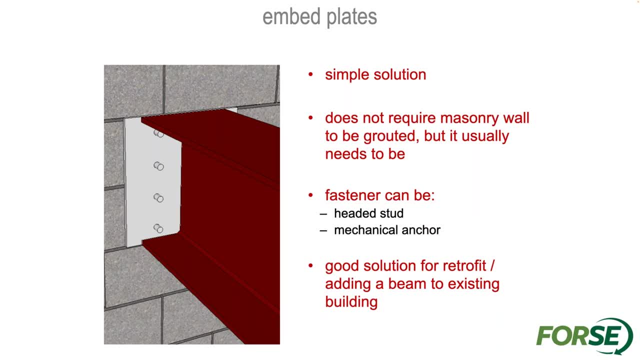 probably use if we were tying into, say, a concrete wall or a precast wall or tilt, a ball or something like that. It's just not the type of thing that we would need to do. I mean, it's a simple solution. 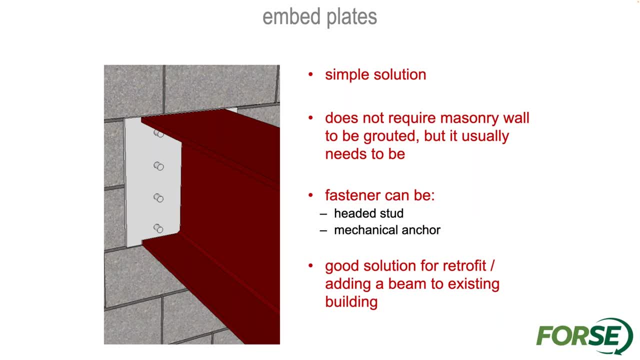 It's maybe what we would do if we had a retrofit situation where we were adding the steel beam in later. We could fill the wall with grout, a couple of grout ports and get some grout in there, But maybe that's something we want to do. 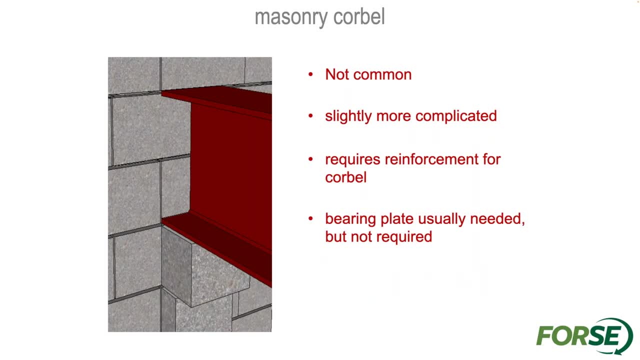 More creative solutions. I've seen people corbelling to pick up either a steel beam or pick up a floor. I've seen this actually more and more recently. Corbelling requires a little bit more detailing. It's not super common, but that can be a very nice. 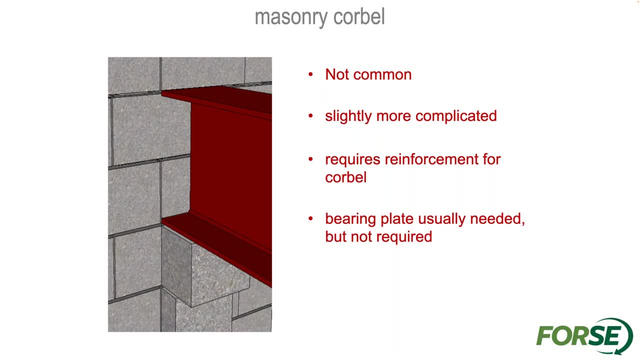 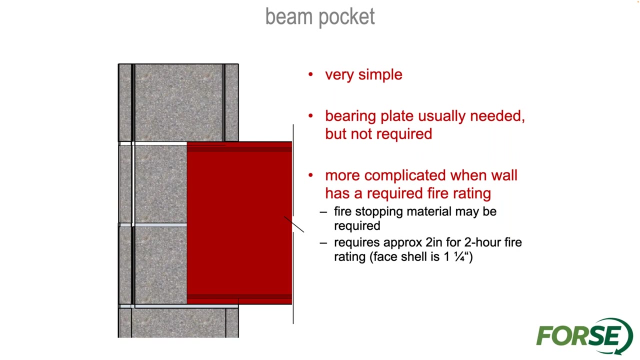 unique way to add a little architectural dimensions to some of these connections as well, And that's a much better solution than the embed plate. It's going to be much more economical. You know, just bean pocket is going to be the very simple way to tie in most floor members into a masonry wall. 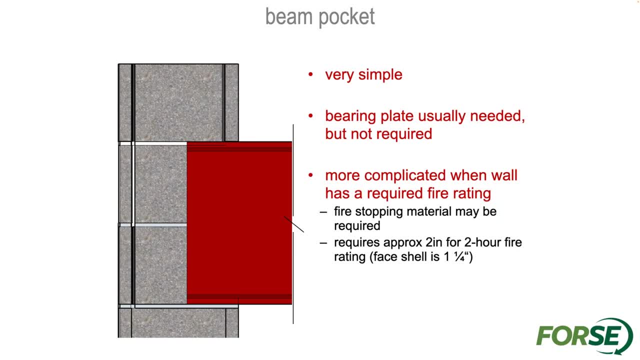 Tying it in and making sure that you know we don't lose fire rating. A lot of times masonry is going to be in the interior building for fire rating purposes. So you know, grouting it solid or putting in blocks and mortar and grout to solidify, whatever the 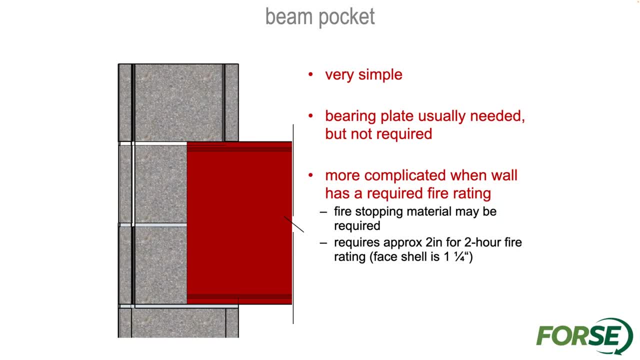 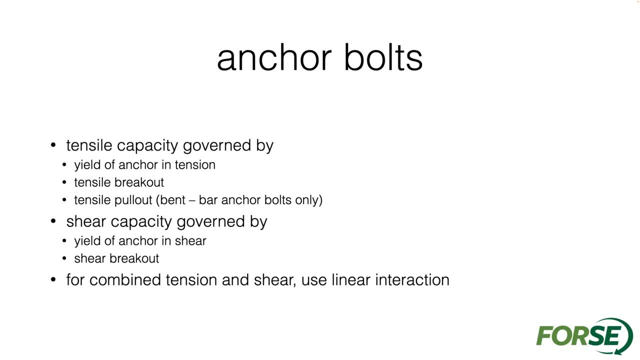 the pocket that's created for the bearing plate is simply going to be what we're needing: Inker bolts and stuff like that for masonry. we have certainly different failure modes that we have to. you know, we have certainly different failure modes that we have to. 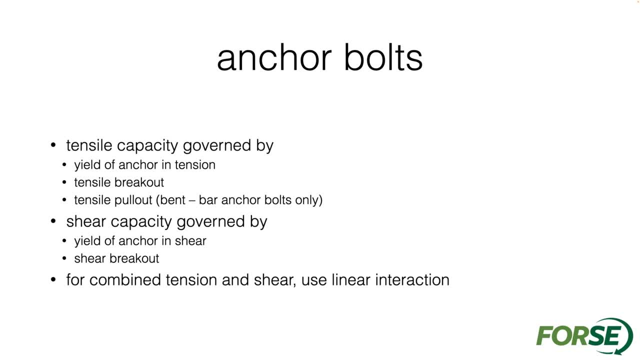 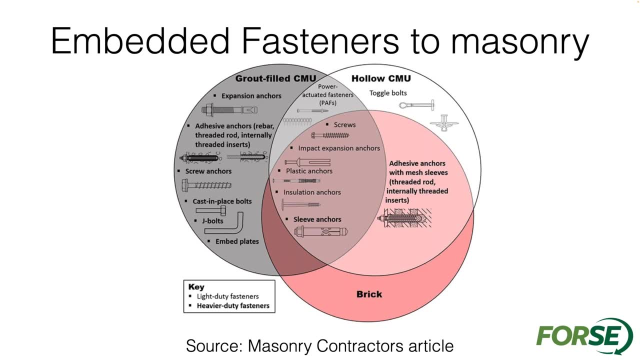 consider. we have tension and shear interaction that we have to look at to make sure that everything works out okay. You know the thing is with masonry. we do have a lot of different options here. We have a lot of different things that are coming into the masonry elements. 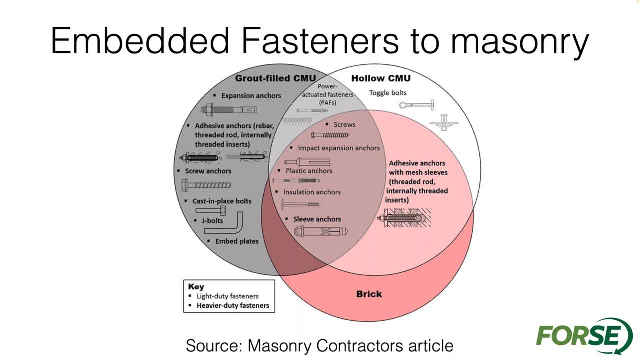 You know and making sure that we have- whether it's grout filled or hollow or brick- we have the right types of anchors that are going to be used for masonry design. making sure that you know we account for the different capacities that can be used. 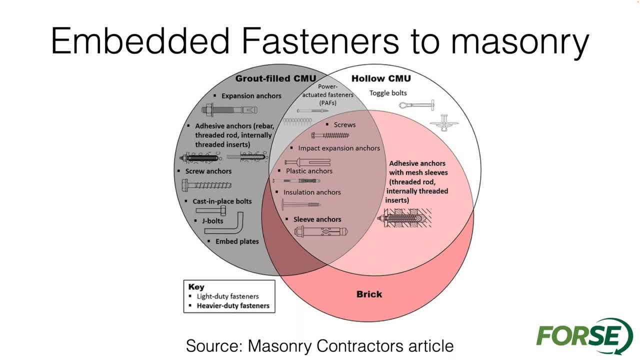 I mean certainly anytime that we kind of a grout filled or a solid brick or a solid masonry is going to be more capacity. But we don't have to if we have a light connection or something that doesn't require a lot of demand. 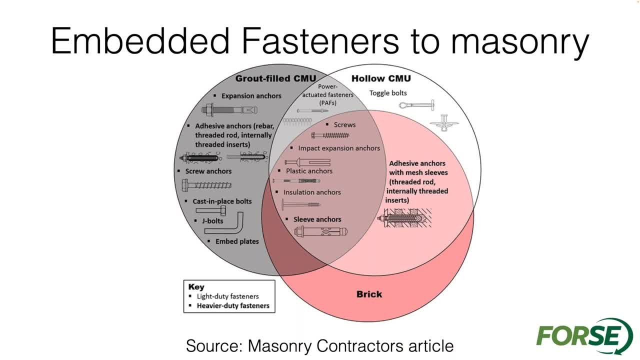 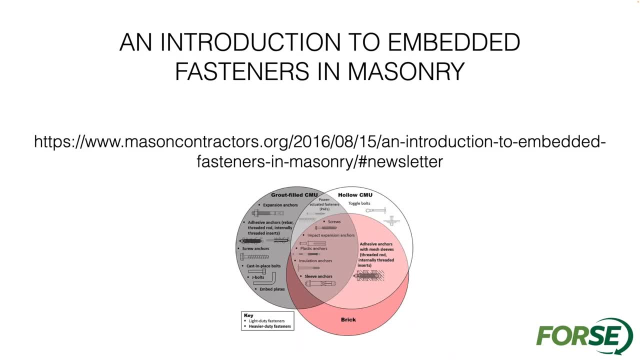 there's some different hollow masonry fasteners that can certainly have sufficient capacity. There is actually a nice article that I reference here on mason contractors that kind of looked at this guide and some talked about some of the differences between some of the different fasteners that you can use. 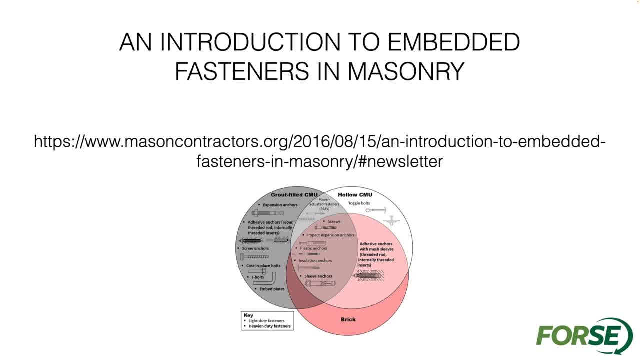 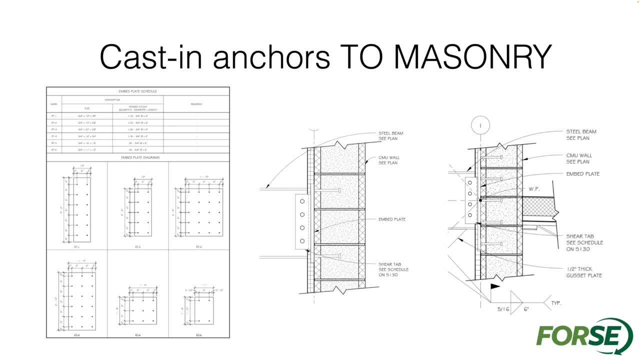 for the various types of masonry walls that you want to tie into Cast-in anchors or any of those types of connections to masonry. that's again anytime we're connecting to the face of masonry or face of concrete the failure modes and just the. 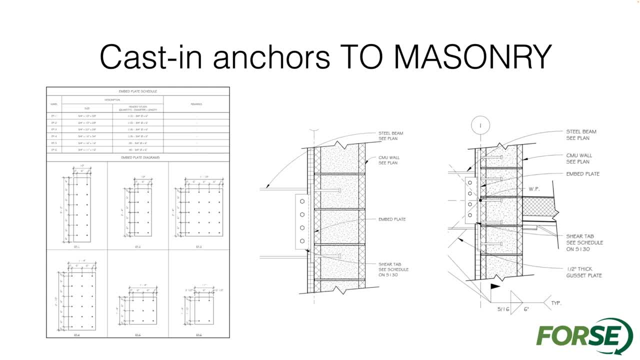 you can see the different embed plates or the connecting plates got pretty large in this project that I worked on. This was actually an architect that wanted to see some of those plates and some of that kind of exposed steel framing into the masonry wall. So it was an architectural demand for some of this design. 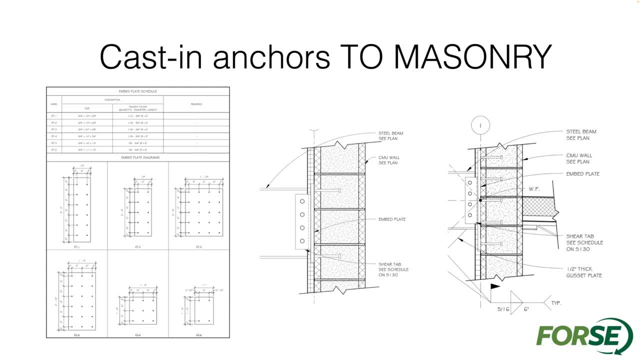 but it certainly became pretty elaborate as we're tying into masonry. Usually as we tie into masonry, tying the concrete, the failure modes that are going to govern the design is usually the concrete or masonry that we're tying into. So just kind of recognizing that is going to be important. 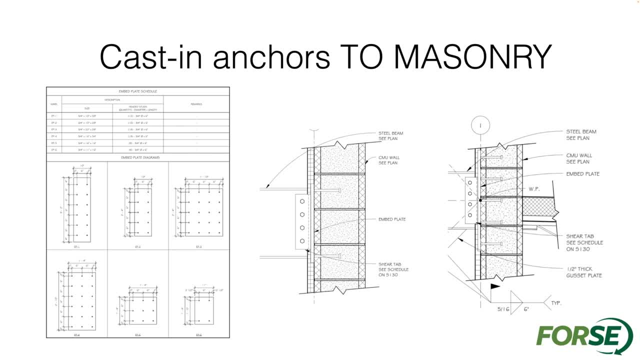 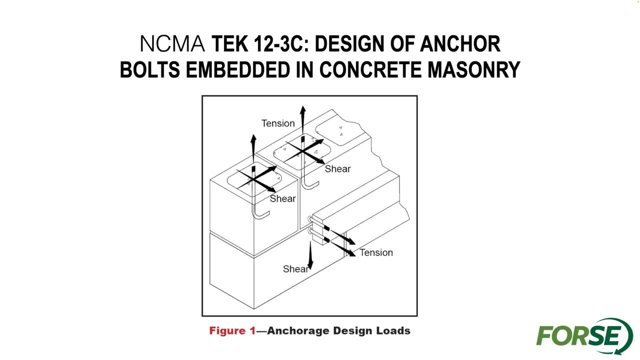 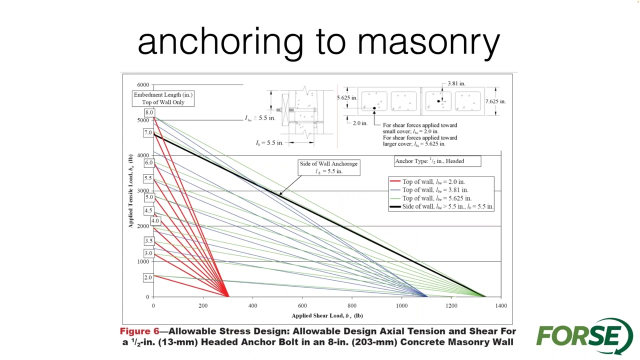 Design-wise. NCMA Tech has another guide which can be very useful here: The design of an anchor bolts embed to concrete masonry. It's got a couple of nice little charts in there for both allowable stress design and strength design. It actually comes with a spreadsheet. 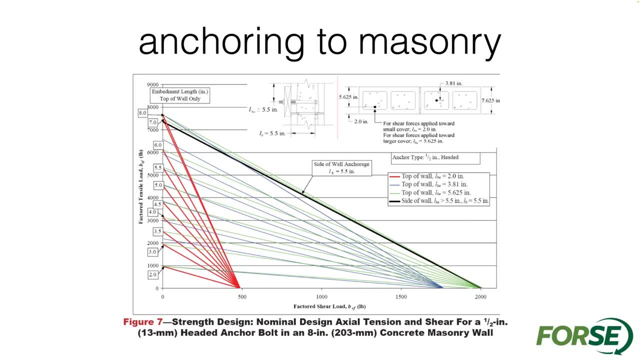 that really looks at the connection capacities as we're tying into masonry walls. It's going to be looking at a single anchor, either at the top of the wall or at the face of the wall, coming up with some of those different capacities. 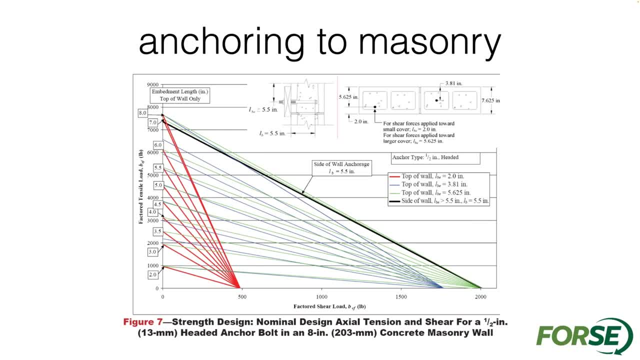 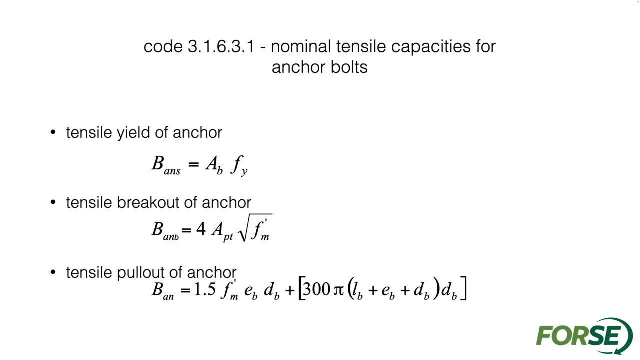 for design, The different failure modes that you have. you have the tension yield of the anchor, you have the tensile breakout of the anchor, which is obviously the masonry area breaking out or the tension pull out of. you know the tension pullout. 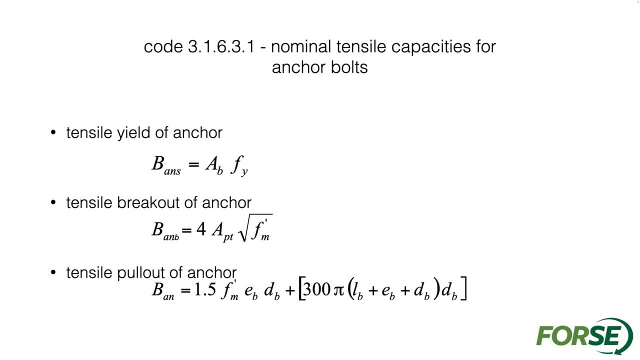 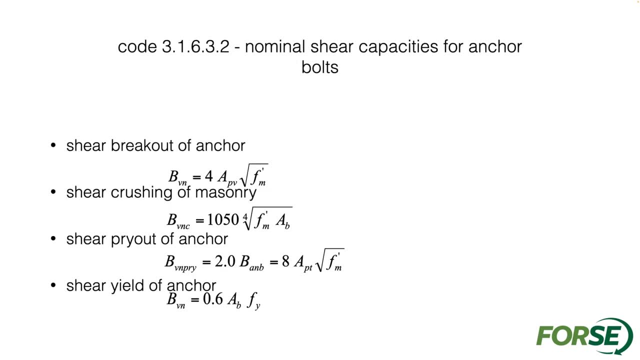 So it's going to be looking at a single anchor, which is obviously the tensile breakout of the anchor. Obviously, the second two equations here are going to be generally the controlling variables for your design: Nominal shear capacities. we have the shear breakout of the anchor. 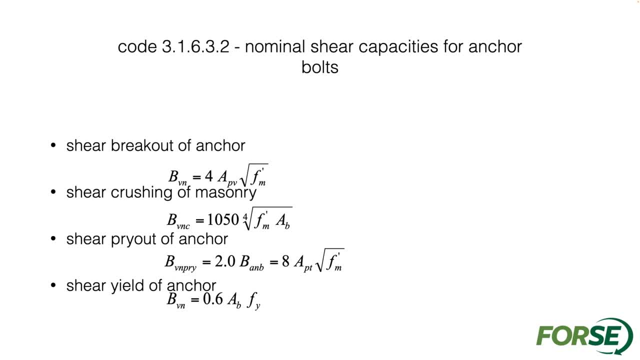 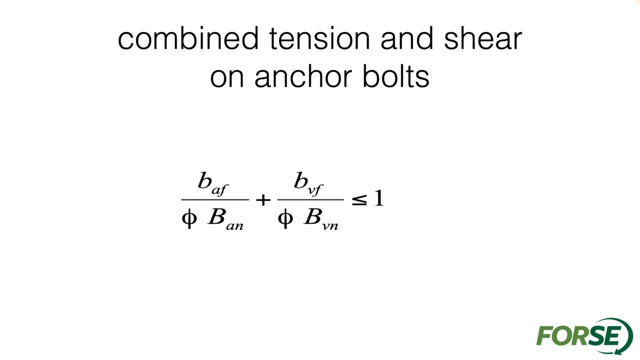 shear, crushing of the masonry, shear, pryout of the anchor, all masonry, controlled failure modes and then the shear yielding of the anchor. Once we come to the bottom of the design, we have the axial and shear and then the shear yielding of the anchor. 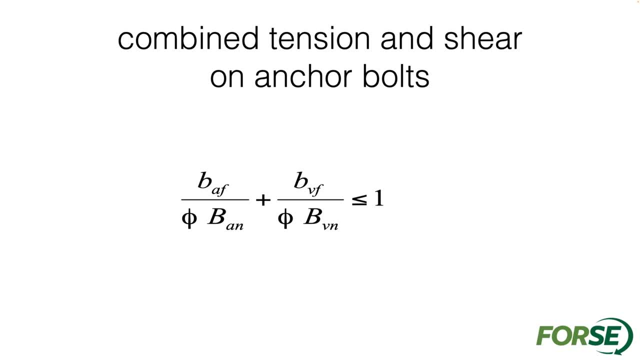 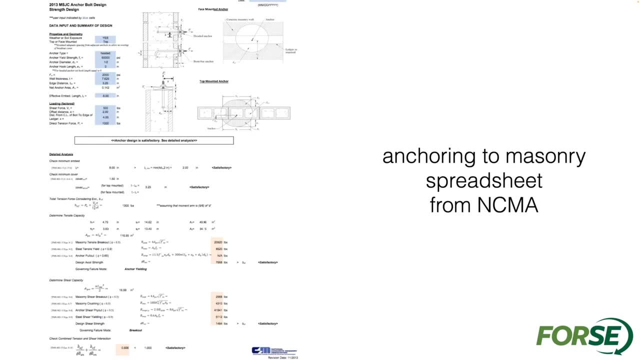 And then shear capacities. we're going to look at both of those in combined and making sure their interaction equations combined is less than one. Again, there's a nice spreadsheet from NCMA that looks at some of these capacities. You know, when connecting to masonry. 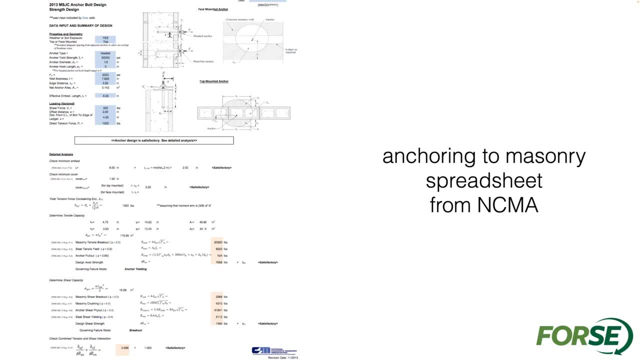 some of the other things that we have to make sure that we think about and consider is we're connecting into these confined spaces. We don't want to have anchors that go through the masonry, through the grout, all the way into say: 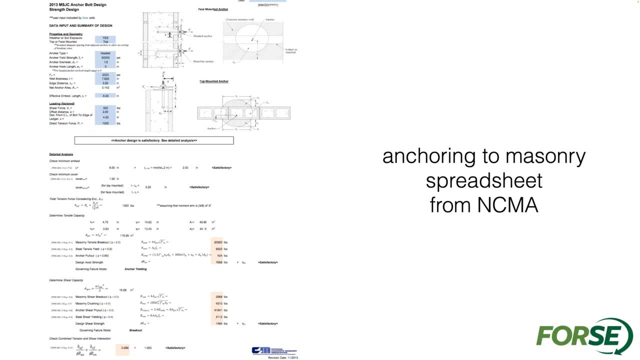 the face shell on the backside or whatever you have, I mean, especially if you have a cast-in anchor. thinking about the confined areas of masonry, the compatibility between your fasteners on the masonry that you're actually tying into is really important. 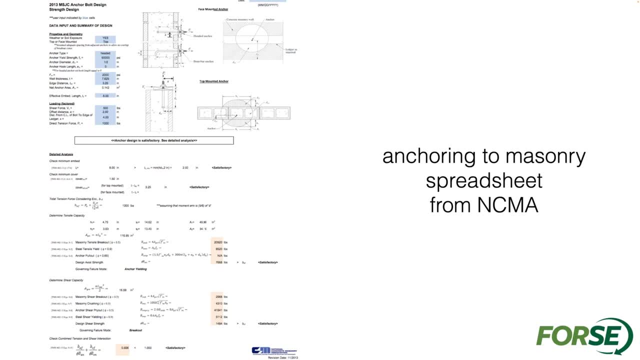 You know, putting in a anchor, you know, at the top of the wall, you know that's not more than the, say, the lintel block depth if it's near a lintel or something like that. I mean trying to consider the different shapes that you have. 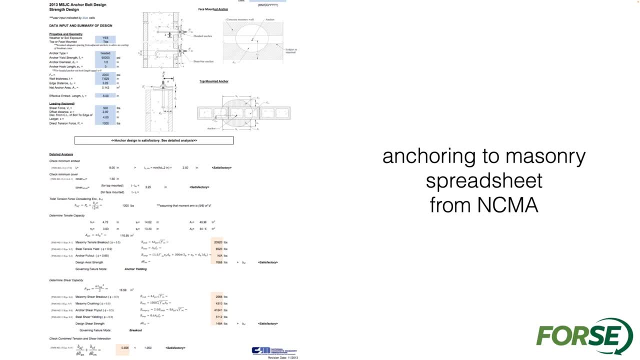 and the compatibility between the fasteners and the masonry units is going to be really important in terms of coming up with connection design. Obviously, the connection design spreadsheets are going to be working well for you And, again, you know this is something. 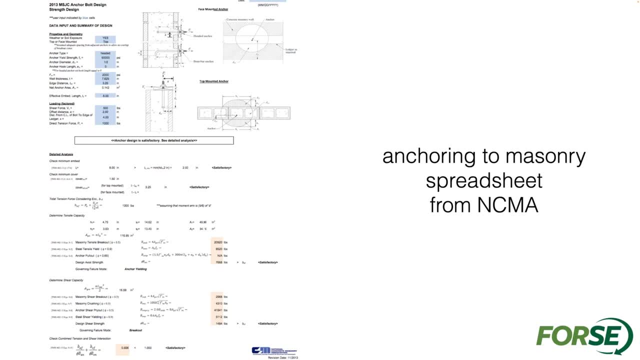 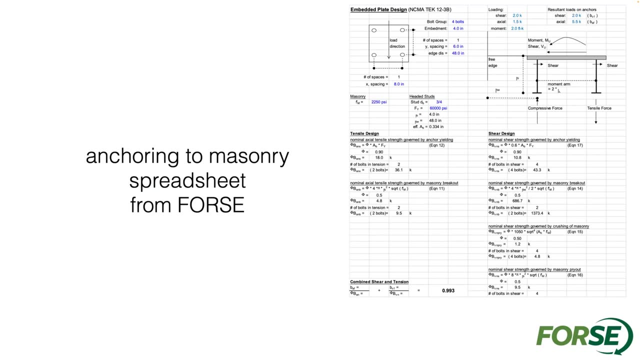 that you can download for free from the NCMA website. One of the limitations of the spreadsheet is going to be looking at it as an individual anchor, looking at groups of anchors. This is a spreadsheet that you know I created. this is going to be really kind of combining. 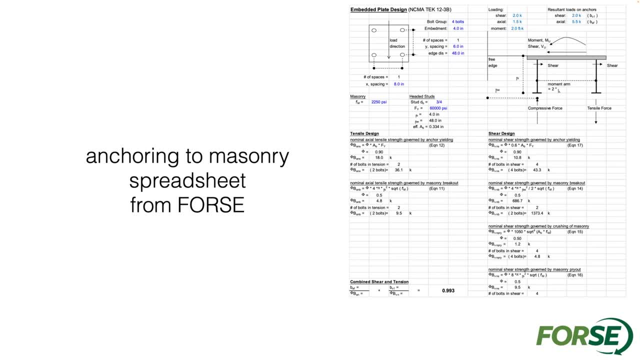 what we have with NCMA and ACI and trying to create a, creating a guide or creating a tool for looking at groups of anchors, because often we have groups of anchors that we're designing for the capacities of them tying into masonry elements. 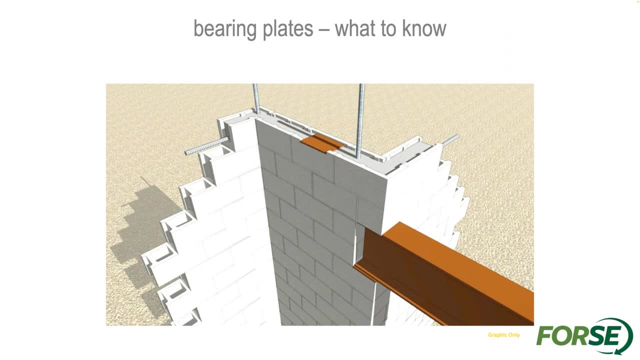 Bearing plates. bearing plates are, like I said, going to be whether at the top of the wall or a beam pocket on a wall. bearing plates are certainly going to be the preferred way to connect to a masonry wall For bearing plates. I think there's a few other advantages. 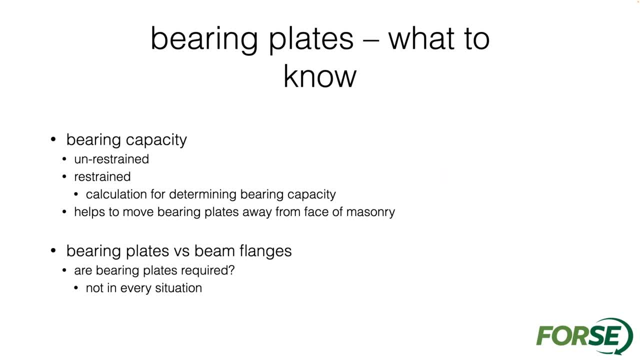 that you know we can utilize. here We have a bearing capacity that we looked at. You know we have an unrestrained bearing capacity. We have a restrained bearing capacity. So the restrained bearing capacity is really looking at the bearing capacity that you have on a masonry element. 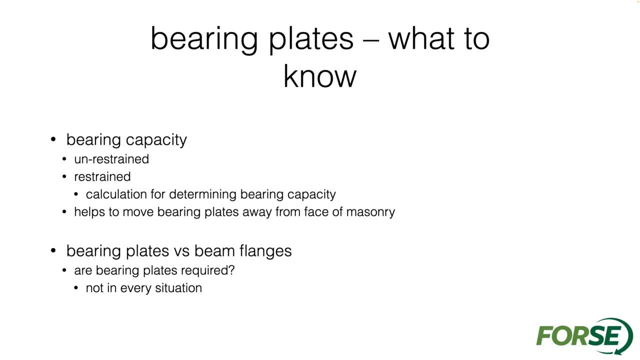 and you're within the interior area of the masonry element. So restrained would be something like a base plate or a bearing plate that stays centered on a wall that has you know, maybe four inches of width for an eight inch wall That's going to have a restrained capacity. 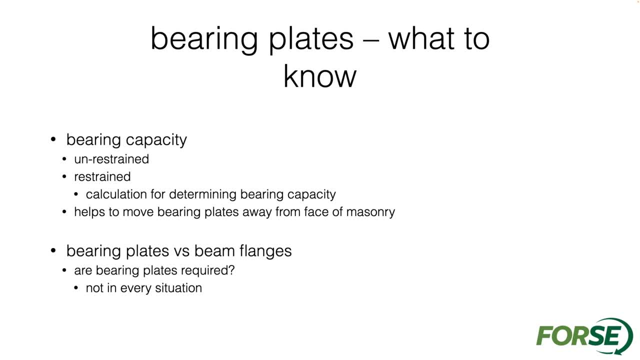 The bearing on it is going to have to do with some distribution of force over a larger area. It really does help us get a higher bearing capacity. Anytime that you would have, say, an eight inch plate on an eight inch wall, that would be an unrestrained 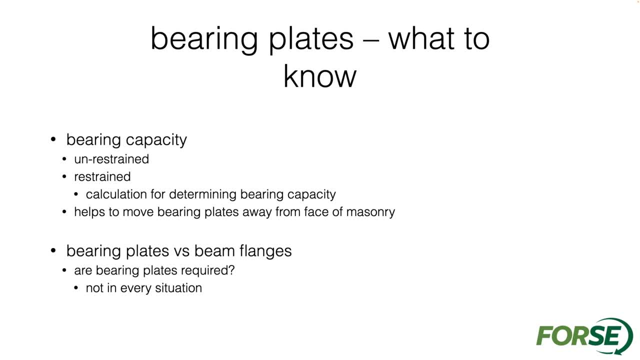 We have the bearing that's going to be stressing all the way to the edge of masonry, which is going to be then unrestrained and have a lower bearing capacity. So anytime that we can move a bearing plate away from the face of the wall, 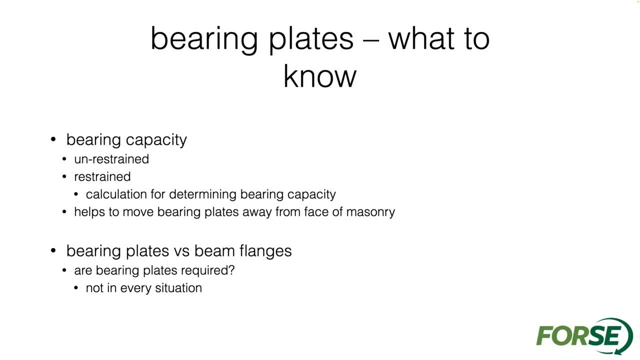 it's certainly going to have a much bigger advantage. You know the other things about bearing plates. the bearing plates aren't required, certainly by code, And anytime that we're doing something like this, you know you're distributing force to a masonry wall. 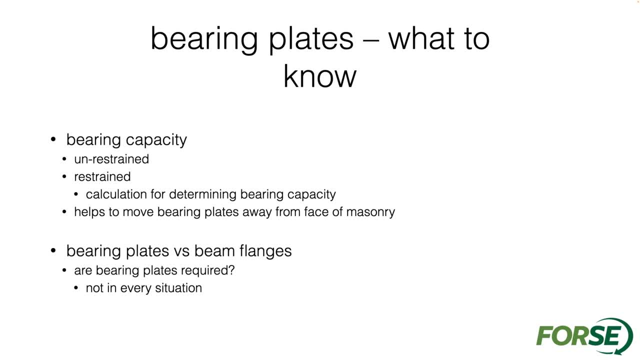 from a steel element, sometimes just setting the steel element on the masonry. maybe you just need a setting plate. Do you actually need a bearing plate to distribute the load? Other things to think about design-wise. So again a couple of little simple illustrations. 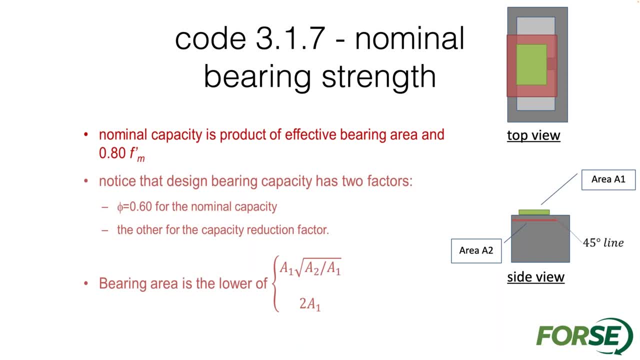 to try to point to you know what I'm talking about here. with the restrained bearing area, The top view in the image, in the upper right, the green area is going to be what I would consider the bearing plate, So the area directly under the bearing area A1. 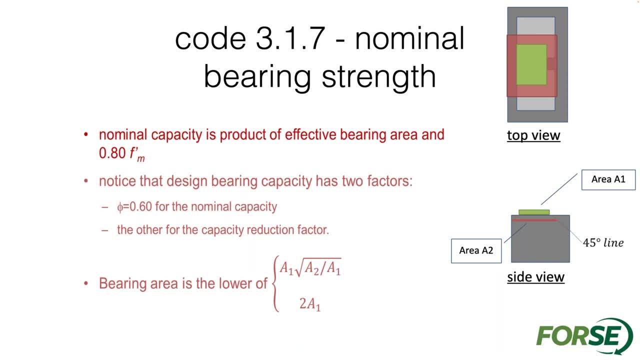 is going to be kind of that primary area. So when I can move that plate away from the edge, then what I can do is I can draw a 45 degree lines down to create a larger area A2. So anytime that I can move, you know. 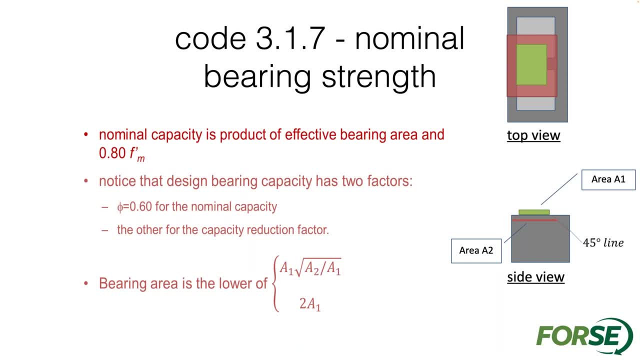 that bearing plate further and further centered on the wall would be the best case scenario. But the bearing area is going to be, you know, all the way up to two times the initial bearing plate size, So we can have a lot higher capacities for bearing. 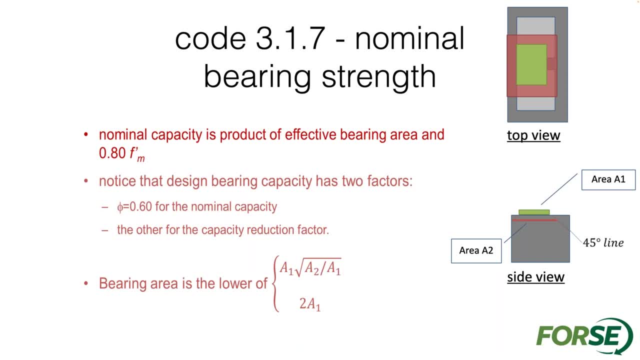 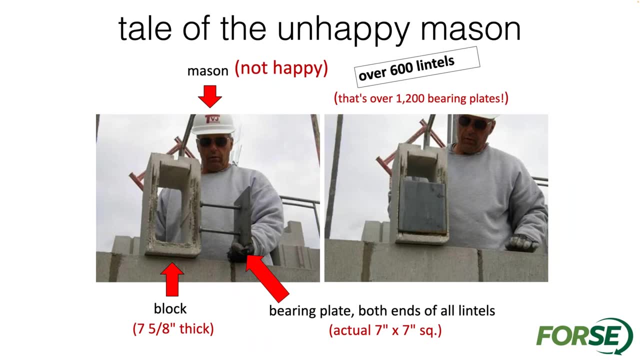 anytime that I can move the plate away from the center of the wall. The other thing with the dealing with bearing plates is, you know, looking at this mason that had a bearing plate, that one was coming nearly to the edge of the block. 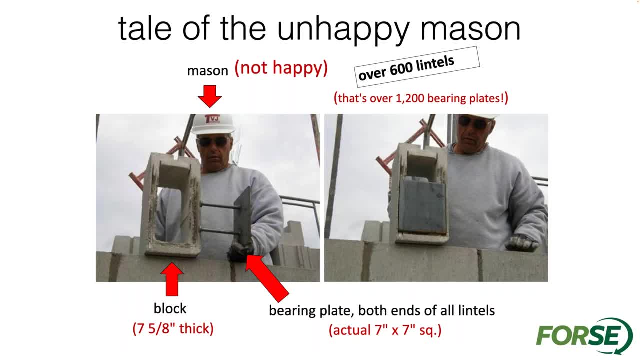 but also it had to be inset into the block because of the size and thickness of the plate. So that required cutting and modifying the block to allow for the bearing plate to fit within the block flange areas And that just requires a lot more construction time and cutting. And the truth of the matter, 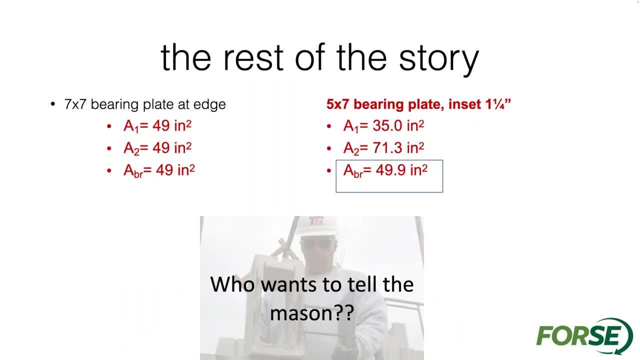 is a bearing plate. So if I look at the two different plates, if I look at a seven by seven plate that comes to the edge, practically to the edge of the masonry, I have a A1,, A2, and the effective bearing area that's 49 square inches. If I had a five by seven, 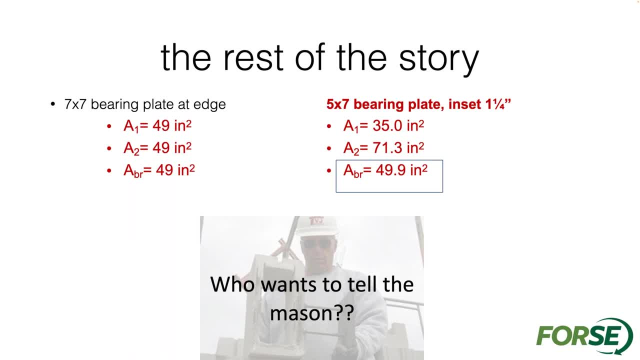 if I have something that's a little bit smaller. the five by seven plate, instead of inch and a quarter, so away from the edge, has a larger effective bearing area. Why larger? Just because the plate actually can grab some more length and not just width. So the seven inches wide, 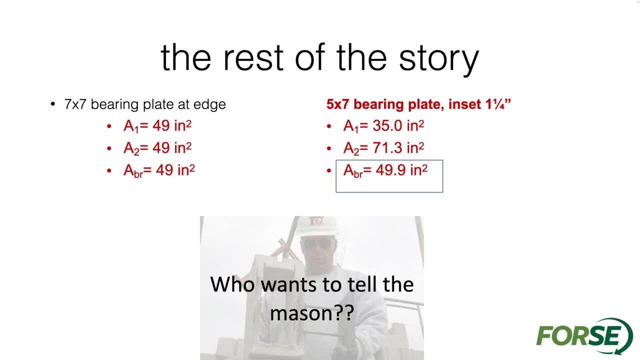 helps me grab what ends up being an effectively larger bearing area. So that that's kind of an interesting. I mean, that's obviously tested and it's. you know, a larger bearing plate can have less capacity when it comes to the edge of the masonry wall, So that's a 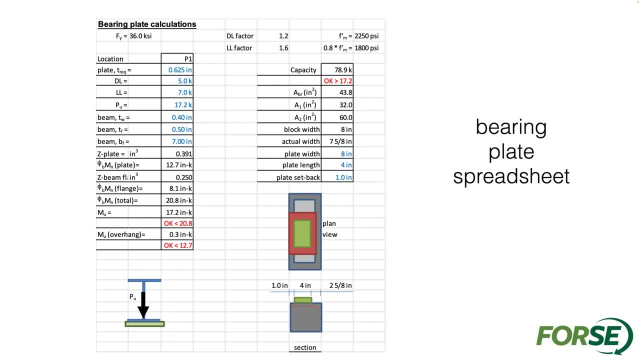 really interesting and very important thing to recognize and look at as we look at a bearing on masonry One bearing plates that come to the edge are a difficult thing to deal with in terms of rust proofing and making sure that it doesn't have any conflicts with, you know, any of the 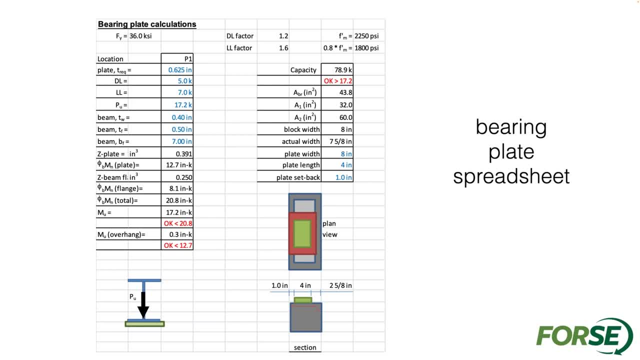 aesthetics that we're looking at, but then also it has less bearing capacity, And so that's something really important to recognize and realize. So, embed plates or bearing plates, it usually depends on the situation and embed plate unless there's an aesthetic reason for. 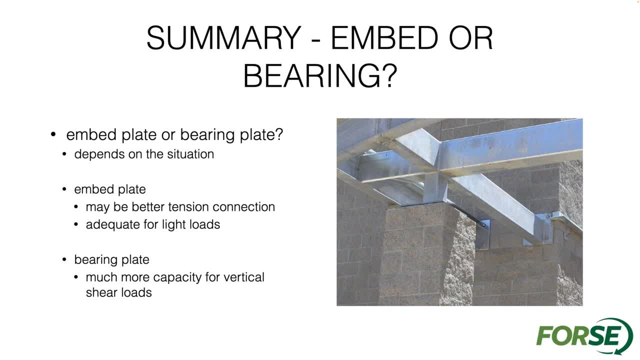 it. it's usually going to have a lot less capacity. It's going to be adequate for light loads. Maybe it's something that is when you post install or, like I said, if there's an architectural reason for doing that, but otherwise a bearing. 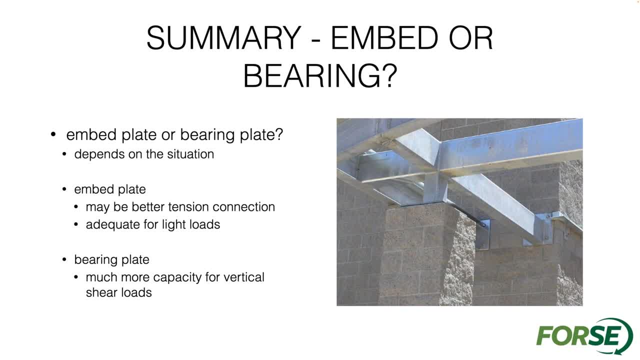 plate is going to have generally more capacity. It's going to have more vertical shear loads. Certainly, if you size the plate correctly, it's certainly going to make a big difference. So, connecting to masonry, other connections to masonry, I think you know, tying in frame. 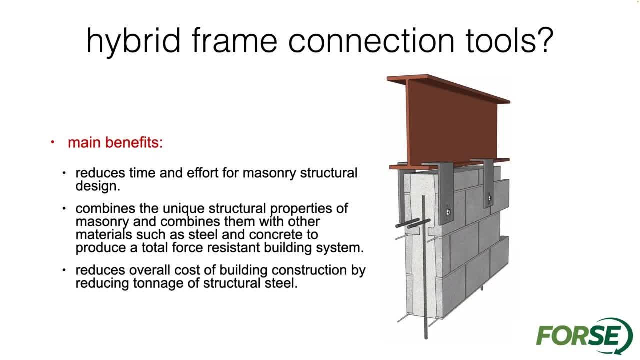 we talked about infills. participating, non-participating, connecting to masonry can be really, really critical. We want to use masonry for resisting shear loads just because it's a, it's something that it's got a lot of capacity and it's got a lot of capacity. 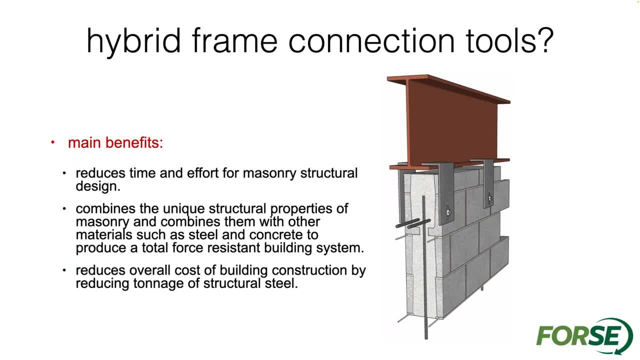 and shear. So you know, connecting to them. you know there's some hybrid design guides that are out there for connecting frames to masonry. There's different types of hybrid designs. I mean when we have a steel or a concrete frame and we infill with masonry, how we distribute and 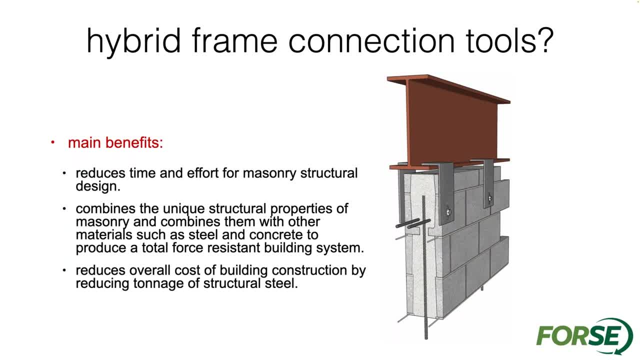 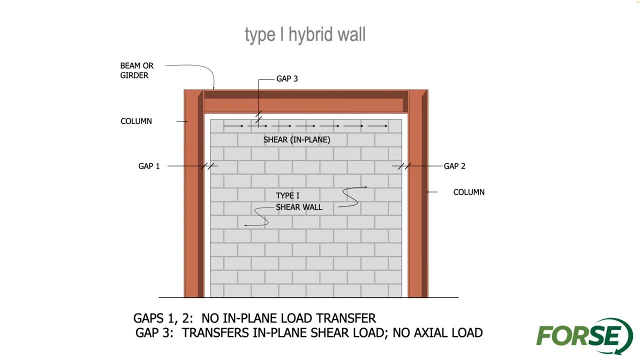 transfer the forces from those other elements into masonry. the code that we tried to look at a couple of different types of hybrid designs. type one- hybrid- would be kind of a gap all the way around. So we're really kind of building the structure, the frame, whether it be again. 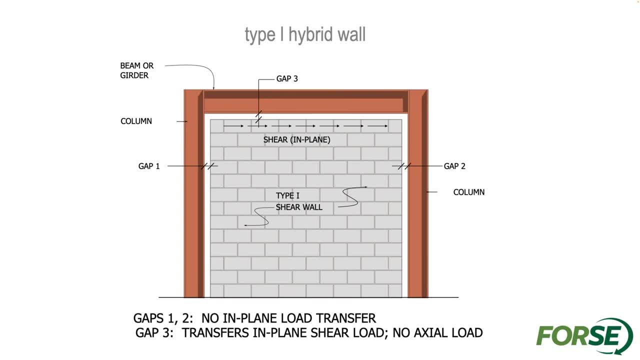 be steel, be concrete. we leave a gap all the way around just because that's easier to build. It's easier to build up. The masonry leaves some spaces around each edges. What that does do is it reduces the masonry to just being an unloaded, non-bearing shear wall, which is 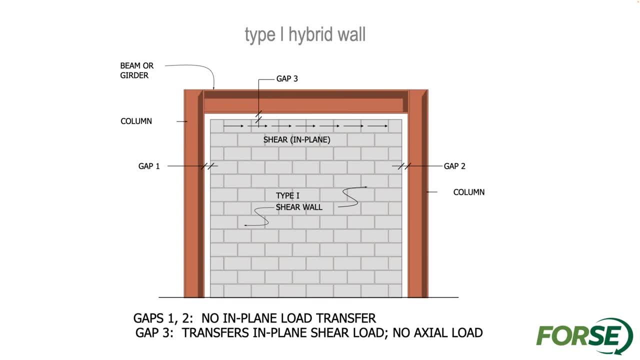 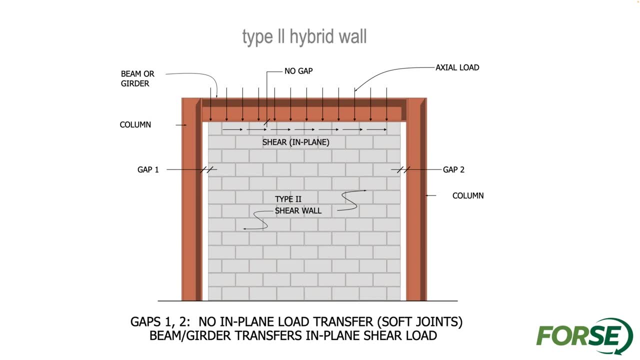 going to have plenty of capacity Anytime that we could go to say a type two hybrid, where we build the masonry up to the underside of the structure. What that does do is it makes it a bearing shear wall. so something that's going to be in bearing is going to be a lot better in shear. 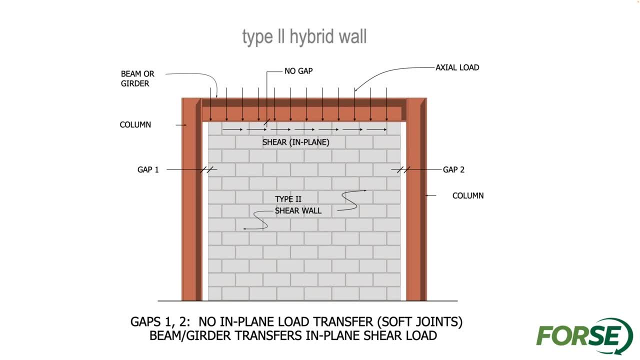 The difficulty with that is that, construction-wise, building up to the tight, to the underside, you can build up and get close and then you could grout solid from the top to the underside of the structure above. So what the masonry groups tried to do is try to create some sort of 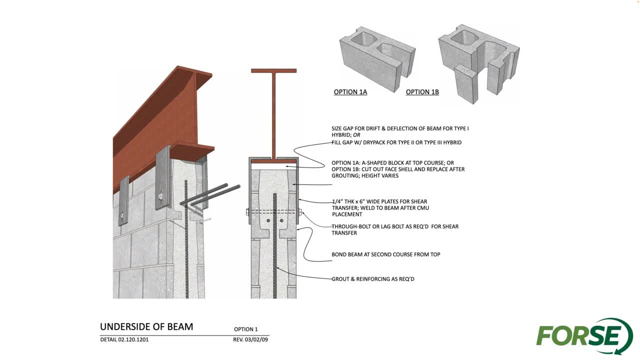 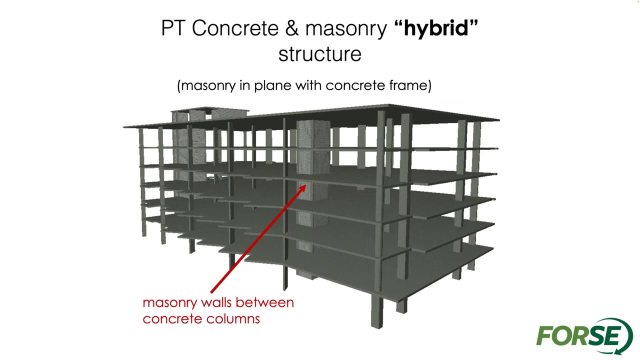 details and methods for giving designers some options for how to create these connections and bring this stuff into masonry design. One of the nice little marriage of materials that I've been exploring and looking at a lot more is post-tension concrete slabs and masonry walls. these infill walls. They're very nice because post-tension. 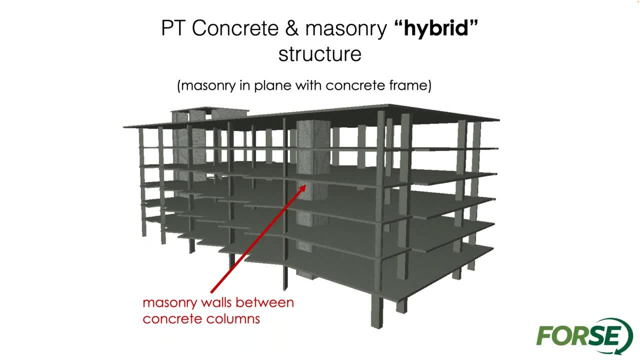 concrete. we don't like to have a lot of walls, in particular when we're building the PT slabs and we stress the slabs. We want to be able to just have the slabs sitting on columns so that they can move effectively and we can create the compression force that. 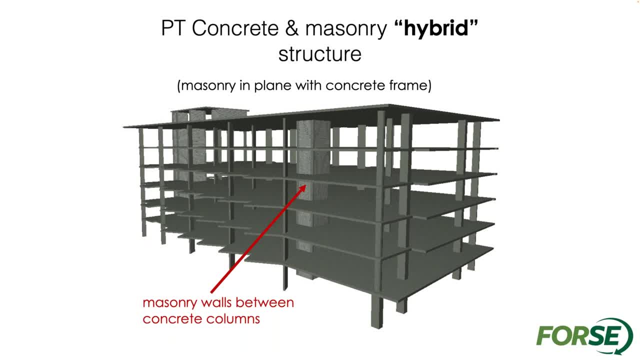 makes the post-tension cables the most effective. The nice little marriage of materials here is the masonry that can come in after the fact and be an infill. It can participate as a hybrid wall, but it doesn't restrain the slab from moving. So it's a very nice little marriage of materials. 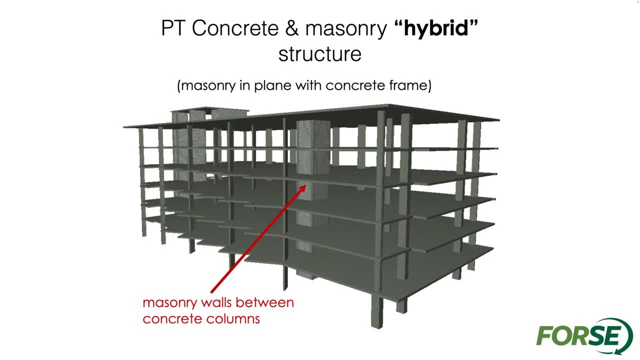 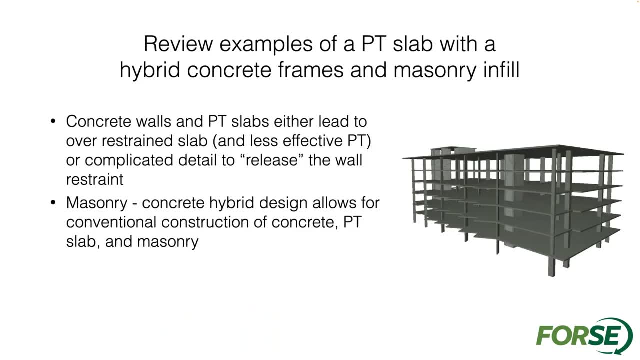 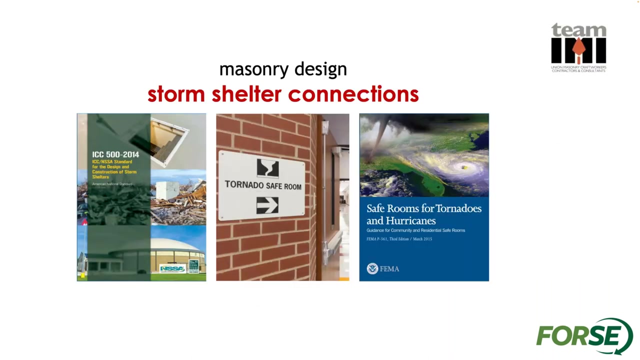 Again, it's a concrete and masonry hybrid frame that works pretty well. So it really allows for pretty normal sequencing of construction and that really can be, like I said, pretty beneficial to the overall masonry design. Storm shelter connections: We didn't get into masonry storm shelters, We didn't quite have. 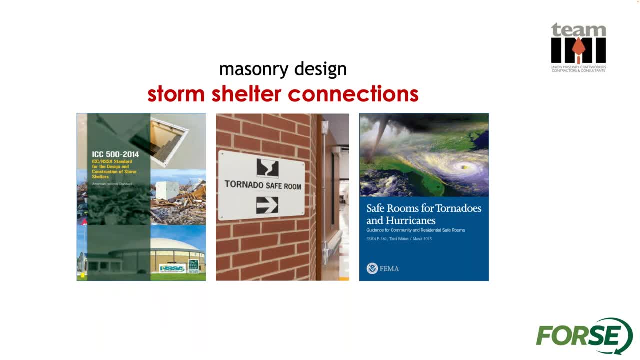 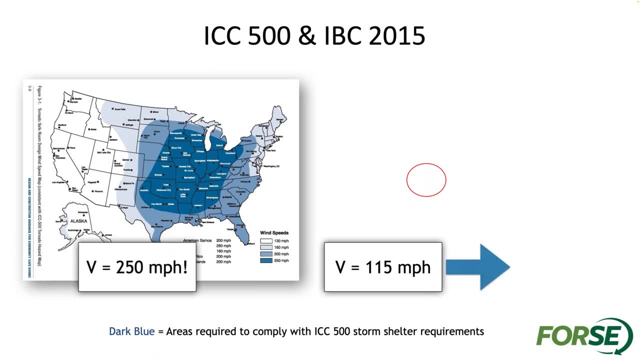 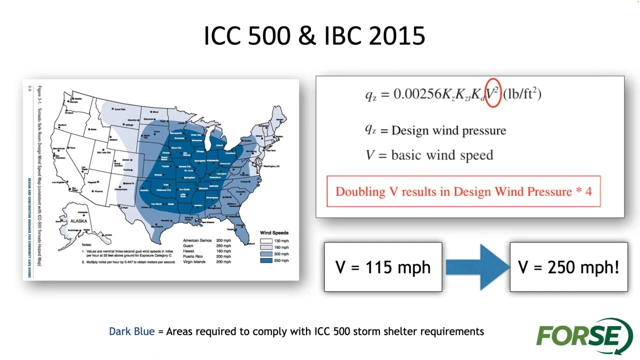 enough time to fit those in today. Just a really brief overview of storm shelters. We have certain areas of the country that have to allow, have to be designed for much higher design loads, having velocities that we have to design for more than two times the standard velocity. 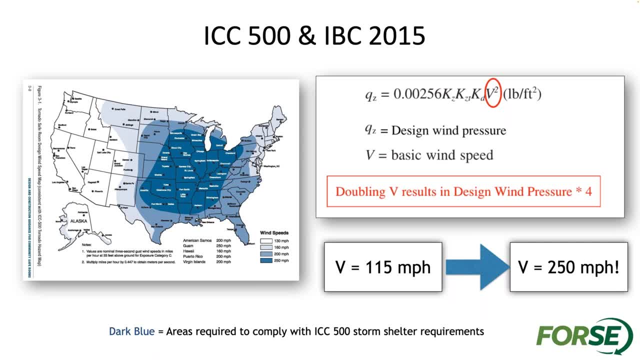 So our design pressures get very, very high within storm shelters And so having masonry being able to be designed for that is certainly, you know, anytime utilizing all of the different capacities of masonry, doubly reinforcing, you know, maybe horizontal, vertical reinforcing. 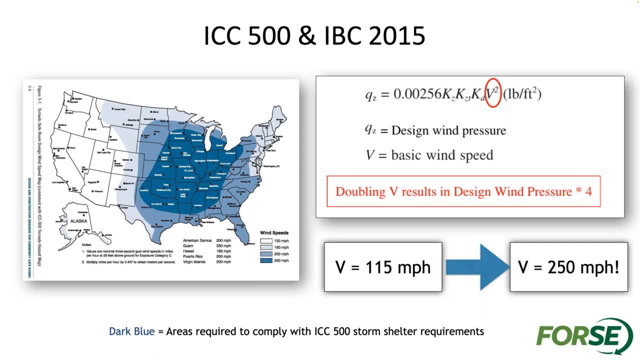 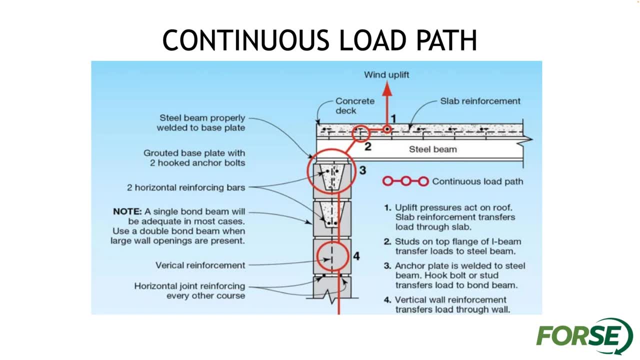 a lot of the being able to make storm shelter work really comes down to the connections. The connections for masonry, you know, into the roof is going to be, you know, one of the things that we have to take close consideration for making sure that we have, you know, the roof. 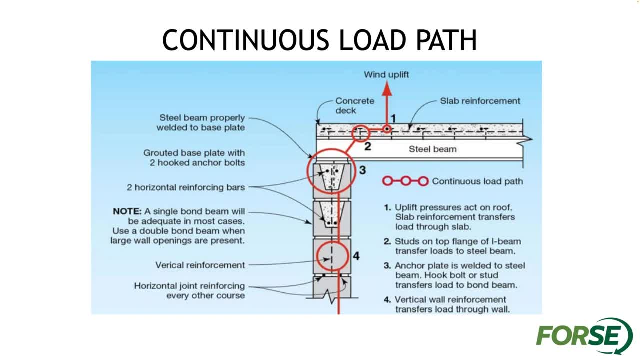 framing or the roof slab or whatever we have actually tied into the masonry wall. We have very long embeds or bars that we have, that we have to develop down into the masonry wall, So creating that continuous load path for, you know, masonry in a storm shelter. 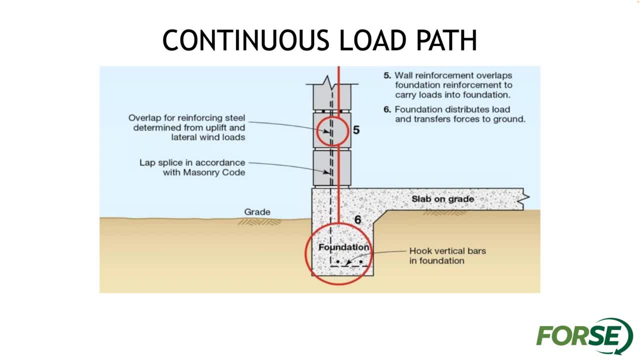 And then that goes all the way down into the masonry, into the foundation, making sure that we fully develop. you know, all of the reinforcement that we have that goes all the way down. certainly, having all of those bars fully developed, that certainly does give the structure that much more. 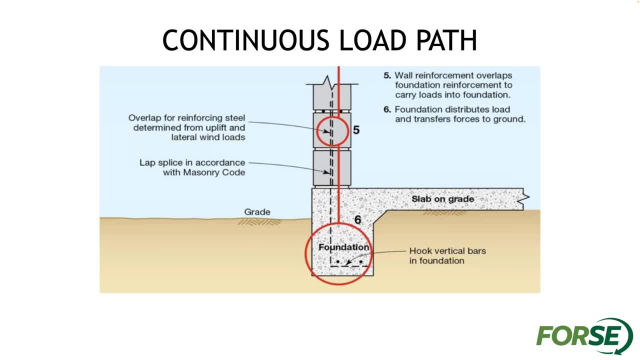 rigidity. we have a lot of connectivity between, say, the foundation and the walls, both the slabs and the foundations and the roofs that we have that are tying into the mainstream wall, so that does make it even more robust. but certainly the continuous load path is going to be important for 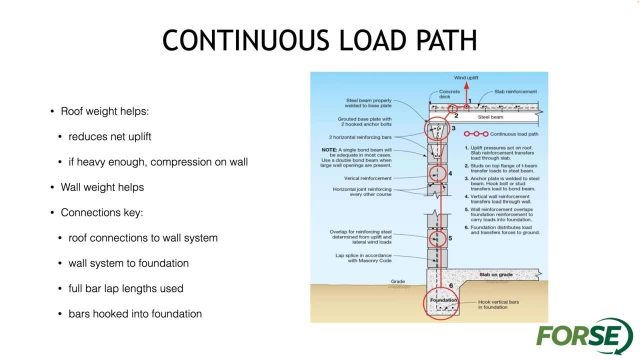 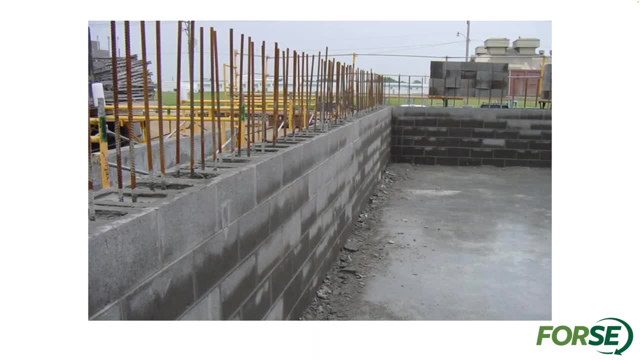 making sure that we have a storm shelter that's able to function without, you know, anything kind of failing here. looking at kind of the practical side of what does that look like? you know, storm shelters do have walls that are reinforced at eight inches on center and they're probably 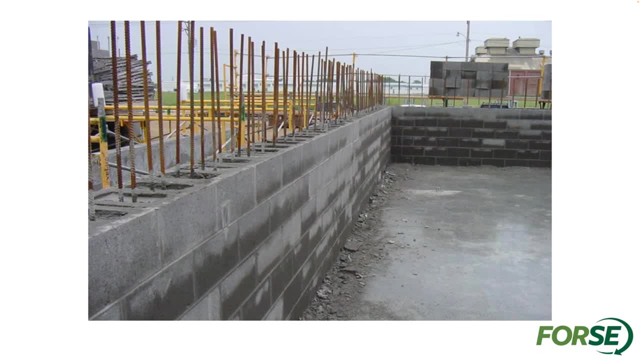 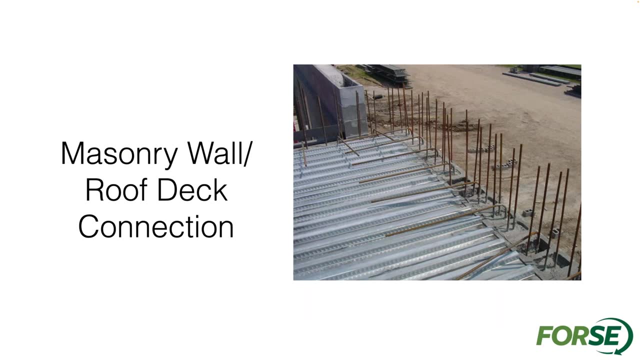 going to be doubly reinforced. so it's going to be a lot of reinforcements that are going to be added in these design situations. you know, like I said, though, the having the hooks and the ties into the roof deck, the roofs have, is going to be really important to making sure those storm shelter connections uh maintain. 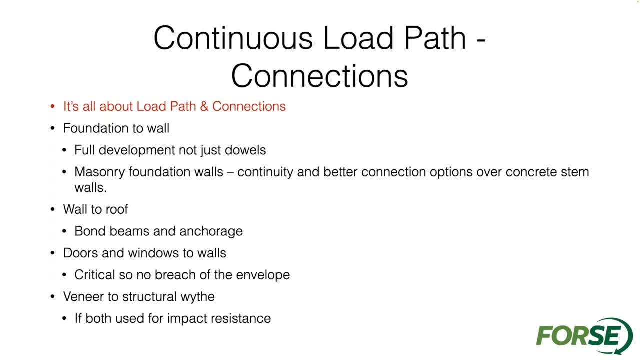 their integrity. so it's all about load path and connections: foundation to wall- fully developed, not just dowels- uh, masonry foundation walls. continuity- better, uh connection options over the concrete stem walls- uh yeah, having similar material all the way down to the actual footer is definitely going to give us a better continuity. we're not switching and and and having different. 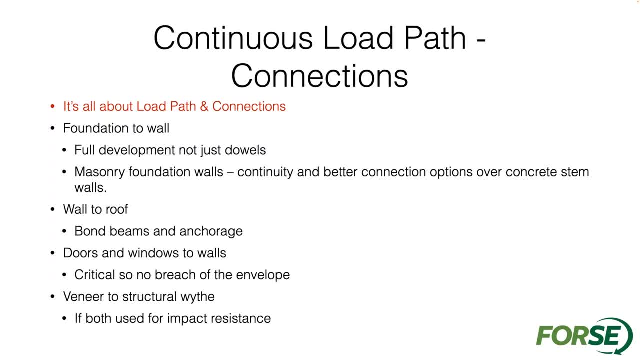 bars and doubles and wrong locations and stuff like that. we have a good continuity between them and we take nature all the way down the foundation and wall to the roof, making sure that we have bond beans. we're probably going to be grouted solid, so we don't have to worry about. 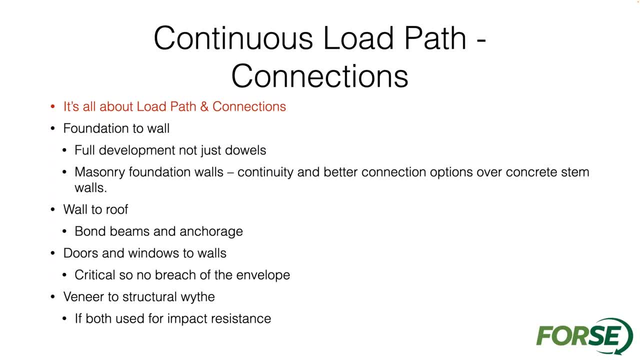 bars being in ungrounded cells, but making sure that we have bond beams and and then anchors. at the top we have doors and windows, uh, two walls and making sure that all of those uh have continuity anytime we get into any of these storm shelters we look at. 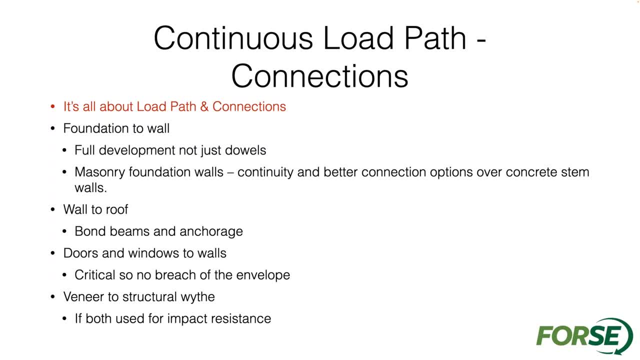 all these different connections and the reinforcement that we have within these walls and and making sure that we don't have unnecessarily uh uh small walls either. we want to make sure that we take control joints out and make these walls, uh, as continuous as possible, both vertically and 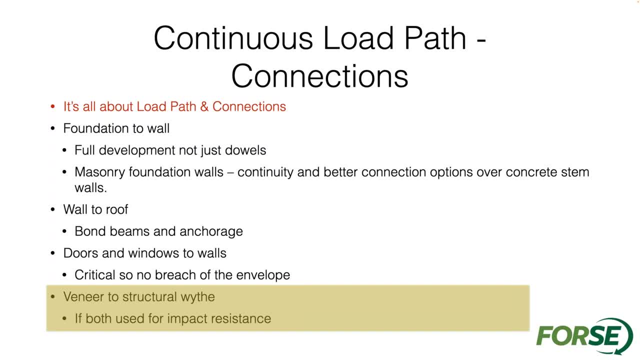 horizontally a veneer to structural life if it's used for impact resistance. you can certainly have a structural brick veneer, which would be something that would work very good for impact resistance, and then that could also, you know, be something that we tie back to the structural wall, or maybe it's a single wipe design. 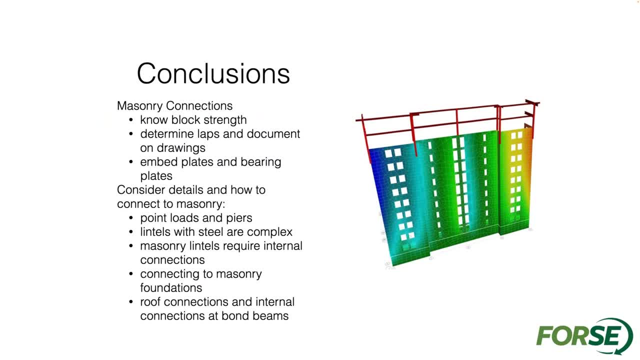 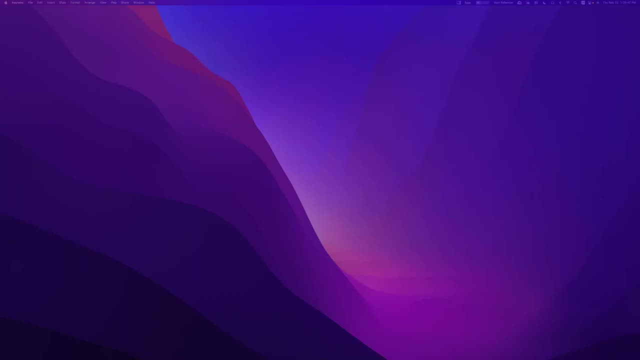 so masonry connections. we need to know and make sure that we utilize that full strength that we talked about this morning- laps and document on drawings and embed plates and a lot of things to consider there- for connections to masonry. so i'm going to switch over to um detailing for masonry. 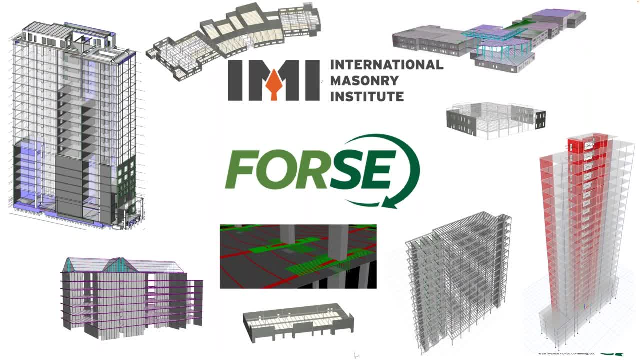 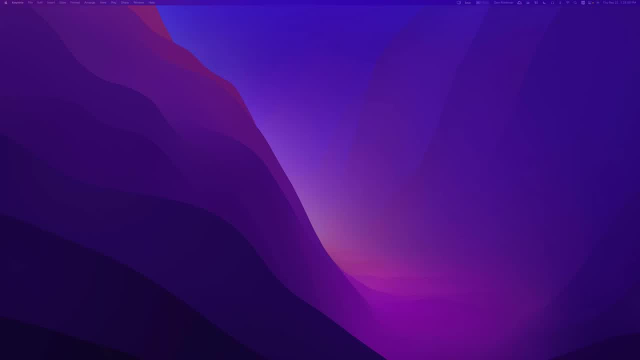 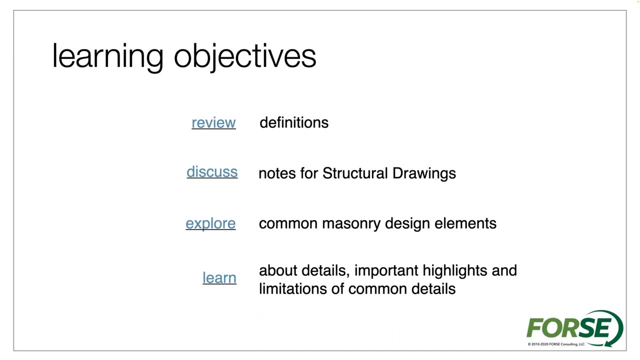 in addition to some of those connection designs that we're looking at and finally getting you know whether it's um specifications for materials or it's um, you know, connections and things like that, so that the masonry is actually. we're going to be considering that, that a lot, and you know it's going to be very important that they're also, uh, not just as like. 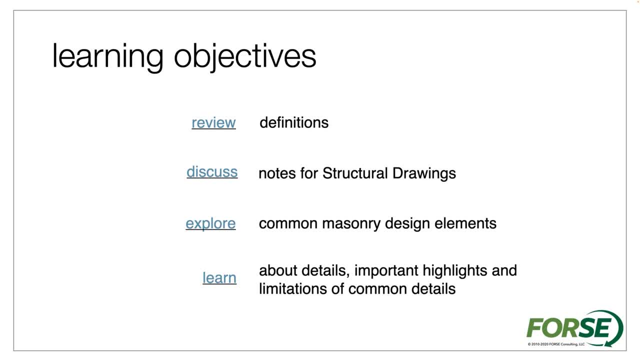 uh, you know, moving forward, um, but that it's that it's. it's almost always the case that you know that if we want to, uh, you know, change the design, you know, then it's going to have to take some time. But kind of bringing all this together and making sure that we get design drawings that actually meet our design intent is really obviously going to be pretty important for us as designers. 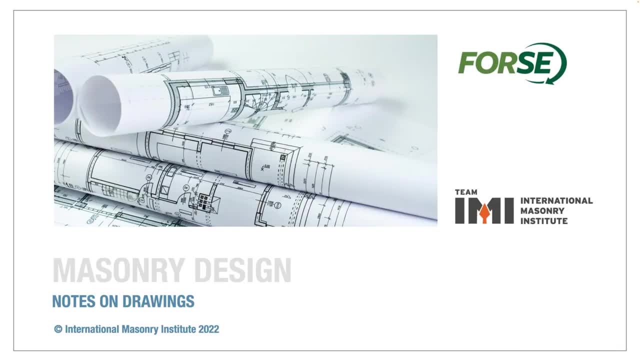 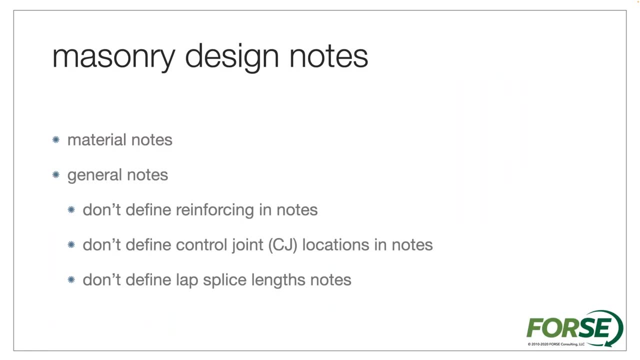 So different notes that we want to put on drawings. I have some do's and don'ts that I think are pretty important and we'll kind of cover some of those here. So material notes and things that we put on drawings, we have general notes. 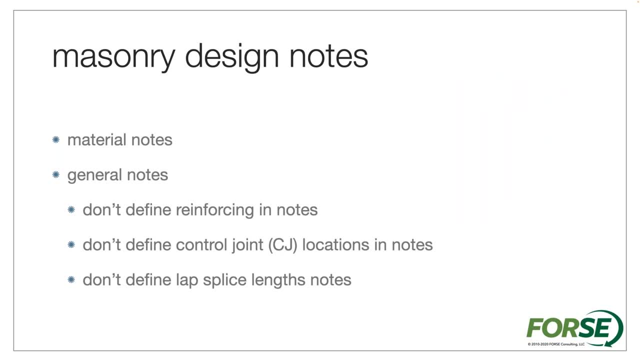 What I try to recommend is: don't try to define reinforcing for masonry in the notes. I mean, we wouldn't do that type of thing for concrete slabs or concrete walls and other important structural elements. We want to make sure that we don't try to do that for masonry as well. 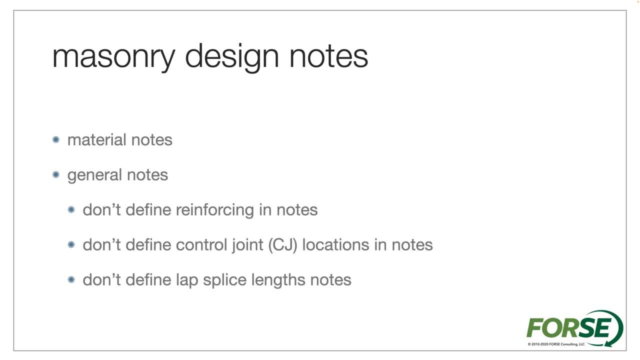 We don't put in catch-all notes where we try to make sure that we have a certain amount of reinforcement in there. I mean, make sure that we do that, Make sure that we actually label it appropriately. Don't define control joint locations in notes. 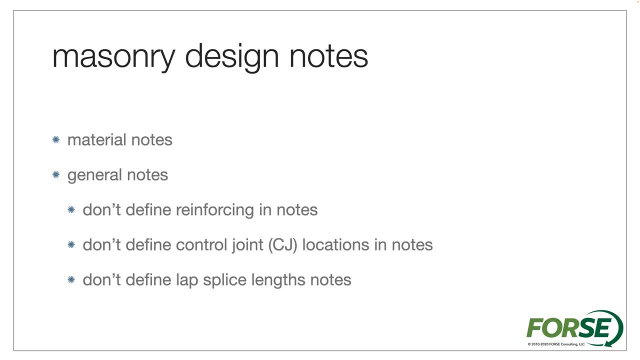 You know we talked about that in the movement joint section. We want to make sure that we put our control joints on elevations or on plans to try to make sure that those are very clearly defined for our contractors and those that are building the masonry walls. 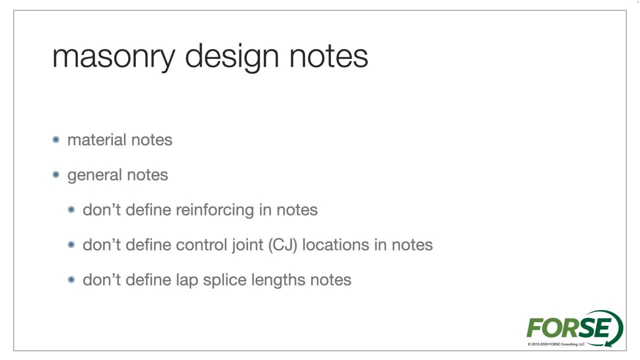 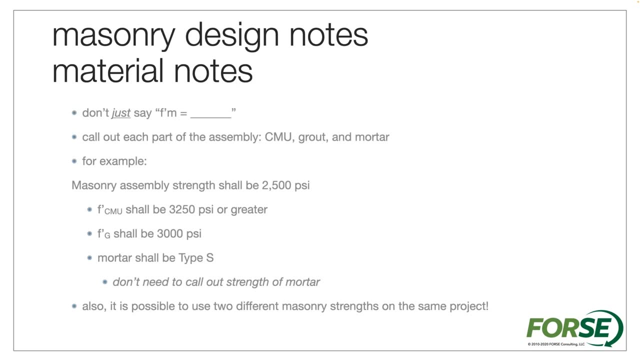 And we also don't want to put lap lengths in notes. No, 48 times diameter bar. We talked about that this morning, How that works. That's something we don't want to use, You know, for the design strengths, we talked about this in terms of F, prime, M. 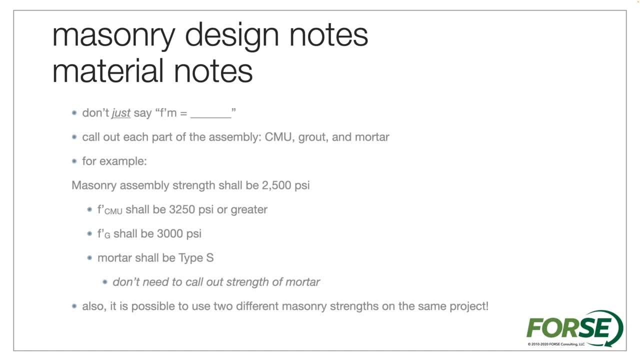 We don't want to just call it the strength of masonry, We want to call it each individual piece, We want to call it the blocks, We want to call out the grout strengths and the mortar types and make sure that that's all working together. 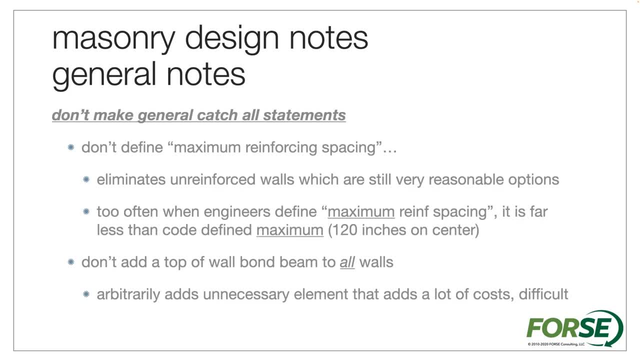 When I say: don't define maximum reinforcing spacing, that eliminates unreinforced walls. I think that's a very reasonable option for partition walls. And you know, any time as structural engineers, if we put a kind of a catch-all or cover or but statement on there in terms of maximum reinforcement spacing, you know, then we eliminate the possibility for unreinforced walls or make that more confusing. 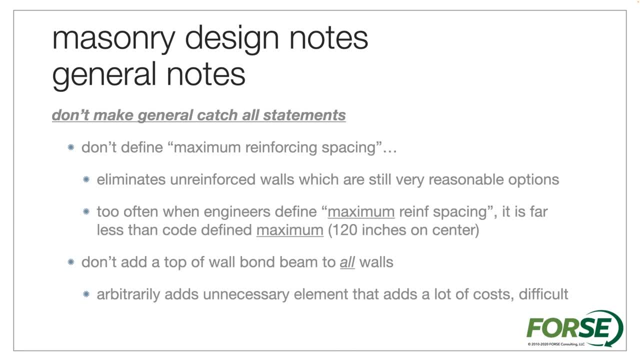 And so we have to be careful with that And remember that when we do start to reinforce walls, we can reinforce them at even 10 feet on center. If it's a shear wall, 8 feet on center, we really can't have a minimum amount of reinforcement. 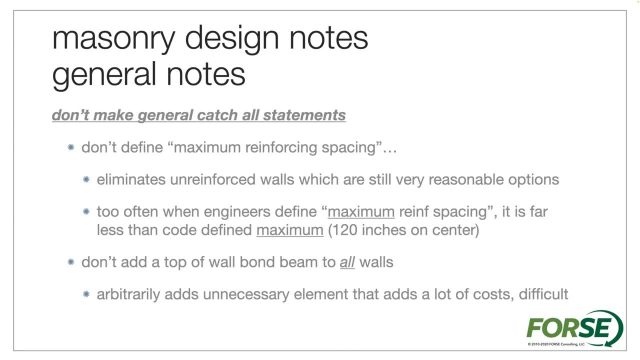 Two walls. we don't want to have to add a top-of-wall bond beam to all walls, especially those partition walls can be pretty costly to add, So putting that in the notes. I've seen notes that indicate that we want to have a bond beam at the top of every wall. 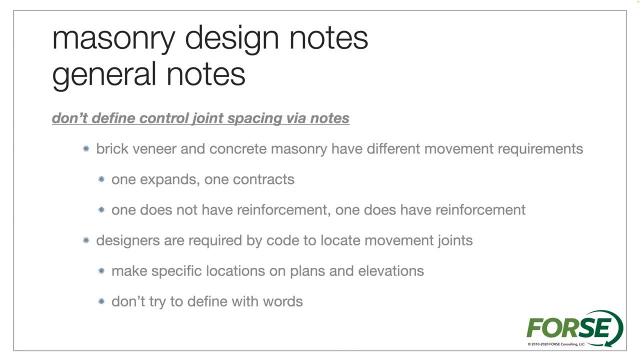 That can be problematic as well. When I say don't define control joints via notes, I mean we have different requirements. We have brick veneer or we have structural brick or we have concrete masonry. that have different movement requirements. You know expanding and contracting. they have different widths to the joints that we have to define. 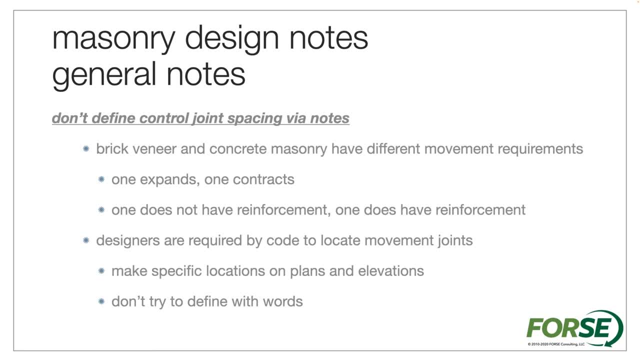 So we want to make sure that we are as specific as possible about those. Designers are required to locate those joints. You know, we can't just put in the, you know no more than 25 feet, We can't put those in notes. 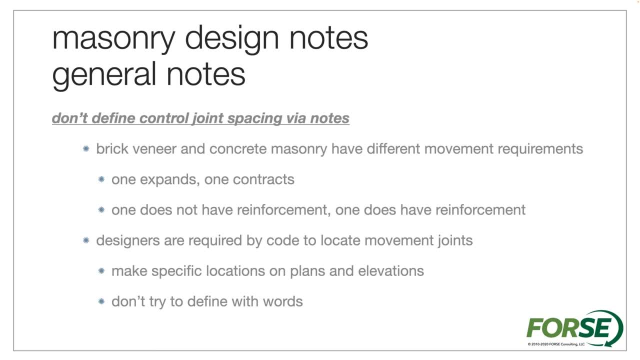 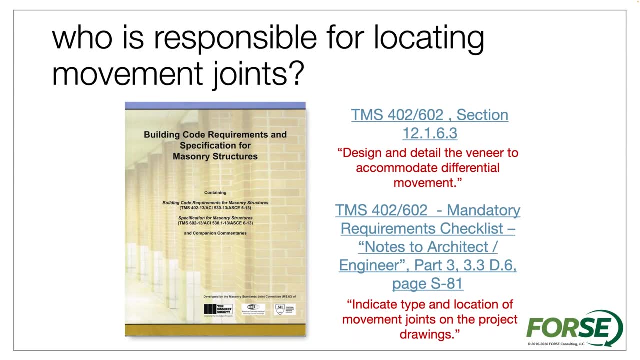 We can't just try to describe. you know where they go. We actually have to specifically try to locate them. Don't try to define it with words. We want to make sure that we are as specific as possible about those joints. So that's one section of the code that actually says design and detail, the veneer to accommodate differential movement and indicate the type and location of movement. joints and project drawings. 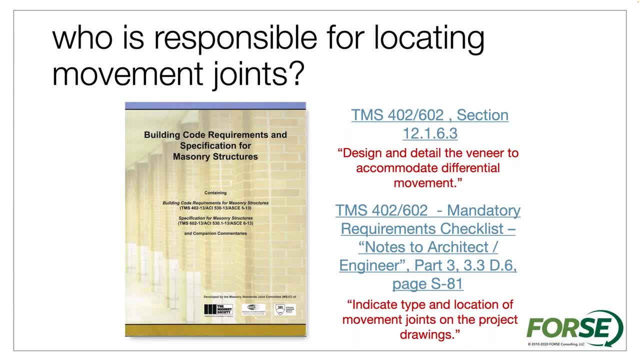 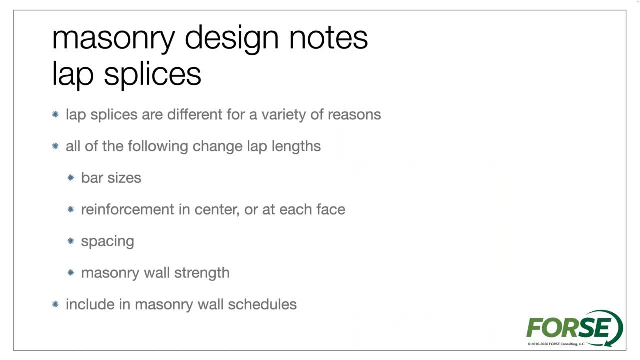 I mean, the code is pretty explicit with wanting us to locate those directly and exactly what they look like on the drawings. Masonry design notes and lap splices. Again, lap splices are different for a variety of reasons. We talked about that a little bit this morning when we were talking about reinforcement. 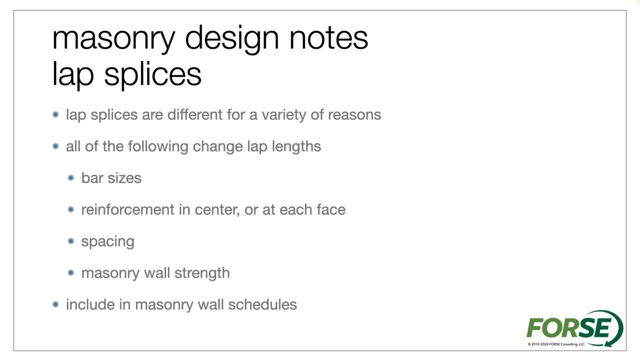 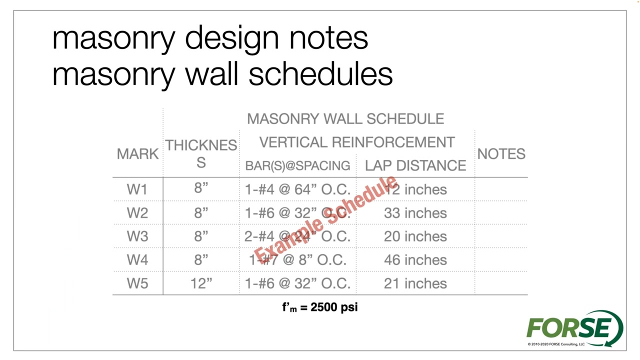 You know all the different variables that come into determining lap lengths. bar sizes certainly have a lot to play, But reinforcement in the center or at each face, that changes lap lengths. Our reinforcement spacing can change Our masonry strength, And so we just want to make sure that we have, maybe lap lengths in our schedules or we have them very explicit in terms of you know the strength of masonry used and then you know the lap lengths that are used. 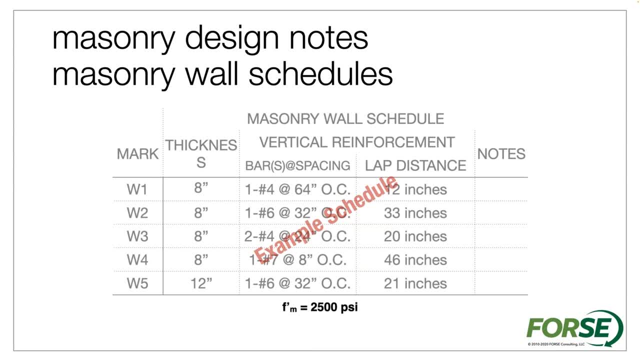 Again, here we have a W1.. That has a number 4 bar that only has to be lapped at 12 inches. And then we have W3 with that number 4 bar has to be lapped at 20 inches. Just different requirements for different situations. 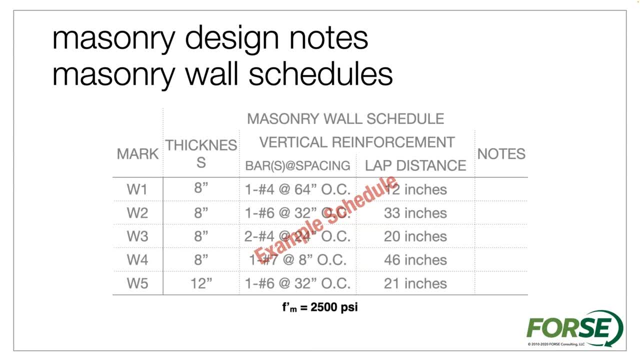 If we have W1 on 90% of the project and we just have a couple small walls for W3, we don't want to lap our number 4 bar 20 inches everywhere. If we can be explicit about this, then that can certainly help design-wise. 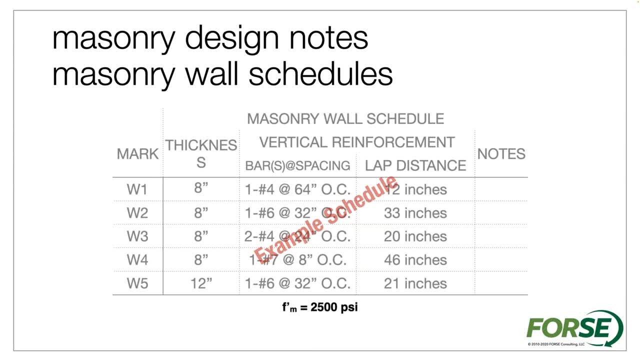 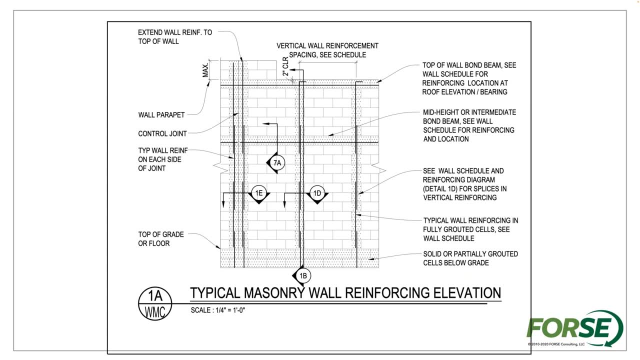 You know detailing. You know details that really show a lot of information I think can be very helpful. You know some of these details in terms of a general layout for reinforcement can be very useful to contractors. You know where we want to grout, where we don't want to grout, where we want to lap the bars. 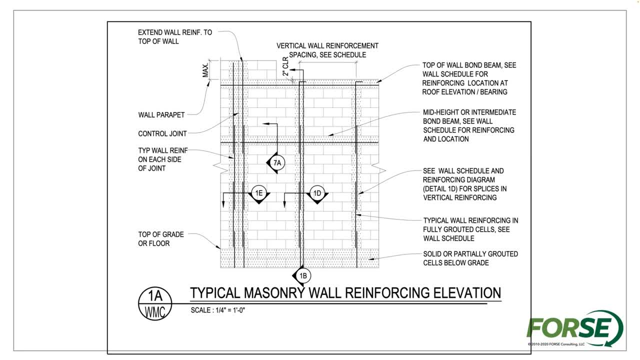 You know what some of those details look like. Do we want to use joint reinforcement? Do we want to use just a mid-height bond beam? You know all those different things that can be useful for whether it's an interior wall or exterior wall. 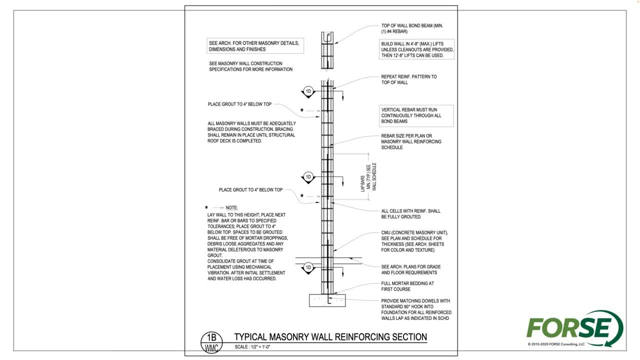 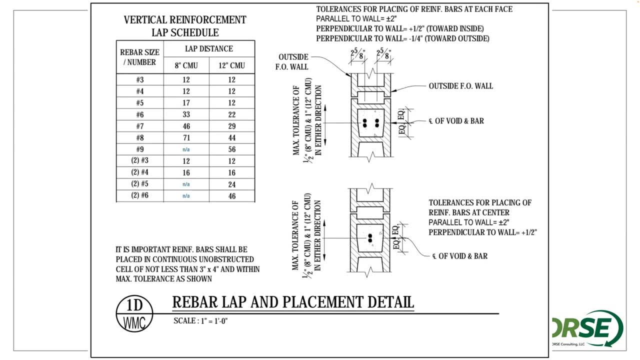 Both showing an elevation and then maybe a section, can really be helpful to determining some of that information. You know I mentioned this morning there was a code provision that showed the different locations and tolerances for reinforcement. So what we did? we just made a detail. 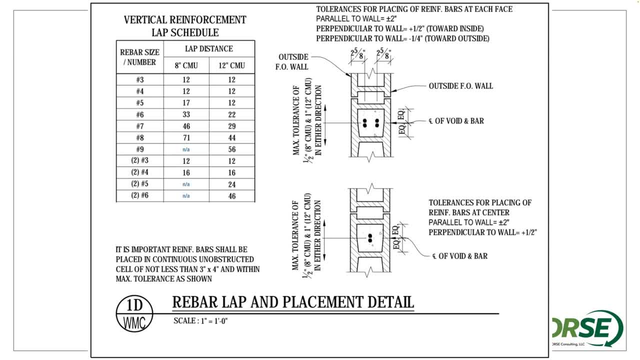 The detail, that kind of shows where the bars can be located. You know how they should be spliced, How they can be. you know the tolerance that we have for the wall. That makes it really, really direct in terms of. 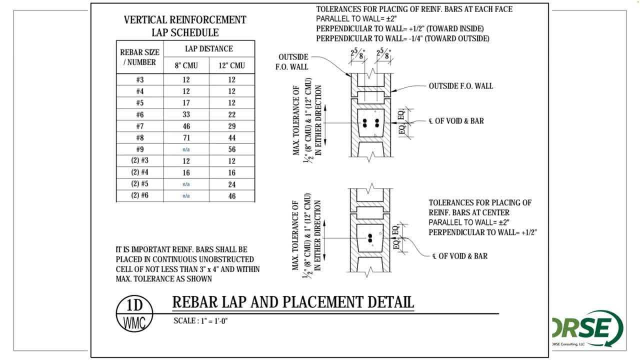 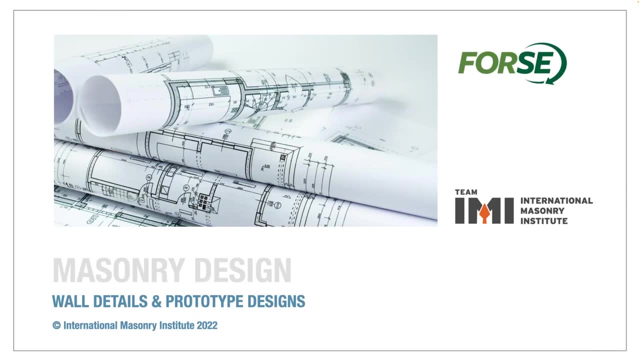 You know how we can place those bars within walls, And then certainly any time that we're out to the job site inspecting a project, we have that information right in front of us, So we know exactly what bar location to expect. Next, we want to talk a little bit about some of these wall details, prototypes and designs. 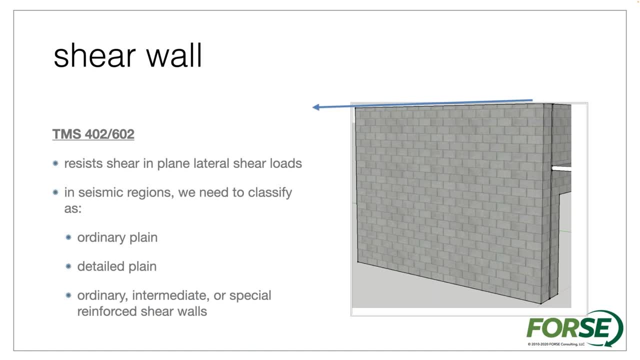 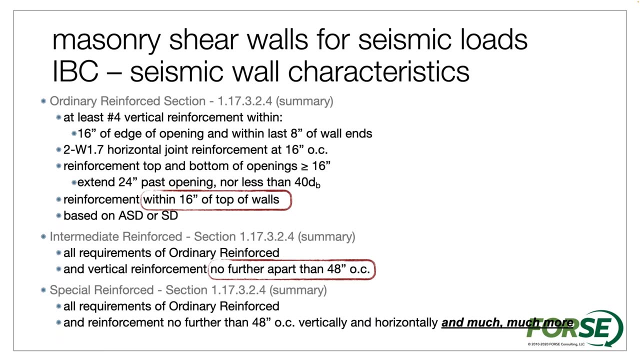 You know again, we talked about shear walls, We talked about the different types of shear walls, We talked about provisions for shear walls. I highlighted a couple of items there because those are shear wall requirements: Reinforcement within the top of the walls. 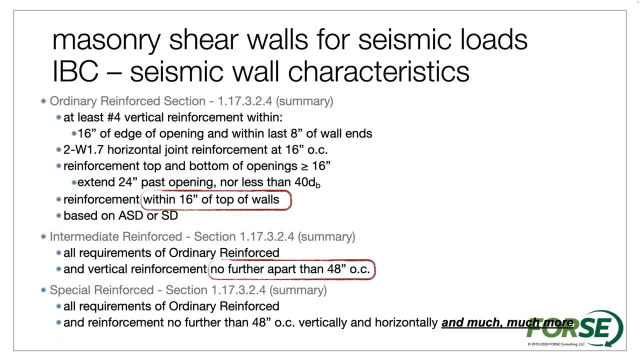 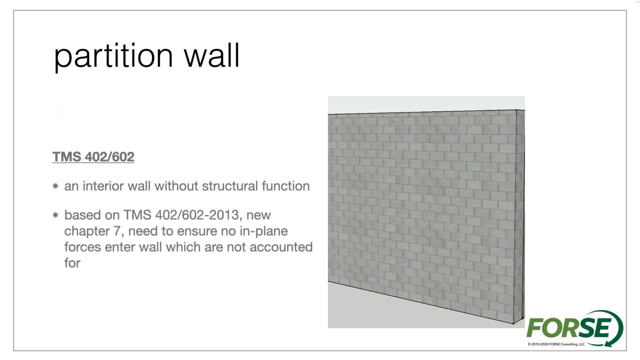 Vertical reinforcement no further than 48 inches on center. Really really important to consider those items for shear walls. Partition walls are not shear walls, You know. so we want to make sure that, as the code gives us the ability to isolate those elements and really lightly reinforce those elements, 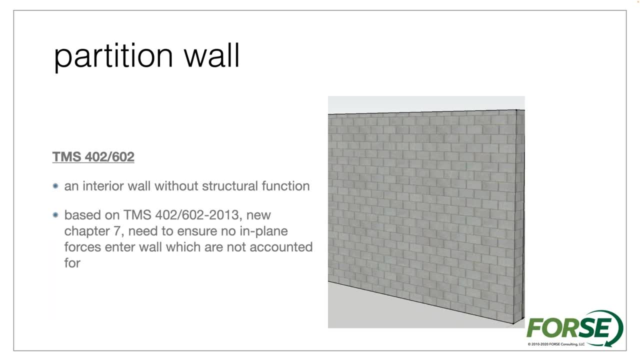 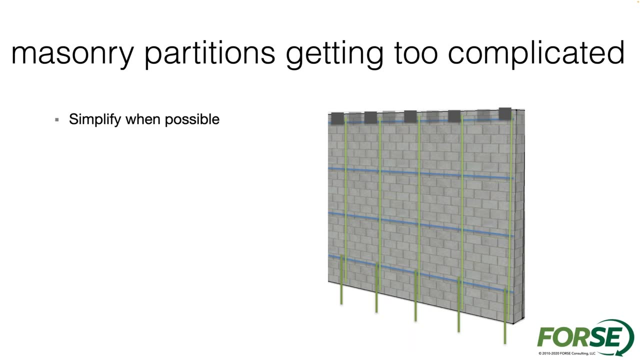 You know, when we look at Value engineering for partition walls We look at simplifying those walls, trying to make sure that we don't have any unintended horizontal. I've seen partition walls that had horizontal reinforcement in a low seismic area. So seismic design categories A, B and C indeed don't need that horizontal reinforcement. 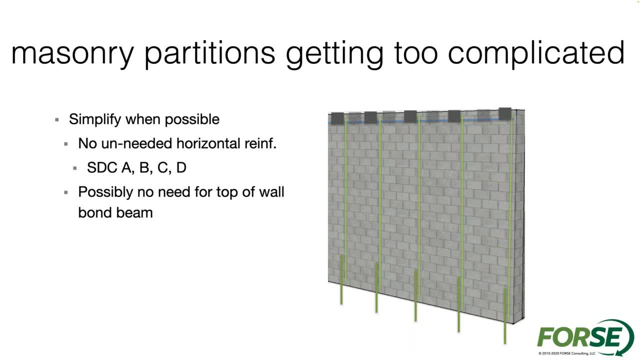 Possibly no need for top of wall bond beam. I mean, you know that's up there for shear walls. That's not necessarily something that we need. Minimize the vertical reinforcement. We don't need to reinforce that 48 inches on center. 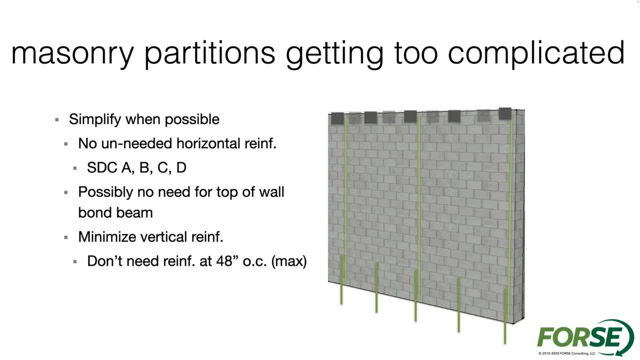 So that can certainly take a lot of cost, Grout reinforcement out of the wall and also limits the amount of connections that we would need at the top of the wall. We only need to connect the wall, Maybe where we have bars located, and then maybe the bottom of the wall. 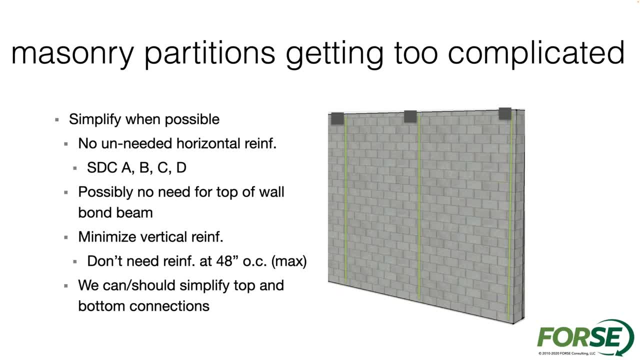 We really don't need much of any type of connection. Maybe we had some minimal connections at the bottom or none at all: Partition walls. Partition walls don't have to have a mechanical connection Or if they do, it can be a very light, simple dowel at the bottom. 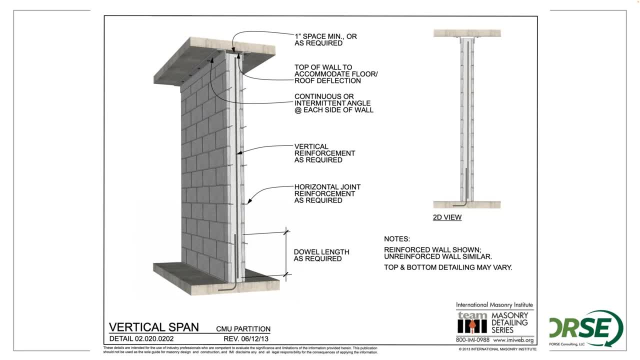 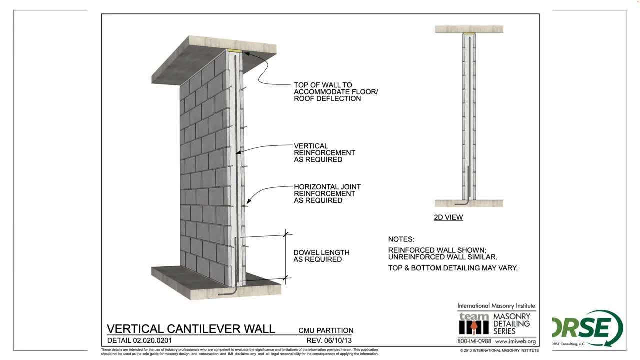 You know. so any details with the 3D detail or just some sections showing that light reinforcement or lightly connected at the top, No bond beam at the top- can be really important. Sometimes we have a vertical cantilevered wall for a partition wall there. 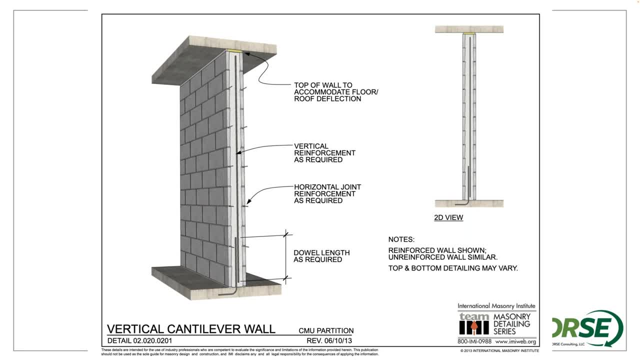 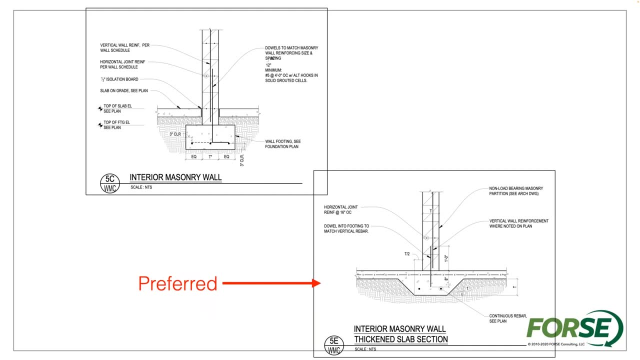 You certainly want to have the dowel at the bottom, But what does that look like at the top? Or maybe we do have it connected at the top. Again, what does that connection look like? What does the base of a partition wall look like? 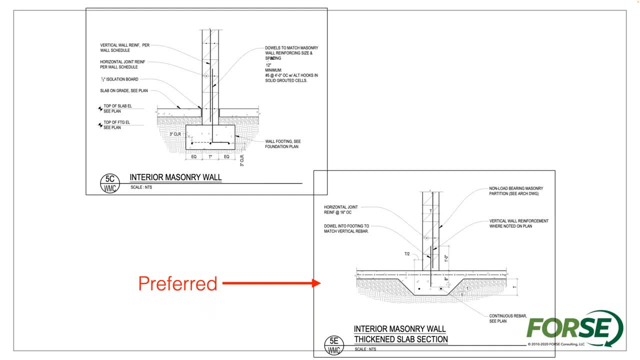 Again, the lighter the dowel can be, the simpler that can be to install. You don't need a separate footing, You usually just need some sort of. it depends on the soil conditions, but oftentimes just a thickened slab and a simple dowel can work very well. 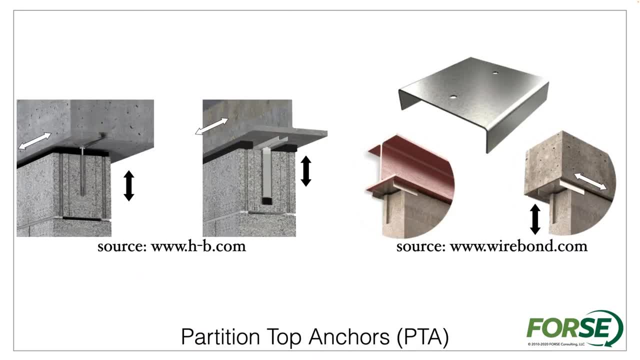 We don't need to have usually that developed Top of wall anchors. I mean, there's a lot to be said here. We have a lot of different ways to connect the top of the wall, But the lighter and lighter the connection is, the easier it is to perform. 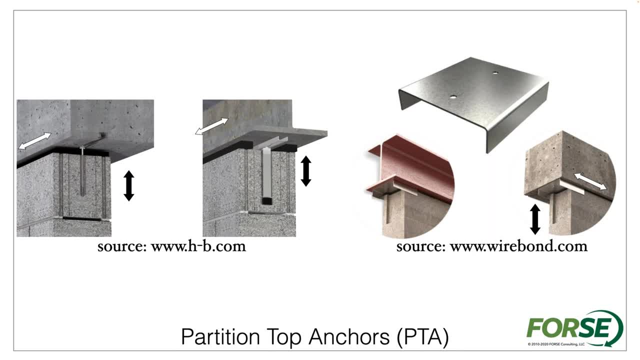 And just trying to utilize some of these connections Architecturally, I've seen more and more of the details on the left where we have a connector that's just enclosed and say, a top of wall that may be grouted solid, you know, or some limited, you know, connection at the top. 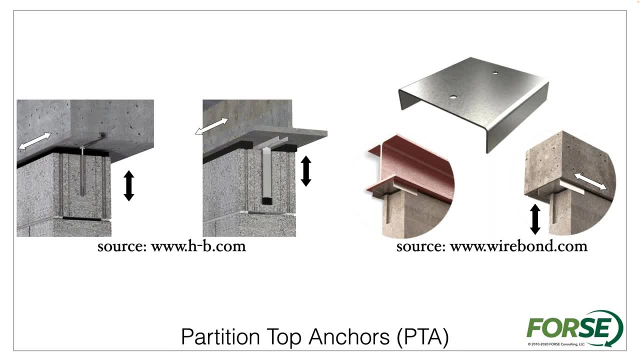 That allows for the wall to move in plane, but it doesn't allow it to move out of plane. So there's some nice connectors that are from Hohmann and Bedard, but then there's also other manufacturers, suppliers, that are giving us some of those as well. 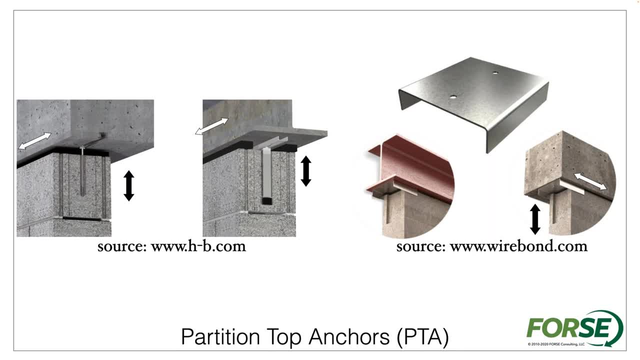 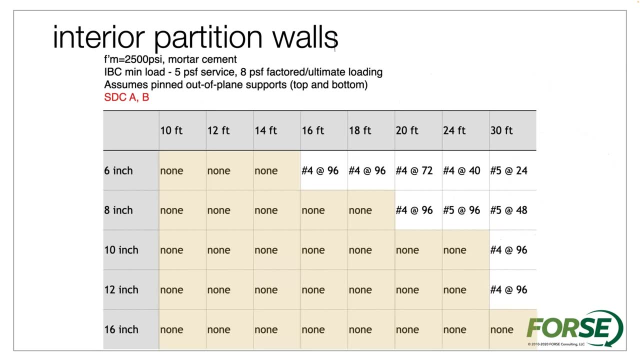 You have channel connections at the top that could be either designed or they could be a proprietary product as well. The other thing that we pointed to this a little bit this morning in terms of partition walls, You know the code is going to give you some requirements. 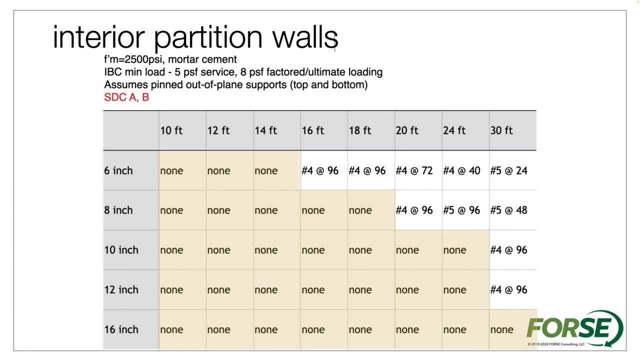 But there's also Just doing some design, quick calculations and seeing that most of your partition walls and seismic design categories A and B don't have to be reinforced. They're very lightly loaded. You know, even a six inch wall going 14 feet high doesn't have to have reinforcement. 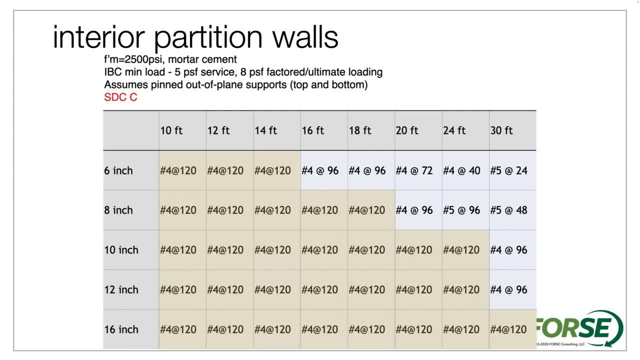 If you get into a higher, little slightly higher seismic design category or you like to put a little bit of reinforcement in your wall, You know this isn't really going to change your cost of your partition wall as much. Put a number four bar at 10 feet on center. 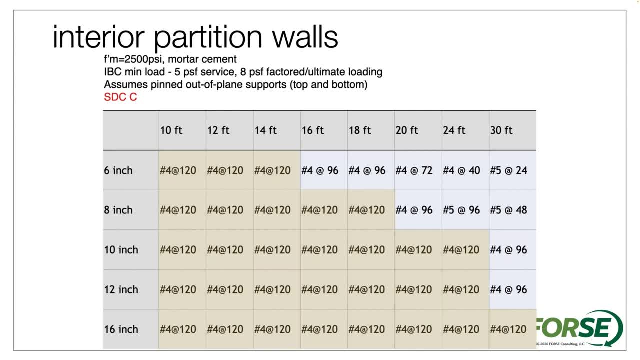 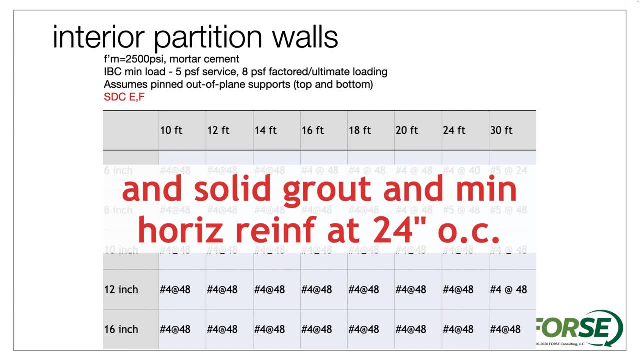 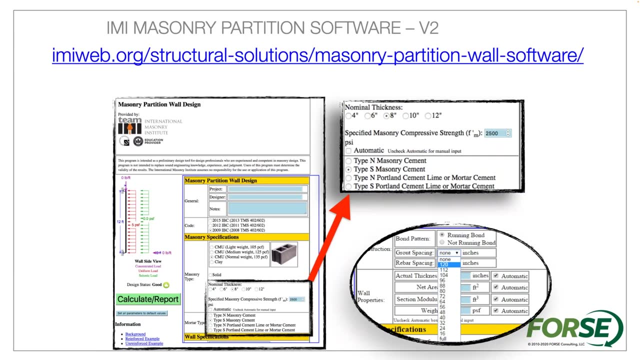 And that's still going to give you a little bit of reinforcement. It's not going to be a very efficient design. It's just seismic design- category D and E and F- where you need to add more and more reinforcement. You know, one of the very nice things that IMI did was they actually created a free online software tool that allows us to look at partition walls for a variety of loads, for a variety of different support conditions and thicknesses. that allows us to review some of these designs. 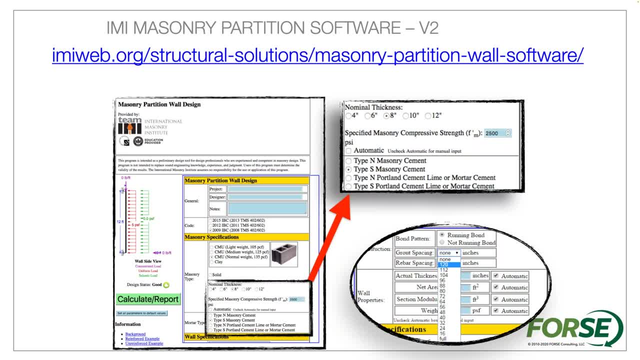 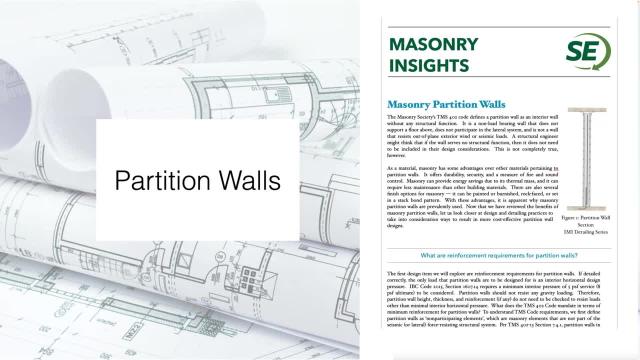 So you see the link here at the top. So partition walls can certainly be much, much more efficient, And so we actually created again These papers that I do show. I think I mentioned this morning. there's stuff that all is available. You can get in contact with me and I can send their free. they're just they're been paid for by somebody else, so it's just free information that we can provide to you that's based on either the masonry code or NCMA guide or a combination of the two. 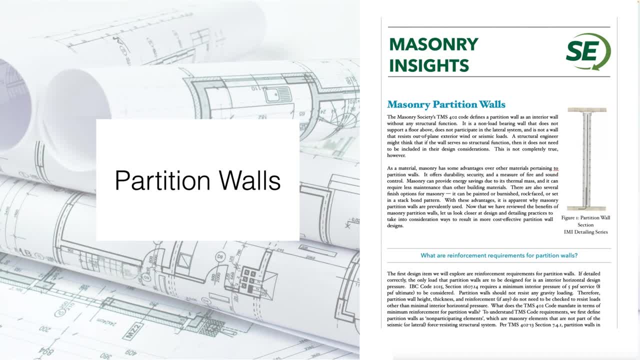 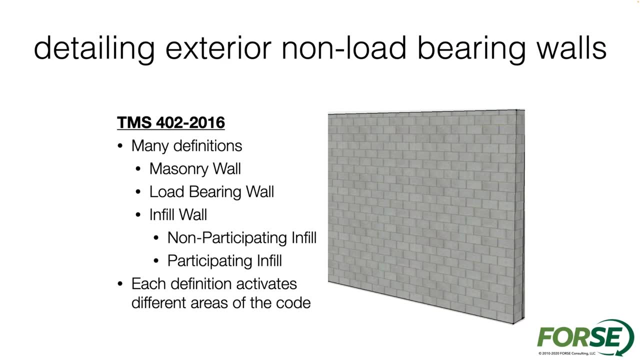 And so that that's where we come up with some of these papers. So we both have interior partitions and exterior non-load barriers, so the non-participating infield walls. There's a lot of different types of definitions, so we have to be careful in terms of what types of wall that we have. 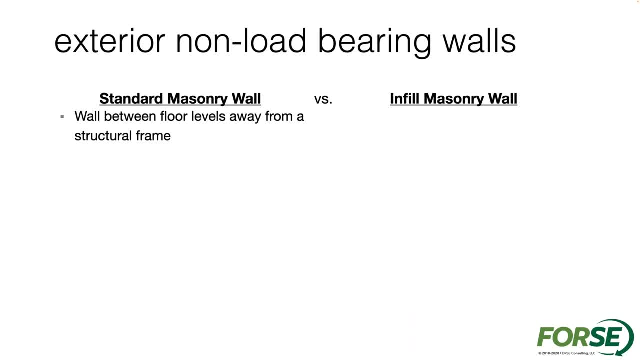 Standard masonry wall is going to be a wall between floors, away from a frame, and infield wall is going to be something that's going to be built in the same plane, bounded by a structural frame. So they're they're quite a bit different. 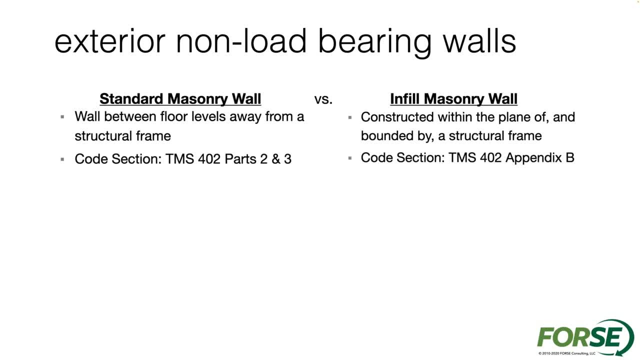 They have different code sections that are going to be looking at them. there's going to be different design provisions. we have a few factors that change When we look at the different types of different types of design. so we have to be sure that we're infield walls, that we're detailing it correctly. I mean it's going to look the same. 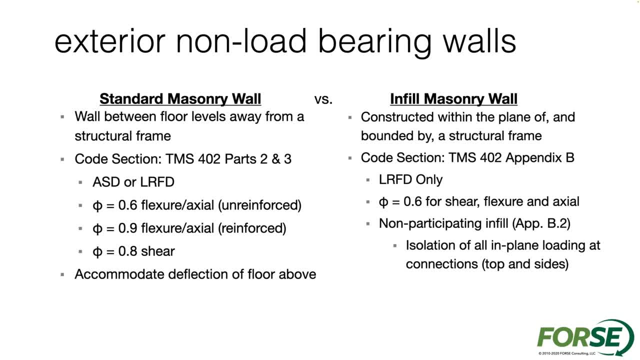 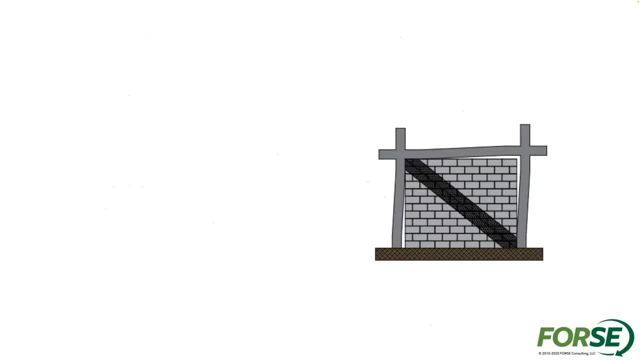 It's going to act the same. it's going to be pretty similar. so what we have, we quantify this is going to be pretty important In terms of what types of design that we have. anytime that we have an infield wall, we're going to have some sort of a strut that's going to be created because we're going to be tight to the frame and we're going to have something that's going to be having different types of design requirements. so, again, it's one of those. 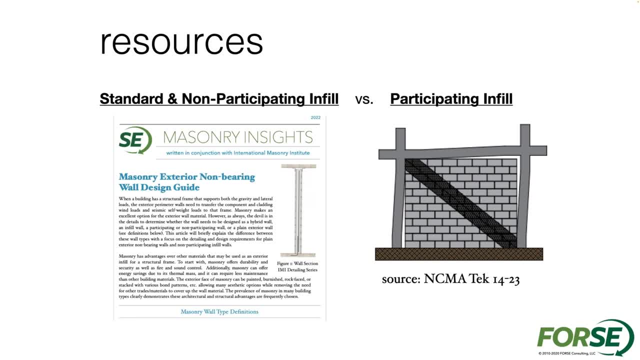 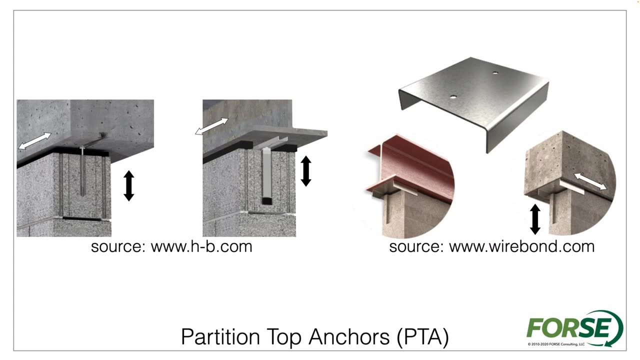 We thought would make sense to put together a design guide or a guide to give people a little bit more direction so that we can do Do these designs efficiently. You know what I looked at: the some of the partition topic anchors. you know a lot of those anchors are going to be pretty similar to what we had for interior partition walls. 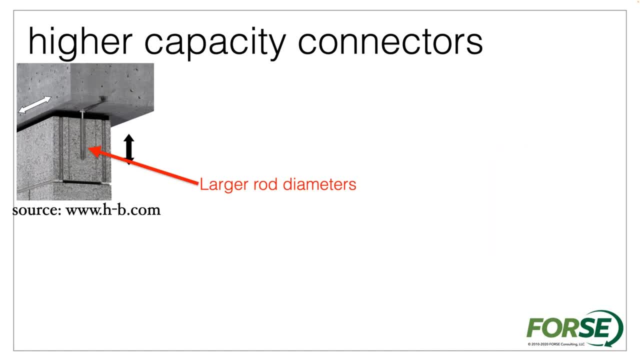 You know, probably to use this on an extra wall- if you think about what the differences are going to be, Certainly you're going to be have some higher demand. you're going to have a higher load demand. we're going to have higher forces that we have to design for. 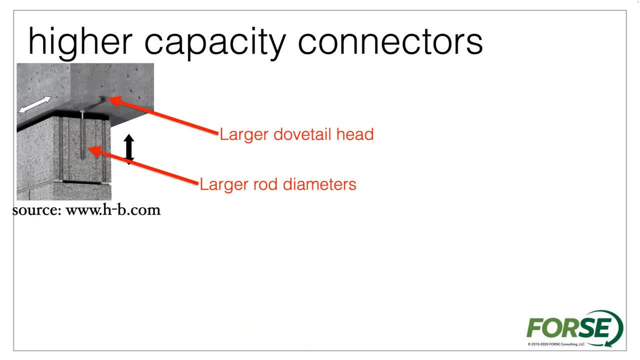 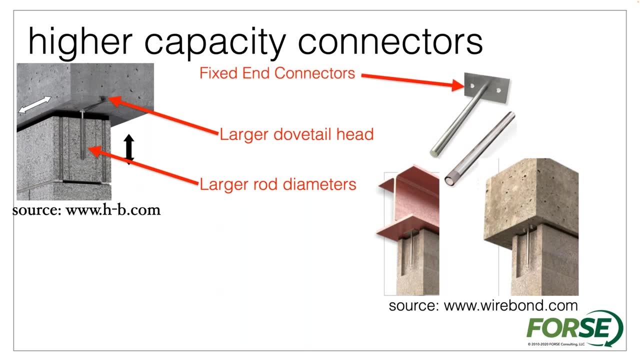 So we're probably going to have to use the larger Rod diameter, maybe a larger dovetail head. We have different types of manufacturers that are looking into this for us as we look at different types of connectors That make sure that we allow for the in plane movement and slipping vertically. 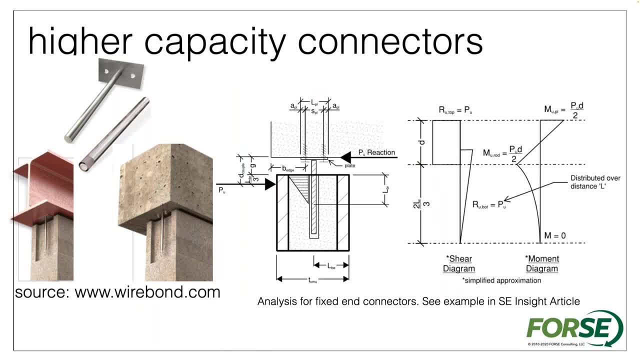 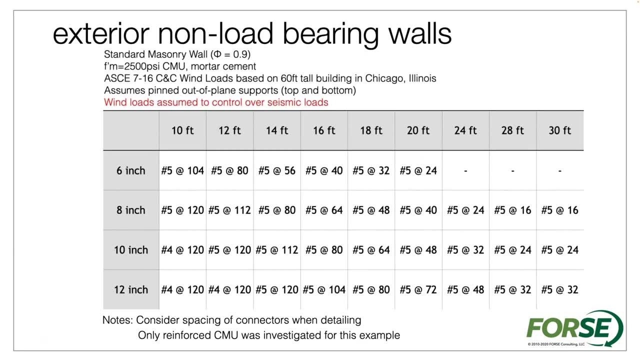 So again with the, with the guide, what we're trying to do is we're trying to give you guys some guidance in terms of the top of wall Connections that you guys would want to use, but then we get into some of the actual tables. again, this is pretty well defined. 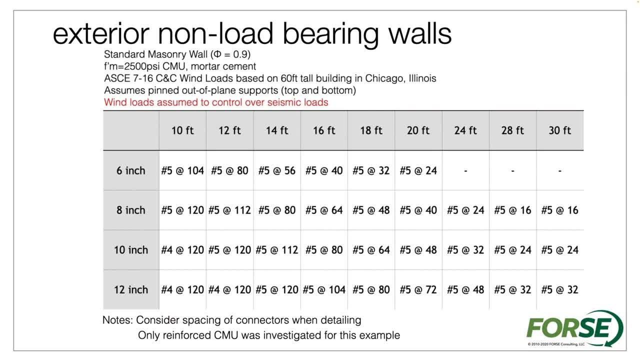 If we can look at different wind pressures, We can come up with the overall design guide. we don't have anything else going on here. So a standard wall is going to have six inches at 12 feet is going to be a five and 80.. 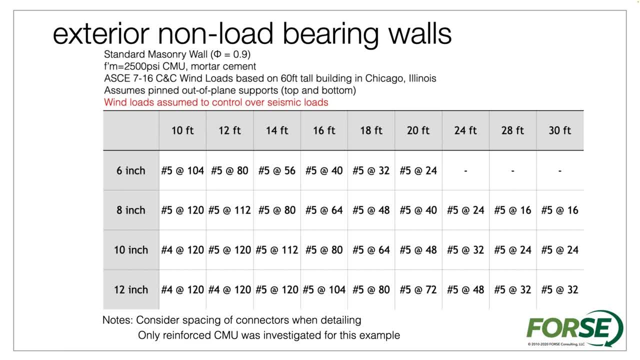 So that's going to be again just a standard mainstream exterior wall, not tied together. It turns into the mainstream, into the wall And again that six inch wall at 12 feet goes from five at 80 to five at 48. So you can see that the type of wall, how it's tied into the structure, what type of forces actually accumulate and actually get applied to the structure, can make a pretty big difference in the overall design. 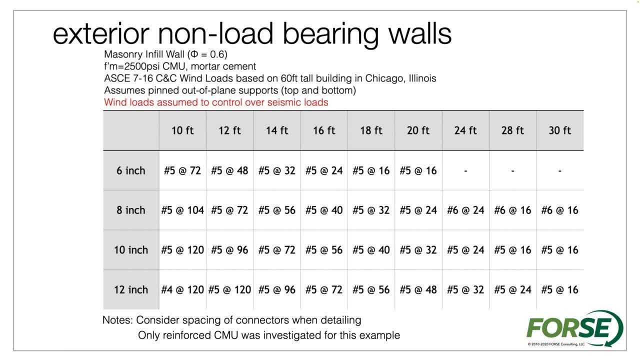 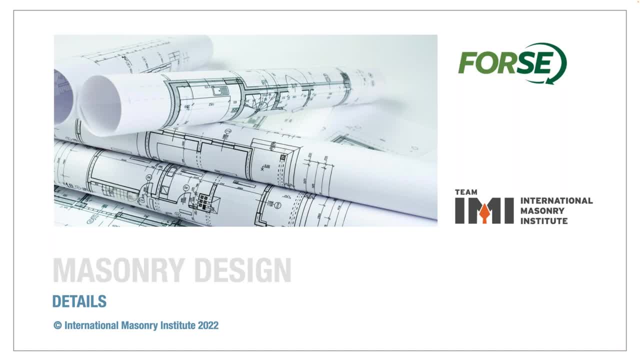 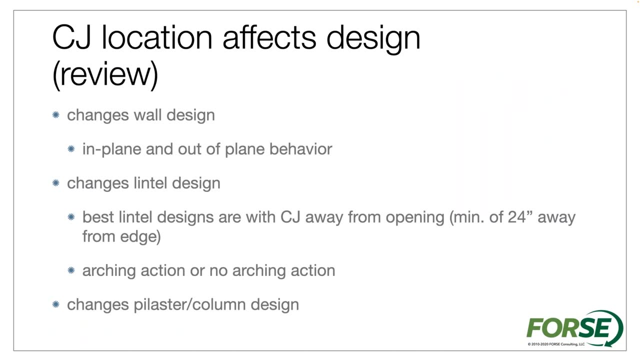 So we do want to use some care And exactly how the elements tie together. So we're going to have a little bit of a review maybe on control joints here. Control joint locations affects design. You know. we've talked about that quite a bit today. you know changes the wall design in plane out of plane behavior. 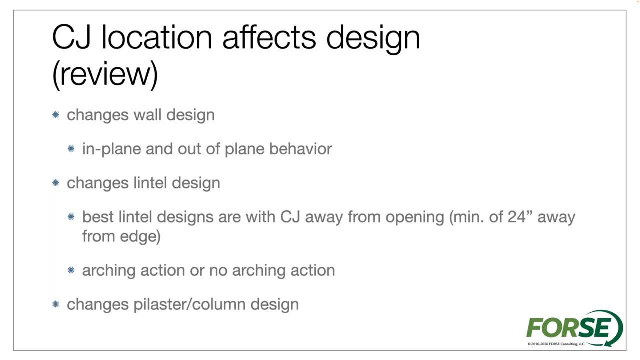 Certainly control joints closer together are going to have less in plane shear capacity of a wall. Control joint locations would certainly change our lintel designs. We talked about arching action. how important that is for an efficient mainstream lintel: Making sure that we have those joints away from the opening so that arching action can always occur. 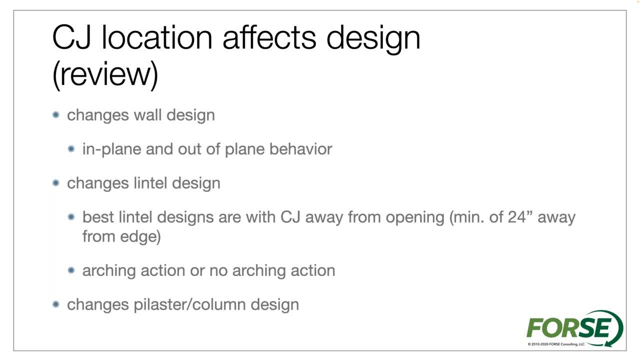 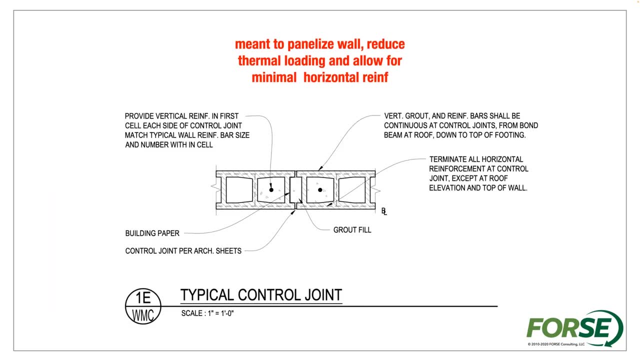 It would change a pilaster capacity depending on how much concrete and masonry would be tied into the design. What are some of the details look like for a control joint? I mean, there's different types of joints. You can put those in and we can actually have a filled with building paper. 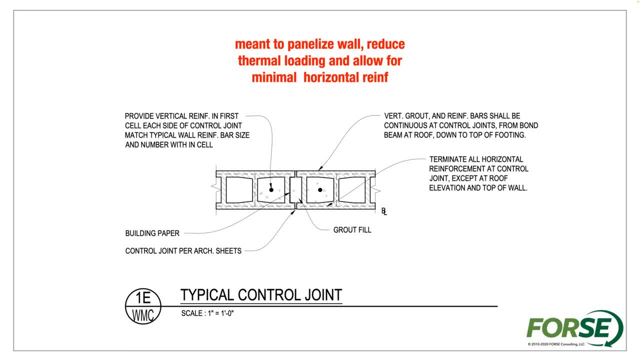 What is this called The Michigan joint? I think by some people. That's how we create some sort of a Grout key that's going to allow the wall to move in plane but it's going to have that key that's going to prevent it from moving out of plane relative to one another. 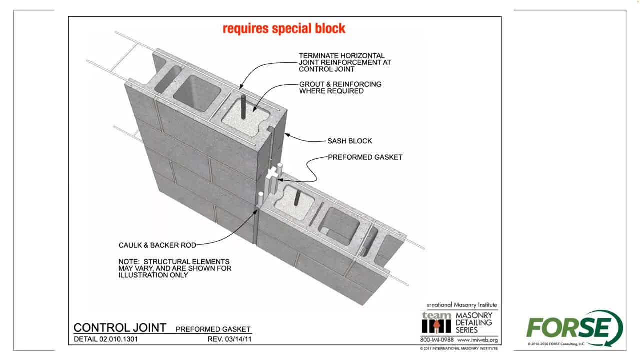 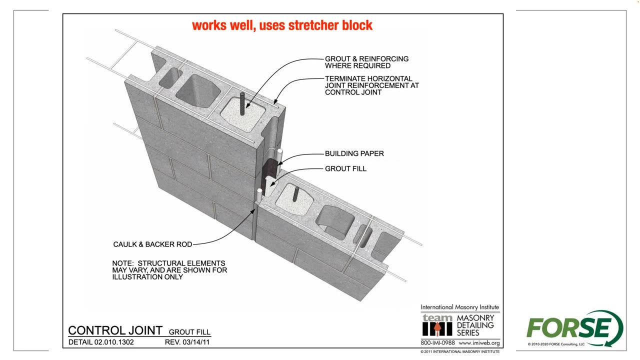 Certainly, there's the sash blocks that we have with the preformed gasket. Again, that's another one of those that allows the wall to move in plane but it doesn't allow it to move out of plane. Again, back to the 3D view of the Michigan joint. 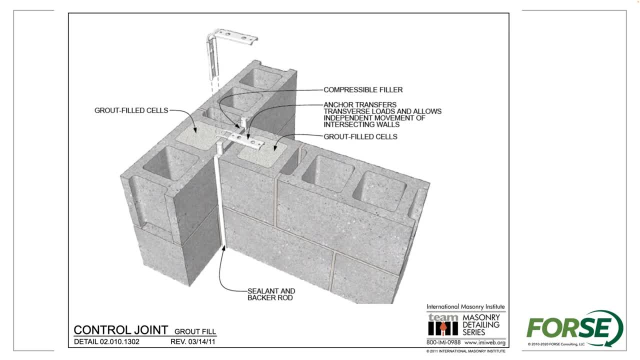 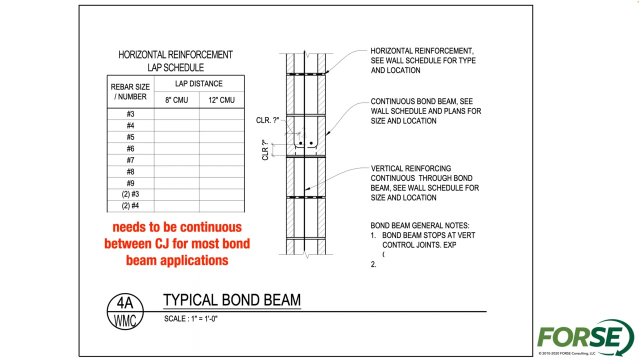 Certainly we can just put in two walls and we can have some sort of a proprietary connector that can tie together the two walls at a control joint as well. Other details to think about: what we have in terms of reinforcement, you know, at bond beams. how do we want to deal with bond beams and control joints? 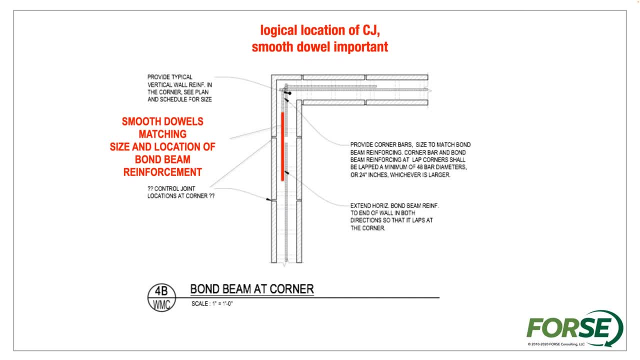 There's a lot of times that people are looking at bond beams to be continuous, except for maybe at control joints. We want to make sure that we have a smooth duct. We can go hand in hand with the control joint to look at what the bond beams are. 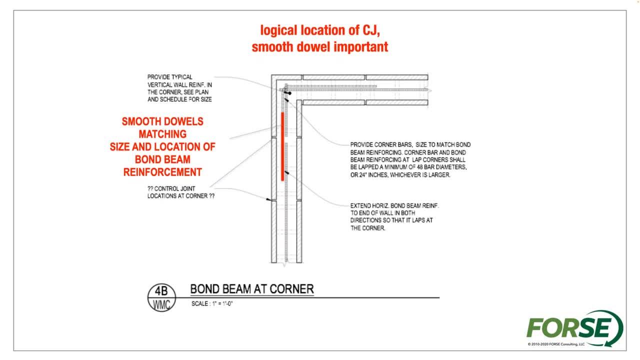 We need to have some sort of a dowel or some sort of means for the control joint to be effective at those locations Without tying the wall together. the purpose of the control joint is to allow those stresses to be relieved. So at those control joints we want to make sure that there's not anything tying those two walls together until the wall is moved or shrunk or relieves the stress enough. 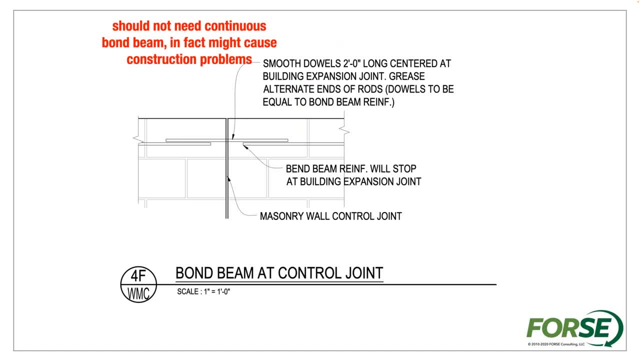 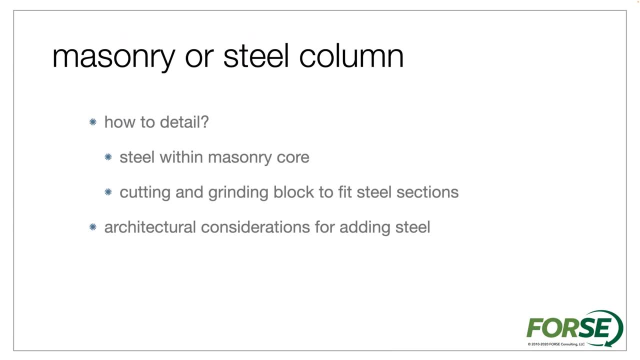 again a couple different details and you know kind of exactly what that looks like: uh, masonry or steel column, you know what do we have in terms of um? um, you know the elements that we have. or what do we need for, uh, vertical capacity, um, you know. 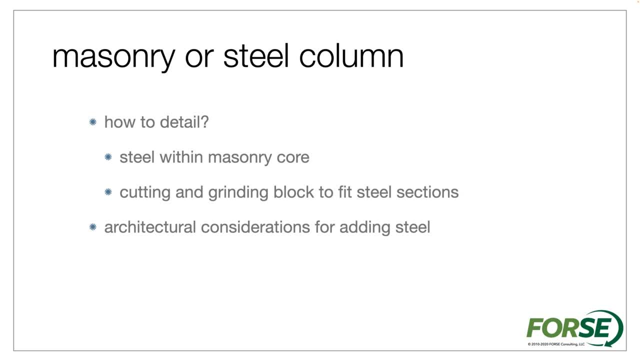 how do we detail it? masonry, uh, certainly can be, um, you know, develop plenty of vertical capacity in a in-plane masonry pier or a mystery pilaster that bumps out from the wall. so a lot of times adding in the steel is just not necessary. there's a lot of, i guess, the capacity that 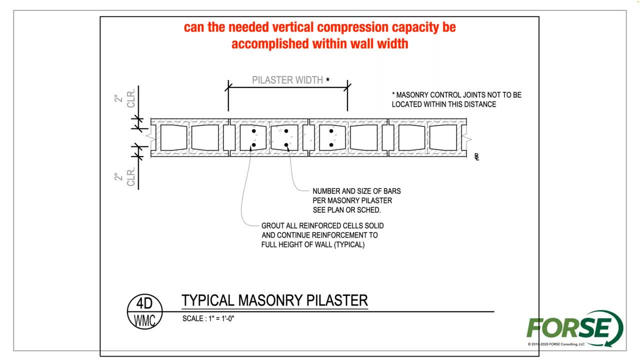 can be created here with this pilaster. obviously we don't want to have any control joints within the pilaster, within the width of the pilaster, but then it can be something that could be added on one side or each side. again, this can be a common location. 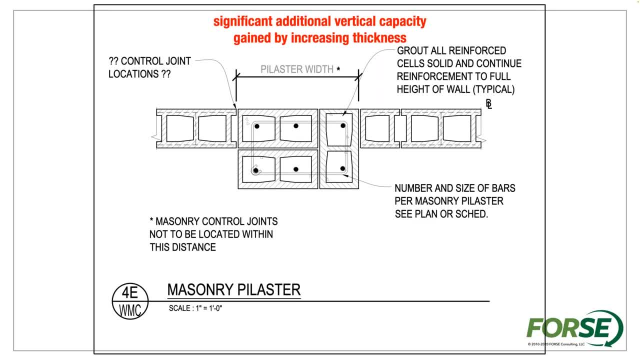 for control joints just from the sense of we have very different vertical loads that are perhaps being applied here. maybe they're going to have a lot of vertical load on the piers and not so much on the walls on each side. so putting in a control joint there would allow for a little bit of. 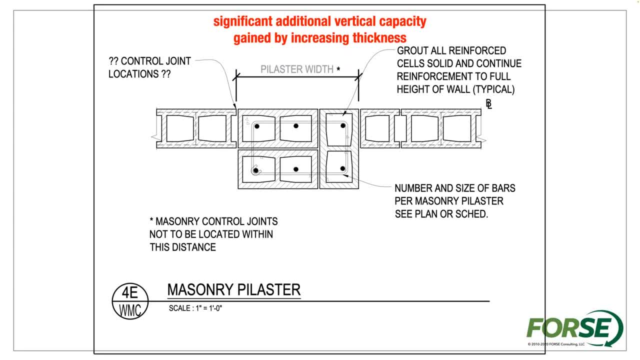 differential movement to occur. or maybe we want to use some of the the wall as a compression element and something to stiffen my pilaster. if i don't have quite this size of 16 by 24, if i had something smaller maybe i wanted to use some of the more wall length. so where those control joints going? 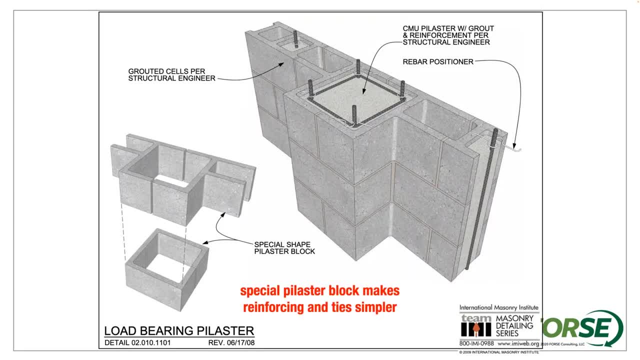 how that uh relates to the pilaster is going to be important. certainly with the pilasters there's specialty blocks that you can have supplied for the project and that can certainly help with getting vertical reinforcement ties and everything being continuous within the wall. you know things that. 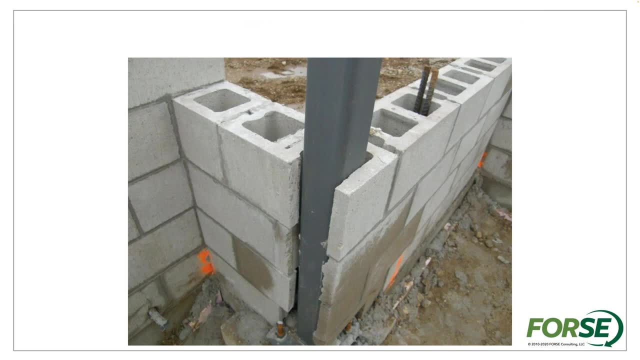 we try to avoid, uh in the mainstream industries you try to avoid uh having uh conflicts between materials, something that a steel frame and a masonry wall sometimes don't always work really well together. we talked about steel lentils and masonry walls. sometimes they don't work together. 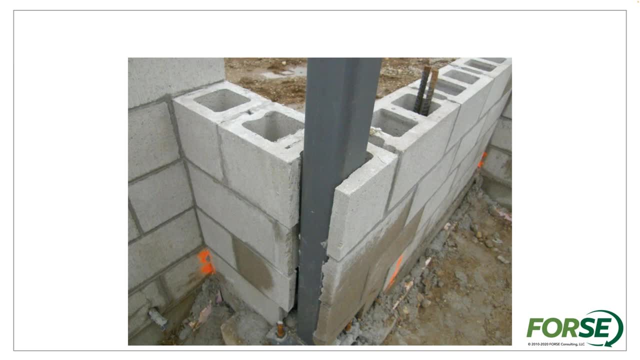 really well. if we take out some of the um uh, take out some of the uh conflicts between the two uh, it can certainly work a lot better and not have what's going to look like a pilaster because you're going to have to have some sort of a cover. 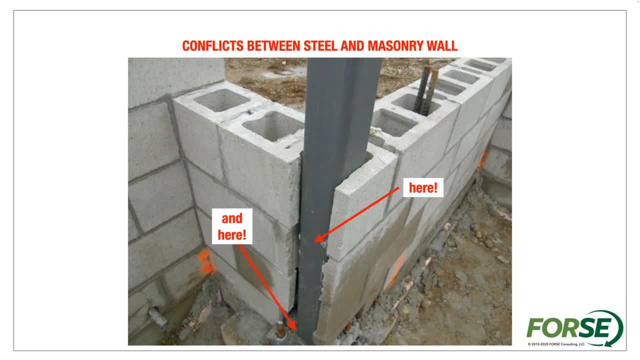 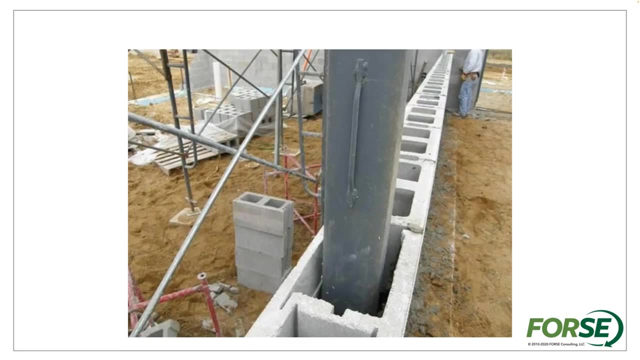 plate, or you can have some sort of a bump out just to cover up what you have there, and then you have anchors at the bottom. you know exactly how to deal with that. you know, sometimes you can't conceal it relatively well. maybe you have to cut down. 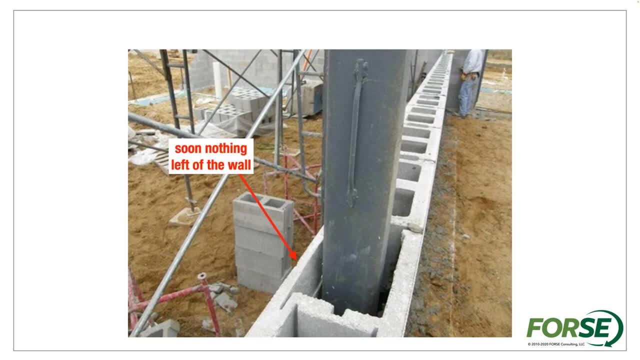 the masonry face shells. that's just, uh, just something that potentially could crack down the road. so again, steel versus uh, masonry. we have to be very careful, you know, if we have to put the steel there. you know, maybe it's a type of construction where the contractor wants to go. 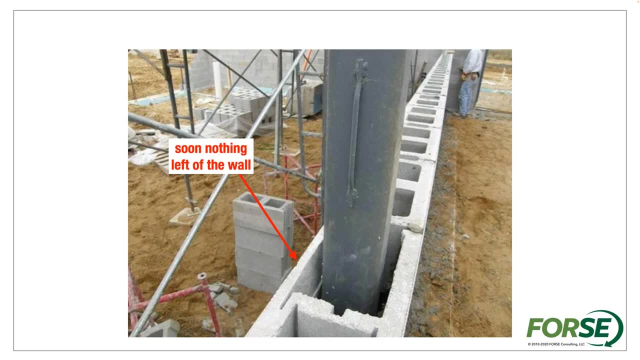 up with all the steel at once and then come back and infill with masonry. well then, we're going to be left with details like this that we have to make sure that we work through and take careful consideration and try to make sure that we're able to get the steel out there, and then we're going to 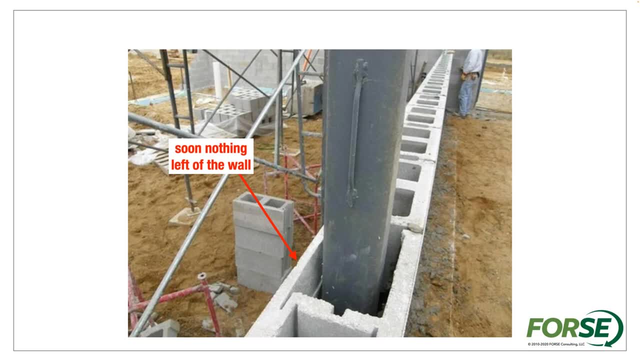 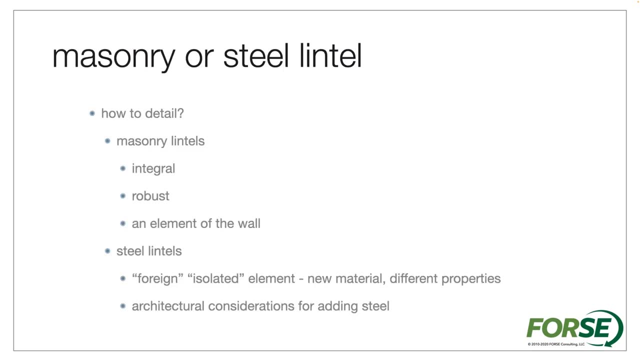 be reshaping it in terms of tolerances for steel and steel locations versus masonry, making sure that we understand the proper dimensions for masonry and exactly how that's going to work relative to the steel. we talked a little bit about steel versus masonry lintels, so we'll kind of clip. 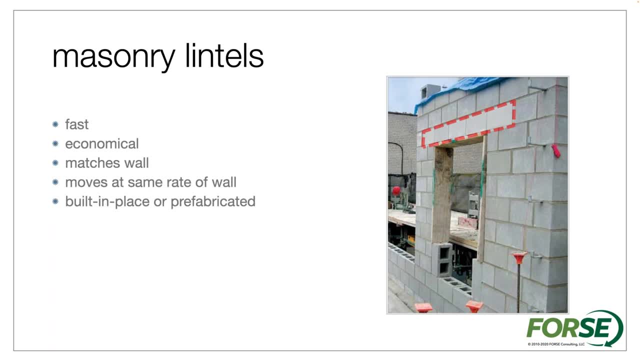 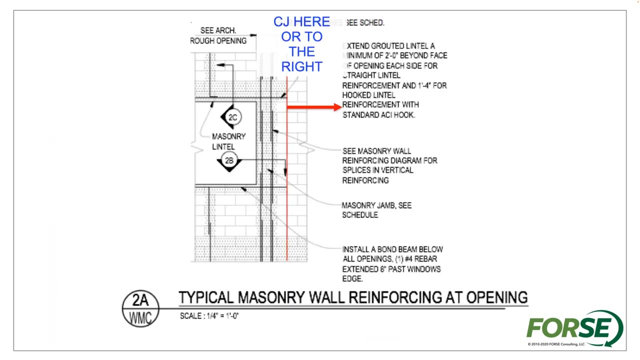 through this a little bit quickly. in terms of benefits for masonry, you certainly have a lot of different benefits. there. we have a pretty long span. we have, you know, like we talked about this morning, prefabricated masonry lentils or precast lintels. making sure that we have our details that reflect this, making sure our control. 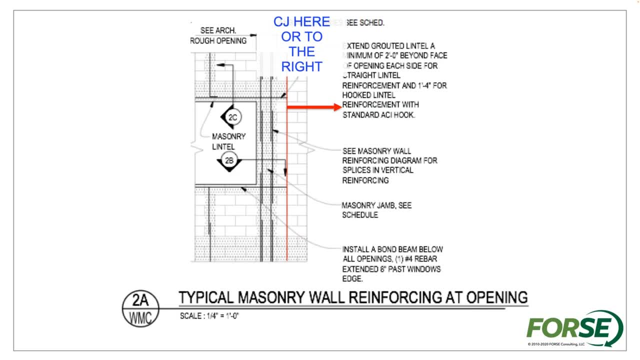 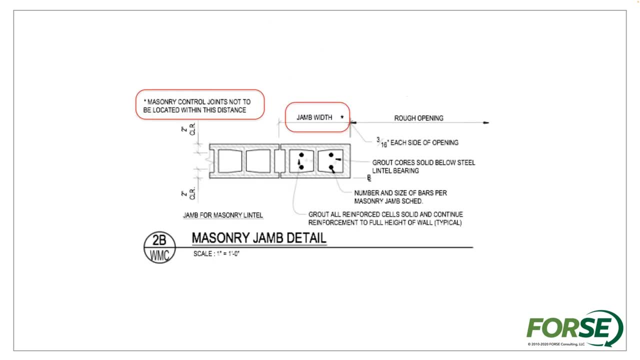 joints are away from the actual masonry lintels and jams that we have located there. so, whether it's an elevation or a plan view, we want to make sure that the control joints are out, in a way, from our lintel designs. and then we talked a little bit this morning. 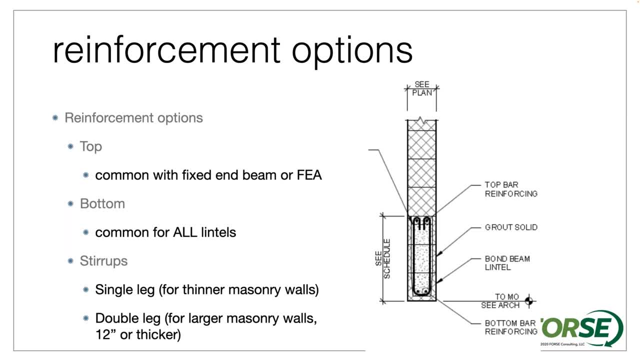 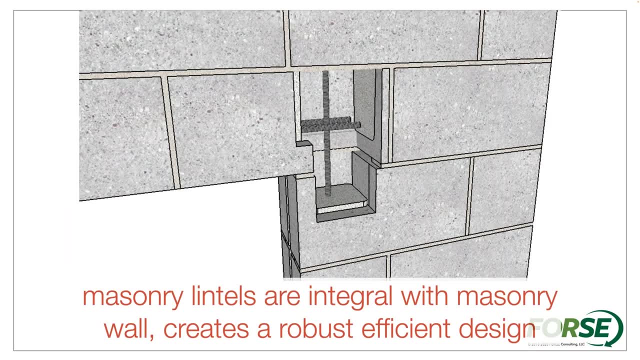 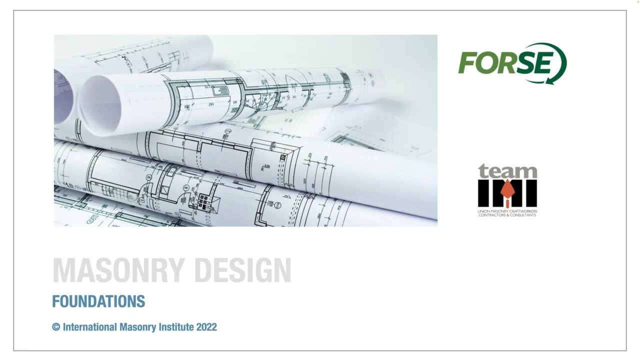 about what types of reinforcement that we would allow for the lintels, the reinforcement vertically, you know, the stirrups, or the top and bottom reinforcement that you can have. that creates that very integral connection with the wall around it. foundation design: we're going to kind of make a few different points in 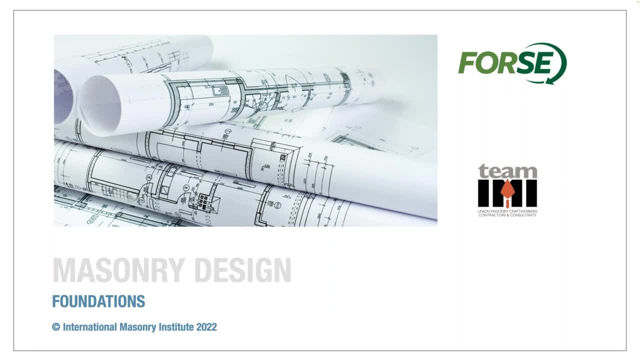 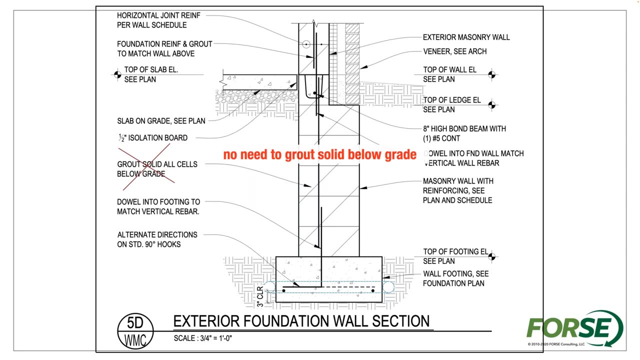 here in terms of the different types of foundation details that we can utilize. just kind of. let that set there for a second. there's no need to grow it solid below grade. i think that the big misconception that the mainstream below grade has to be grounded solid. a lot of times people will reference the fact that they don't want to have any water infiltration or 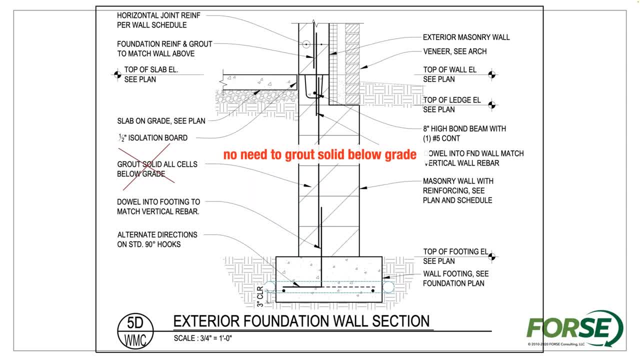 they want to prevent any water from collecting here and really it's not going to be the masonry that prevents the water or the grout that will be in the mainstream that will prevent the water. it's going to be, you know, waterproofing that will prevent water from coming in, just like concrete. 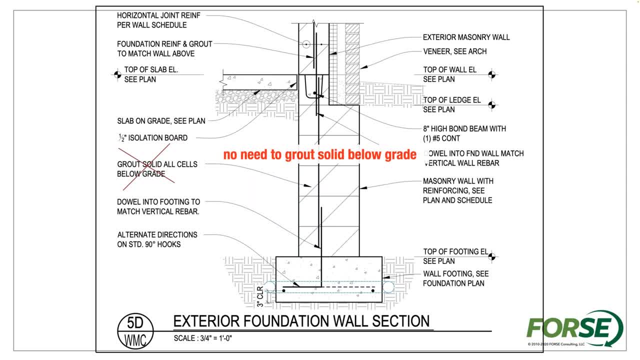 concrete masonry is going to be maybe a little more porous. it's going to, it's going to let water through if the water is going to exist. so if we want to keep the water out, we really want to waterproof it. grout and solid really doesn't have anything. you want to grout, solid, say in this detail, you want to? 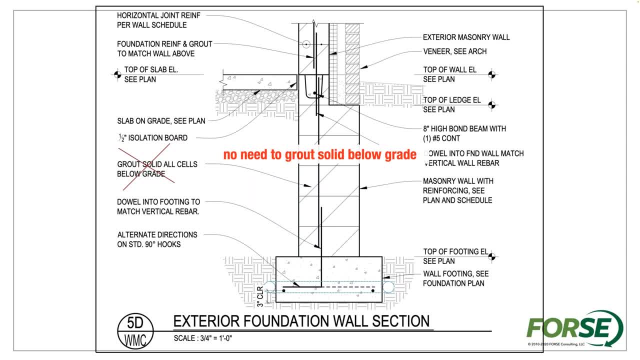 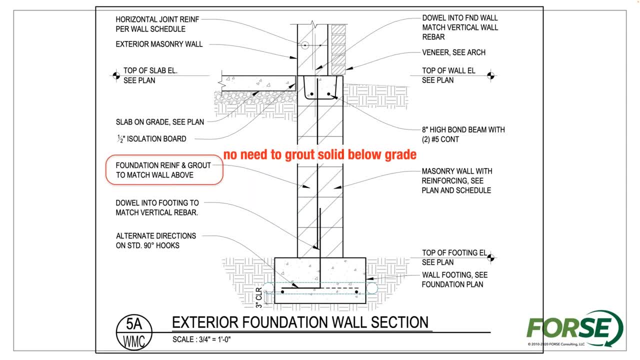 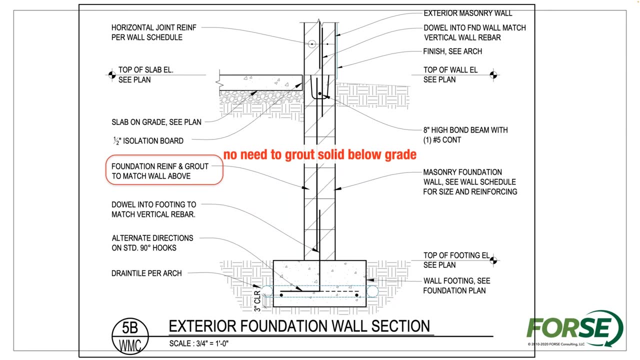 slat and have a bond beam at that transition, uh, from thinner to thicker wall. but there really isn't a need to grow solid below that, um, design wise, uh, no need to grow solid here as well, or here, especially here. when we have that continuity, we have the same wall. that goes. 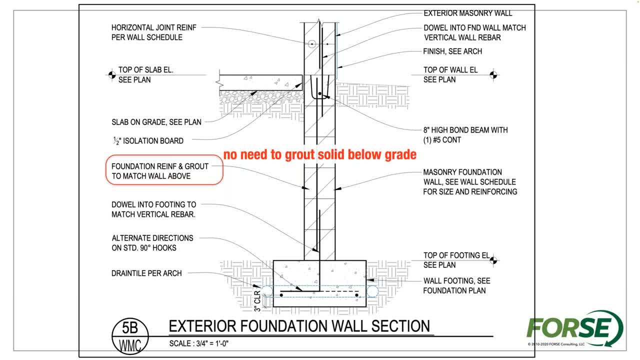 up and down. uh, don't need to grow out solid. and here even putting that bond beam in, having that transition and dowel would not necessarily be something that we would have to do unless we'd have some sort of a connection or connector that would tie the two big two walls together. 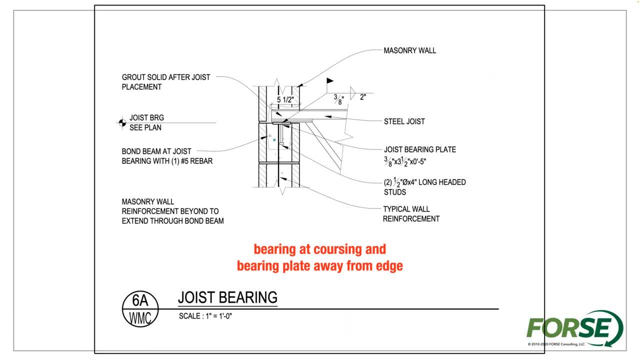 if we look at roof details again, we talked about those bearing conditions and bearing plates and making sure that those can stay towards the interior of the wall, making sure that we have, um you know, those and the headed studs that stay within- if it's a lintel block- that stay within the 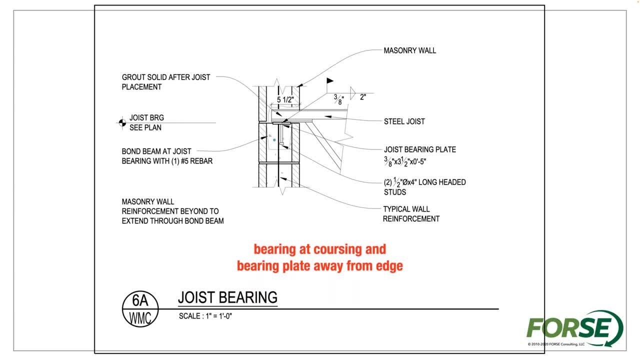 depth of the lintel block so that we don't have conflicts there between the headed stud and the actual block itself. so you know, something four inches long would always work, something six or seven inches long you'd have to use either a bond beam block or some other special block to make. 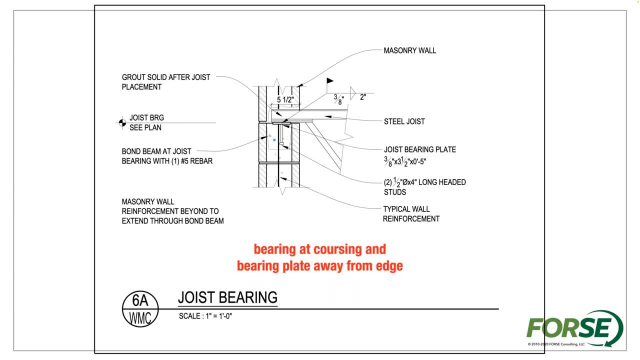 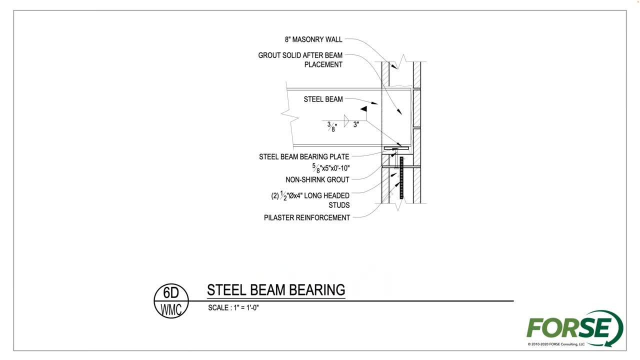 sure that that bearing plate works out just fine. so that can be a joist or you could have a steel beam that again you want to pull to the center. i mean steel beams. if it's a steel beam it's maybe a heavier, um, heavier connection, uh. so maybe you have some limitations there, but still putting it towards the center is. 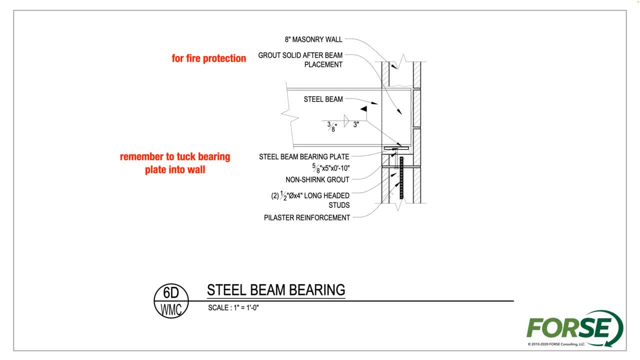 still going to be better. uh, you're going to grow that solid afterwards for fire protection. you're going to make sure that we try to tuck that plate into the wall as much as we can and making sure that we have a good stub length. that the 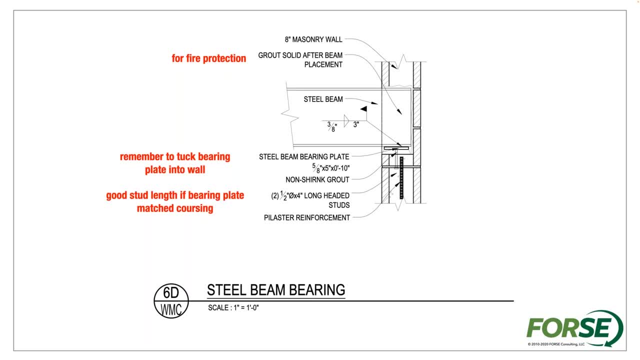 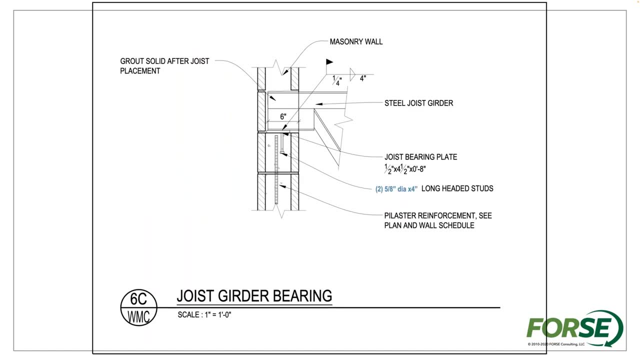 you know, we're making sure that we have the ability to have that headed stud not go through the lintel block. and here the lintel block is probably sitting down a course or two. same goes for joist girders as we had for a steel beam. a lot of the same comments: grounding solid or 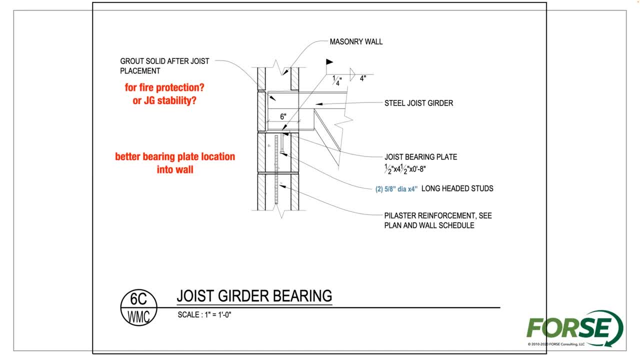 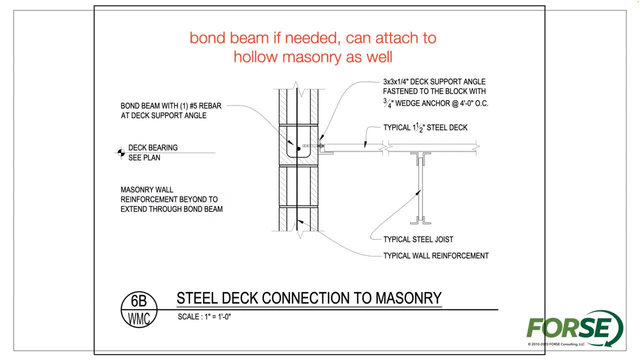 joist, girder, stability- sometimes grounding those solid has to do with that as well- and again, trying to center, center those studs and have the right stub like. so all different details that we want to think about and consider bond beams needed, especially if this is a diaphragm. 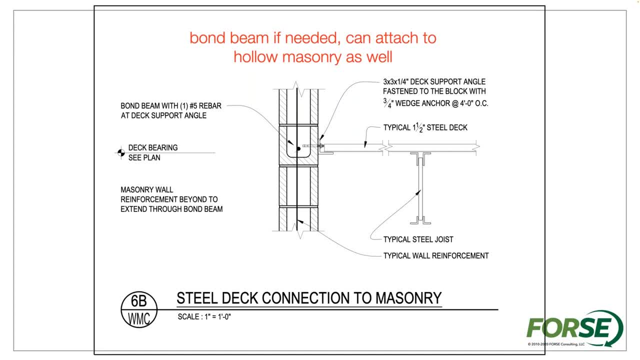 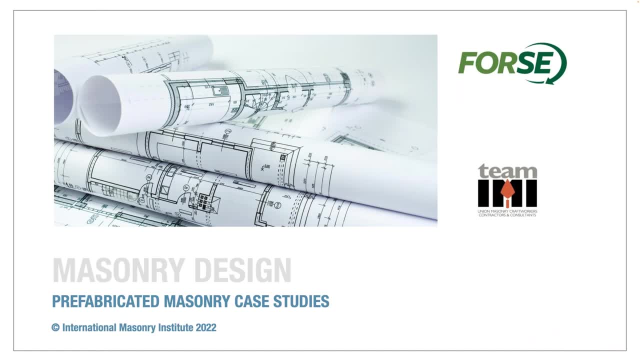 and this is a cord element in the diaphragm. maybe that's one of the times where your bond beam does stay continuous along the top of the wall. and then just a couple uh bits here on details and in case studies for pre-fabrication. prefabricated masonry, i think, is becoming more and more of an. 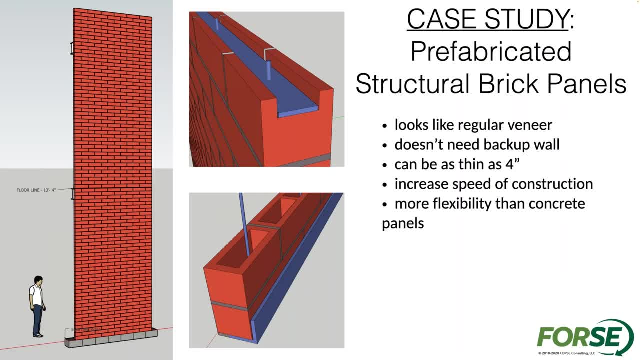 option that contractors want to consider. prefabricated structural brick panels are something that i think can really speed up construction quite a bit. um, it looks like regular veneer. it's really going to be, you know, if it's interstate or belden or if it's some of the 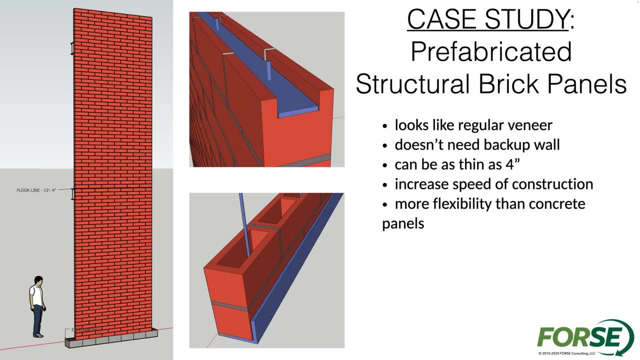 different uh structural brick manufacturers. they make common brick too, so you really do have the ability to have the structural brick panels match uh any sort of a brick that you would have. um, it can be as thin as four inches and reinforced it can increase view to construction. uh more. 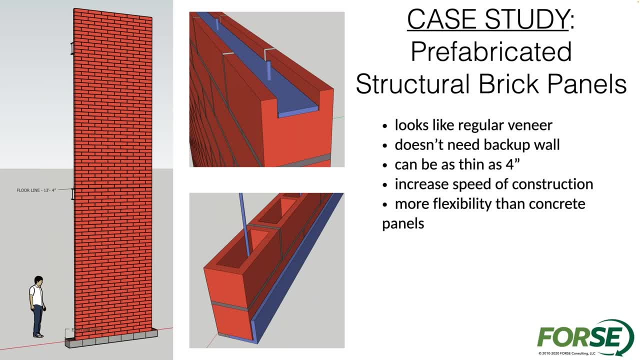 flexible than, and then concrete panels. i would say that the more of a block-based type of panel it is thing about structural brick panels is. just, you know, the size of the panel usually is dependent on lifting capabilities that you have on site. so making sure that you have the ability to, you know, lift the panels and set them in. 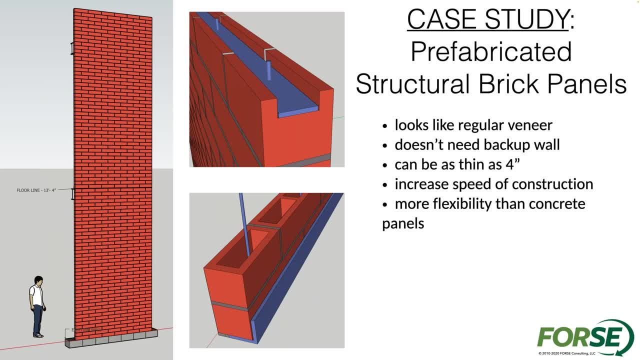 place. you know, a lot of mason contractors aren't going to have necessarily that lifting capability, so it's going to probably be a general contractor that would have to be valuing whether or not they wanted to lift and set panels. so it can be a structural brick panel or it could also be. 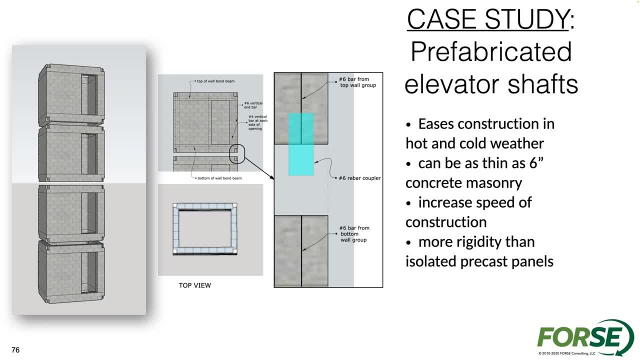 prefabricated elevator shafts. you know we're taking entire shaft walls and setting them on one another to one speed up construction. this could be cold weather construction. anytime that we can get into prefabrication of mainstream, we're obviously eliminating a few steps in terms of cold weather construction. 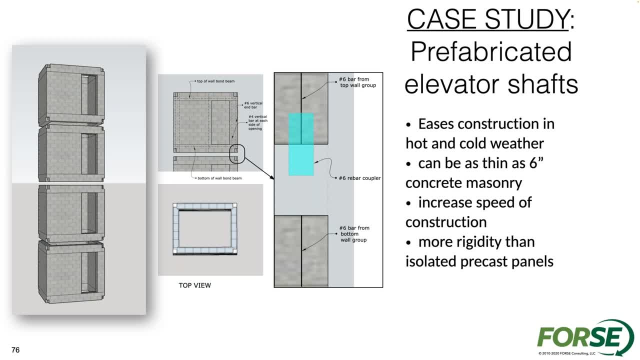 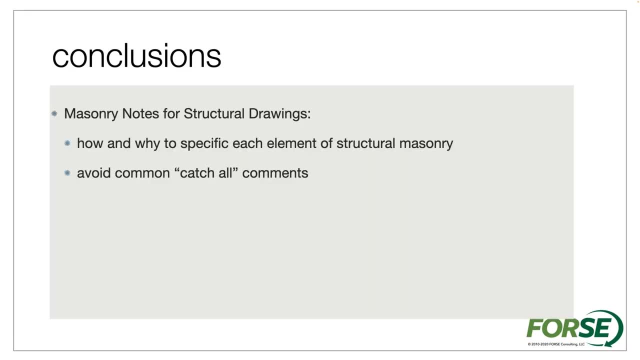 that can really be helpful for the overall design. so just some conclusions on the section notes on structural brick panels and the construction of the structural drawings. try to avoid, you know, some of those catch-all statements. try to be specific with each of the materials that you're defining and the 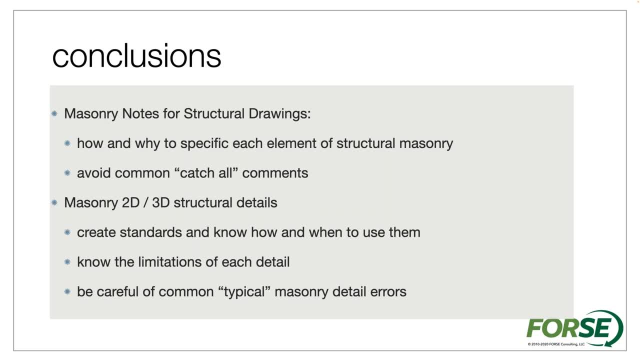 masonry 2 and 3d detail makes sure that you create standards and have them that are going to be coordinated with some of the detailing parameters that you set forth and some of the other sections that we've talked about, some of the design that we have. be careful of typical masonry detailing errors that we 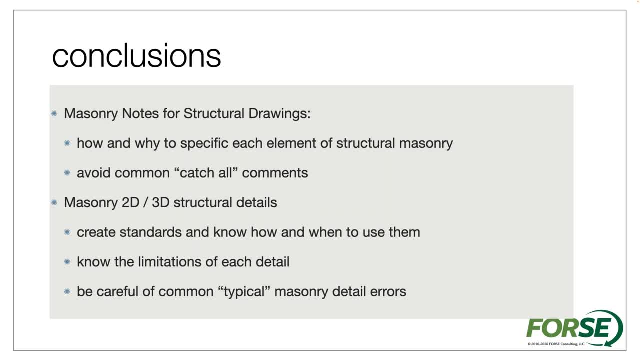 don't have well, maybe conflicts with other materials or what some of the tolerances might be between masonry and 3d panels or structural drawings. if the contact features are not that good with some of the materials, that might be right in the work space. 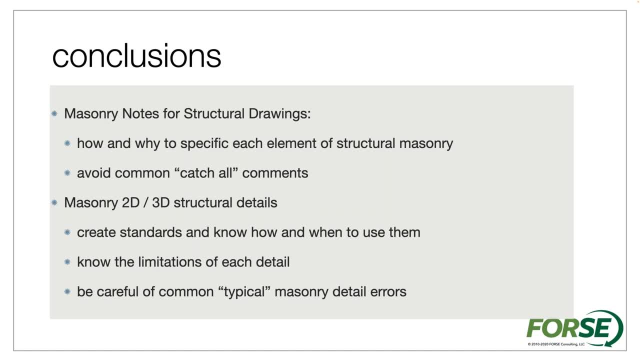 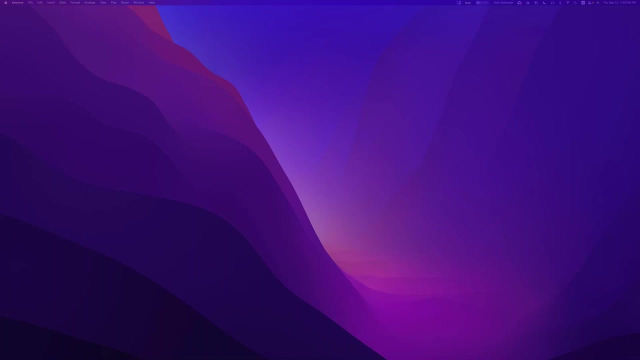 materials can certainly lead to potential issues. so that would be some of the notes and details and connections part of the presentation today. take a minute or two if you guys have any questions on that. you you all right. so next i think what i'm going to do is let's talk about sustainability of 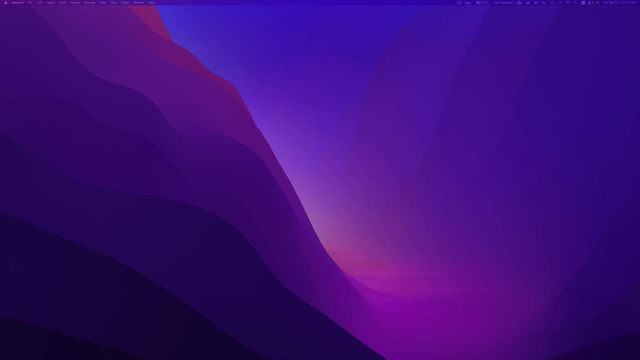 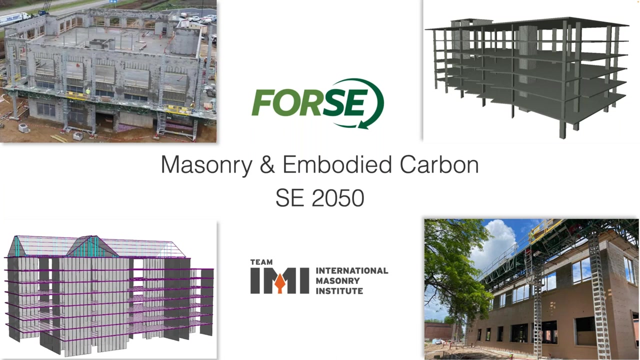 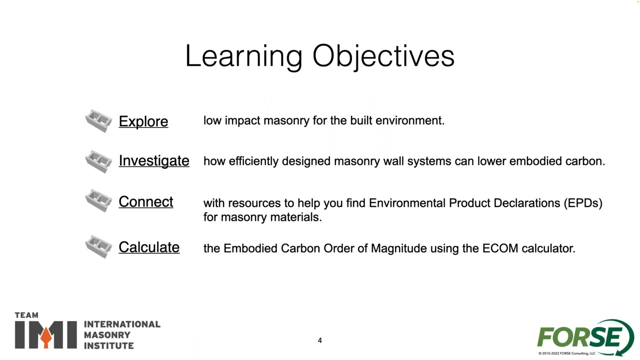 masonry. i think that's a next in the list of the items that we wanted to talk about today. it doesn't look like we had any questions come through. no, i didn't see any new ones myself, so all right, excellent, all right, so this section. what we want to do is we want to look at again the low impact. 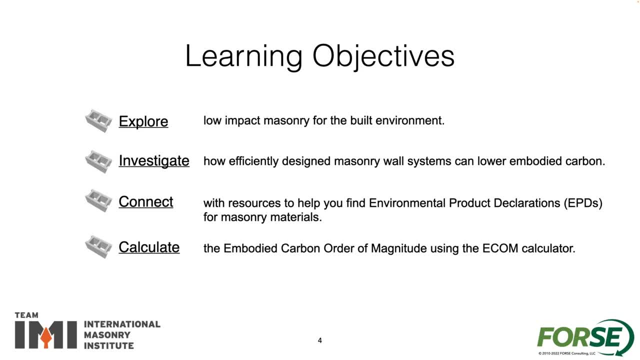 masonry you can have on the built environment. investigate how efficiently designed masonry walls can lower embodied carbon. look at different resources to help find epds- environmental product deck relations with masonry materials. and then just kind of point to embodied carbon order of magnitude using the ecom calculator. so, um, you know we're going to talk a little. 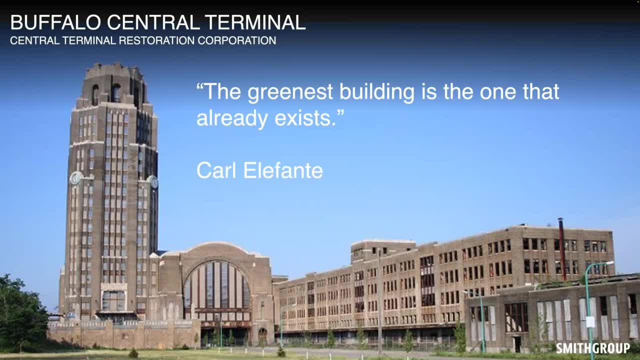 bit about what you can do with masonry and what we can do with it. for sure, but the thing about masonry is some of the obvious. you know, the greenest building is one that already exists in terms of the construction of the actual building. you know, i get there's a lot. 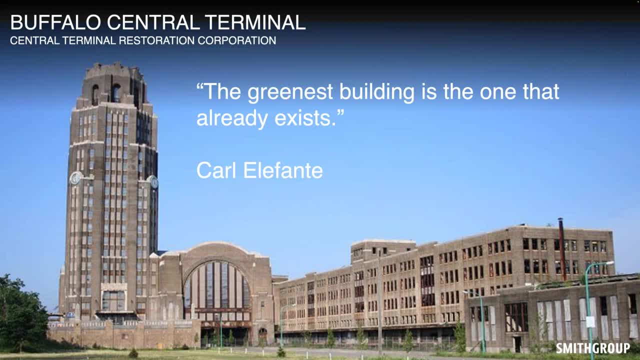 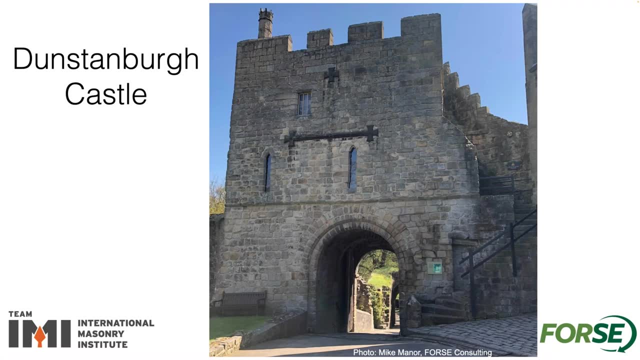 of mechanical and a lot of other things that we have to consider. but you know, looking at, uh, masonry structures, you know they last a long time. this is a castle that one of my colleagues was able to kind of come through and obviously that's built, that we didn't. 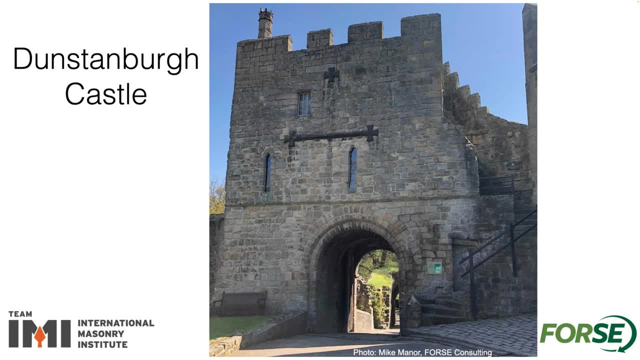 put a lot of carbon into building that thing for many, many years. so, uh, we're going to have. Um, there's a lot of things that we have to think about and consider with masonry design and the sustainability aspect of it, anytime that we can reuse. 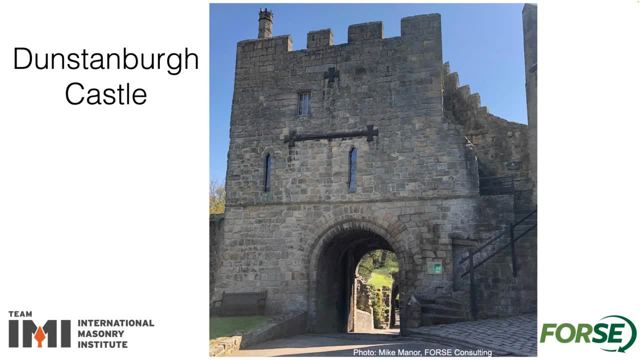 And you know, looking at existing masonry structures is not something that we covered in a lot, but we didn't cover hardly at all. today, if anything, Um, and that's certainly something where, um, you know, we can have a 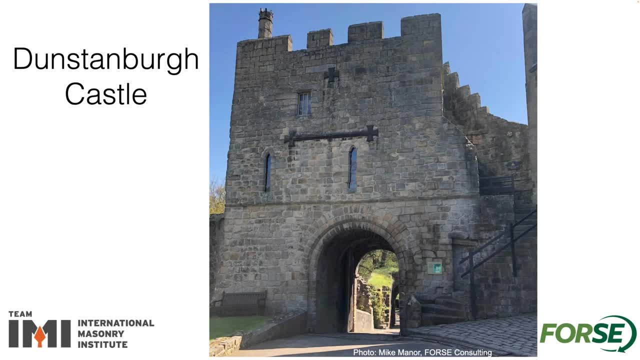 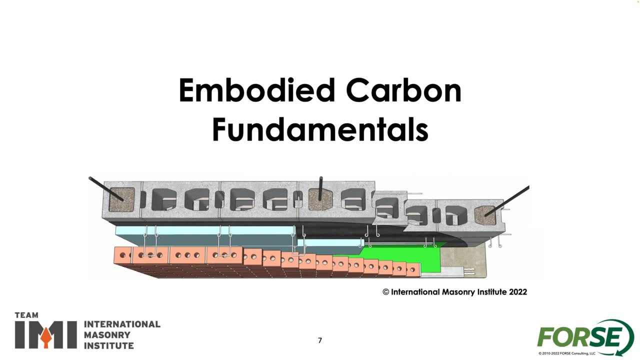 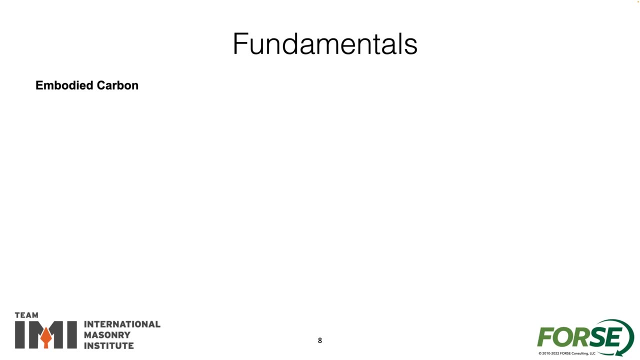 separate conversation and look into that, but it's a that that's certainly a place that we have, um, a lot of, a lot of room for, uh, with the sustainability in masonry. So some of the fundamentals. I'm not sure if you guys had a lot of discussions. 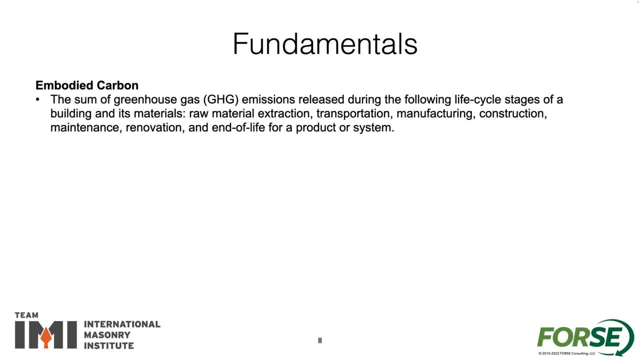 here, but just a few of the key um terms. embodied carbon is going to be the sum of the greenhouse gases- uh emissions- released during the following life cycle stages of a building and its raw materials. So you have raw material extraction, you know, pulling out whatever. 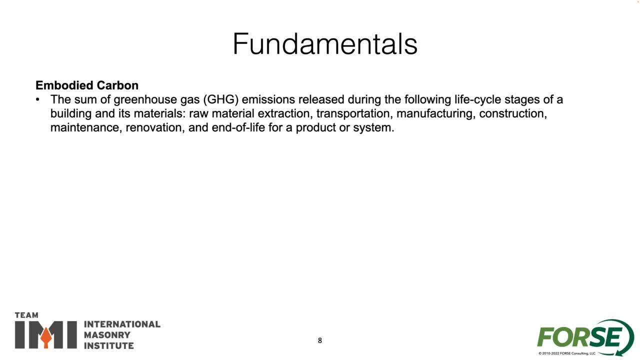 material. you need to make the concrete, concrete masonry, clay masonry Uh. you have transportation and manufacturing. you have construction uh, maintenance, renovation and end of life uh for a product or system. So when you have to tear the thing down, you know what does that look like in. 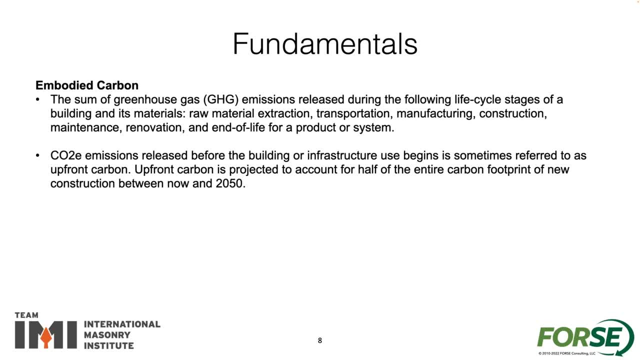 terms of uh, the overall environmental impact. the CO2 emissions released for For a building or infrastructure use begins is sometimes referred to as the upfront carbon. So you know a lot of that stuff in terms of uh, uh manufactured products. 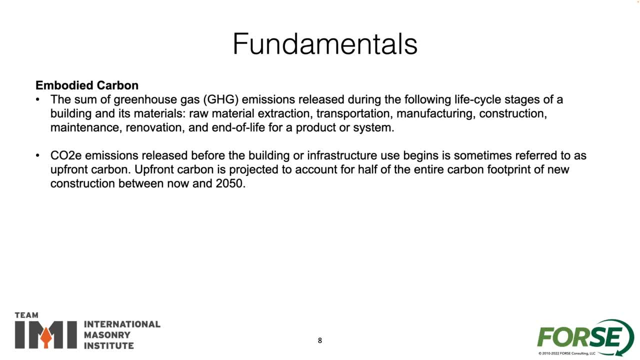 you know they can help you with a lot of the upfront carbon, uh, that's going to be used, You know, for the creation of the structure, some of the you know using the building, the renovating, the end of life, that's obviously going to be outside the hands. 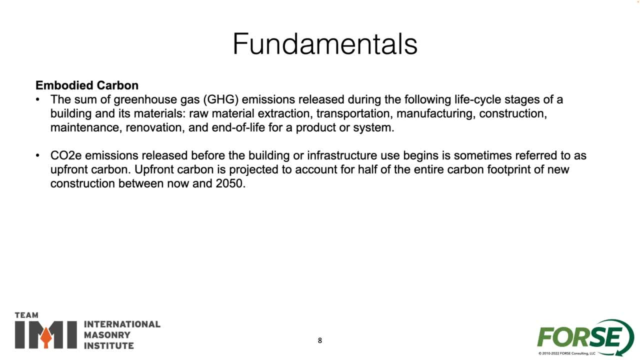 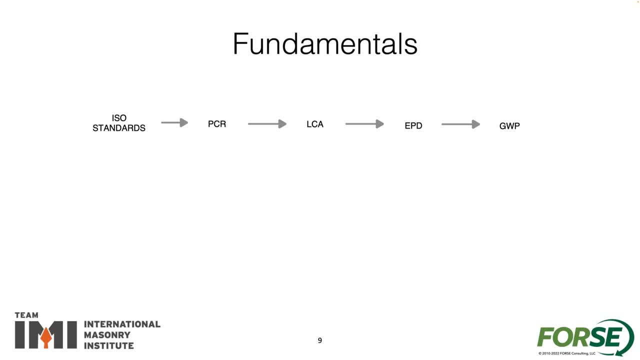 of the manufacturers, so that we're going to be a limited, a little bit limited, in terms of what they're going to be able to provide. uh, for some information. So ISO standards, um, you know how to imagine a body: carbon for a building. 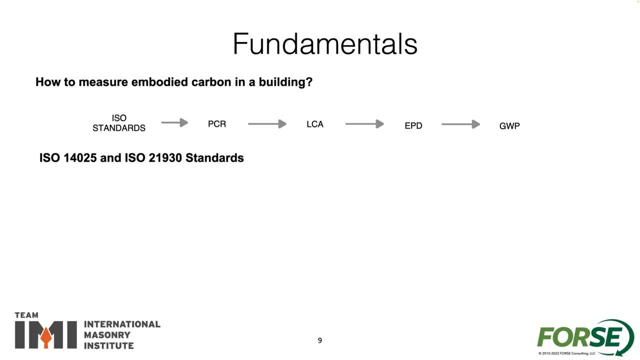 We have the ISO 14,, 0, 25 and ISO 21- 93. So international standards that uh control environmental product declarations and kind of establish a core set of requirements. uh will be considered as the PCR Uh. so product category rule provides rule, requirements and guidelines for. 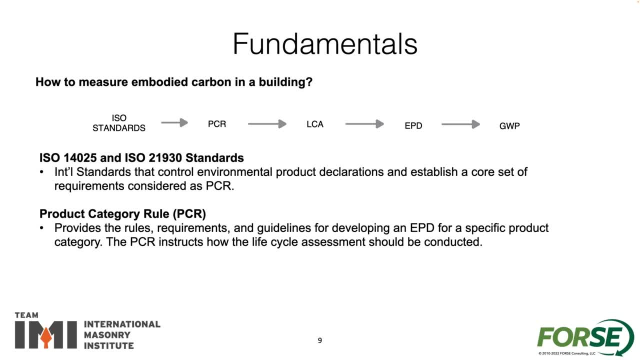 developing an EPD for a specific product category. PCR instructs on how the life cycle assessment uh should be conducted. Life cycle assessment is going to be a systematic analysis of the potential environmental impact of a product uh during its entire life cycle. 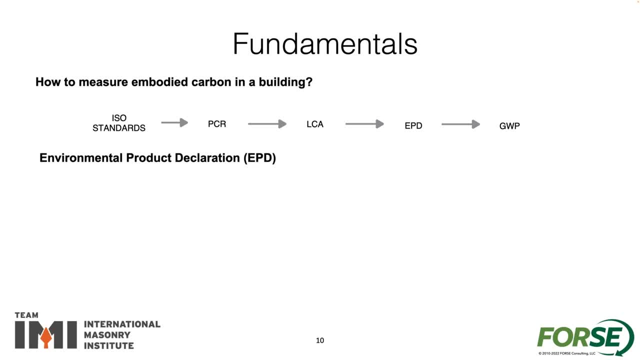 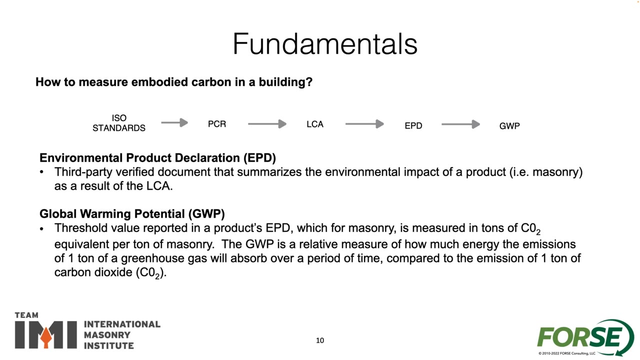 So how do I measure embodied carbon in a building? Environmental product declarations is going to be a third party uh verified document that summarizes the EPD of masonry, for example. uh, as a result of the LCA global warming potential, it's going to be kind of a threshold value in a product's EPD, which for masonry. 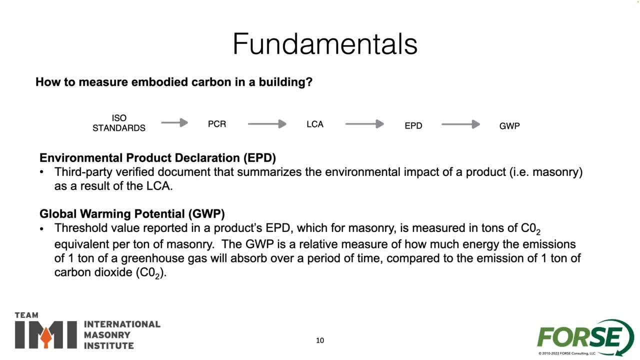 is measured in tons of equivalents. Per ton of masonry, you do a relative measure to how many, how much energy the emissions of one ton of greenhouse gas will absorb over a period of time, compared to the emissions of one ton of carbon dioxide. 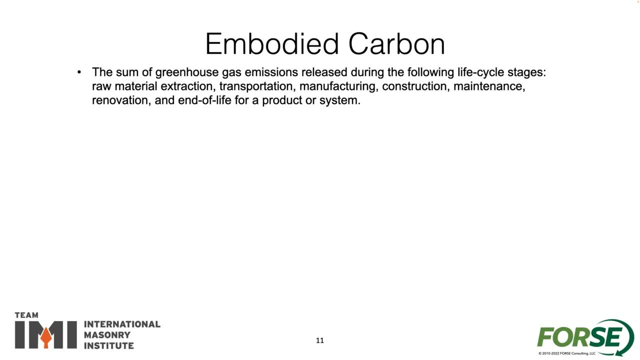 So now everybody wants to reuse those existing buildings, right, So they don't want to keep going with some of the some of this, All right. So, uh, embodied carbon, some of the greenhouse gases released during life cycle stages. So again those extraction, transportation, construction, maintenance, renovation, um. 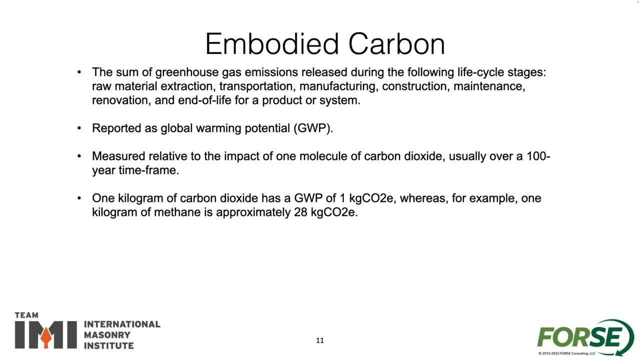 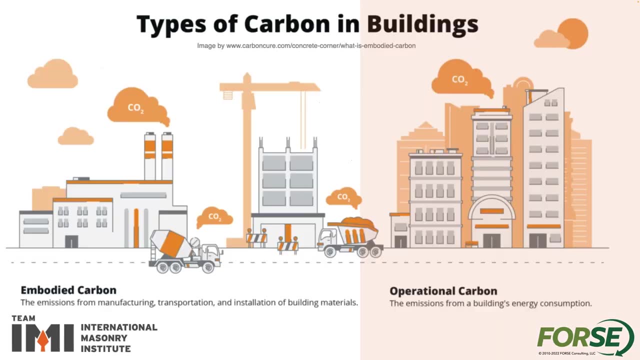 reported GWP measure relative to again. So again, some of the CO2 emissions before the building infrastructure uses, sometimes referred to as up again, upfront carbon, is really really be kind of focused on. So everything kind of delineating here the embodied carbon you kind of see by manufacturing. 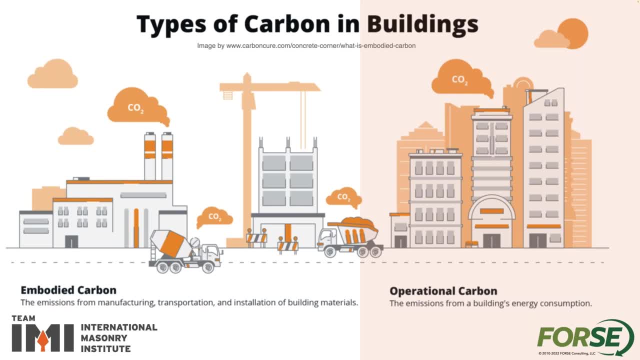 and getting to site and everything, to getting a building up and ready to use, And you know that's really where? Uh, a lot of them, They're a little bit more of a يد n? n, but it takes a little bit of time for those. 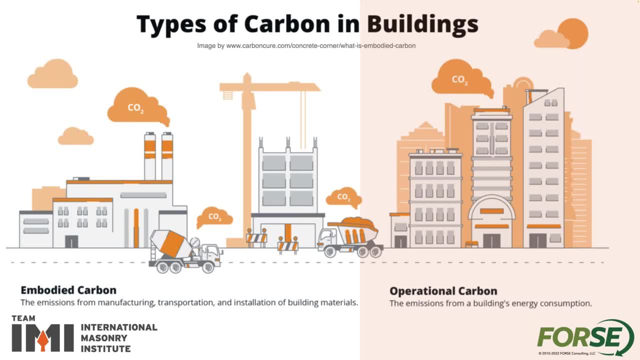 models to do what we do, which is to kind of understand the structure of the building structure a little bit, for to get it, the structure of the building structure and how that would work, And and to really kind of figure out what information can kind of be gathered. 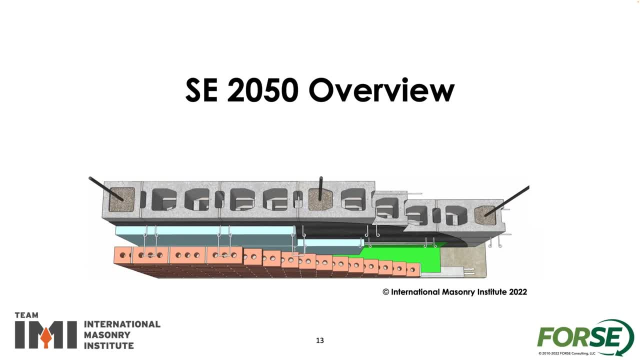 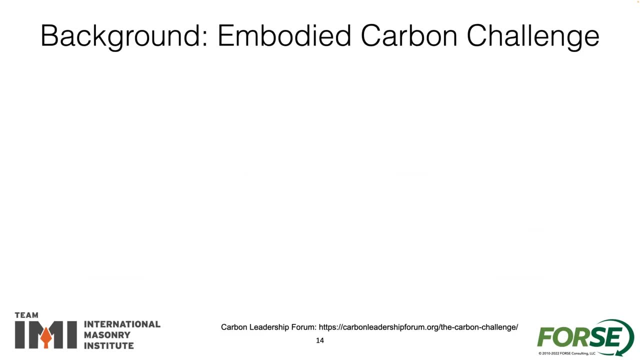 Uh, it's going to be, I think, a long time before operational carbon, before we can, you know, kind of have some studies on buildings and how they work over time and you know issues. so embodied carbon challenge was kind of something issued in 2019 by the carbon leadership forum. 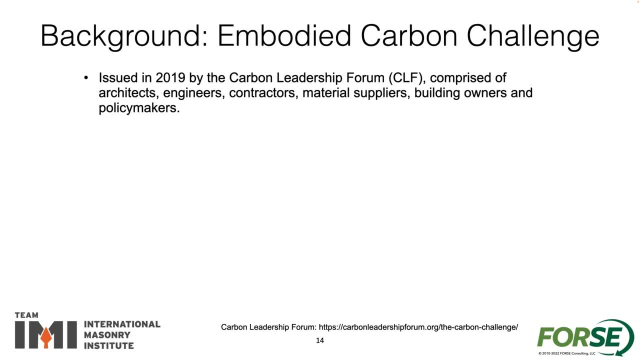 it's a group of architects, engineers, contractors, um, building owners, policy makers, just trying to take some big steps and decarbonization of the built environment. i mean, if anything, just trying to have a little bit of a focus on making sure that we do things uh, responsibly, i think would be. 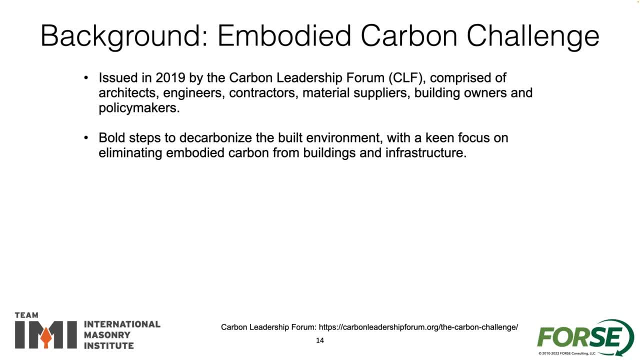 um, that would be a great statement to add in here as well, trying to make sure that we don't unnecessarily add a lot of material or embodied carbon to some of these buildings. globally, building constructing sectors that account for nearly 40 percent of the global energy related carbon dioxide emissions, and constructing- that's a pretty big number. 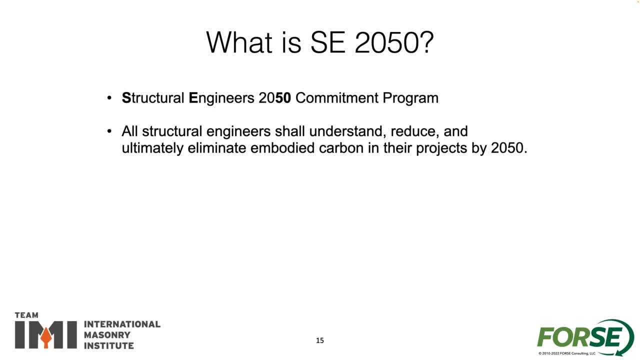 so se 2050 was a structural engineers 2050 commitment program. it's all structural engineers to understand, reduce and ultimately eliminate embodied carbon in their projects by 2050.. it's a bold goal but, like i said, that's a something that we can try to. 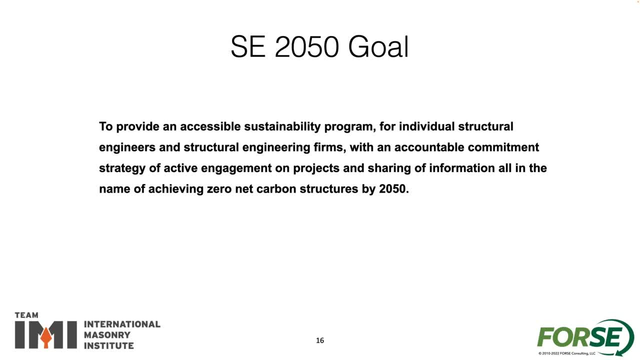 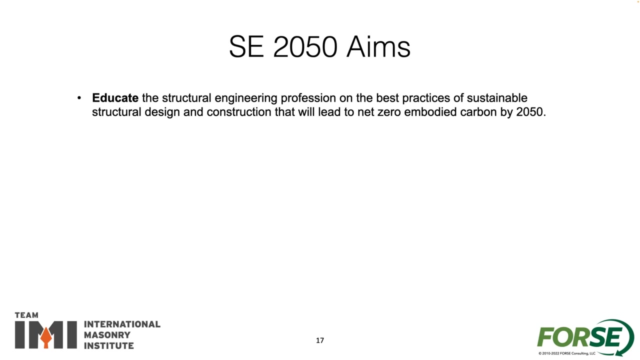 try to achieve by you know different means and methods. so the 2050 goal: to provide an accessible, sustainable program for individual structural engineers and firms, with a accountable environment of strategy, to active engagement on projects, sharing information, all in the name of achieving zero net carbon structures by 2050.. so educating structural engineering professionals. 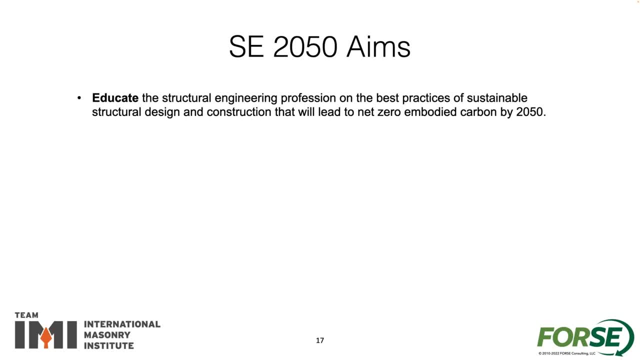 and the best practices of sustainable structural design and construction that will lead to zero embodied carbon by 2050.. and it aims to engage in embodied carbon tracking program within the structural engineering profession, thereby enabling the establishment of appropriate embodied carbon reduction targets until net zero is realized. so 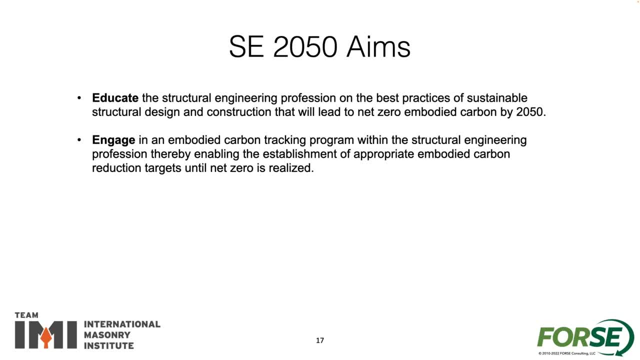 obviously, any things that we can do to move in this direction is going to make a better and better impact on the overall environment. you know so any sort of reports on current embodied carbon impacts and trends of various structural systems of different regions throughout the country. advocate and communicate with clients, design, community, community public. i mean it's really. 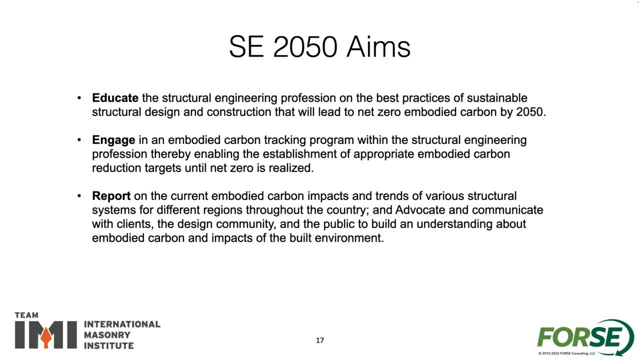 trying to create a kind of an accountability tool for structural engineers to try to be more responsible with our designs and try to make sure that we're trying to move in the direction of of being more sustainable with the structures that we create. i mean, anybody can design something that- um- you know it was- is going to have a very large. 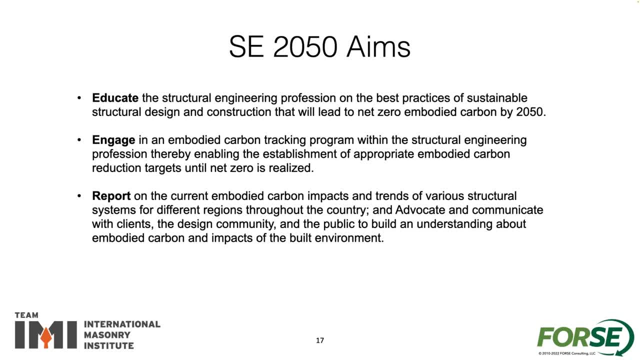 carbon footprint and something you know that obviously costs a lot design-wise, but in terms of the material usage and stuff like that, we want to be working smarter and better and, and you know, we want to be able to do more of that, and we want to be able to be able to do more of that. 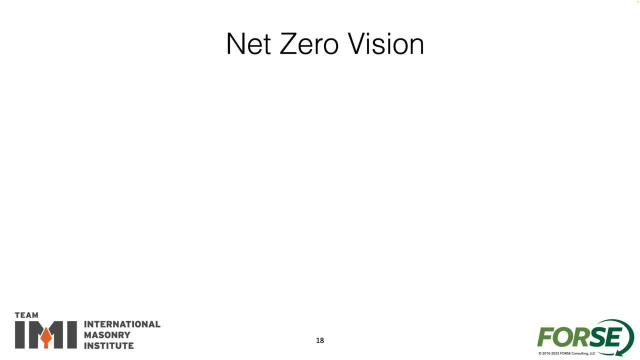 trying to achieve some of these goals, trying to reduce our carbon footprint nonetheless. so i would say the um, you know the vision, the net zero embodied carbon by 2050- um, it's a pretty big goal. that's, i mean, considering what they're looking for. i mean that that's, that'd be pretty. 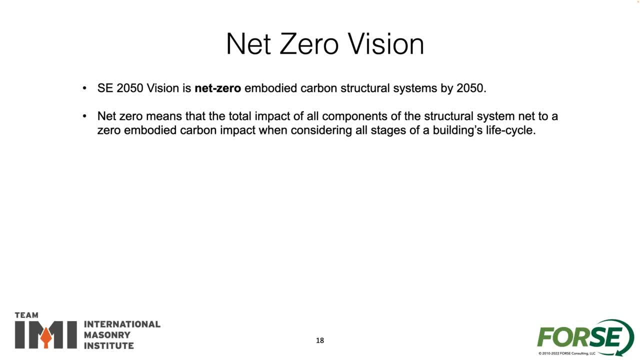 fast, i think, um, but that net zero means that the total impact of all components of the structural system net to a zero embodied carbon when considering all the stages of the building's life cycle. so getting to net zero will require change in both the design and construction, as well as in areas where structural engineers very 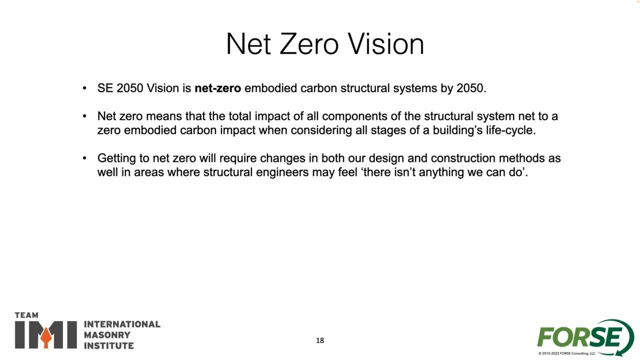 maybe feel that there isn't anything that we can do. i think that that's a big statement. i mean, you know, certainly it takes energy to make new building materials, so you know there isn't anything we can do is certainly a statement that, you know, i have felt from time to time. 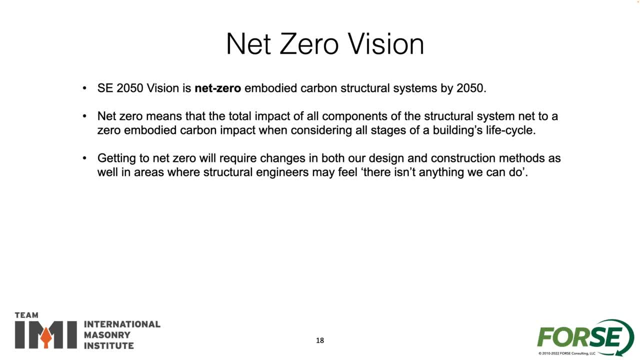 when i look at some of these different objectives, but the more that we can do, the better is definitely something that i can wrap my arms around. so you know, the more that we can do, the better is better than there isn't anything we can do, i think. 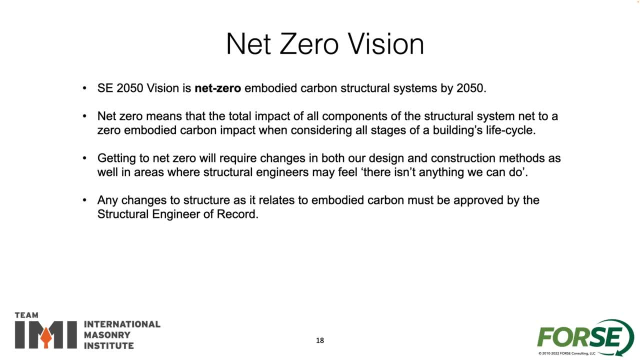 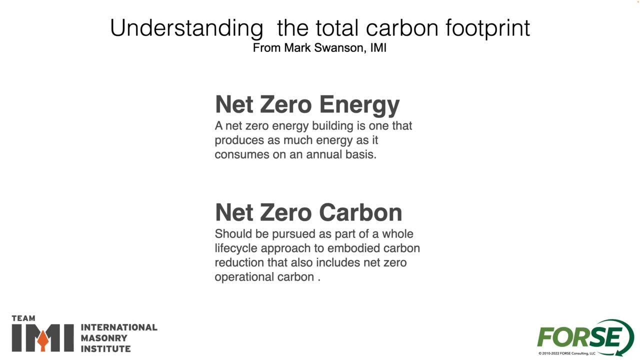 um, so moving in this direction. so any changes to a structure as it relates to embodied carbon must be approved by uh se ser. so just a little bit of a distinction. understanding total cover footprint, uh. so net zero energy? uh, a net zero energy building is one that produces as much energy as it consumes on an 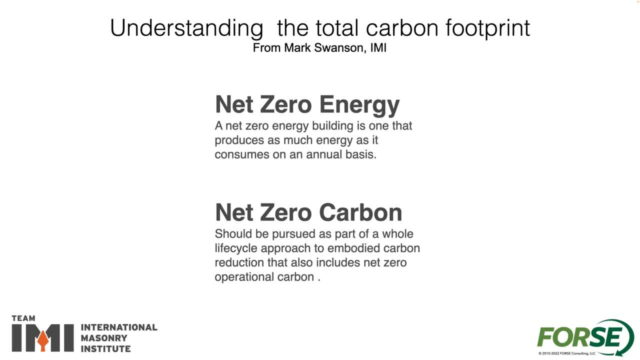 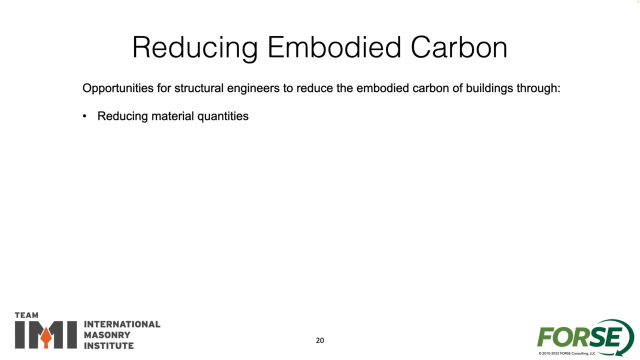 annual basis. so net zero is certainly different than a net zero carbon. uh should be pursued as a whole life cycle approach to embody carbon reduction. that includes net zero operational carbon. so some different opportunities for engineers to reduce that embodied carbon in buildings, reduce the material quantities. I mean that's just efficiency in design, that's looking. 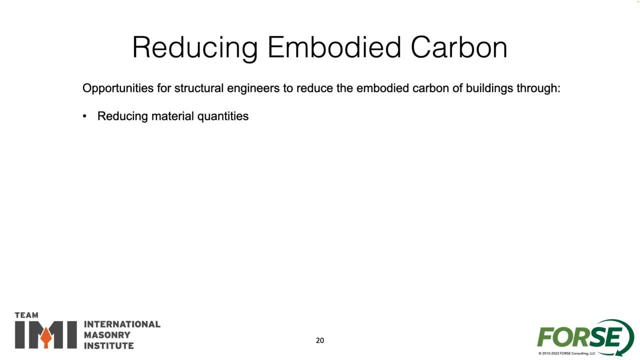 at a design and trying to see where there's potential for using less material to achieve some of the same goals. you know, I think you know, masonry definitely leans itself to this, to this. you know gold- right here, I mean it's masonry- is in itself inherently less material. if you look at the similar 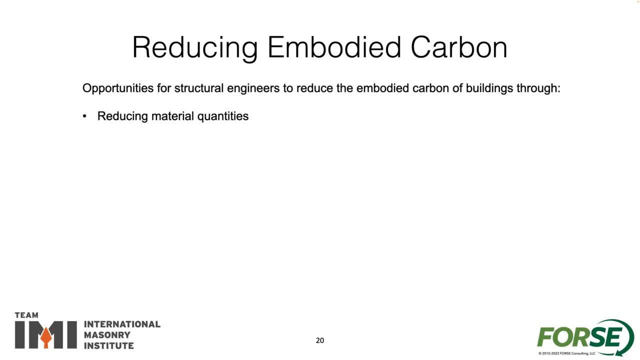 design element of a, say, a solid grouted wall or a solid concrete wall. most masonry should be designed as partially grouted and reinforced. it's got voids in it. it should be a lot less material than the design using larger bars and left grout would be a lot less material. I mean there's differently definitely ways. 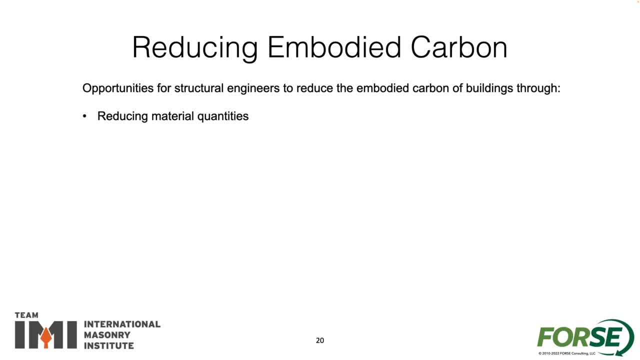 that we can start to explore using less than less material with masonry design, because it starts with the voids that you know. um bubble deck was always something that i thought was a fascinating uh design concept. we use uh. bubble deck would be a concrete slab where you place uh voids within the deck or within the 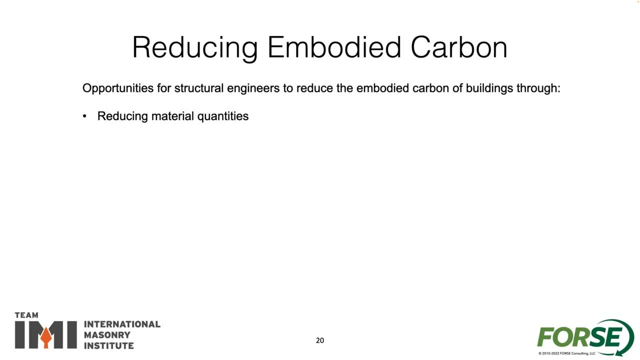 slab, so that it can be a avoided concrete element which has similar strengths and stiffnesses but has a lot less material. i'm like, well, that'd be great for reducing material quantities. and then you inherently you think about that, you inherently have that, uh, with masonry, so that 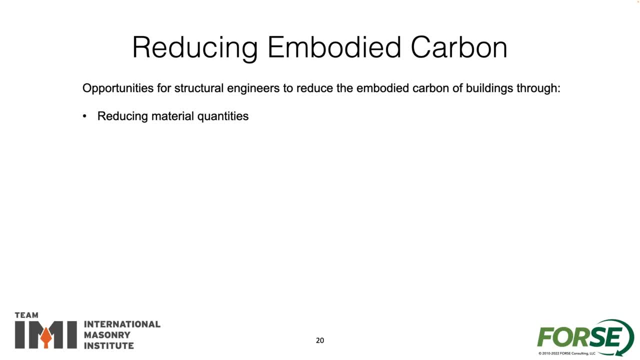 that's, uh, obviously a very good thing for masonry to to look at reducing material quantities. um, mitigating thermal bridging, you know again, that's some of the. you know anytime that we can move away from some of the thermal bridging that we have, you know, whether it be a steel lintel, um, you know in. 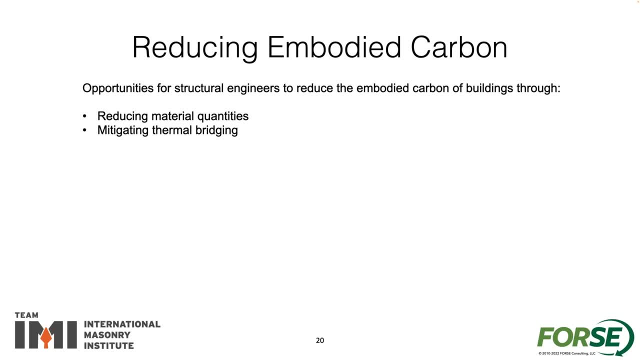 the backup wall that has that big steel bearing plate. you know, sometimes that's a big concern. designers are used to having that plate there, you know. but just kind of seeing that that's a pretty big thermal bridge from the outside to the end and you know any place that we 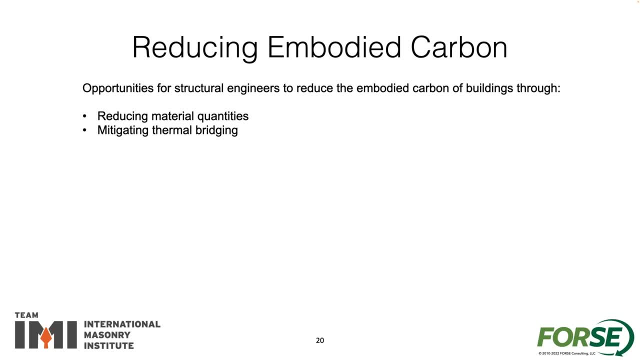 can reduce. that could be better if we can eliminate it all together by using a masonry lintel and then maybe a masonry or a floating um steel lintel in the veneer. you know, we can almost eliminate some of that thermal bridging. you know, if we have a structural 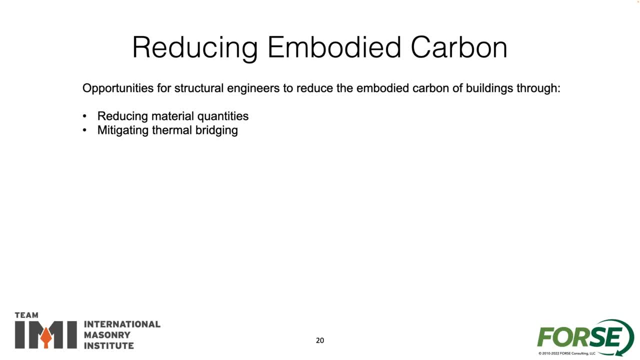 veneer. that's another place where we have very few connections between the outside veneer and the back. so again we can mitigate some of the thermal bridging. so a lot of different potential in places where masonry can come into play in both those first two options, exposing the structure. 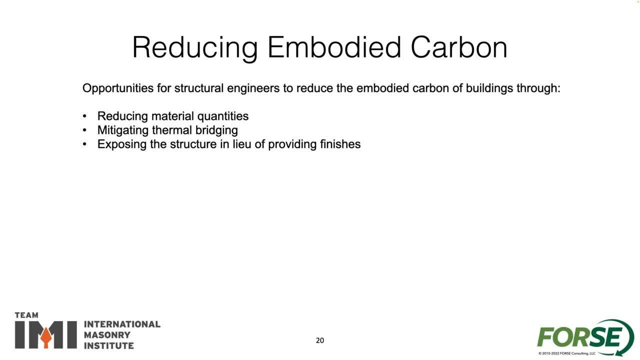 in lieu of providing finishes again. masonry is obviously going to be something that is made to be kind of exposed and- and certainly it's been of the aesthetic that a lot of people look for throughout the years. use protective systems with performance-based design, using alternate systems that then typically use for a particular 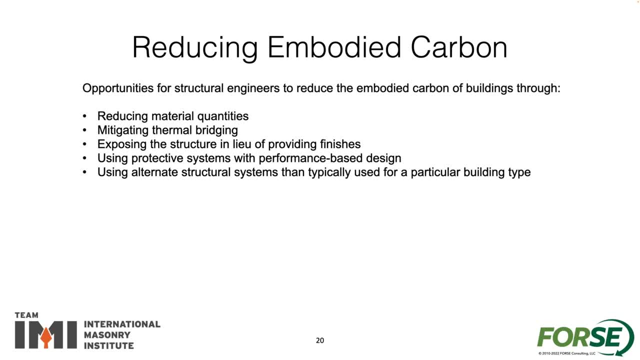 building type. you know things that i think of there when, uh, you know the different topics that we talked about today. you know, looking at a hybrid system, you know, sometimes we have, uh, the frames that are there, and then we have these masonry infills. you know, does it take more design effort? 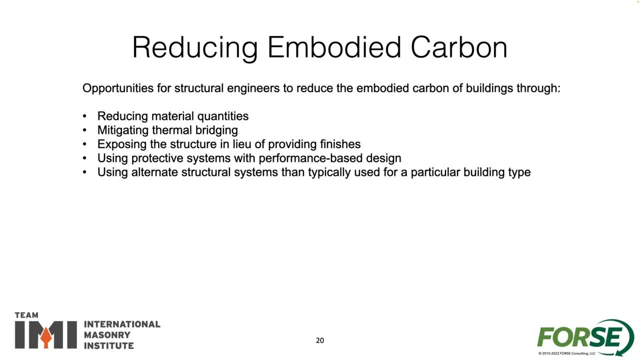 and work to think about how to connect those frames and connect those elements uh, so that we can have one uh kind of homogeneous system. uh, definitely a different way of thinking about it. um, that would be an alternate system that's taking use of uh the elements that are there. another: 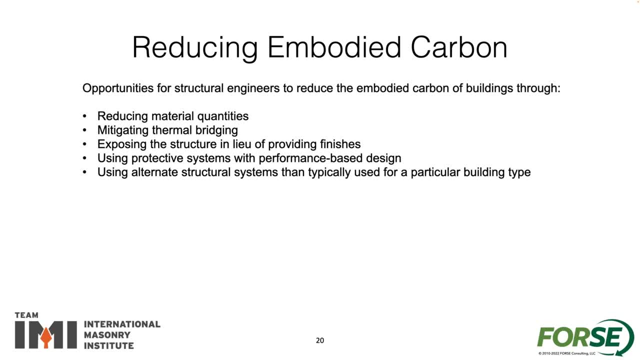 thing that i always think of when i read this line is: you know, you have shaft walls. there's a lot of times in a wood or a stud building that we have, uh, masonry shaft walls that are there for fire, for you know, just kind of the hardened element that you want in a project. um, those are very, very. 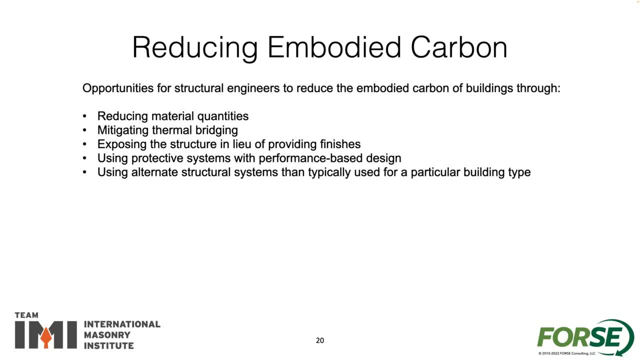 stiff, rigid, strong elements. i've seen designers isolate, you know, from those shaft walls so that, um, just because you have some differential movement between this, the stud structure, and the shaft wall, well, let's figure that out, let's connect those systems so that those can work together and we can use the full capacity of masonry utilizing lower carbon materials. 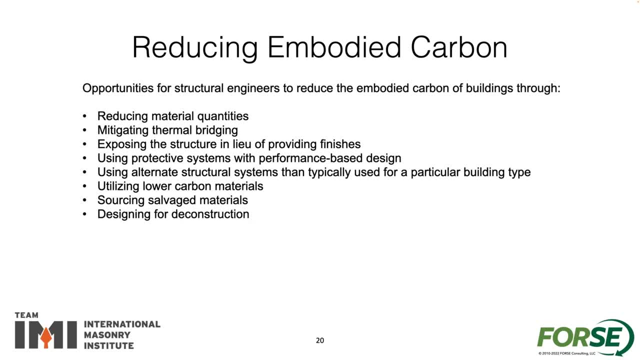 sourcing salvaged materials, designing for deconstruction, specifying materials with lower embodied carbon, producing materials is near the site reduces the carbon footprint and transporting the material. So all different things where masonry can certainly be, you know, can be reused. It can be something that can be salvaged. 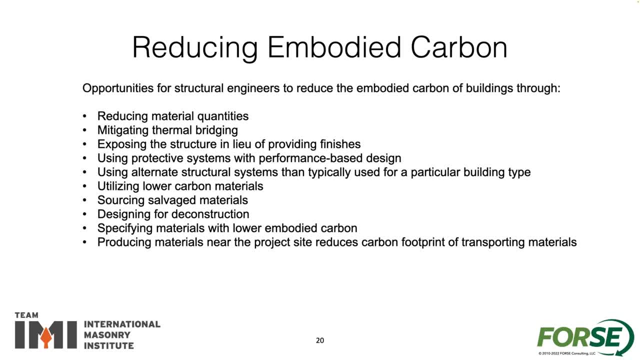 It can be something that can be used again. producing materials- I mean masonry, concrete masonry materials- are certainly produced locally all over the place, And so that certainly does help a lot with reducing the transportation costs for some of the materials. 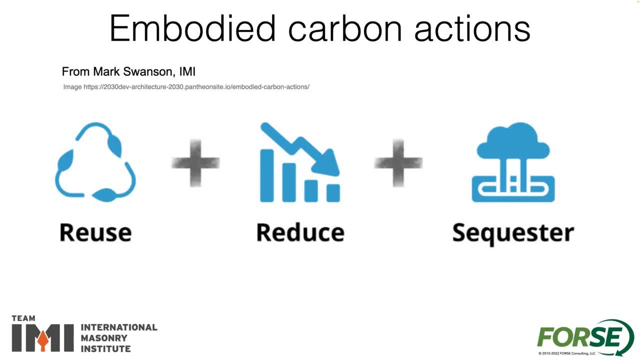 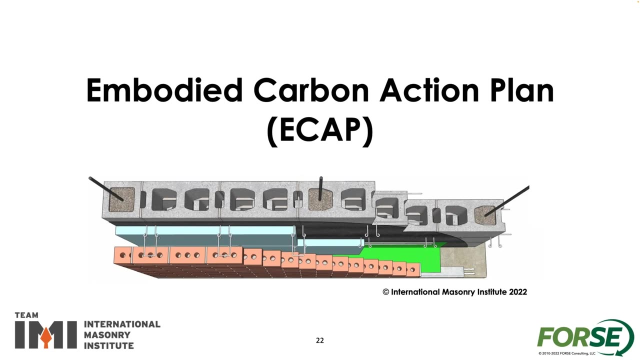 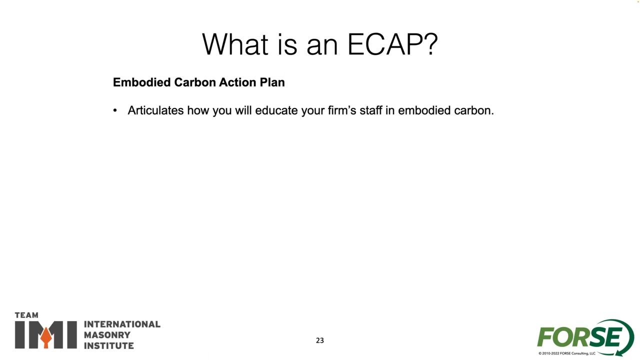 So embodied carbon actions, reuse, reduce and sequester are all different mechanisms for taking some actions on reducing that embodied carbon. Having an embodied carbon action plan in ECAP or ECAP, you know, articulates how you educate your firm staff and embodied carbon. 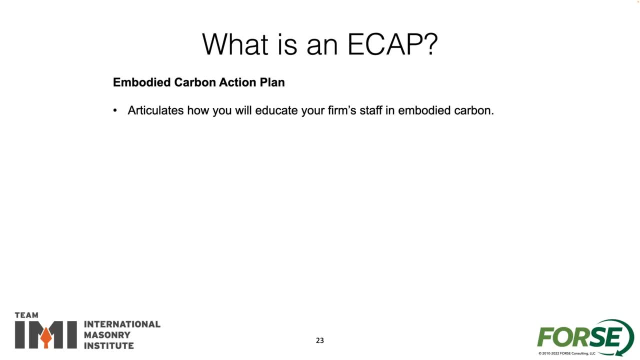 I mean go ahead and go in, through the paces of understanding and learning some of the pluses and minuses for some of the different systems that you might have, or some of the different designs that you might want to consider, You know, describe how you want to report. 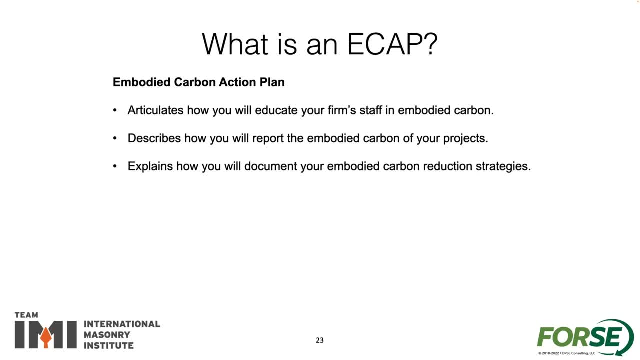 the embodied carbon of your projects. Explain how you will document your embodied carbon reduction strategies. I mean, I think some of these just in you know, I guess. address how you will advocate within the industry. I think all of those things are going to be. 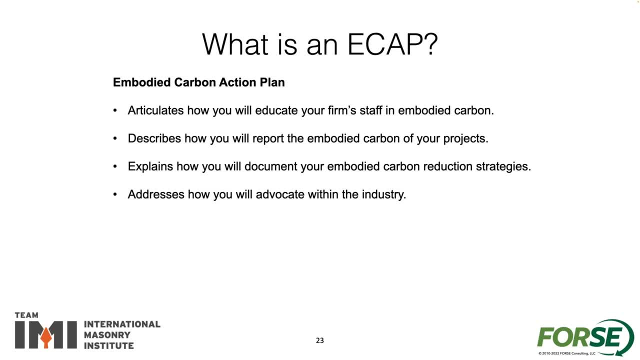 you know, just going through some of those steps are going to be helpful for you know, again, moving in that direction. Maybe we're not going to be able to get there in a specific timeframe, but as we're going through some of these steps, 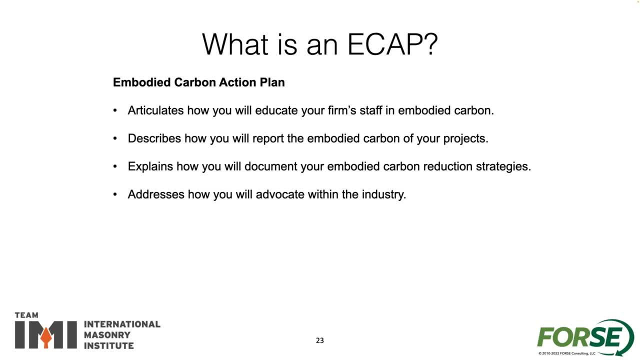 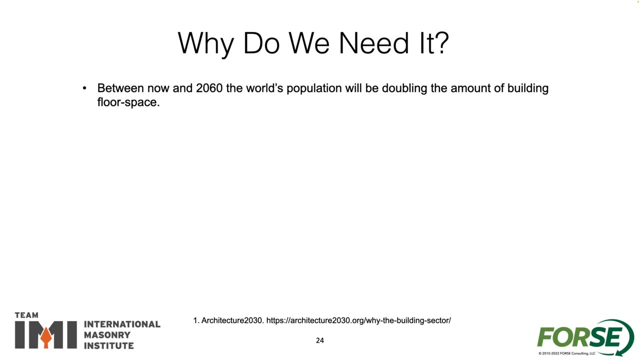 in education, and having a plan and trying to kind of push this initiative forward certainly is going to help us make a lot of progress along the way. So one of the things that is out there is: between now and 2060, you know, we're going to be able to do a lot of things. 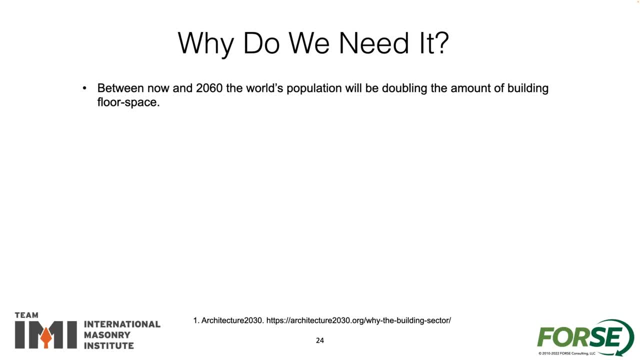 So one of the things that is out there is between now and 2060, is the world population will be doubling. the amount of building floor space, I mean the amount of built environment that we have- is certainly increasing, And so we want to make sure that, as we are looking at that, 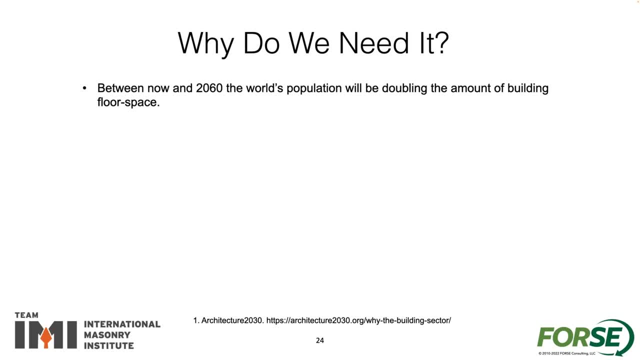 and building up. we are trying to do that as responsibly as possible. As you can see that the amount of carbon that we have and we use to build this environment is pretty, pretty high. So embodied carbon will be responsible for almost half the total new construction emissions. 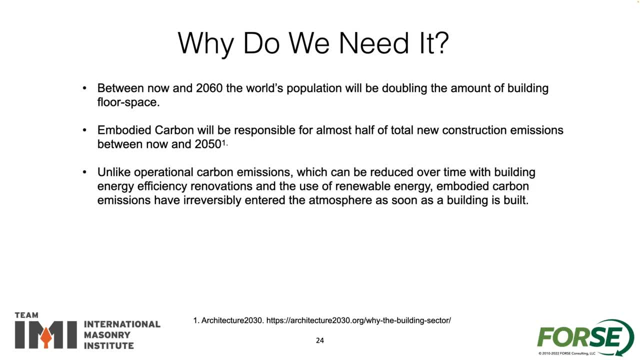 now in 2050.. And like operational carbon emissions, which can be reduced over time with building energy efficiency and the use of renewable energy, embodied carbon emissions are reversibly entered into the atmosphere as soon as the building is built. So right it's. once it's built, it's done, it's built. 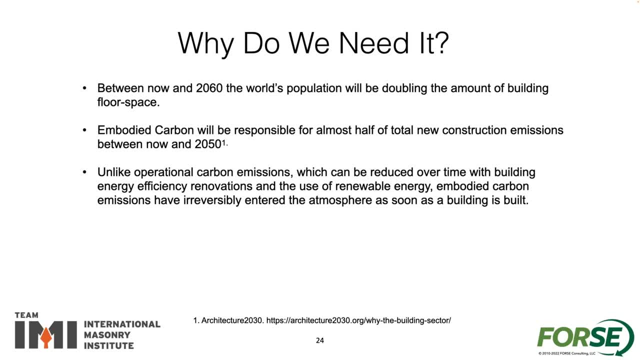 There's not a lot that you can do with all of the embodied carbon that went into constructing it. So, operationally, I mean now there's a lot going on. I mean obviously we can make improvements over time and we will. I mean there's, so there's a lot of time. 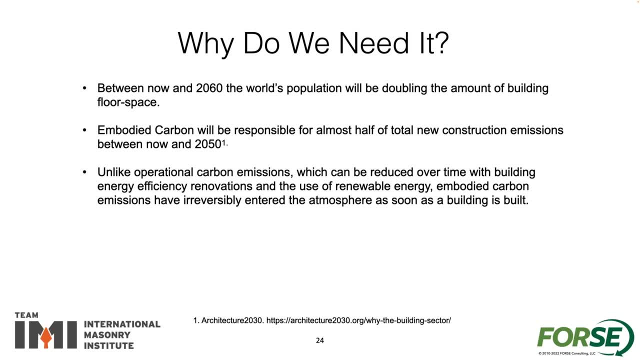 you know is on the side of you know the operational carbon emission. So you know, as different innovations come into play, we can certainly utilize those, but the embodied carbon is something that's gonna be there once the building is built. 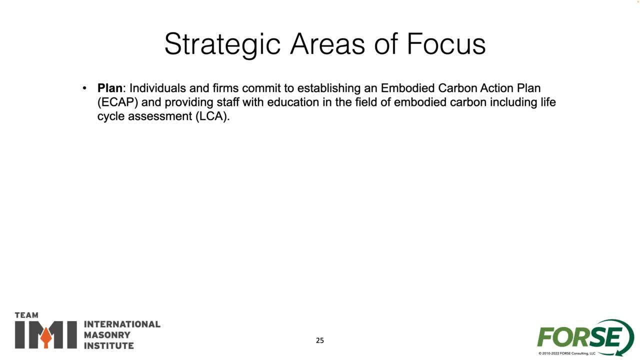 and there's really not a lot we can do with it. So I'd say some strategic areas of focus is just having that plan for individuals and firms to commit to establishing an ECAP or E-C-A-P and provide staff with education. the field of embodied carbon. 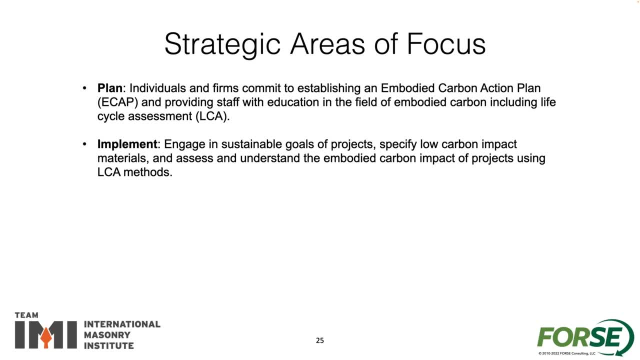 including life cycle assessment, engaging the sustainable goals of projects and specific low carbon impact materials- Again, we talked about that already a little bit- and then sharing embodied carbon with your structural system to a central database for understanding. Now, that could certainly be, hopefully within a firm. 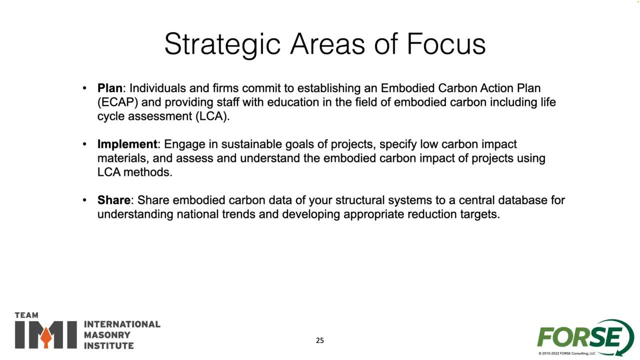 for sure within branches of a firm, but hopefully across firms. And you know, I think that's a great question, And I think that's a great question, And I think that's a great question, I think that's a great question. 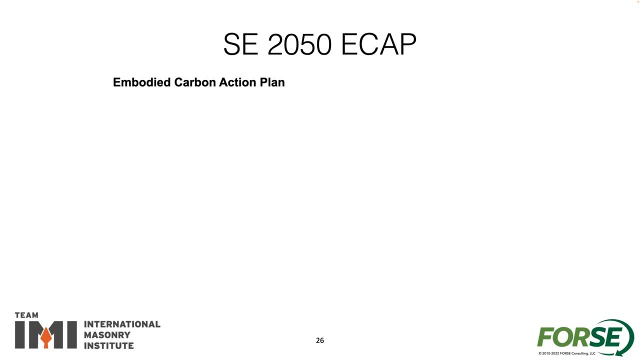 And I think that's a great question, And I think that's a great question, And I think that's a great question. So the SC2050 ECAP- the embodied carbon action plan terms- are given six months to develop an ECAP. 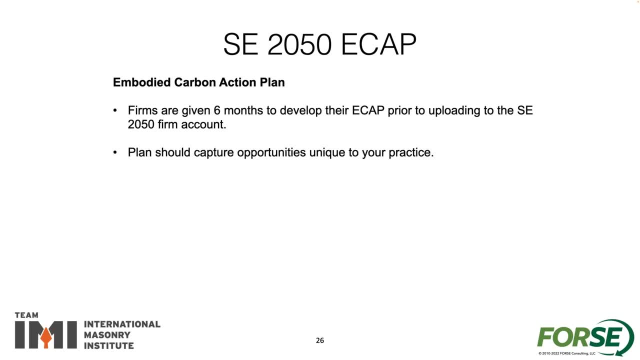 prior to the uploading of the SC2050 firm account Plan to capture opportunities unique to your practice. All the ECAPs are public, So I guess, again trying to get this out to the larger community, Firm will have the option to upload their ECAP document. 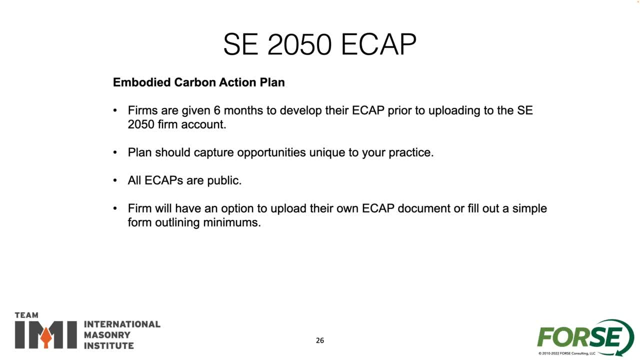 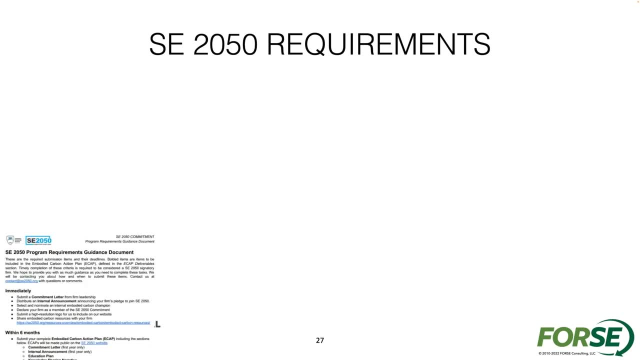 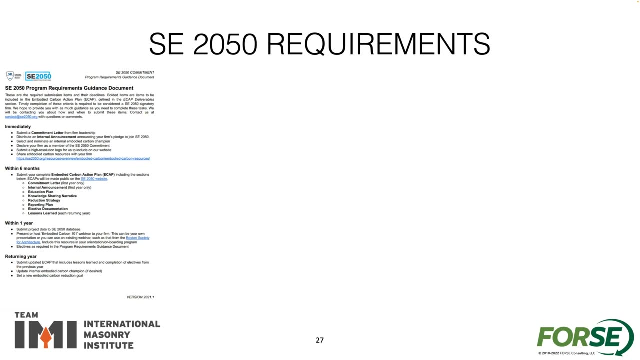 or simply fill out Firm outlining some of the minimums that they're looking at. So there's a lot of different requirements for SC2050. So they have kind of the step-by-step program, immediately within six months or a year, the returning year. 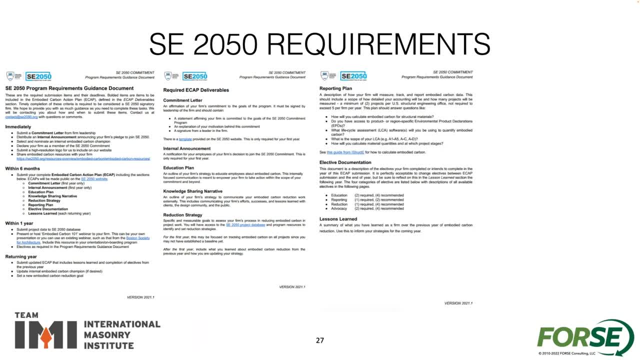 There's some of the deliverables that they want to see within a reporting plan, for you know how things have went and lessons learned. So, again, all different things that we can try to implement to build into making a better built environment, kind of going on and into the future. 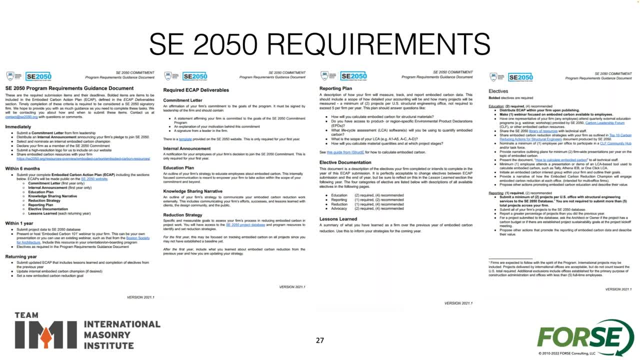 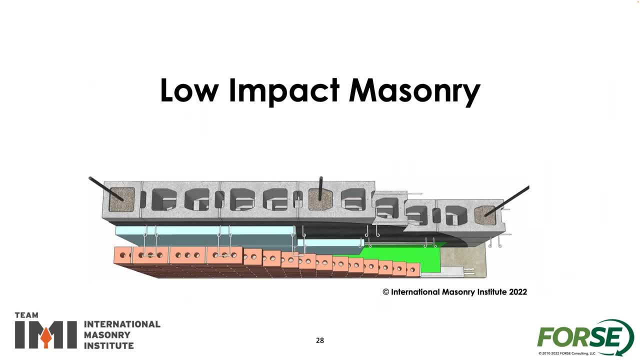 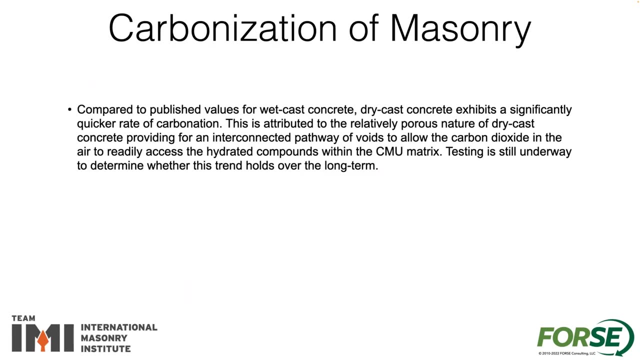 So everything from SC2050 is up online SC2050.org, where you can download and look at any one of these documents. So, looking at masonry in general: low impact masonry, carbonization of masonry, Compared to publish values from wet cast concrete. 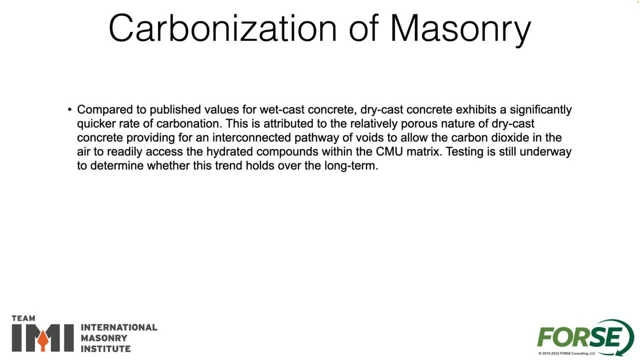 dry cast concrete exhibits significantly quicker rate of carbonization. This is attributed to those numbers that are, you know, Max, two days to the poorest nature of dry cast concrete or interconnected pathway of voids to allow carbon dioxide in the air to readily access the hydrated compounds in the CMU matrix. 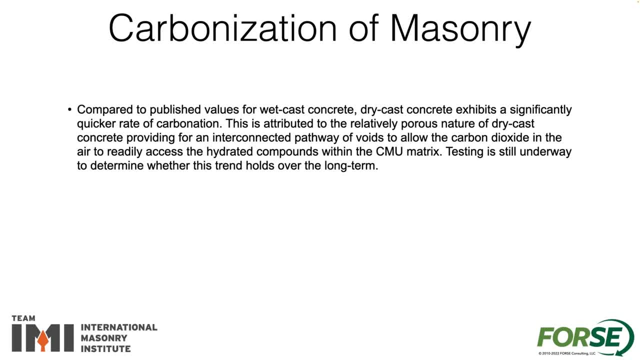 That's a multiple testing is still underway to determine whether or not this trends hold over time. So I think Mastry's got to have again. just with the voids and the way that it's manufactured and built, that has a good chance for a quicker rate of carbonization. 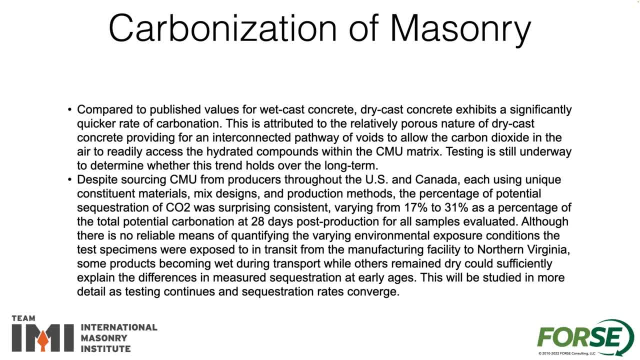 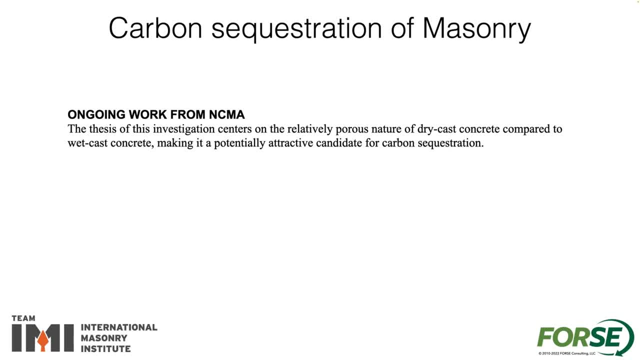 So you know NCME, you know, like I said, I've cited them several different times. They're going to be kind of working behind the scenes to try to do a lot of the work here for some of the reporting and information. 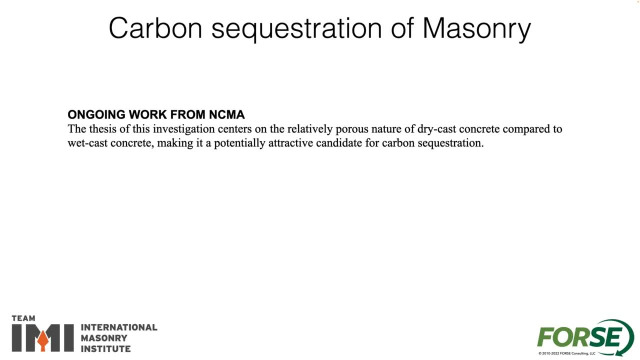 on mainstream material, obviously trying to get more and more information out there, you know, trying to focus on the poorest nature of a dry cast compared to wet cast. I think it's going to be a really good- could be some really good reporting. 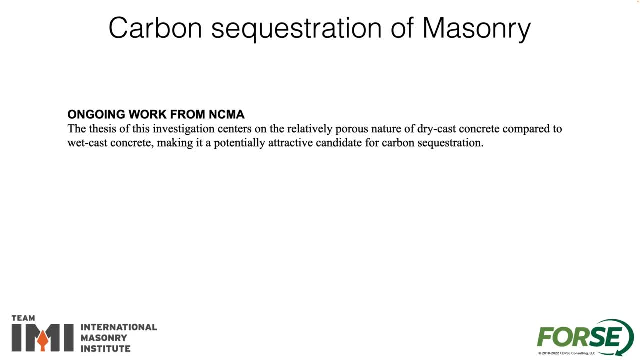 So there's a lot of, you know, potential with Mastry, just in the terms of not just the void that are inherent within Mastry itself, but just the material itself is a lot more porous. You know, it's something where you can obviously have air. 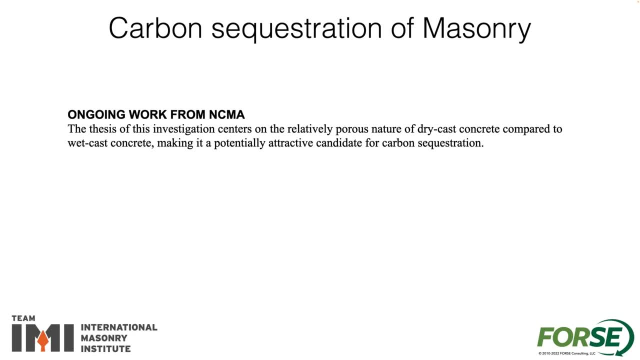 and water that can move through the material. It's obviously not like a totally voided, but it does have a very good material. it does have a very good material, the setup for being able to work very well. So, with all the research that we conducted, 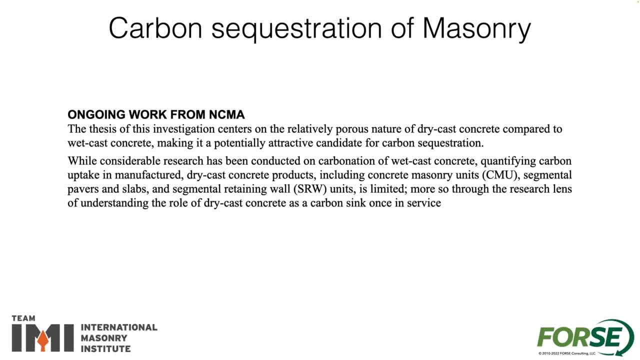 on carbonization of wet cast quantifying carbon uptake manufacture. dry cast concrete products, including CMU segmental pavement, slab, segmental walls- is limited, So more research is needed in understanding this. And you know this. carbon is a carbon sink. once in service. 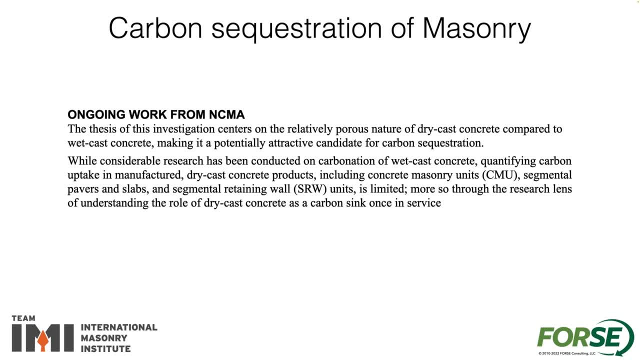 So there's a lot of stuff that's going to be coming out from NCME. A lot of this stuff is still relatively new, And so we're just trying to keep up from the industry perspective and try to get that information out as quickly as possible. 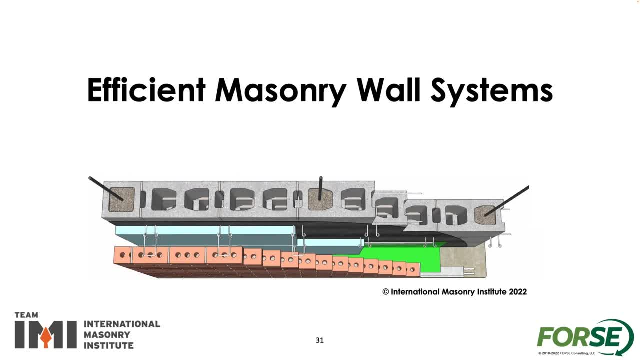 The biggest thing that I think that we can do with Mastry- before some of the reporting is done, before some of the trying to define exactly what Mastry is, is just having efficient Mastry wall systems. That's going to be a huge part of making sure. 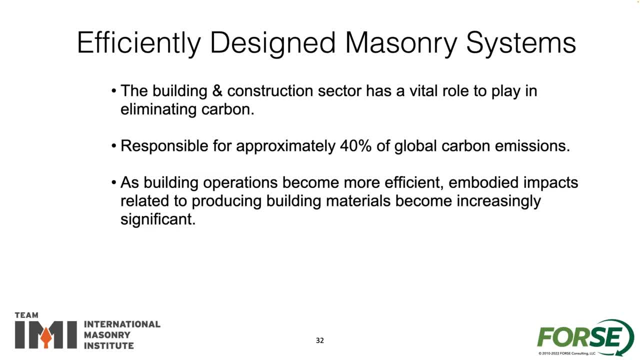 that we have thinner walls, less reinforcement and grout, less material And that's going to be in there for our lintels and all the different elements for our Mastry and wall systems. It's certainly going to really help to try to control some of the overall impact that Mastry has. 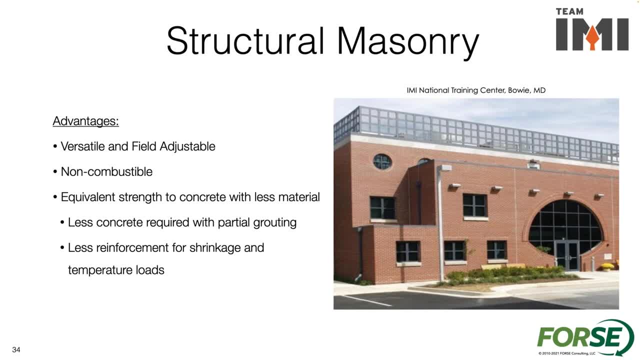 You know, efficient Mastry systems overview. I mean the advantage is you have versatile, field adjustable materials, You have non-combustible materials, You have equivalent strength to concrete with less material. I mean that's just inherent to what you're looking for. 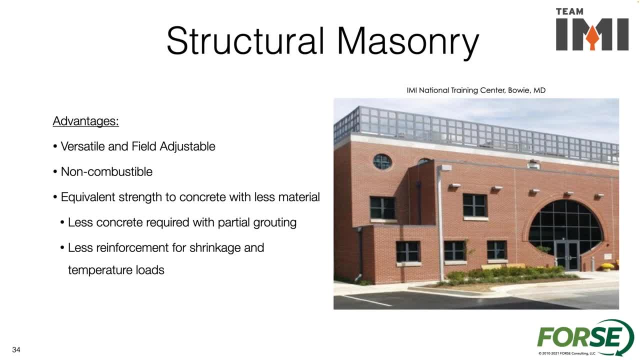 You can have partial grouting and reinforcement. You can have reinforced brick so that we can utilize even higher strengths of masonry and less material, thinner walls. I mean, there's a lot of things that you can take advantage of there. Less reinforcement for shrinkage of temperature. 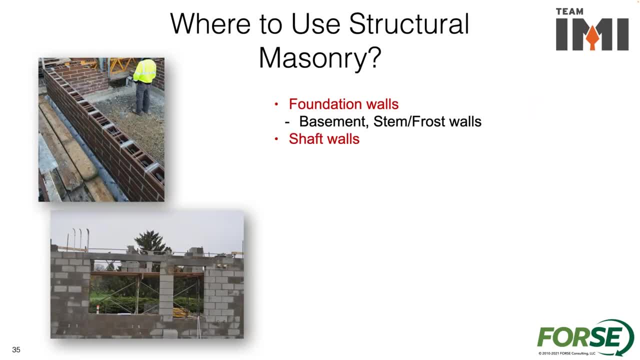 loads just because of the prefabricated nature of masonry. So where do you use structural masonry on projects? I mean trying to utilize the material in new areas where we can. you know again where we need hardened materials: foundation walls, base and stem walls, frost walls. 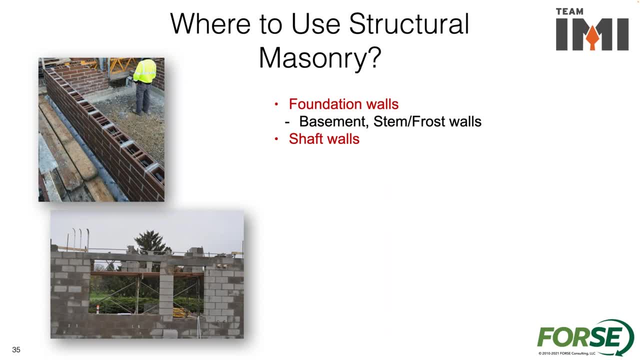 Those are typical areas where we see a lot of concrete still being poured into the ground And it's obviously places where we can put in a masonry foundation wall. You can save a lot less, have a lot less material being put into those walls. 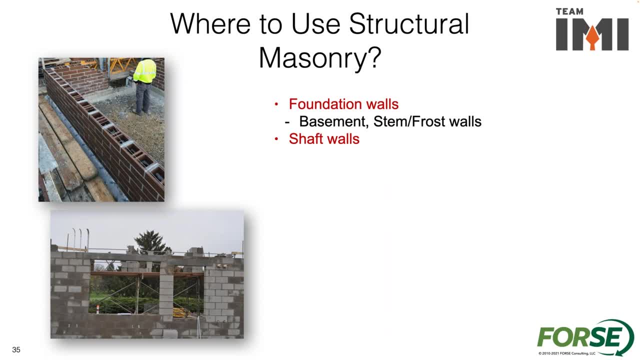 And then with the partial grouting and reinforcement, you know we really don't need to fill them grouted a solid full of grout just because there's really no need for it. And if we need to keep the water out we just have to waterproof. 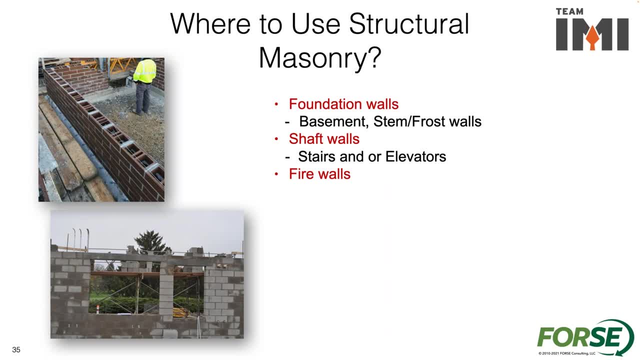 Shaft walls, stair and elevator shafts- again, those are probably firewalls, But those are also elements that, once we have them there, we want to make sure that we are utilizing them from a design perspective. Firewalls, shear walls- we have long perforated shear walls. 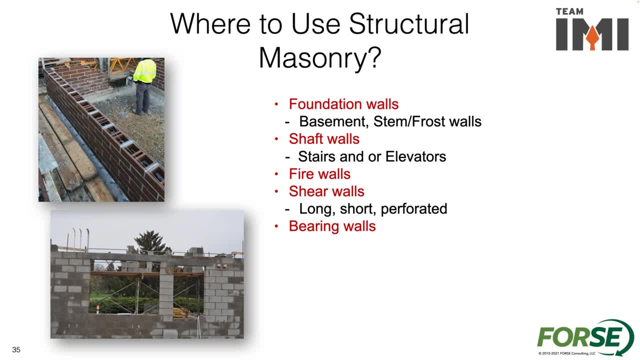 that we want to use Bearing walls, interior and exterior partition walls. you know no structural function, but you know those certainly can be thinner and unreinforced and grouted. You know there's all kinds of places for efficiency. 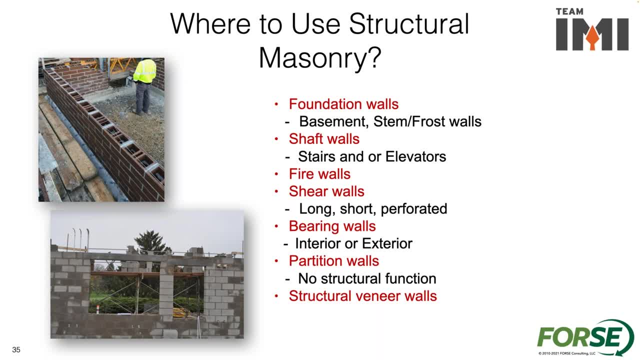 You know, a lot of times when I look at masonry and design, you know I often am talking about efficiency, efficiency. I want to make sure masonry isn't valued and engineered on the projects that it should stay in for. You know, and a lot of those same conversations. 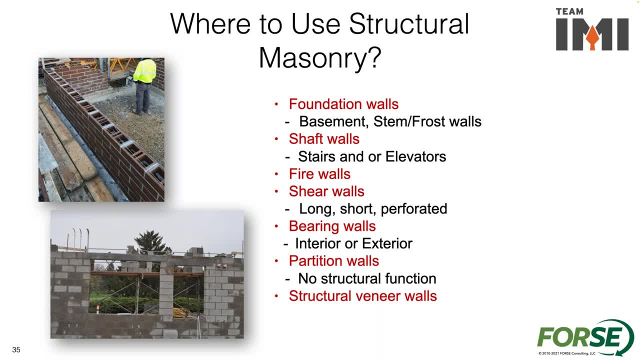 and comments also apply for reducing the embodied carbon in a building. If we are efficient with materials and using less and less materials, it's certainly going to cost less. It's certainly going to cost less up front, but it's also going to be having a lot less embodied carbon. 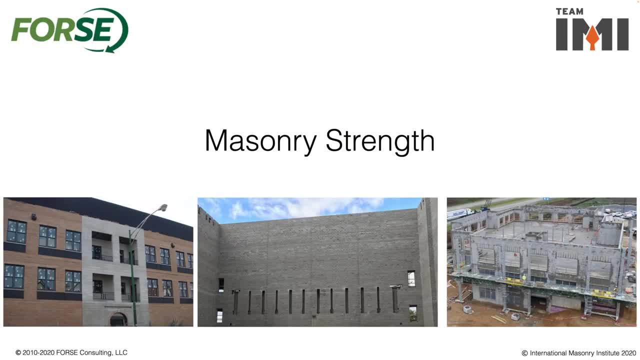 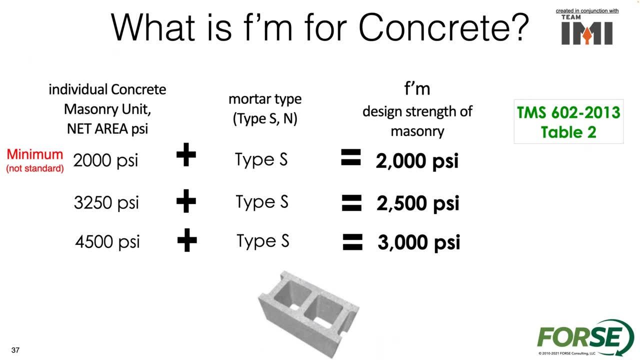 in the structure as well. So again, masonry strength- this is something that I've made mention to once or twice today, making sure that we take advantage of the stronger. You know, the minimum is the minimum, That's 2,000, the maximum 4,500. 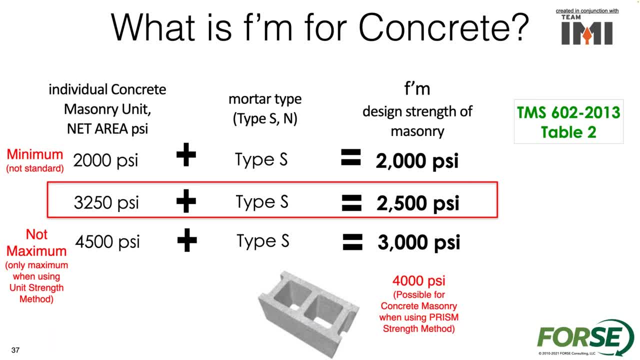 You know that's something that we want to make sure that we utilize. We have that typical 2,500 that we want to make sure that we do consider. You can even go up to 4,000.. to 4,000, if you need to. 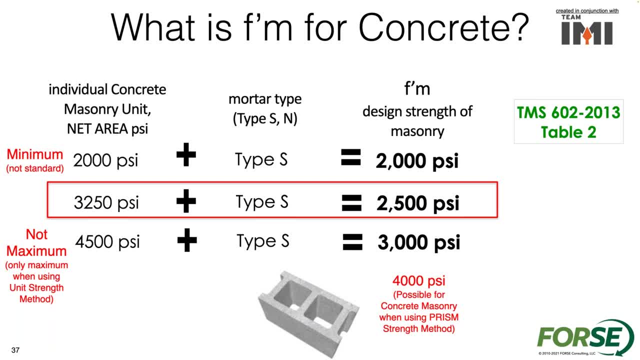 If there would be some special reason to get higher strength masonry, we can do some prism tests to get you know even a thinner and more efficient wall, But you're looking at the typical concrete masonry at 2,500,. well, that's an environmentally friendly perspective. 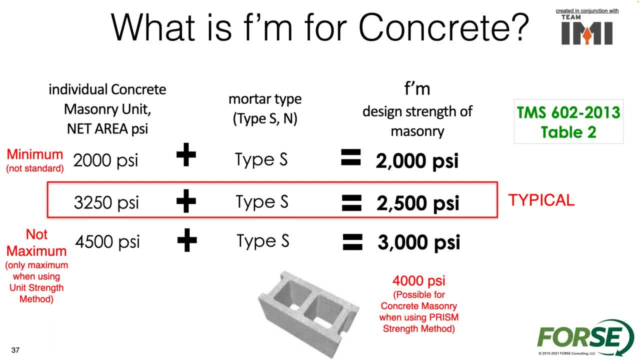 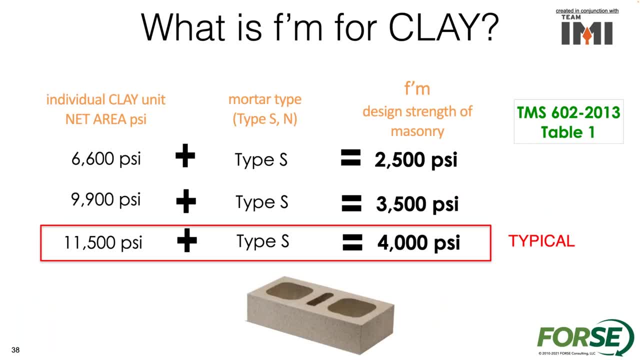 right there, just trying to take advantage of what we already have with masonry, instead of designing to a lower strength. Certainly, any time that you do venture into clay masonry, reinforced clay masonry is. you can even go even higher with it at prime m. 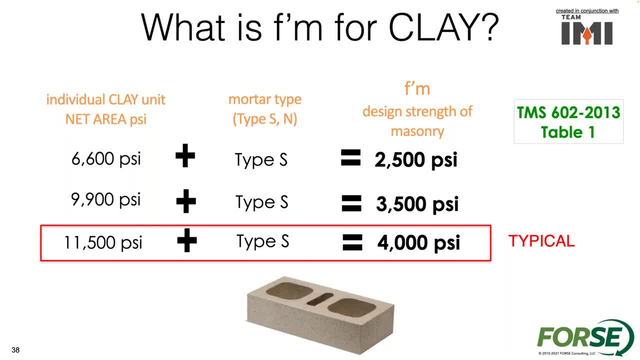 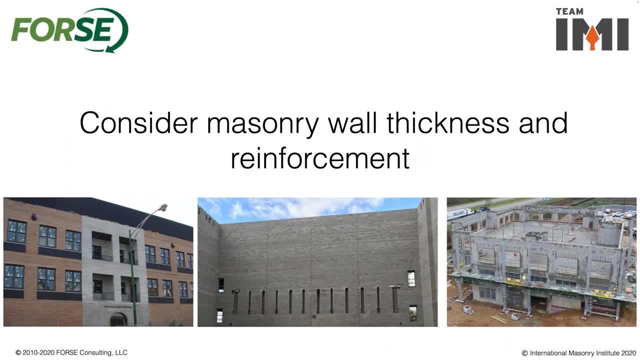 you know, definitely not at 2,000, 2,500, but all the way up to 3,000 and 4,000 for the overall design. So again, consider some of those wall thicknesses and heights. you know, thinking about, you know. 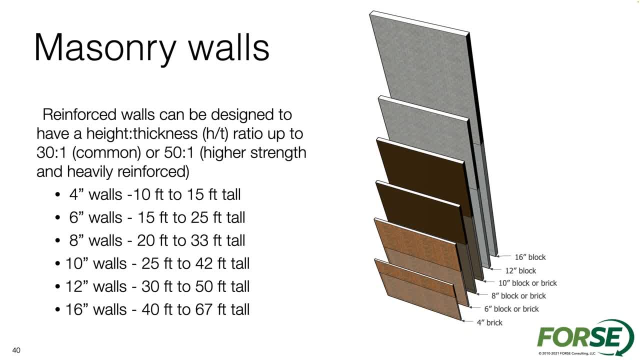 the overall design: four inches, all the way to 16 inches. with our masonry walls, you know. four inches can be a reinforced clay masonry design. You can go all the way to 16 inches reinforced concrete masonry design. A lot of times looking at the efficiency again. 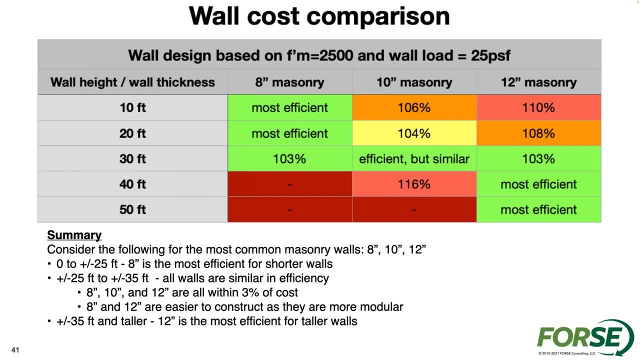 you know what's gonna be the most efficient. It's gonna depend on the height of the wall. A 12-inch wall isn't always the most efficient. Sometimes there's just way more material there than you need. So a chart like this- this is a chart that I created- 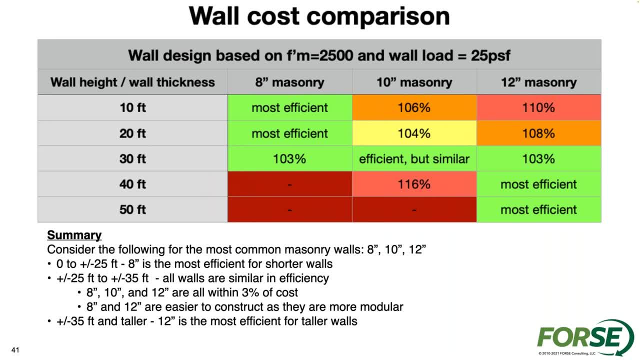 for local contractors to try to point them to. you know when 12-inch walls should come out of projects. Any time that we have a shorter design, you know it should be a six or an eight inch wall. So this chart's kind of giving them, you know. 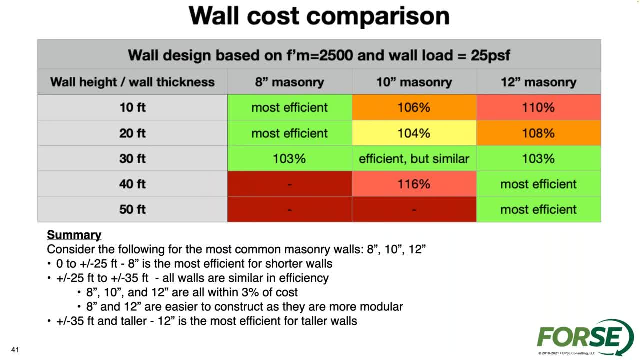 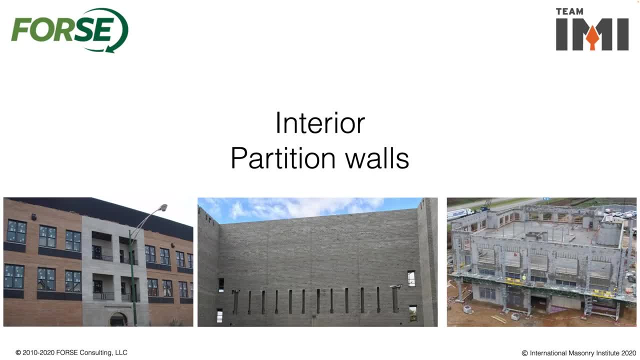 at certain heights, when does it start to make more sense to use thicker masonry and for shorter walls, when to make sure that we use less masonry? You know those partition walls that we talked about, making sure that we have those as efficient as possible. 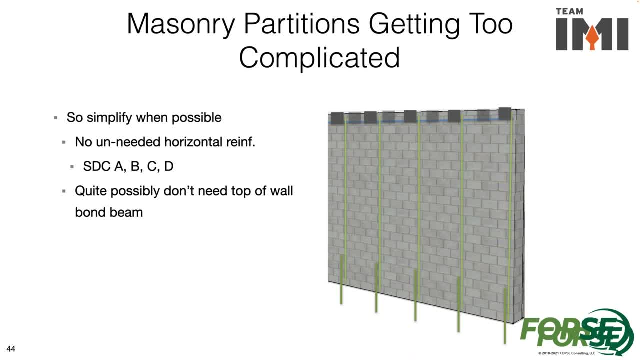 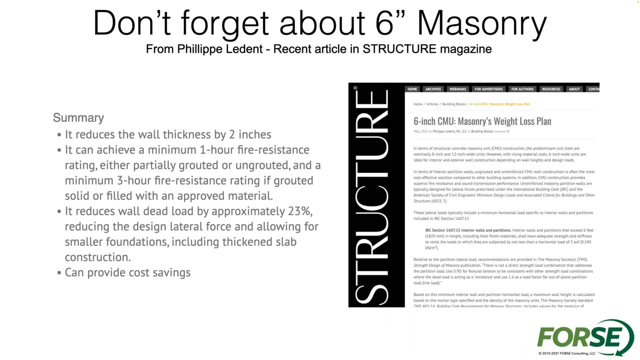 least amount of material as possible. try to get as much reinforcement out of those and all the connections. any time that we can make all of that stuff more efficient is gonna be better and certainly gonna help with the environmental impact of the design. You know, don't forget about six-inch masonry. 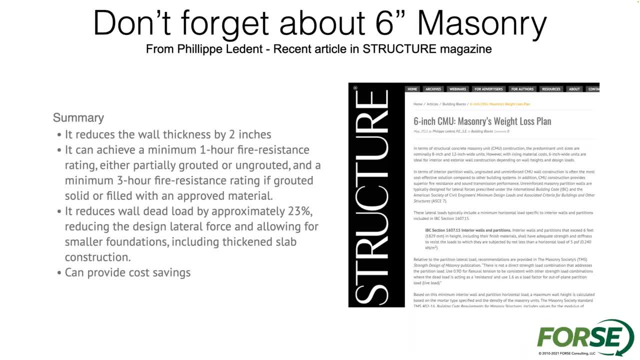 When we look at materials and availability. you know six-inch masonry is certainly something that can achieve quite a bit. You know I had it in a lot of the partition wall charts but you know a six-inch masonry can certainly help. 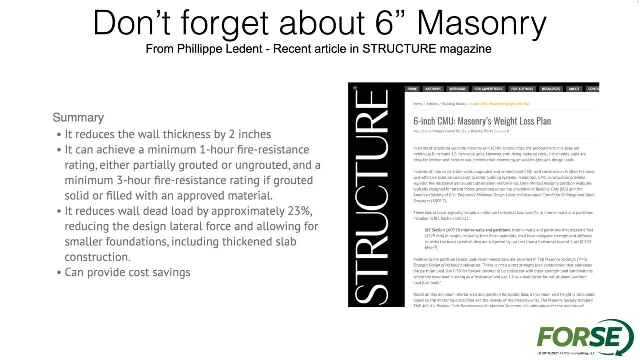 save material on a project. So any time that we're looking at reducing the carbon footprint and limiting some of the material- sometimes six, you know, the move to six-inch masonry might be a really nice move in that direction to try to save some material on projects. 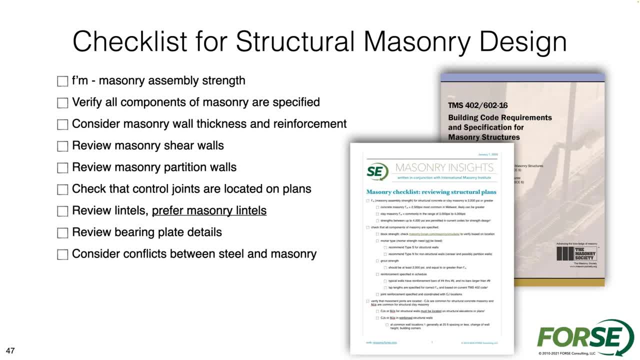 So you know what we did with the masonry society, NCMA and IMI is we developed an overall checklist for structural masonry design, trying to make sure that everybody's again more efficient design-wise- but certainly that really does from the cost perspective. 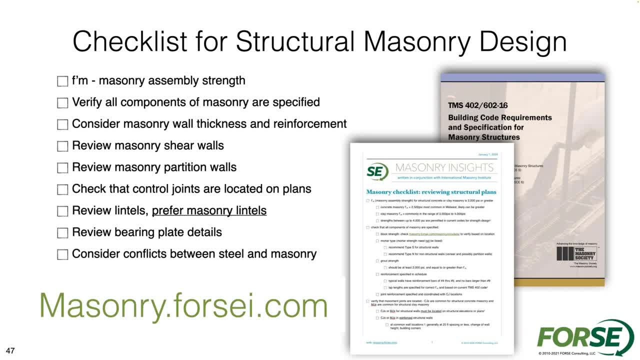 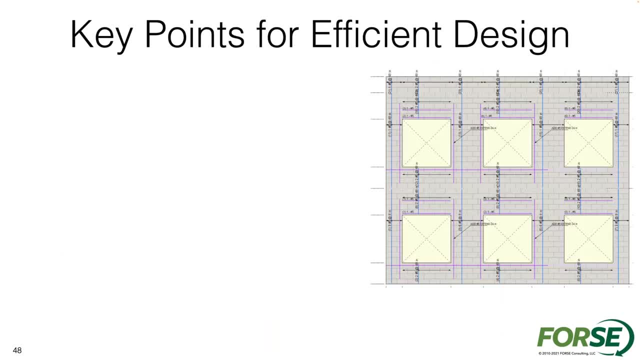 but that certainly does help quite a bit for making sure that we're efficient in terms of environmental impact. So we have some key points for efficiency again: using that higher strength of masonry, using masonry lintels instead of steel. control joints away from openings. 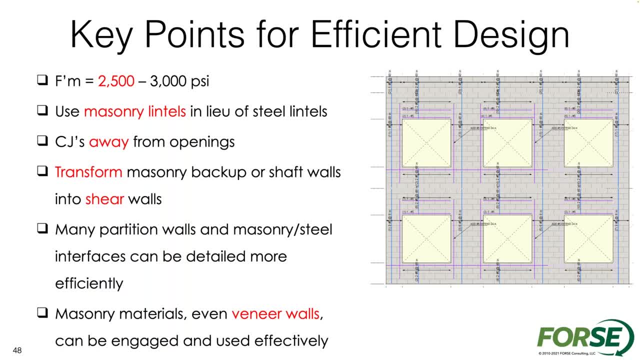 that's just going to give us a much better design. Transform from masonry backup to shaft walls into shear walls. Try to use your masonry as much as you can. If you have a shaft wall, make it load-bearing. If you have a shaft wall, use it as your lateral system. 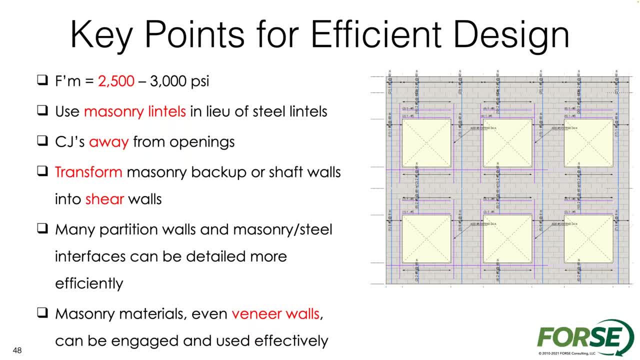 You know that shaft wall's there for durability and fire protection. Try to utilize that wall for as much as you can for your overall structural design. Many of the partitions and interfaces can be eliminated and designed more efficiently than some of those top-of-wall connectors. 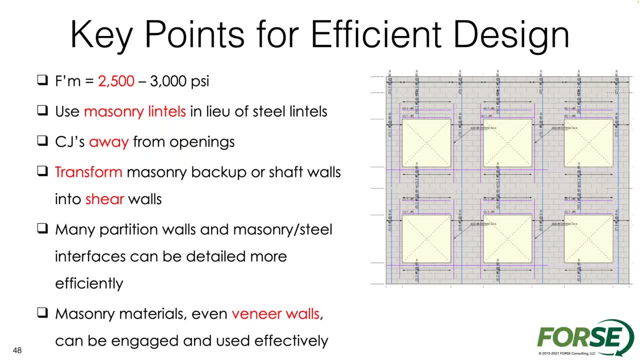 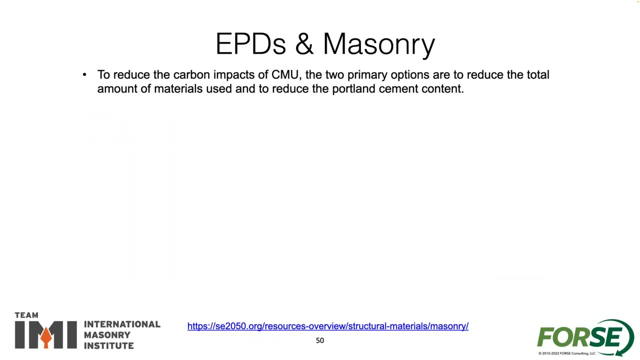 We're trying to get much, much lighter connections again from a cost perspective, material perspective, and then just trying to use less and less veneer material- any materials that you can. Environmental product declarations reduce the carbon impacts of CMU. 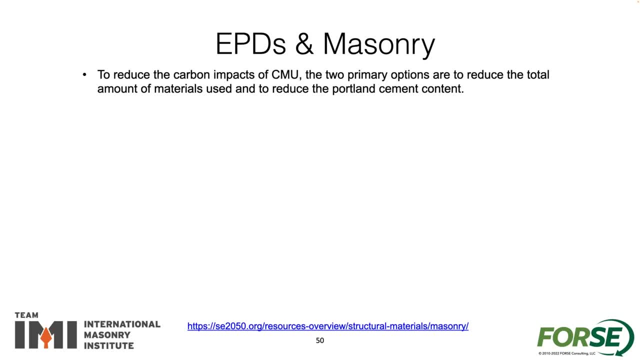 The two primary options are: reduce total amount of materials. Again, efficiency: Use total amount of Portland cement. Reduce the materials. Use strength design and ESD. Don't rely on empirical design. That's something that we talked about all day today. 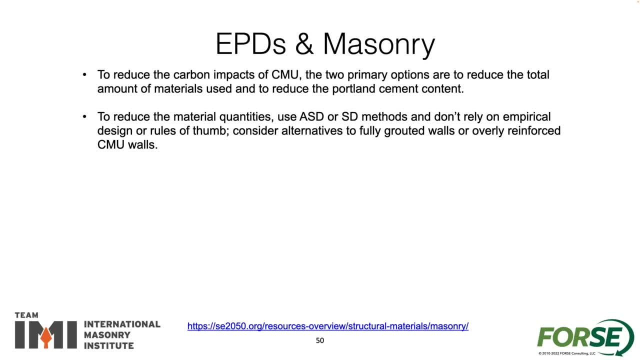 Empirical methods are moving into the appendices of the code, and so we just want to keep moving away from that and keep going. There's no reason to do that Empirical. why do I? why am I so hard on empirical methods? 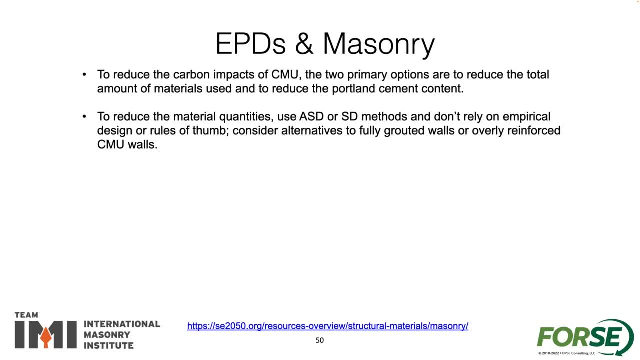 Because they're conservative, overly conservative, to save designers time. Any of those rules of thumb or any of those time-saving tips from a design is always going to cost a lot more on materials, So always try to use something that can be more environmentally friendly than that. 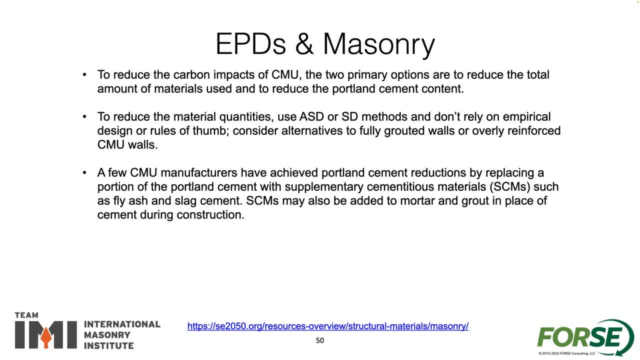 There's some different block manufacturers that have achieved Portland cement Portland cement reductions by replacing Portland cement with supplementary cementitious materials like fly ash or slag content. So try to make sure that you ask about it, you look into that, see if that's a possibility. 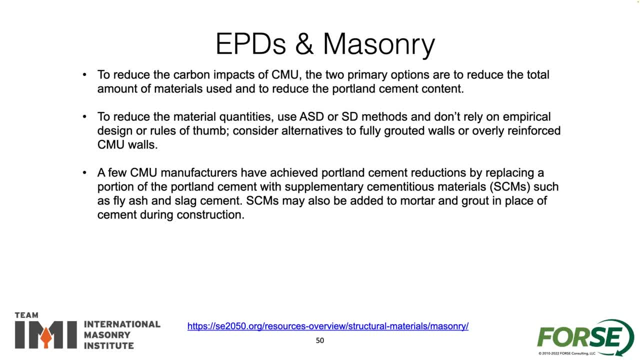 Again, if we're creating a specialty mix, maybe that's something that comes more into play, or maybe that's something that they produce off the shelf, and then we certainly want to understand that And then specify a prism strength method rather than unit strength. 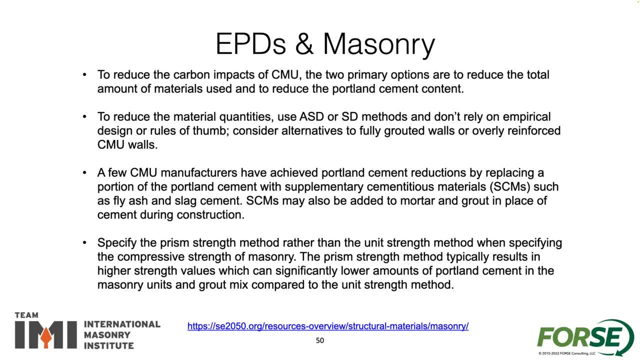 method. That's certainly going to be more similar to what you would do with concrete, but you definitely want to have some knowledge when going into it. You want to have some knowledge for what the actual products typically are so that you can have a reasonable understanding. 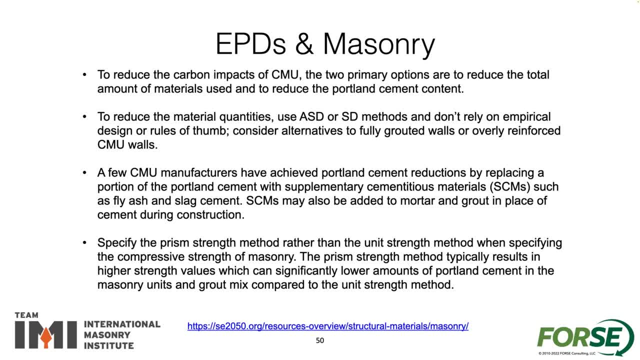 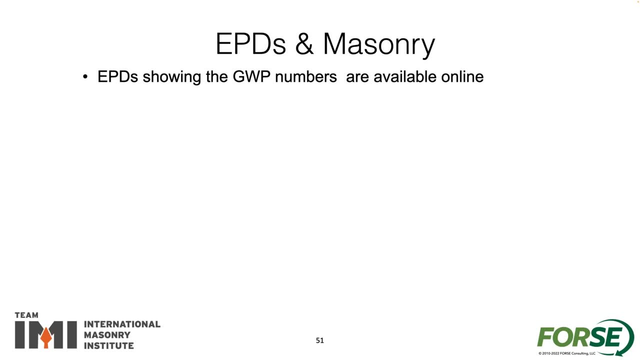 for what a prism strength. Usually prism strengths you can have 15% to 20% to 25% more capacity. so any time that you can do that, you're certainly going to be using less material in your design. So EDPs and masonry EDPs showing GWT numbers. 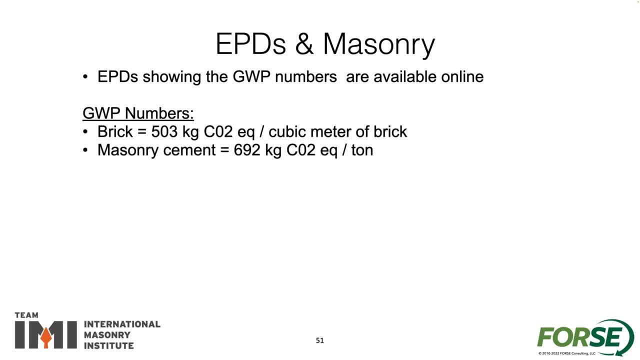 are available online Some of the different numbers, just so you can see where they are: brick and concrete, masonry, cement, non-fabricated steel. you can see the low GWT numbers for some of the masonry materials versus some of the steel counterparts. 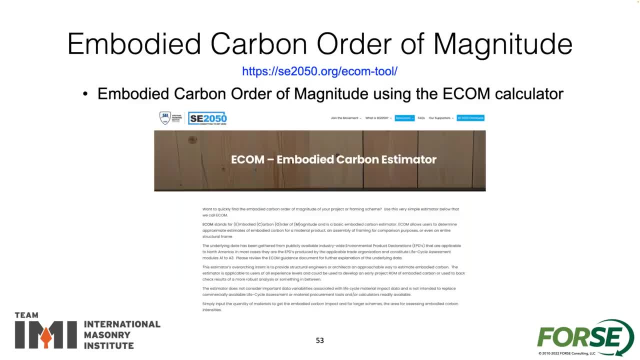 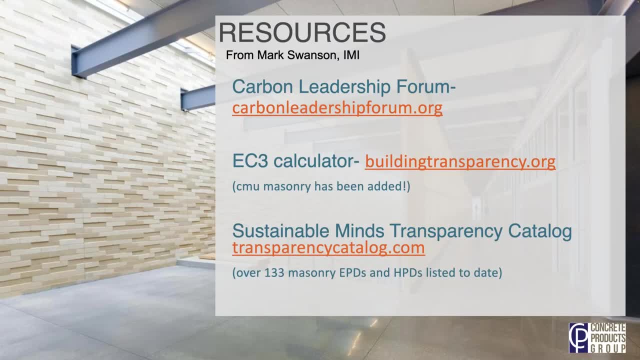 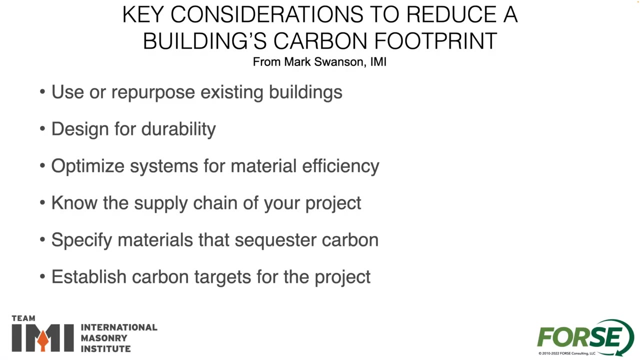 Some of the other resources that are available out there: carbon leadership forum, EC3 Calculator, Sustainable Mines Transparency Catalogue- all different places where we can get more information on EPDs and information on environmental impact of masonry. to remember here is to use or repurpose existing buildings. 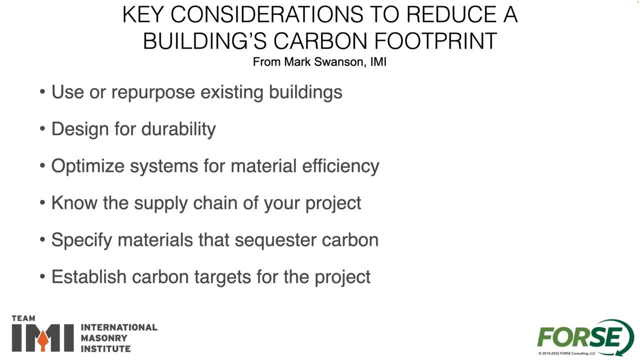 I mean that's obviously the greenest way that we can be designers: A design for durability, optimize systems for material efficiency, no supply chain of the project, specify materials that sequester carbon, establish carbon targets for projects. I think all of those things that we can do. 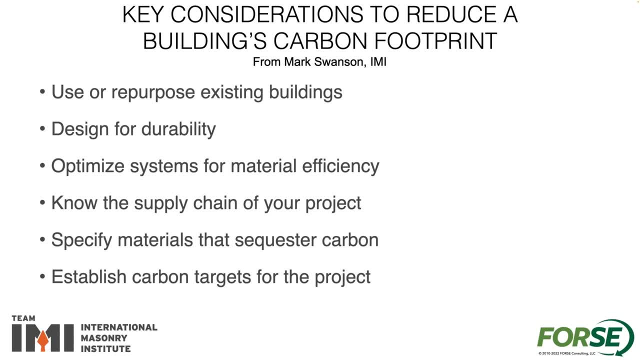 to try to move towards the net zero, move towards the kind of that key place that we want to be. 2050 is certainly gonna help us be more and more sustainable with masonry and other materials, certainly over time. All right, so that takes us to another end of another section. 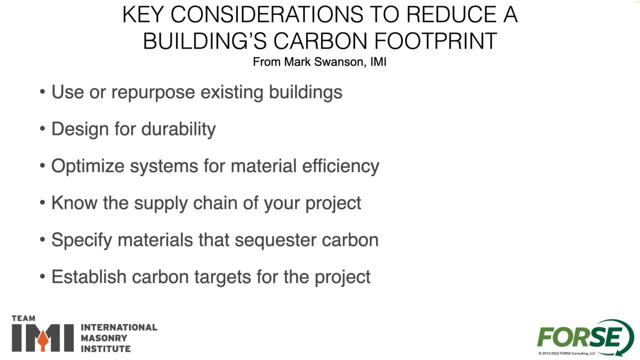 of why don't we take a five or 10 minute break, when maybe a 10 minute break be okay at this time and we could start back up at, say, 2.40, and then I think we'll go from 2.40 all the way to four o'clock. 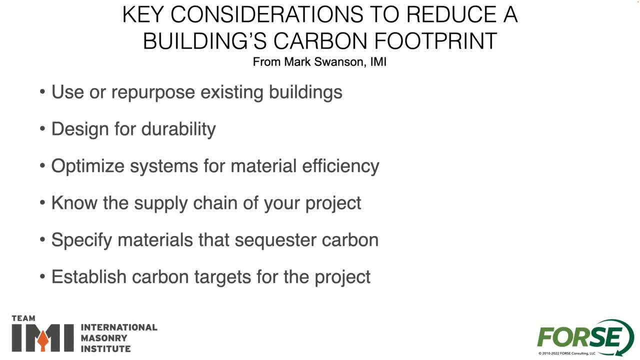 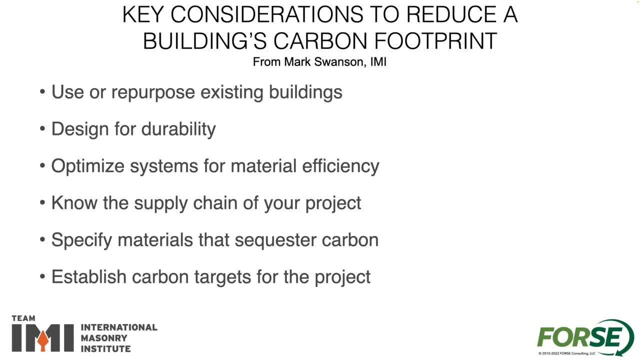 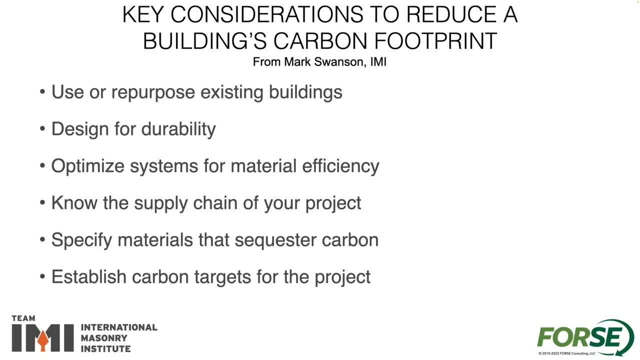 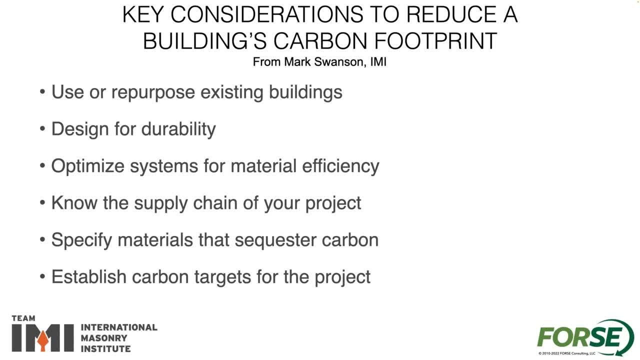 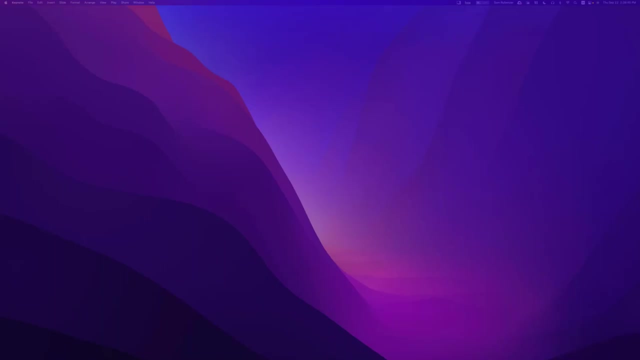 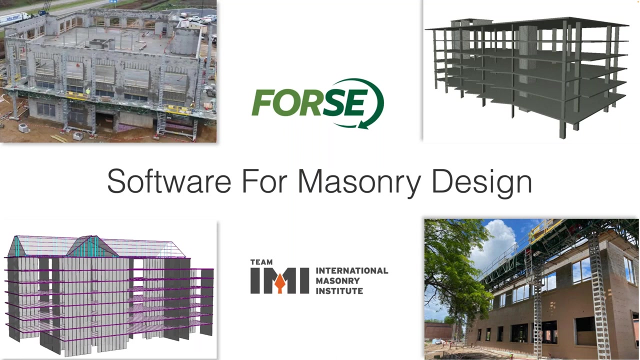 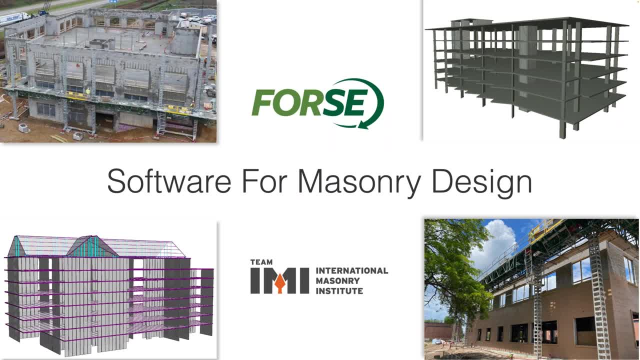 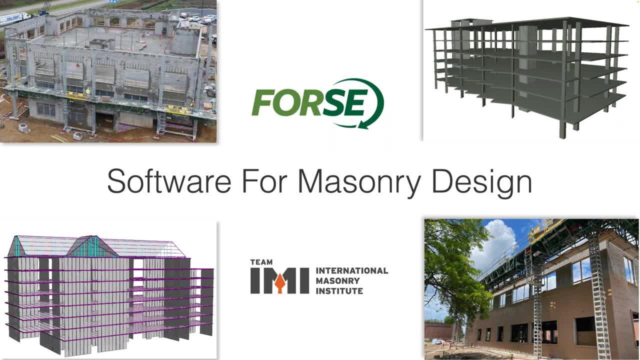 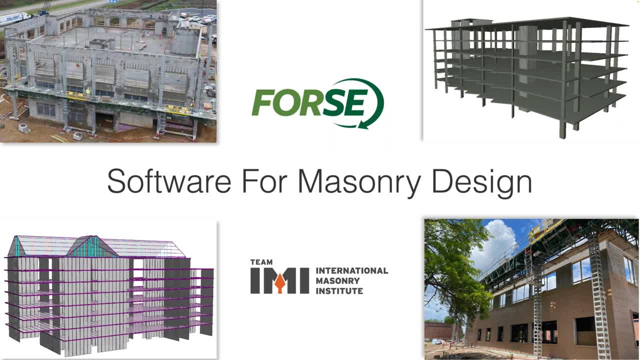 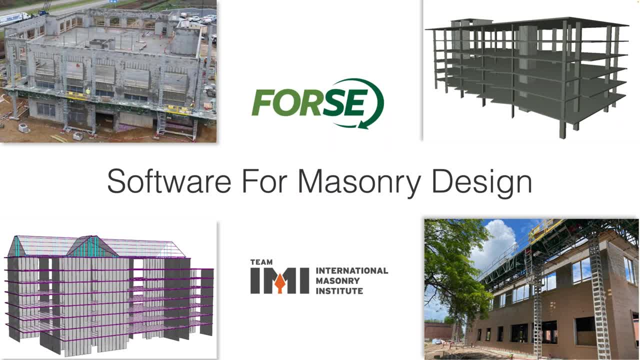 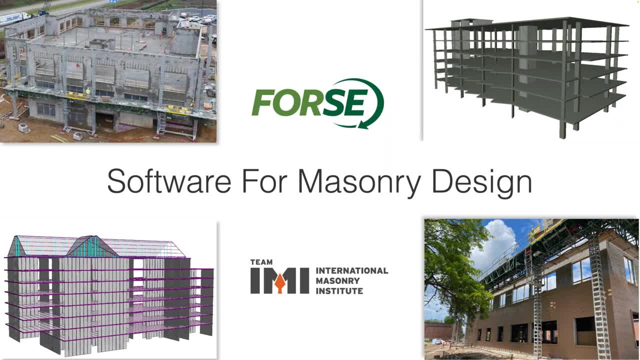 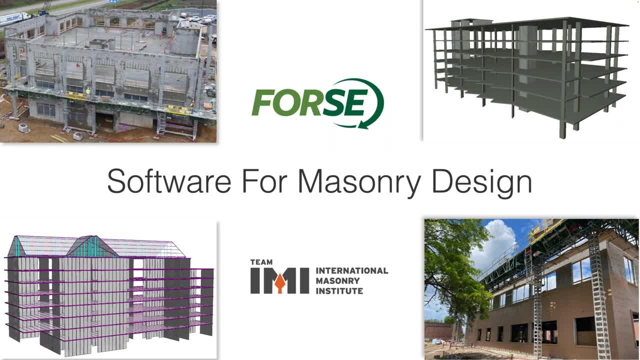 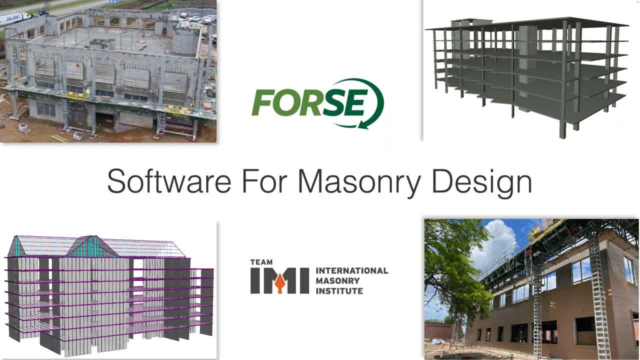 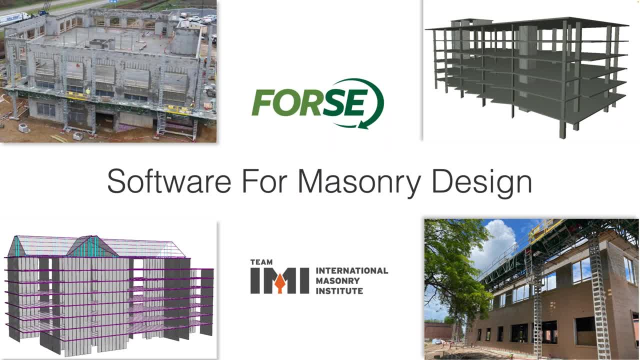 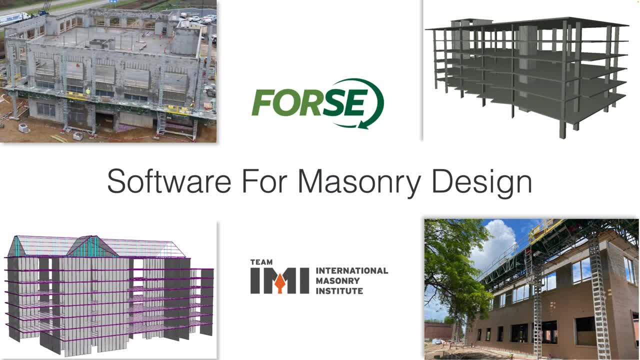 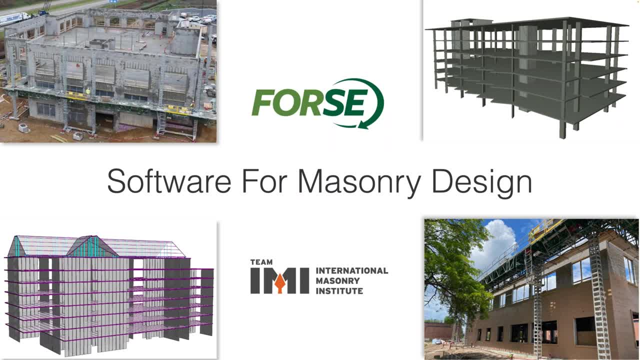 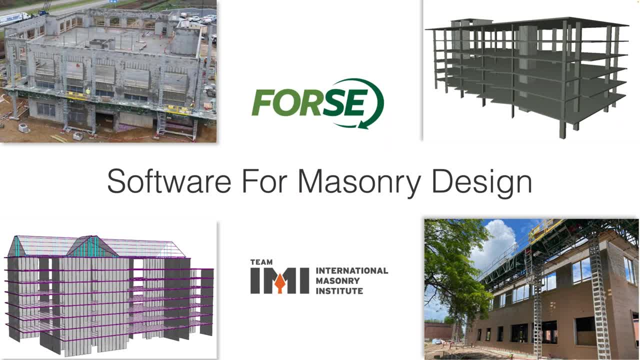 I think that's the end of it. yep, okay, So certainly you guys can certainly ask: oh there another question? Yeah, so the prism strength method is different from the unit strength method. I think that's what you meant. 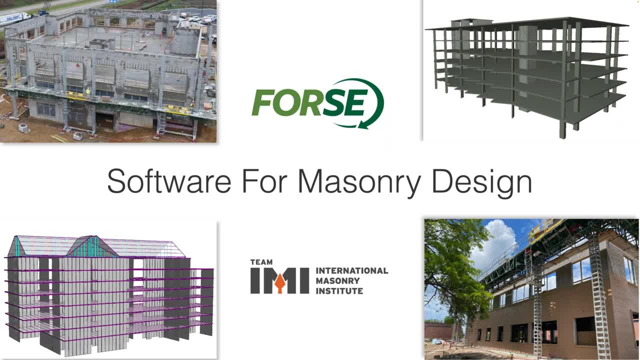 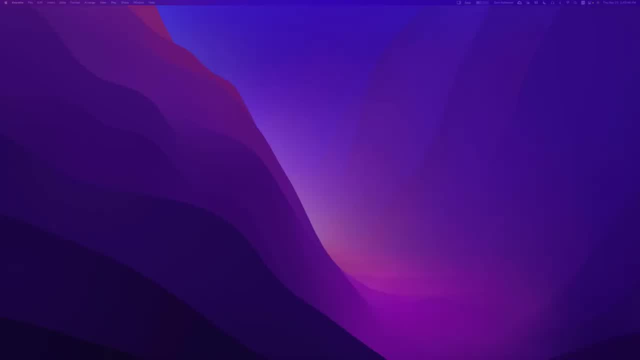 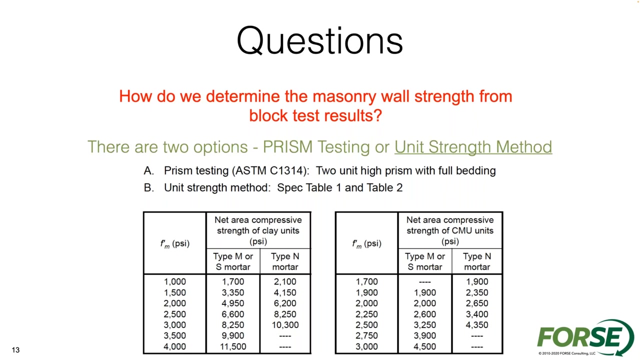 Let me see I could probably pull up. I'm gonna pull up that part of the presentation. Okay, so here's kind of looking at the two different, the two different options that you have: A being prism testing, ASTM C13, 14.. 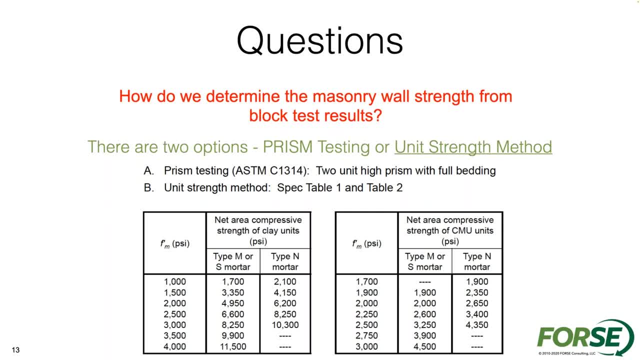 Really, you're gonna build a two unit high, two blocks mortar and you're gonna be doing the testing for, like I said, three different samples for prism testing. That's gonna be one testing method for determining the strength of masonry. The unit strength method is gonna be fundamentally different. 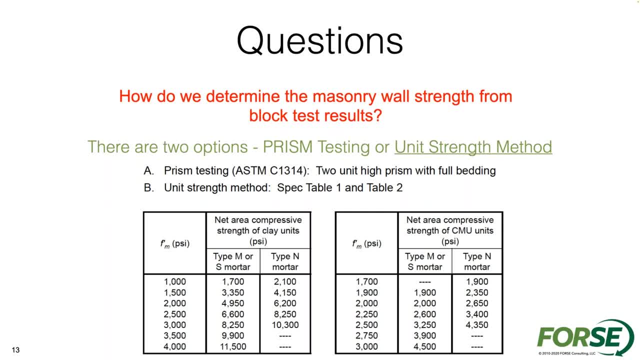 in that you don't do any testing. Unit strength method is just taking the materials that you have, that you're gonna be having for your project, The block strength you're gonna be using that. I don't know if anybody can see my cursor. 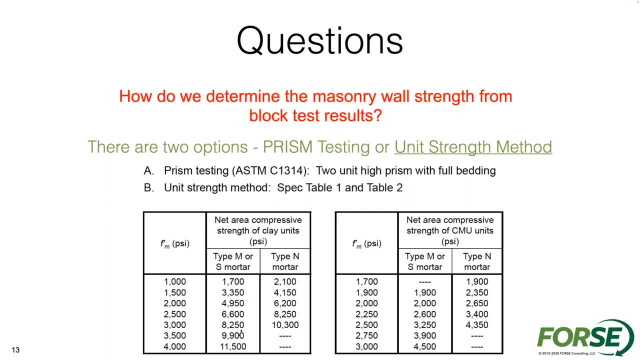 but the block strength. say, if I had type M or S again, if I had like 9900 or 1150 in terms of the overall block strength, if I have S mortar, then I know that my design strength would be 4,000.. 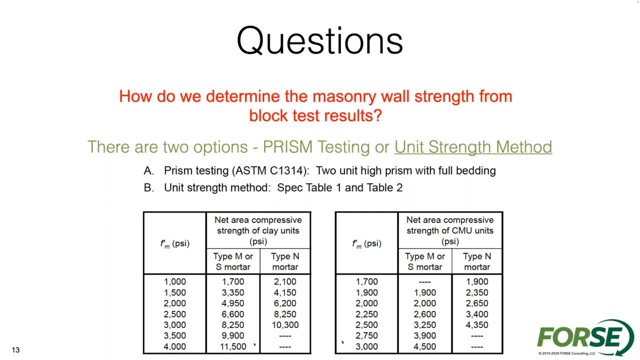 So unit strength is just taking material samples and utilizing those material samples and the mortar type that you're gonna be defining to determine the overall design strength. So it's just using tables in the code, The unit strength method. it's gonna be more conservative. 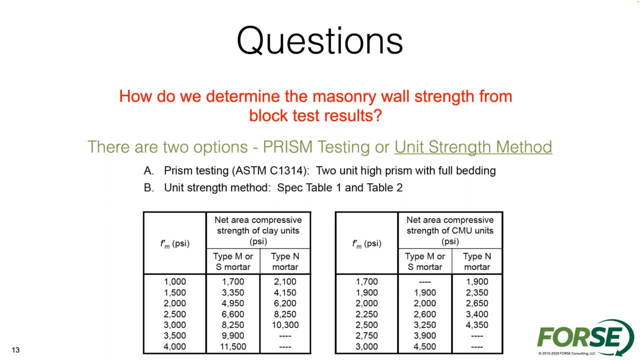 It's going to yield lower strengths. Prism test method is always gonna have a higher design strength that you could be able to utilize for your project. So two fundamental differences there If you want to get the most out of your masonry product in projects that you're looking at. 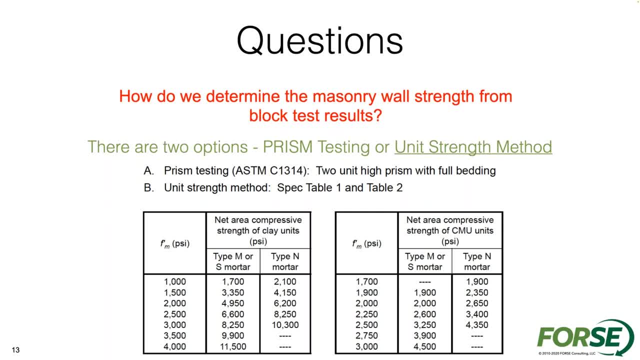 use a prism test method. The reason that people don't use the prism testing method is just because the prism tests are taken generally close to the actual project construction. And so if your design strengths, if they aren't meeting the prism tests, aren't showing your design strengths. 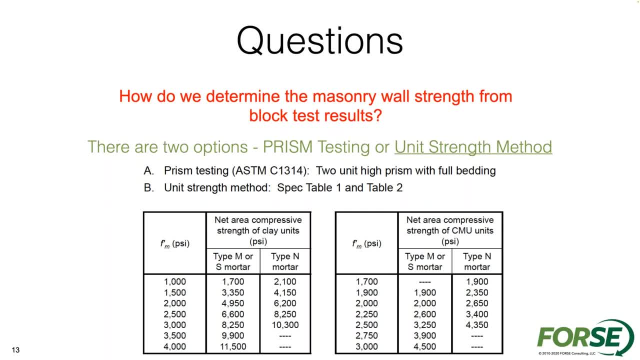 being met, then you have to go back to the drawing boards. Maybe you have to get the block manufacturer to make more block. There can just be some slight delays. It does require a manufacturing process to happen in between asking for more strength. So it's a little bit different than the concrete in that way. 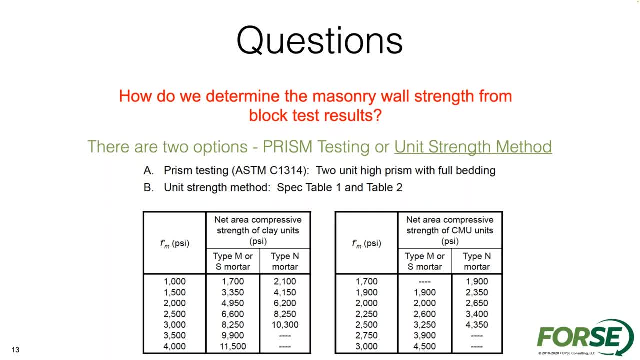 and the prism strength method takes some time for the results to come back and then it actually there's time involved in making the new units and having them shipped to site. So prism strength is always gonna give you a higher design strength, but unit strength method more conservative. 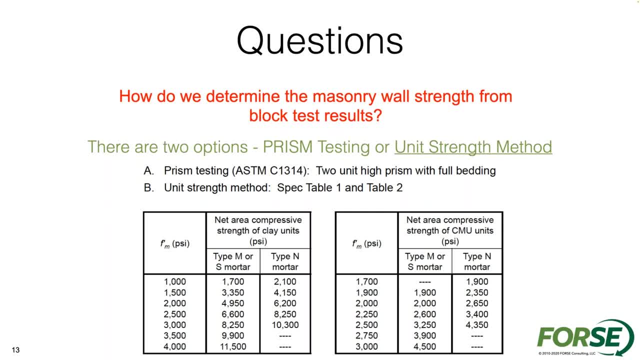 it's gonna be a little bit easier to do months and a year before a project is. oh, you can use the unit strength method. So one's more conservative, more reliable, one's gonna be more exact, more efficient, but require it to be done a little bit closer. 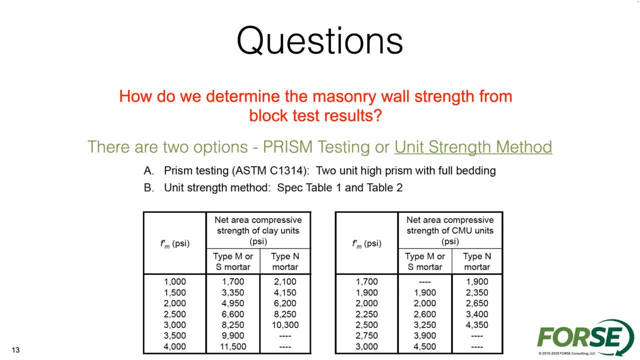 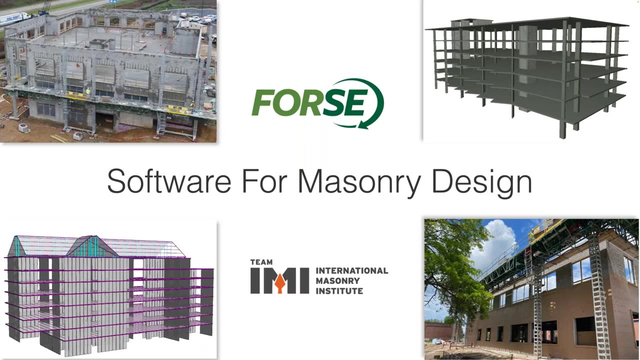 to the actual construction of the project. Hopefully that helps. Okay, Switching back to software or masonry design, And then, if there's any other questions, certainly maybe we'll stop in a hour or so and we'll kind of have 10, 15 minutes. 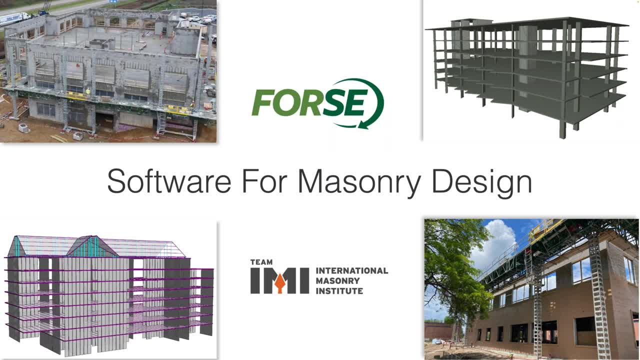 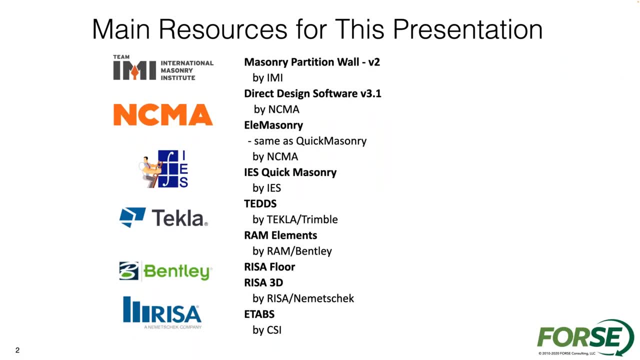 for kind of just a wrap up and any other questions that you guys might have on any one of the sections. So the resources for this presentation. I just tried to put up there the different software programs and different companies that created the different software programs. 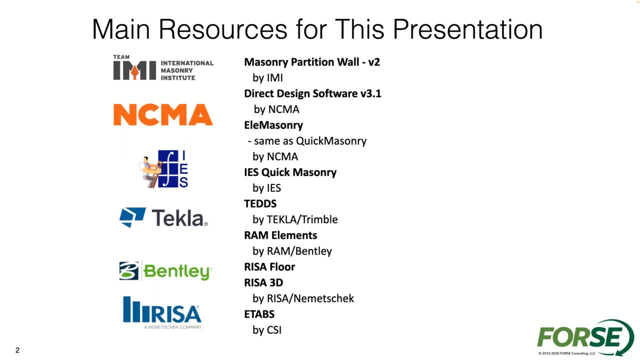 for just kind of the software review, A lot of different varieties of programs that are up there. You know full disclosure. I actually worked for a software company for five years. It's getting back almost 13 years ago, 12,, 13 years ago. 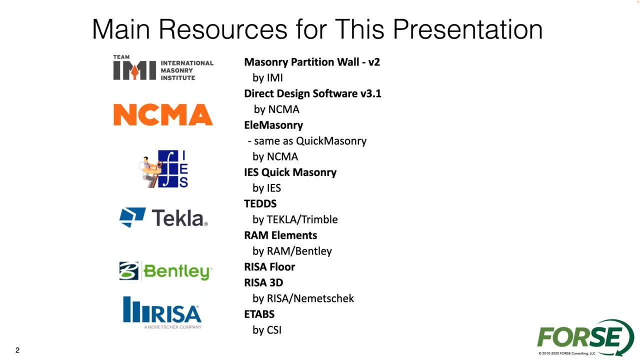 And so, working at the software company, I certainly had a perspective on utilizing software as much as you can. Since working in practice again and on my own, I understand that there's a time and a place for when to use software and when not to. 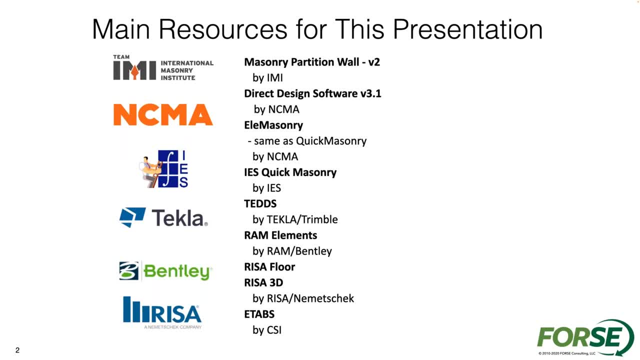 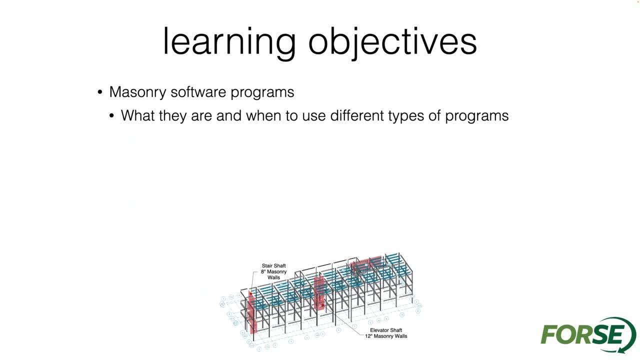 And so I'll try to make sure that I keep that in mind as I kind of go through today's presentation. So learning objectives: with many mainstream software programs you know what they are. when to use different types of programs, I break apart software into kind of two different categories. 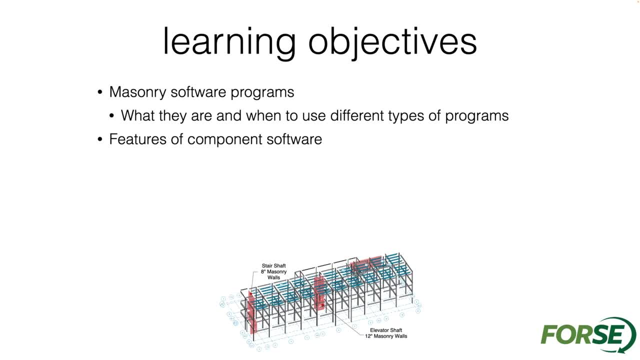 Component design software is gonna be a software programs that look at one element at a time, whether it's a wall, could be a sheer wall, could be an out of plane wall. looks at that one wall, looks at a single lintel, you know. 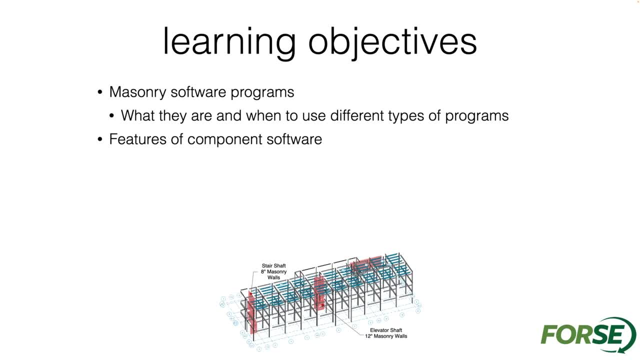 designs that look at just an individual part of the project, kind of one at a time. Hold on one second, everybody. So component design software is really gonna be meant to be a program. that's just for it's very simplistic programs, but they're very easy to use. 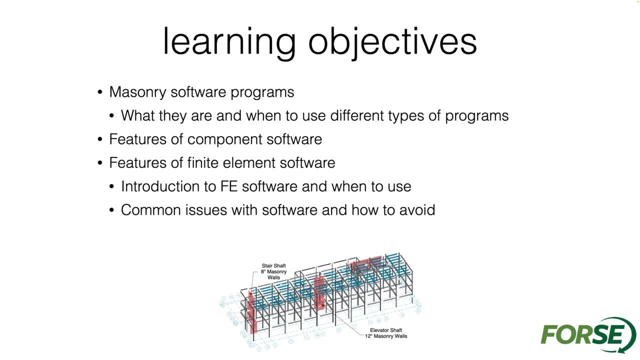 Find an element analysis program would be a separate category of programs. So we'll talk a little bit about FEA programs- when to use, when not to use- and then maybe some common issues with software and how to avoid them, and then just kind of a summary of features at the end. 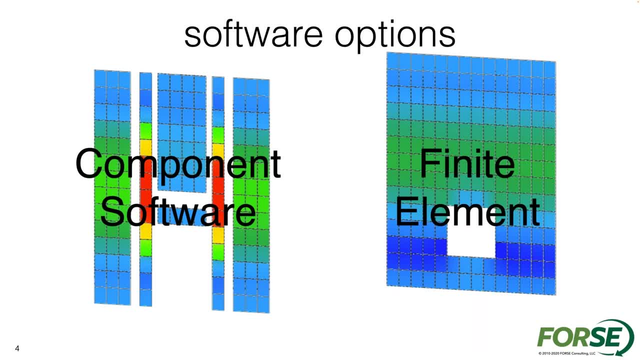 So really, if I was to look at two different categories of programs again, I would say: component design softwares really look at individual elements, Find an element. softwares look at entire walls and all of the elements kind of interconnected with one another. 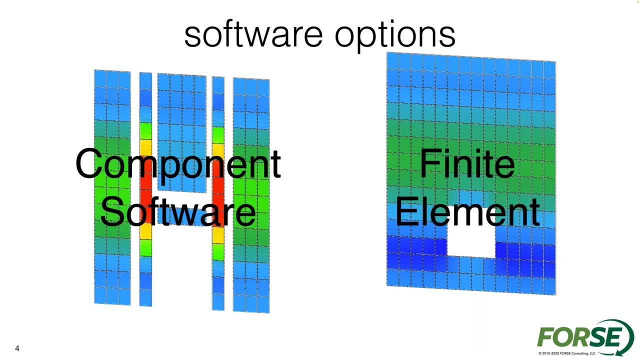 Component design software is gonna be more conservative. Find an element analysis software, I think more more exact, but it takes more time. certainly gonna be a little bit harder to use than a component design software. So component design software: common wall. 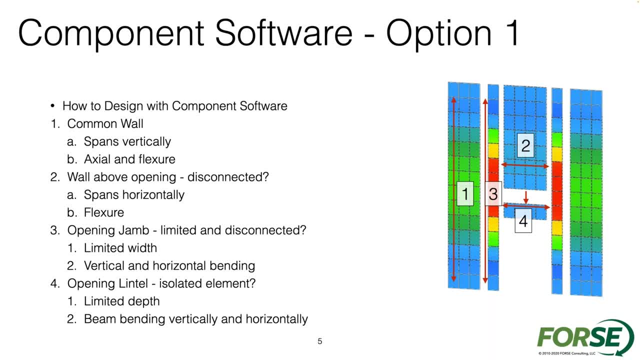 it's gonna look at the design spans of vertically kind of an axial inflecture design Walls above the opening disconnected span. horizontally inflecture opening- the jam's gonna be limited and disconnected Leads to usually a component design software's jam designs. 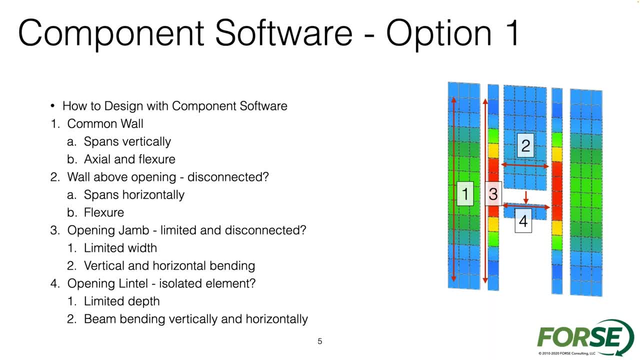 get very, very conservative. a lot of low demand on those And the lintel is also an isolated lintel, usually simply supported, as we talked about this morning, not necessarily realistic but very conservative for the overall design. The other way to use component design software: 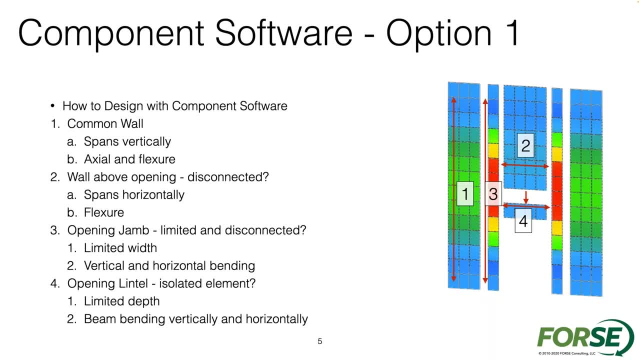 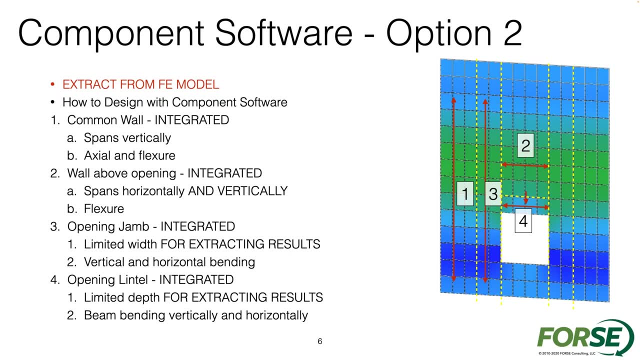 so option one would be kind of doing it kind of as it was kind of drawn up to be used. The second would be extracting results from component design software or from a find an element analysis program and just use the because component design software's work. 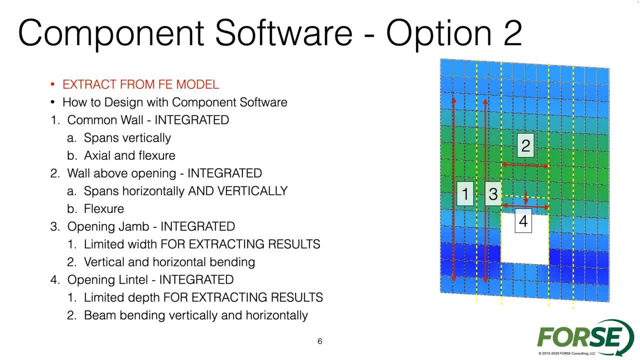 really really good for code checking. You know they're very poor at analysis, but they're very good with doing code checks on elements. So if we can pull out information from an innovative find an element analysis model, it doesn't matter if it has, you know. 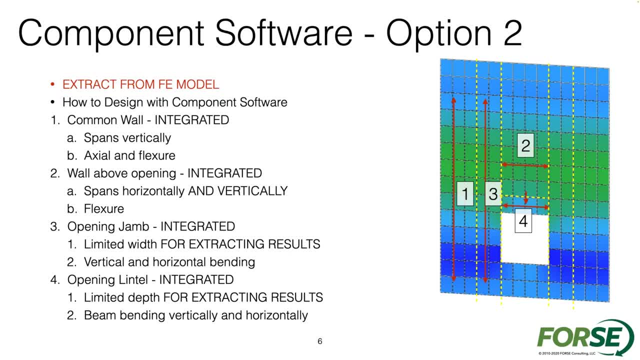 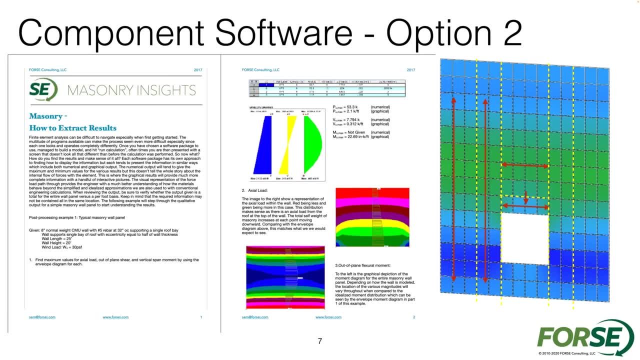 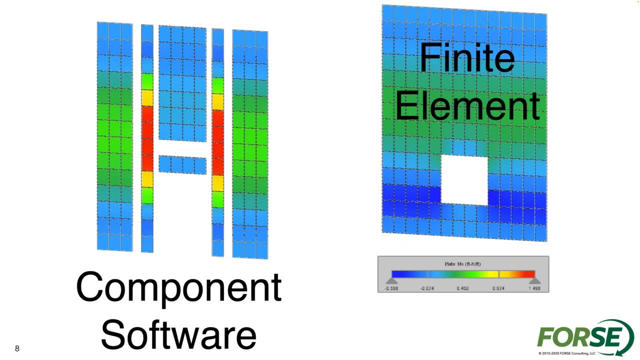 masonry design capabilities within the program. we can utilize component design software to do some of the design checks. So here we wrote a quick paper on how to extract results from some common programs, on how to make use of some of those to be able to do the overall design. 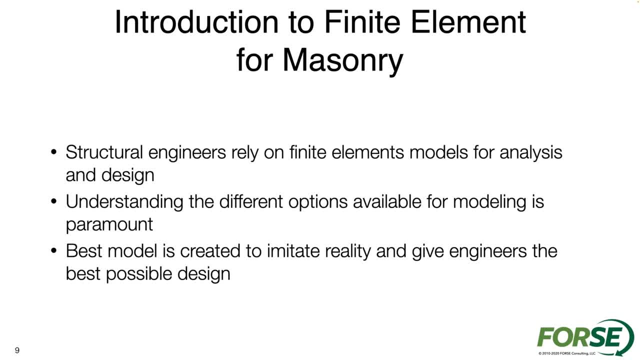 So find an element analysis. I think more and more people are using more find an element analysis for everyday analysis and designs And I think that certainly we want to start utilizing it for the same reasons for masonry design. Hopefully it's going to be more exact. 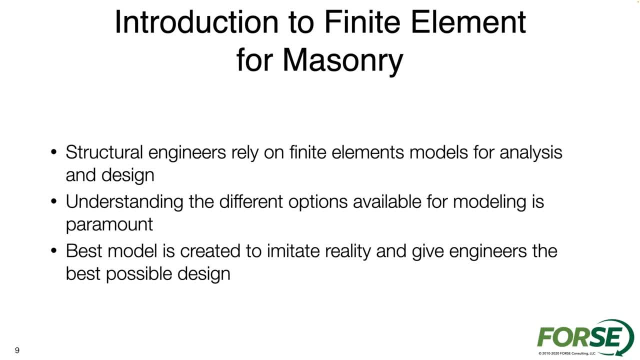 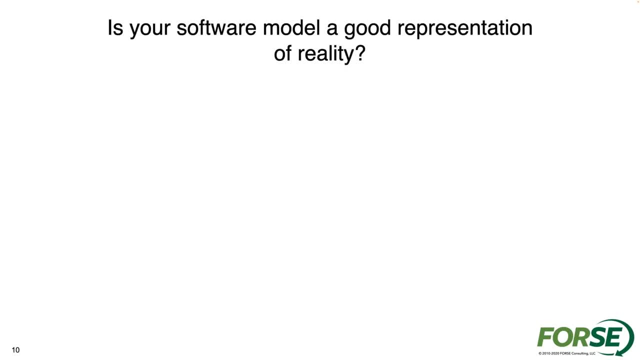 Hopefully it's going to be something that's going to be a closer representation of the real structure to give engineers like the best possible design tool to have a economical, good design. But I would say it's a good representation of reality. So just kind of stepping back a little bit. 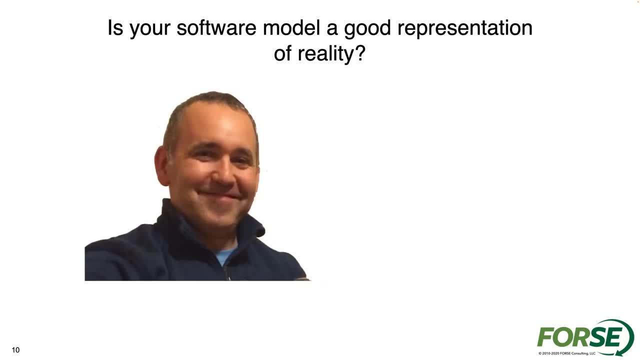 what do I mean by this? I mean so, if this is me right, this is a picture of me. what I want to make sure that I do is I don't create a find an element analysis model that looks like this, just kind of a sketch. 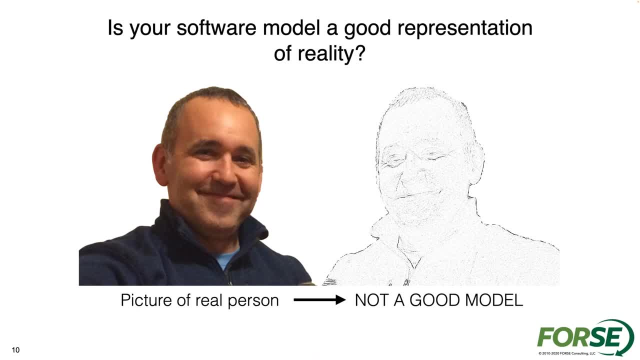 just the poor representation of the structure. A lot of times that's what we end up with like a component design model is. you just have a very poor representation of the real structure. You want to get something closer. You're not going to be. 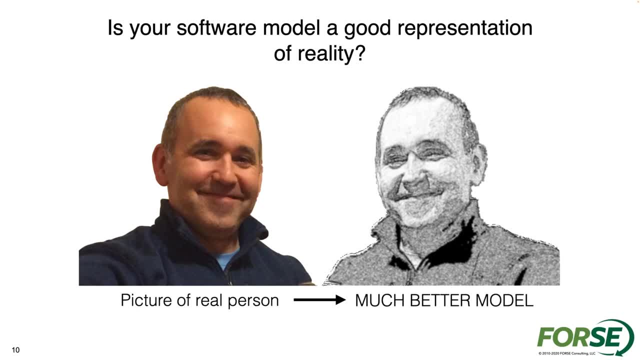 it's not going to be reality, It's not going to be the real model, but we want to do something that's closer And I think find an element. analysis kind of helps us bridge that gap. It helps bring us closer, to say, the real. 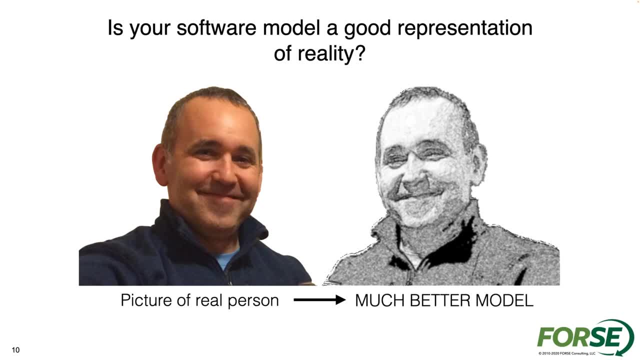 the structure similar to how this sketch is going to be a lot better representation of me than just that line sketch from before. So hopefully that helps kind of paint a picture of what we're trying to do with FEA. So look a little bit at some of the FEA stuff. 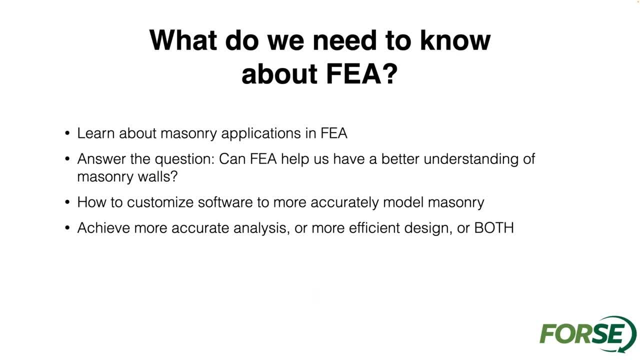 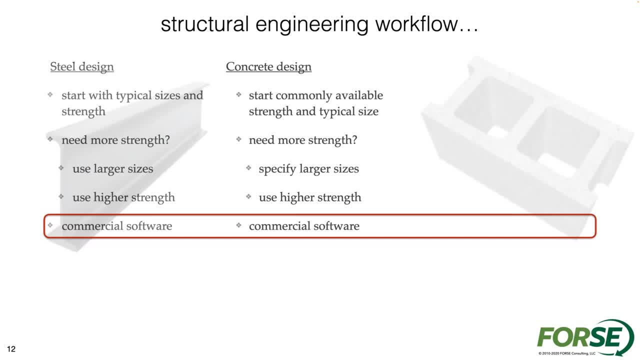 and how it can help us be a little bit better designers, be more accurate, more efficient. So I had this workflow up there before about all the other different stuff, And so if I add in software, it's the same thing, You know, with masonry. 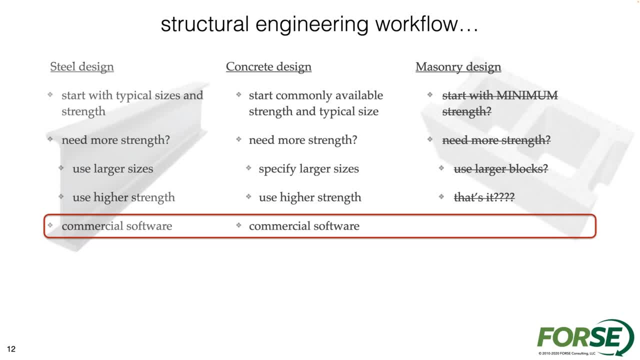 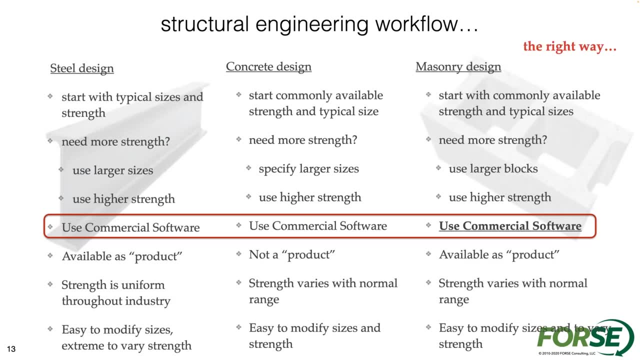 you want to make sure that we don't stop short and use the wrong materials and just use bigger blocks and minimum materials. but we actually use software, We actually utilize it and we start doing similar things with masonry as we do with some of the other material. 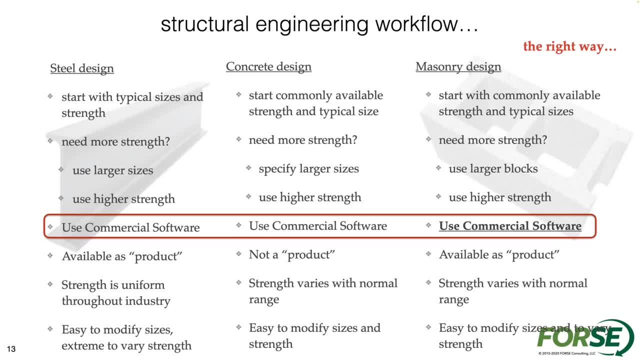 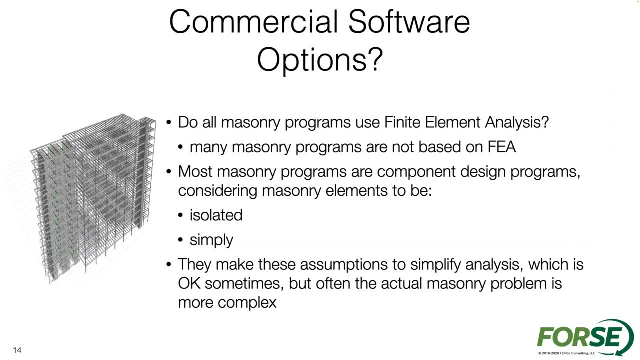 material: steel or concrete. So do all masonry programs use FEA? Certainly not. There's a lot of, like I said, component design programs where the analysis is going to be an isolated, simple analysis and you know so finite element analysis is going to allow us. 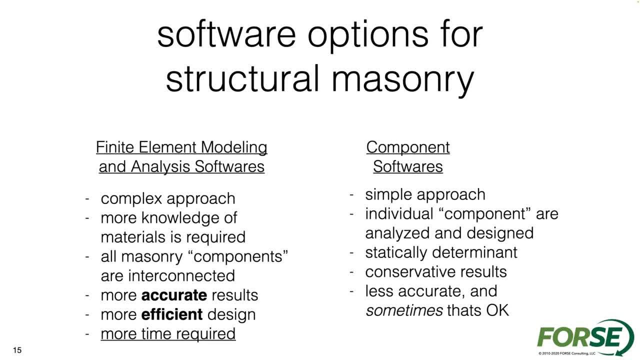 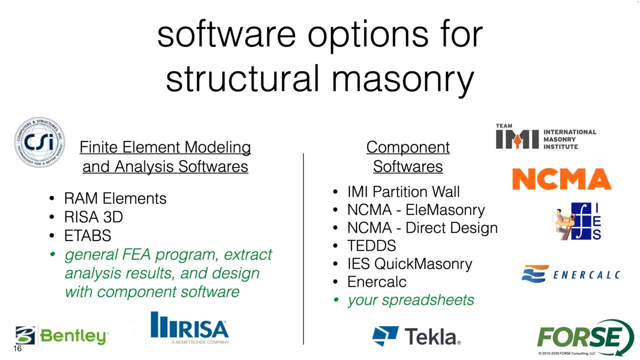 to let things get a lot more complex, interconnected, I think, more accurate results, more efficient designs. but definitely more time goes into building these models And so definitely there's a plus and minus in terms of the overall analysis and design. So finite element analysis softwares, you know. 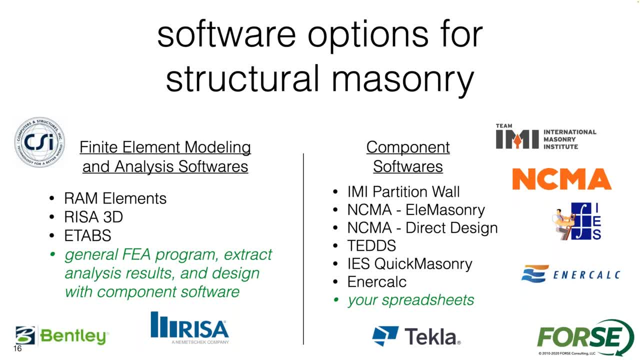 if I look at the softwares that are going to be in this presentation, there's really two different categories Again, the finite element softwares, which is going to be the RAM, RESA and ETABS or any general FEA program that you can extract results from. 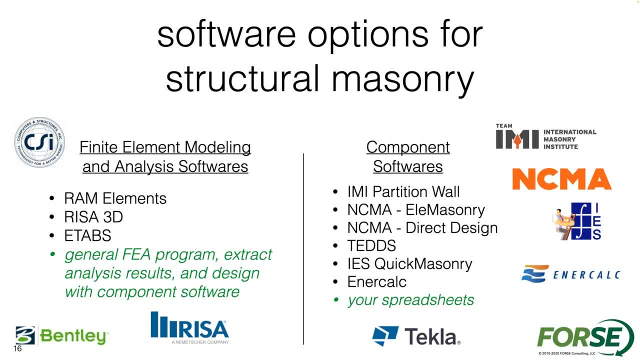 And then component design softwares are going to be IMI's program, NCMA's, two element masonry of direct design. There's TED's, there's a quick masonry, EnerCalc, or again, your spreadsheets would all be. 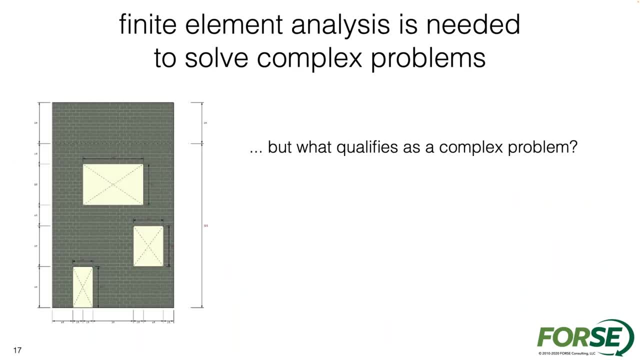 component design, simple, straightforward programs. Well, it's going to be a complex problem. I think the elevation that we have on screen, that could be a common elevation for, say, a warehouse or something like that, with a couple of doors or a couple of windows and a door, you know. 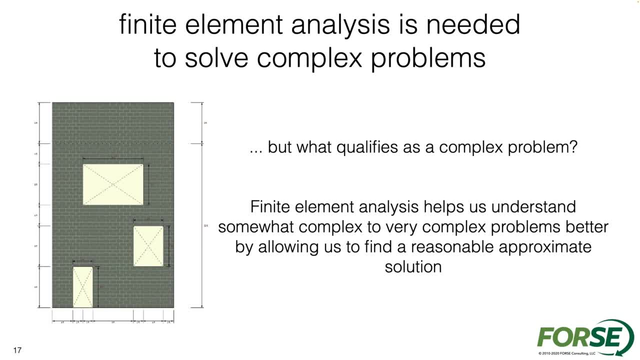 all of that gets pretty complicated. Sure, we can break that down into a simple model that we could design with component design software, but that would be very incomplete. you know, really that's going to be something that you know. utilizing software for masonry is going to be the same. 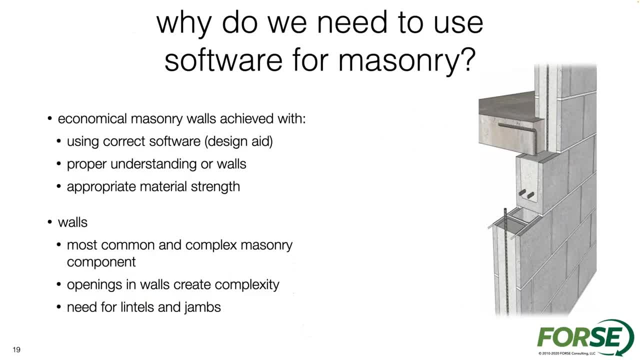 as the other materials. We're going to have a lot better economical design. We're going to have better understanding of the overall structure. It doesn't mean that we have to use a finite element analysis. This is the practical side of me. I don't have to use finite element analysis for everything. 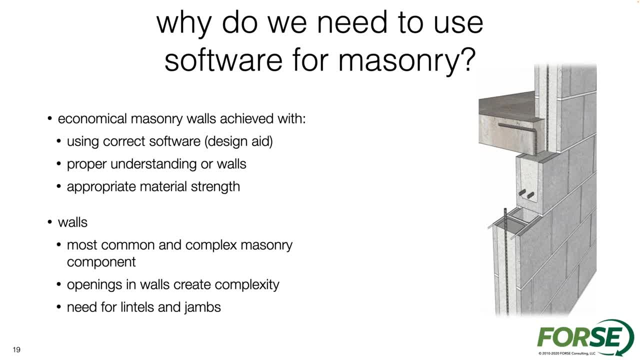 You know, kind of like I did for the lintels this morning. I looked at the lintels with a finite element analysis tool. I don't look at every lintel like that, but now I know that lintels, masonry lintels. 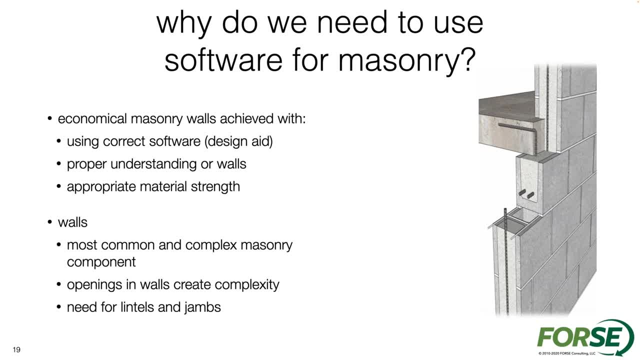 that are integral with the wall are fixed end elements with just a triangular load, like arching action would allow. I mean, that's a fundamental thing that I learned by using the FEA And now I can just use a simple analysis to determine what the forces are for my lintels. 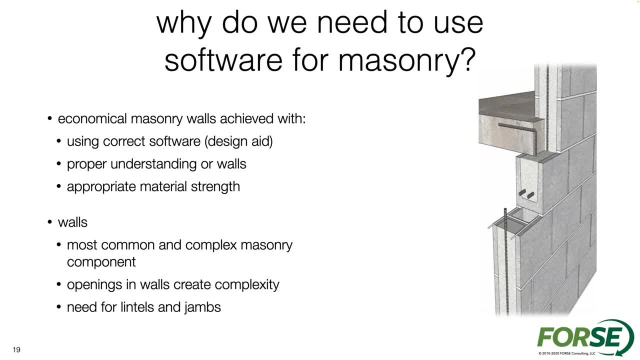 I don't have to build an FEA of every lintel that would ever be created. I could use my simple, you know analysis with some of those understandings that I had for my FEA. So but the other things that you can certainly do, 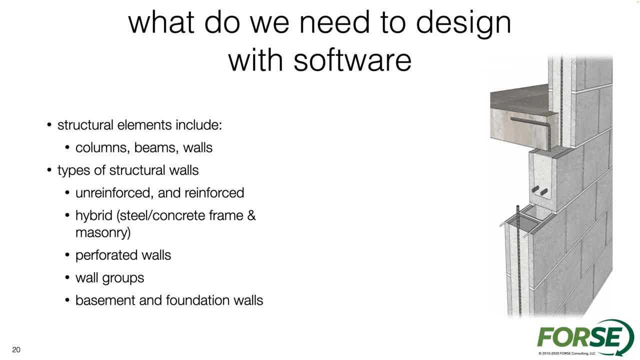 with the software is you can look at hybrid structures where you have steel and concrete frames and masonry, how that shares those load perforated walls, wall groups- you know continuous basement- and foundation walls with the main walls. you know all of those things. 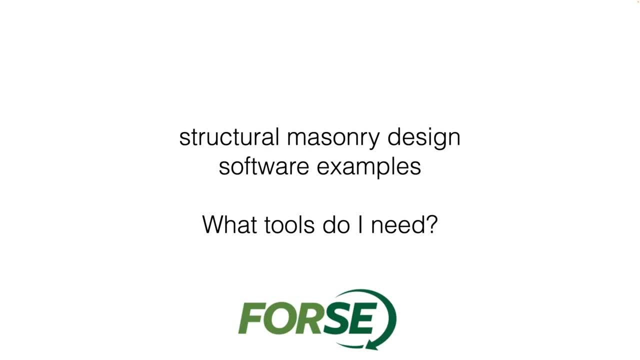 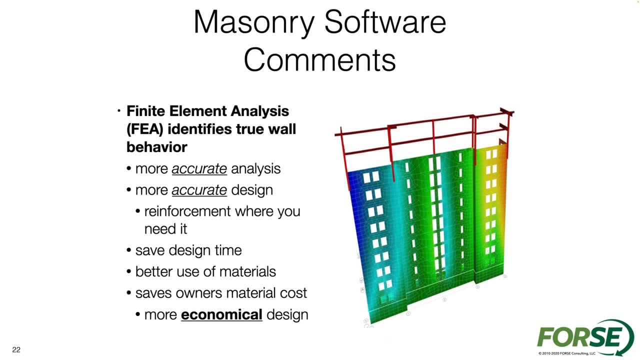 that you can do with software that really does make a big difference. So you know, if I looked at the finite element analysis and the different types of models, certainly a multi-story building like this, an FEA, would certainly help me have a good understanding. 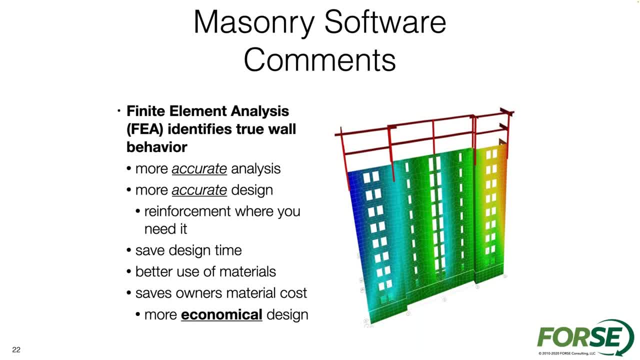 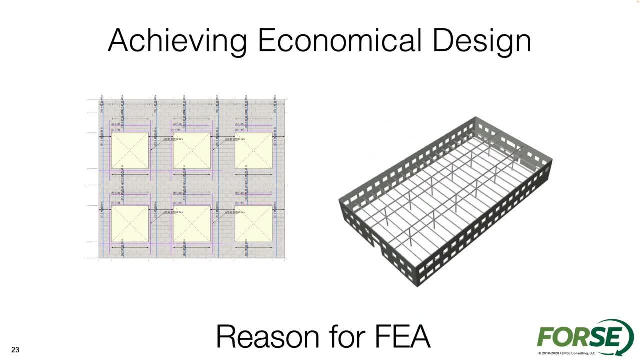 And for some of the forces that flow through that structure, you know, through multiple different elevations, you know. but even something like this, where I have a pretty straightforward, say rectangular box kind of an engineer's design- we still have FEA- would really help with, you know. 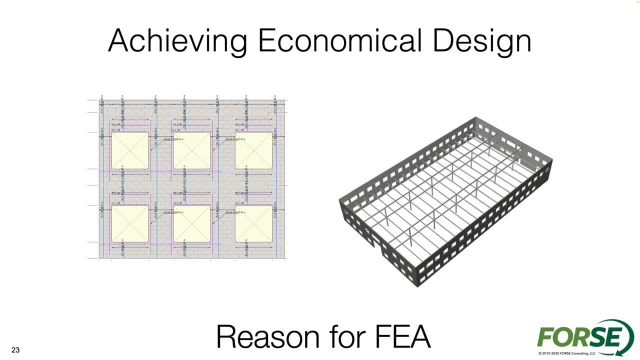 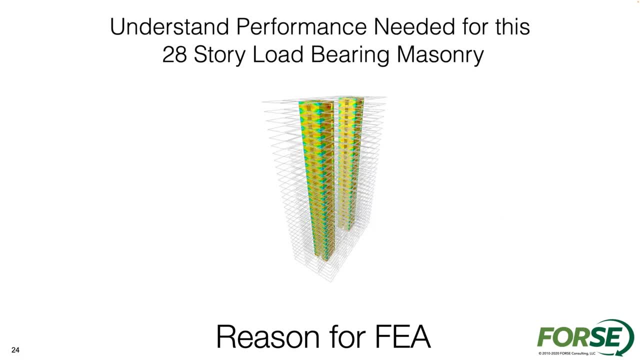 keeping those shear walls long and making that design pretty efficient. So in economical design you still have some good places for an FEA to be used. We have 28-story load-bearing masonry with cantilevered post-tension concrete plates. 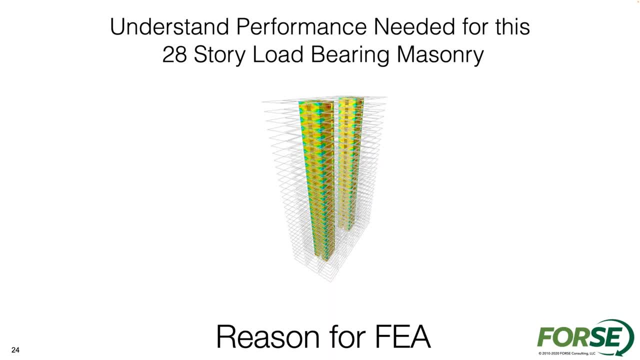 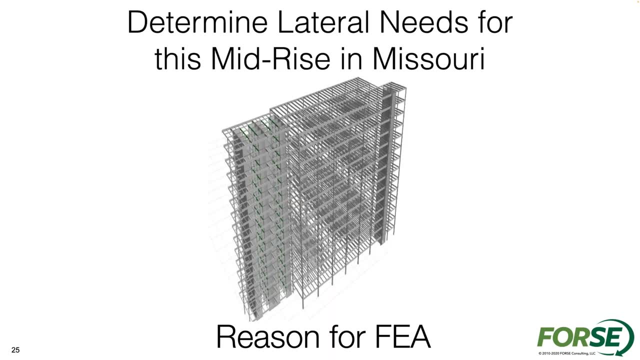 that certainly. we're going to use the finite element analysis for the rest of the building. We might as well include it for the masonry. You know FEA works really well on a building like this. This is going to be kind of a mid-rise building in Missouri. 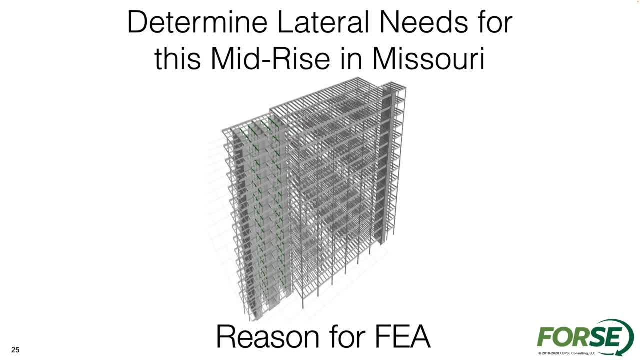 It's going to be a little bit higher seismic, taking use of the masonry shaft walls and the stair shaft that it has within the project to use that FEA to understand what the actual forces are going to be those elements. You know, this would be a building where I would say: 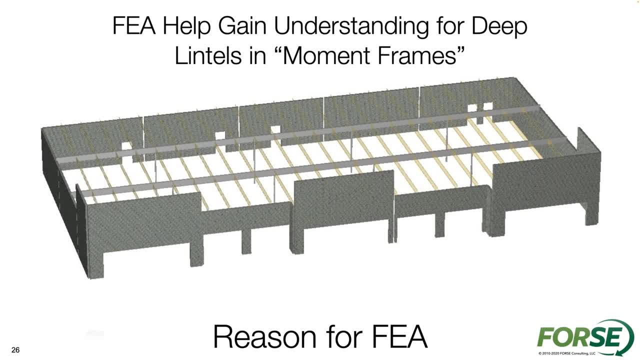 three sides of the building. you really didn't need an FEA. In fact I wouldn't use it for the whole building, but I would probably use it for the front, that front elevation where I have long span openings, how the lintels interact with those piers. 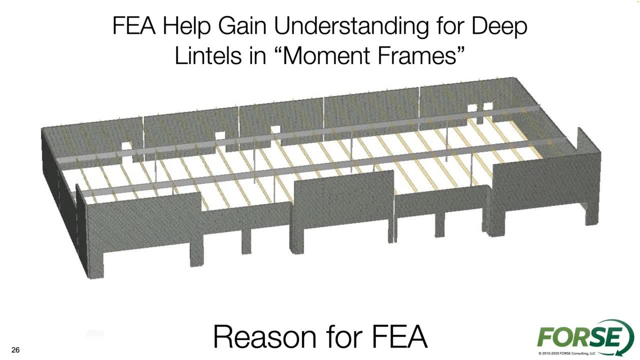 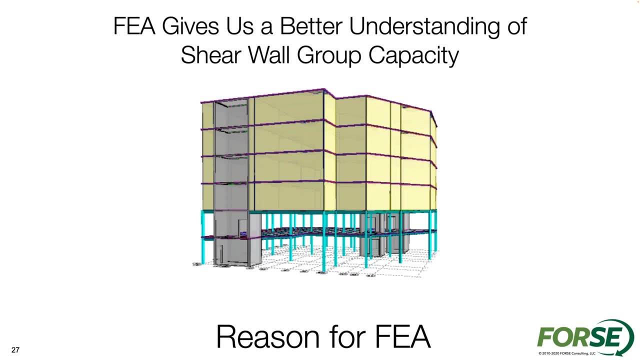 I don't know that that's really straightforward. Maybe that's arching the action to a certain extent, but how does the actual forces actually develop in that elevation? You know, I'd probably use an FEA for something like that. By the way, FEA is finite element analysis. 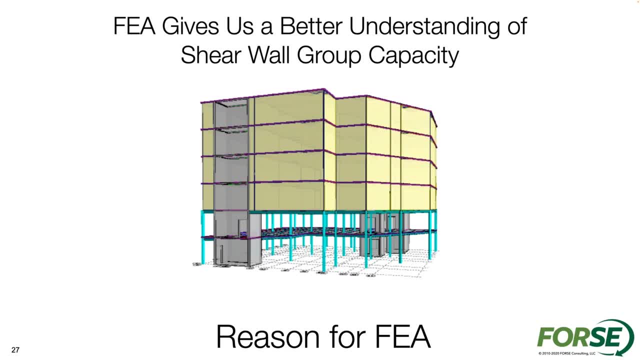 Whenever I just say I use an FEA- finite element analysis- is what I mean by that. So here are the other types of structures that you know: podium structures, where I would maybe have wood walls on top of steel floors, where I have less columns. 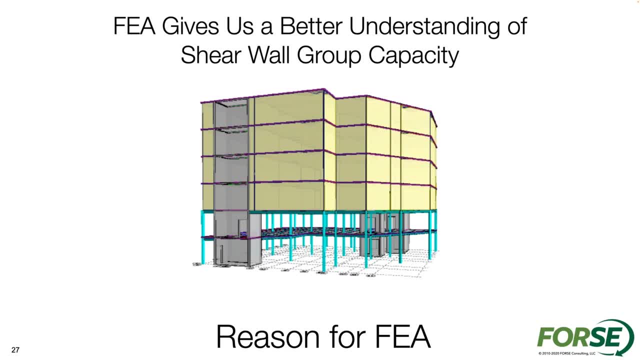 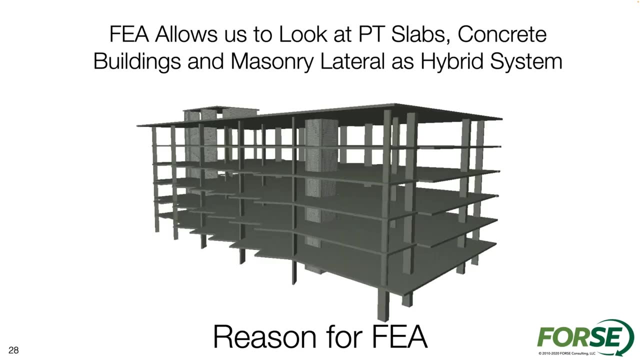 I have masonry walls that would say be continuous between the two different material types and building uses. That's another really good reason for finite element analysis, Having all those different elements coming together. it would be certainly helpful to have that design-wise Here. this is an example of what I talked about before. 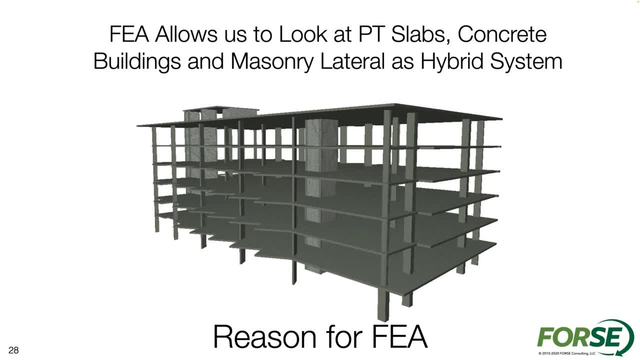 with the hybrid systems, PT slabs and masonry walls- A finite element analysis is going to give us a really good tool to be able to develop that design. You know, looking at school projects again, we have a lot of different things going on with schools. 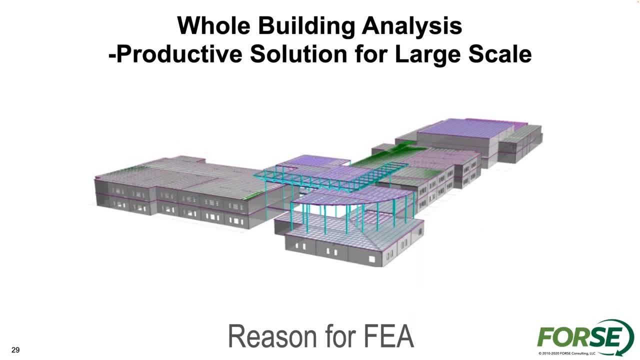 and a lot of windows and openings and a lot of forces. you know, putting all of that together, you know all of that in an FEA helps us design, certainly all of the steel elements, but then how that load transfers into, you know, some load-bearing masonry walls. 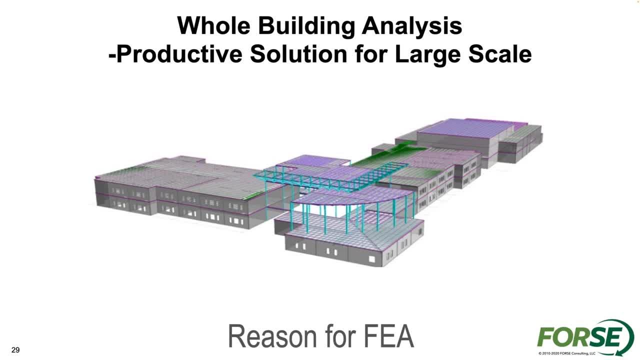 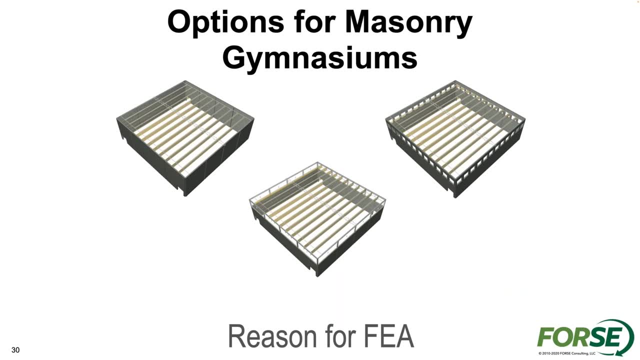 and elements like that can certainly help as well. You know options for gymnasiums. We looked at this project that we were kind of doing a study for a designer in terms of: do we have solid masonry walls for the gym? Do I have ribbon windows at the top? you know, 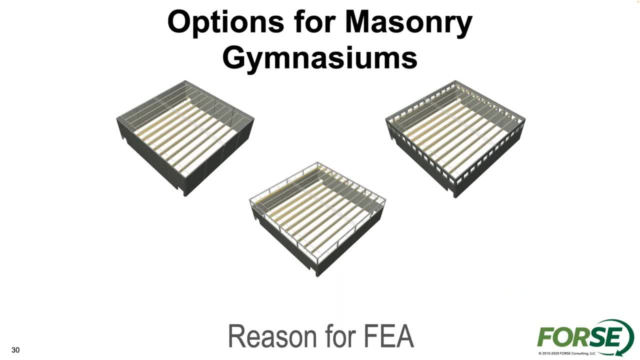 where it's just steel protruding above, where it's kind of a hybrid design, or do I have a series of openings? I mean finite element analysis really helped us determine the design that they wanted to use for that structure. You know hybrid designs with the steel masonry frame. 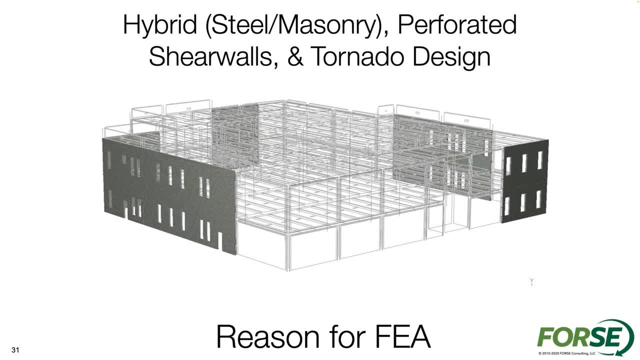 this is a building that I used a little bit earlier. in terms of shear walls, Finite element analysis obviously allowed us to look at perforated shear walls. you know the lintels and the shear wall capabilities in that design is certainly something that we needed a little bit heavier. 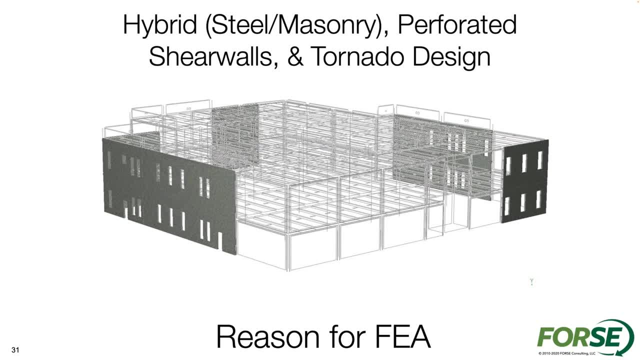 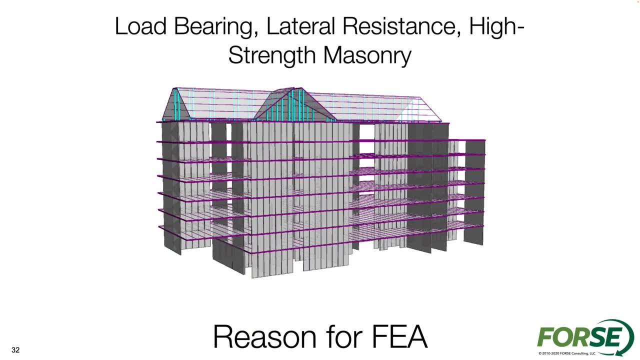 better tool to be able to do some of that design. You know this building in terms of multi-story condominium. this is a project on the east coast where we had a finite element analysis that really allowed us to evaluate many different options. You know we were looking at different strength of masonry. 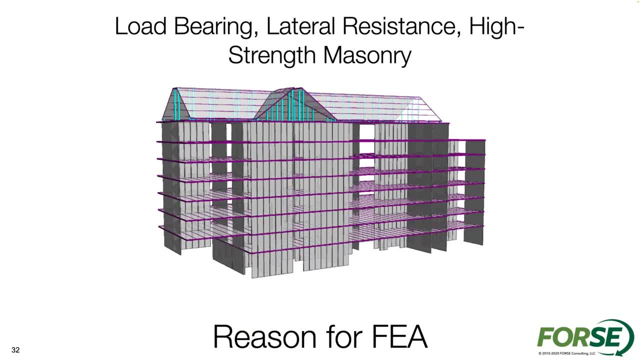 for the lower levels. We wanted to use the common say 2500 for the upper floor, but then we got the lower levels and we didn't want the reinforcement and the wall thicknesses to change. So finite element analysis really helped us evaluate. 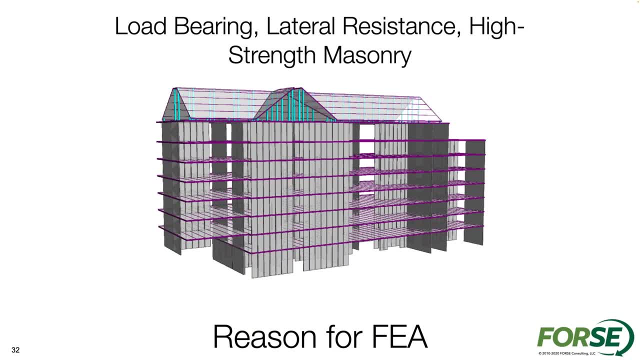 many different options there, So a lot of the reasons that I'm giving you would be really similar reasons for using finite element analysis for concrete or masonry. You can do all of these different scenarios and a lot of the reasons would be true for masonry. 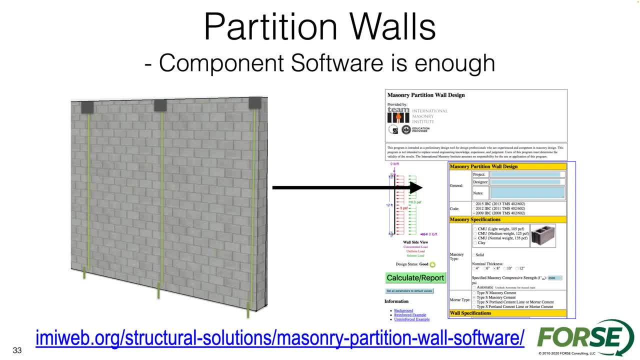 But it doesn't mean that I always use finite element analysis software. Certainly I would never use the finite element analysis software for a partition wall. It's just way more programmed than actually is needed. It's a pretty simple analysis. That's the fundamental component design software. 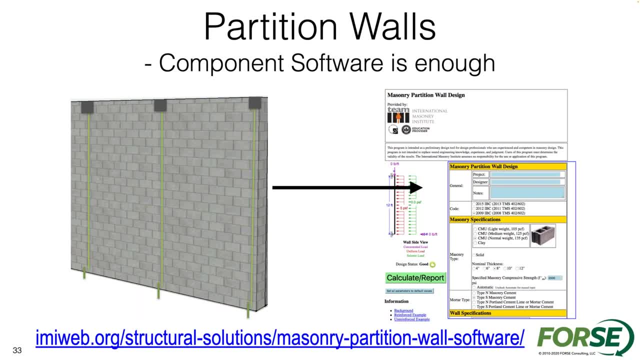 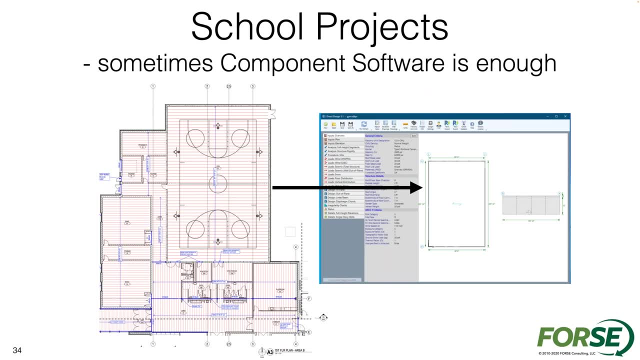 this IMI tool that's online. That's a great program. It's easy to use and certainly works very well. Sometimes a gymnasium is going to be something that we can put into a component design software, A direct design, is going to be a program from NCMA. 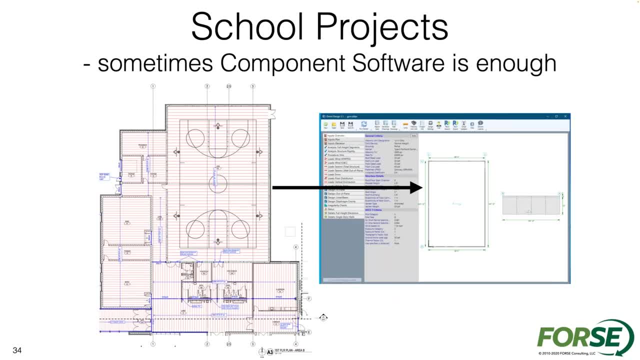 that really works pretty well in terms of laying out a part of the building and designing all of that. They're component designs, but there are many, many component designs All at once, So that can be very useful. Sometimes I have projects like this school, where I have several. 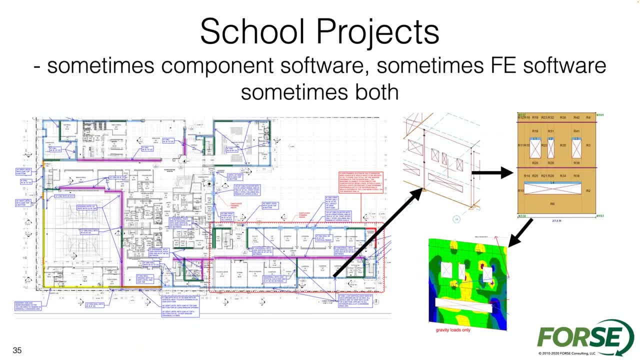 different programs going on. I have parts of the building that we can use component design software, and then I have an elevation or two where it's just complicated. I have a long span opening. I have a certain use of that space in the school building. 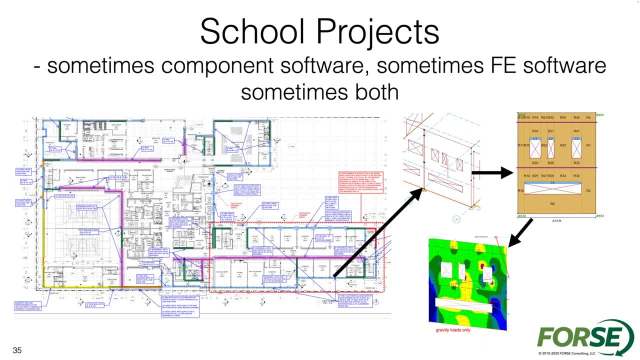 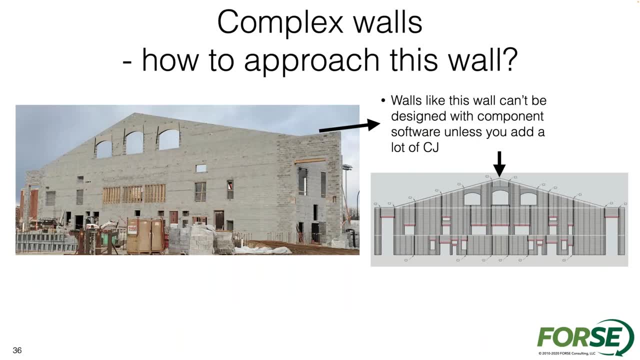 that requires a big opening, And so a finite element analysis might be necessary just for a few panels here and there. So that's something that we can use in the design. Again, school buildings, large projects- I can evaluate walls like this. 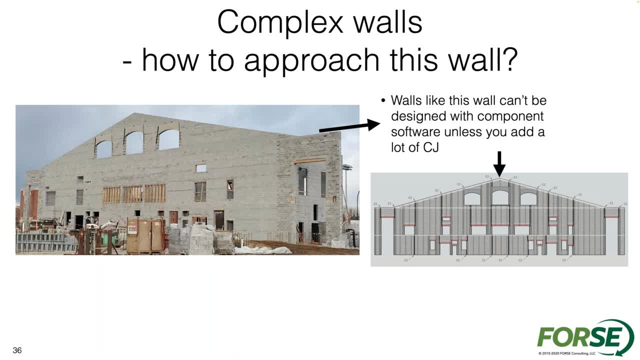 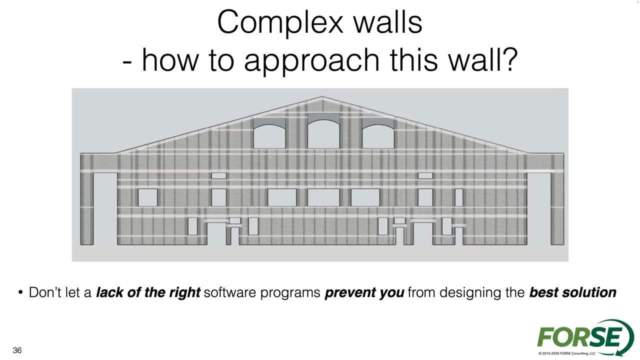 Do I need to have control joints- kind of traditional control joints of this project- or do I want to look at this entire wall elevation And using a finite element analysis software I obviously can put the whole wall in at once. I can have it all interconnected and I can see where the 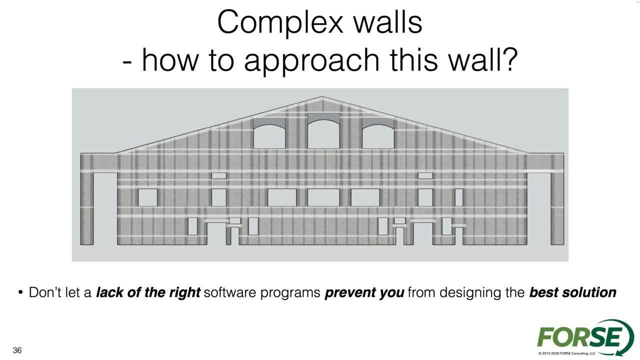 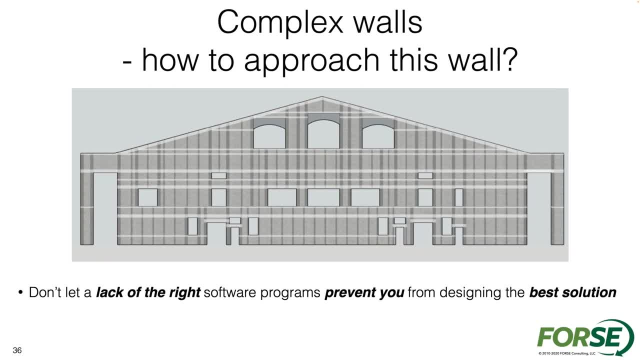 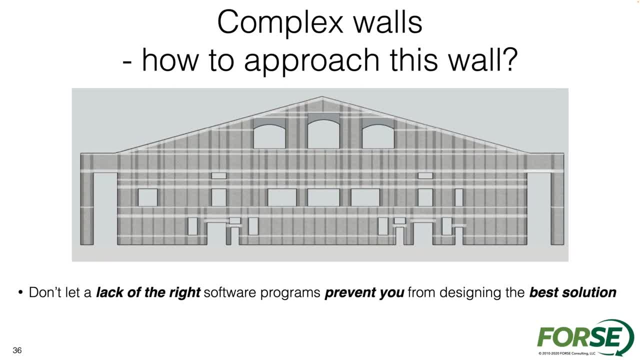 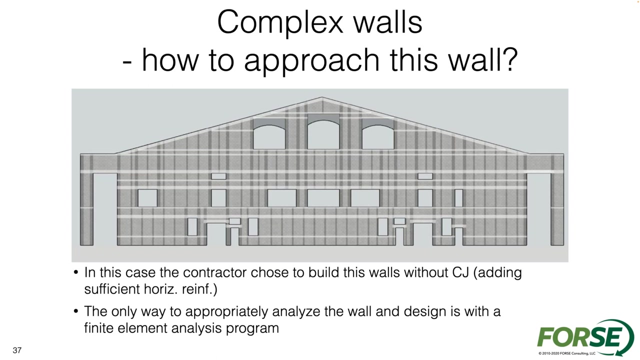 The finite element analysis really helped us with this design. utilizing the stuff that we learned before about minimum amount of reinforcement that you would need to have be continuous to eliminate control joints was another big part of making this design work And so limiting that and using a finite element analysis software. 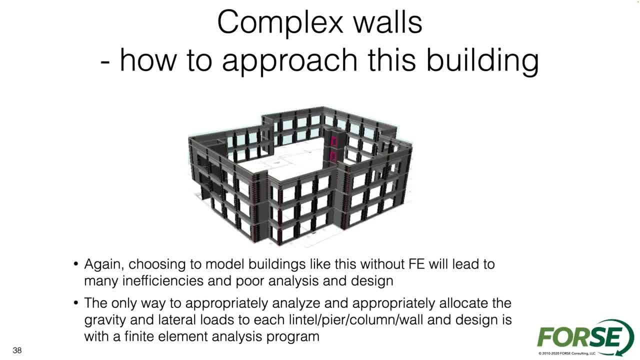 really helped with this design. Other elements: a building like this is a project that started as a, I believe, a steel frame structure and they wanted to go to a load-bearing masonry- for the aesthetics, I think, as well as some of the sound attenuation and stuff like that for the project. 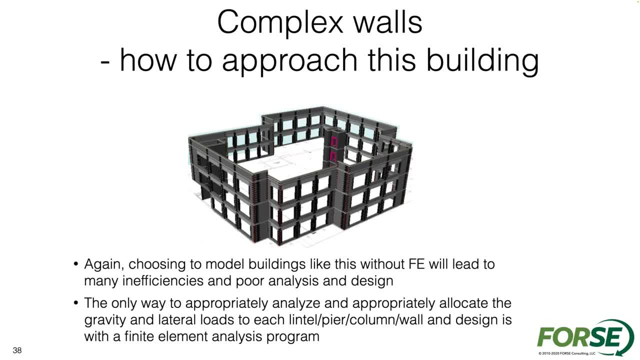 So, again, this type of building wouldn't necessarily lend itself to a component design approach. We have a lot of complexity with the exterior frames that really look more like moment frames. we have a lot of load sharing that would happen between, say, solid shaft walls and. 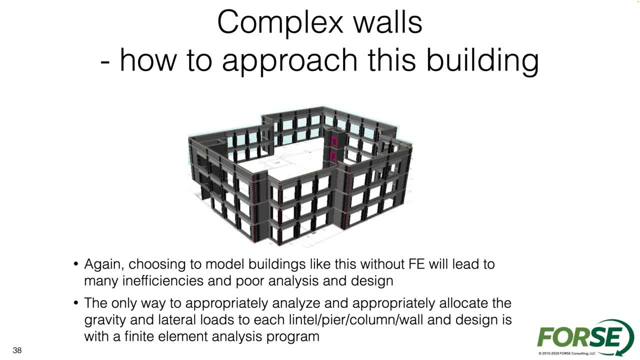 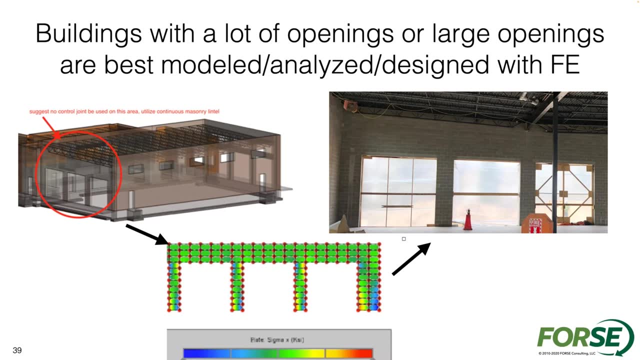 these exterior frames. So understanding how the force distribution would work in a project like that, also required to find an element analysis to get the right forces and stresses for the project- These continuous lentils that I talked about earlier in terms of how to make those work. 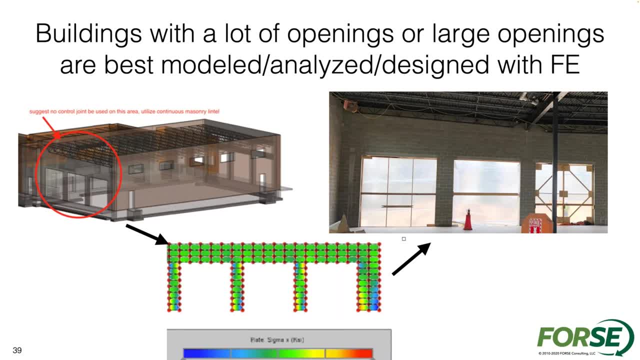 and eliminate control joints. you know, maybe that's just one elevation Of this fire station. you know, we have these apparatus bays that have, you know, pretty big openings, and the rest of the masonry project is going to be pretty standard. 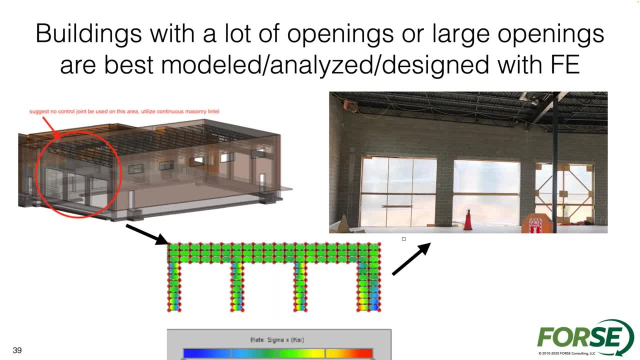 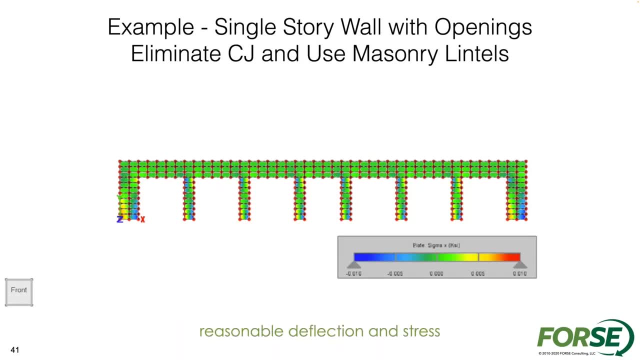 So maybe that's going to be one elevation that we look at with a finite element analysis And we can utilize that. you know whether it's three doors, five doors, seven doors, I can look at. you know what the actual stresses and forces, what the movement's going to look. 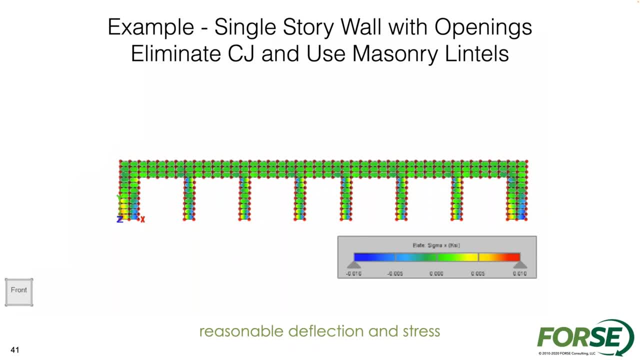 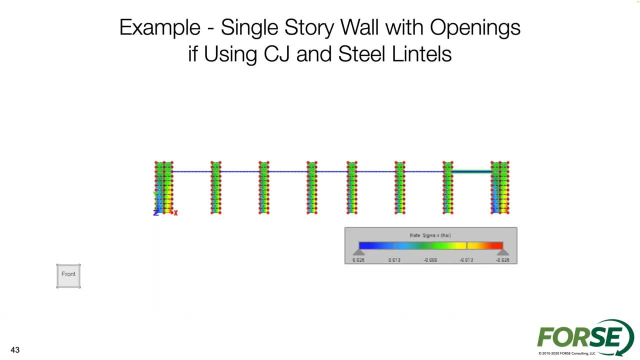 like you know, for that elevation I also can do a comparison and contrast. If I had isolated lentils, if I had something like this, you know what is going to be my deflection on that elevation. If I have in-plane loads, I'm going to have all of the load. that's going to be resolved. 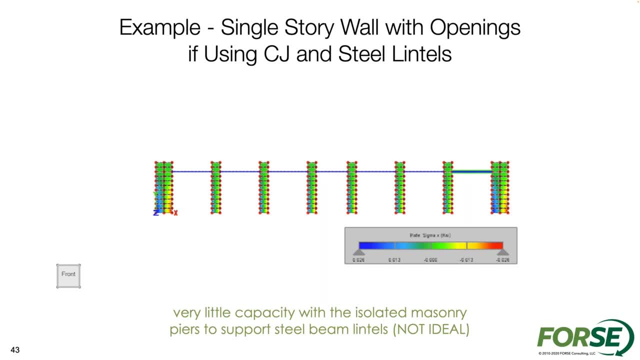 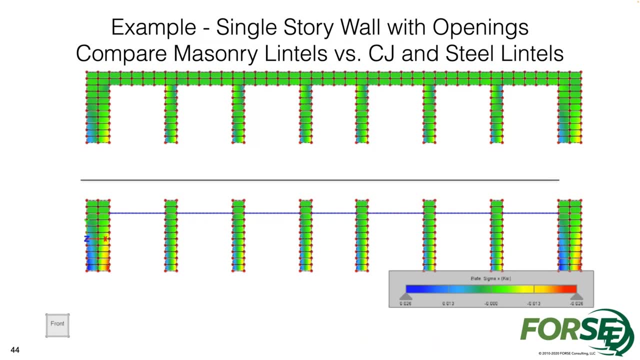 with very thin, tall piers. So I'm going to have that stresses that are going to be a lot higher. I'm going to have a lot higher load demand on those piers, and then I can also do a compare and contrast between the two of them. 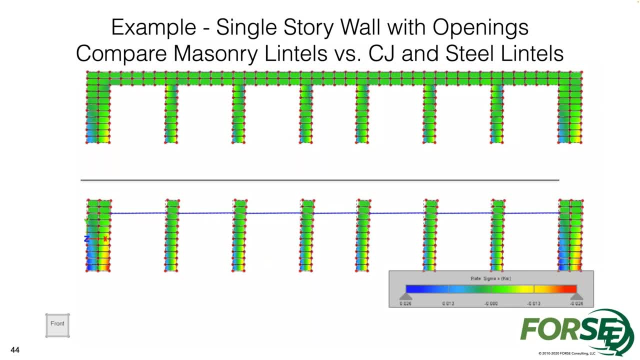 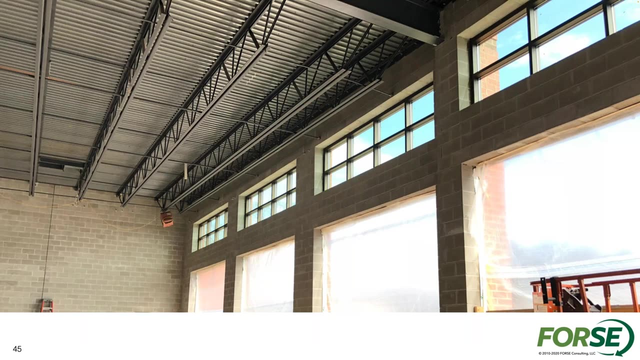 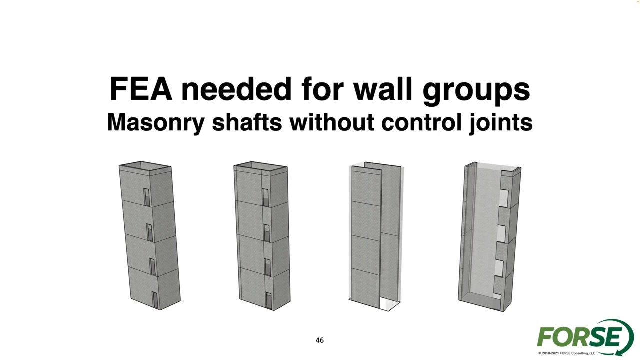 I can see which one's going to deflect a lot more And which one see again. what are the relative stresses are between the two different solutions. Other elements that I think are fairly complicated and certainly can utilize tools like finite element analysis anytime we have shaft walls. what I encourage designers to do is one. 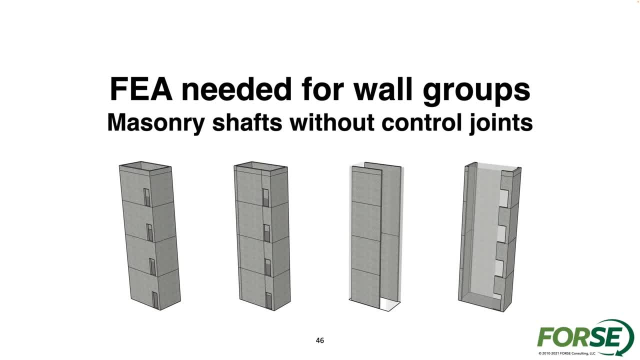 to use the shaft walls, whether that's a cost-saving perspective, whether it's a reducing your carbon footprint, or however you want to look at it. the more we use the shaft walls- for again, they're durable, they're fire-resistant. that's usually why they're in there. 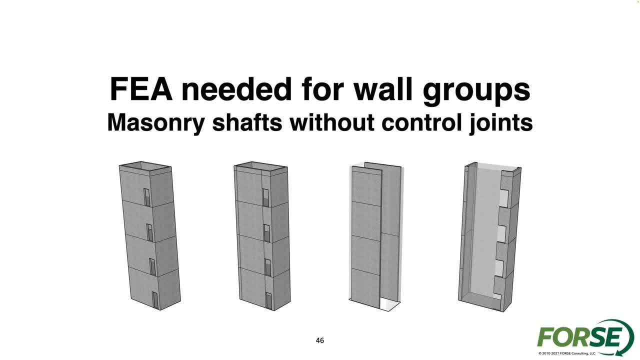 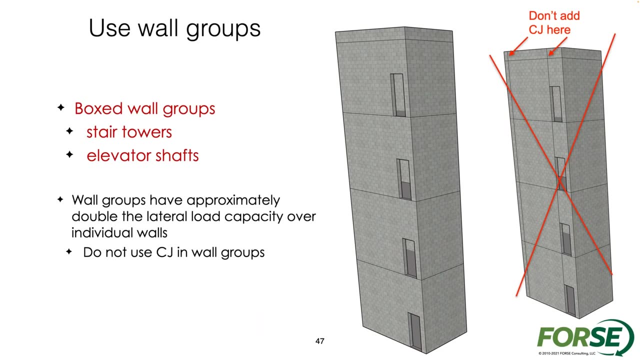 But then they're also very good at resisting load vertically- the gravity loads, the lateral loads horizontally- So it really can be used for a multiple number of purposes Once we have the shaft walls. what we want to make sure is we don't unnecessarily add. 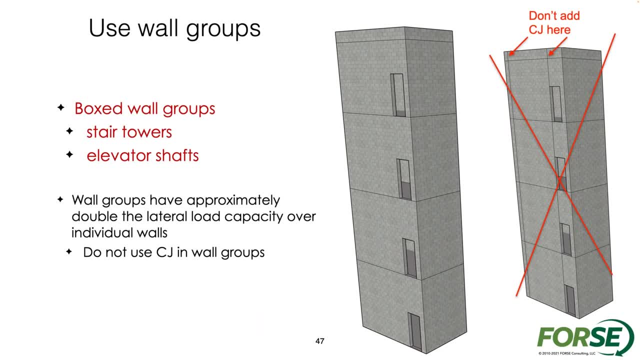 control joints. just because it's masonry doesn't mean it needs control joints. We talked about that in terms of eliminating control joints. Having a boxed wall group, though, is a little bit more complicated. Individual wall panels is easier to do by hand. 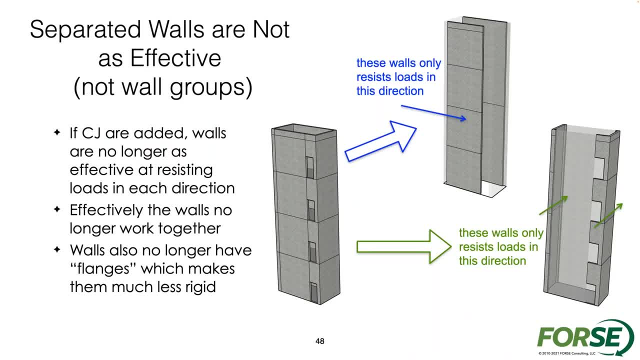 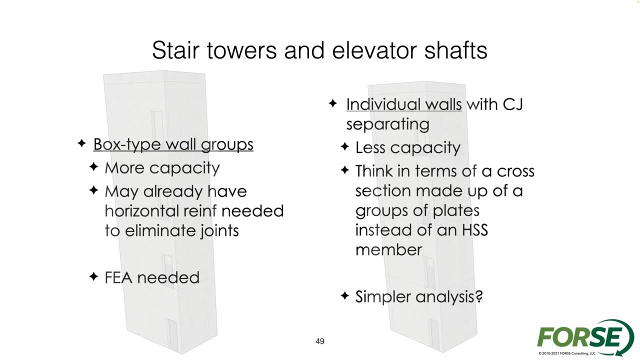 Once I have a boxed wall group, I have a lot more complexity. Like I said, I have about half the capacity You know. If I break these apart and try to design these by hand, I'm able to evaluate that and look at the actual overall demand. 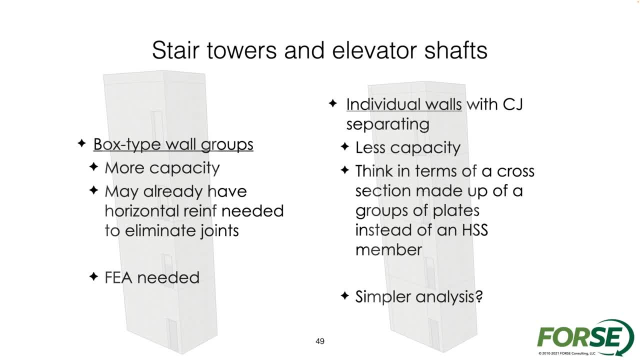 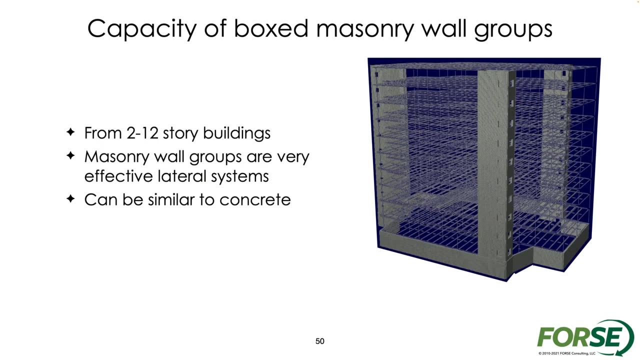 But it does require a more complicated model and a much more rigid tool to be able to design those elements as a boxed wall group. So again, anything 2 to 12 stories masonry can be pretty effective. It can be pretty comparable. 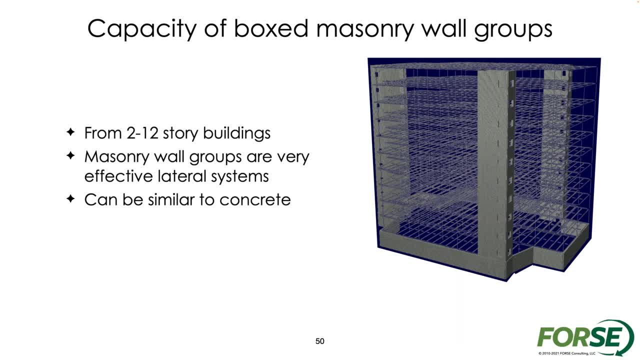 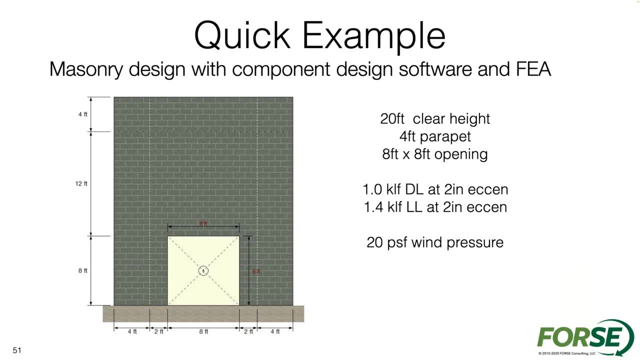 It can be comparable to concrete, As long as I have those boxed wall groups that we use all the way up the building. So just again, a really simple example in terms of how component design compares the finite element analysis. So again, before we talked about if we had component design software, we really break. 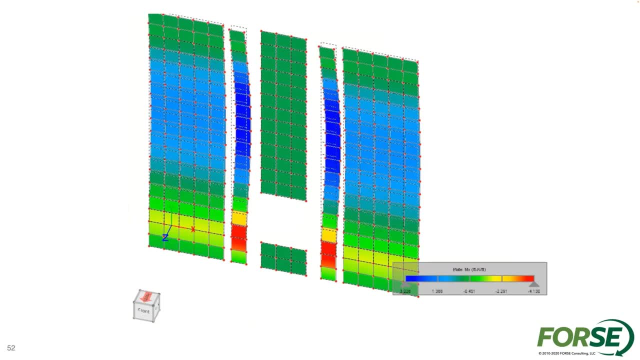 walls apart into different pieces And so what you can see when we look at the animation for the slide, As you can see, the different parts of the wall are moving differently than other parts of the wall And if we think about you know that's based on the stiffness of the elements that are. 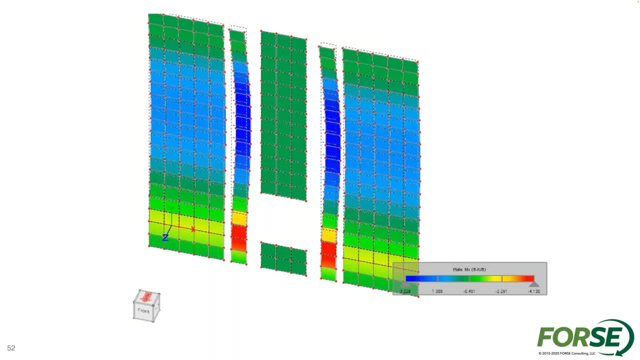 in there. the load that I traditionally would put on those different elements- And I quickly recognize, if I think about it for a second- is masonry doesn't work that way. When we build this wall, we have it all interconnected and masonry is really going to be moving together. 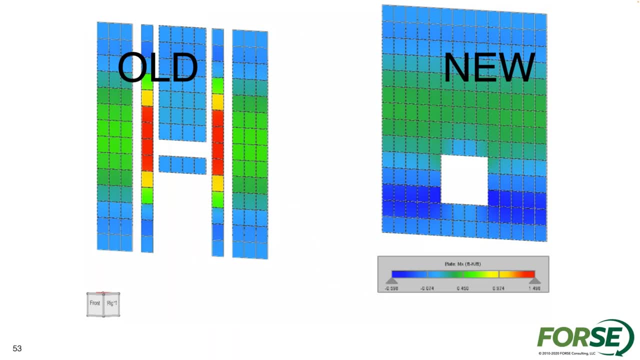 So if I do a quick comparison between the old methods and the new methods, You can kind of quickly see. you know the masonry, as long as we let it be connected, is going to share the load pretty effectively across the wall. I need to have some vertical and horizontal bending capabilities, but I do have vertical. 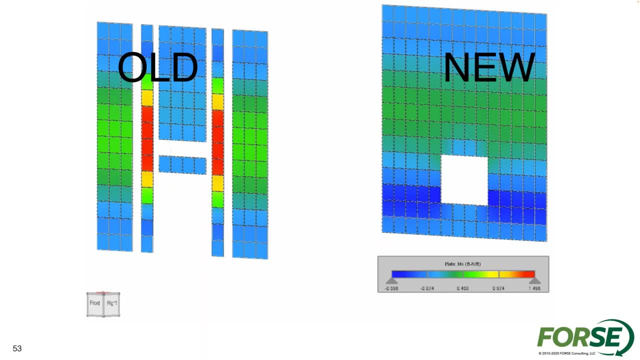 reinforcement. I do have horizontal reinforcement and joint reinforcement And I also could have some additional horizontal reinforcement with the lintels and sills and other elements. If I look at the moment distribution, I can kind of see what some of the forces are. 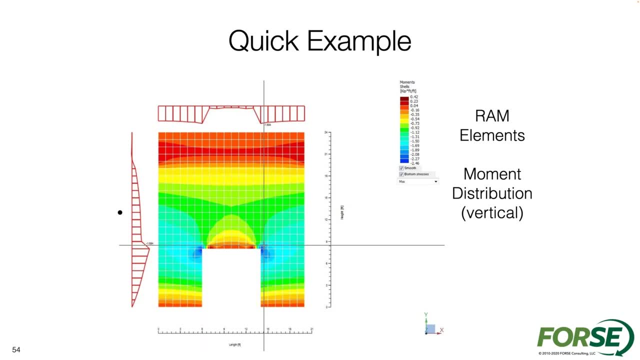 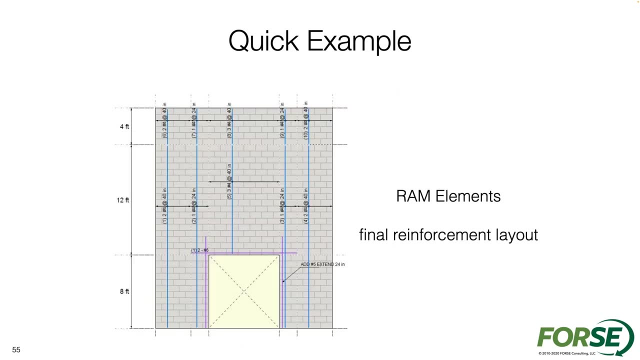 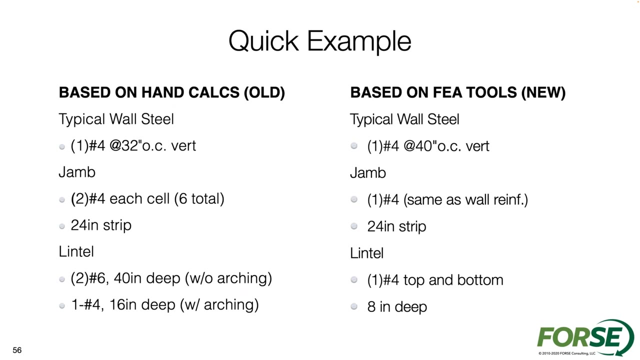 We could look at it and kind of tunnel down like we did for the lintels, before We can look and see what the exact forces are. It's going to have the reinforcement that's going to be laid out Basically, the quick example of, you know, reinforcement. I'm going to have less reinforcement. 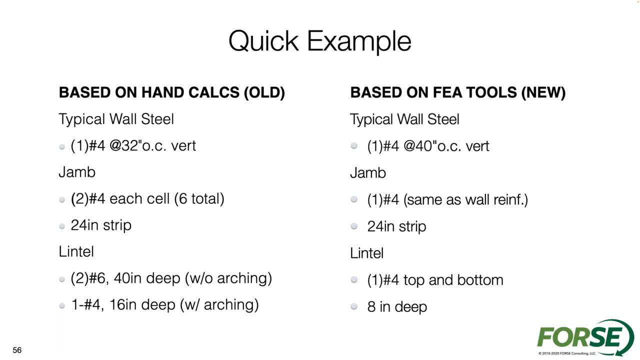 on the typical wall panel If I use a finite element analysis, just because it can take into account the continuity between the wall, the foundation and the parapet, So I have some efficiency that are going to be built in there by having some of the continuity. 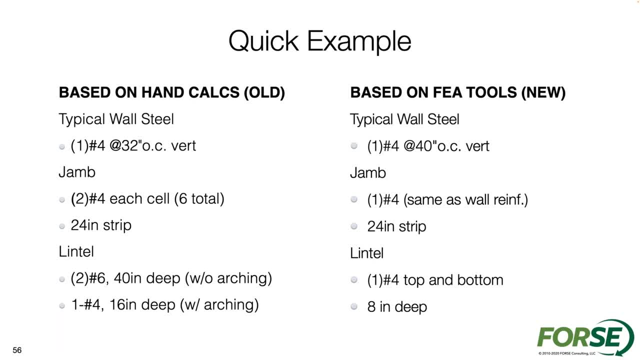 that would be considered. So that helps. I have jams that are going to be far more efficient because we're going to see the loads sharing capabilities of the wall as it's able to span horizontally. So my jams have far, far less reinforcement. 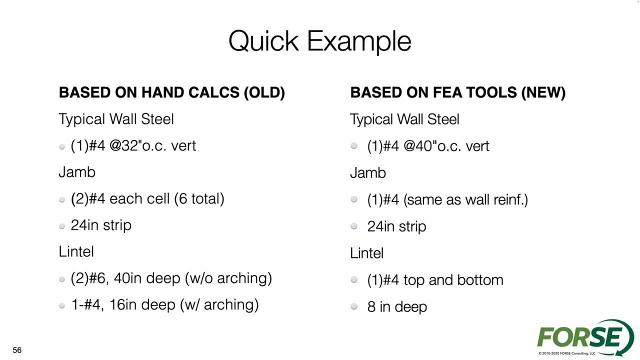 My lintels have a lot less reinforcement because I have arching action. If I do consider arching action in my simple support that I'm going to be able to get pretty close with hand counts, I'm going to be able to get pretty close to what the overall finite element analysis. 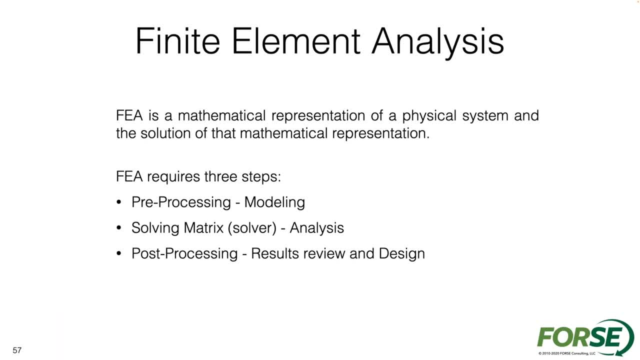 gives us. So again, I'm not just you know if. if anybody looks at this and says, boy, this is, he's just trying to sell finite element analysis. I'm not trying to do that. I'm trying to help people understand why this tool is important to use. 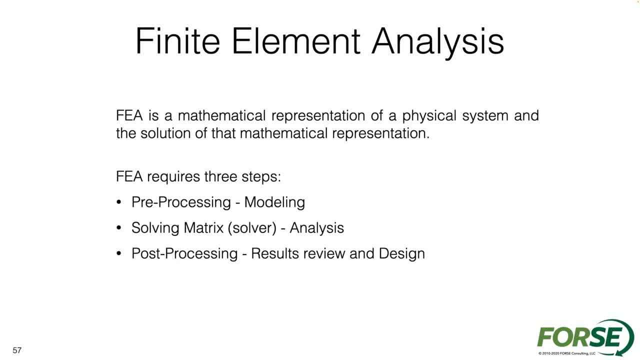 It's not the tool that you would use for everything You know- I tried to talk through that- where there's certainly plenty of designs that you wouldn't need this tool, but when you do, you need this tool It's. It can be really beneficial for the more complicated elements of design. 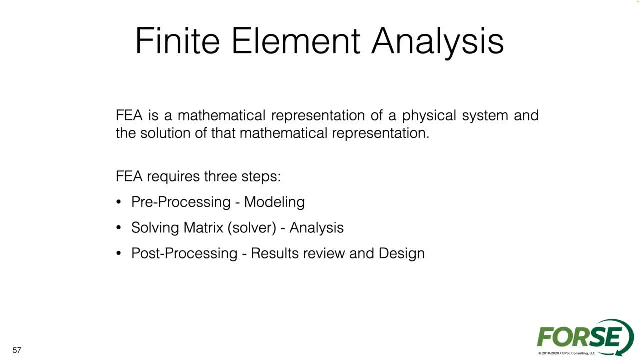 So for finite element analysis, when we teach on finite element analysis, we really try to break down the finite element analysis really into three different steps: pre-processing, which would be considered modeling, solving the matrix, the solver, the analysis. That's really the software, that's. that's the power of the FEA, is the ability for it. 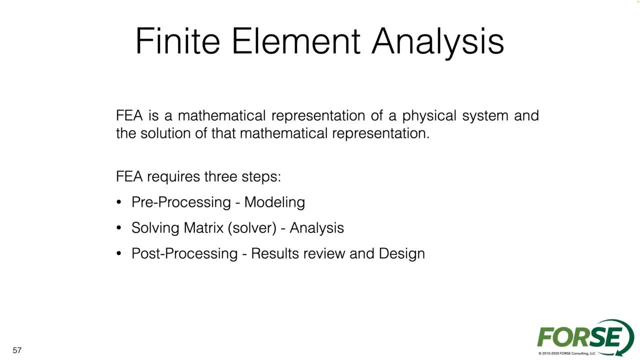 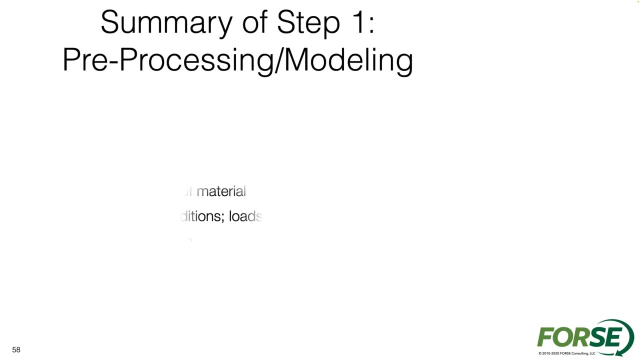 to crunch a whole bunch of numbers very quickly. So the analysis piece, kind of step two, is, is the software and then the post-processing is really going to be two different pieces where it's going to be results review and, separately, the design. So step one, building the model- 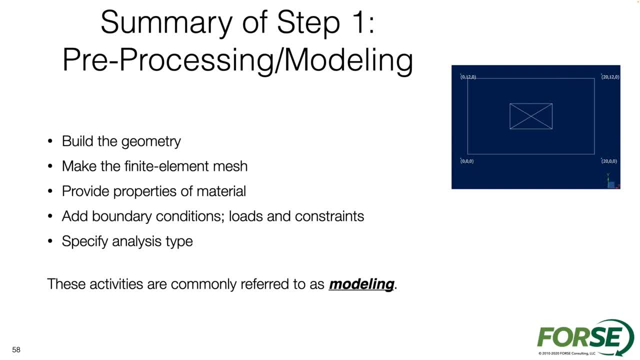 What I try to encourage people to do is: don't just build a sketch up model, Don't just build The overall geometry And the open, The opening, and stop thinking about it. but the program is going to do is it's going to. 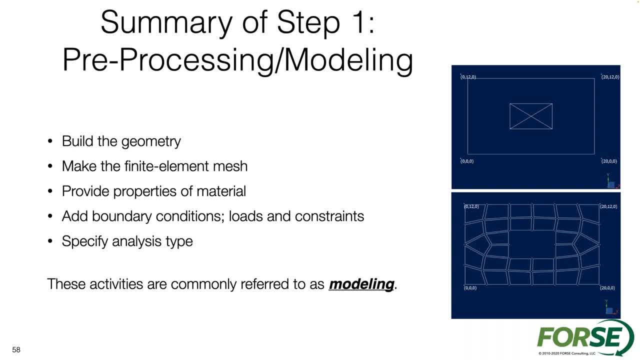 build the finite element analysis message. It's going to take the general geometry that you enter in instead of break that wall down into different pieces, so that it actually can have evaluation, because it's going to evaluate the forces and movements at each individual node. So when we have all of those, that meshing creates an opportunity for the nodes to be. 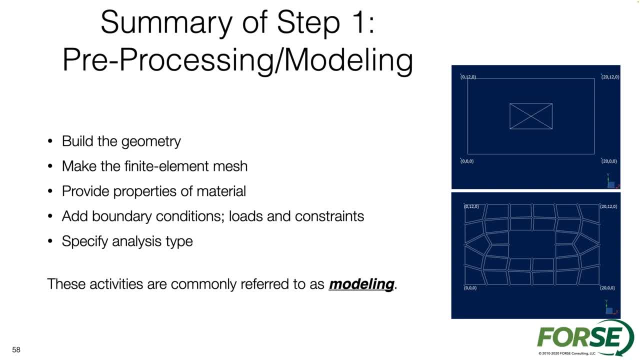 created and opportunity for all the forces to be evaluated, all those different points. So you need to have a match, You need to have something that has multiple different places of analysis within the wall panels so we can understand a lot about the forces and deflection. 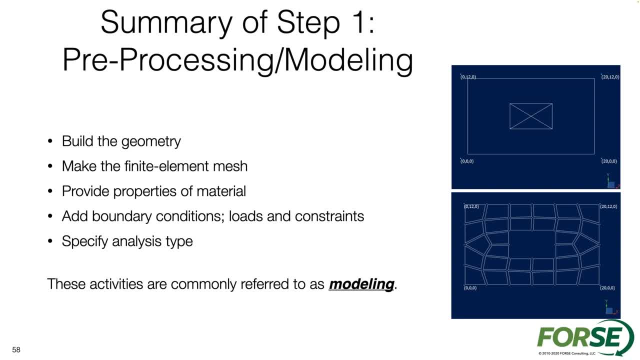 And so we want to make sure that we have an appropriate match. We want to make sure that we have appropriate material. as we break this thing apart We're going to use, to make sure that we use the right material for the design. We have to make sure that we have the right boundary conditions, how the different plates are connected to supports. 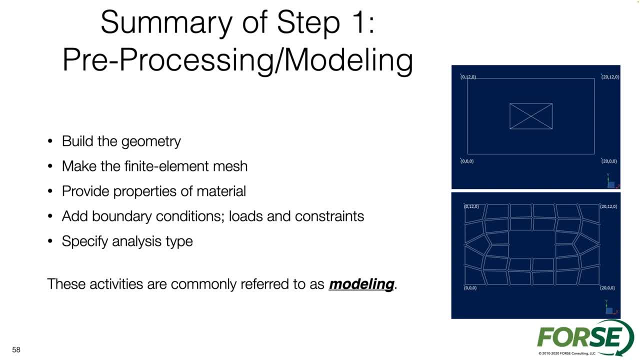 Is it vertically? Is it vertically and rotationally? How is the slab connected to the wall? How is the? if there's a concrete slab, Is it fixed? Is it pinned? So a lot of the detailing has to come into account as we build this model as well. 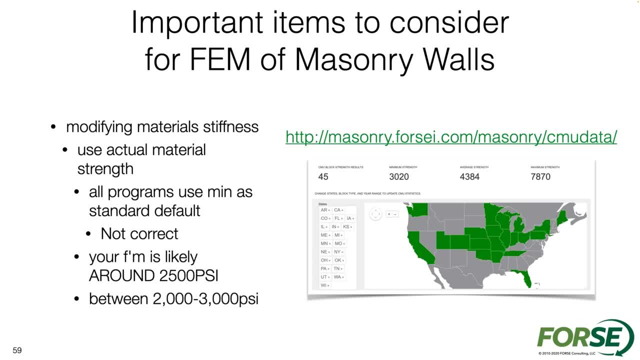 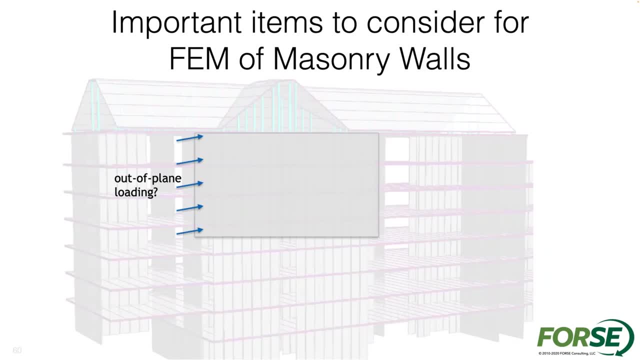 So this goes back to again using the right material. This is a slide that you've seen a couple of different times today. Again, concrete masonry- two to three thousand clay masonry were even up above that, But when we look at the actual masonry wall, 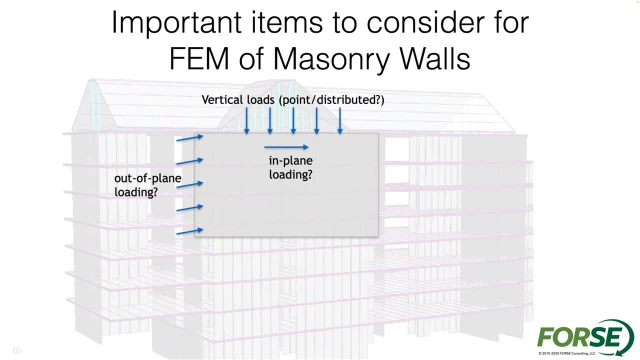 we have to consider out-of-plane loading, vertical loads, in-plane loading: Do we have a fixed base or a pin base? Do we have fixed or pinned top of walls? All those different elements to consider in terms of connectivity. And then in terms of stiffness, do we have a crack section factor? 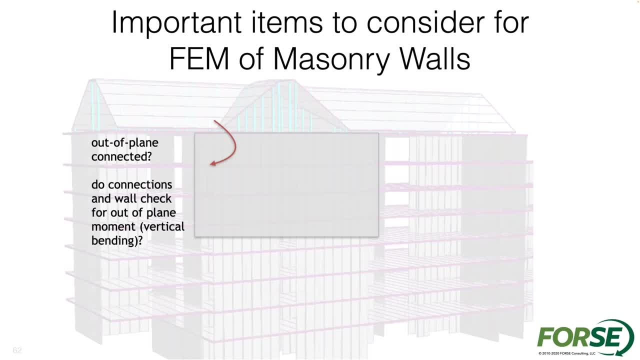 Again, that point five is kind of from the code. way back earlier this morning We talked about using a reduced cross-section for masonry. So when we put it into a finite element analysis we make sure that we have used that reduced cross-section in our finite element analysis. 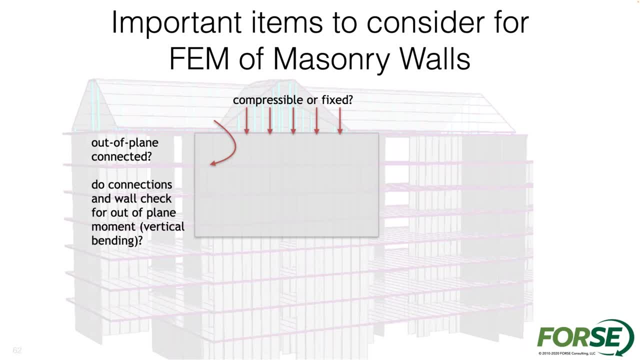 Do we have compressible or fixed? That'll make a difference in terms of the vertical load distribution. Do we have horizontal bending considered included? Are we checking horizontal bending? Do we have out-of-plane crack factors considered? Do we have in-plane crack factors that we have to consider? 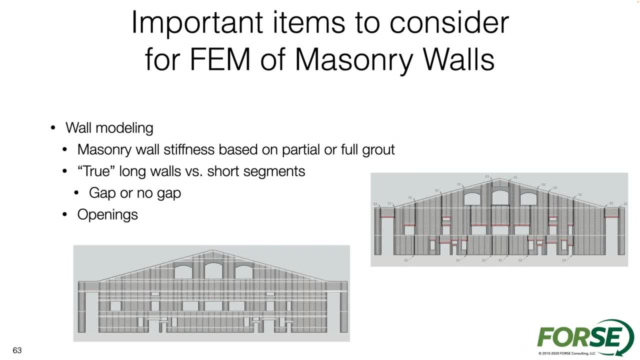 Looking at the logs, Looking at the logs wall versus the individual walls. do we have that? if we do have all the different control joints, and then we have to make sure that we model in gaps in our plate elements. we have two different plate elements, two different. 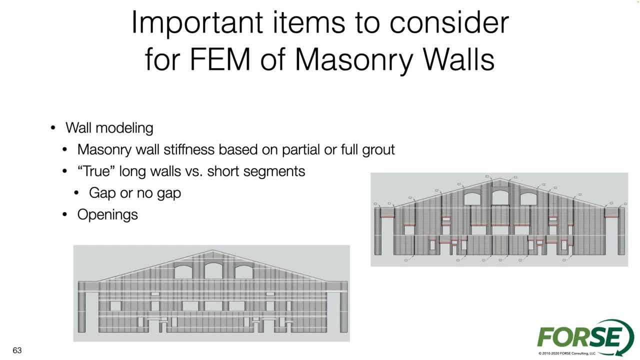 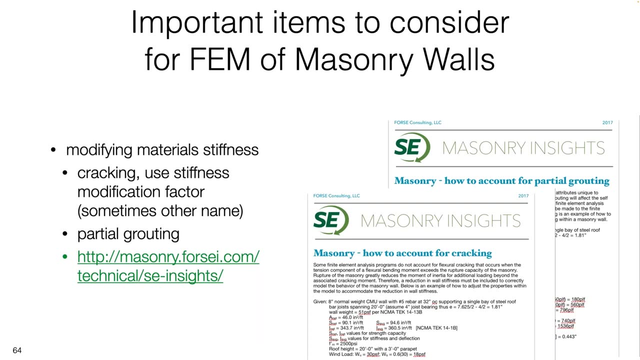 nodes. we don't have a common node between them. we actually model in a physical gap for our model. so it's going to be important to make sure that we build in all the different complexities of the model. so, again, I talked a little bit this morning about using that 0.5 crack factor modifying the material. 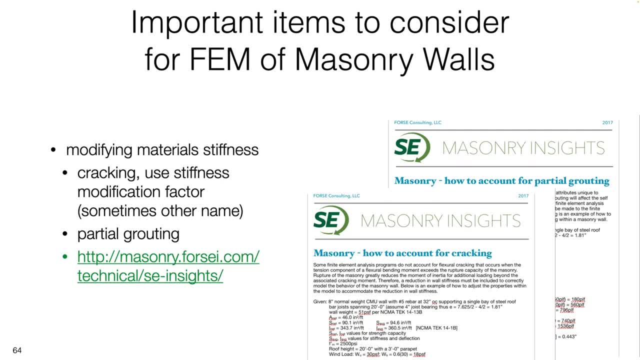 stiffnesses. we actually created a couple papers for a how to modify, account for partial grouting and a final analysis, how to account for cracking. I determine what your crack factors could be for your structures again depends on the different types of forces that you have have. crack factors can be different in 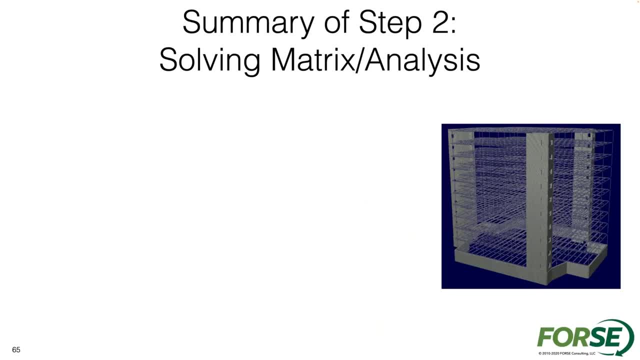 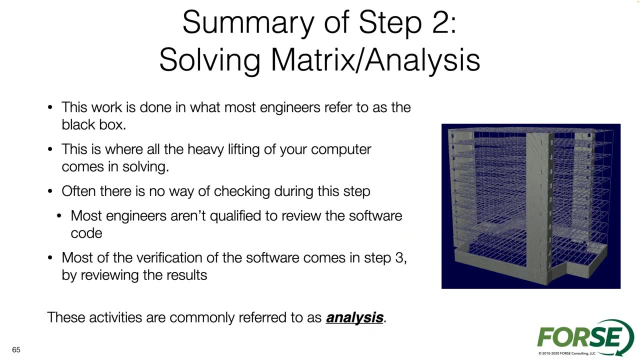 our designs. you solving the matrix. this is a typically the analysis part. this is usually what most designers when it engineers. when they talk about software being a black box, they're usually talking about this part. we go from creating this model, this beautiful model that's an imitation of reality, and then all of a sudden we 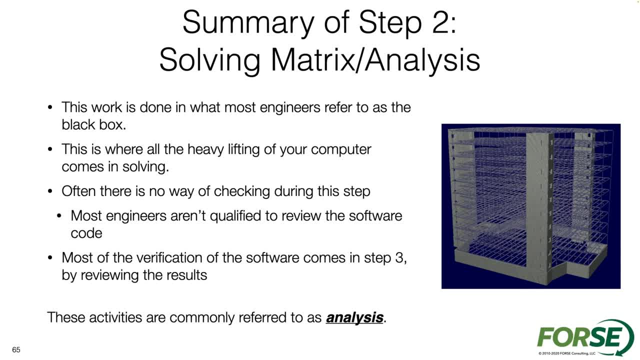 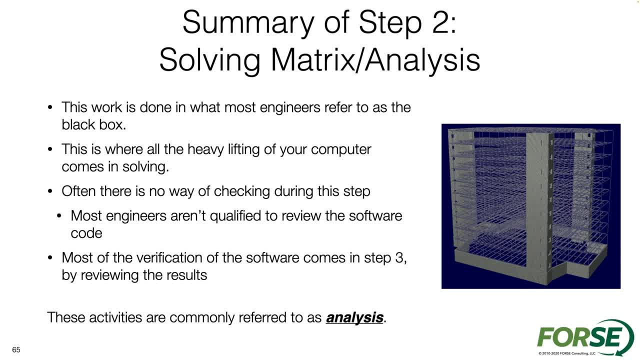 seeing the work get good results and we bring down videos for this to better demonstrating it. I hope that was helpful to you. thank you for listening. thank you, llevar, and for all your questions about the research on buzzy ledger's digital Rings. that's cool. I appreciated it, even though it's pretty much expensive outcomes. but 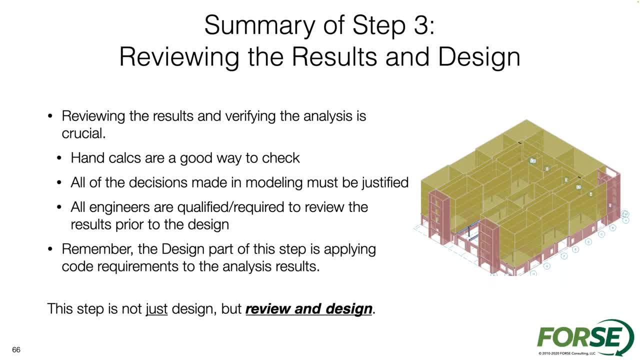 still, we're just filling it out there. hopefully it supports what you're talking. looking at the individual parts and pieces, you know what I try to suggest to people is verifying: verify the analysis, and how do you verify the analysis? well, it doesn't start with a complex model when we want to verify analyses. you 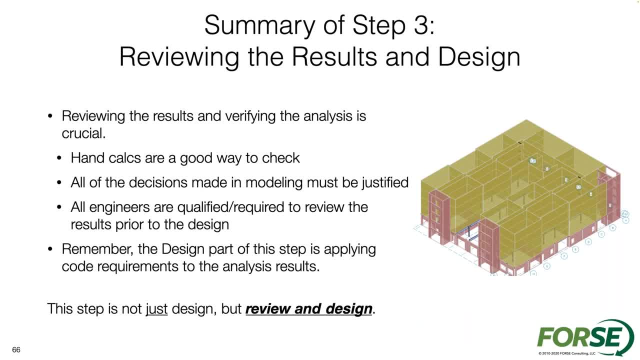 really have to create a model that's a lot simpler, smaller model that we can get our arms around a little bit so that we can't have um, we can have an ability to check the analysis. don't just build a complex model and use it as a black box. 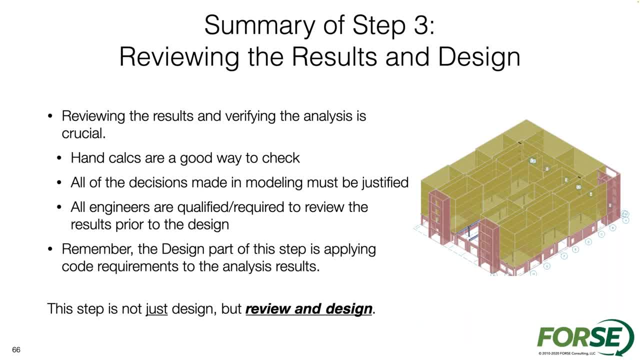 try to use a simple model, understand the analysis and understand. you know some of the results and then you can move into the more and more complex, add into the complexities over time. so again, it's not just design. I would say step three is definitely the two parts of the reviewing the results and the design. 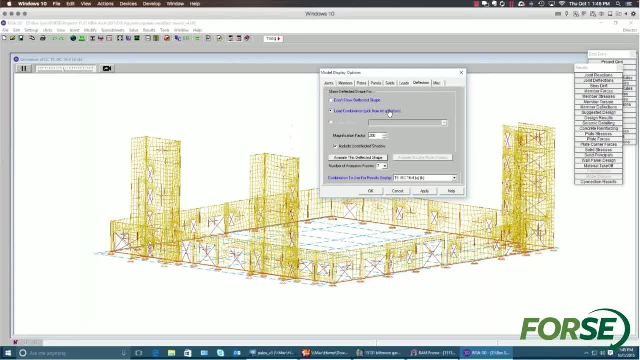 some of the best parts of reviewing the results is just going to be animating the structure, and I think there's so much that can be learned about the overall building or the design of the building or the design of the building or the individual results by just reviewing the structure, looking at. 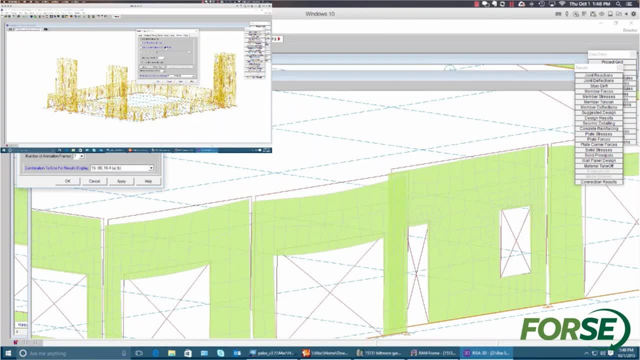 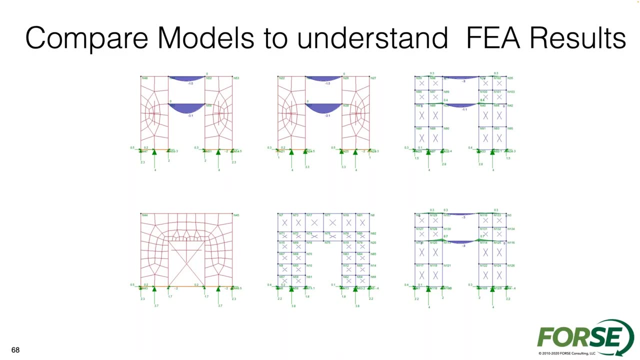 different parts and pieces to make sure that we agree with the design. other parts of understanding, of finding an element, analysis would be. you know, looking at different elements, we have different options within the program and within those different options it's going to create different results and so 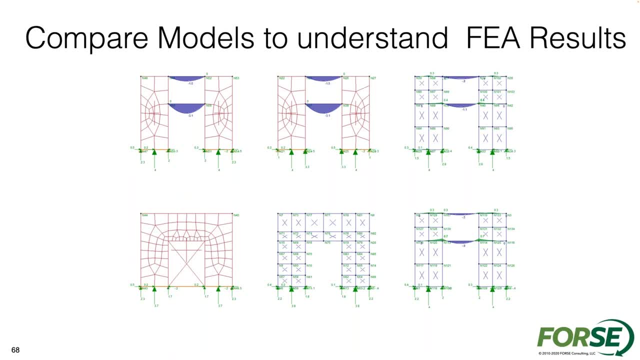 I suggest to people often: build a model that's a little bit more complex and build similar but different models. you know, if we don't understand exactly how the program's designing lintels or analyzing to create the forces for lintels, build a lot of different, simpler, similar models so that we can kind of 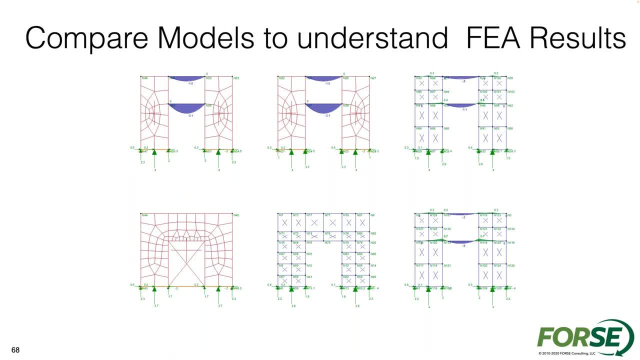 step-by-step go through them and kind of see what some of the forces look like. so this is kind of similar to what we did before, but this is kind of looking at the overall wall, not just just the lintel elements like we were looking at earlier. 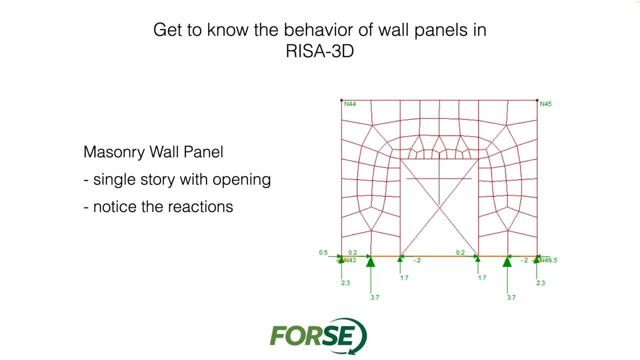 earlier in the lintel section. so if I have a masonry wall panel, a single story with an opening, let's just look at the reactions. you know, looking at the reactions for a wall, you know, oftentimes we have walls that I was gonna have, you know, with no opening. it's gonna be, you know, the the nodes at the end I'd expect. 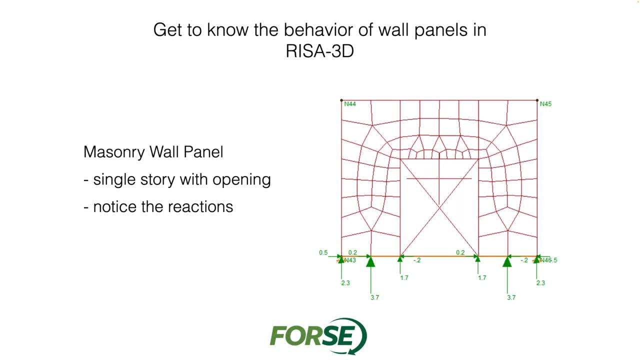 them to be a little bit less in terms of the vertical reaction. but then the- you know, all of the nodes along the length of the wall are gonna be similar to one another when I add an opening. there's a little bit of complexity there, you know does. 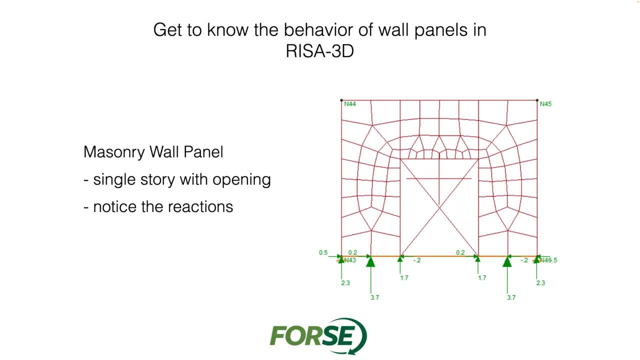 the opening. you know what are the low goal that's above the opening. you know how do the reactions kind of get distributed. what are some of the behaviors in the area above the opening that changes. you know the way the reactions are created. so if I look at the model I see these reactions. you know. 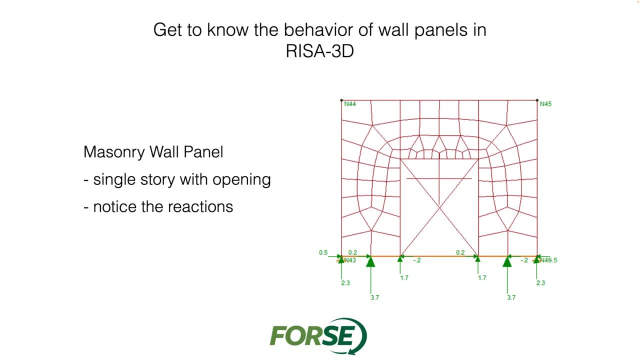 I would expect the reactions next to the opening to be higher, because that that's not what I expected. area above the opening certainly had some vertical load on that. how is that load getting shared? you know, it looks like the end of the wall has a higher reaction. well, how is that possible? how? 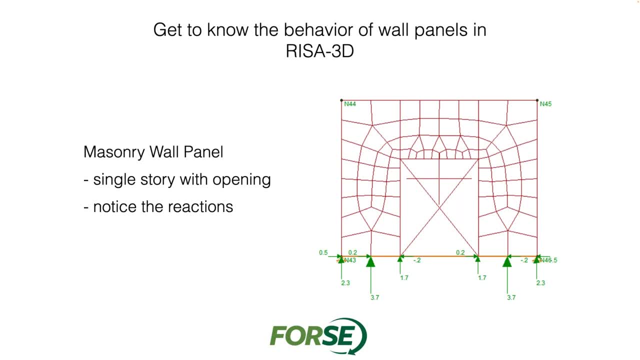 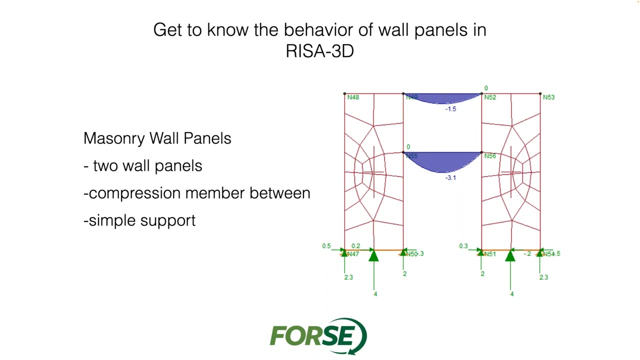 does the load get out there and kind of skip some of the interior portion of the model? interesting, let's look into it a little bit. if i play around with the wall and i i create the wall panels and i create a compression member, just at the top and bottom, it's simply supported, but it's a. 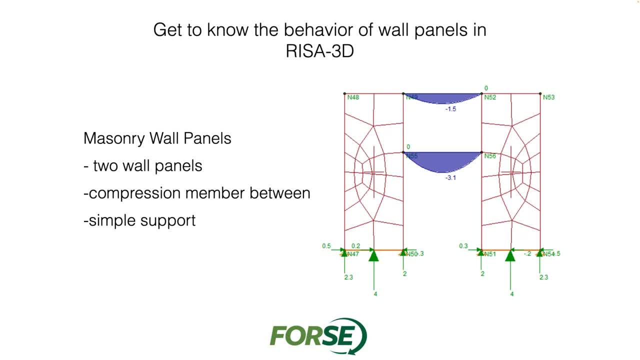 compression member. apply all the same loads, i can see the reactions change, i can see the forces change a little bit, you know, and how the loads get distributed, um, you know so kind of: how is that affecting the overall model? now, if i change it a little bit more? 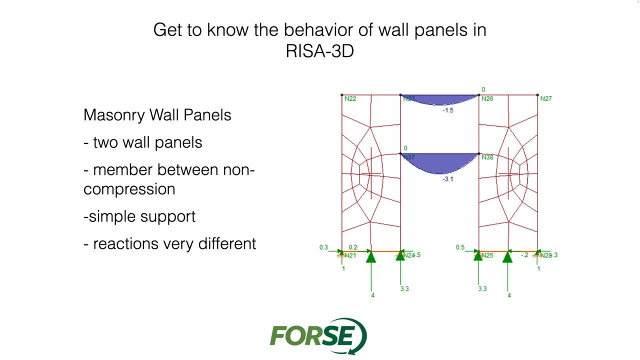 i have the two wall panels, remember, between our non-compression but still simply supported. now i can see kind of the that expected behavior that i was thinking of. if it's a non-compression element and it's simply supported, then i can see the end reactions be. 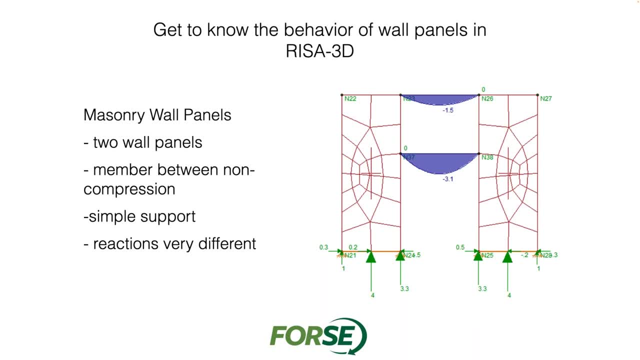 minimal. i can see the reactions next to the opening be a lot higher, and then i have to start to ask myself: well, the reactions are different. does this make any sense? do i have the ability for the area above the opening to be non-compression if i don't have a control joint in there? you know, masonry is actually very good in compression. 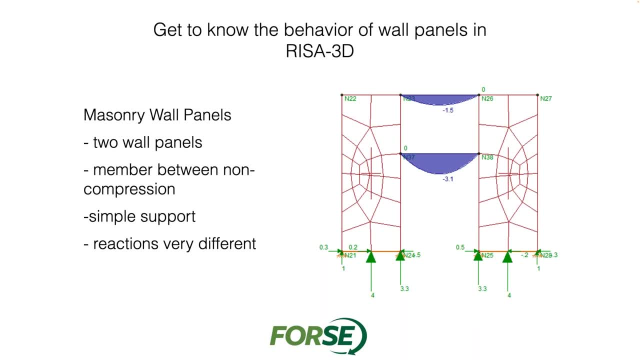 so you know, although this is maybe what i would have expected in terms of the reactions, maybe this isn't exactly, um, you know what, what i should be designing for you know, maybe i'm trying to learn something as i'm using the finite element analysis model, so let's take another step. 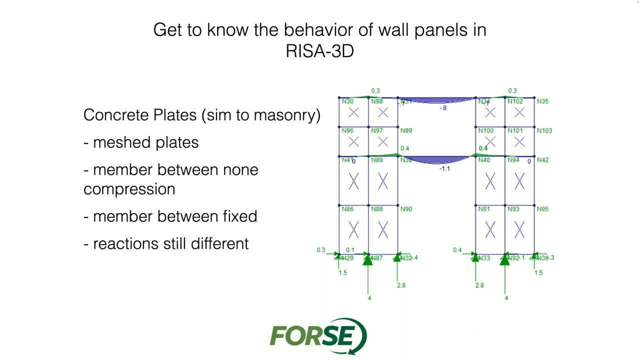 so if i look at the mesh plates, i look at the member as a non-compression element, but the elements are fixed, so again. so if i say the masonry lintel is going to be fixed, so the walls on each side, if i say, you know, the element at the top is going to be fixed, 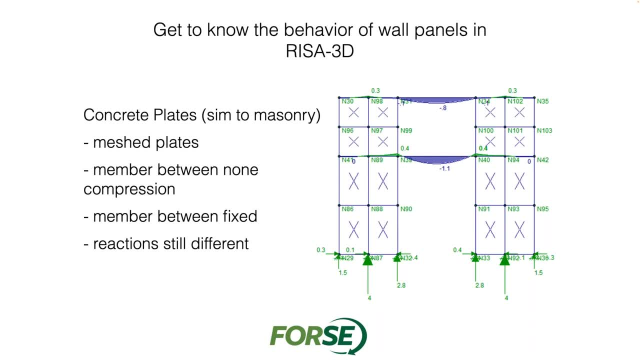 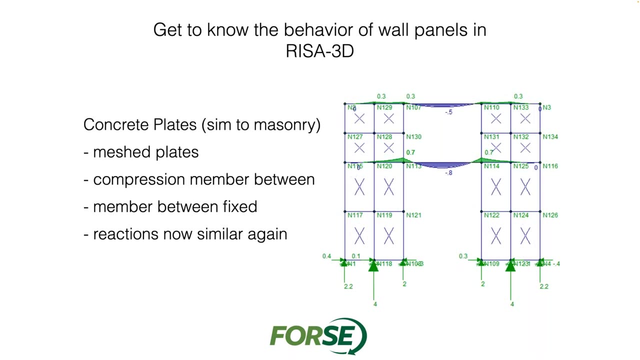 i can start to see some of that load getting pushed out from the center. i don't have compression, but i have continuity in the fixity that i have between the two elements. so interesting. i take another step. so if i look at it again, um, again, compression. 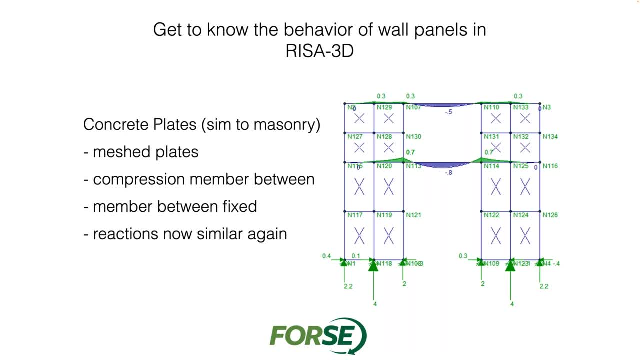 between the members. i have it fixed. now i see reactions that all of a sudden look like the forces, um, at the opening, at the edge of the opening, are less than what the forces are at the ends of the walls. that's kind of back to that original analysis. so you know, with 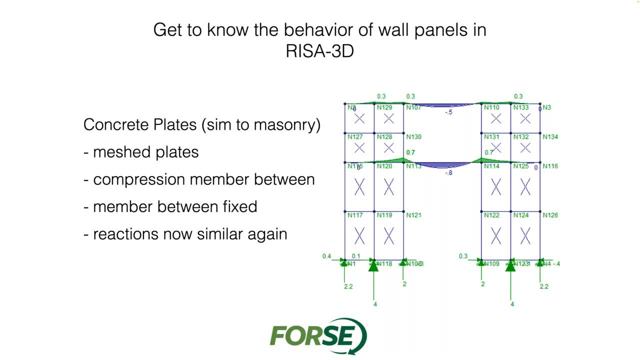 a masonry wall, do i have those lintels that are actually going to be fixed end members, that are going to be compression elements, that are going to be having that force, uh, not be allowed to arch over the openings. so if again, if I take another step, so that's looking at. 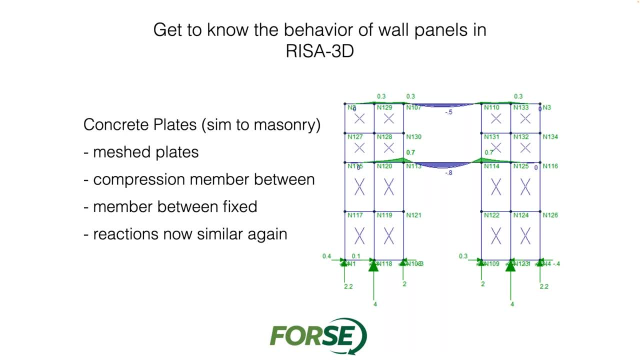 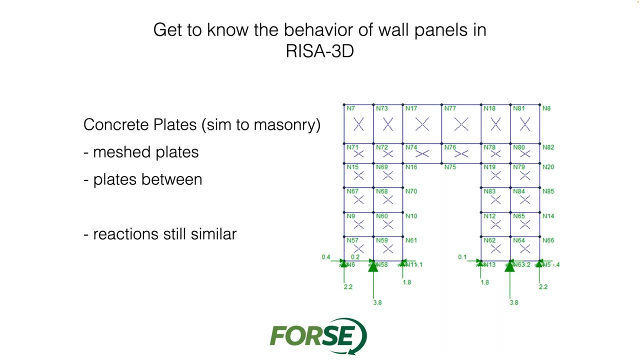 all with member. and why do I use 1d finding element members is because those are a little bit easier to understand behavior and think about how the different, how I can change them and tweak them. now I look at plates. if I had plates back in there I can see similar, similar features. here I can see the 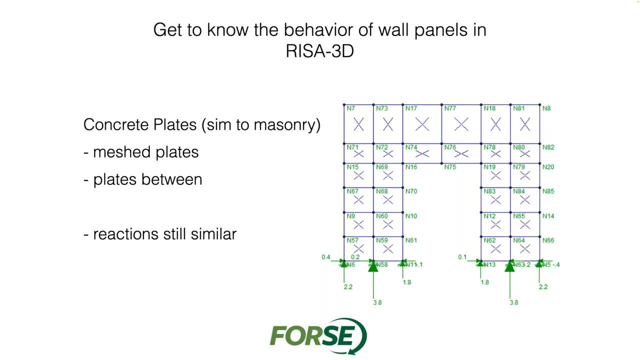 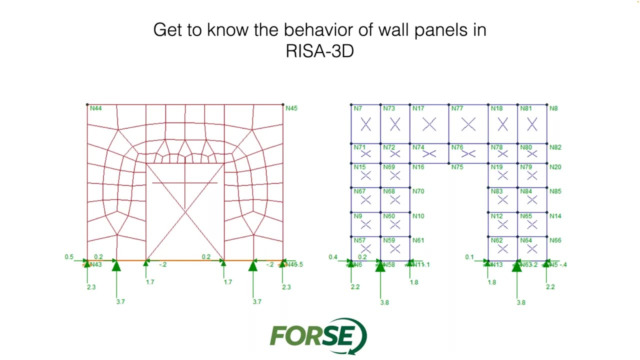 reactions changing as well, I can see again the force kind of moving away. and so then I move all the way back to kind of those wall panels. if I have wall panels, how do those? what are some of the boundary conditions? what are the things? that are a little bit different, you know. so I start with a wall, I look at the 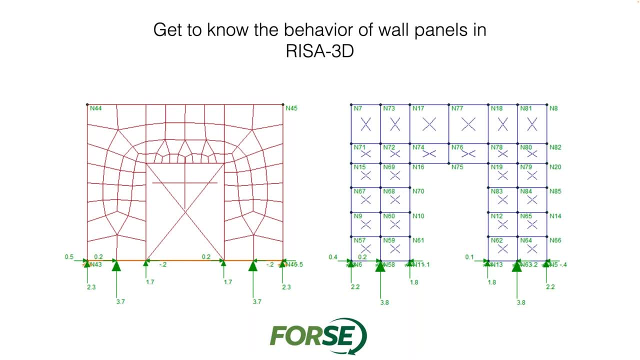 reactions changing as well. I can see again the force kind of moving away reactions. I really break that wall apart. try to create a simple model. make some 1D line elements so that I can modify the properties of those line elements, see what those varying 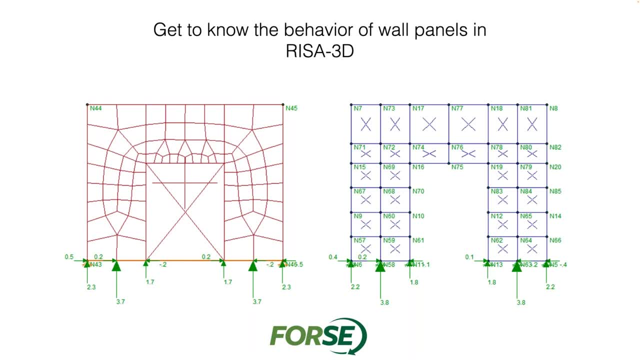 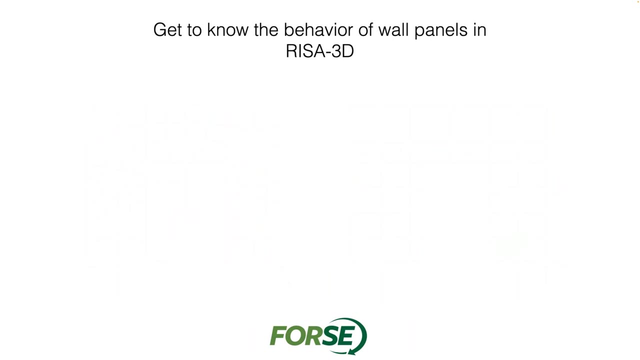 properties. see how that changes my reactions. All of this time I'm thinking about how masonry is actually performing, but some of the modifications that I'm making is just trying to understand what finite element analysis is doing for the model that I'm looking at. 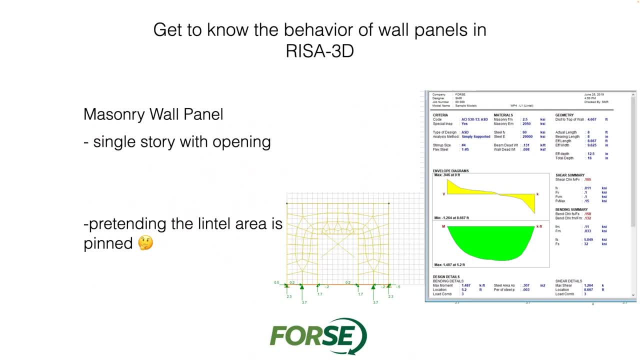 Some of this exercise was looking at again that lintel above the opening. sometimes looking at that lintel as a pinned element really is silly. it doesn't operate that way. the analysis doesn't support it being a pend element. it doesn't support it being a non-compression. 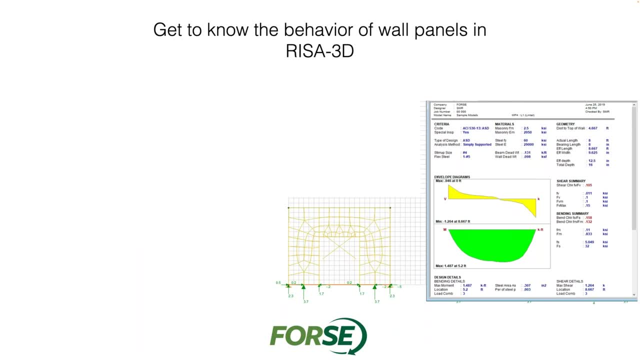 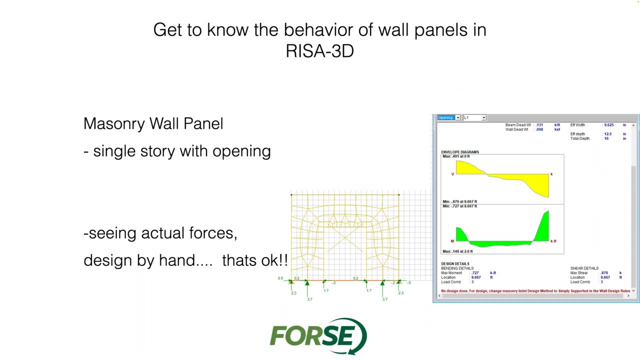 element. Really, all of the analysis has pointed to it being a compression element with something that's going to have fixed-end conditions, with negative moments at the ends, some positive weather conditions, Some of the most disruptive annual conditions of the two Fr. continuing in this process is lure pruning, and verifying what the material is doing does reduce the 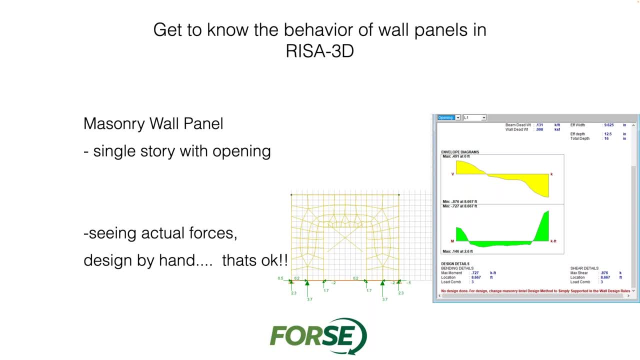 rate of the yield being released, not just clearly, but it can have an effect also reducing. moment in the center, again utilizing, utilizing everything that I know and again starting from simple and adding in the complexity really helps me to get to that understanding of both the software and of the lintels that I'm looking at. 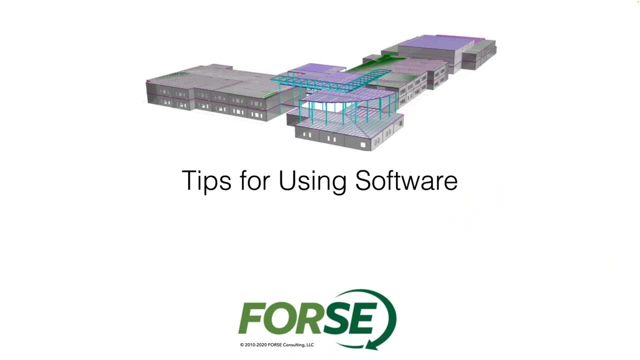 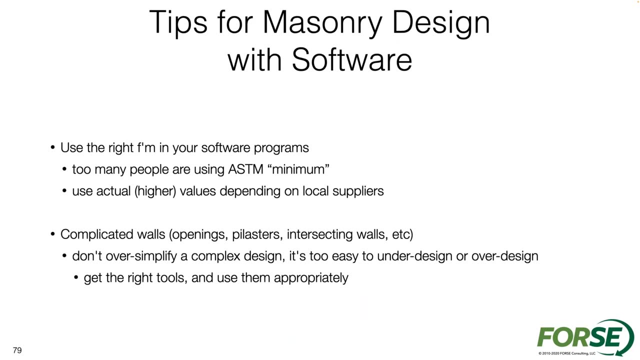 for design. so so, from tips for using software, make sure that I use the right strength of materials. try to understand what the actual strength is. maybe use those prism tests to understand what the strength materials. let the walls be complicated, put in the joints- for I need joints- and take them away when we don't. 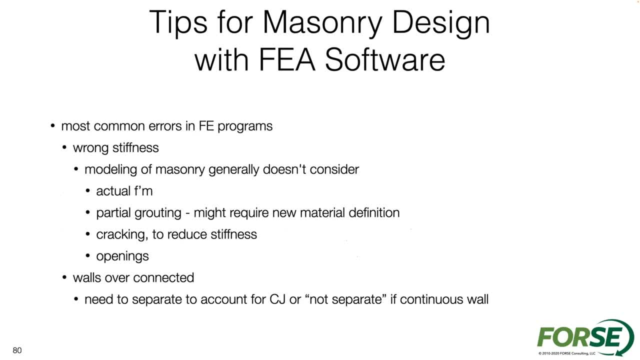 have joints there so that we have a continuous wall. make sure that we make the modification to a partial grouting and cracking. you know that's going to be something that could be really important to modify the properties of masonry anytime that we do have different materials. if we have steel and masonry, you know how the load 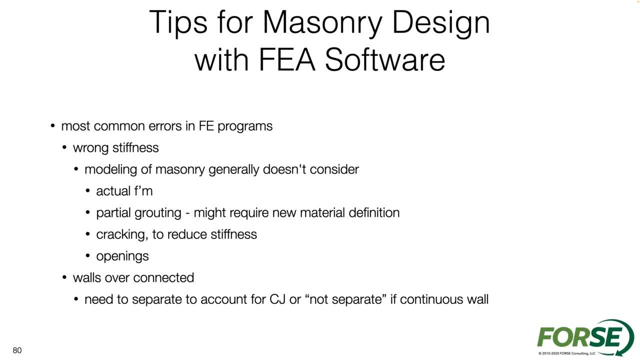 is going to be differentiated in and and how the program is going to assign the lateral load to the steel members is going to be really depending on its stiffness, and if something cracks and it has less stiffness, we need to make sure that we tell the program that so that it can attribute the load to the right. 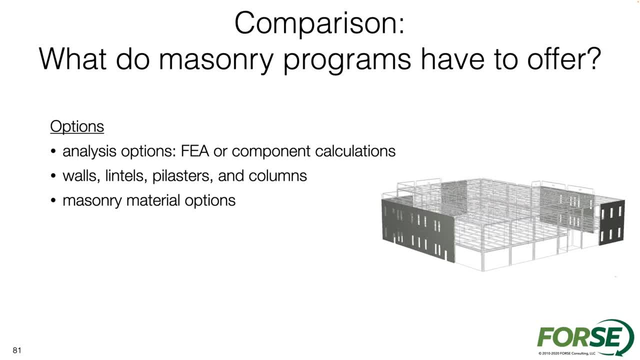 element. so, within all these programs, you know, what I'm going to do is I'm going to do kind of a comparing and contrasting across different programs. you know, I'm going to try to evaluate the programs and again it shows. you know, if you were looking for a masonry design software, it can help with that. if you're looking at 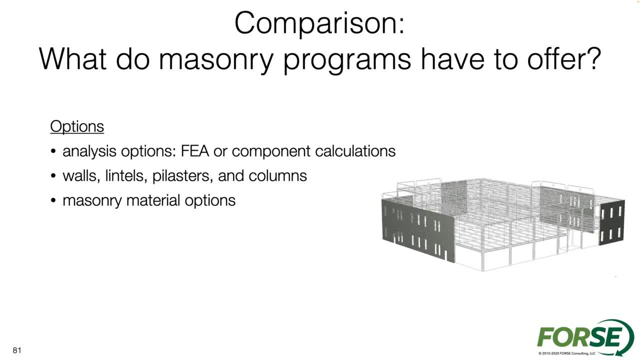 kind of understanding, when I go from one program to another, why I get different results. well, just seeing the different features, that'll help you understand that if you are looking to do some different types of designs, or if you're trying to, you know, can just really help you with understanding what different tools 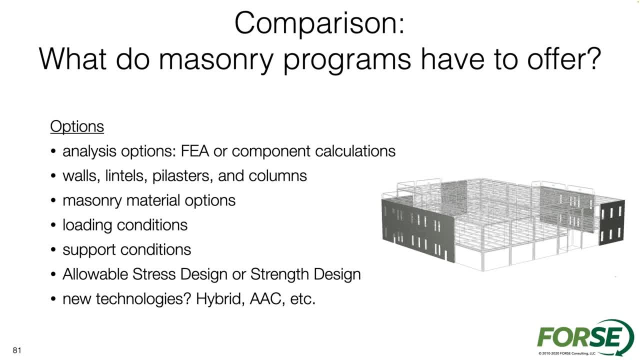 you have. so, whether or not it's a component, design or fea, we'll separate those two categories out. we'll look at how the different programs handle all the different types of mainstream elements. we'll look at material options. we'll look at loading and support conditions and then we'll look at whether or not it supports. 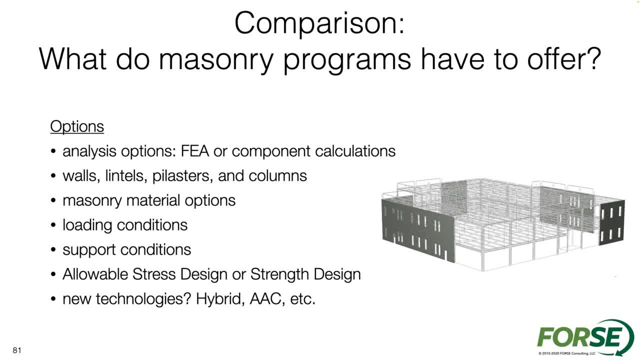 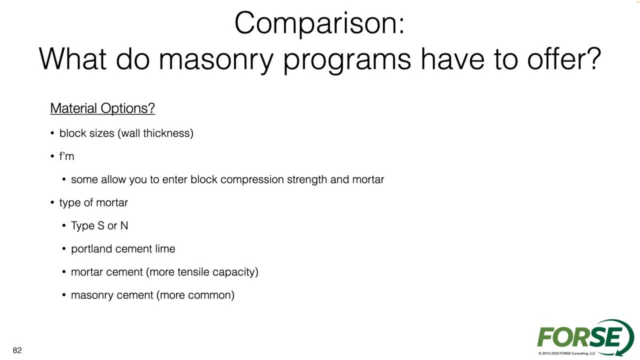 asd or strength design and other materials or other technologies as well. so material options again. a lot of times for these programs we're just going to define strength of masonry. sometimes the programs are going to ask us for mortar type, you know, um. so sometimes it's going to be using a block and mortar to determine what the overall 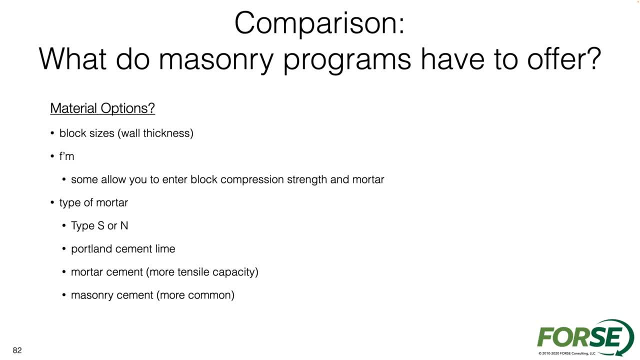 strength of masonry. that's not common. most of the time you're going to enter in an f prime m and the only reason that it's asking about mortar is if you want to define design masonry, you're going to want to define the strength of masonry. 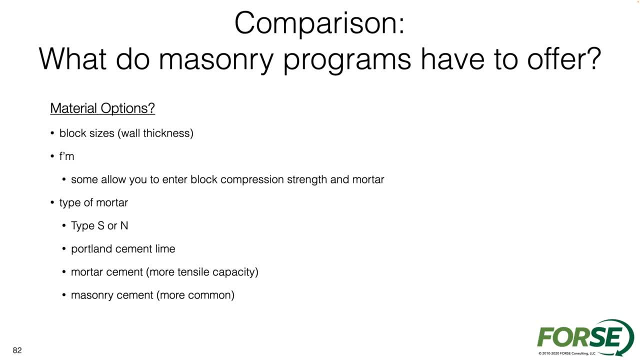 you're going to want to define, uh, unreinforced masonry. so it depends on what type of mortar you know, because they have different tensile capacities, the the mortar supplement having the more tensile capacity. um, whatever you're looking at, whenever you look at a program, a software program, uh, don't use. 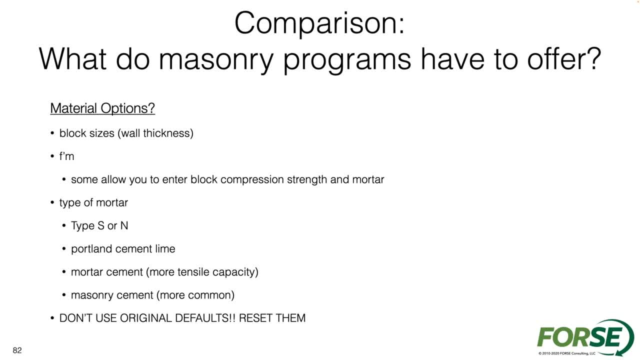 defaults. i say that often. i said that uh 12, 13 years ago when i worked for the software company. defaults are just starting points. they're not meant to be uh standards. too often people will look at a software program and be like, well hey, they're using this uh value and that. 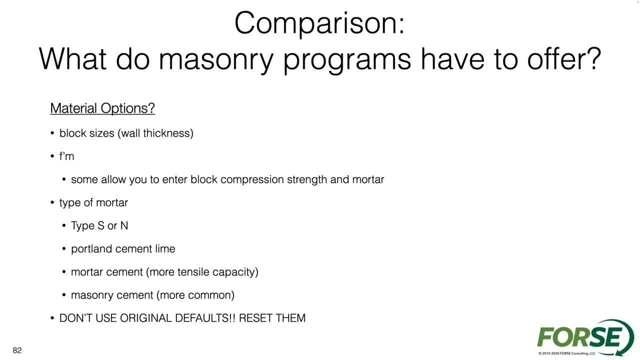 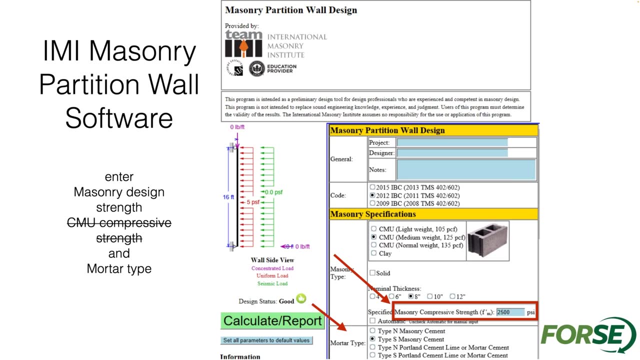 that must be an industry standard. it's not an industry standard, it's just a single point to start, single point of reference. so reset the default is always really important. so here again a good example of entering in masonry strength. i'll enter into f, prime m. make sure we start with the actual. 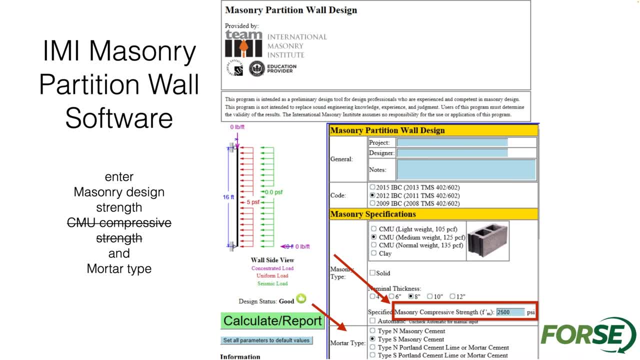 strength of masonry. and then we put in the mortar type. again here the mortar type is going to be used for, uh, determining an unreinforced masonry option, whether that's going to be relevant. if it's, if it's reinforced and the motor type really isn't going to- 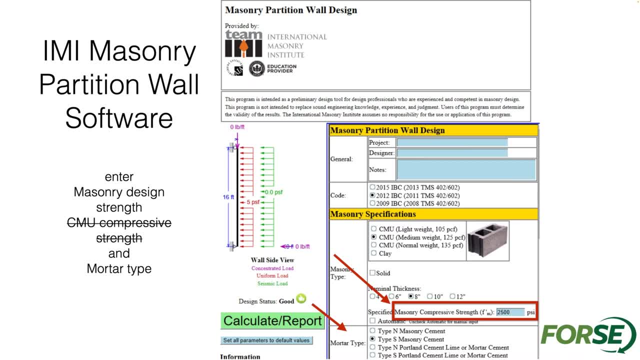 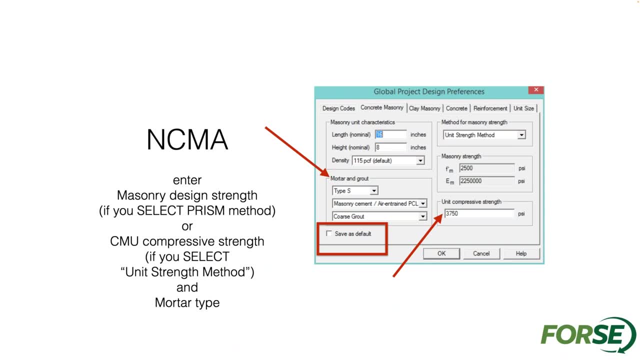 have anything to do with the overall design. so ncma has a program, masonry design system where you actually can enter in the block unit compressive strength, and so that program you look at not the f, prime m, but you enter in the unit strength of the block and the mortar type and then what that program is going to use, whether 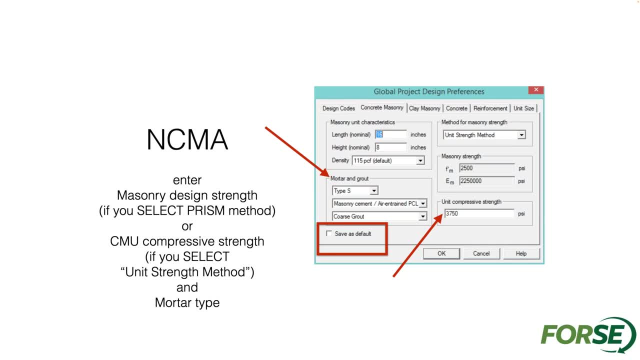 it's reinforced or unreinforced is going to be using the mortar type, because if it's reinforced it's going to be using still the mortar type and the block strength to determine what f prime m is for you, kind of a nice little little feature, um. or if it's unreinforced, then it obviously matters. 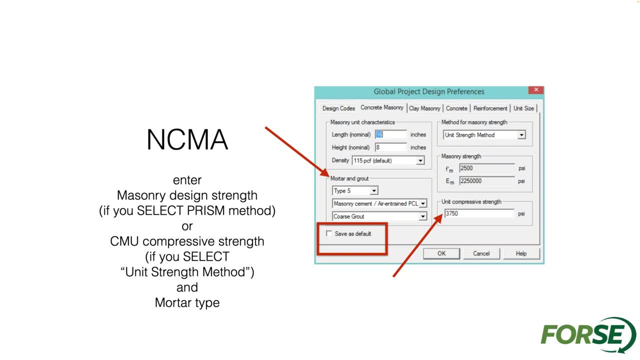 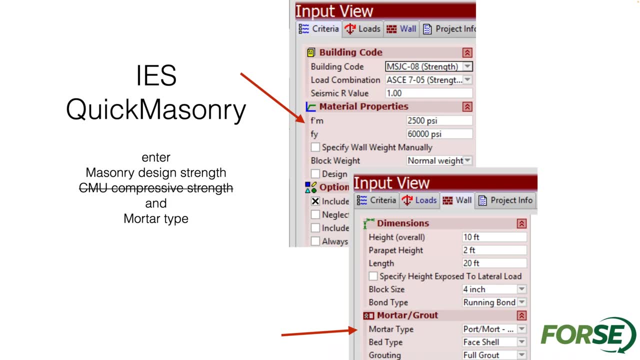 the mortar type and the type of mortar to determine the tensile capacity if it's under enforced ids, quick masonry, that's another one where we're going to put in the strength f, prime m of masonry and then mortar type, for again, if it's unreinforced. 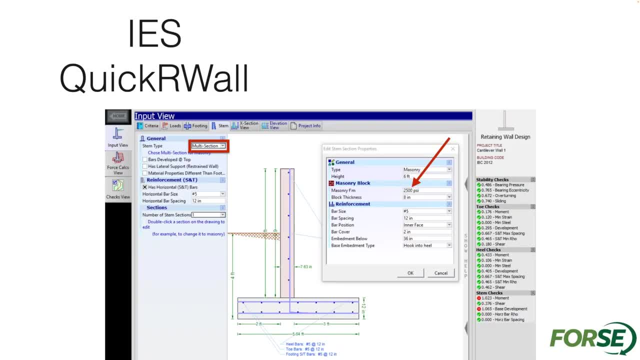 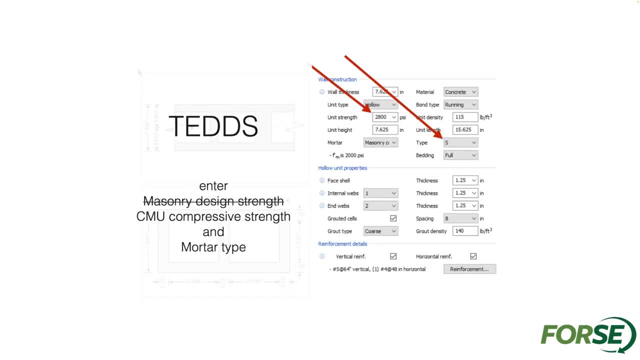 you have quick r wall, which is the retaining wall program. so a lot of different software programs. i'm just kind of trying to show you a lot of different ways that they enter in f, prime, m or ted, where you can actually put in again the unit strength of the block and the type of 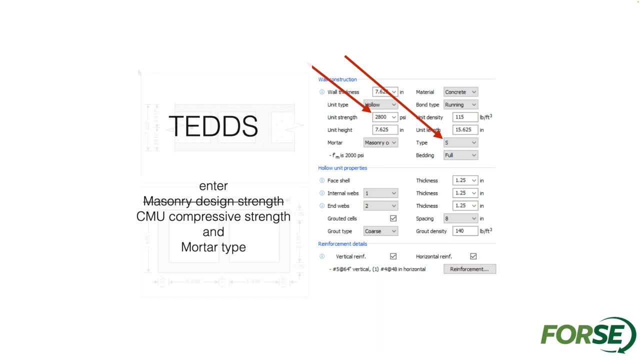 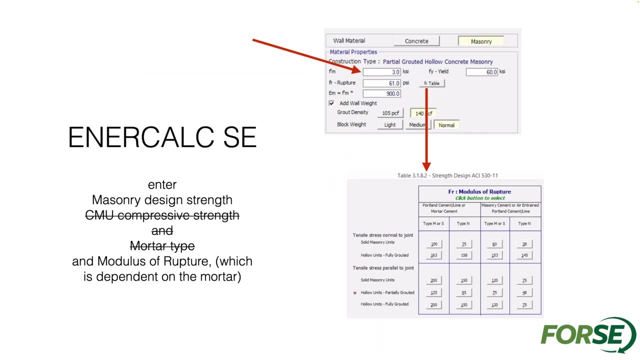 mortar so that it can determine the overall f prime m and then enter kelp as well. we're going to actually put in f prime m. then you can also put in the modulus of rupture. so if any of those values are different than what's in the code, i think most of the time you're just going to use code, but then it gives you. 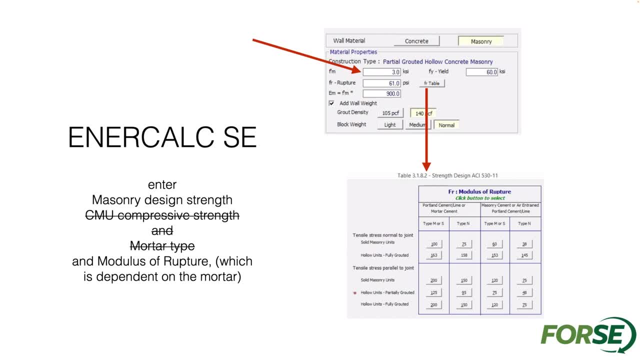 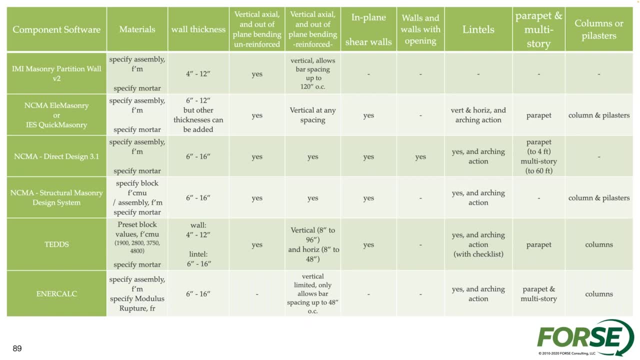 kind of again the specific tensile capabilities for an unreinforced masonry design. so, getting to uh, this table, this is one that, um, you know i use for uh people from time to time to help understand. you can see, if you just kind of look across the. 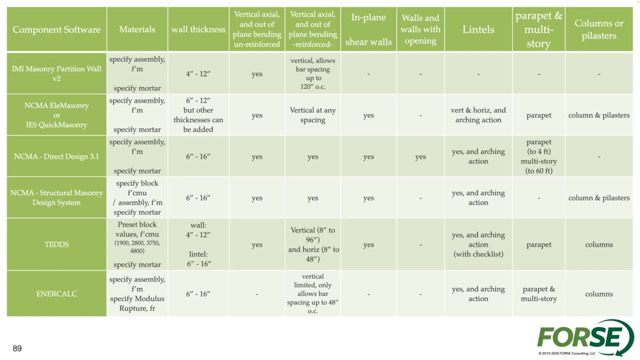 table all the different options that you have with different software programs. it really does give you a lot of different abilities to vary the the strength of materials up and down the different programs. some of the programs have limits to the wall thicknesses that you can look at. 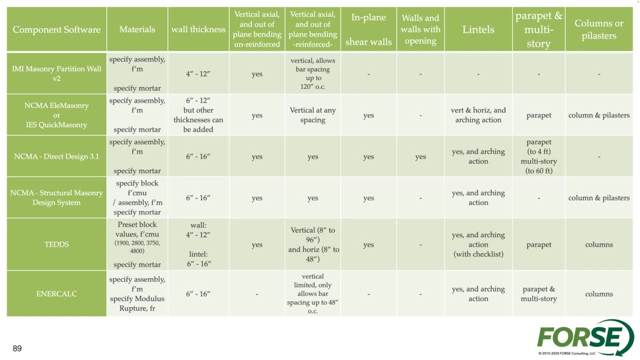 i'm not sure exactly why programmers would do that, but you do have some differences there. we have vertical- um, you know, axial out-of-plane bending, the in-plane shear walls. you know that's not supported with the partition wall program, which makes sense. partition walls aren't sheer walls, you know walls. 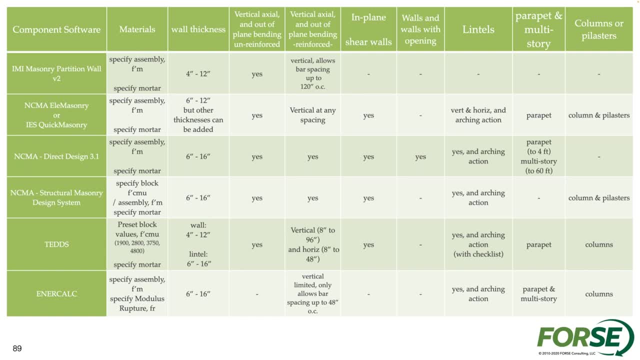 with openings. you know, again, a lot of programs aren't going to necessarily look at walls with openings, because it just wants to look at a rectangular wall. so these component design programs, as they're trying to stay very simplistic, the one that does allow you to put in openings- 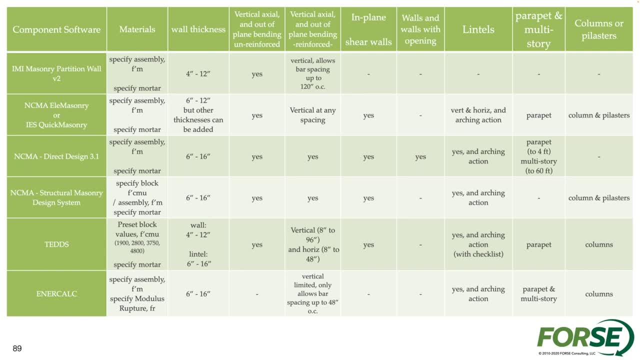 with the program that's going to do is it's programs going to break out the wall and put it into the different components, so the direct design where you can put in an overall building, but it's going to do a lot of component design calculations, uh, kind of all at once. lintel designs will be a vertical and horizontal. 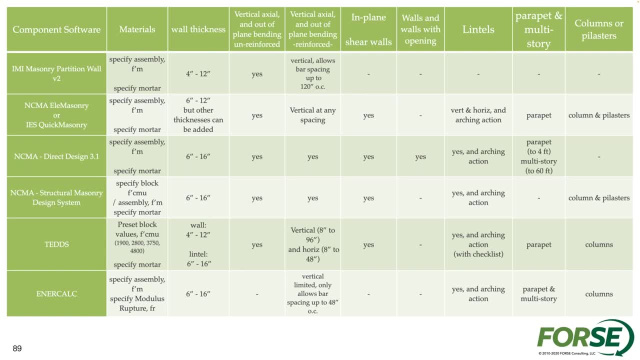 and arching action that we can consider for a lot of these programs. some of these component design programs allow parapets, some of them don't, so understanding whether or not you put in the parapet what the parapet pressure is going to be, 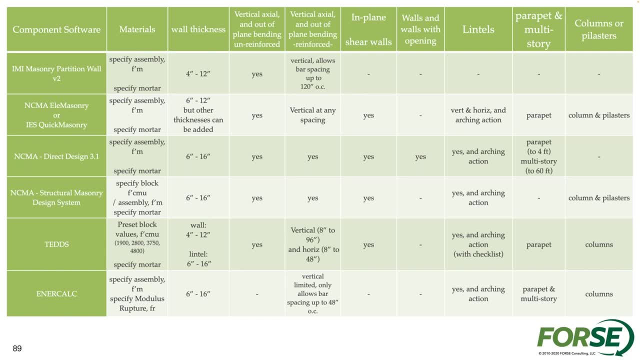 um, are all going to be different parts of making sure you design right and then whether or not you have column pilasters. so that's component design programs, those isolated elements, uh, kind of you know their approach to masonry design. if i get into ram elements, that's going. 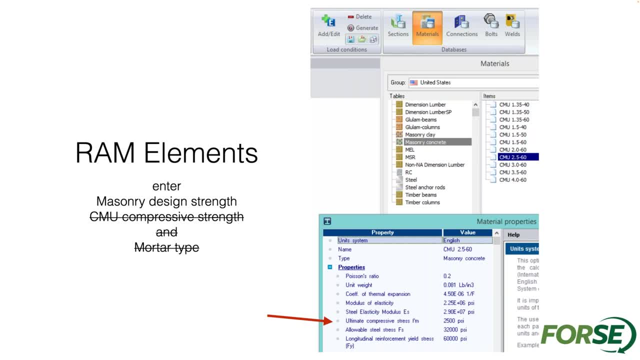 to be one of the finite element analysis programs. uh, here you can see, we're putting in the f prime m. we're just putting that in directly for the design and then within the design tool for ram elements. you can see again, it gives you back the material. 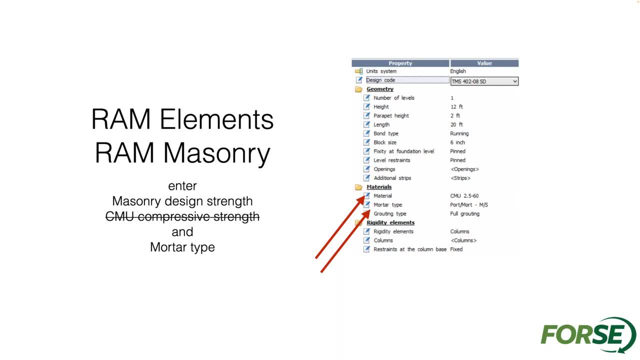 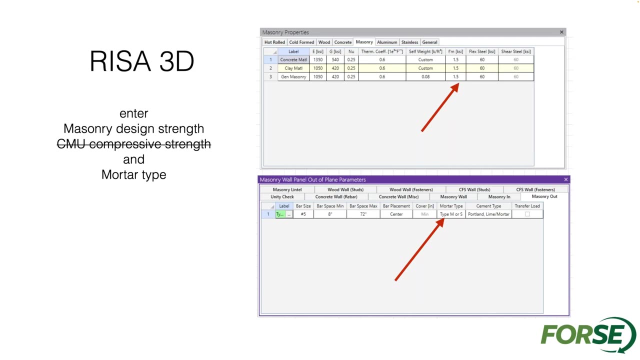 that you selected. but again asking for the mortar type, it's not going to change the material, it's just going to again be used if we get into an unreinforced design situation. similarly with reset3d, we asked for f, prime, m and then we asked for mortar type for unreinforced design. 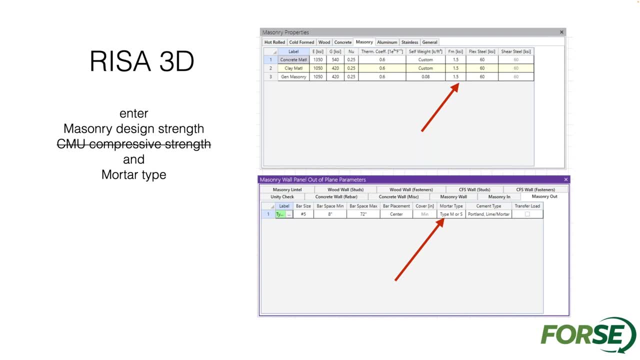 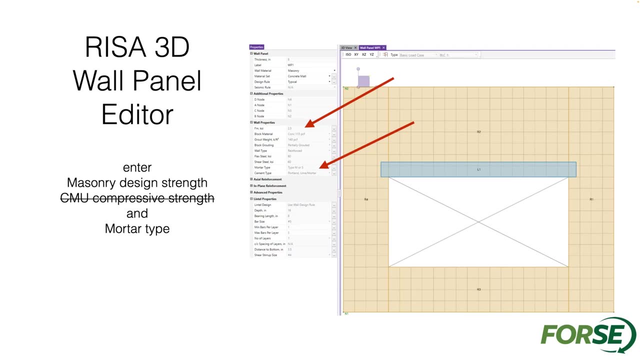 so that the general program and then the sub program are going to be the same, but you're going to be using it as a specific design tool for major walls. wall panel editor: it gives us again more options for utilizing the default values that we've put in, or? 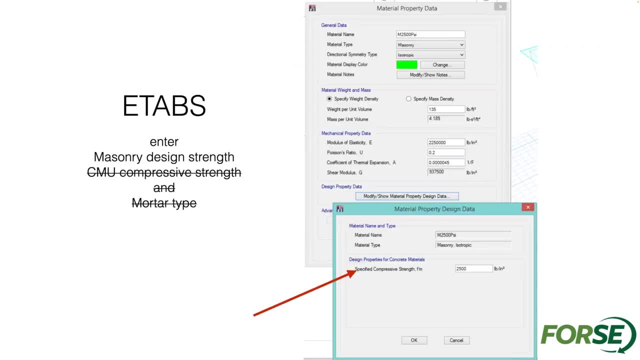 making special accommodations per panel. e tabs is going to be another one where we enter in the overall f prime m for design strength. this one's not going to be looking at an unreinforced wall, so it's not going to ask you for the mortar type, it's just going to ask you for the fm. 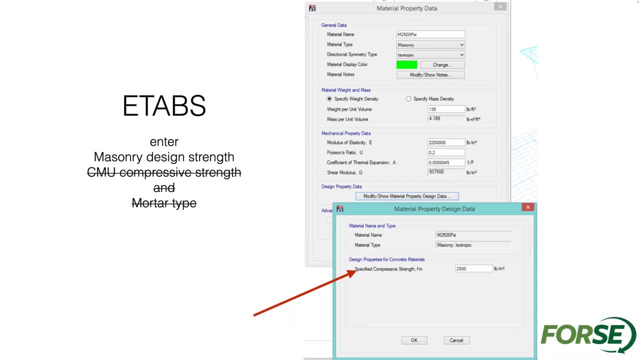 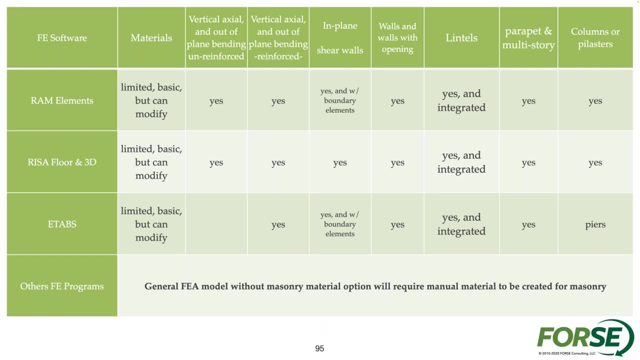 design a lot of times with solid grouted masonry shear walls. it's going to be the time when we use e-tabs. the thing about finding element analysis is we do have you know all the different options here for materials. we have options for in-plane, out-of-plane loading. we have lentils that are 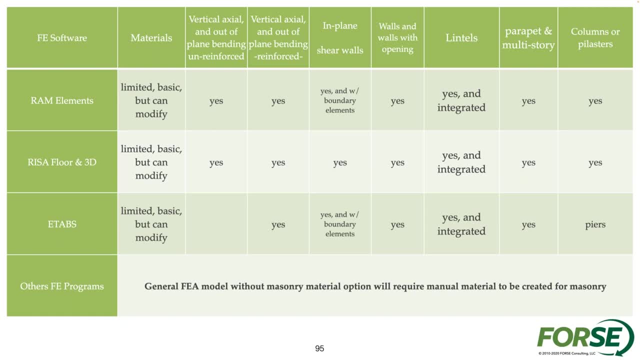 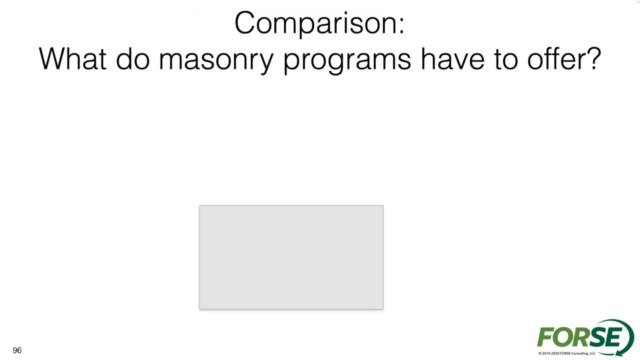 going to be integrated in the overall wall itself. we don't have isolated elements. and then we have parapets and poly pilasters and columns- all that can be added in. so other things that i think are important is when we get beyond some of those initial capabilities or materials or what do? 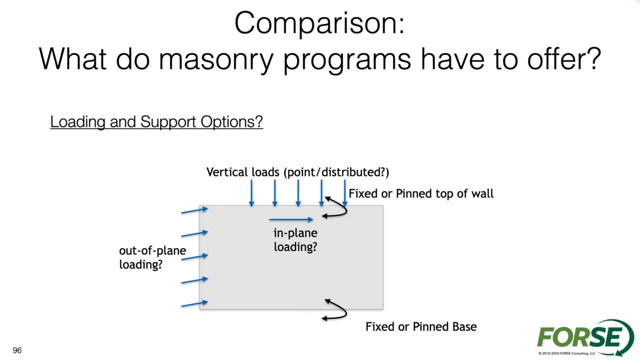 we actually have in terms of support conditions and adding in some of these factors for modifying the stiffness of these elements. a lot of times the the support conditions, loading conditions- there's going to be a lot of variability with the different types of materials that we're going to be adding in, so we're going to have a lot of 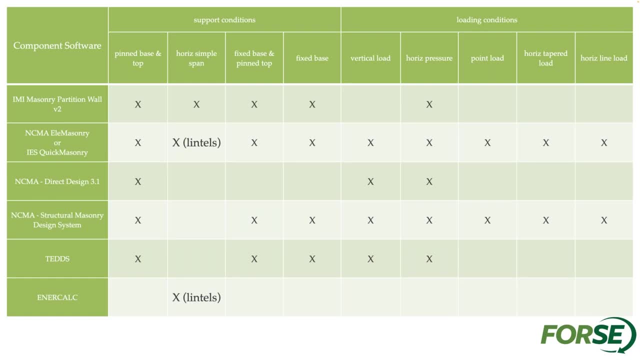 variability with the different types of materials, that we're going to have a lot of variability with the different types of materials, that we're going to have a lot of variability with the different types of programs, and it usually comes down to these component design programs. it comes down to 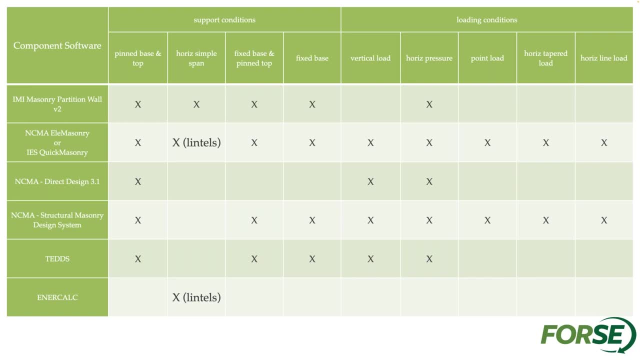 what was the intent for creating the program? obviously, a partition wall program is not going to have a lot of different loading options. it's going to have some other options that will be available for support conditions. relative to the different ways you could connect the partition wall is something like elementary. it's going to give you all the different. 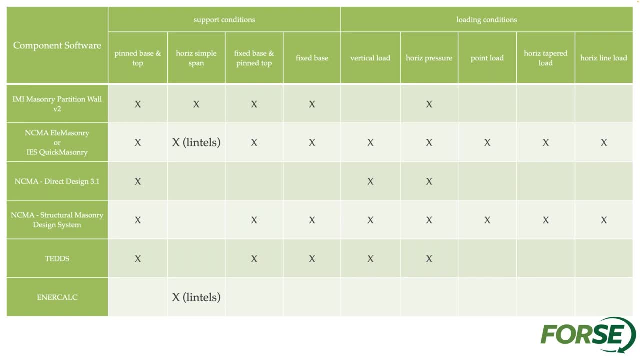 support conditions up and down, or is it something that's going to be mainly going to be turmeric in the fixed space? you could be building something, but not going to be building solid rock or even just a solid rock. you could be building things in the fixed space. so what we're? 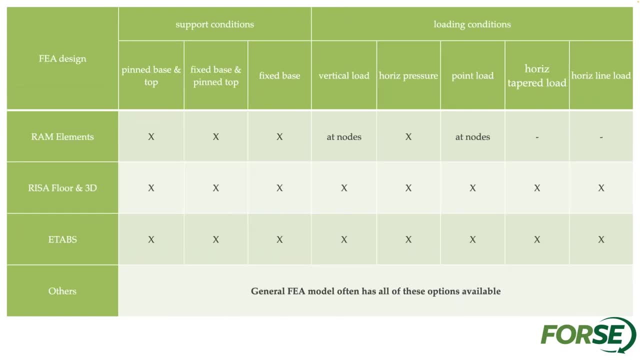 working on is to have a lot of different solutions out there, not just the typical like moving those things back and forth, but also to allow us to create more support conditions that we can use in-house, so we can create a lot of different support conditions for the. 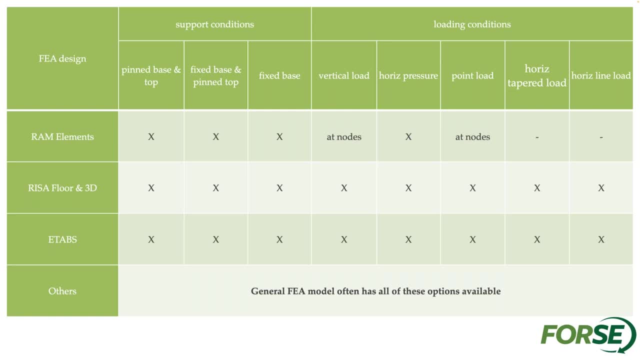 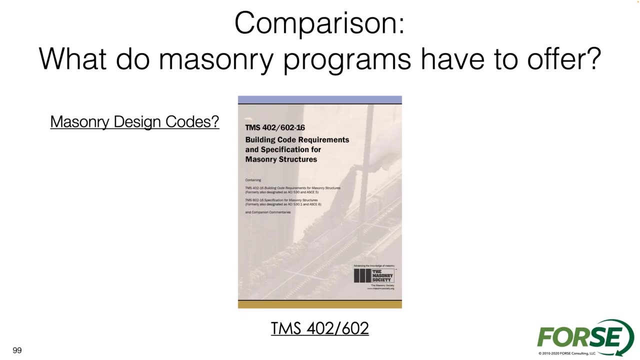 system. so that's where we're going to be looking at our local site. we'll be looking at some of the different support systems as we move forward. it's going to be a lot of different support systems that downfalls of finite element analysis here in a second. Really, when we look at the different 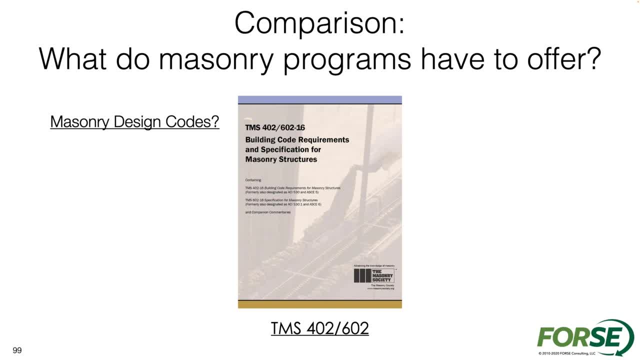 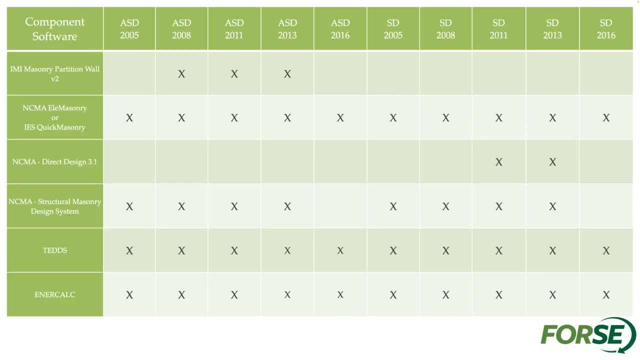 design codes. This morning we talked about from 2011 to 2013 to 2016 to 2022.. Well, if I look at different software programs, the application of codes is really varied quite a bit over time. Component design programs are always going to be better in terms of code implementation. 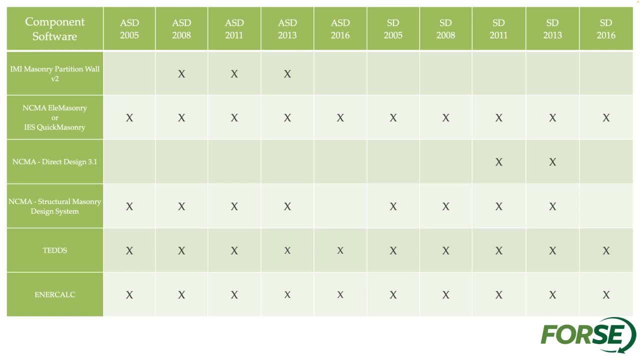 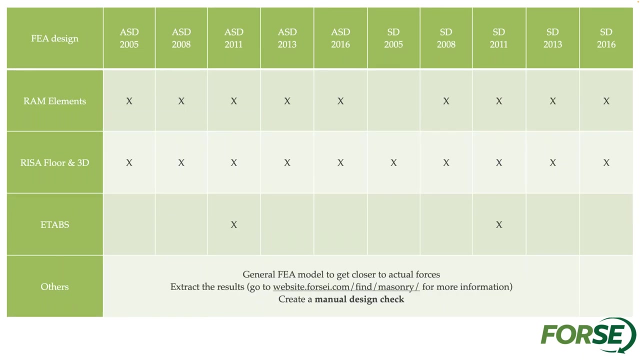 They're going to be the design arm of software. So anytime that we wanted to use a current software using something from NCMA, LMA or something like that is probably going to give you the best code support for design. If you get into the finite element analysis world, it can be a. 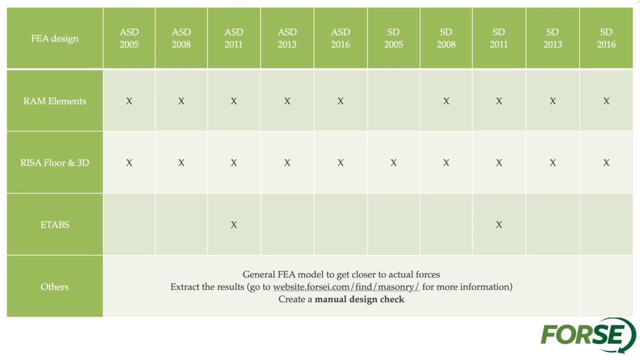 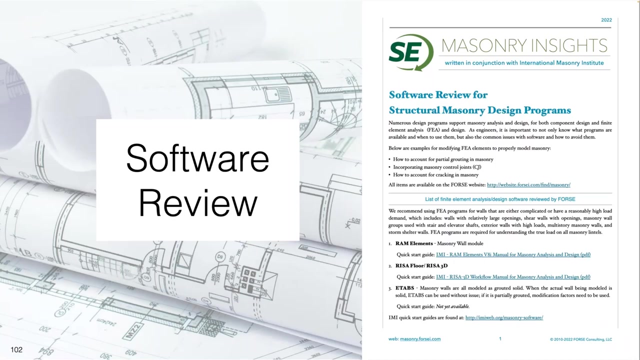 little bit sporadic. It's not necessarily going to be the full options and abilities to be able to do some of the design. It's going to be a lot of different code implementation that we've talked about earlier today. So a lot of what we talked about from the software review. what I try to do is I put 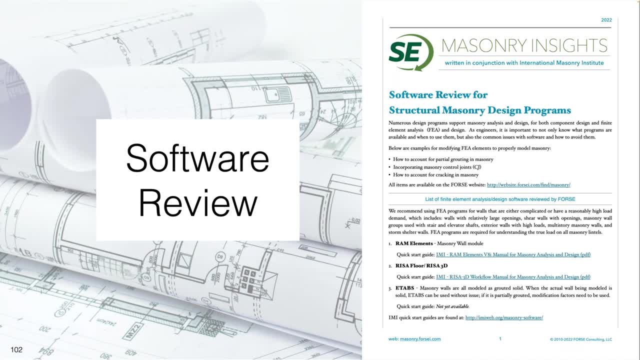 a lot of that stuff into some design guides or some guides that are free and available online both from my website or IMI's website. I have a tool for how to use masonry design within ram elements. I have a quick start guide for using. 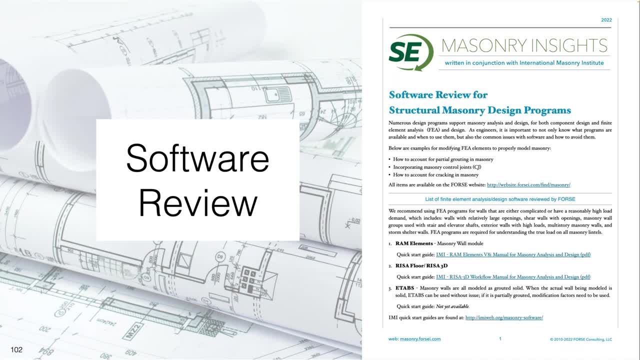 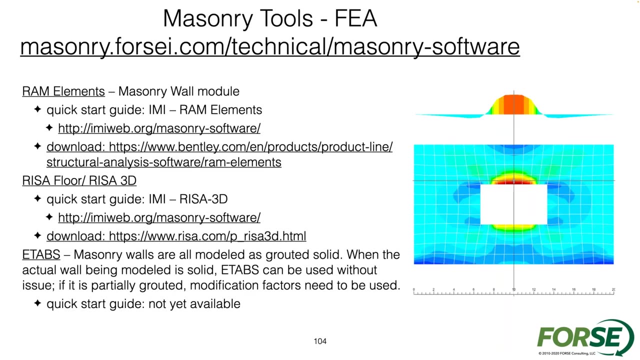 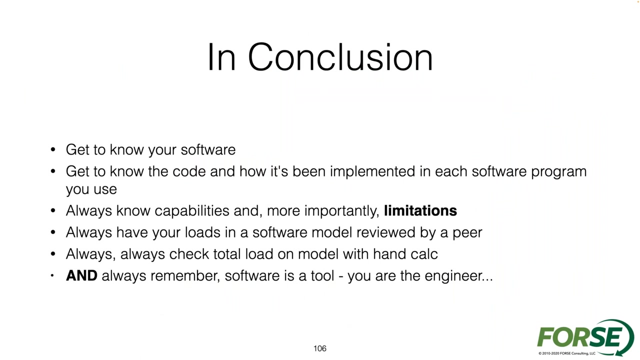 masonry design within visa. We're working on the guide right now. Component design programs. a guide is not really needed. I just kind of point to where they're available so that you can download those anytime that you would need to use that software. So really so kind of, in conclusion, get to know the software, get to know the code. 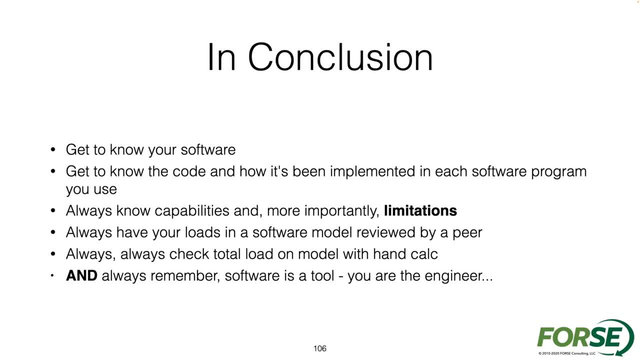 and how it's been implemented into each software program. There are a lot of different capabilities And in limitations that we have to take into consideration and understand. you always have to understand the capabilities But, more importantly than that, limitations, whether it's 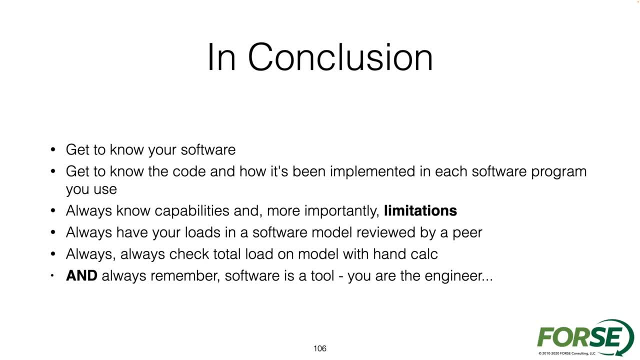 how it supports the code or the different options that you have for masonry design. Always have the loads in your model reviewed by a peer. that applies for any material, but that certainly applies for masonry as well. Check the load in your model with hand. 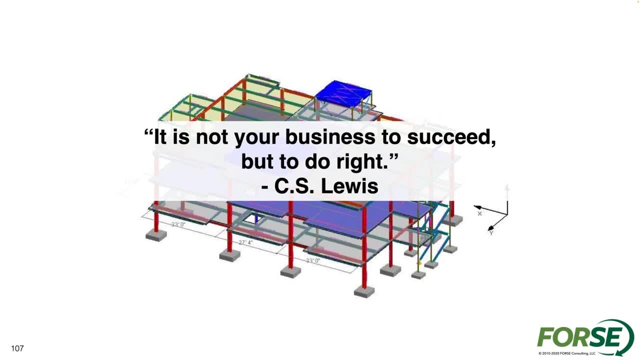 and remember, software is a tool. you're an engineer, So that's. I kind of like to end with a little bit of philosophy. It's not your business to succeed but to do right. I think with masonry we certainly have a lot of different capabilities. We have a lot of different options. Sometimes I think masonry 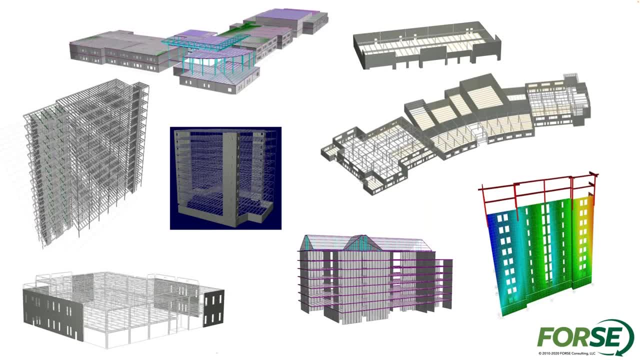 over the years has been boiled down to taking the path of least resistance, trying to just use empirical design methods And hopefully you can see over the course of today- you know when we started with codes this morning- there's a lot of good code development. I actually just got the 2022. 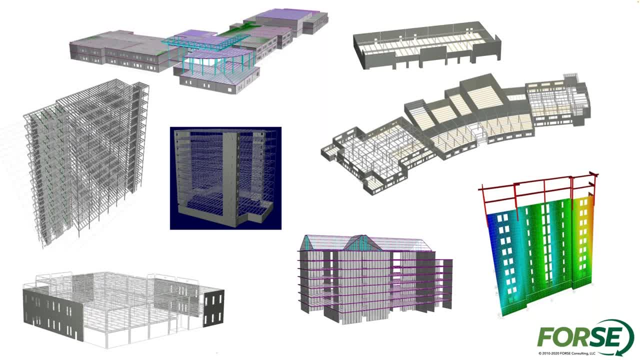 code this morning, So it's sitting on my desk right now. I'm going to be looking through that. There's a lot of different things that are built into the masonry code for moving masonry into the design arena similar to steel and concrete. We have a lot of different. 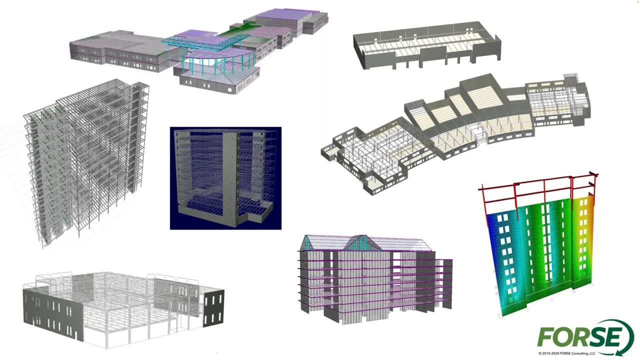 options and capabilities with masonry elements. We have a lot of tools available and that's why I wanted to end the day with software. Using different software programs really does help you model and design masonry structures and pretty complex masonry structures. So, whether or not you have a 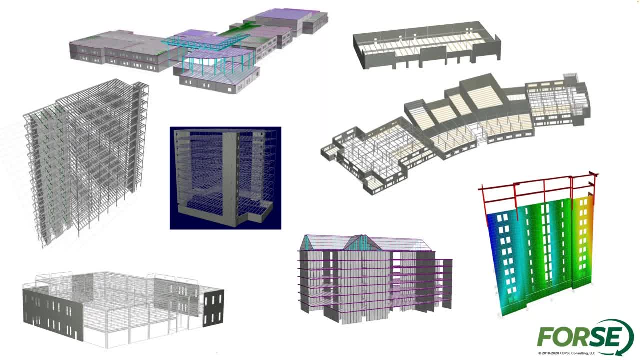 reinforced brick or you have a concrete masonry, you should be able to put in whatever different types of designs or analyses that you need in any one of the software programs. So I try to encourage people to look at masonry, for you know all these different types of building types and 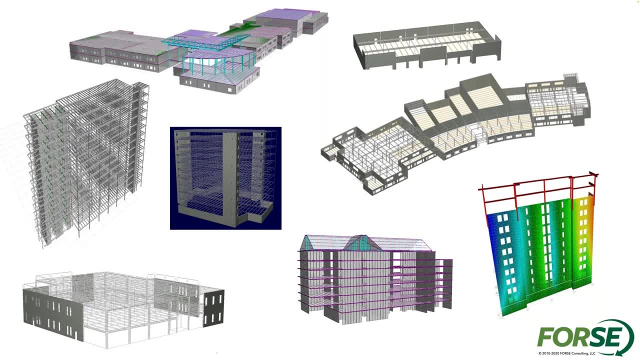 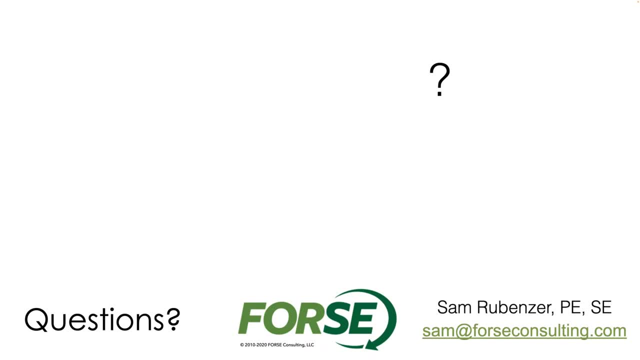 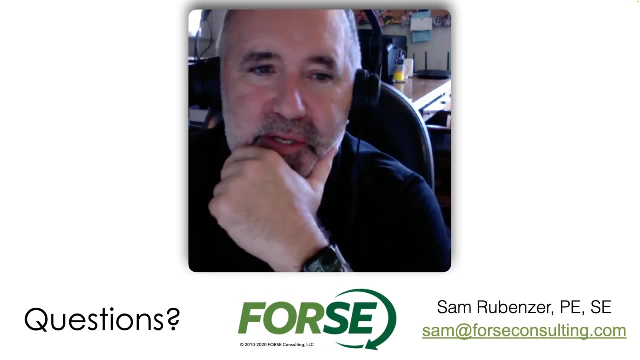 try to stretch their understanding and capabilities with masonry. So that takes us to the end. There's a little picture of me in my office. Hopefully, if you guys have any questions, I'd be glad to answer those at this time And really we can kind of open it up. If it's a software question, we can look at those, Or if you, 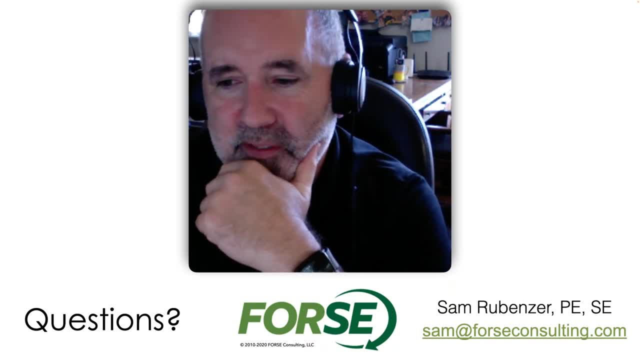 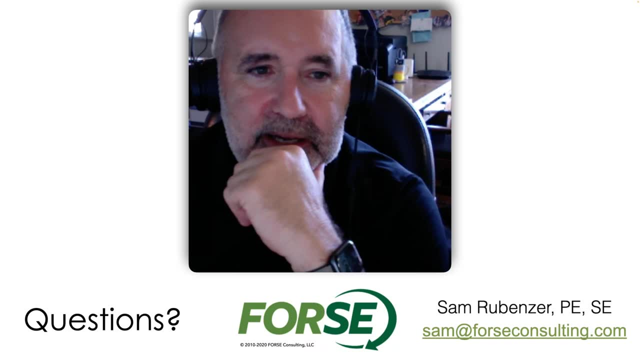 guys have any questions on any of the other sections, I'd be glad to kind of go back and review and look at any one of the sections from today. So thank you so much for joining me today And I'll see you next time. Bye. 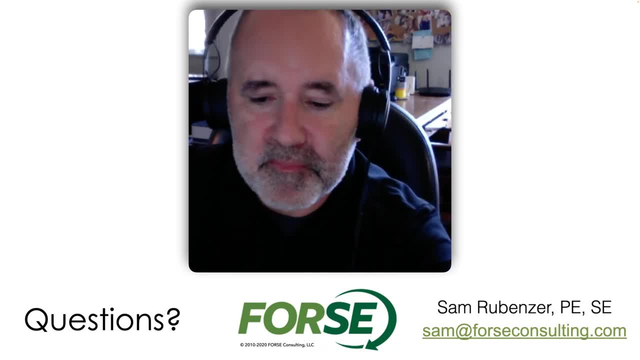 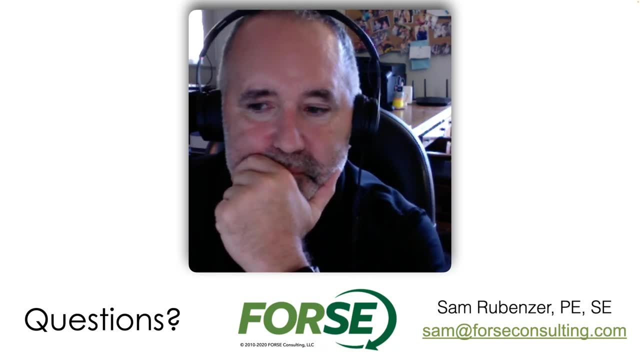 Rick Haverkate. Yeah, definitely. You know we got about 20 minutes here till we're officially supposed to end. So yeah, definitely, If you guys have any questions. we got some time and now would be a great opportunity to do that, So we'll leave. 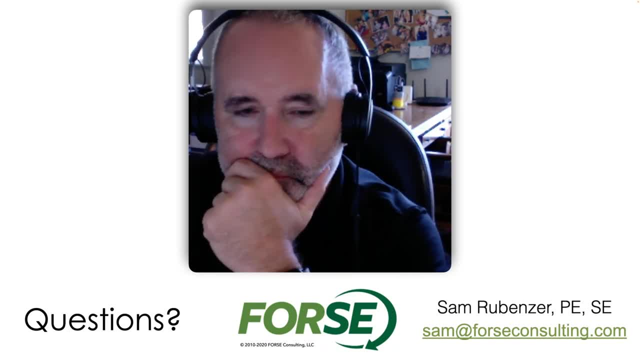 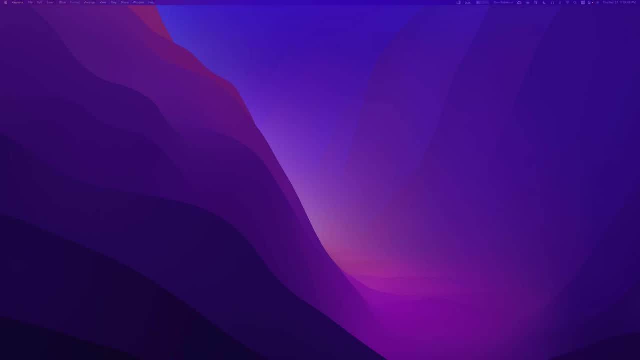 it open here for a little bit. If we don't get anything in, it's not going to hurt to close a little bit early if we have to. But we'll just wait here for a little bit for any questions or What not, and then we'll kind of go from there and and just go from there. So give you guys, you know. 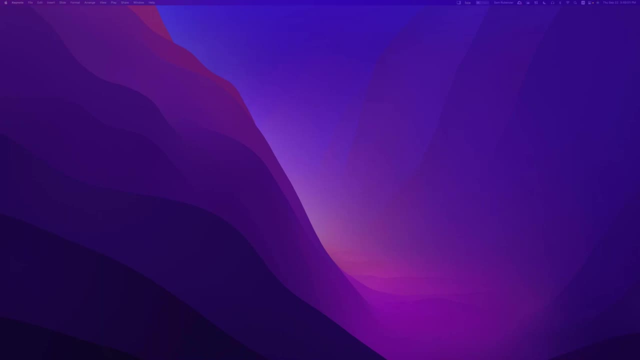 five, some more minutes to enter something, I think, Other thing we like to offer, but we don't really talk about them. You can definitely Send me a question and I can pass it along to Sam if he doesn't mind to afterwards. that's something we do often and I 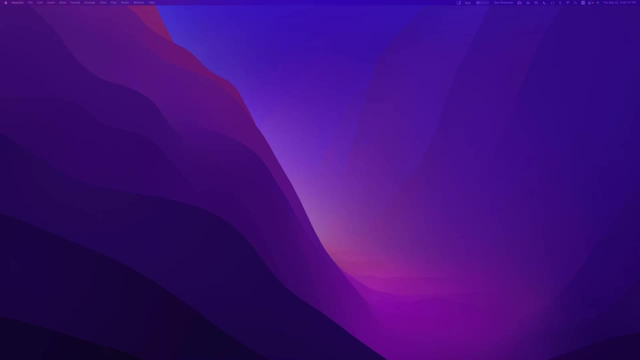 I don't want to put them on the spot, So I didn't ask him beforehand, But usually people don't mind if that takes place. No, that that, yeah, No. I'm glad to answer any of the questions down the road if you guys have anything with mainstream design that you're looking at. 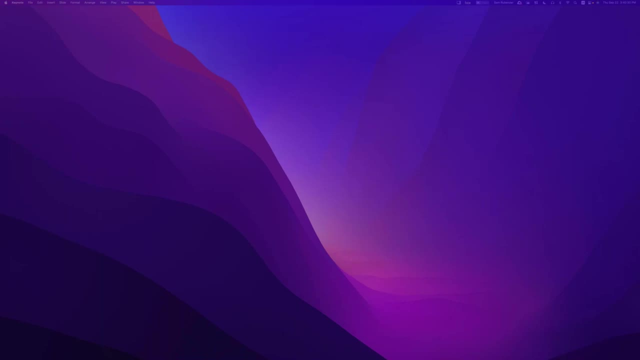 We wanted to look at something. I'd be glad to answer something over email, And I'm not really seeing anything coming in. I have a few things to say, so up, Excellent, There's one. Could you please show a brief design example? That's really good. 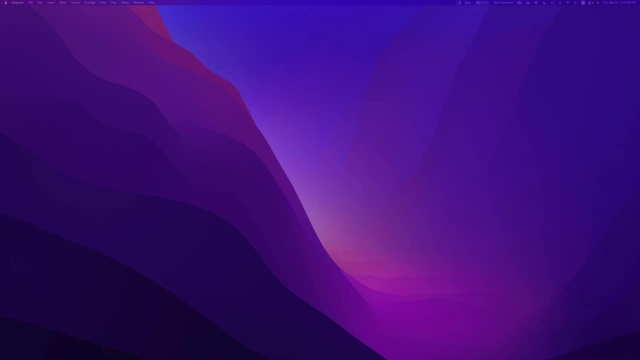 I don't have anything prepared in terms of a design example, So that would be a little bit difficult to do. Trying to think, if I have a presentation that would have some examples in that, I can't think of anything off the top of my head. 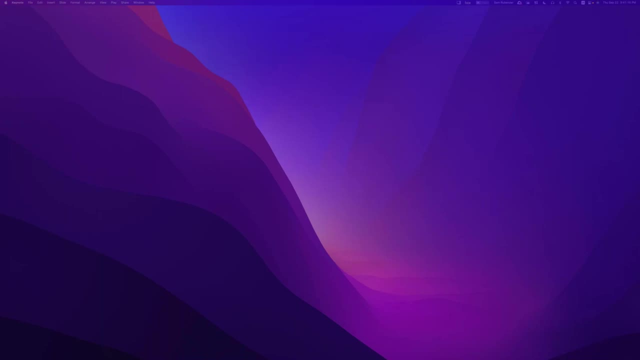 in terms of a design example for masonry, And I'm left in the middle of the session here, And so I'm gonna read the questions for that. but before I do that, I'm gonna take this time to jump in and talk about some of the things. 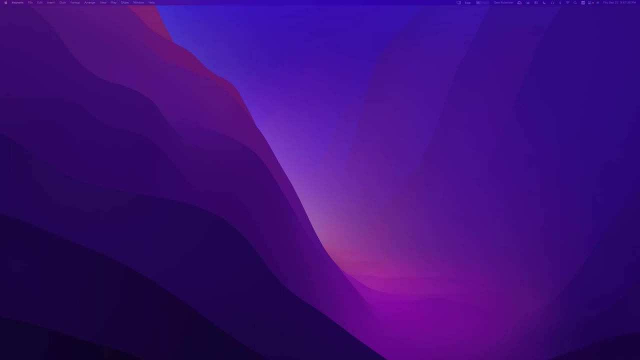 that we talked about. So I'll start and get going. We'll do this right now. All right, thanks, This is a question that came up: What is the meaning of masonry and how does it mean that it can be used in masonry? 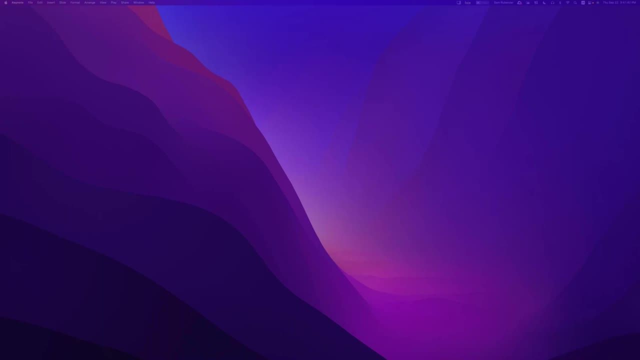 And what do you think the importance of masonry in masonry large scale? I just want to get to that first question. Thanks so much, Thanks, Thanks, Thanks. wrap up, but I do want to thank Sam for all this time and expertise and for 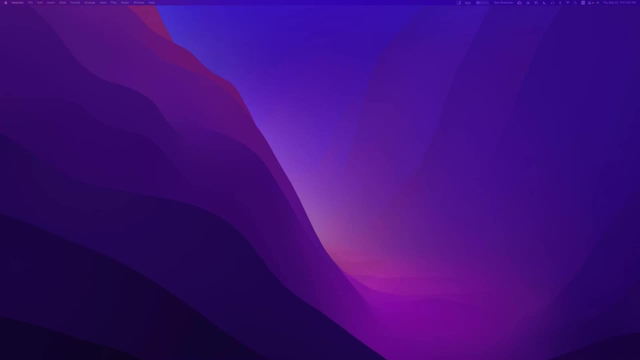 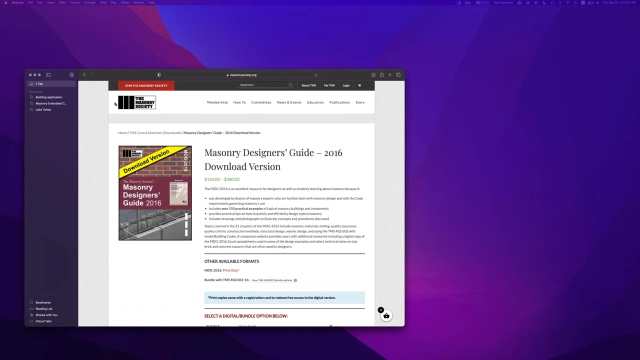 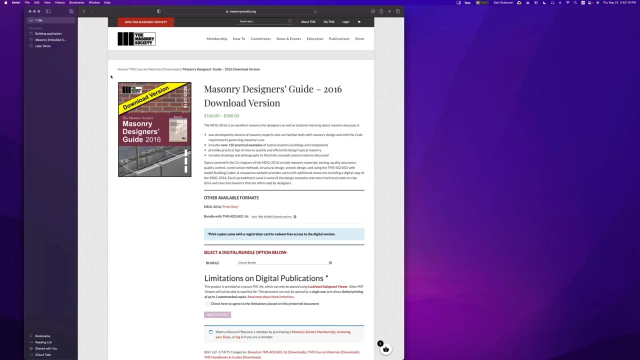 giving an excellent program this afternoon and I want to thank everybody for joining us. to the attendees: remember I'm going to send you that quiz that you need to take here in a little bit and then, once you've successfully passed that, you'll be asked to download the verification of attendance further for: 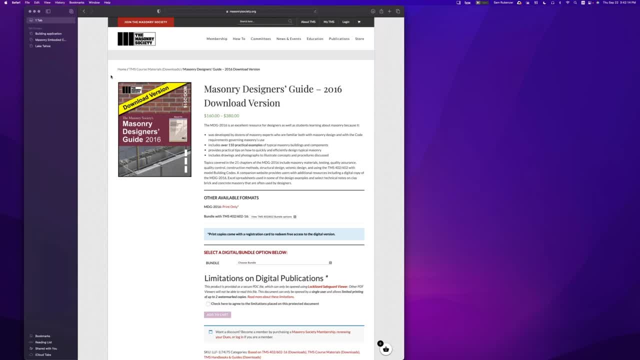 the class and note that you can take that as many times as you need to, and there's also no deadline on when you need to take it. so you know if you are busy right afterwards or something, don't feel rushed to do it, you can do it. 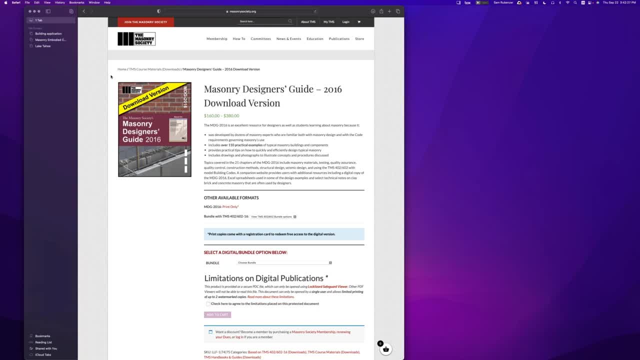 whenever you want. in that same email is going to be a CE request form. if you are a member of one of the groups listed in that form, make sure to fill it out and get it back to Half Moon. if you are not a member of one of those groups listed, 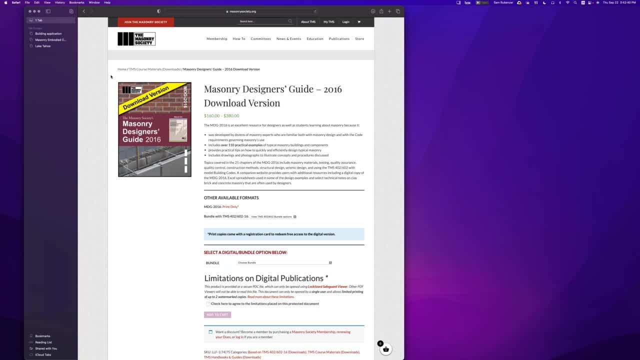 then you do not need to worry about it. if you have any problems in the future, of course you can call our customer service and they'd be glad to help. but I do want to let you know that you can always feel free to email me. the best way to do that is just respond to the quiz email that I'm going to send. 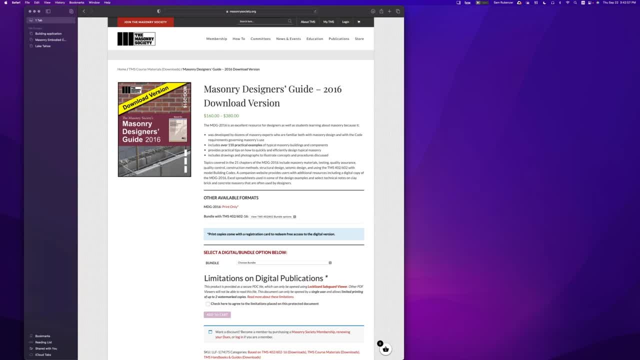 and I get people who ask for certificates or tests or something from literally years after the course. so anytime you need to ask a question, feel free to. I still don't see any questions or anything. so again, I know we're a little early, but I don't, it's not too bad, it's not a big deal. I'm going to go ahead and send that to you. 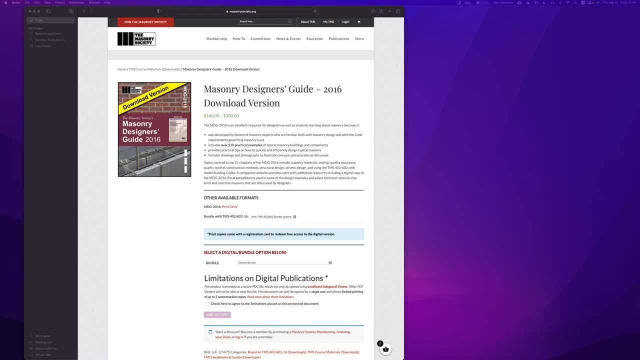 so we'll go ahead and finish up again. thanks, Sam, for everything. it's where we have Half Moons in Eau Claire. it's where we have another person from Eau Claire with us, so that's pretty cool. thanks to everybody for joining us. we're finished.